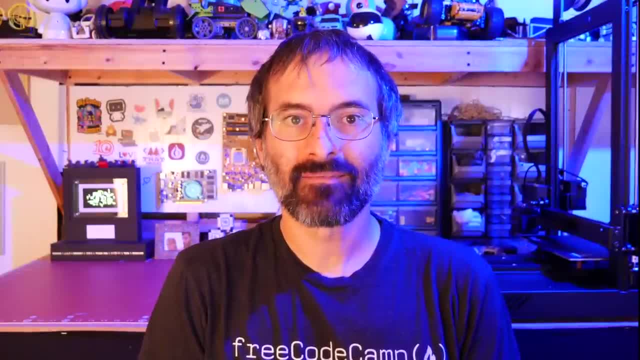 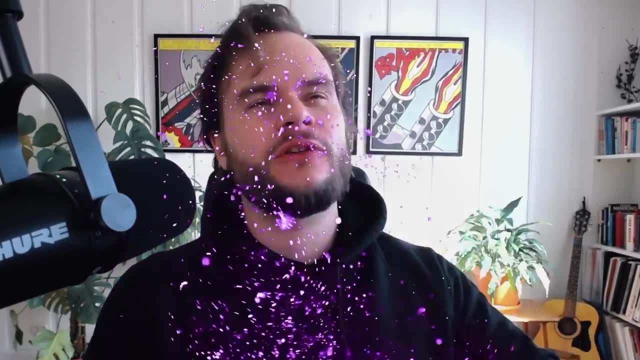 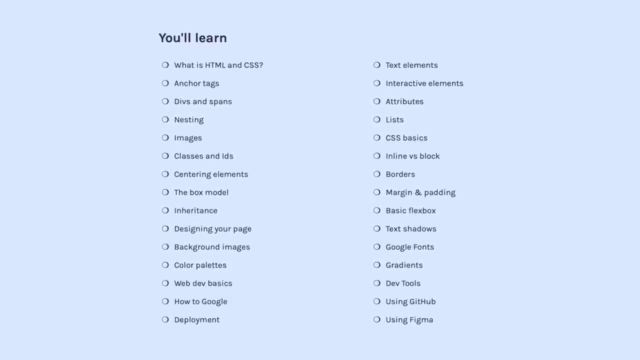 This course makes it easy to learn HTML and CSS. Hi there free cold campers, and welcome to this interactive scrimba course where you are going to learn how to build beautiful looking websites using HTML and CSS. we're going to go from scratch, so there are no prerequisites required. However. 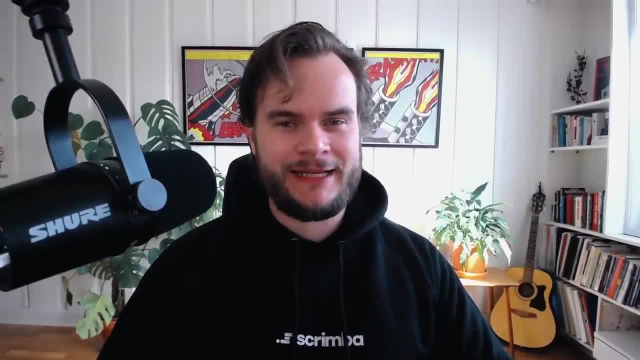 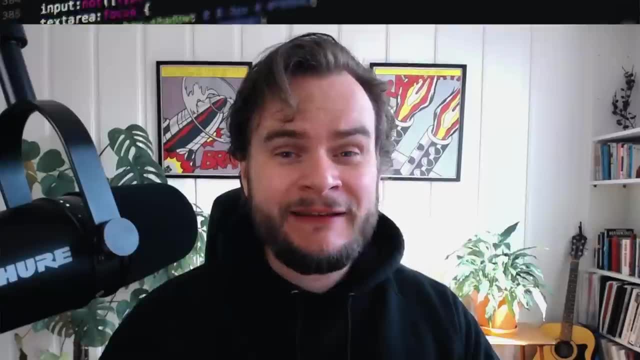 the special thing about this course is that it's fully challenge based, which means that you will need to get your hands on the keyboard again and again as you progress through this course. If you now are a little bit afraid or like setting up your local dev environment, don't worry For that. 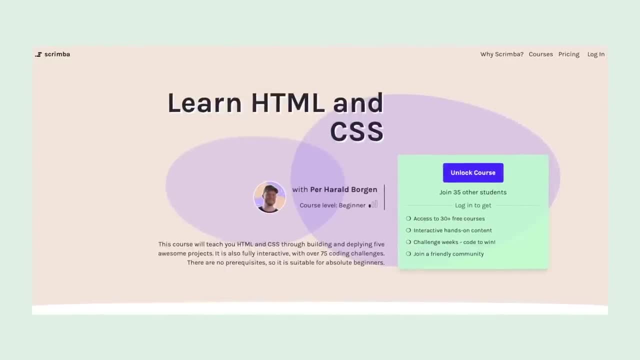 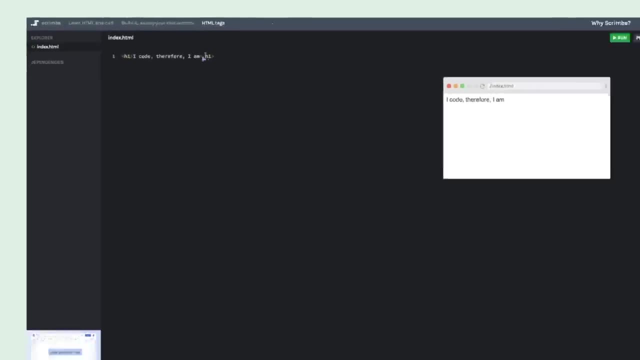 reason we have created an interactive version of this course over on scrimbacom. There you'll be able to solve all of the challenges directly in your browser. So just click on the link below and you'll get to that interactive version. Now, if you prefer to instead solve the challenges locally, 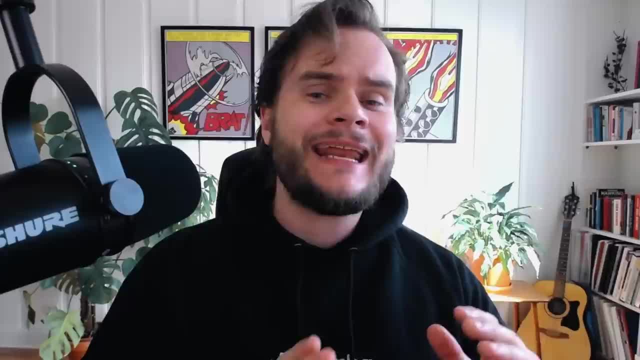 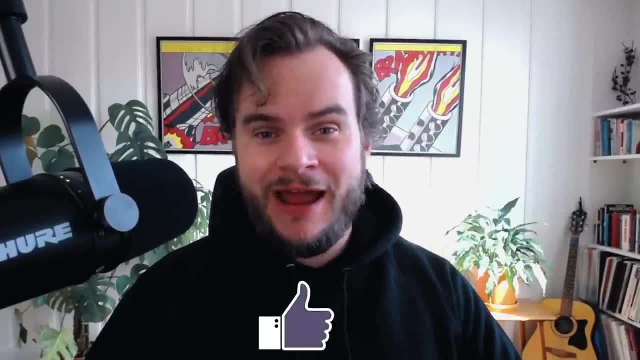 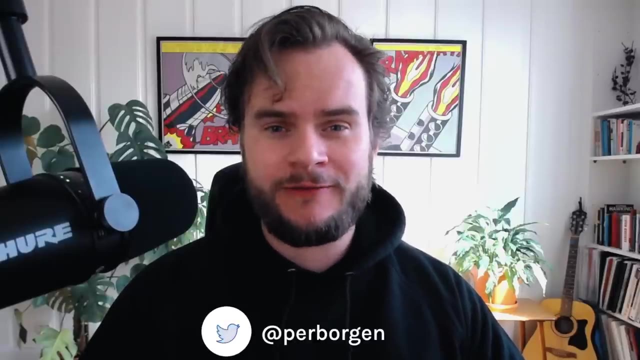 I've created a GitHub repository that you can clone, And there you'll get access to all of the starter files for the challenges. One final thing: if you like this course, please give it a thumbs up here at YouTube. that is highly appreciated, And if you have any feedback for me, just reach out to me at Twitter, at Pear Borgen, With that. 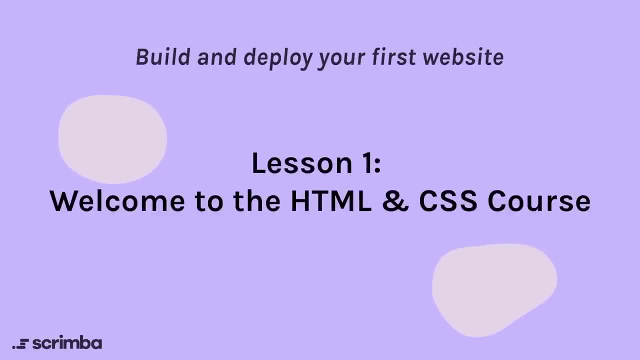 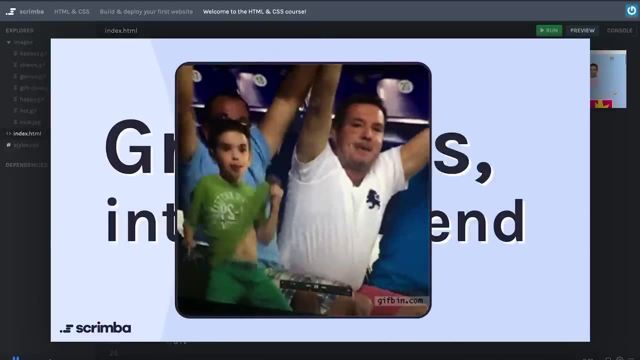 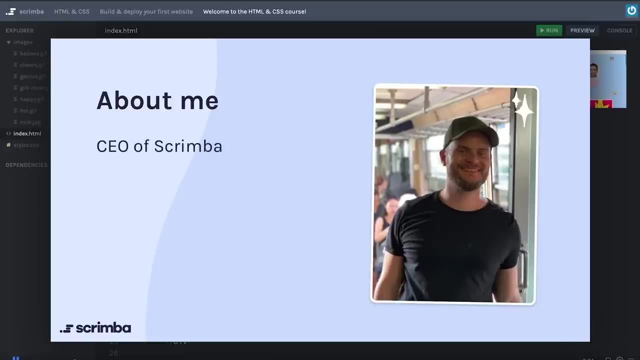 let's get started. Hello there, my dear internet friend, I am so happy that I get the opportunity to teach you two of the most important technologies on the World Wide Web: HTML and CSS. And who am I? My name is pear, I'm the CEO of scrim book And I'm also a front end developer and coding teacher. and 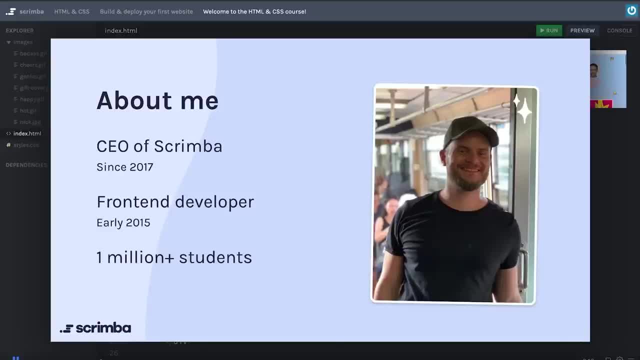 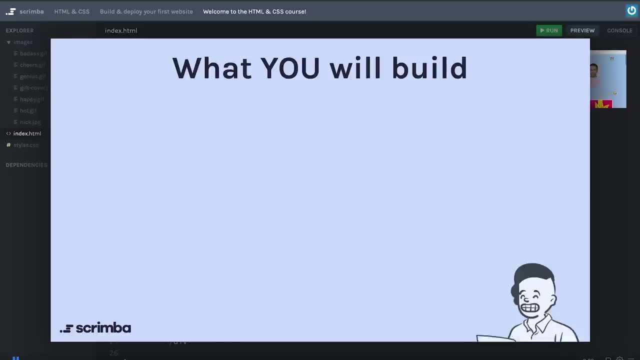 over a million students have gone through my tutorials. When I'm not coding, I enjoy posing in front of fast cars. But enough about me. I'm going to show you how to do that. Let's get started. Let's talk about what you are going to build with your own two hands throughout this course. 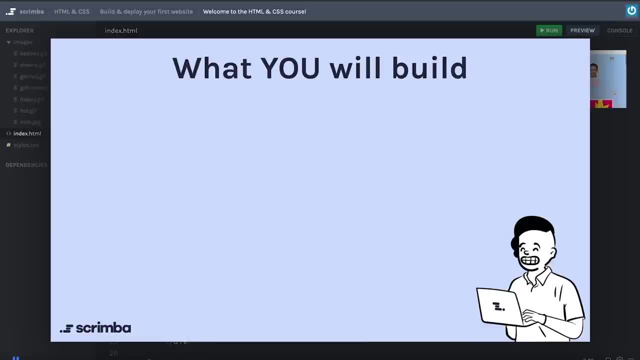 The first project you'll build is the world's most popular website, the googlecom homepage. you're also going to build a space exploration landing page, a digital business card and even a birthday site, which we are going to deploy to the web. 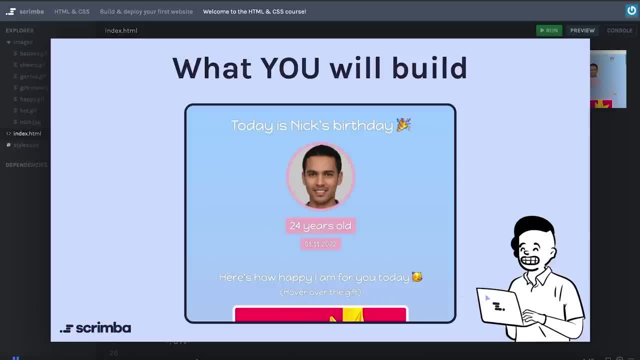 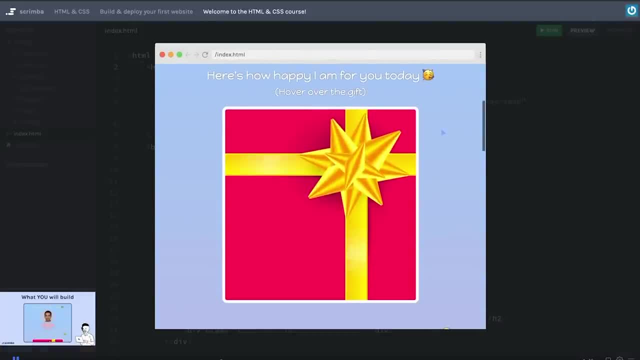 so that you can send it off to your best friend on their birthday to make them feel special. Because, check it out, It has these virtual birthday presents that reveal themselves when you hover over them. So this gift says: here's how happy I am for you today And when your friend 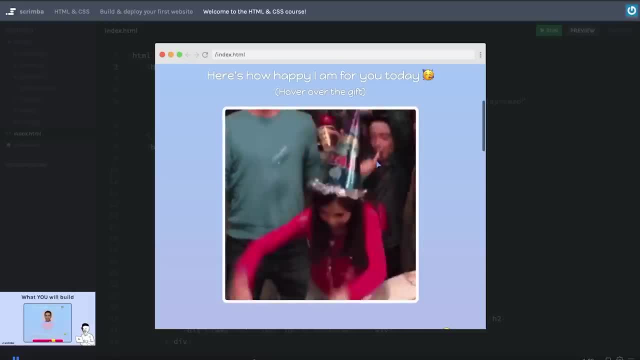 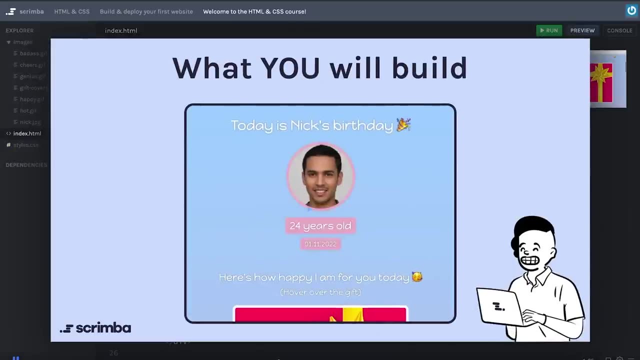 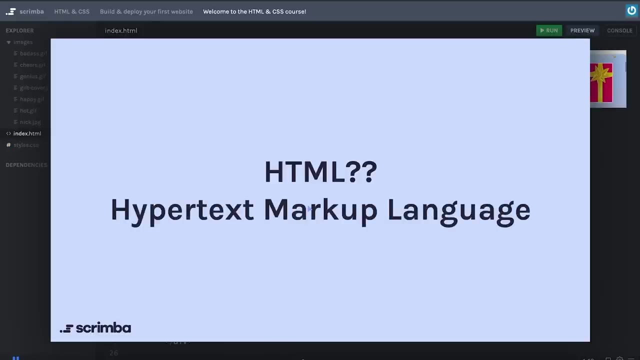 hovers over it, boom. they will feel your love flowing to them through the magical tubes of the internet. And we are going to build all this in HTML and CSS. So now you're probably wondering: well, what is HTML? It is short for hypertext markup language. Oh my god, I'm getting tired. 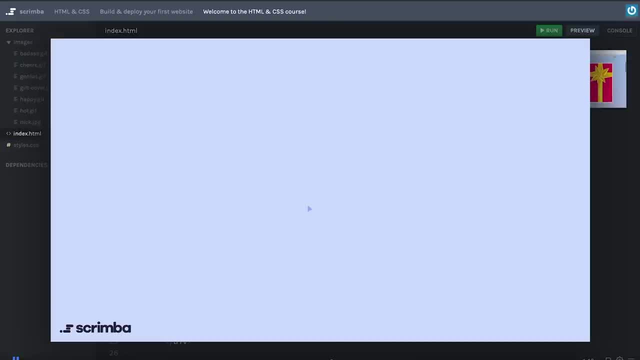 of all this theory. Let's instead say that you're going to build a car. Well then you'd start with probably gathering the contents of the car, So like tires, doors, steering wheel, mirrors and stuff like that, And that is kind of the HTML of your car When you stitch it together. 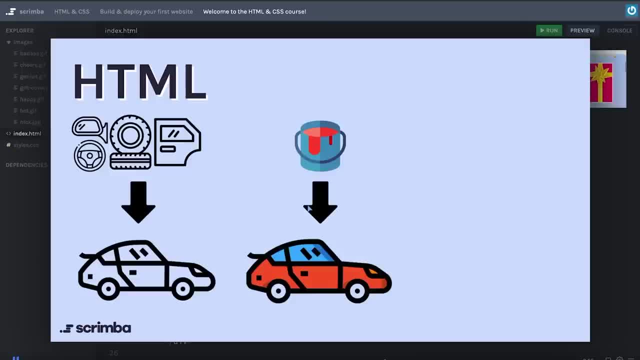 you at least have the shell of a car. The next step is probably to paint the car so that it looks good, And that's the CSS. And finally, if you want your car to drive, you got to give it an engine, And that is kind of the JavaScript of your car, or very often referred to as J. 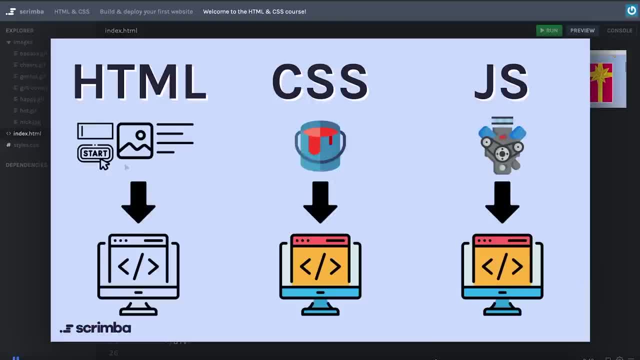 s Now in a World Wide Web context. the HTML is then the content of the website, that is, buttons, images, text and so forth. The CSS is the styling And the JavaScript is what allows your website to solve problems, so that users, for example, can check off tasks, communicate with databases. 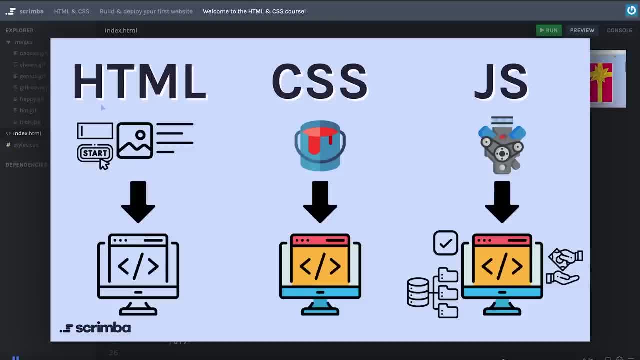 you can also handle payments and so forth. Now we're only going to focus on HTML and CSS in this course, And then you can learn JavaScript and another course I've created here on scrimba as well. But knowing HTML is already hugely valuable in today's job market, And it is also the most 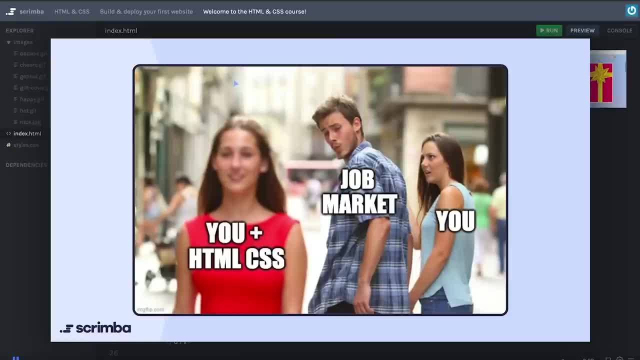 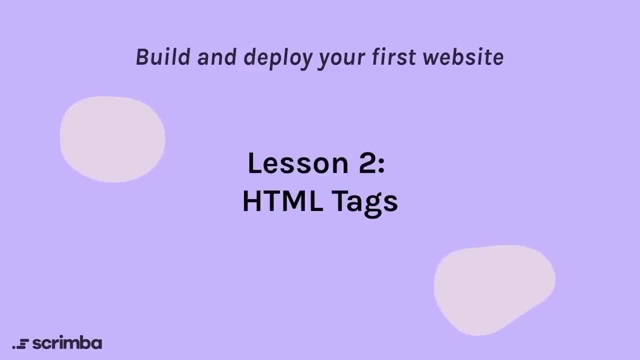 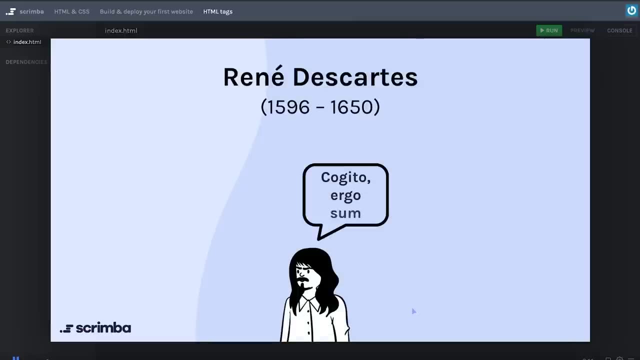 natural first step as you embark on a journey into the world of web development. So I hope you are ready for this. Let's get started. The French philosopher Rene Descartes once said three clever words: Gito ergo sum, which translates in English to I code. therefore, I am. 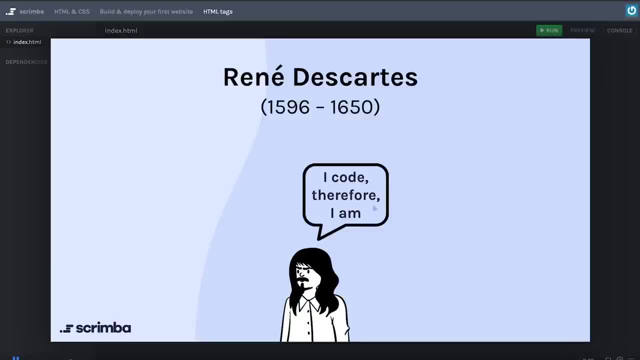 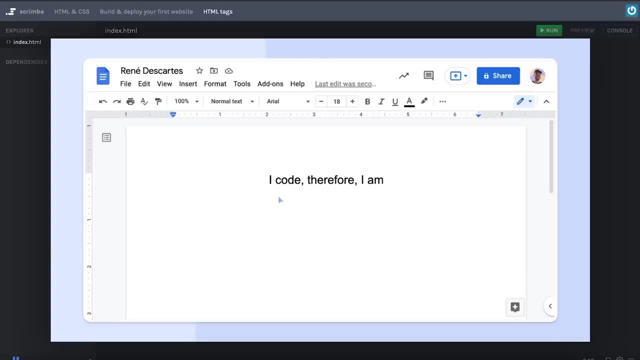 So let us prove to ourselves that we actually do exist by coding this out in HTML, And the way we do that is actually not too different from how you would write this out in a regular text editor, As there you would simply write out the sentence, And then, if you wanted a bit more prominent, you'd probably 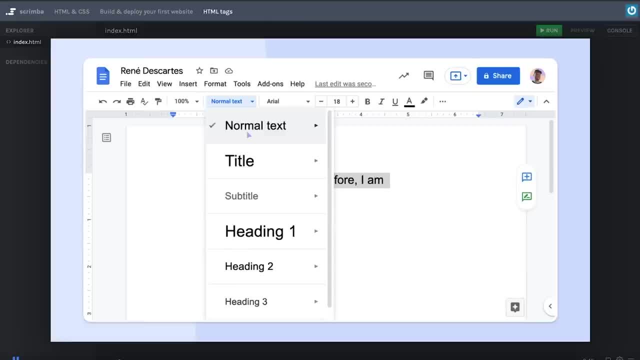 highlight it and then click on normal text here and choose another contents type for your text. You can see heading one, heading two, heading three. let's hover over heading one and then click on it And there you can see that the text became. 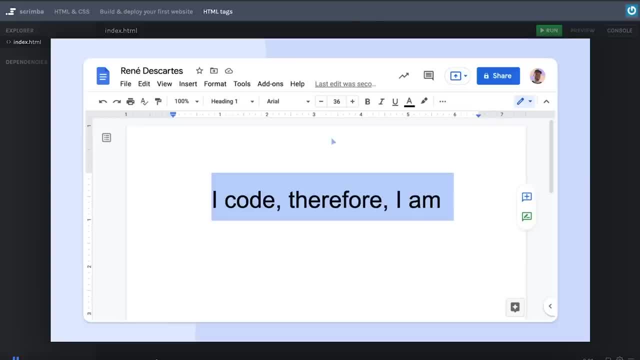 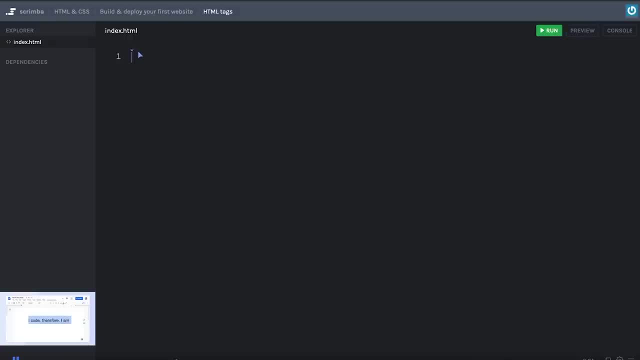 a lot more prominent. it became a heading one. Now, if we want to do this in HTML, we'd simply create an HTML file, which you can see here. it's called index dot html, As that is a common name to give your HTML files, And here I would write: appears for iam. Now, if we open up a browser, 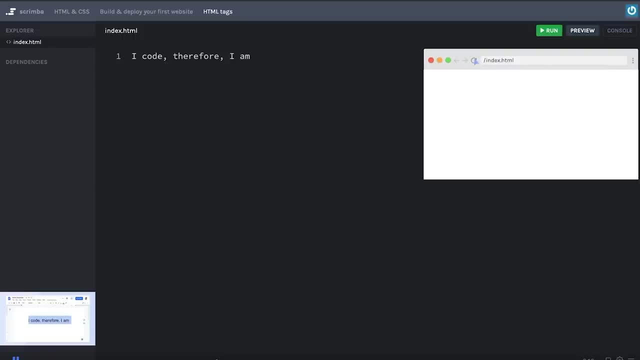 and pointed to this browser, to our HTML file, and then run it. then we can see that the text indeed appears in the browser. However, it's impassive, not So. now we define it with a 14 sentence grid, which we would say, which will give this heading one. And here, what you see here is a heading one. 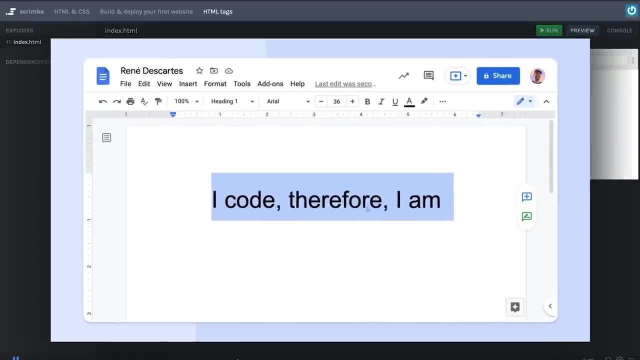 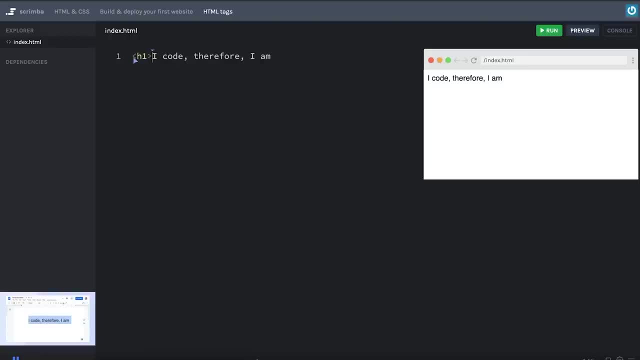 However, it's pretty small, So if we wanted to turn it into a heading one instead, what we do is wrap the text in HTML tags, So before the text we'll do this, two angle brackets with the text age, one inside of them. that's short for heading one, And then at the very end of the text, 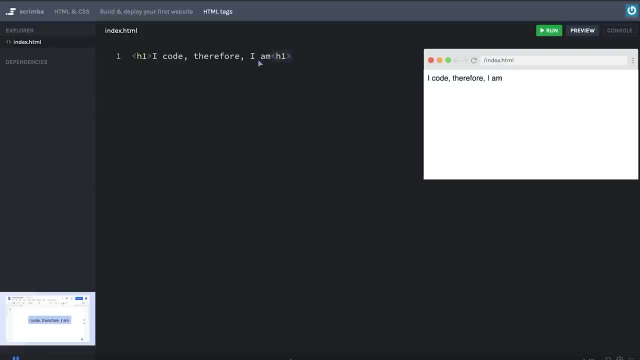 I would do the same age one, But since this is a closing tag and not an opening tag, I would also have to give it a slash before the text. And now, if I rerun the code, there you go. we have made our text a lot more prominent. Now I think our websites should give proper. 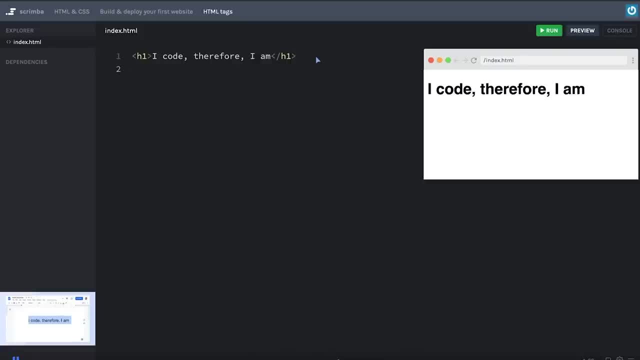 credit here. So let's write Rene Descartes underneath the age one, Like that. if we now rerun the code, you can see that the text is just normal. it's not an age one. that's because it is only the text which is within the opening age one and closing age one that 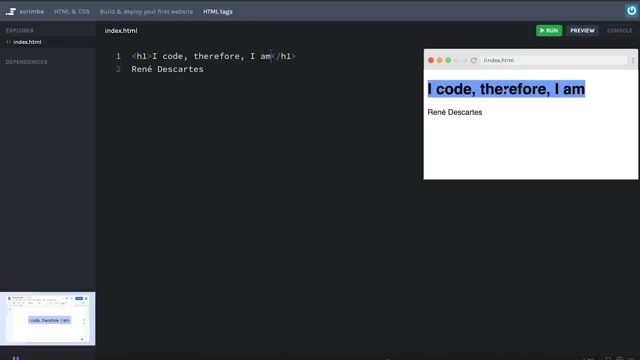 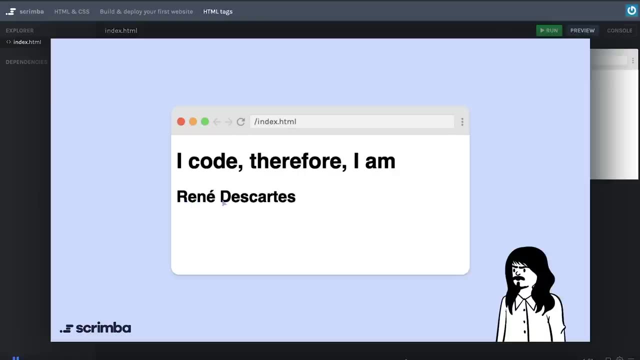 gets formatted as a proper heading in the browser. In my view, this line right here should be a bit bigger. I wanted to instead look something like this, where the name is pretty thick and big, but not as big as the heading one. And that brings me to your first. 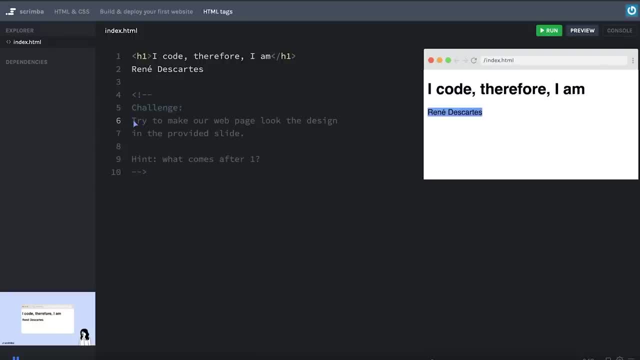 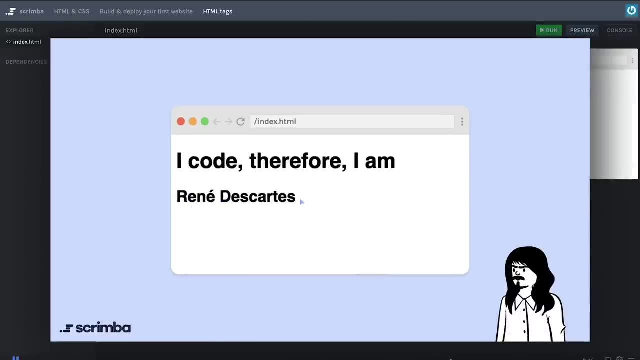 challenge, I'm going to paste it in here. So what you are going to do is try to make our web page look like the design in the provided slide, And if you're struggling to think of what kind of HTML tag, you'll have to wrap this name in. 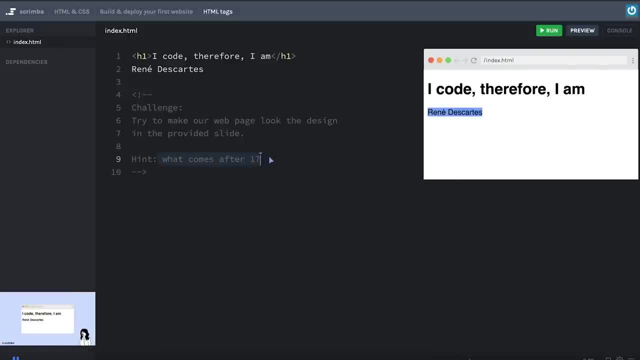 Well, I've got a little hint for you: what comes after one? So pause this scrim, jump into the code and try to solve this challenge right now, And then, when you return back to me, I will, of course, show you the solution as well. Good luck. 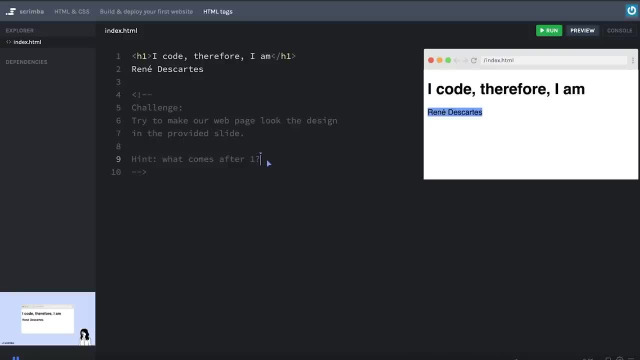 Okay, hopefully that went well. we'd solve this as by, instead of using the h1,, using its smaller sibling, the age two. like that, it has the exact same so called syntax as the h1,: instead of a one, use a two. If we now run this, there you go. 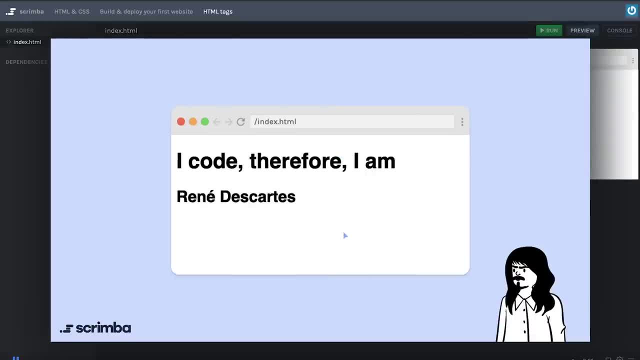 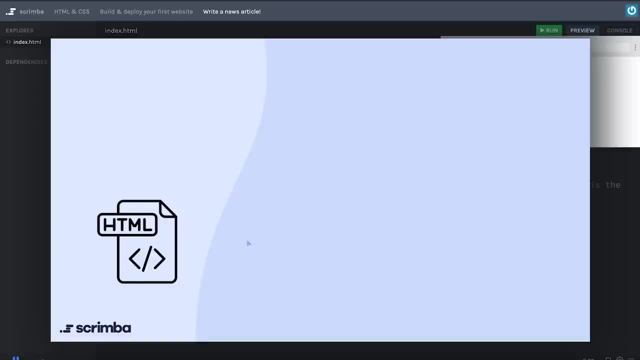 we have achieved the design we wanted. So great job. Let's move on. Before we move on to the next challenge, there's one thing I want to make sure that you are aware of, And that is that if you have an HTML file locally on your computer and you have a browser, 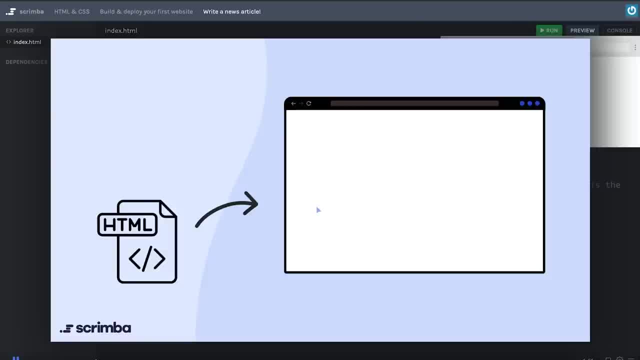 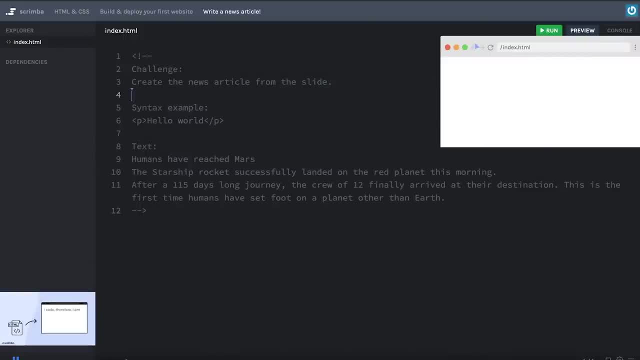 what you can do is simply drag and drop that file into the browser, and then it'll be rendered. So that is actually more or less the same thing that's happening here on scrim bar, Though here we have a mini browser and the 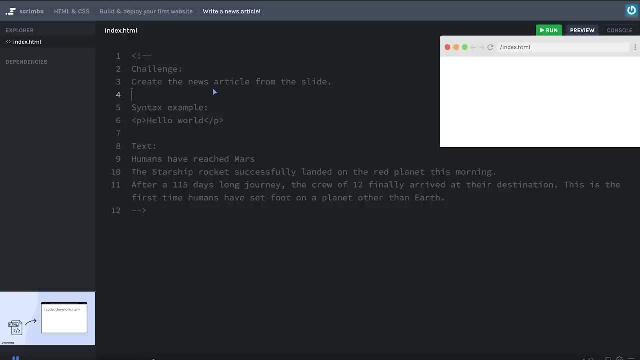 text editor inside of, well, your browser, because scrim by itself is browser based, so a little bit meta, but it's essentially the same thing. Okay, now it's time for you to get some more muscle memory on how to write HTML tags and. 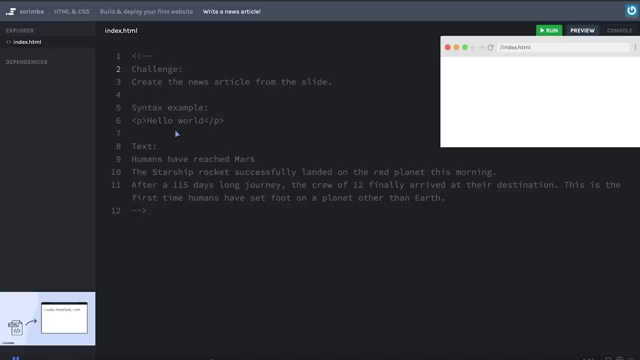 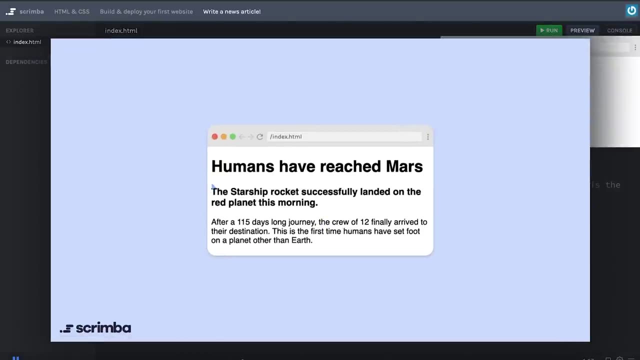 also get to know two new tags, because I want you to create a news article And more specifically, this news article right here, which has a title that says humans have reached Mars. it has a subheading right here and also some regular text, And the HTML tags are h1 for. 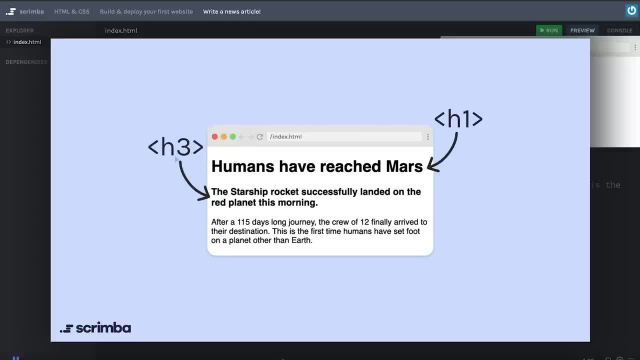 the title h3.. For this one you haven't used an h3 for, but I think you know how to do it. And then there's finally a P tag for the text at the bottom. P is short for paragraph, And I have provided a little syntax example for you here. However, if you've understood the 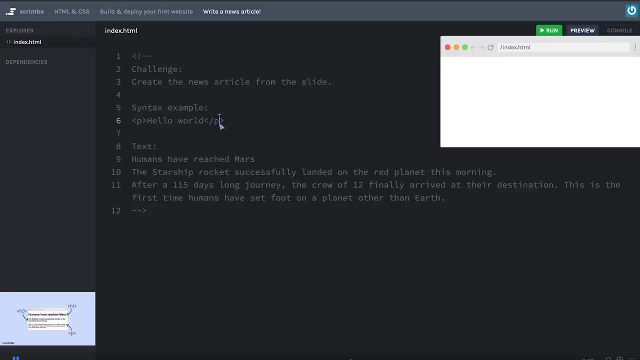 logic of how to write these tags by now. it shouldn't come as a surprise how you're going to do that. Okay, here is also the text, so that you don't have to write all of that out, you can just copy paste it instead. So now, starting here, in line 13,, write the: 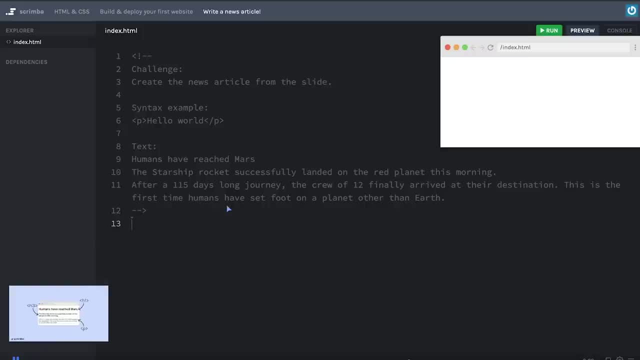 HTML we need in order to create this news article. Okay, hopefully that went well. Let's start with the h1,. I'm going to create the open and closing tag and then paste in the text like that, running the code. Yes, it works. 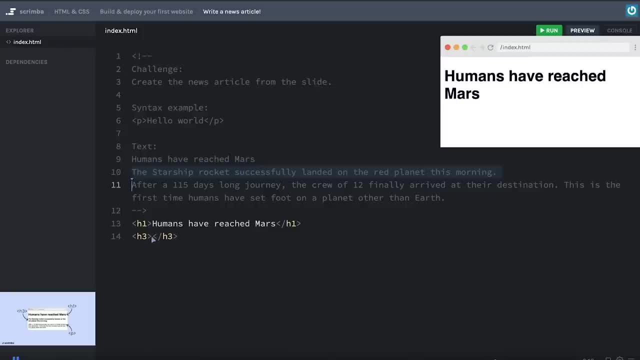 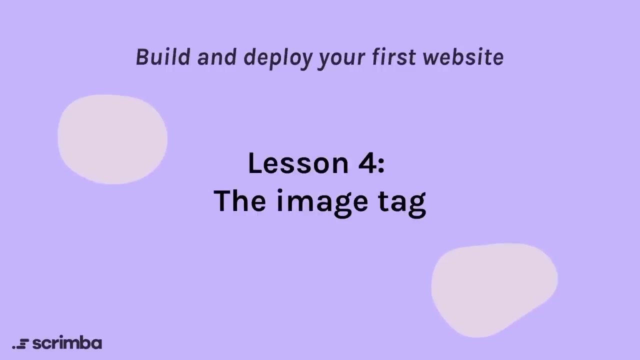 Moving on to the h3.. copying the text, then rerunning the browser, And there we go. Finally, there is the paragraph Like this: rerunning the code, And there we go. we have achieved this exact layout. Great job, Let's move on Now. you're going to learn about images, because 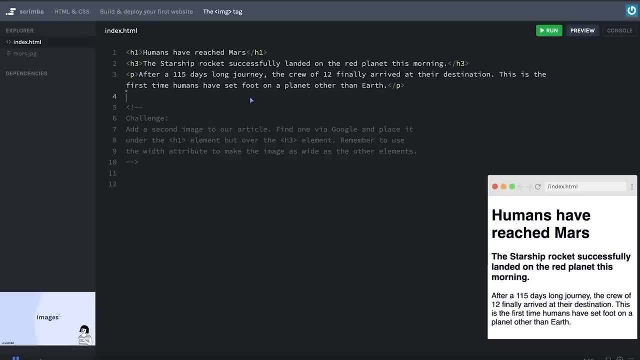 I really think Our Mars article needs an image. The way to do that is by using the IMG tag, So we start with our angle brackets and then write simply IMG inside of those, And what's unique about this tag is that you don't need a closing tag, So there is no closing IMG as there. 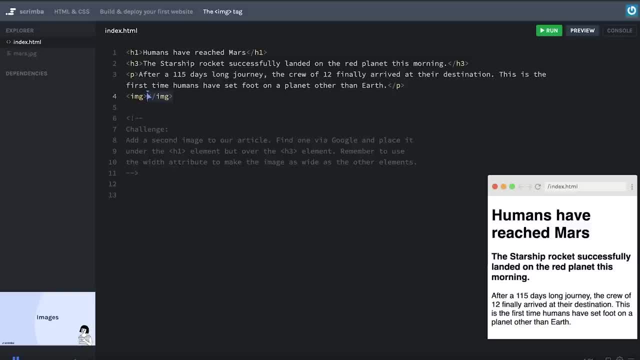 is a closing h1 or closing paragraph. This is simply not needed, So it's often called a self closing tag, And some people use the slash at the end of the opening tag like this just to signify that it is closing itself. However, it's not really needed, So 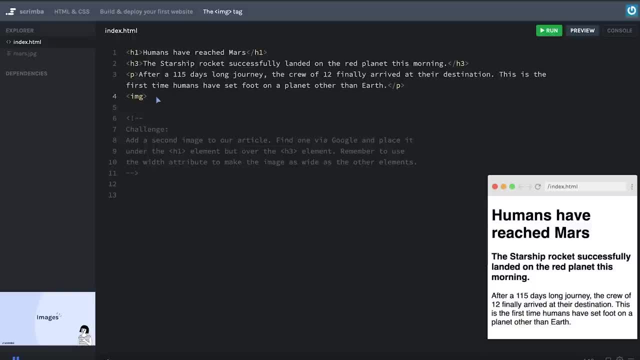 we can skip it, And I think, in general, that less code is better code, So I am just going to skip it. However, if you prefer to have it like this, that's totally fine as well. Okay, enough syntax. How do we get this image to work? Because right now, if we rerender 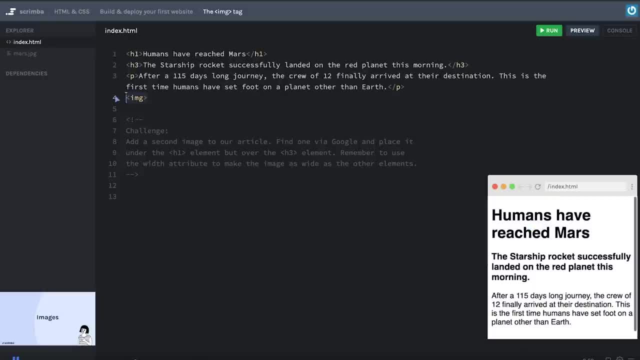 this page. nothing has happened, And that is because we haven't told the image tag which image we want to render, And the way to do that is by writing s r c, which is short for source. then we write equals, then two quotes, because inside of these two quotes 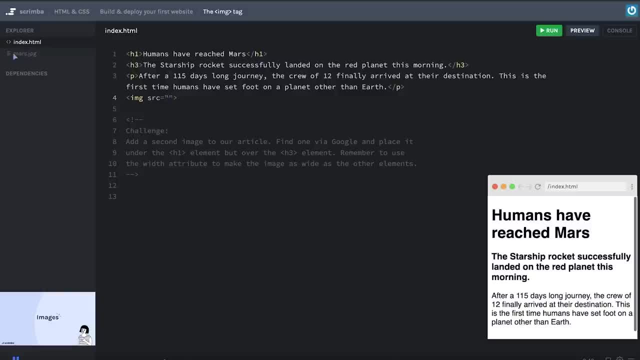 we're going to specify the image we want to render, And here on the left hand side, you can see I have Mars dot jpg. it is in the same directory as our index dot html file, meaning I can simply do Mars dot jpg, then run the code And there we go. we have our 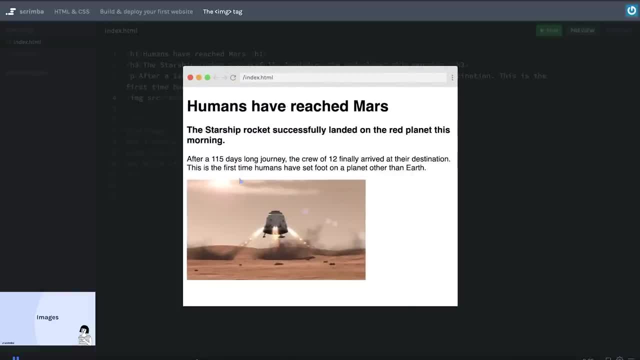 image that is super cool. However, you can see that this image behaves a little bit differently from our paragraph, for example, because, whereas the paragraph take up the entire with the image just take up whatever with it needs, leaving us with white space on the right hand. 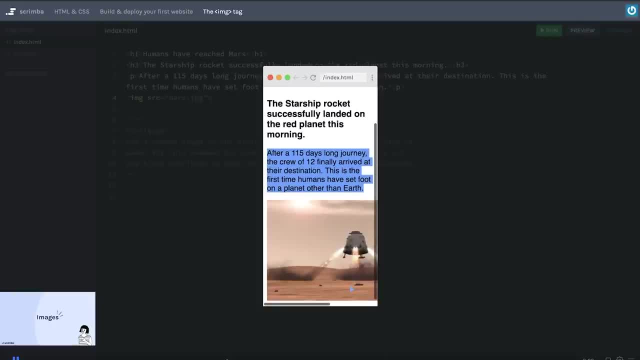 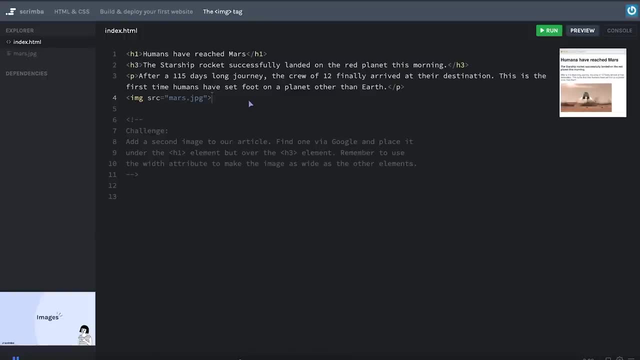 side if the browser is too wide or cutting off the image, if the browser is too narrow, and I actually want this image to behave like our other paragraphs, So I'm going to show you a little hack to do that, Because normally you'd use CSS for doing this, But there is. 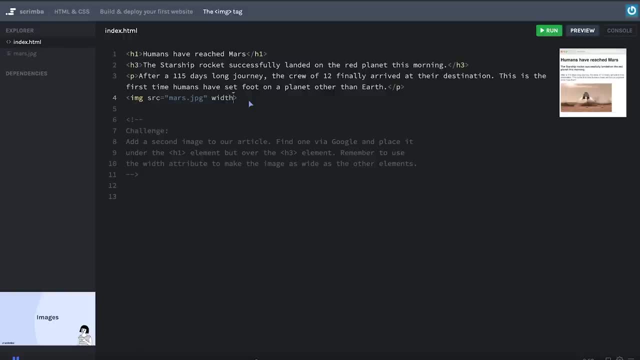 a little trick we can use by simply utilizing the width attribute. that is an attribute, just like source is an attribute, And it uses the same syntax. we'll do with equals and then two quotes, And then, inside of the quotes, we: 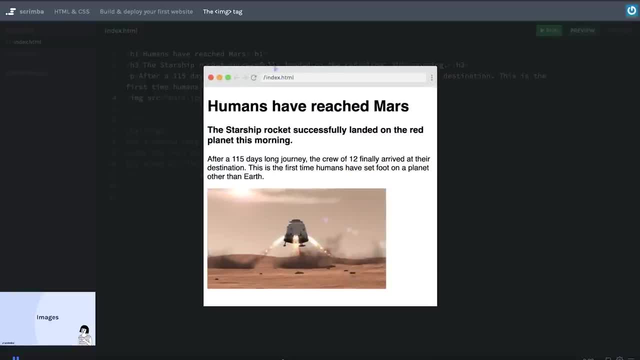 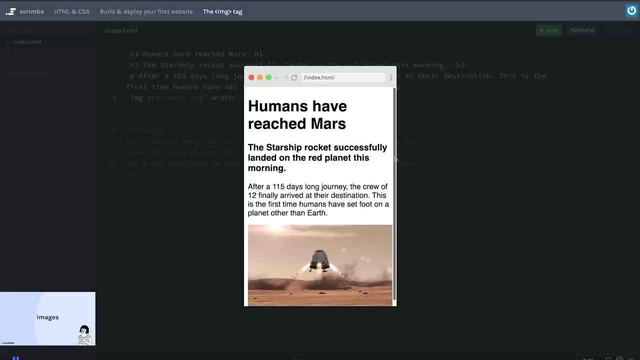 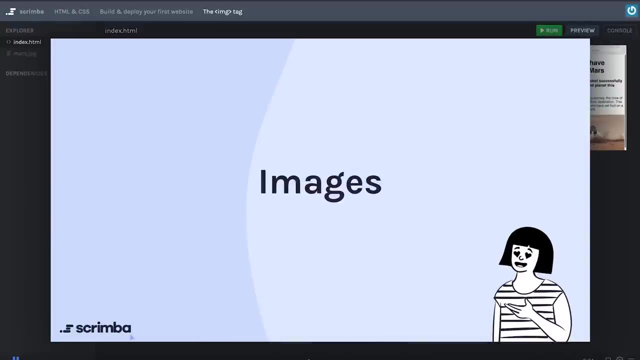 can write, for example, 100%. We now rerun this. you can see, yes, our image is now scaling, with the size of our browser looking super neat. Now, as I said, this is a hack, So if you show this around to people, you might get this annoying guy saying: Well, actually. 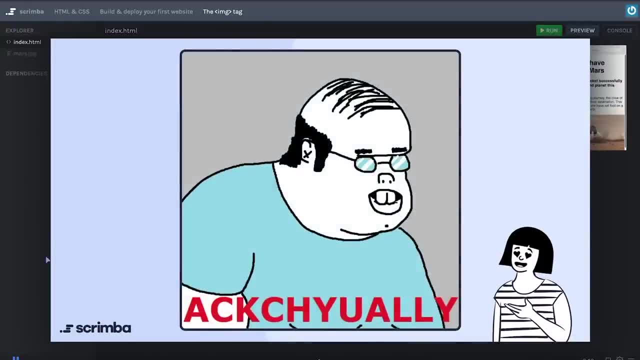 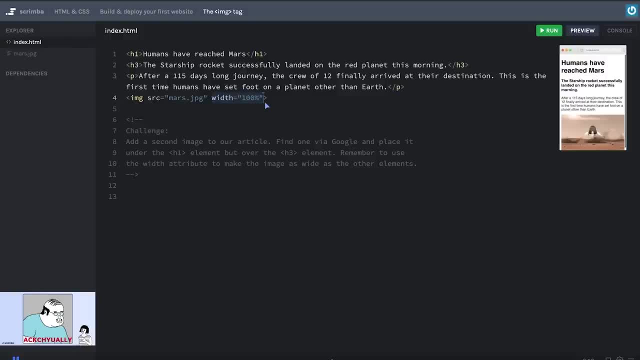 that's not valid HTML according to the specification. But you know what? let's not care about that At this point. you should not give a darn about specifications, validity and aka correct HTML. you should instead look at yourself like a hacker who grabs whatever tool you 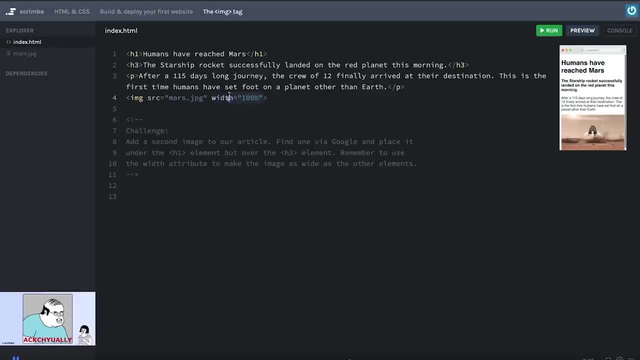 need in order to get the job done. So now we're going to use this, even though we know it's a hack, because later down the line you're going to learn the proper way of doing this using CSS, the language we use for styling websites. 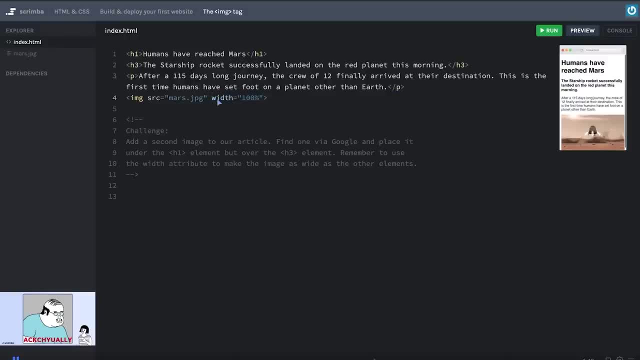 With that out of the way, I want to show you one more thing before I give you a challenge, Because one thing that's super cool is that you can actually borrow images from wherever you want online. So if you find an image you like, you can borrow it and use it in your 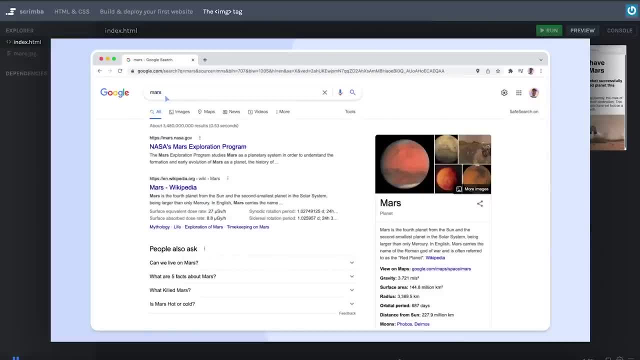 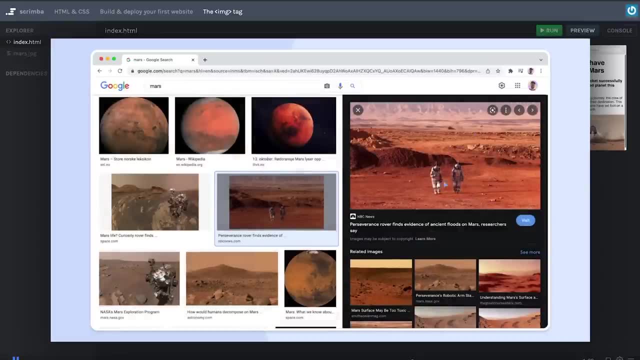 project. Let me show you how. So if we Google Mars, for example, and click on the images tab, and then click on whatever image we think is cool, for example this one right here, And then in this image view on the right hand side here you can right click and choose, 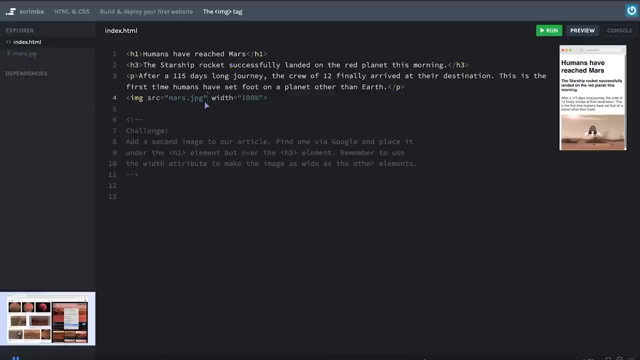 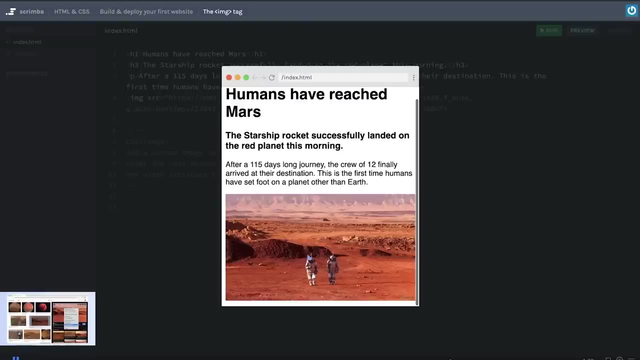 copy image address. With that you can simply paste it into the source attribute. So I'm going to remove marsjpg and paste in the image address which I just copied. If we now run the code, you can see there we go. we have borrowed this super cool image from another website online. 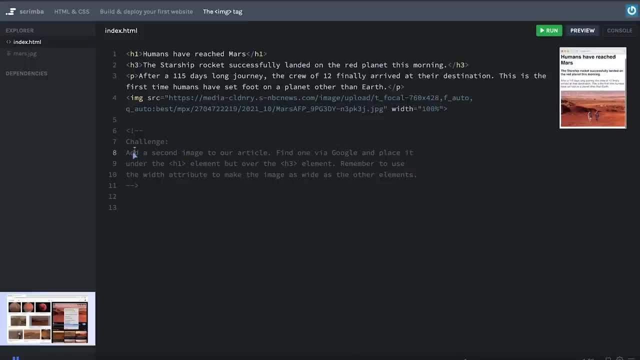 So it's time for a challenge. What I want you to do now is add a second image to our article. I want you to find one via Google and then place it under the h1 element, But above the h3 elements. that is right here. And finally, remember to use the with attribute. 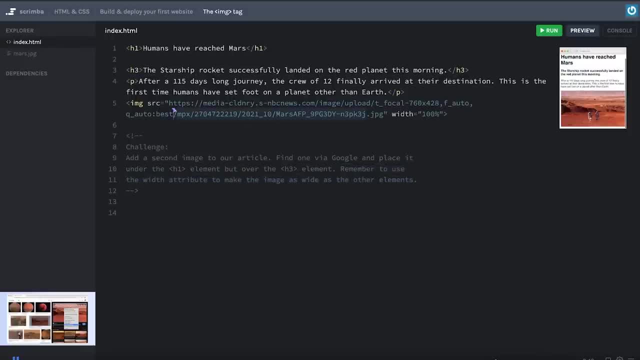 to make the image as wide as the other elements. I'm going to leave you here with the Mars image again and wish you good luck. go ahead and solve this challenge right now. Okay, hopefully that went well. what you need to do is write the angle brackets: IMD. 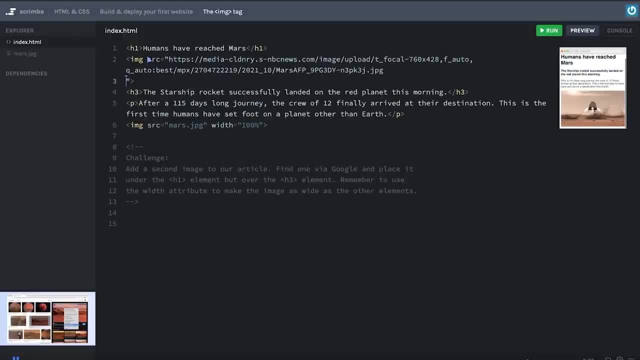 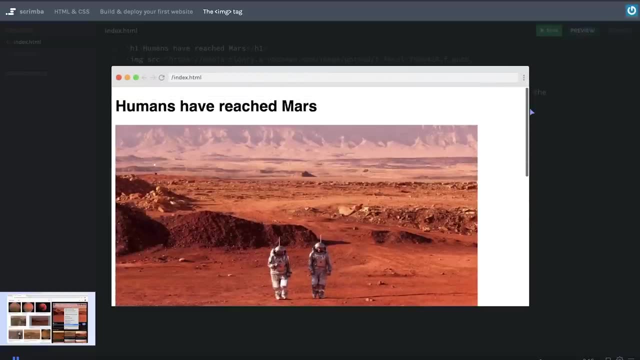 and set the source to whatever image you found online. I'm going to reuse the one I found earlier like that. if we're rendering this, This is a really wide image by default. that's not what we want. we wanted to scale with. 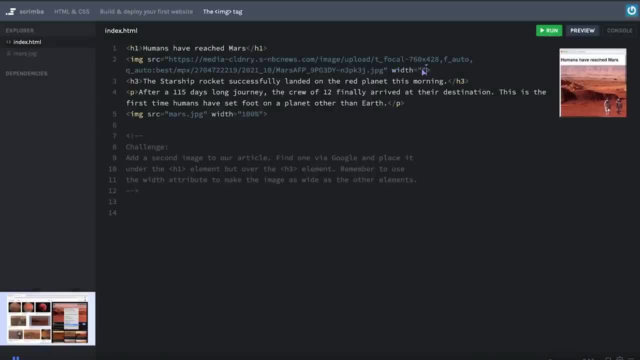 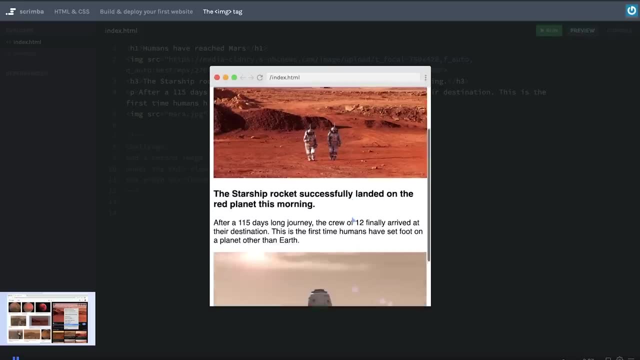 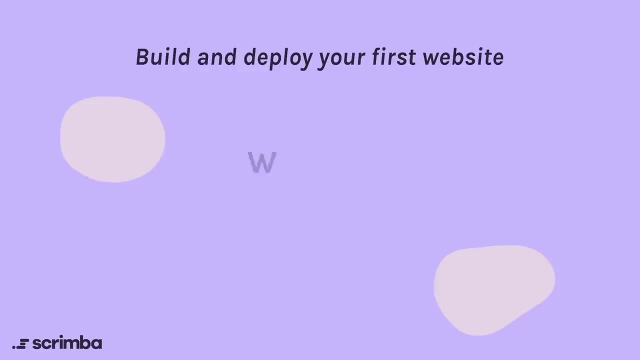 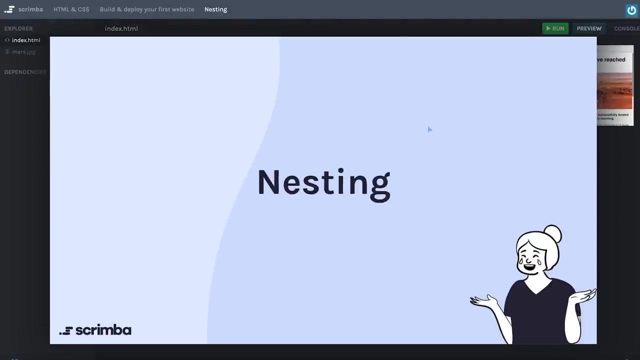 our browser. So we need the with attribute with equals- a hundred percent, like that. And now we have two super cool images in our article, both scaling up and down with the size of the browser. Great job, Let's move on. Okay, now you're going to learn about something called nesting. which is the image that we're going to be using for our article, And we're going to do that by clicking on the image. and then we're going to go to the image and we're going to click on the image. and we're going to click on the image and we're going to 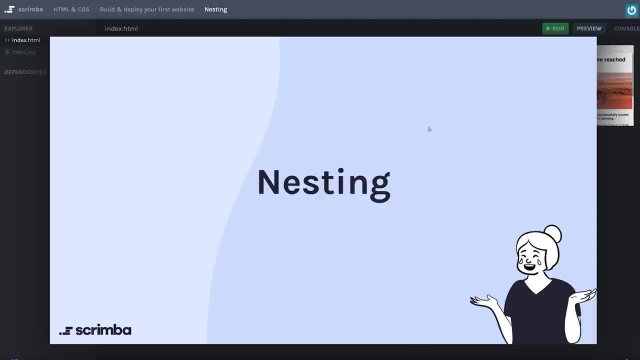 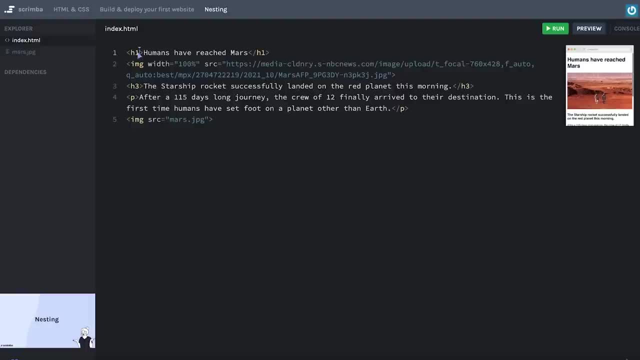 do the act of nesting HTML elements inside of other HTML elements. So let me show it to you in practice. Let's say that we want to group all of these elements here together. what we then do is, above all of the HTML tags, write a another HTML tag And in this case, 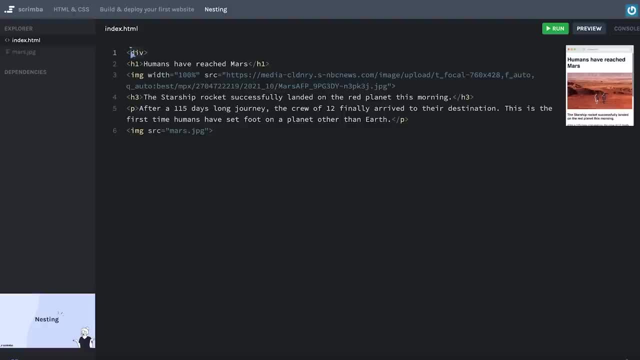 we'd use the so called div, which is short for divider. However, I don't think that is a very good name. I would rather call this, for example, a container, though div is what it's called, So we're just going to have to stick with that. 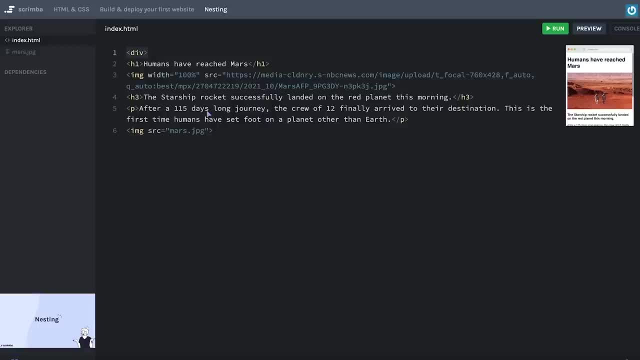 Now, in order to nest elements inside of this div, we'd write the closing tag below all of the HTML tags in our article And then, for readability purposes, we'd indent all of the tags in our article. So now our h1, image, h3, P and image here are all children. 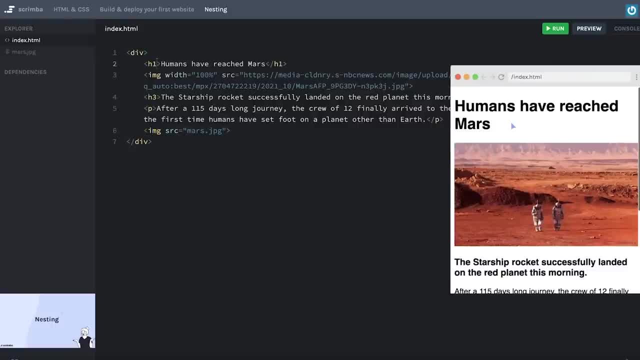 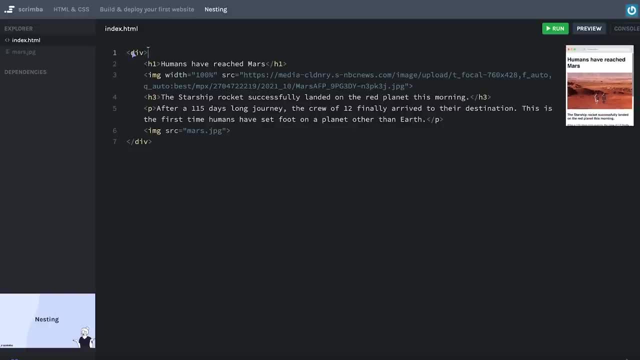 of this div tag right here. This doesn't change our layout at all, So this div tag here is invisible. However, it has now given us the ability to target the entire article, and that is useful if we, for example, want to add some styling to our entire article using 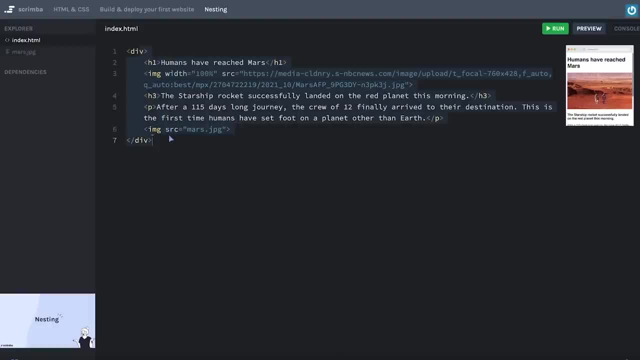 CSS or somehow manipulated using JavaScript, which is the programming language that you use in browsers, And very often you'll actually see a ton of divs on a page. So, for example, you'd see another div round this image element here, which then would have been indented. 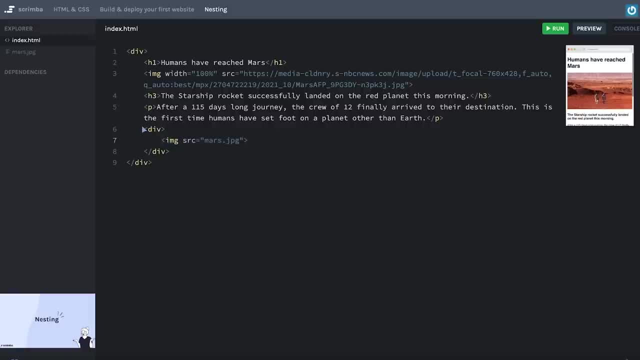 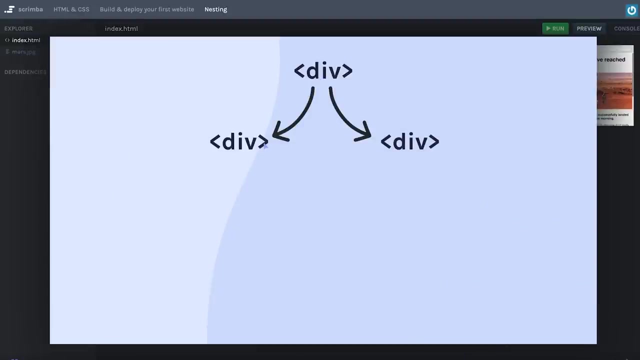 yet another time in order to signal that this is indeed a child of this div, which, again, is a child. Now, if we were to visualize an HTML document, it would look something like this: you'd have, for example, a div up here and it would have two children which could be their own divs. 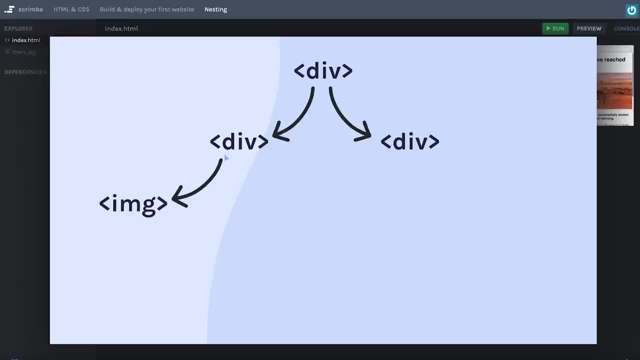 like this. And then this left hand div here would, for example, have an image tag as its first child and also an h3 as a second child. The other div on the right hand side, could have an h1 tag as its child, P tag as its child, maybe even another div as its child. 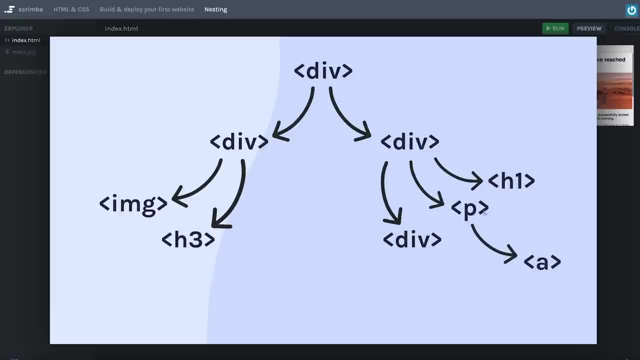 And then, if we go yet another level deep, we'll see that this div here is a child. And if we go yet another level deep, this paragraph tag might have its own child, which could be, for example, an, a tag which you haven't learned about yet, but which you'll learn. 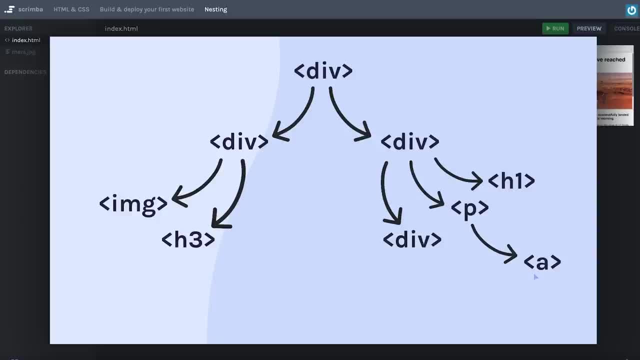 about soon is. that is the so called anchor tag that allows you to create links on websites, And looking at this visualization, you might think: well, this kind of looks like a family tree. And yes, it does, And that is exactly why we call this structure the HTML document. 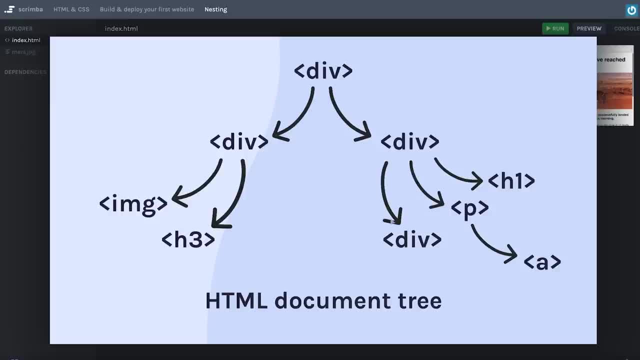 tree because we are inside of an HTML document and how they are nested inside of each other. it becomes kind of like a tree where you have a trunk and then branches going out from that and then yet again new branches going out from those branches and so on and 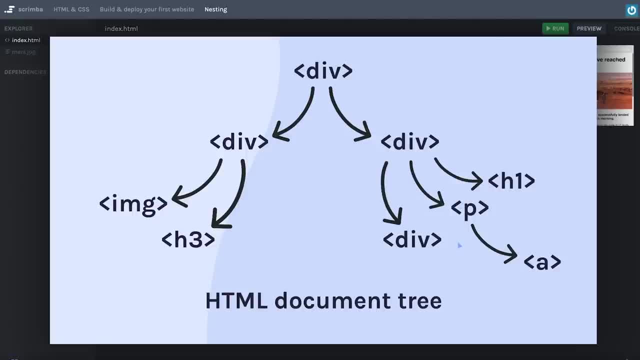 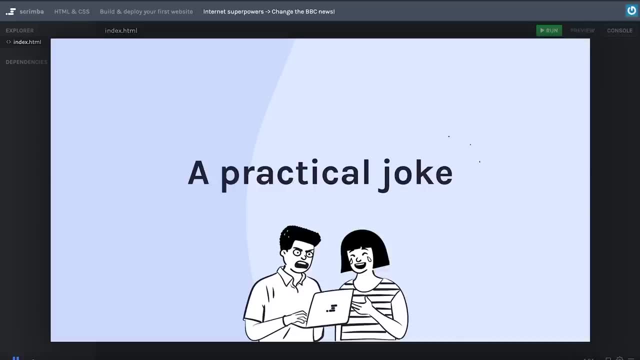 so on. So now that you know that, let's move on to the next grim. Okay, now we're going to use your newly acquired internet superpowers in order to perform a little practical joke, Because you might have a friend who is far too obsessed with a sports. 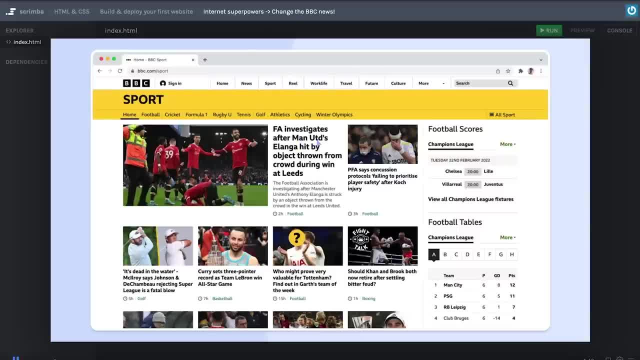 team, For example, if I'm a Manchester United fan, and one of the worst things I can imagine is if some rich billionaire buys the club and changes its name. that would make me truly outrageous. So what we're going to do now is change the news on BBC Sports so that 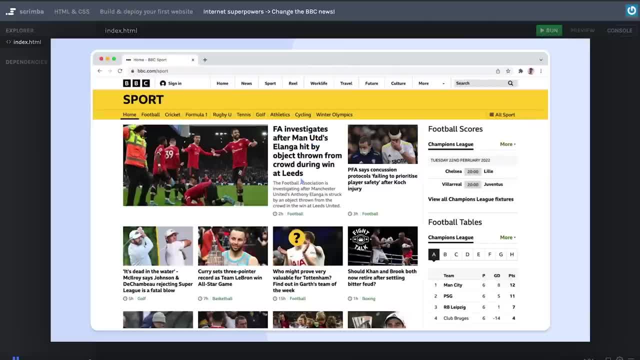 you then can show this page to a Man United fan and thus make them really upset while you get a good laugh. So let's go ahead and do this Here on the BBC Sports page on this top article here I'm going to right click on the text And then you can see it gives me the option to 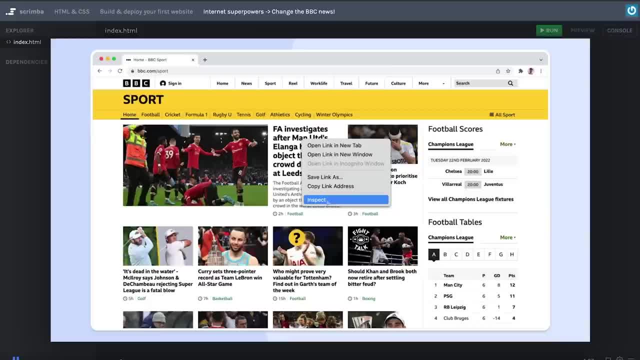 choose inspect. Now note that this is on a Chrome browsers, as that is what I'm using. If you're in a different browser, there might be slightly different steps here or a different wording, But overall, in general, the steps are the same, So I'm going to click on expect. 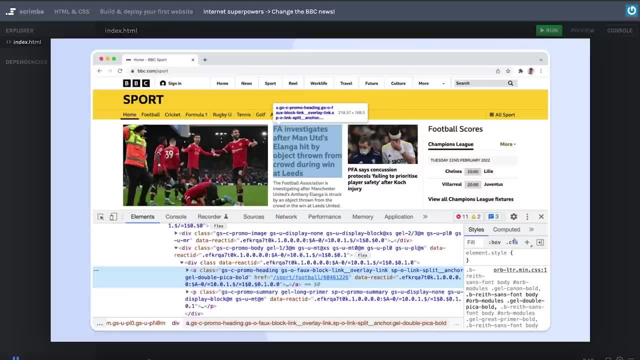 And then you can see that it opens up this panel on the bottom of the browser. This is called the developer tools, And here you can see we are in the elements tab, And that shows the HTML elements that are on the page, And here the one we have chosen now, which happens. 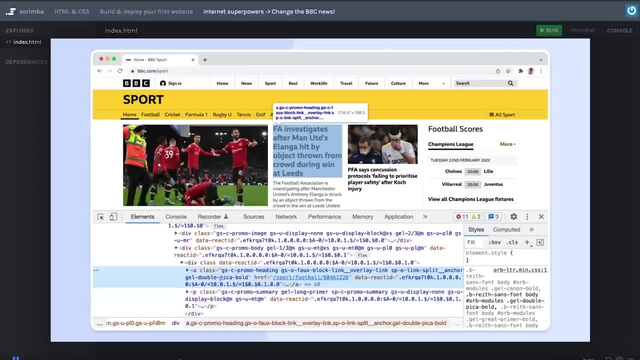 to light up this area on the BBC site contains the title of our article And it is an, a tag which I've just briefly mentioned and that you're going to learn more about later. Now we can't see any text here, So I'm going to click on this age tag And there you can see. 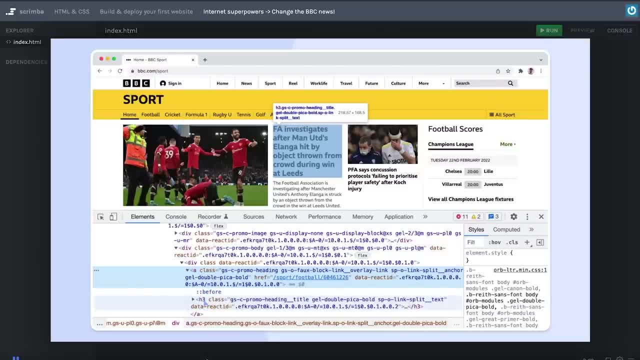 it contains an age three tag nested inside of it. If we click on that one as well, you can see that there we see the text that is rendered in the browser. So I'm going to click on that one as well, And then you can see that there we see the text that is rendered in. 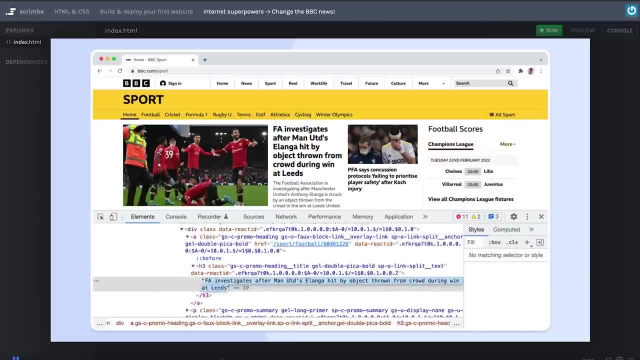 the browser And then you can see that there we see the text that is rendered in the browser. So here we can double click on that text and change it, for example, to something as awful as Jeff Bezos to buy Man United and rename the club after himself. Oh my god, that is. 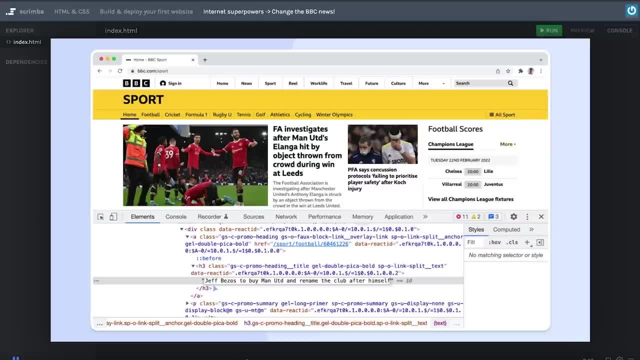 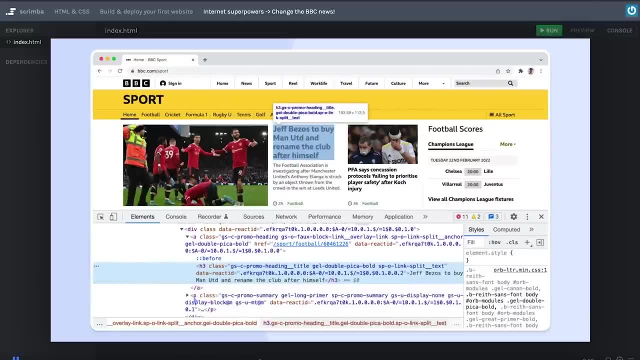 about the worst piece of news Any United fan can read. So if we now hit enter there, you can see: boom, we have changed the text on BBC. Now let's click on this paragraph here as well, Open it up, Because there we can also change the text that is written underneath. 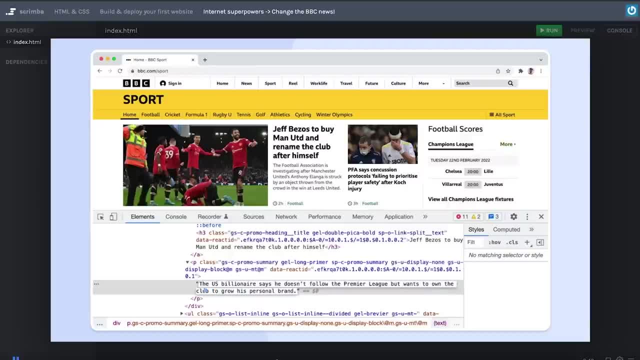 the title. So here we can see that Justin the US billionaire says he doesn't follow the Premier League but wants to own the club to grow his personal brand. Oh, this just gets worse and worse. So now, if we hit enter, that is also rendered in the browser. Now I'm going to scroll a. 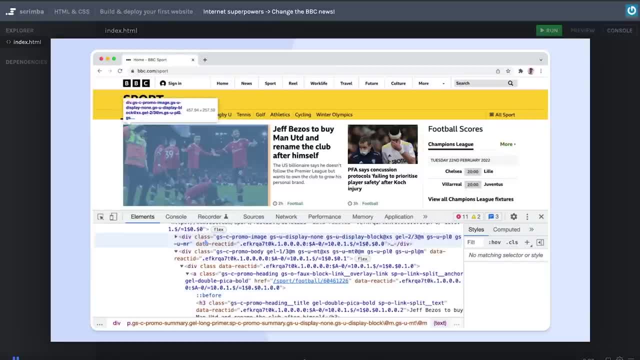 little bit up in the dev tools here and hover over this div tag here, Because, as you can see, that highlights our image. So it seems to be that our image is nested inside of a div tag. Let's open it up by clicking on this triangle And there we can see another div. 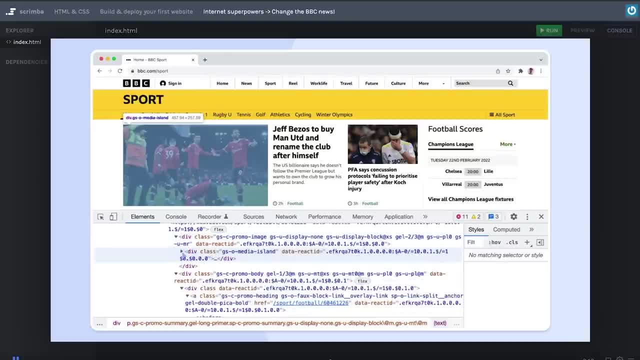 tag. Okay, still highlighting the image, Let's open up that one as well. Oh wow, There we have yet another div tag, a div inside of a div inside of a div. This is web development in a nutshell. Let's open it up again And there, Yes, we can see our image tag. I'll 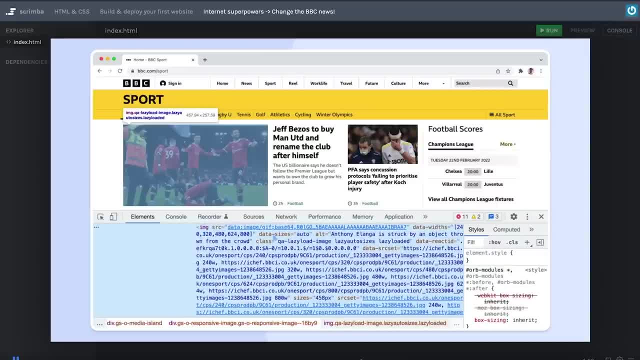 scroll a bit down And you can see there are tons of different attributes here. we're going to ignore almost all of these and then instead direct our attention towards the SRC attribute, that one we know, because that is the one we need to check. So let's go ahead and hit. 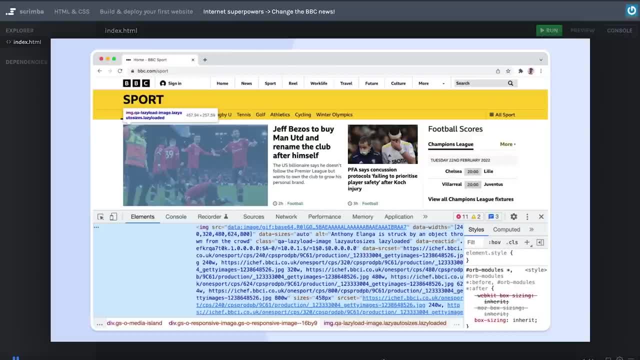 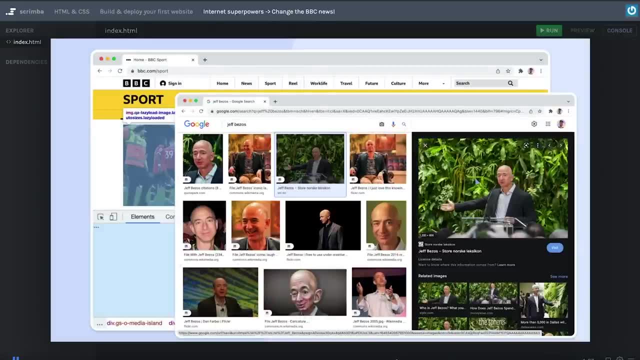 enter. Let's go ahead and hit enter And we can see that our image tag has been changed in order to change this image. So now let's open up a new window. search for Jeff Bezos. click on an image we like, for example this one right here, right click on it and choose copy. 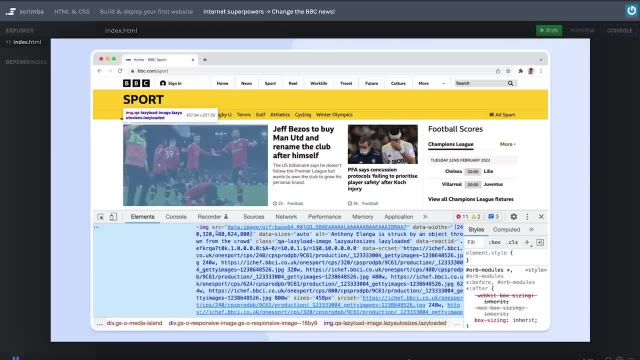 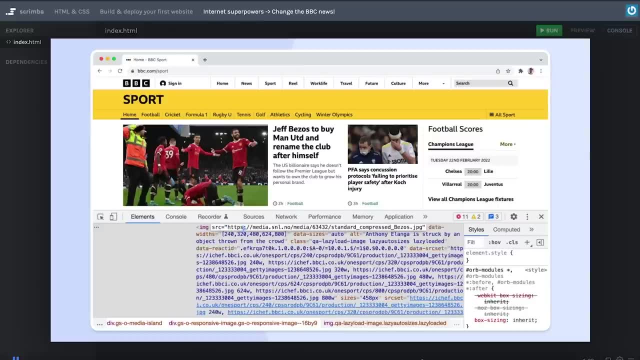 image address then can do now is double click on this source and then remove the existing source inside of the quotes like that, and then paste in our image of Jeff Bezos. However, if we now hit enter, you can see nothing changed, And that is because BBC is a little bit fancy. 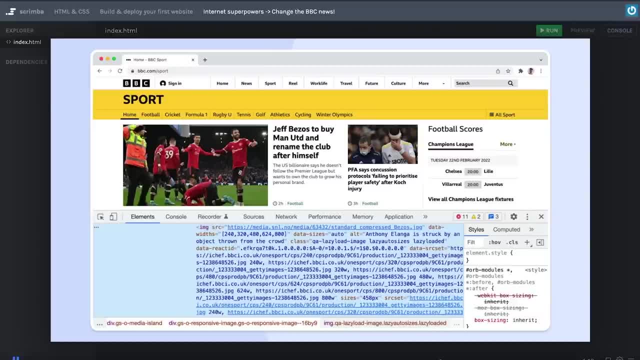 here We have another attribute called SRC set, which helps the browser render different sized images on different types of screens, depending on what kind of image is appropriate for the given screen the website is rendered on. So what we're going to do here is just double. 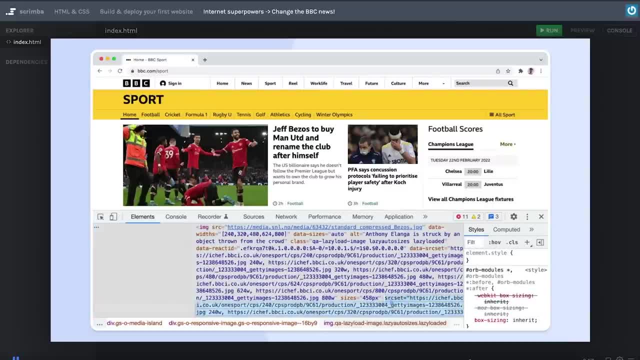 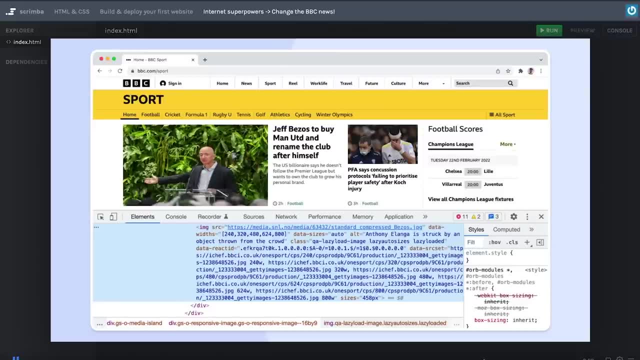 click on the SRC set so that everything is highlighted and just delete all of it and then hit enter And boom, there you go. We have Jeff Bezos looking pretty ready to acquire this football club and rename it Bezos United. Finally, we have the next image, So we're going to hit enter And then we're going to 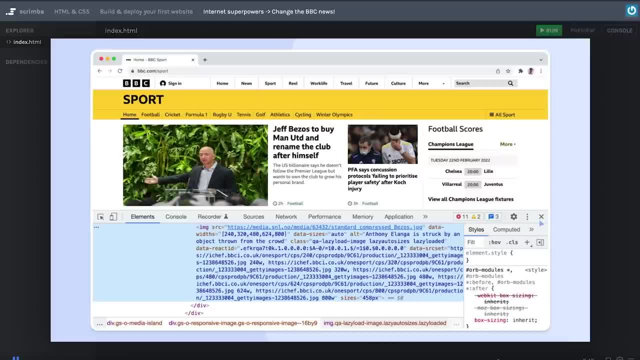 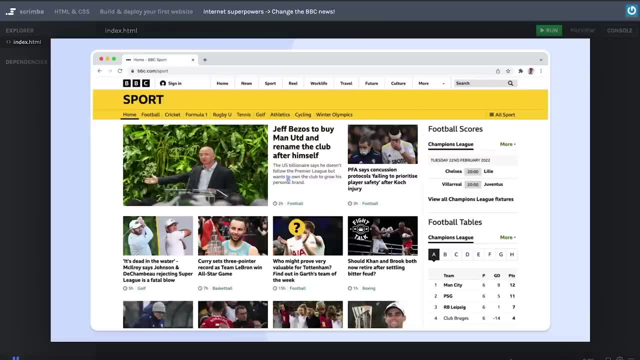 close this panel by clicking on the X in the right corner. here And there you go, we have our article. So now the final step is just to take this site, show it to someone who is a Manchester United fan and get a good laugh. Now a final notice, if you refresh. 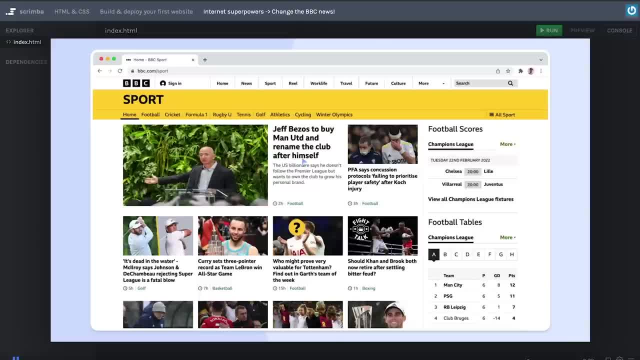 this page. you will lose your changes because you only made your changes locally. And when you refresh it, the entire page gets the fresh data from the database of BBC and not from whatever local changes you did. And since it is local, that's fine. But if you want to, change it. you can do that by clicking on the X in the right corner. here And there you go, And now we have our article. So now the final step is just to take this site, show it to someone who is a Manchester United fan and get a good laugh, And then we're going to. refresh this page, show it to someone who is a Manchester United fan and get a good laugh, And then we have our article. So now the final notice: if you refresh this page, you will lose your changes, because you only made your changes locally, And that also of 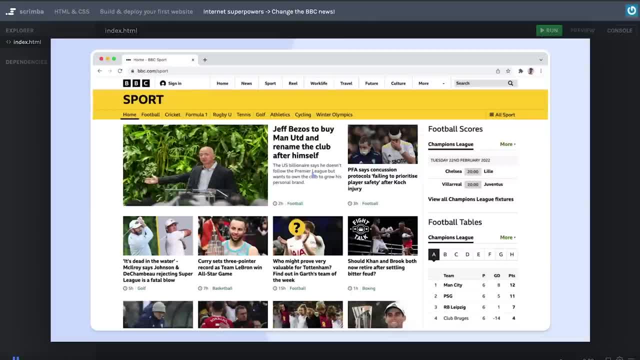 course implies that your changes only happen on your computer. you don't change BBC in production, of course, So go ahead and play around with some sites online, See if you can come up with a fun little practical joke for a friend. Have fun and I'll see you in. 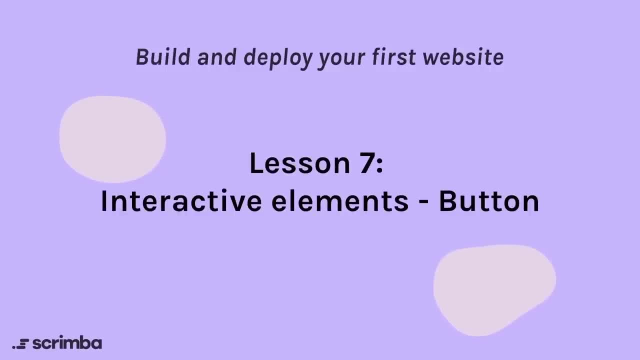 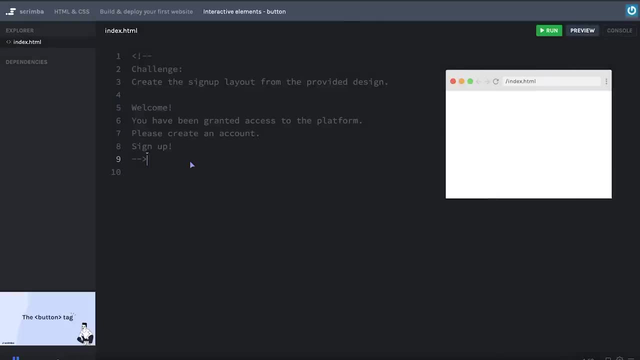 the next trim. Now you're going to learn about your very first interactive HTML element, And that is the button tag, because buttons are all over the web. So to create a button, simply start with a button. So if you right click a button and choose the button tag. 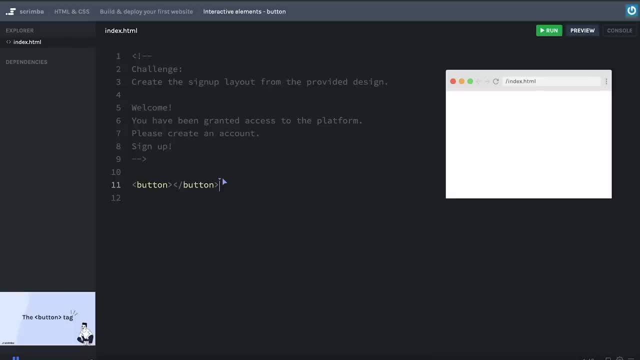 start with your angle bracket and a button opening tag and then a button closing tag, like that, And in between the two tags you write whatever text you want inside of your button. Now, as you can see, it's styled with a background color that also has a border. 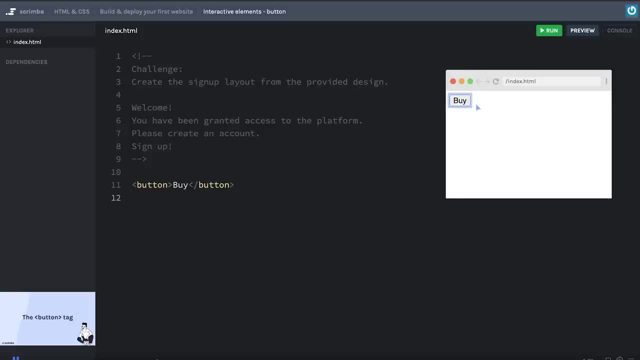 around it And you can even click it. Now, this button doesn't do anything. in order to hook this up with some kind of feature- for example, trigger a purchase- then you'd have to learn JavaScript, And that is outside the scope of this course. It's something you'll. 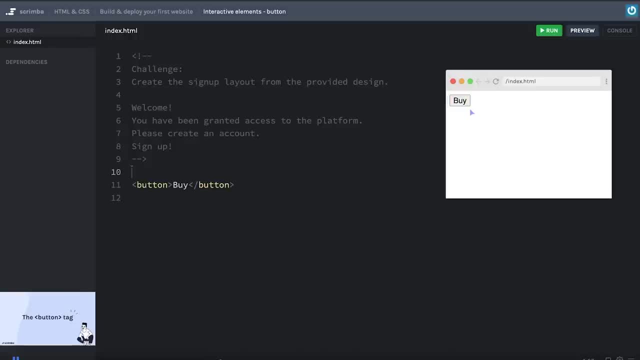 learn later in the front end developer career path. So for now, our button will just be there and pretend to do something, while actually being pretty useless. Now that you've seen this once, I want to put you on the spot and give you a challenge I want you to create. 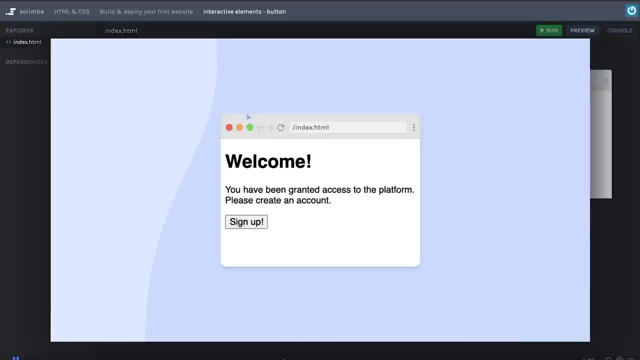 a layout according to the design in this slide. So imagine that you are building a website where people are to sign up. then it would be very natural to have something like this: we have an H one at the top welcoming them, a paragraph with a little message and then 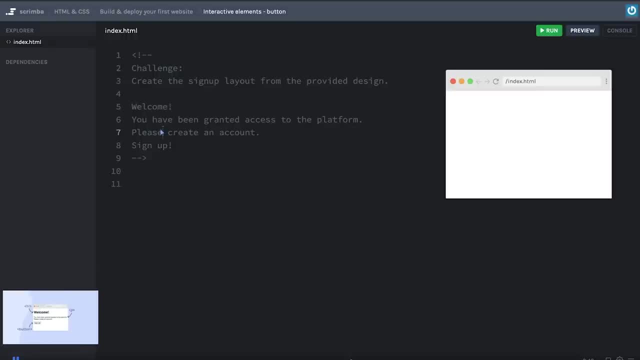 a sign up button. So I want you to create this layout. you don't have to write the text, because I've provided it here. Just make sure that you set up the HTML tags correctly so that renders properly on the page. Good luck. 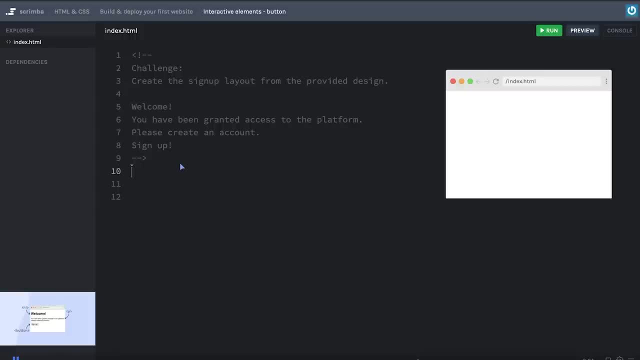 Okay, hopefully that went well. Let's now do it together. I'll start with the welcome H. one tag like that. they start in and boom, there we go. Next up, there's the paragraph opening tag, closing tag. 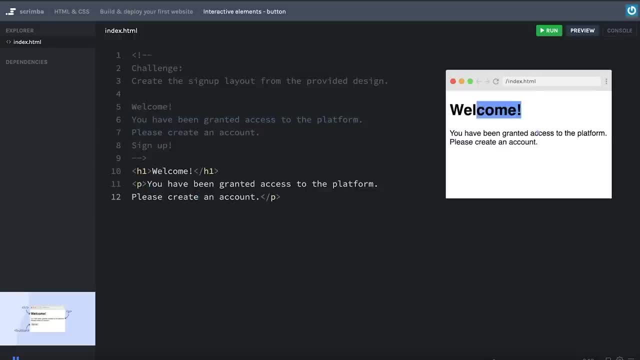 Then pasting the text. in between running this code, it still looks correct. Finally, the button like that with signup written inside of it. And boom, there we go. we have our completely useless signup form that doesn't do anything. But in the next screen we're. 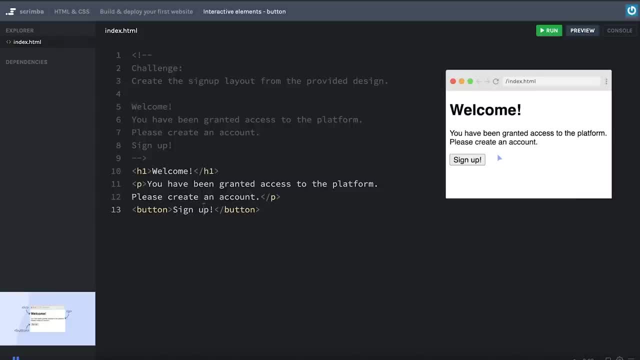 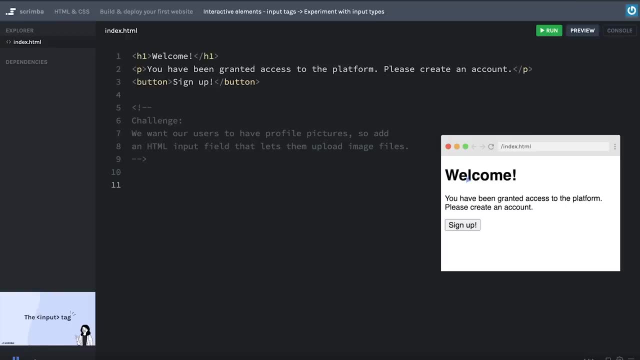 going to add on to this, So stay tuned and then I'll see you there. The signup section we have here is actually pretty useless because there's no way for our users to add, for example, their username or password. So in this group we're going. 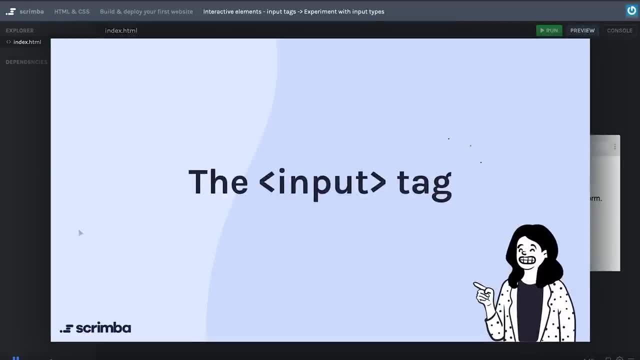 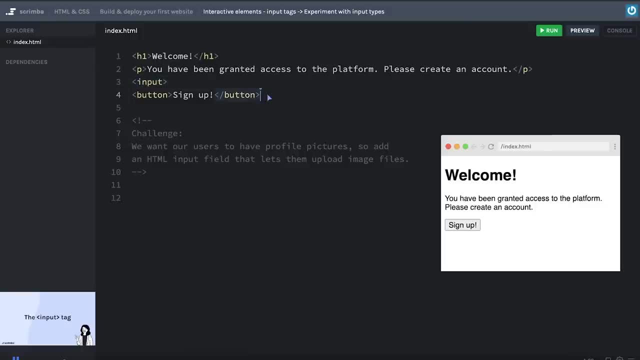 to fix that, which leads us to the input tag. the input tag is, just like images, a self closing tag. So we only write the opening tag and not the closing tag, like we do with buttons, for example. However, we have to specify what kind of type our input should be, So it has. 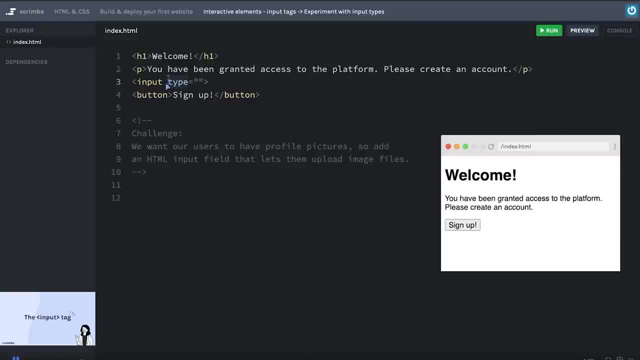 this type attribute, just as the image has a source attribute. And the value of the type can be a range of different options, But we're going to start off with the most common one one, and that is text. If we run this, you can see we get this nice little text box in. 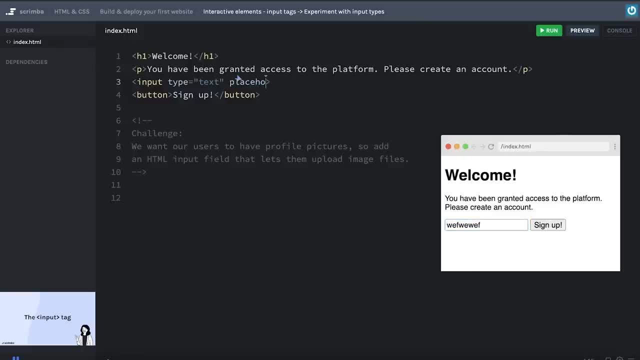 the browser. Another handy attribute is the placeholder. That's where we can give the user a hint about what kind of data we're asking for. So, for example, enter username. like that. If we run this you can see it says enter username. Okay, let's do a mini. 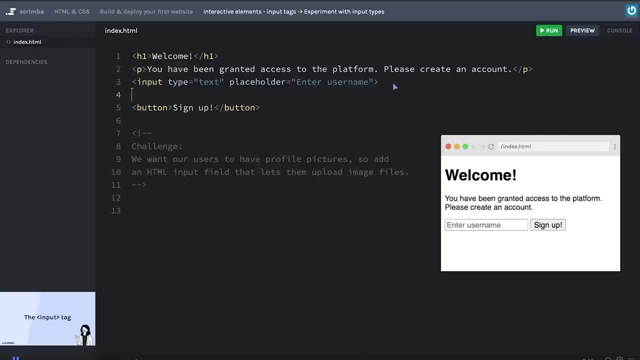 challenge. We, of course, want them to enter their password as well, So I want you to create a new input field on line four, which is identical to the one on line three, though it should say enter password in the placeholder as opposed to enter username And don't just. 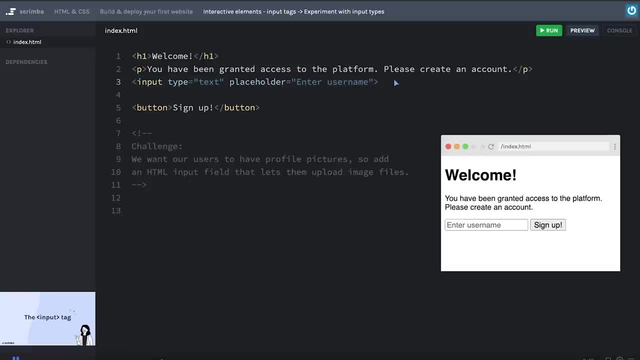 copy this line and change this word. I want you to get some muscle memory here, So go ahead and do that right now. Okay, hopefully you did like this. input type equals text, placeholder. enter password, like that. And there we go. Now you can enter a username and the password. 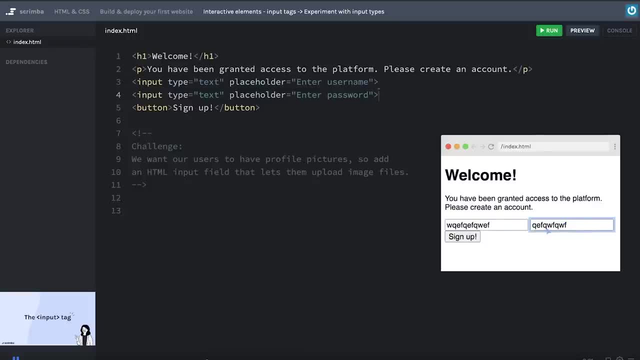 However, in the real world, passwords are never exposed like that. The characters are always masked, And the way we achieve that is simply by changing the type from text to password, like that. If we run the code now, you can see the username is shown, but the password is masked. Really. 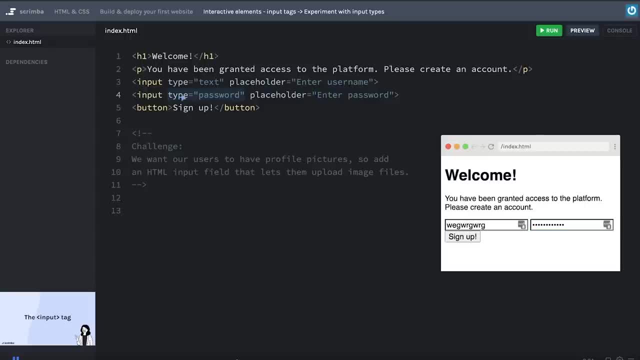 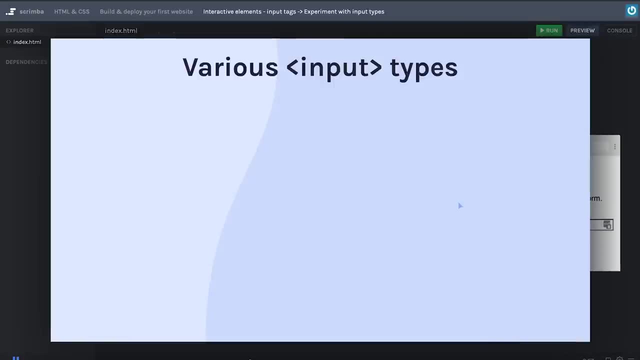 nice. And speaking of this type attribute, here it can take a range of different values which turn into really interesting interactive elements on the page. For example, you can do type equals date. let's say you want the user to add their password. Let's say you. 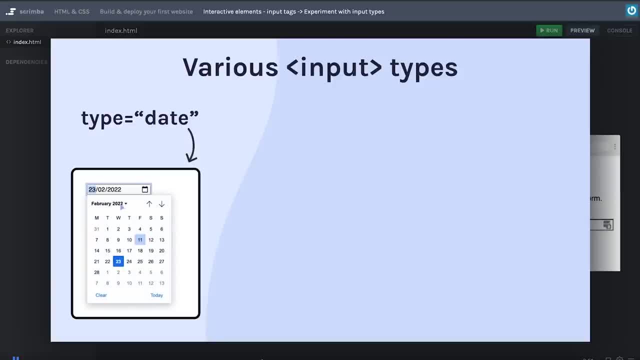 want the user to add their birth date during signup And then you get this nice little date picker. Or you can do type equals time, For example, if you want the user to be able to configure when they should get some kind of notification that gives the user a nice. 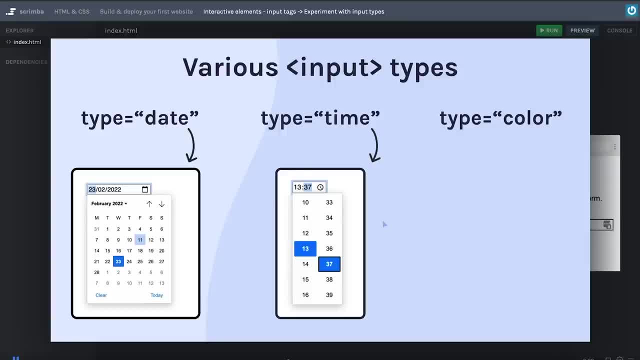 time picker. Or let's say you want to give the user a way to configure the theme of their profile with colors, then you can do type equals color And then you get this powerful color picker where the user can add basically any color there is through moving around on. 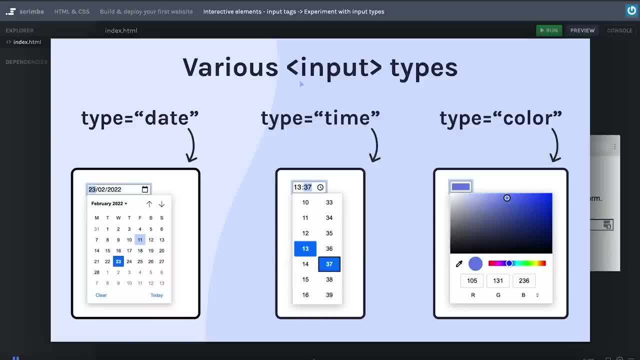 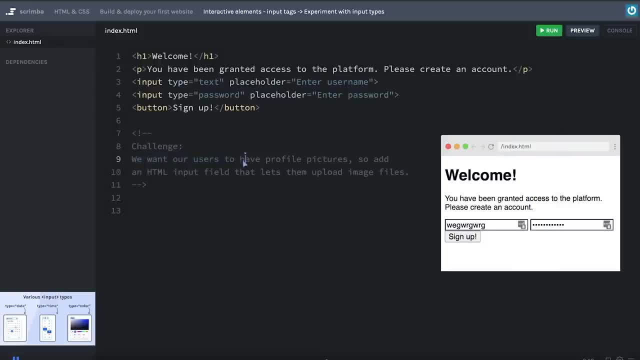 these dots, So the tag is a really versatile tool in your toolbox. Okay, let's move on to the main challenge, Because I want our users to have profile pictures, which means that you need to add an HTML input field that lets them upload image files, And I'm not going to tell you what kind of type. 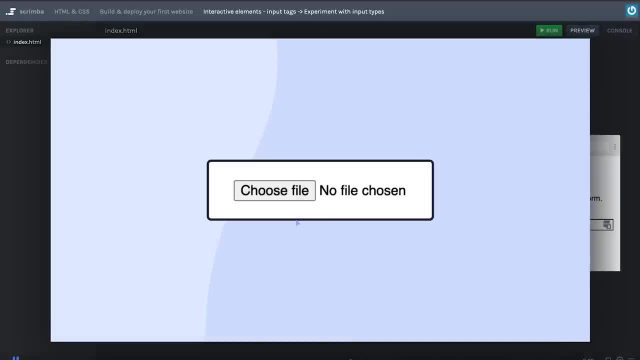 that input field has- I'm just going to show you how it looks- which is like this- you've probably seen it online before. It's basically a button And when you click it, it lets you choose an image from your local file system. 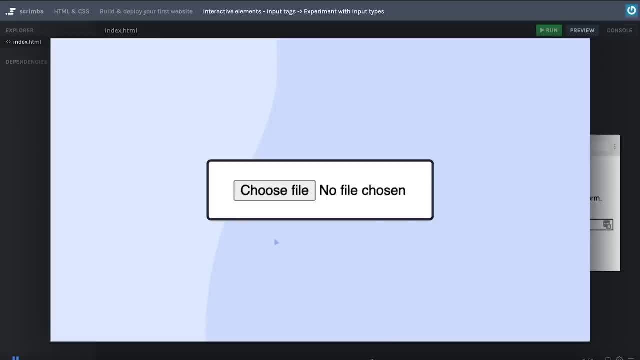 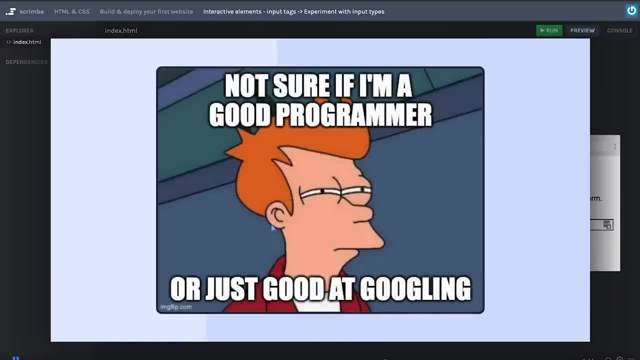 And the reason I want you to figure out what the type attributes should be here is because being good at googling is actually a huge part of being a good programmer, And the two are actually not that easy to separate from each other, So this gives you a way to practice. 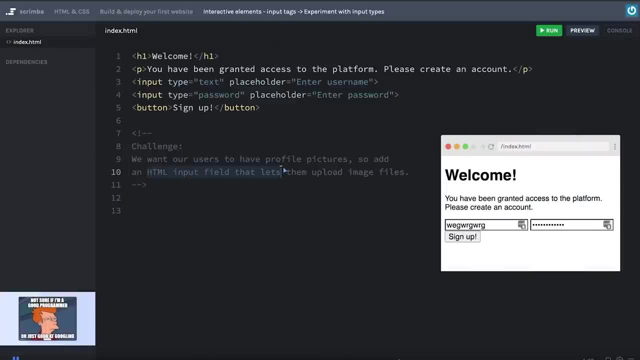 those googling skills, And I'm going to give you a hint that the keywords you should use are found in this last sentence, right here. So go ahead and solve this challenge right now, And then I will, of course, show you the solution when you return back to me. 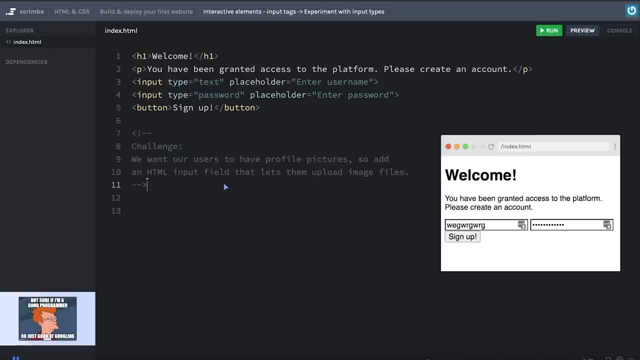 Okay, hopefully that went well. let's do this. The keywords I think are important here are HTML inputs, because we know we're looking for an HTML input tag. And then what is our intent? Well, it is to upload image files, And I think Google can handle this just by. 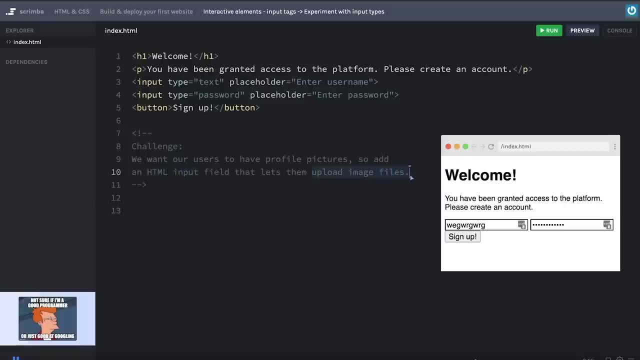 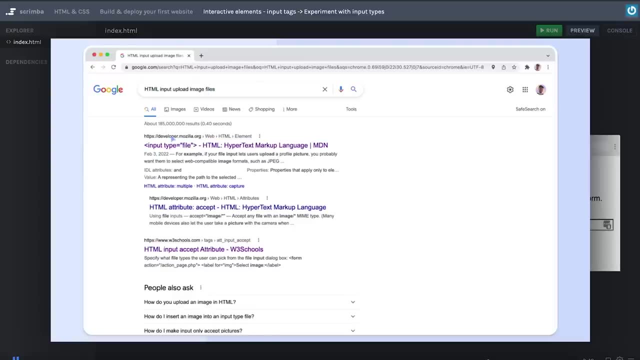 combining HTML input, upload image files. if we just paste that into Google, let's see what we get. And, as you can see, when we search for that, we get a first hit from developermozillaorg. Let's click into that And here you can see. 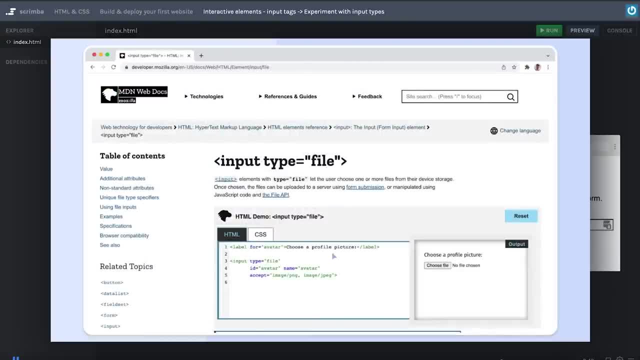 the title is: input type equals file, And we get this little code snippet here And it also says: input elements with type file. let the user choose one or more files from their device storage. Sounds pretty good So far. let's zoom in on the code here And there. 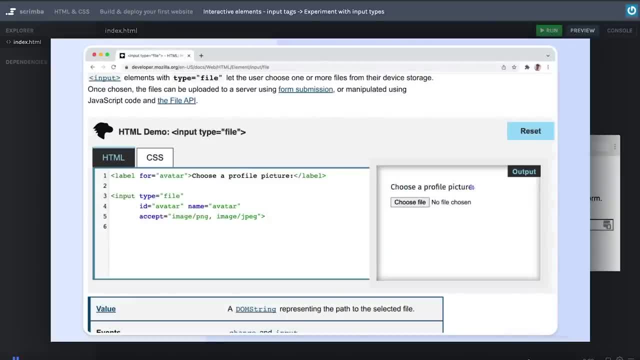 you can see that they are actually using the profile picture example themselves. choose a profile picture With this button, which looks suspiciously similar to what I just showed you a couple of minutes ago. So I think we've found it. What we're looking for is type equals file. 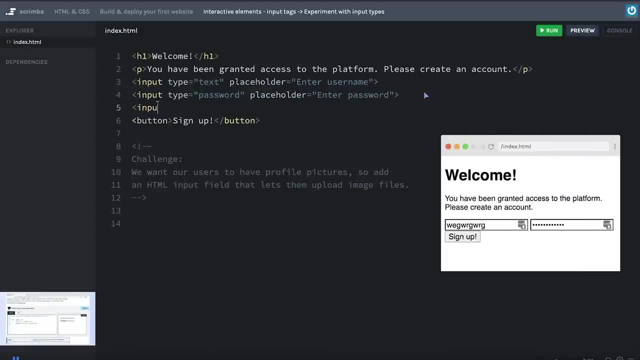 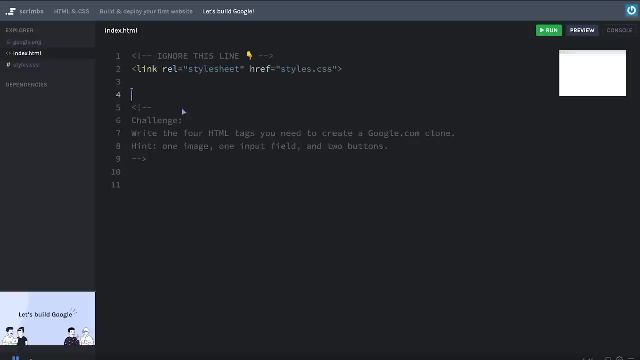 Let's add this up above the signup button: Type equals file, like that. We run this code: Yes, there we go. We get this button, which looks like exactly what we're looking for. Okay, now we're going to move on from using Google. 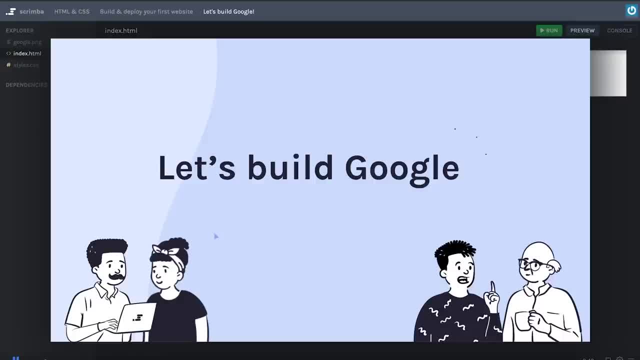 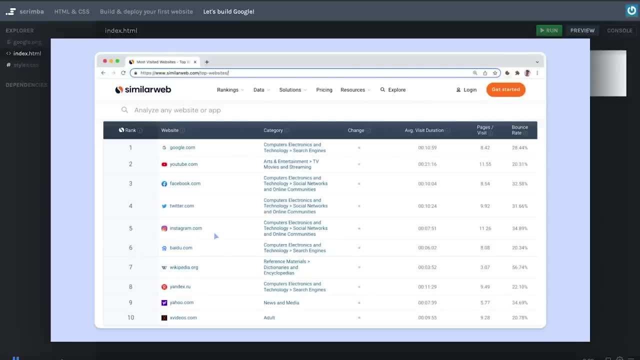 To building Google. I mean, how cool is that? You've learned HTML for just about 30 minutes And now you're going to build the most visited website in the world. That is just amazing. As you can see here on the similar web overview, Google is at the very top amongst the most. 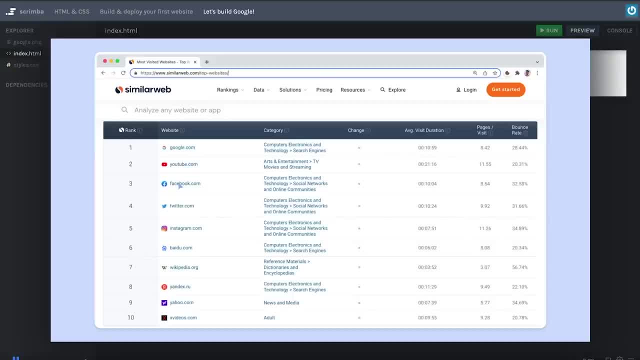 visited websites in the world, beating sites like YouTube, Facebook, Instagram, Wikipedia and, all the way at 10th, a pornography site of course- And, by the way, it's a little bit sad- has almost three times the average visitation of Wikipedia, So a pretty deep insight about. 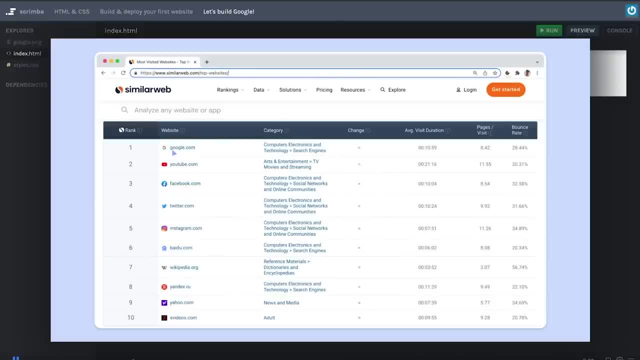 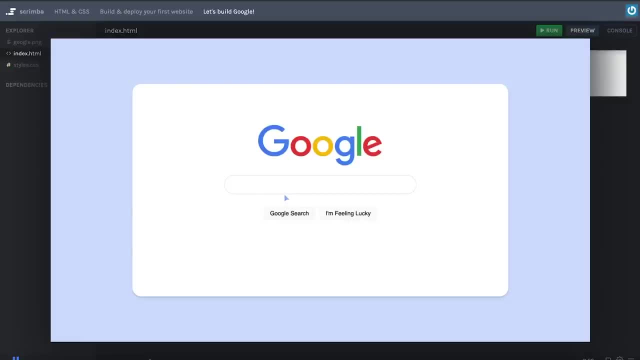 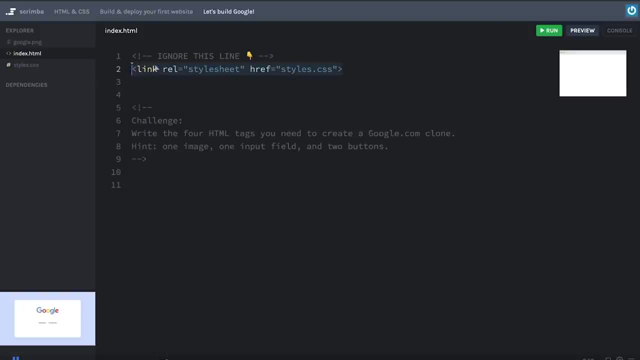 humankind right there. Anyway, we are going to build googlecom and it'll look like this. However, now you're probably wondering: how can we make a page look like this? this doesn't look like regular HTML, And that is because I've cheated a little bit and added this line up here, which is: 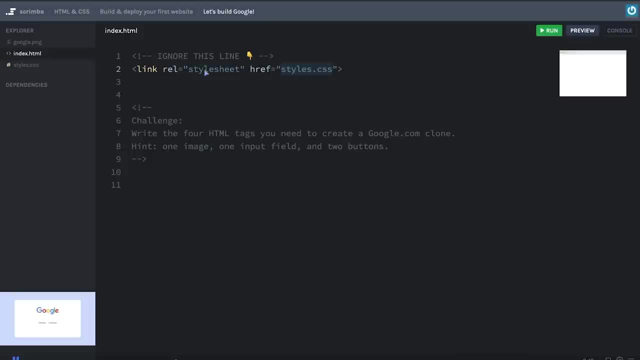 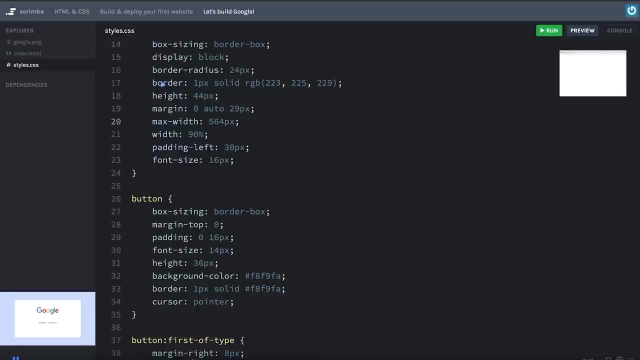 a link tag to stylescss And if you look at the file menu in the left hand side, you can see that actually we have a file called stylescss which contains exactly that: cascading style sheets, which is the language for styling websites and which you're going to learn all about a little. 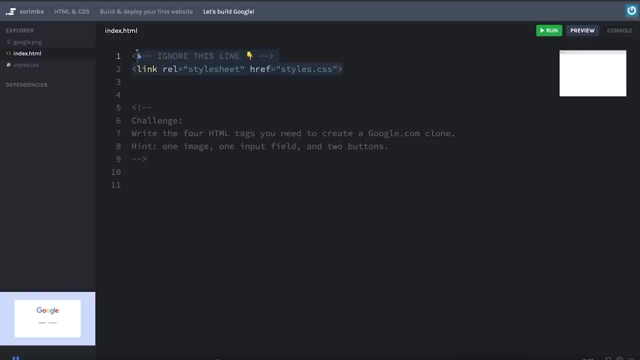 bit later in this course. However, for now, I want you to completely ignore this. what you should do instead, it's just create the four HTML tags we need in order to create a googlecom clone, And then we're going to create a link tag to stylescss. And if you look at the file menu in the left hand, 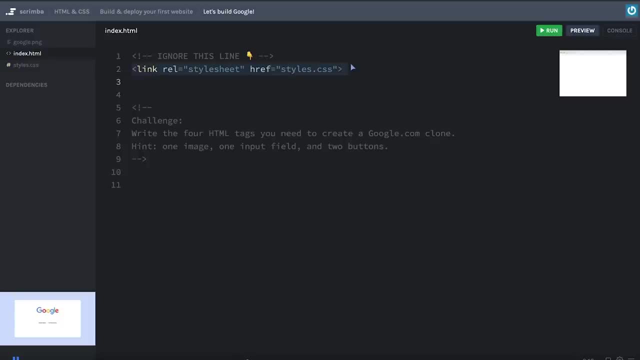 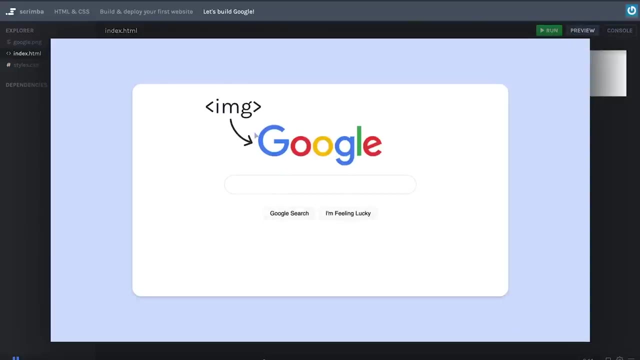 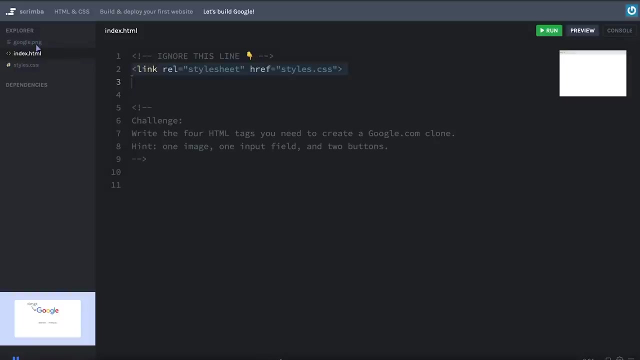 then this CSS will be pulled in and take care of styling the elements as they should be, so that it will look like this. And, to give you a hint, this is an image file pointing to googlepng, the file I've added here, and png is just a file format, just like JPEG. you can use it in the exact same way as 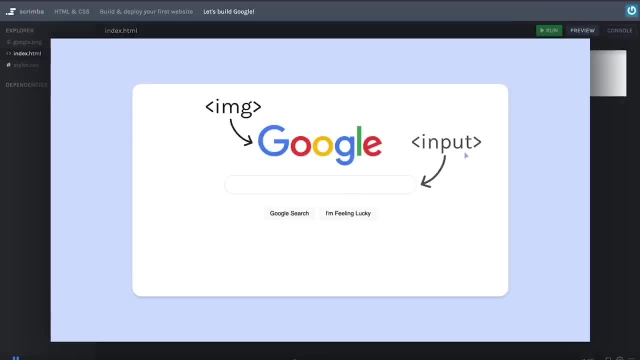 we use JPEGs earlier on, So you should know how to do that. And this is an input field. you have to figure out what kind of type it is. I think you might have a clue. This is a button on the left hand side. And this is a button on the left hand side. And this is a button on the right hand side. 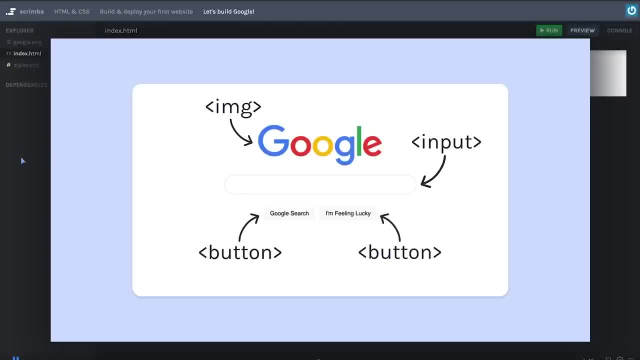 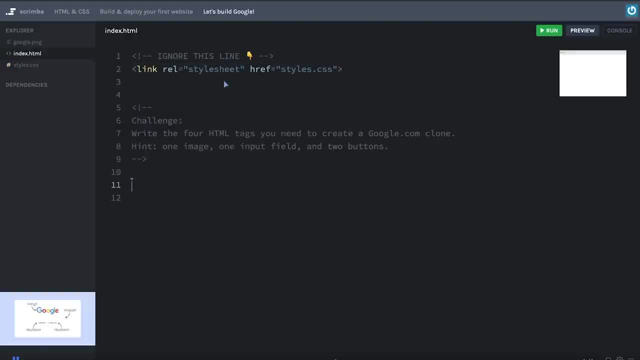 And this is also a button. So, basically, it is these four tags you need to create in order to build a clone of the world's biggest website. So go ahead and do that. Start down here and ignore the line up here, And then, when you return back to me, I will, of course, show you the solution as well. 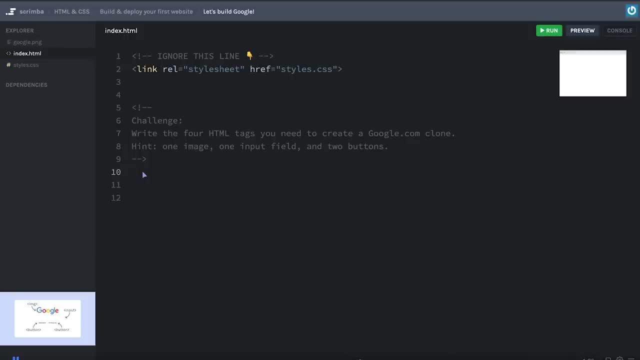 Good luck. Okay, hopefully that went well. If not, no worries, Let's do it together. So, starting with the image tag for the Google logo, I'm going to do IMG like that And it's a self closing one, So I don't need a closing tag, but I need a source attribute And it should point to: 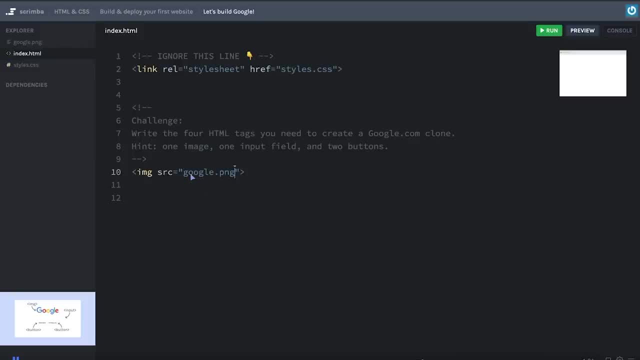 the googlepng file. So I'll just do googlepng like that And let's run this And oh, there we go, We got the logo. Okay, moving on, Let's do the input field also a self closing tag. 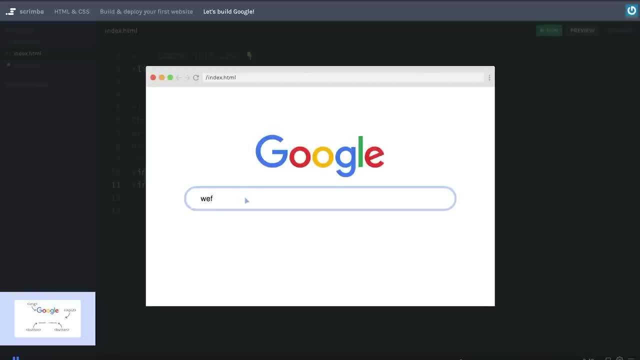 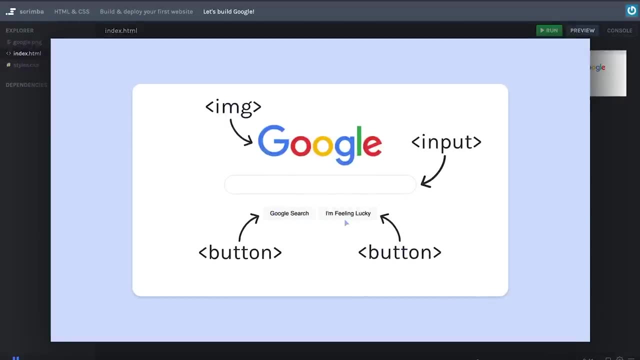 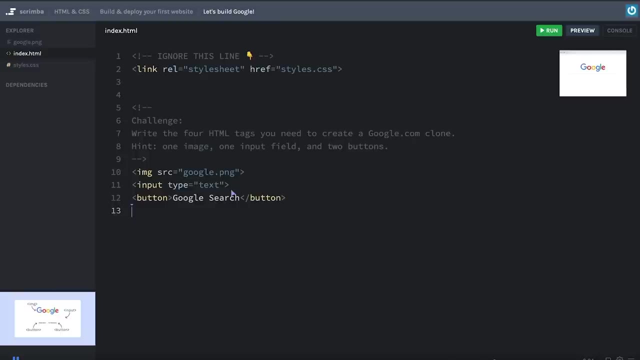 Running the code. And there we go. We have a input field looking pretty good, Okay. next up there's the two buttons, one saying Google search and one saying I'm feeling lucky. So I'm going to add both of these button Google search. And then, since I'm lazy, I'm going to copy it and do I'm. 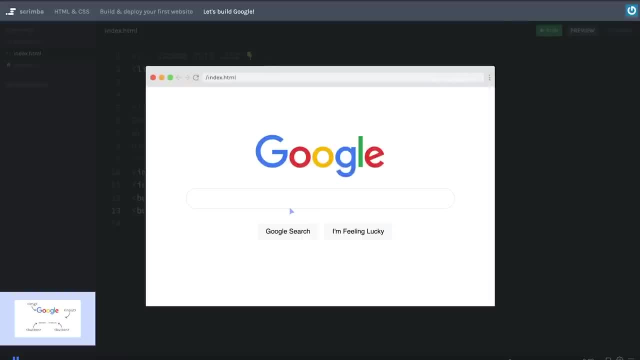 feeling lucky like that. Let's run this And there we go. We have a Google clone with just four HTML elements. So if you did this, give yourself a pat on the back. it is fantastically well done. you should really be proud of yourself. And if you didn't manage to do it, just try it again, And I think 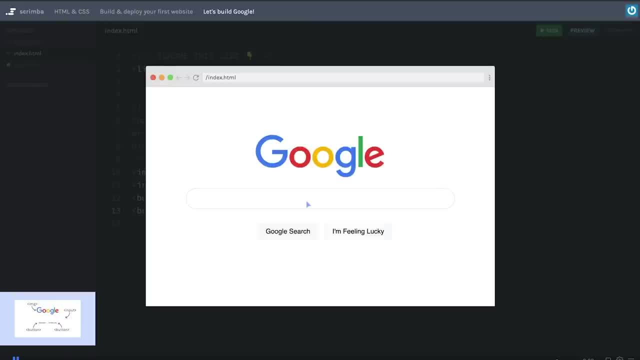 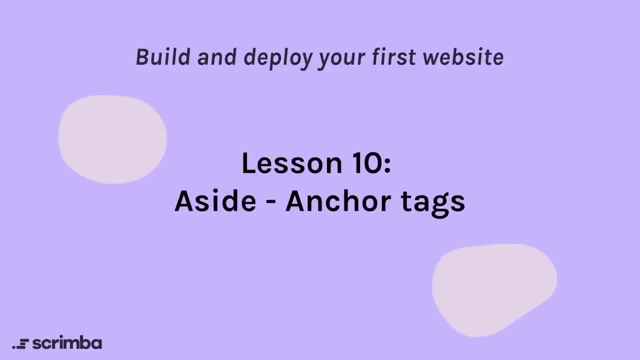 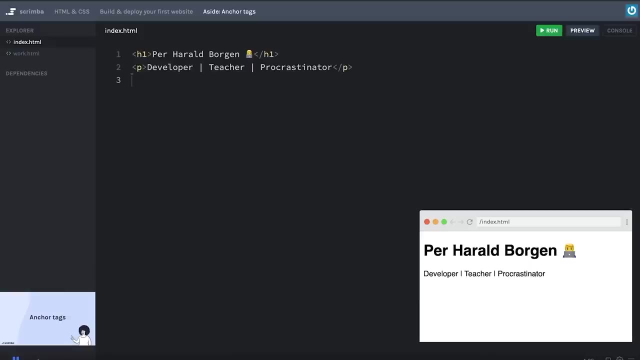 you'll make it. At this point, it might be a good idea to take a little break and digest everything you've learned And then, when you are ready to continue, I will see you in the next scrim. Okay, now that you've built googlecom, you probably want to showcase your project on some 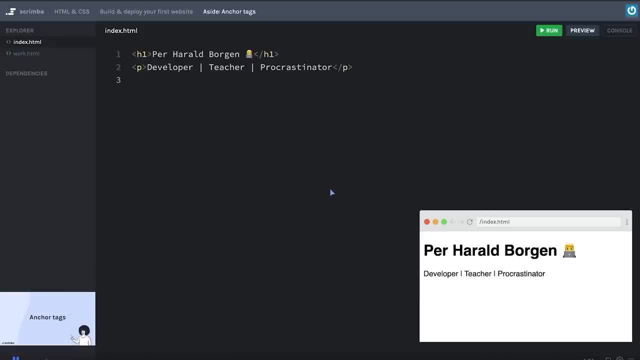 kind of portfolio page. So let's pretend we're creating exactly that. Here we have the index dot html page, the main page of our portfolio, And, as you can see, it says peer Harold Borgen, developer, teacher, procrastinator. 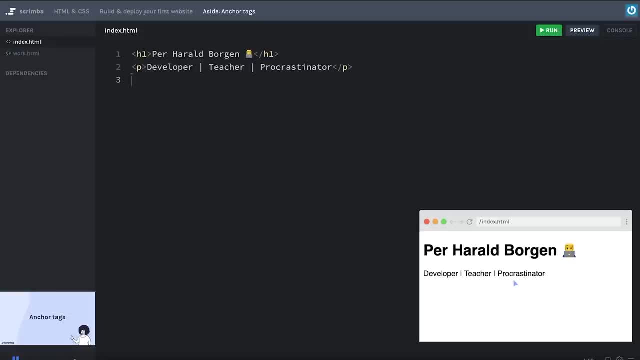 So a really good description of myself, though what it lacks is some kind of page or section which describes my projects, though I have actually created the underlying page for exactly that over here on work dot html. As you can see, this is a few tags. that describes my googlecom. 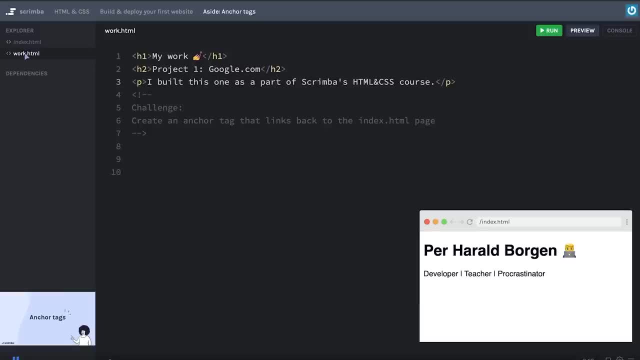 project. However, there's no way for the users to know this. the only way they can get to this page now is by actually typing work dot html up in the browser here, and then it is rendered. we don't want that. Instead, we want some kind of link from the index page, That is, this one that points. 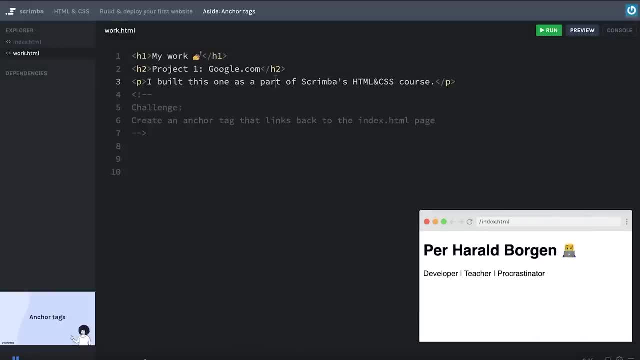 towards the work dot html, And in order for us to achieve that, you have to learn about anchor tags, aka links. An anchor tag is simply an HTML tag with an A, So if we open and close an anchor tag and write, for example, check out my projects here. like that: 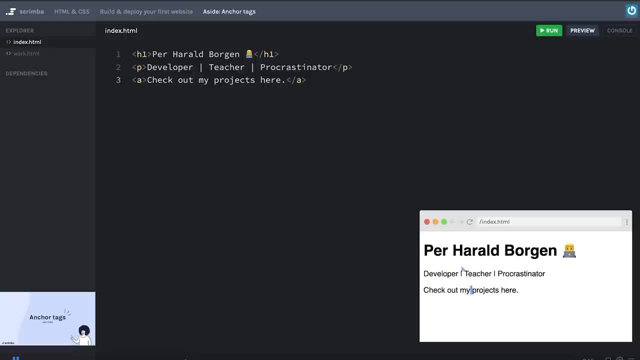 if we run this, it seemingly looks just like our paragraph and we can't click it either. And that is because for anchor tags you also have to provide it with an age ref attribute. that's short for hypertext reference. really fancy, scary looking word right there. don't worry about it. 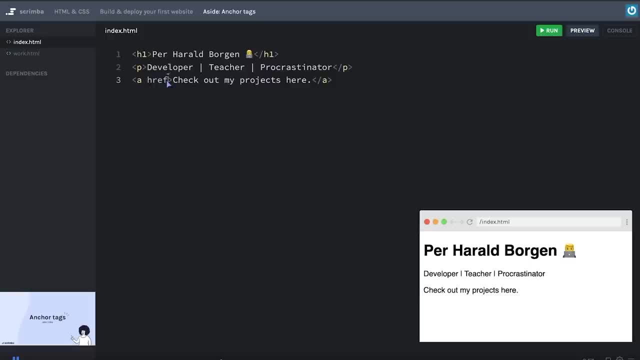 all this attribute does is decide where the link should point to. So if we do equal and then two quotes, we can inside the quotes simply write work dot html. If we now run this, you can see that renders as a link And when we click it, boom, we're taken to the work dot html. 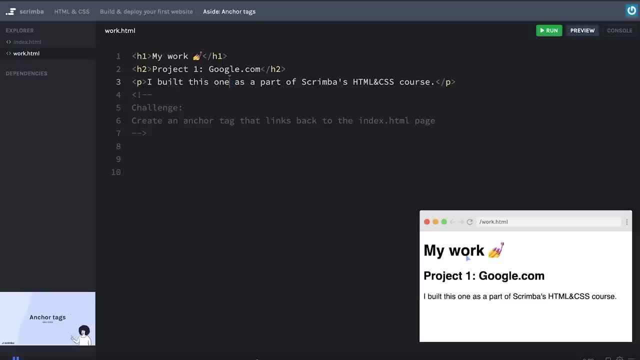 page Really nice. Now, another thing I want to show you with with anchor tags is that you can nest them inside of other tags and actually in line in a text block. So let's say that we want to link to googlecom from this site. then we'll create a paragraph. 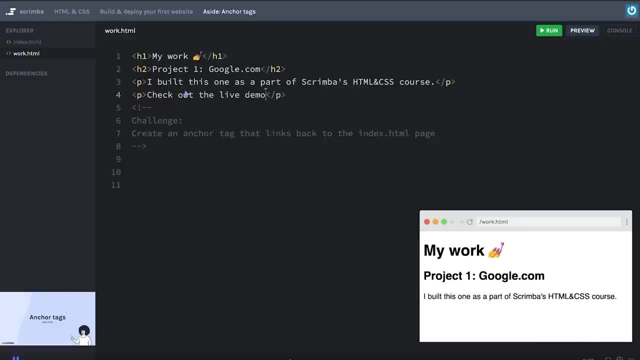 we can say something like check out the live demo here, And we only want the here word to be a clickable link. Well then, we'll simply wrap the anchor tag round here as well And we'll close it before we close the paragraph, And then we'll do the age ref paste in the URL to googlecom Now. 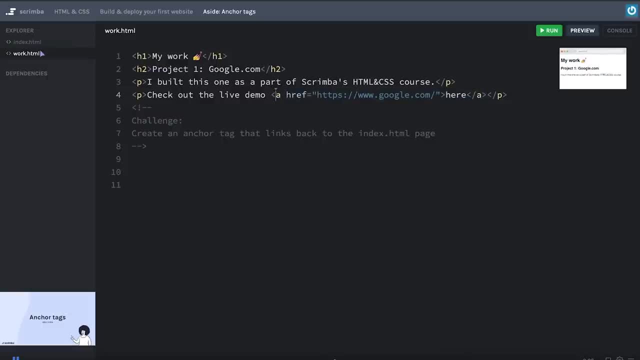 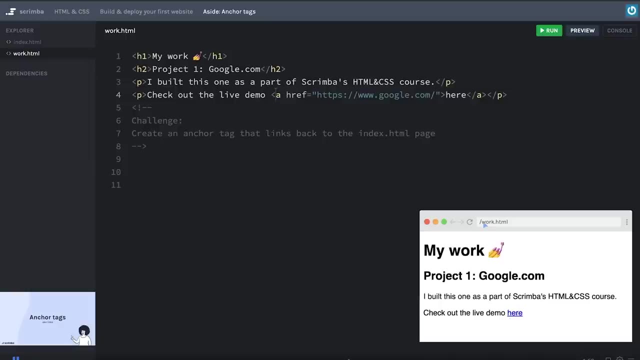 this is a link that points to an external website, not to any of our pages. So if we run this, you can see that the link is now only over the here word. However, if I click this link now, the scrim bot mini browser will try to head over. 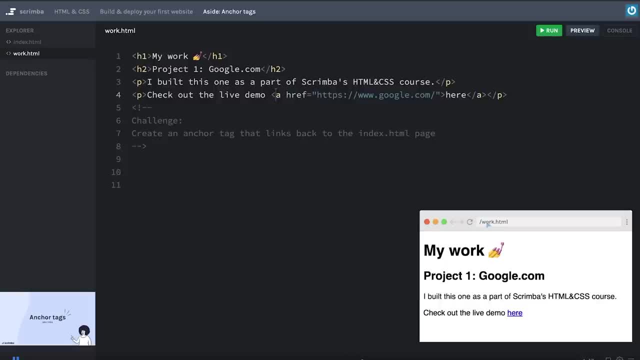 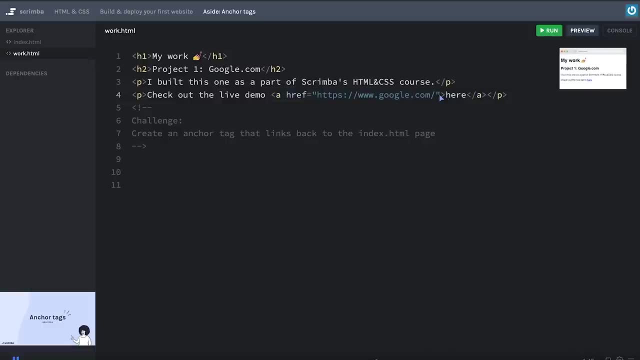 to googlecom, And we only allow the mini browser to render scrim projects at the moment, So that won't work. Instead, what I'm going to do is make this link open in a new tab, And the way we do that is three new attributes. So first, I'm just going to break this into a new line, just to 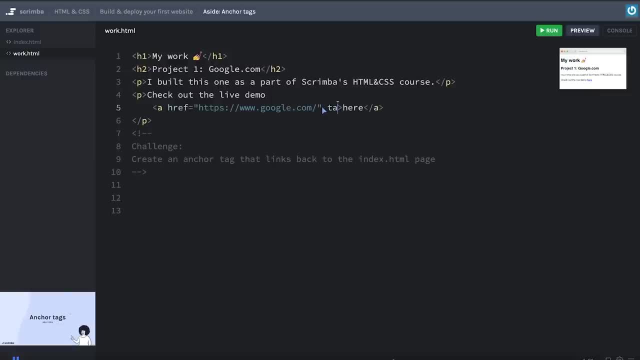 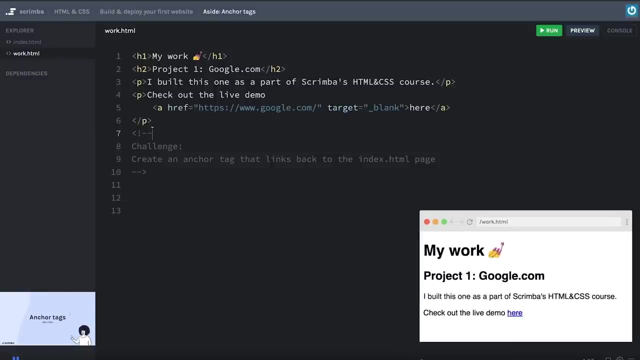 improve the readability a little bit. And then here I'm gonna write: target equals, underscore- blank. Now that is a cryptic way of saying that you want the link to open up in a new tab, I know, But if we now run this, if you click on this link, what you'll see is that in your main browser. 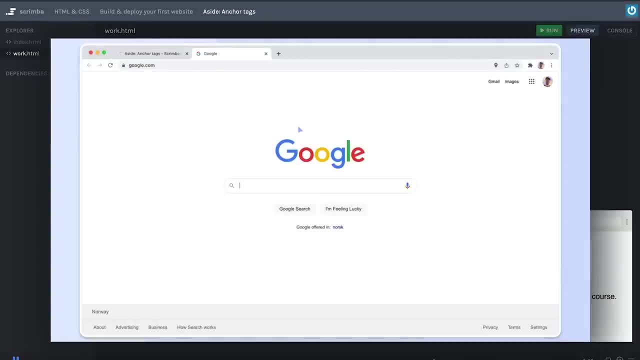 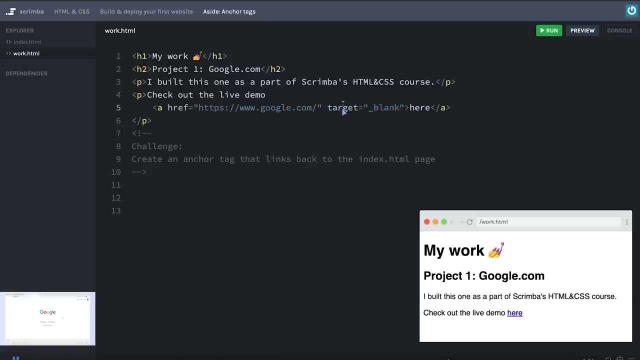 a new tab will be opened at the googlecom homepage, So I'm not going to go deeper into why it's called target equals underscore blank, But this is the way to do it. I of course wish that would have made a lot more sense to me, But this is how it is. you just have to accept it, Okay. 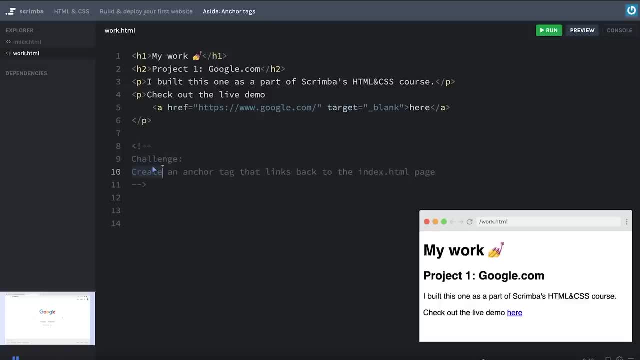 that was a lot of talking for me. Now it's time for a challenge. I want you to create an anchor tag that links back to the index dot html page, Because if a user ends up on this page, they also need a way to get back to the main page. So create that link here, however you want. 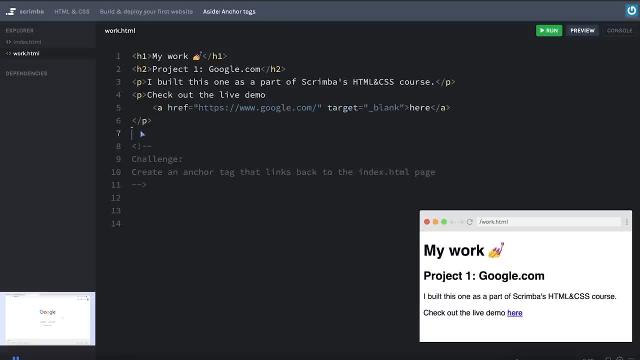 And then I will show you the solution when you return back to me. Okay, hopefully that went well. let's create this anchor tag. I'll wrap it inside of a paragraph, right turn to homepage And then I'll simply wrap the homepage word in an anchor tag, like: 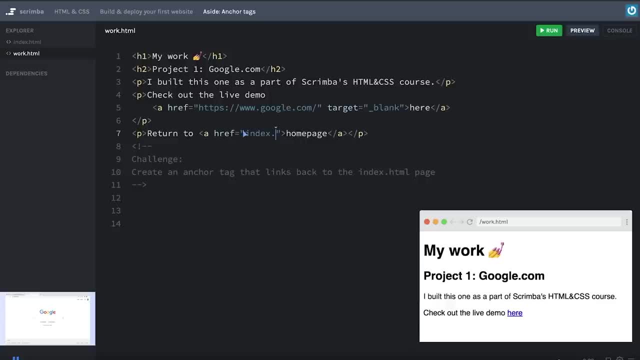 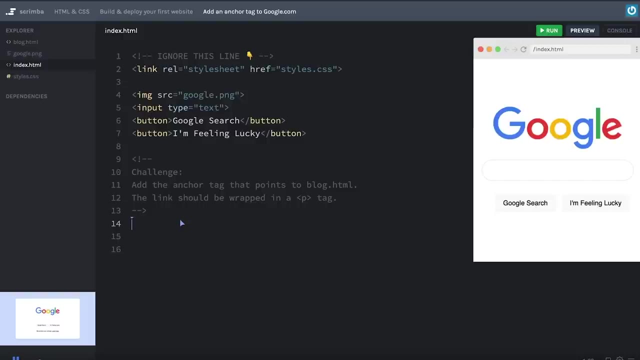 that And point that anchor tag to index dot html. If we run this, you can see return to homepage And if we click that, we are back at the homepage. Great job, Let's move on. Okay, we're back at our Google example here And now I want you to add a anchor tag to the page Because 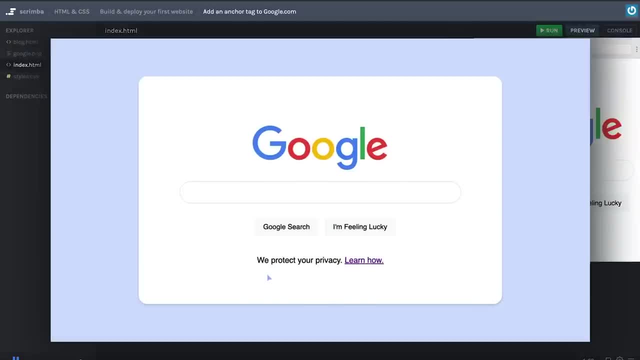 sometimes you'll see that Google adds a little text underneath the buttons, for example, something about privacy, like we protect your privacy, then with a learn how link that you can click on to read more about that. So that is exactly what I want you to do. I want you to add an anchor tag. 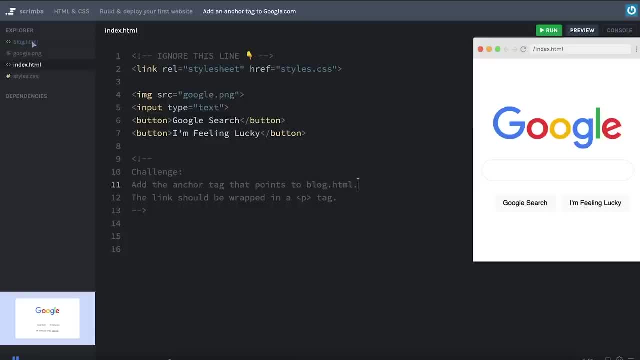 that point to blog dot html. As you can see, I've added a blog dot html file up here And I want you to wrap the link inside of a paragraph tag, And then I'm going to add an anchor tag that points to blog dot html. As you can see, I've added a blog dot html file up here and I want you to wrap the link inside of a paragraph tag. 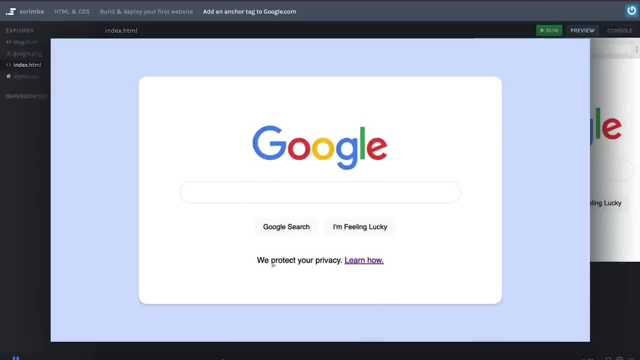 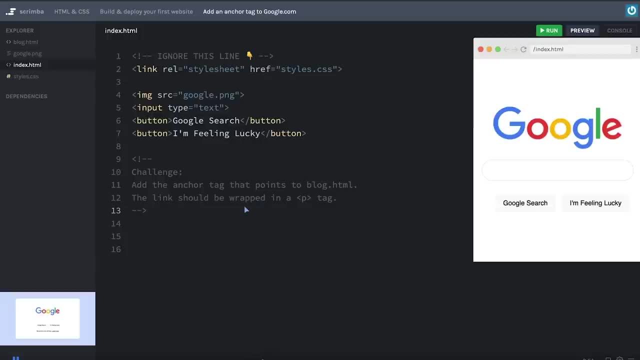 So, just as it is here, you can see it's an entire paragraph here, But the anchor tag is only wrapping the second sentence. So go ahead and do that right now. Okay, hopefully that went well. Let's do it. We'll start with the paragraph opening and closing tag. 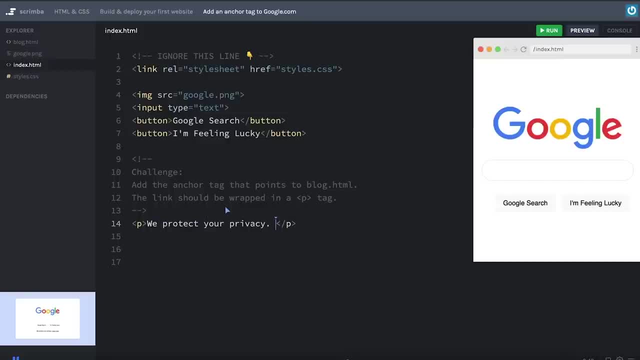 And then do we protect your privacy like that? Here we're going to add the anchor tag in line, So I'll do a open and close and do an href as well. point it to blog dot html And the text should be: learn how. 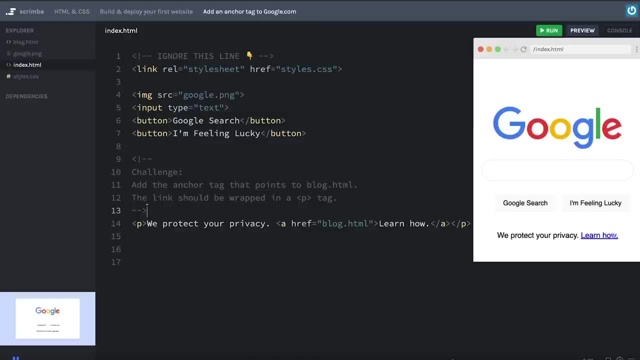 let's run this And boom, there we go. We have added a nice little link here. If we want to learn more about Google privacy, then we can click this link, But not much to see. here Turns out that privacy probably isn't as important for a company who makes money by showing ads to users. Anyway, 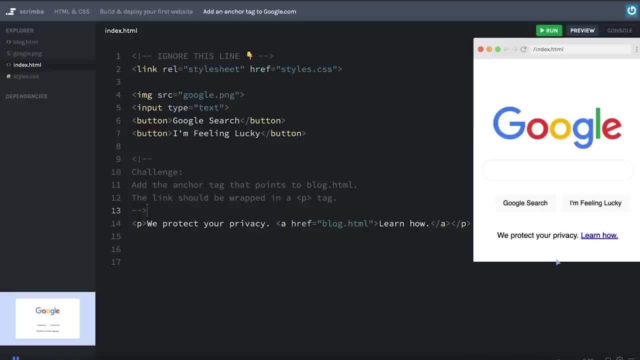 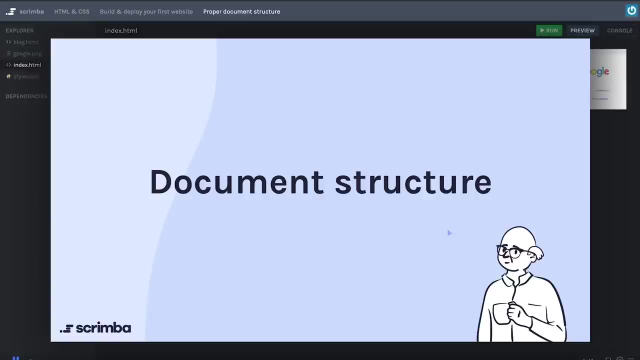 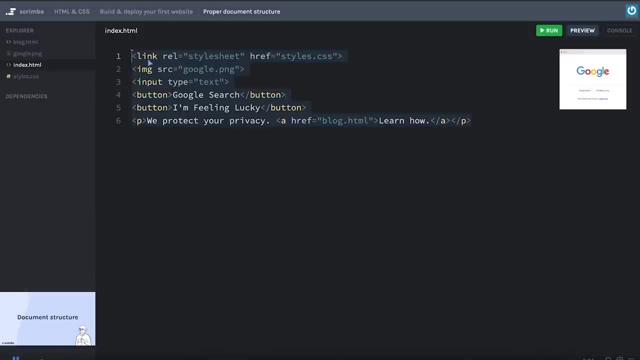 we can click on this link, Return back to Google, And there we are. Great job solving this challenge. Let's move on. Okay, now we're going to talk about how to structure HTML documents, Because the structure we have here isn't actually correct. It's a very simplified structure compared to how it should be. 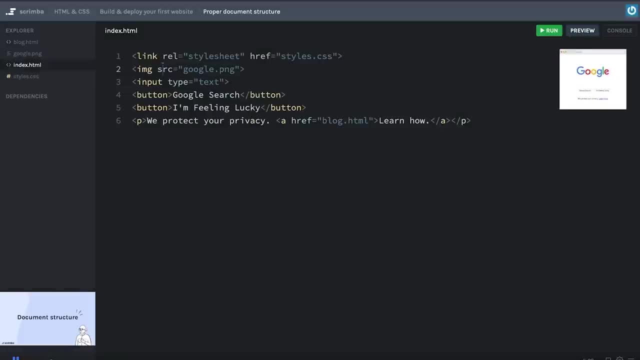 though it does work. So I didn't want to give you all of these theoretical, boring structure things up front. I wanted you to build stuff from the get go, without the added complexity of the HTML structure, As my philosophy is first make it work and then make it better. However, now we're 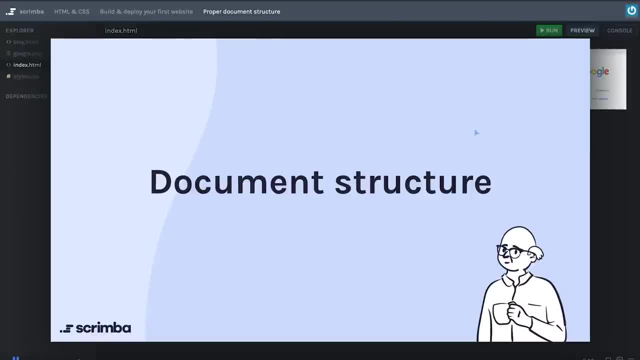 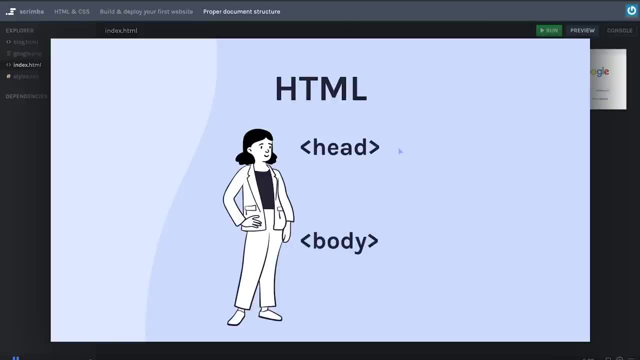 at the point where we should make it better. So let's have a look at how to structure HTML documents properly. And HTML is actually quite like us humans: it has a head and a body. And what you place inside of these elements? Well, in the body, that's where you place the tags, you see. 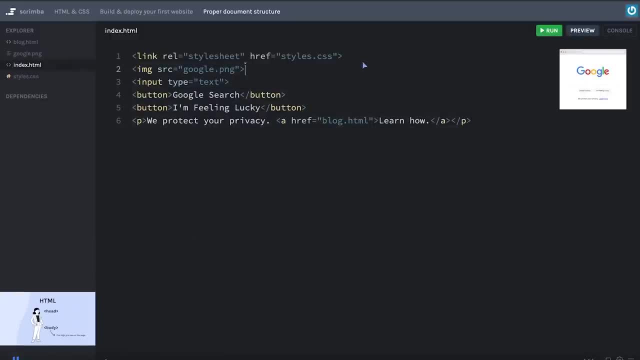 on the page, And that is these tags here, So our image, our input button paragraph and our anchor, because these are visible on the page. Now, of course, the CSS styling up here also results in a different layout, But the link tag in itself is not something that is rendered on the page, So it. 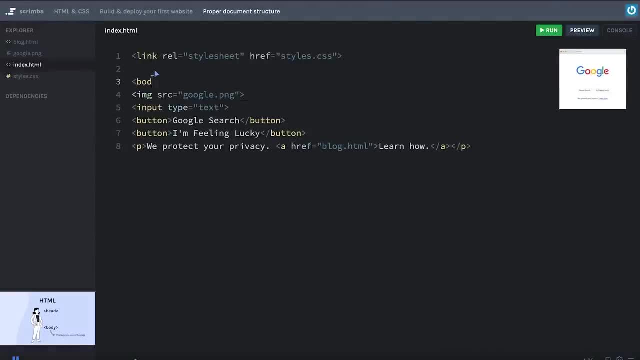 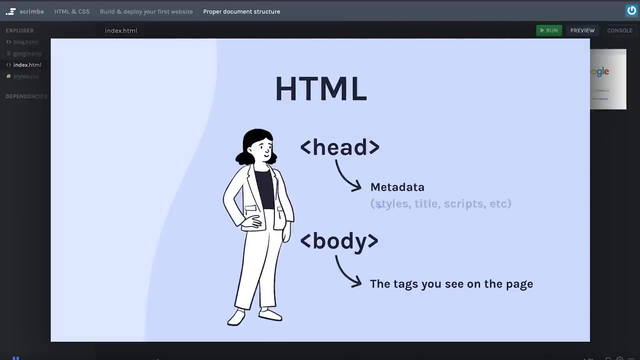 should not be in the body tag. So let's just add the body right here, Robbie, starting tag, and then the closing tag down here on line nine, and then we'll indent everything inside of the body like that. So, moving on to the head, that's where we add metadata. And what do I mean about that? Well, 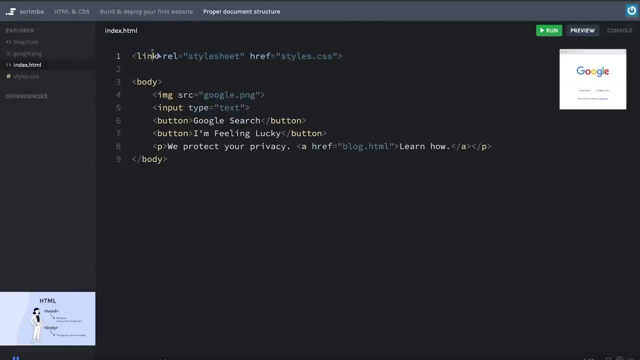 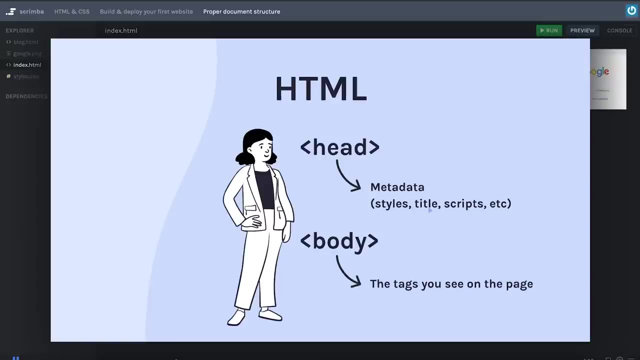 we can add the title tag to the head. So, for example, styles. so this link right here should be inside of the head. we'll do head and then close it off here, like that other things will have. in the head is the title tag. So let's have a look at what that is. If we navigate over to the 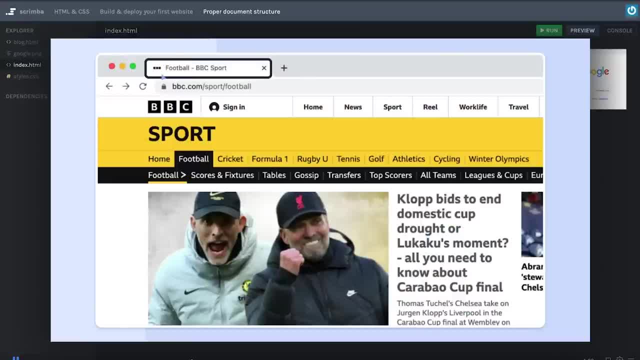 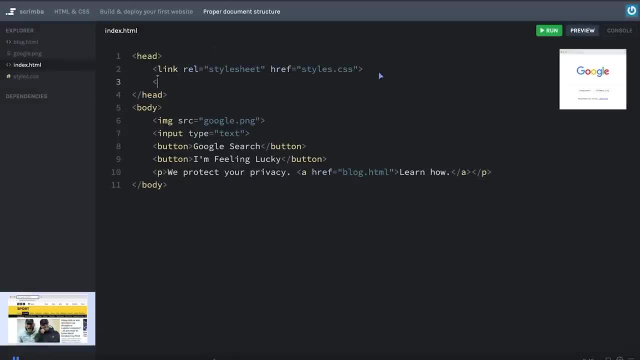 BBC football page and zoom in on the top, you can see up in the tab. it has a icon. it says football dash, BBC sport And all of this data. both the fav icon at the beginning here and this sentence is elements we place inside of the heads tag. So if we want to add a title text in a tab, 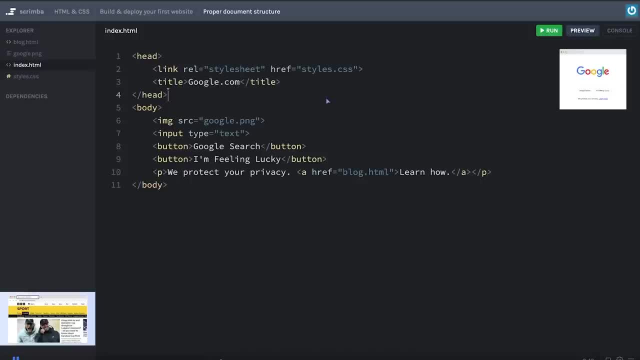 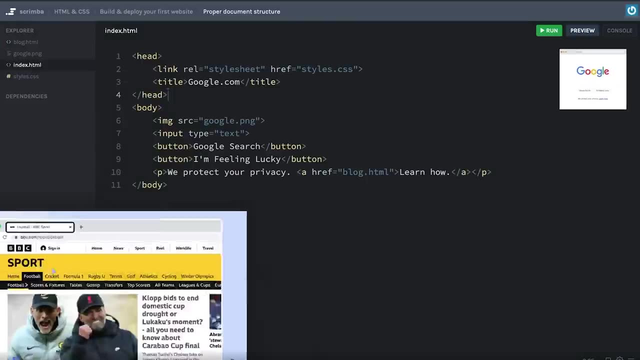 simply write the title And then, for example, googlecom would be natural to right here, though we haven't implemented tabs in the mini browser here on scrim bar, So you won't see that, But had we done that it would have looked like this load, of course, would have. 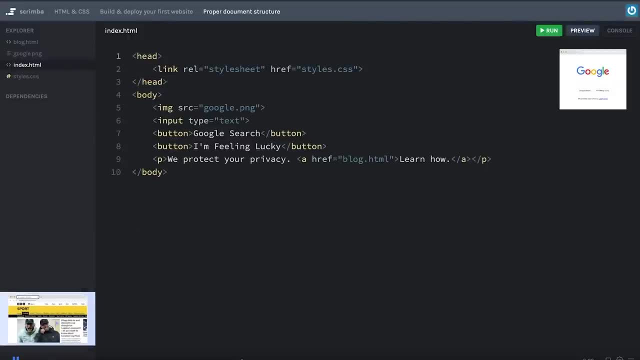 said googlecom instead, So we don't need that, So let's just remove it. Another thing that is controlled by tags inside of the heads tag is how articles are shown on social media. So if we zoom out a little bit here and click in on this article at the top here, and if 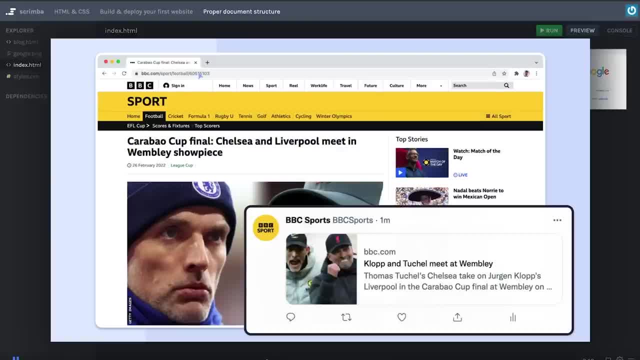 we now were to take this URL and share it, for example, on Twitter, what we then would get is a different heading on the Twitter card than what the article natively has, and also a different image than the main image on the article. So this is metadata, that is. 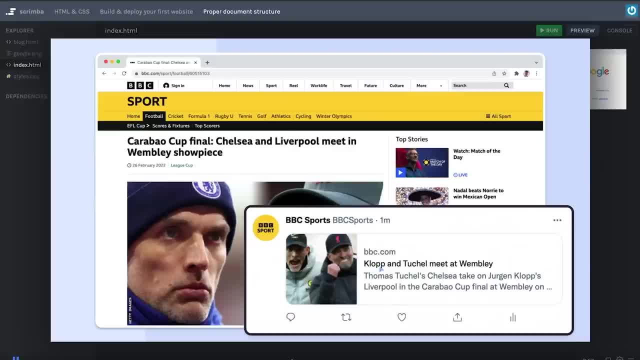 told Twitter that if this article is shared on Twitter, we want you to use this heading instead of the heading that is inside of the article, And also this image instead of the head of this image right here. So that was a lot about the head tag. we're not going. 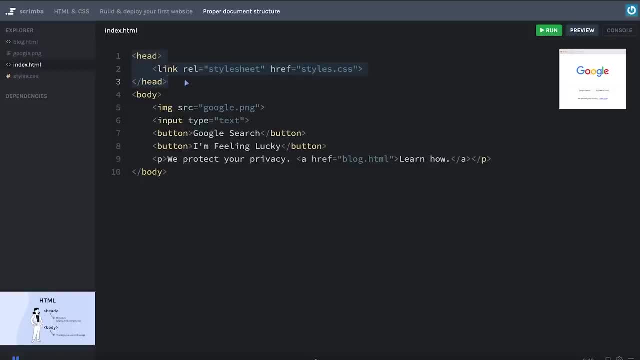 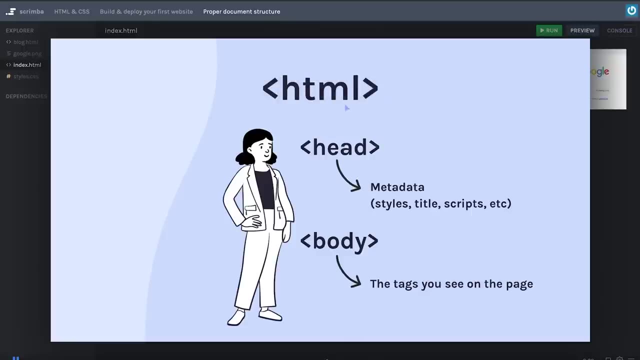 to use the head that much, But I wanted to give you an understanding about why it is important. Now there's one more HTML tag we need, And that is the HTML tag in itself, which should wrap all other HTML tags. So we need to up here at the very top right. 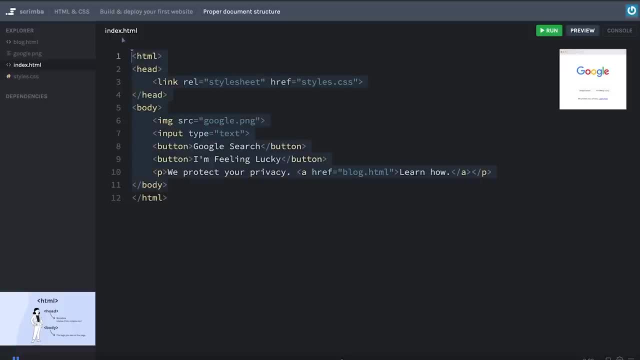 HTML and, at the very bottom, close it off And also then indent everything inside of it like that. Now, one more thing which is to me a little bit annoying that we need that is the doc type declaration, because you have to tell the browser that we're actually using HTML. 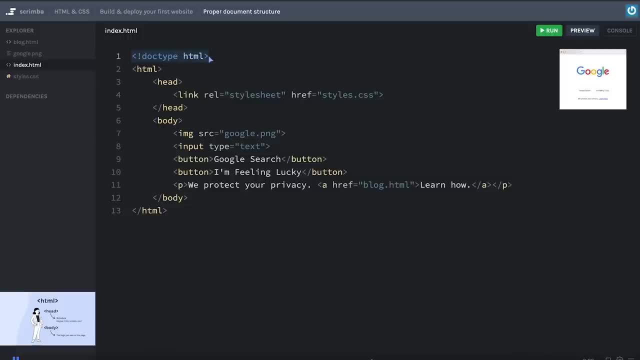 five and not HTML four. that's just a version of the HTML specification And that is done by this line up here. you can see it's blue and it starts with an exclamation mark. So it's actually not an HTML tag, it's just metadata for the browser. Because if you don't do this, 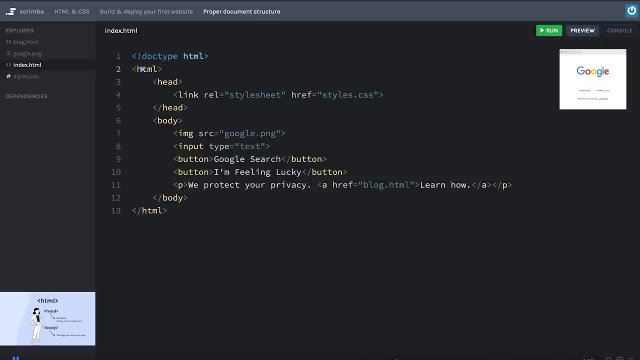 the browser will assume that you're not using HTML five, but an earlier version of HTML, and that might result in some quirks on the page. So in 99% of cases there will be no difference between adding this and not having it. So at times you'll probably see tutorials. 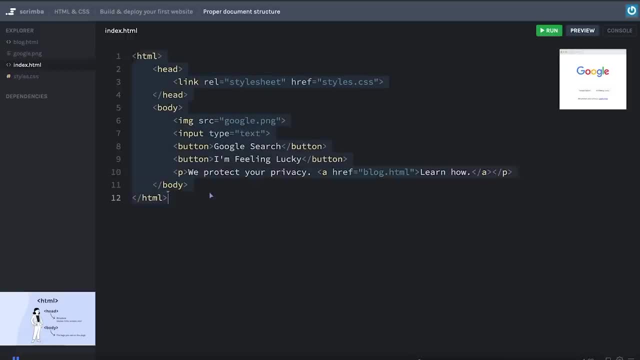 on scrim bar, where I've forgotten to add this because for the purposes of our example it won't make any difference. But if you have something that you want to deploy to the world and have in production, then you just have to accept that you need this sign up at the. 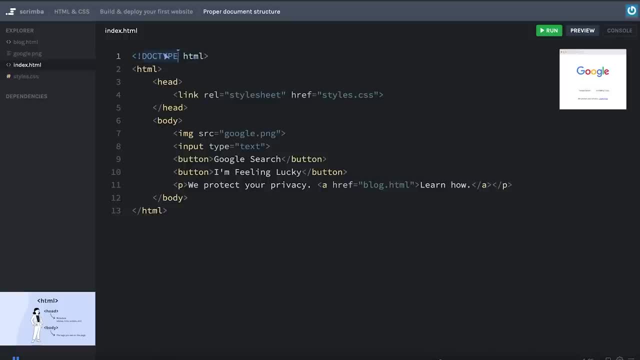 top, And sometimes you'll see people write it in capital letters as well. doesn't really matter, I prefer having lowercase letters. Okay, that was a lot of theory. it's time to get your hands on the keyboard, And, luckily though, we have a blog dot HTML file which doesn't have the proper HTML structure. So 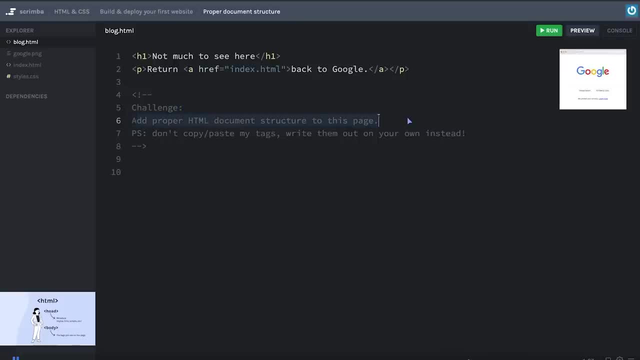 your challenge is simply to add the proper HTML document structure to this page, And I don't want you to copy paste my tags, but write them out on your own instead, so that you build up that ever so important muscle memory. go ahead and give this one a shot. 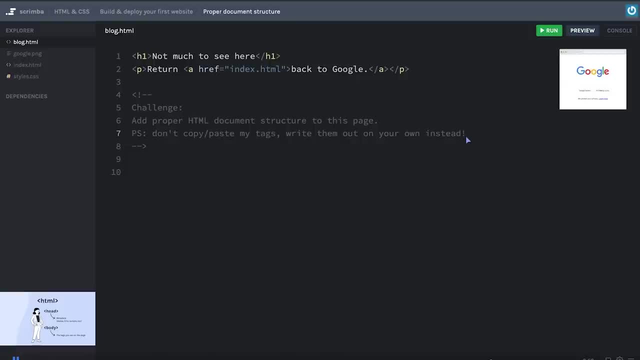 right now, And then I will, of course, do it myself when you return back to me. Okay, let's do this. I'll start with the body That should wrap our visible elements on the page like that. Then I'll do the head, though we haven't linked to the styles on. 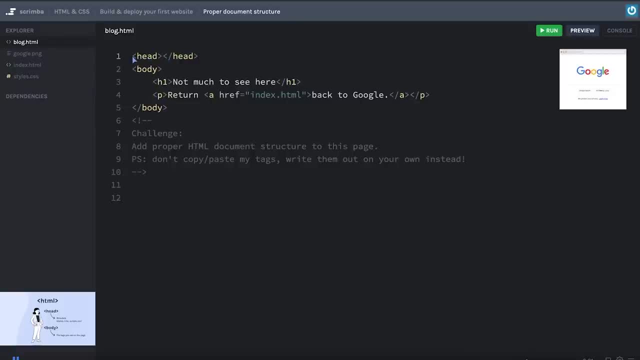 this page. So the head will actually just be empty like this. So I'll keep it on one line moving on. It is the HTML document and that should wrap everything. So I'll do like that And at the very end I'll add the doc type, HTML, to tell me what I need. So you can. 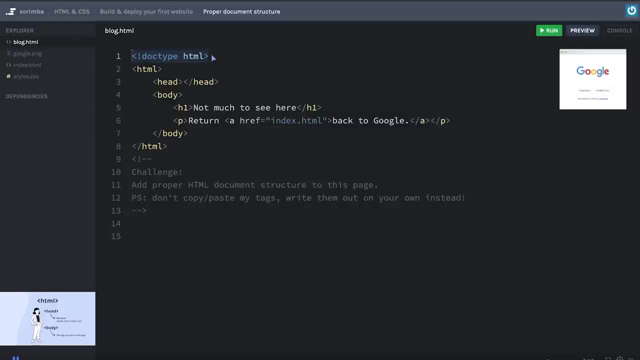 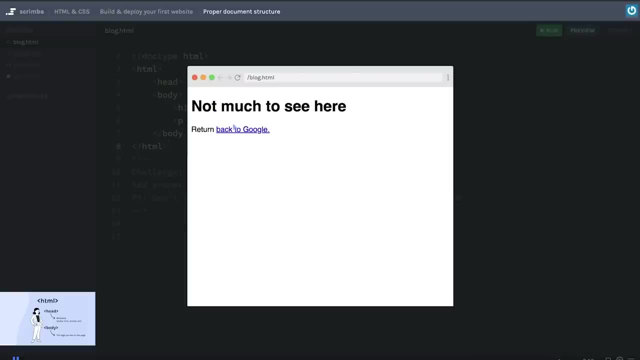 the browser that we are working with HTML5 and not HTML4. So if we now navigate over to the bloghtml site, you can see that nothing has seemingly changed, And as goes for the main page itself. the structure we've added doesn't result in any visible change. we just 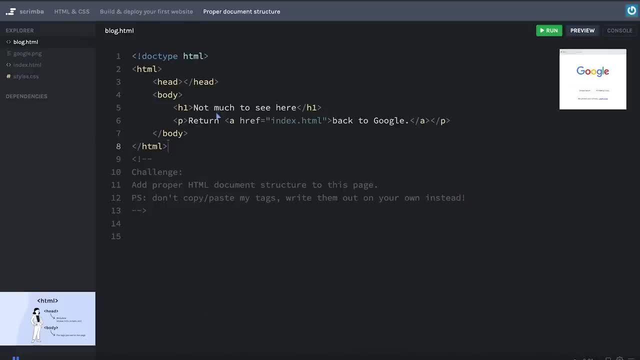 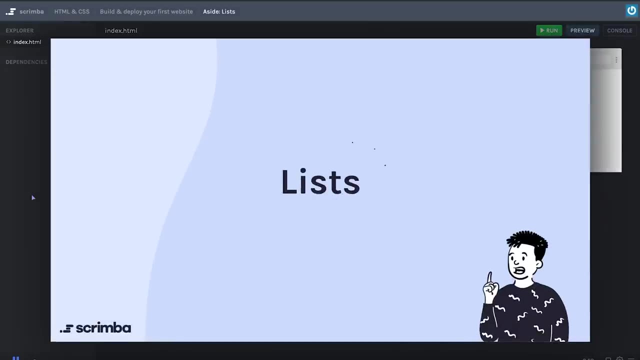 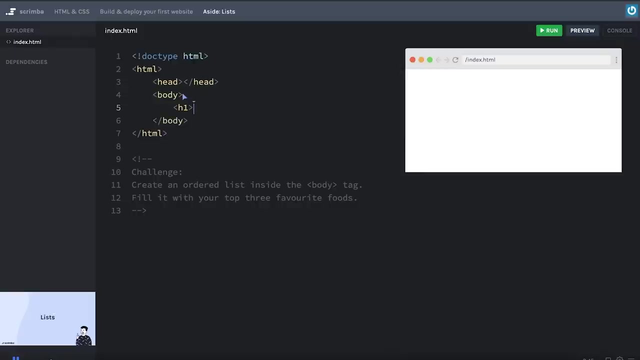 have a more correct underlying code file to work with. Great job, let's move on. Now you're going to learn about lists, Because let's say that you, for example, want to create some kind of a tribute site. it could be for whatever, for example, I don't know- the Beijing Winter. 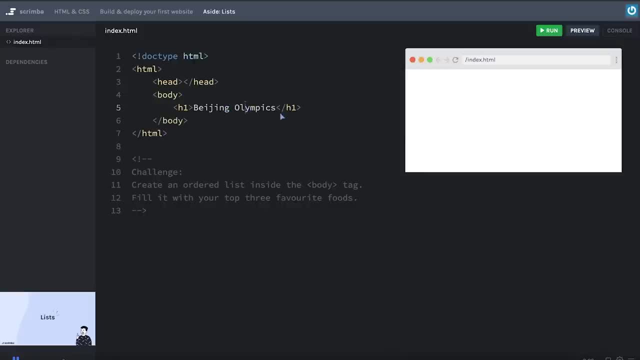 Olympics. If that's one of your interests, you might want to create a tribute site where you list out the top nations who competed, or something like that, And if so you would have to use an HTML list. So let's first just figure out which nation actually won the most. 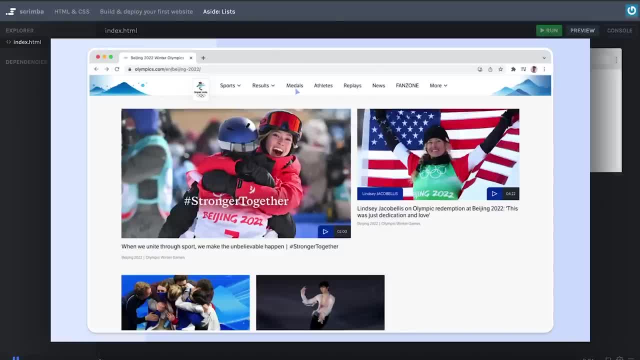 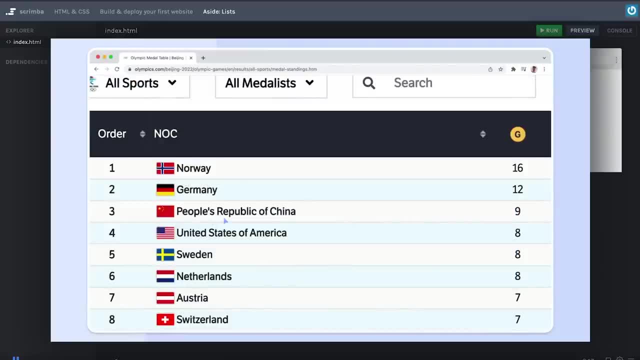 medals in the Beijing Olympics. So I'm going to click on the medals tab Here on the Olympic site And here we got it, and zoom in a little bit and oh wow, it turns out that actually Norway, my country, completely obliterated the other countries. 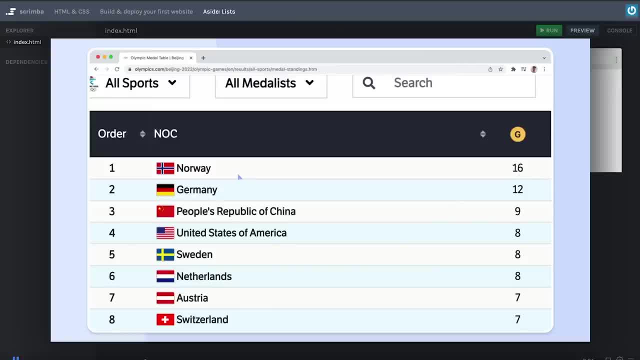 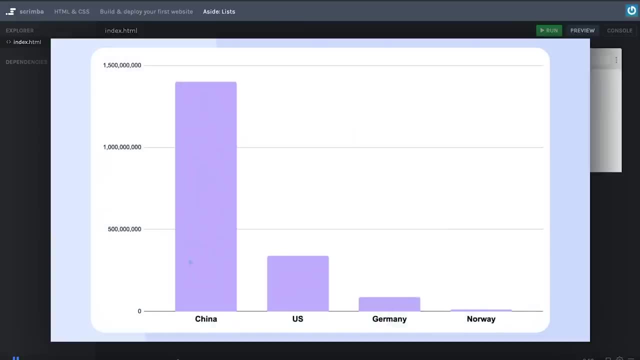 with 16 gold medals over other nations like Germany, China and the US. That is really astonishing, especially considering the fact that the size of the Norwegian population is this compared to the other nations. here I mean: way to go, Norway, we gotta create. 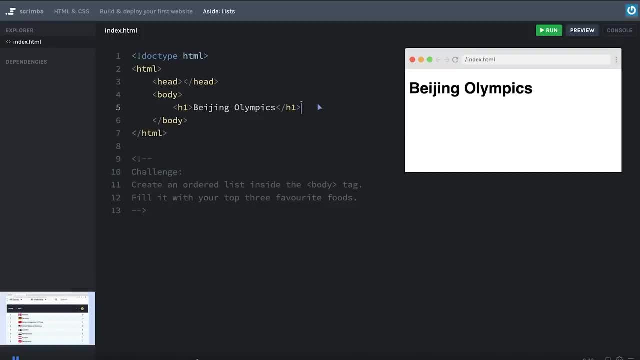 this list in HTML. Okay, so how do we do that? Well, we have to use two different tags: one tag for wrapping the entire list and another tag for each list item. The wrapper tag is one called ol, that's short for ordered list. And then, inside of the ordered list, we place: 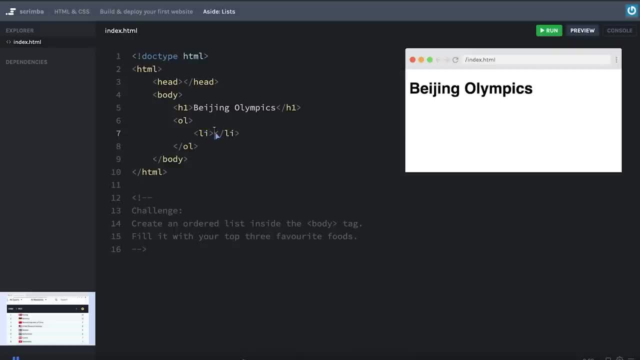 the list items, The li tags. When we do this and write Norway here, render this, you can see that the browser gives us a number, as it is the first item in the list and also indented a little bit from the left hand side, So adding another one here. it then gets the number two and 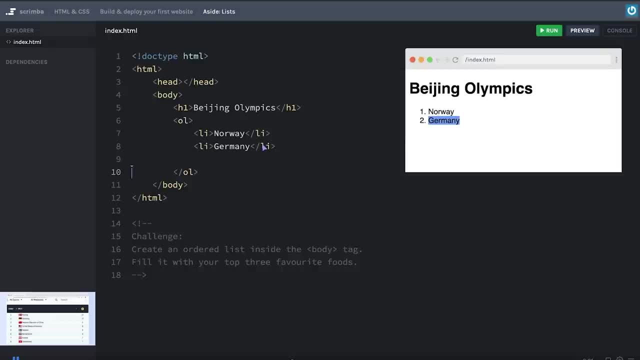 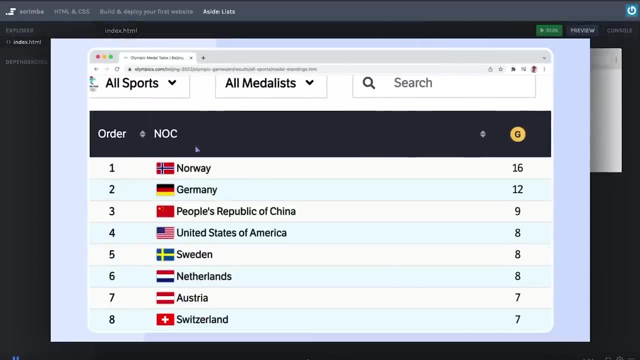 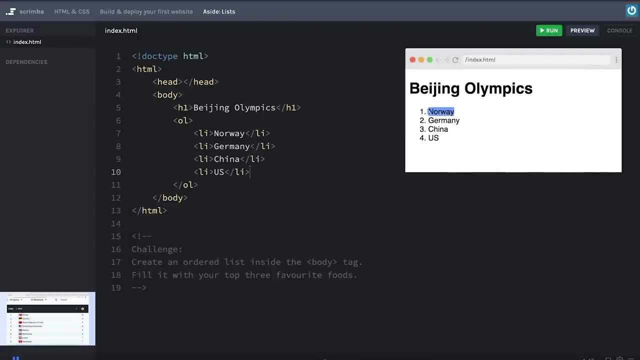 is stacked below the first one, So let's add the final ones. Like that looking pretty good. And now we have a list, just like on the Olympic site. Now, if we want it to be a little bit more diplomatic here and not brag too much about this insane victory by Norway, we could 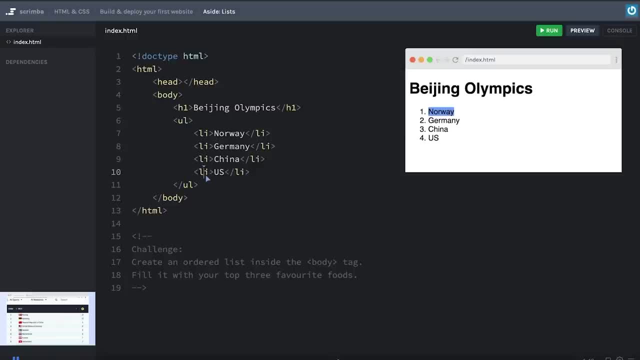 change this ol to a ul, That is, an unordered list, And, as you can see, then the numbers are replaced with dots. And now you might ask yourself: well, why do we need these unordered lists? they look like kind of boring elements you just use in Word documents or something. 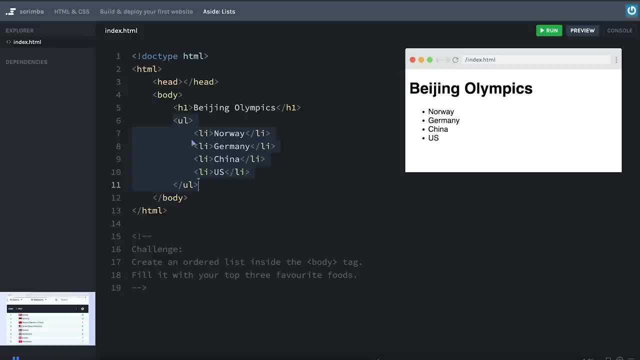 like that. Well, once you learn about CSS, you're going to be able to do a lot of things here, So let's start with CSS. So let's start with CSS. Let's start with CSS. Let's start with CSS. You'll be able to style your list however you want and thus make it much more usable. 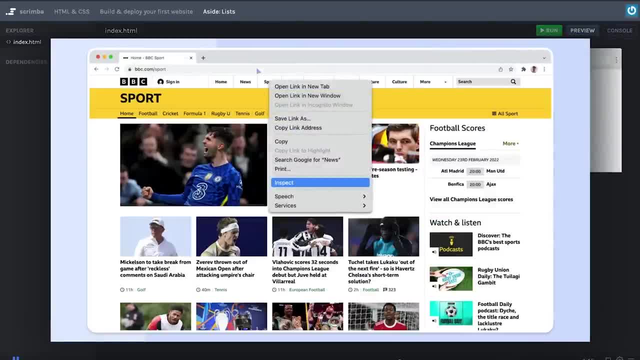 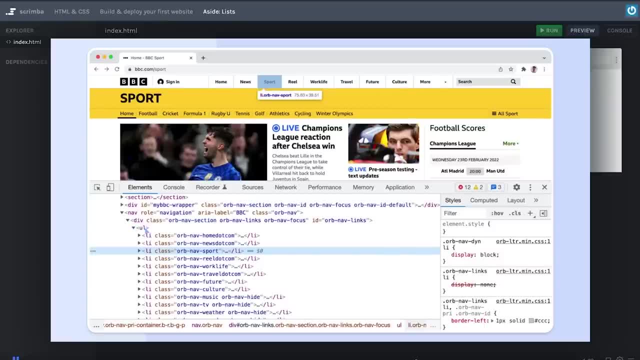 If we, for example, head over to BBC sports here and right click on the navbar here and click Inspect, then we'll see that actually this entire navbar is an unordered list item, with each of the categories being its own list items. So lists are all over the web. 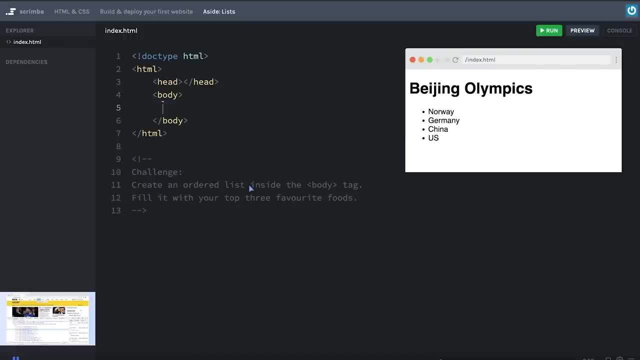 and important to learn. Okay, now I'm going to remove all of this and give you a quick challenge, Because I want you to create an ordered list inside of the body tag and then fill it with your top three favorite foods. So go ahead and give this a shot right now. 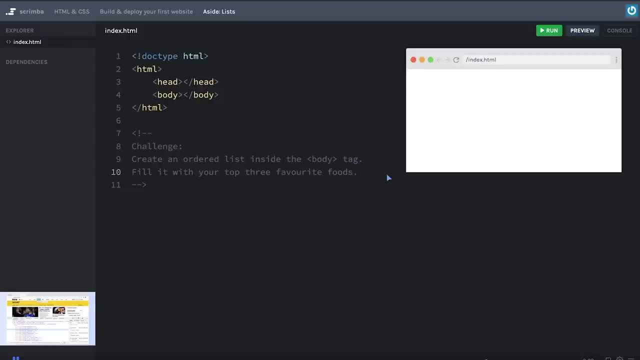 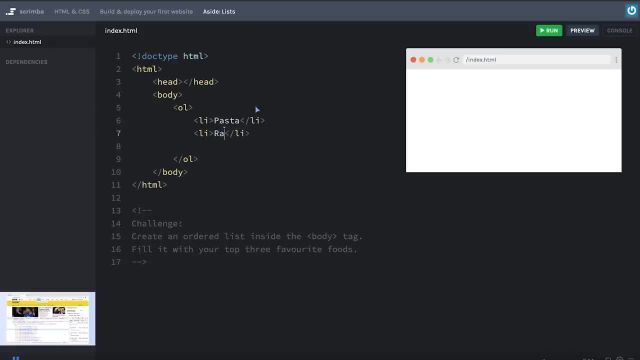 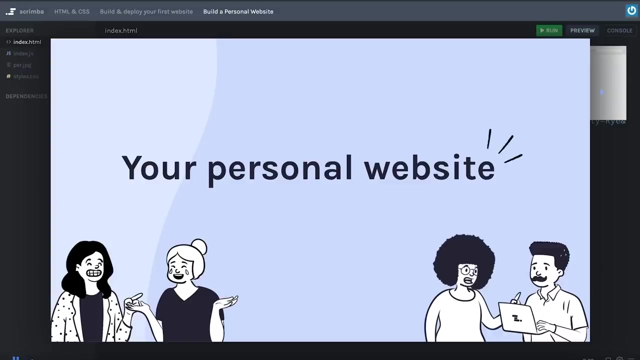 update. Now I could just update my host's list item, So there we have it rendered out on the page. Really good job learning about HTML lists. Let's keep up the pace and move on with the course. Okay, now you have arrived to the main project of this section. you are going to build a website. 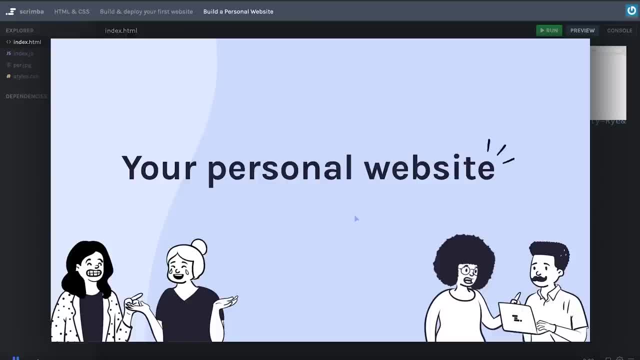 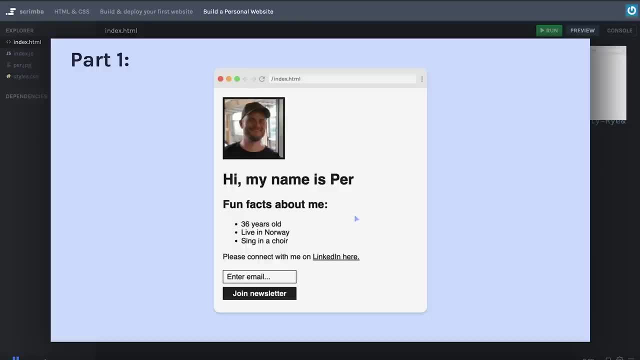 about yourself, And we're going to personalize it as well, Plus ploy to the world so that anyone around the world can visit this website. it is going to be so much fun. And here is the website itself. As you can see, it's pretty simple, with hardly any styling by default, just a little bit. 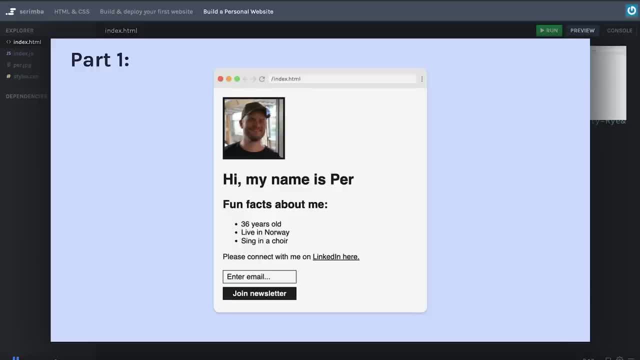 on the button and the input field here, as with the border around this image And building this lightly styled design is the first part, part one of the challenge, And then in part two of the challenge, we are going to go crazy on the styling, with just a few parameters that you are to tweak. 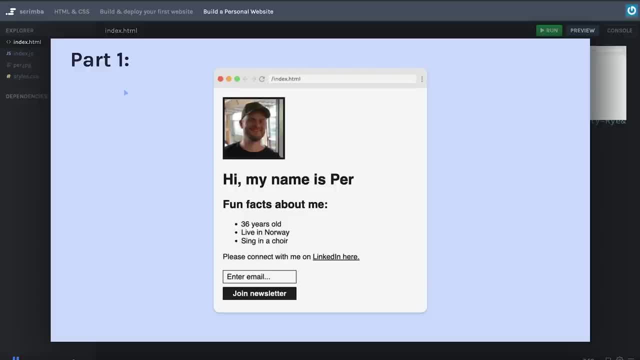 and it's going to look so cool. But let's not get ahead of ourselves here. Let's first just run through what kind of tags you need in order to build this Website. So, first off, there is an image tag, And the image you should use should be added to the. 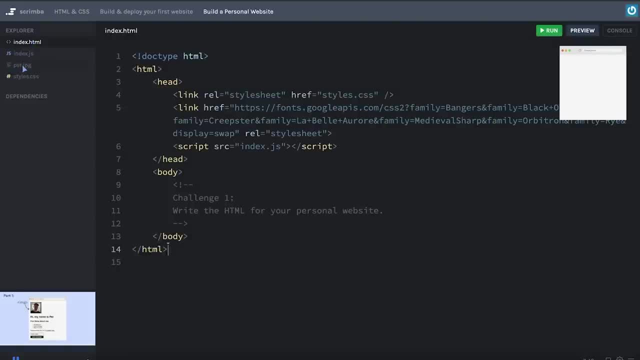 file system on the left hand side. here, As you can see, there is a pair dot jpg image here, And the way to add an image to this file system is simply by drag and dropping it over this section Next up. there's an h1 here as well with the title. Of course, you should write your own name, not my. 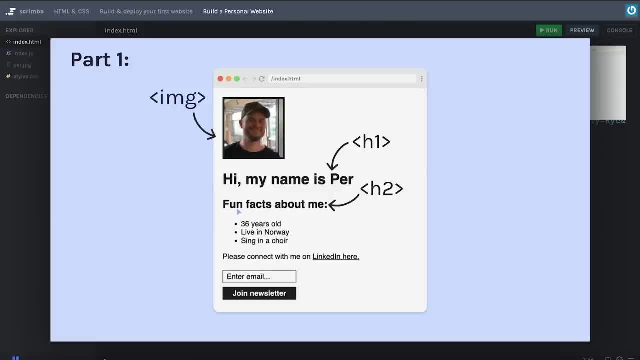 name, And then there's an h2 heading, As we need some fun facts about you. The fun facts itself are built using an unordered list Plus list items inside of the URL element, And then there is a paragraph with a link nested inside of it that should go to your LinkedIn profile. So the point here obviously is to replace. 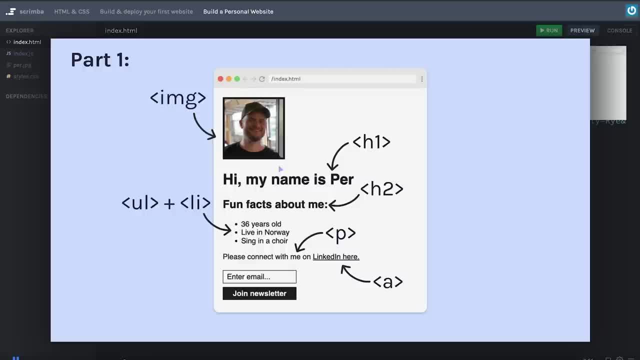 all of this information with fun facts about you, with your name, with your image, your LinkedIn profile, so that, when you share this with the scrimba community, other people will be able to get to know you better. And then, finally, we have an input field here and a button that won't really. 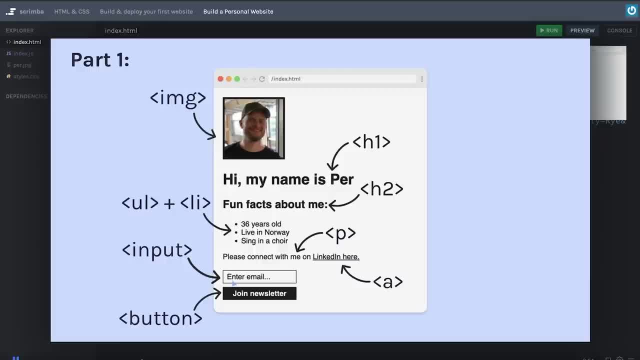 do anything, because we're not hooking this up With a real newsletter. we are just pretending that you have a newsletter that people can sign up to. So once you've done this, you've completed part one of the challenge And you've also filled. 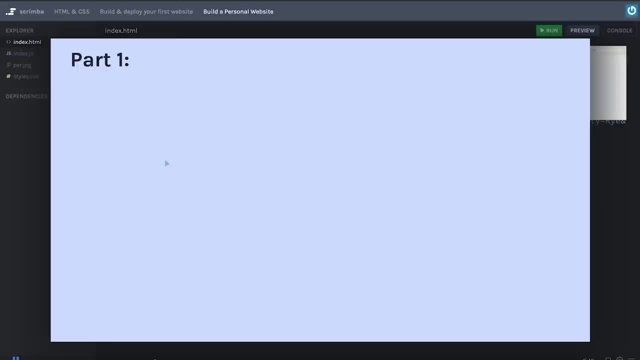 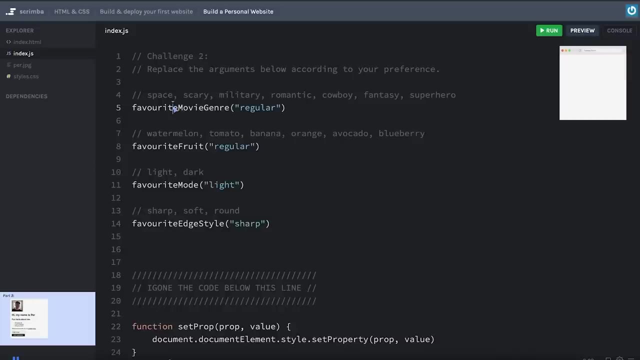 up this body element here with HTML tags. Next you'll move on to part two of the challenge. What you'll do there is take your existing design and modify it. So if we head over to the index dot JavaScript file, you can see that there are a bunch of so called JavaScript functions which 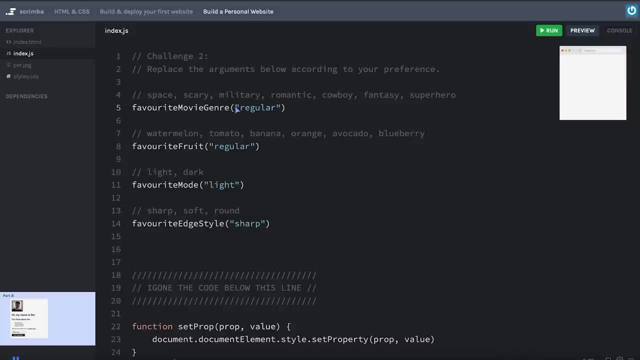 probably look really scary at the moment, But if you go to the index dot JavaScript file, you can see that there are a bunch of so called JavaScript functions which probably look really scary at the moment. point. But don't worry, the only thing you're going to do here is take the word that you see. 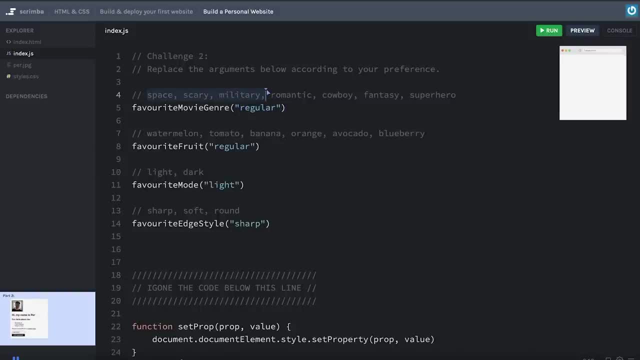 inside of the quotes right here and replace them with one of the words that are commented out in the line above, Because this will give you the opportunity to change the styling on the page according to what word you change this argument to. So what you're to do here is look at the name. 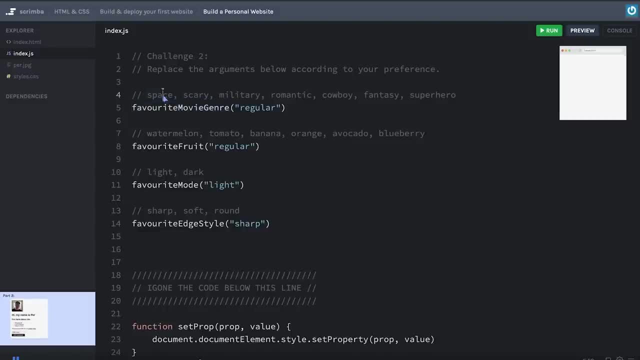 of this function. It says favorite movie genre. And what is that? Do you like space movies, scary movies, military movies, romantic movies, cowboy movies and so on? And then just take your preference and change it like this: So if you choose cowboy, for example, what then will happen? 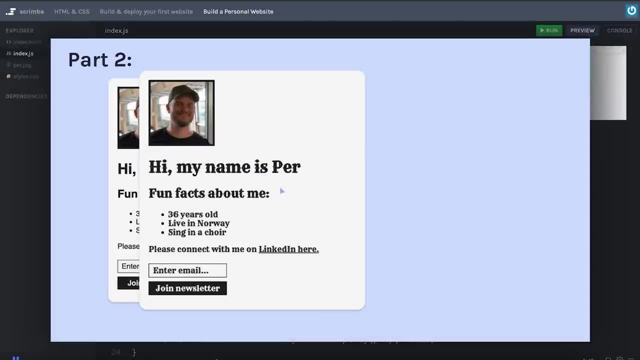 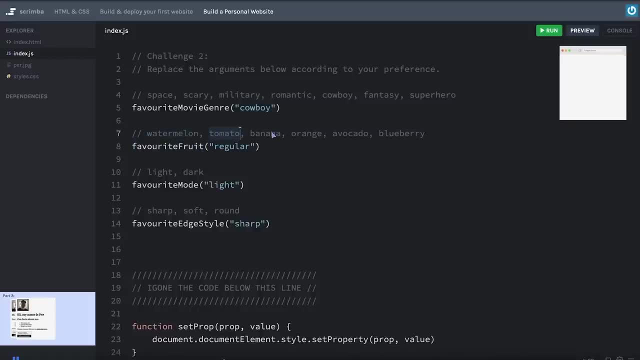 is that the font on the website suddenly became like a western movie. That's pretty cool. And moving on, here, you are to answer. what is your favorite fruit? Is it watermelon, tomato, banana? If it, for example, is banana, 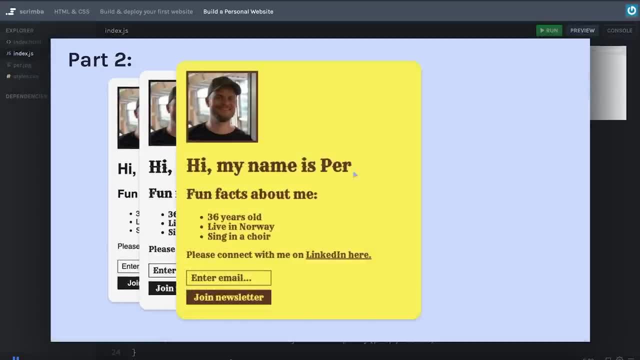 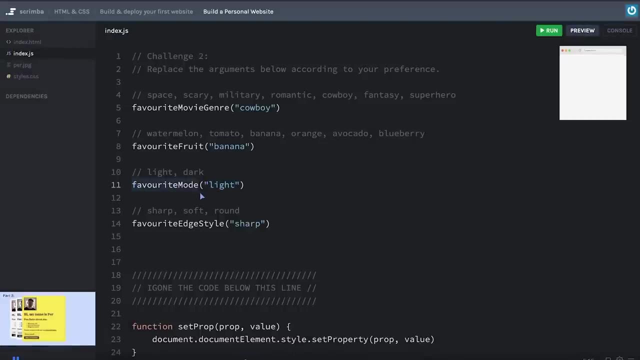 then you should replace regular with banana. And what will then happen? you run the code. suddenly your page is banana colored. Really nice. Now you are a cowboy banana. That's pretty cool. Finally, there's two more parameters you can tweak. First tell me it's your favorite mode. 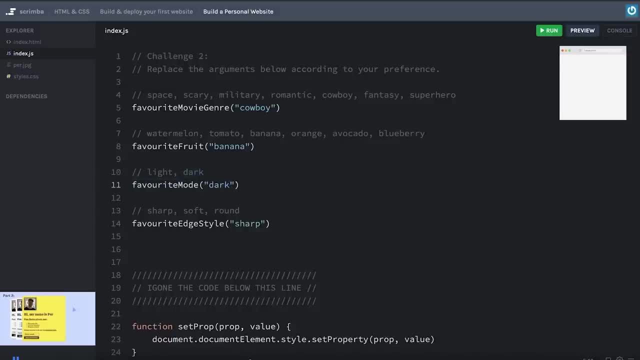 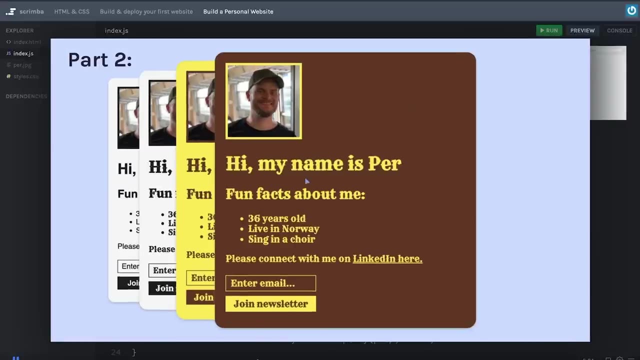 on your computer: light mode or dark mode. If you choose dark and run the code again, then you can see the colors have flipped And now it is primarily dark, with the brown background and the light yellow color, as opposed to how it was previously with the yellow background and 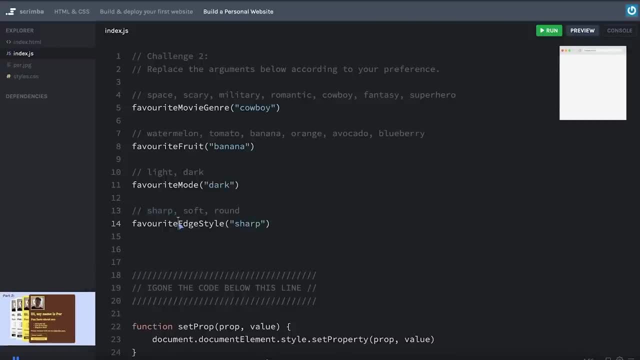 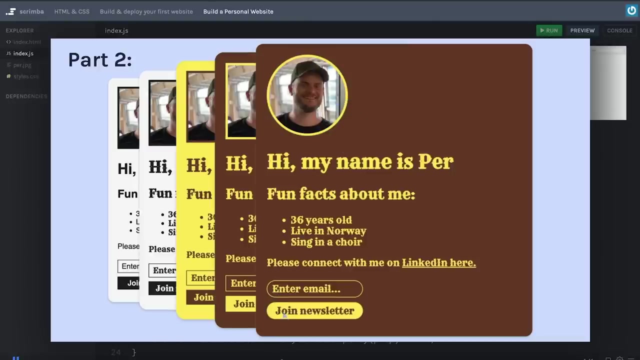 brown text color And then at the very end, you are to choose what kind of style you like your edges to be: sharp, soft or round. Let's say you like round, well then, you'll simply replace sharp with round, And there we go. We have a nice round layout where the image and the input and button 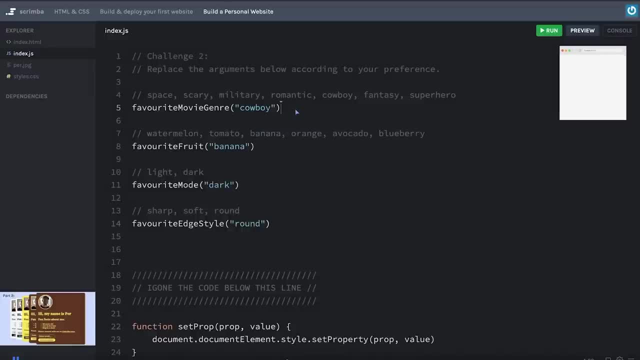 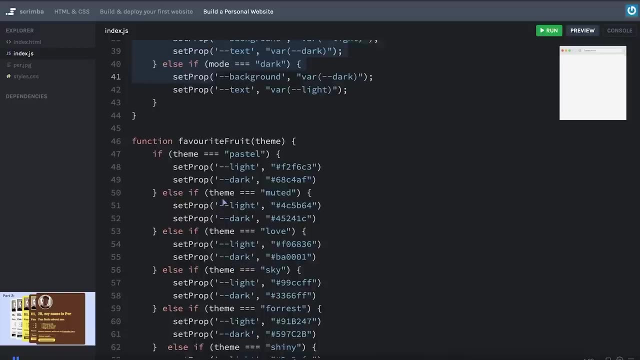 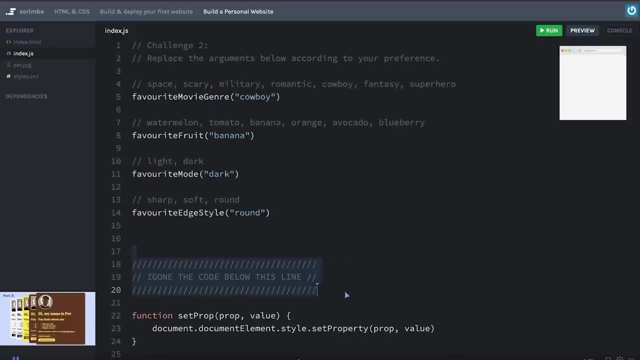 j s file and change the layout accordingly, though you should ignore everything below this line. don't even try to understand it. It's far outside the scope of this course, And you're going to learn JavaScript later in the front end developer path anyway, So it's nothing for you to. 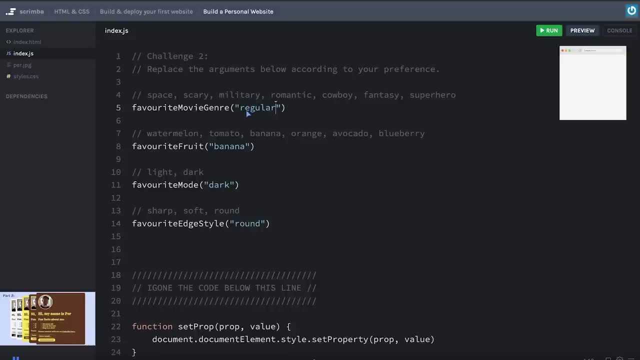 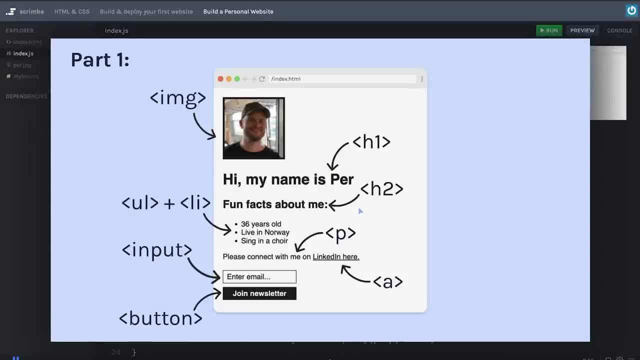 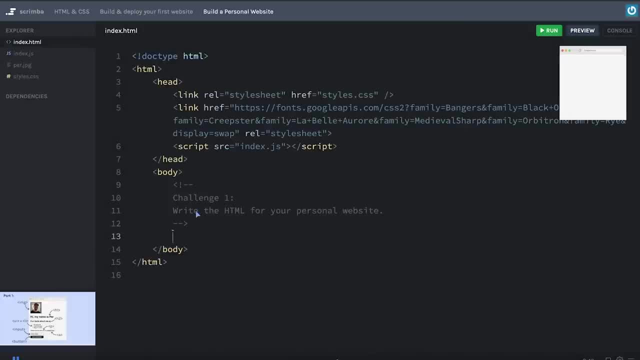 images will be there. I'm already opening the file. we wanna add some details to it. the file rule on it right here. as it now is your turn to build this layout, personalize it with the JavaScript functions so that you have your very own, completely unique website. So go ahead and do this right. 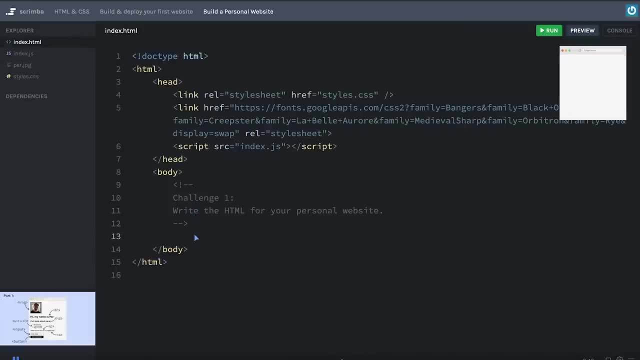 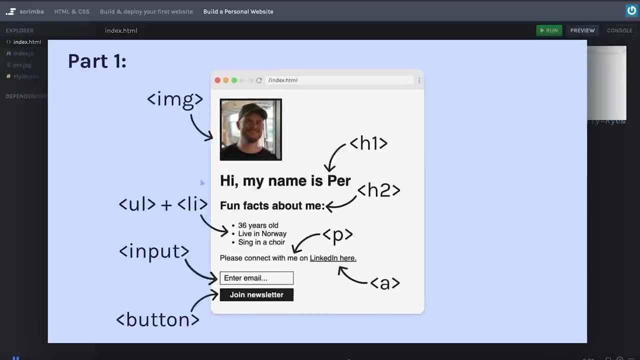 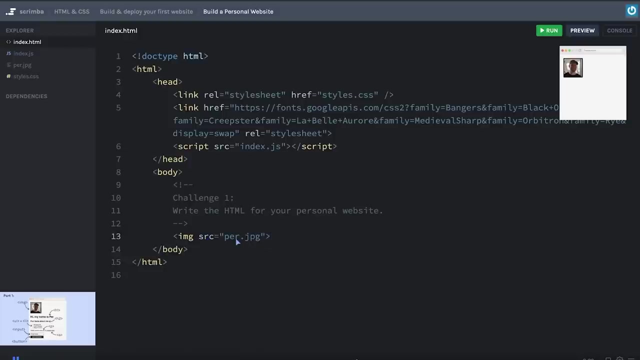 now, And then I will see you when you return back to me. Okay, hopefully that went well. Let's now do this together. First we need the image tag, So I'm gonna do IMG. The source is the pierrejpg which I'd already added. Yes, 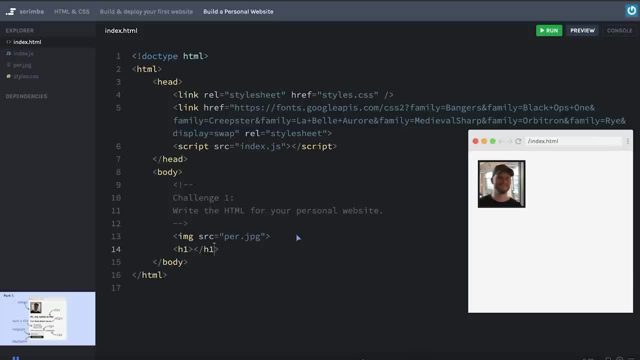 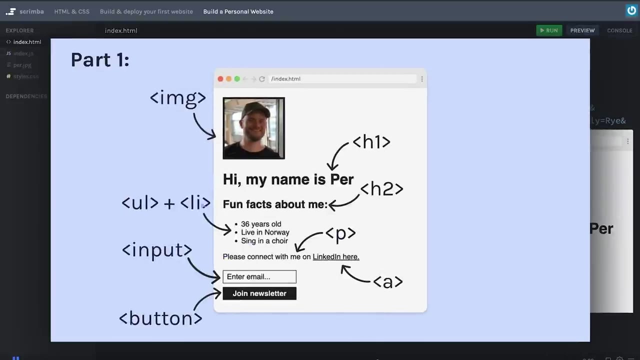 there we can see it is rendering properly. Next up there is an h1.. I- my name is pear, like that. Very good. Moving on, we have the h2.. Fun facts about me, like that. And then there's the unordered list and the list items. 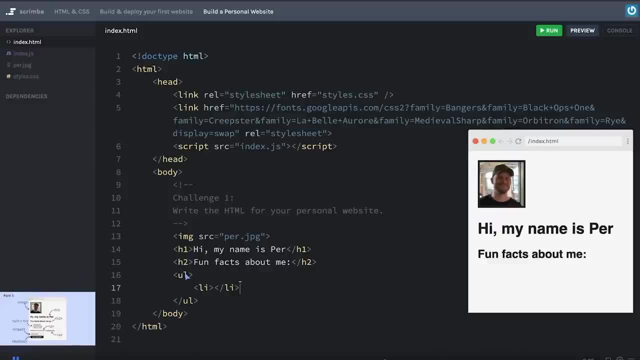 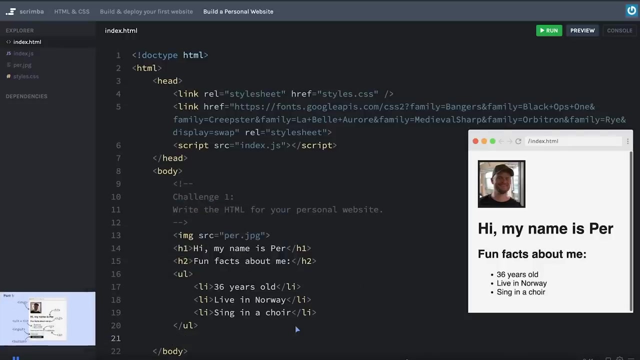 So I'll do UL, close that UL, because the list items need to be inside of the URL And the first one is 36 years old. I'm gonna copy this one like that. And I live in Norway And I sing in a choir And there we go, Looking pretty good. Next up, there is the paragraph with: 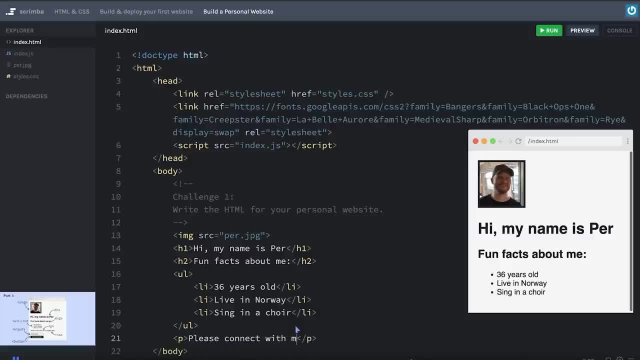 the inline anchor tag. Here's the paragraph Connect with me On LinkedIn, like that. Oops, it should take me on LinkedIn here. and then we are to wrap LinkedIn here into an href Like that, And then I'm going to paste in the URL to my LinkedIn. 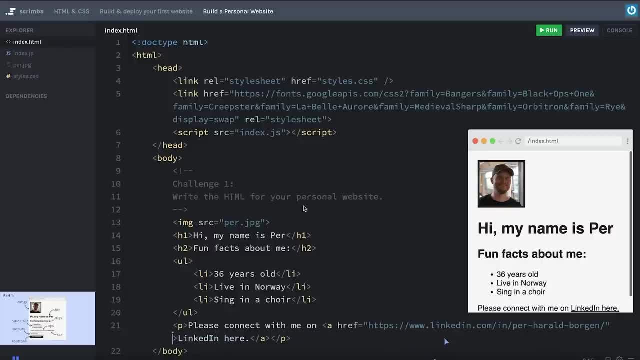 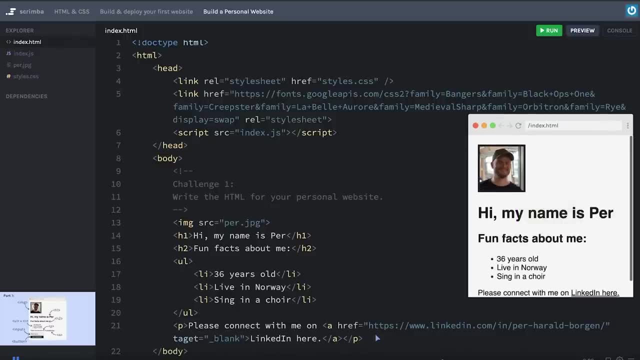 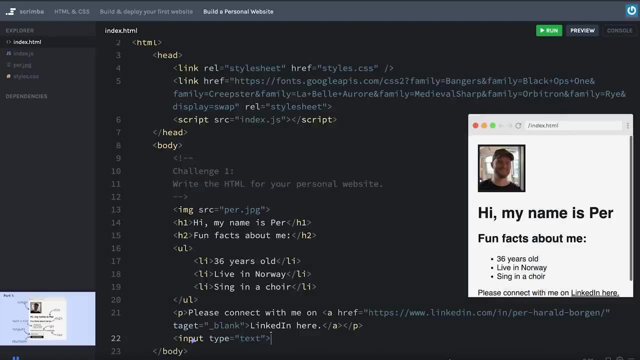 right here And if you actually want to connect with me on LinkedIn, feel free to click on this link. as soon as I've added the target, equals underscore blank, so that opens up a new tab. Okay, finally, we we need to add the input and the button. Input type text like that And button. 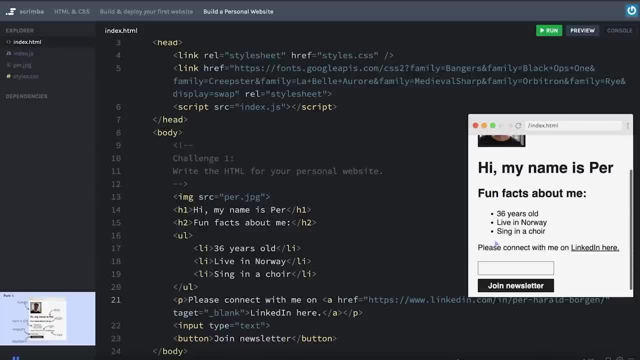 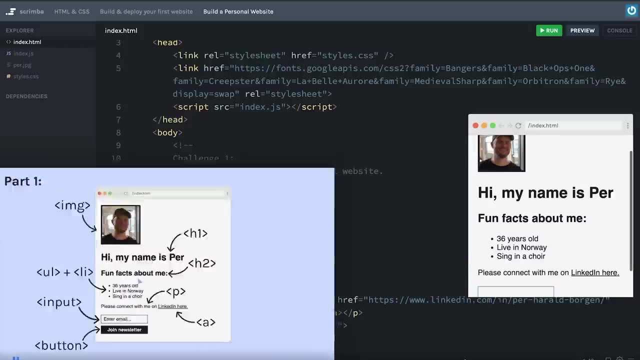 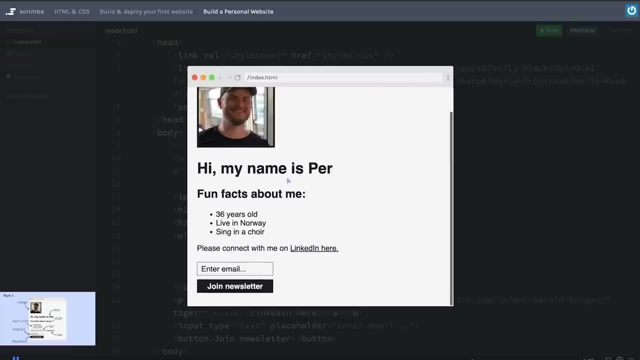 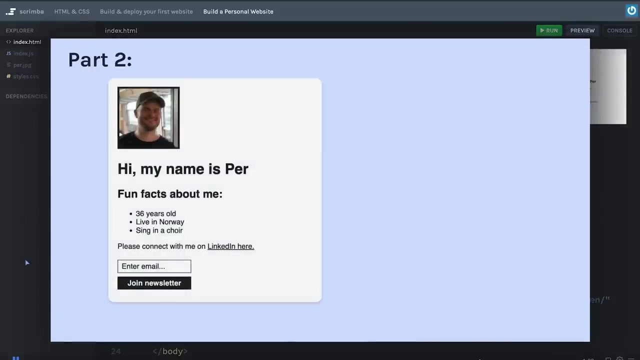 with join newsletter as the text. Yes, that worked, And we finally just need the placeholder in the input, And here we're going to write enter email, enter email, like that, And actually looks pretty good to me. That is what we were looking for. Yes, Okay, next step, we are. 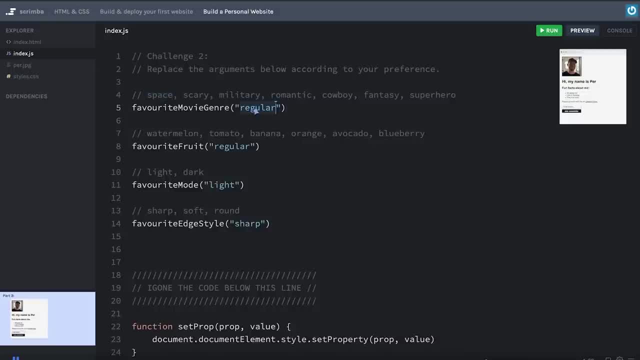 going to personalize it. This will be easy for me. I really love movies about space, So I'm going to choose space here as my favorite movie genre. It gives me this really neat sci fi ish font, And I am a huge avocado fan, So gotta do that. Whoo looking pretty good. 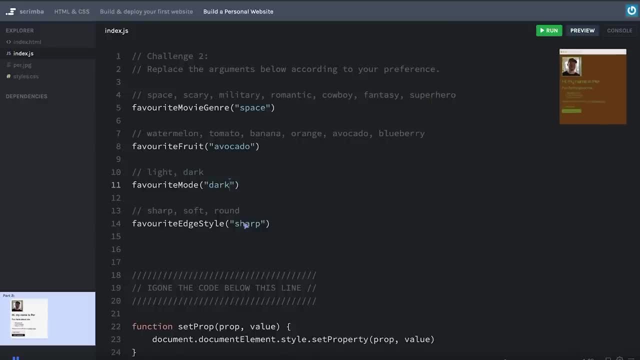 I tend to prefer both light mode and dark mode, But let's try dark. Yeah, not bad. And as for favorite edge style, not going to do completely round, not completely sharp, but something in between, As I think the answer often is something in between. And yes, there. 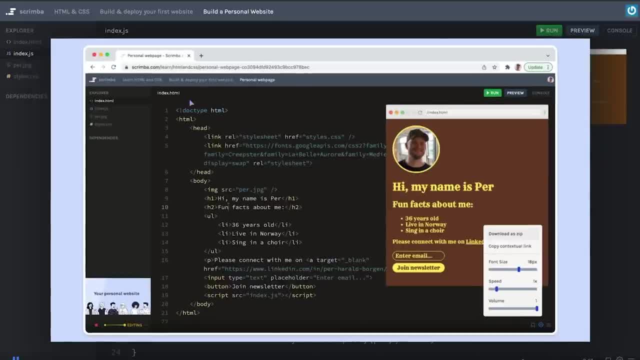 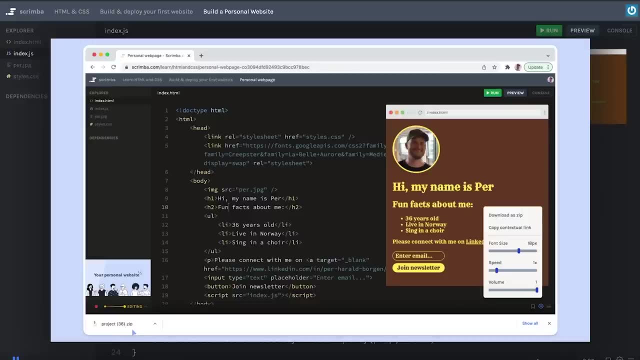 we go: Pretty cool website. Now the final thing I want you to do is head back to your note, where you created your website, And then click on the bottom right icon, the cogwheel, and choose download as zip, because that'll download your project through your local machine. 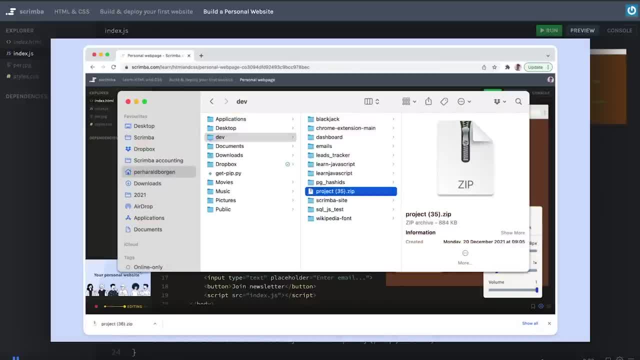 Only that, in order to deploy this project over the next few scripts. So what I'd recommend you to do is, on your computer, create a dev folder and move that zip file you just downloaded to this dev folder. double click on it to open it. that'll give it this long, obscure. 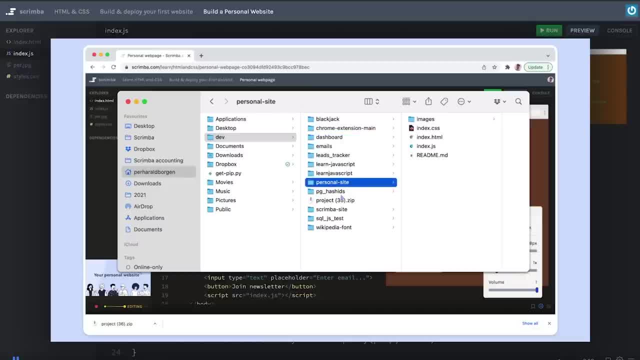 ID. So if I were you, I would change that to something understandable, for example personal site, and just save it so that you have your project neatly placed with a good name on your local computer so that we are ready to share it with the world. 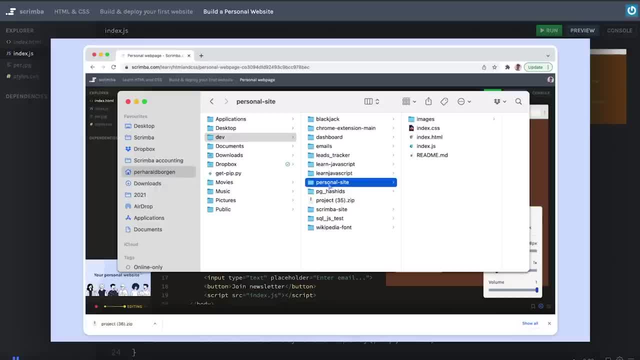 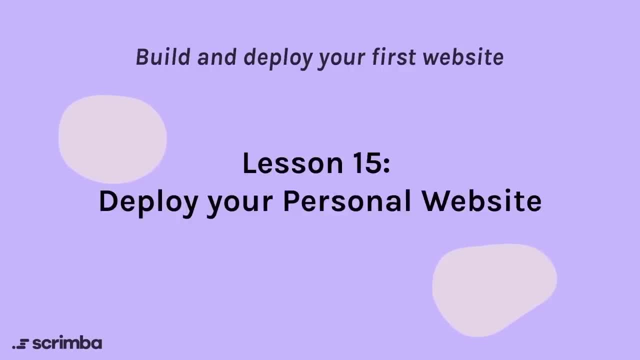 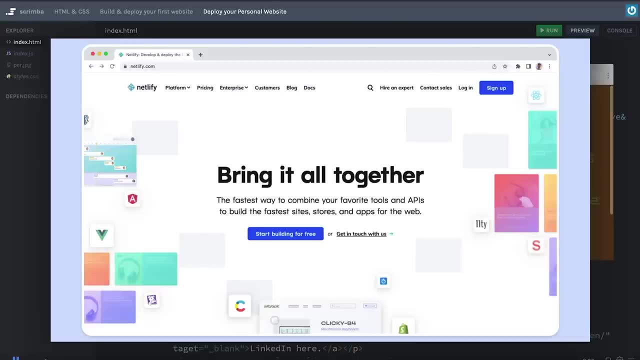 Over the next few scrims. it is going to be epic, So I look forward to see you in the next room after you've done all of this. I'll see you there. In order to get your personal site live on the World Wide Web, we are going to use a service called Netlify, as it is both. 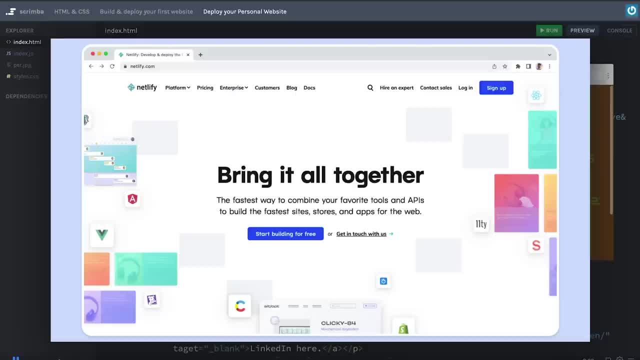 free, easy to use and powerful, as it's used by tons of professional developers. So if you're following this course on scrimbacom, just click on this slide right here and you'll get to Netlify. Or if you're following this course on YouTube, just head over to Netlifycom. 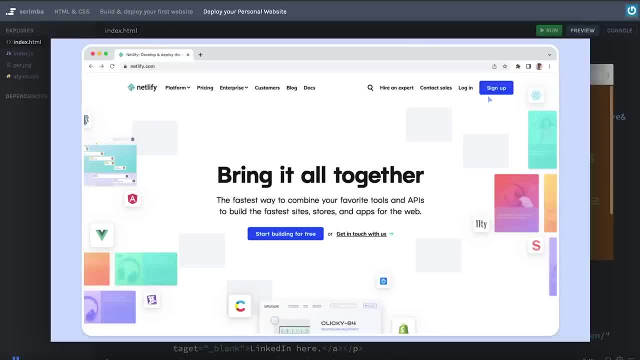 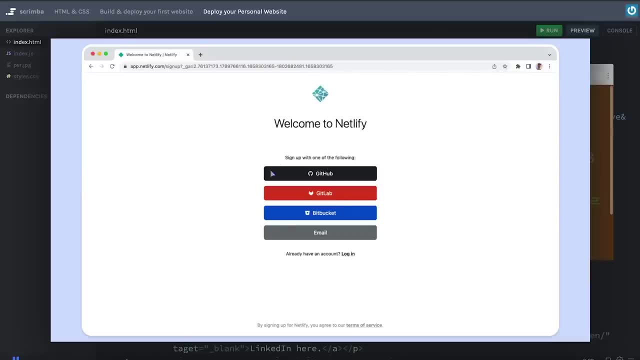 And you'll get to the exact same page. Once you're there, I want you to click at the sign up button, as that'll take you to an authentication screen. we can choose a bunch of different options. I am going to go with the email option, So I'll click on that and fill in my email. 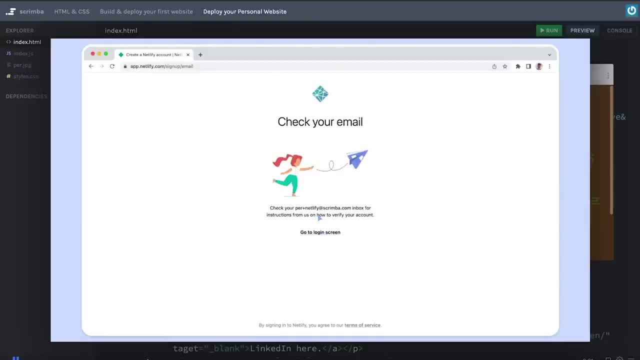 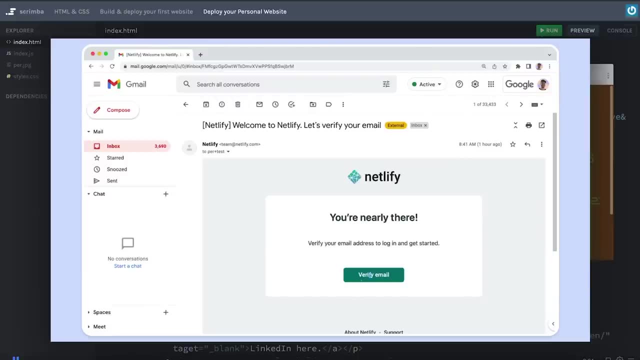 and also choose a password. Then I'll click sign up, which again will trigger Netlify to send a verification email to my inbox. So I'll head over to my inbox And click on verify email. that'll take me to the Netlify onboarding page where I have 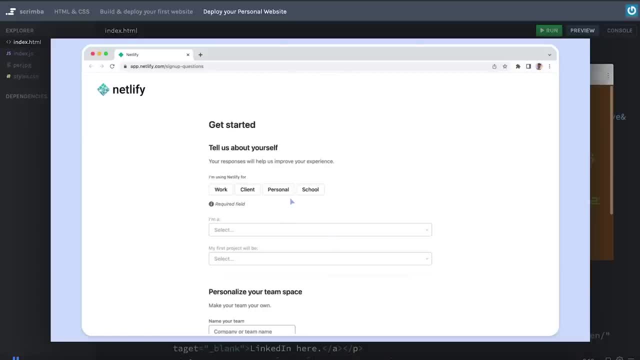 to tell them a little bit about myself. So here I'm going to say that I'm using Netlify for personal reasons And, opening up this select box here I'm going to classify myself as a hobby developer And my first project will be a personal slash portfolio site. then 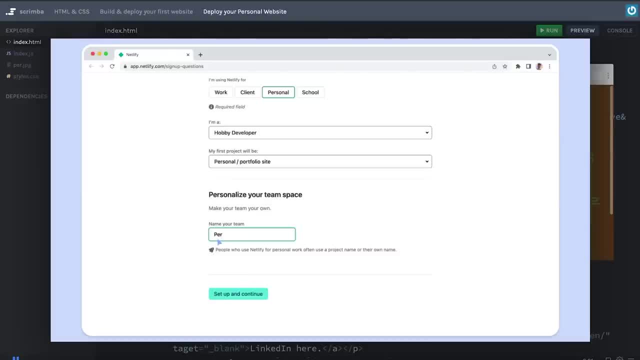 I'll scroll a bit down and give my team a name. I'm just going to call my team pair, as it's common to use your first name, but you can choose whatever name you want on your team. So first click on the setup and continue. then you are taken to the page where you are. 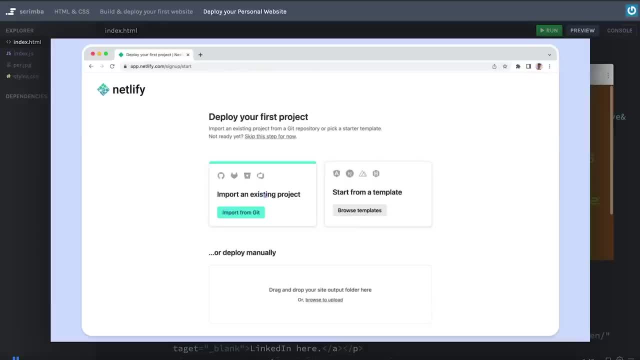 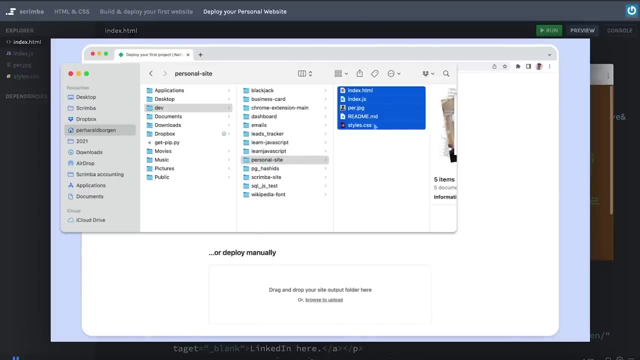 to deploy your first project. you can either import an existing project, start from a template or deploy manually, And that's exactly what we are going to do. So what I want you to do here is return back to the folder you created in the previous scrim, called personal site. 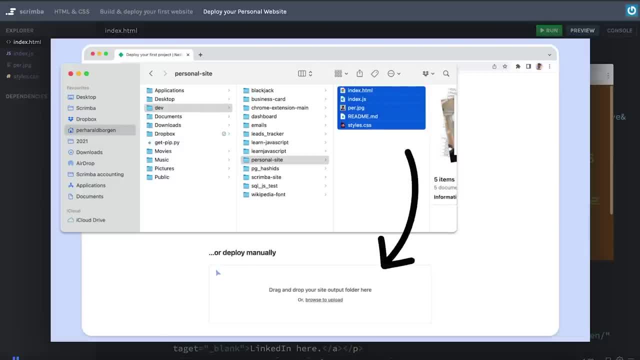 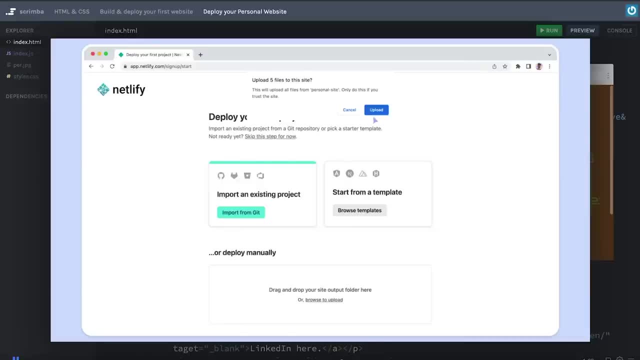 and then mark all of the files and drag and drop them into this rectangle. Once you've done that, your browser might ask you if you actually want to upload them. If you want to upload the files to the site, just confirm that by clicking on upload and. 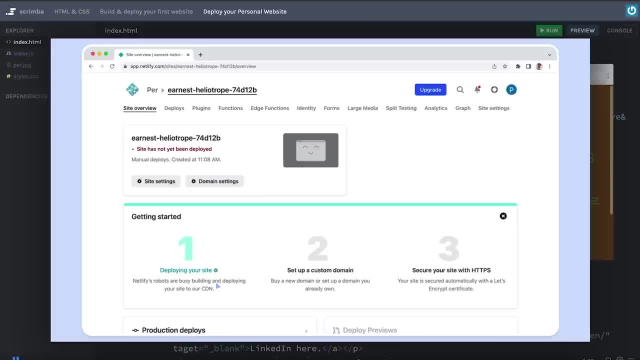 then Netlify starts its magic. At this point they are working under the hood, deploying your site to the web. So here you might have to wait for a couple of minutes until you see this icon right here turn into a screenshot of your personal site. Now, if that doesn't, 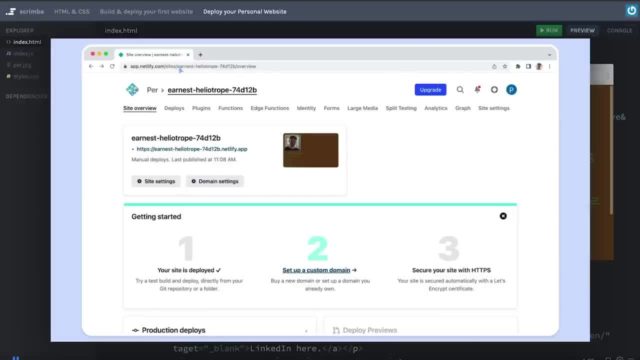 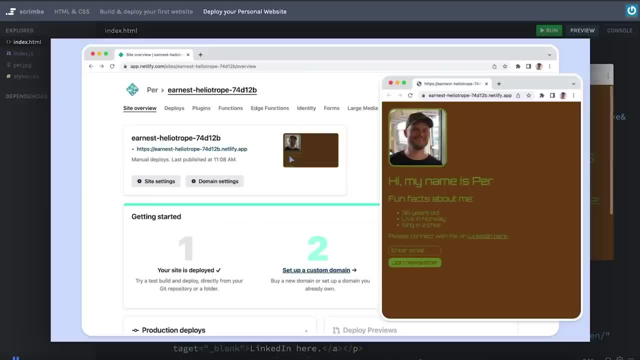 happen within a couple of minutes. just try to refresh the site itself, as that'll probably do the trick. then you can simply click on this URL right here and boom: you have deployed your site And now you know that anyone in the world can access it. That is a phenomenally great 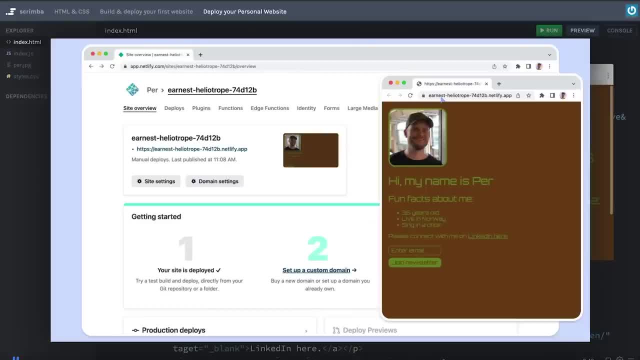 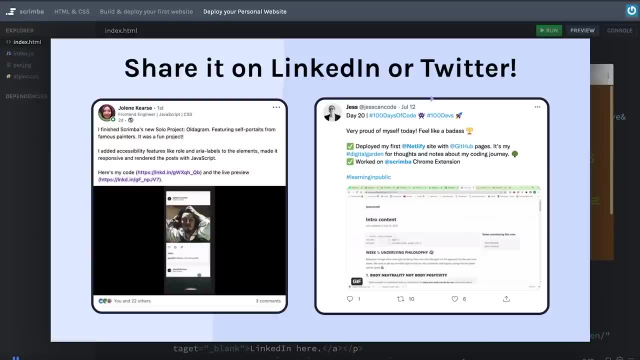 job, and you should truly be proud of yourself. The final step I think you should do now is to share your creation with the world. I would recommend you to use either LinkedIn or Twitter, as both of those have huge communities of developers, So what you should do is basically. 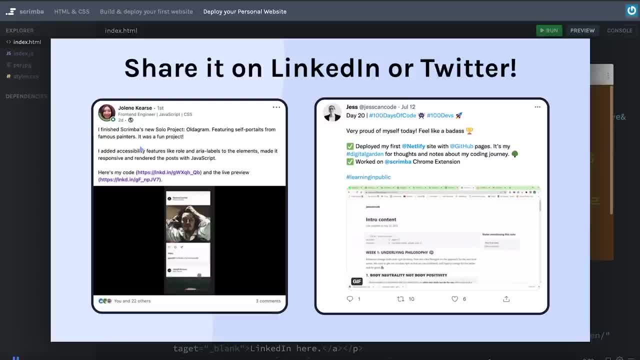 what Jolene and Jess are doing here: share a link to your personal site, write a couple of sentences about it, And also feel free to mention anyone else who've been involved in this project And add a relevant hashtag, like Jess is doing here. for example, 100 days of code, But that. 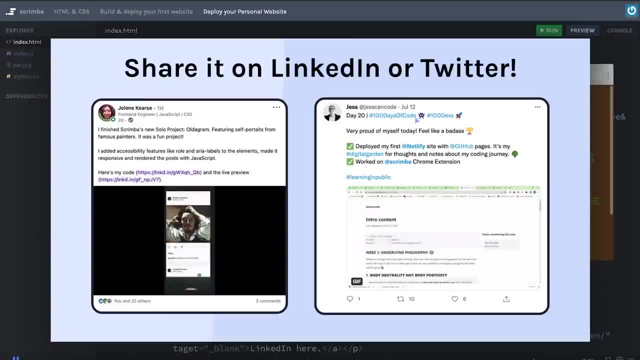 is a great hashtag to follow and to use, as it puts you in touch with a bunch of other people online who are going through the same learning journey as you are. So I am looking forward to see your personal site either on LinkedIn or Twitter, And I'm also looking 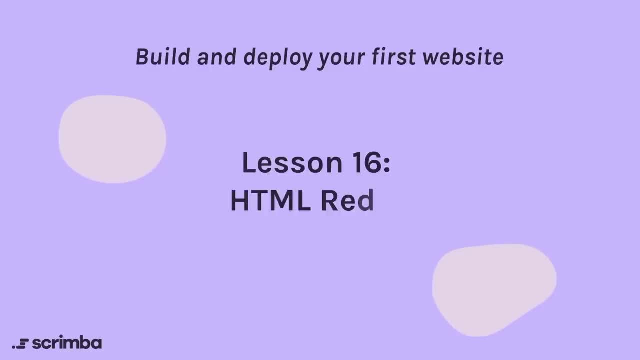 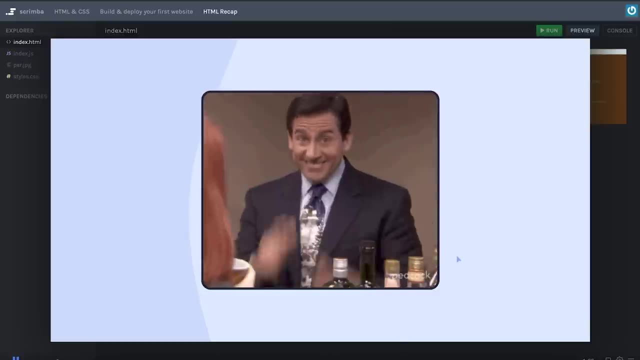 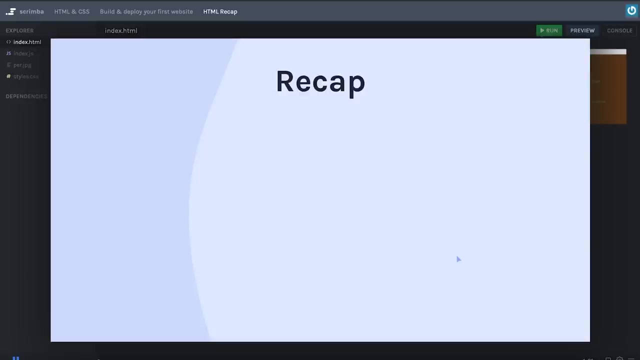 forward to see you in the next scrim. Guess who is my favorite person in the world right now? You are, because you have just completed the HTML section of this course, And that is really well done. Now let's have a quick look at what you've learned. Starting off, you learned 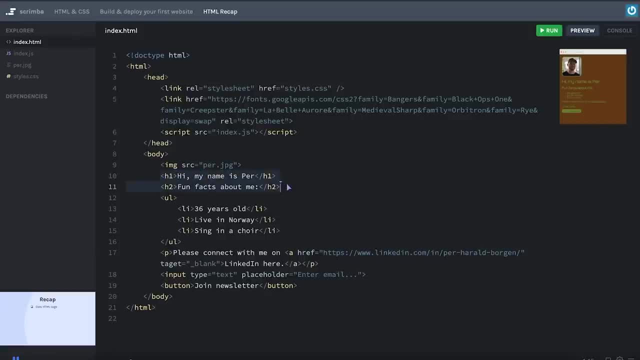 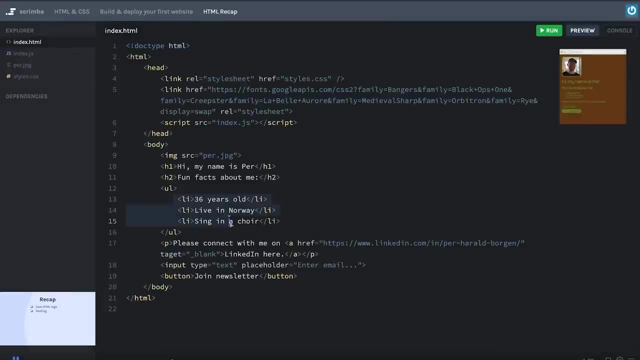 about the core HTML tags, that is, for example, the heading tags like the h1 and h2, and also the paragraph tag. Next, you learned about nesting, which is how we place certain tags inside of other tags, which again are inside of other tags, creating this tree like HTML. 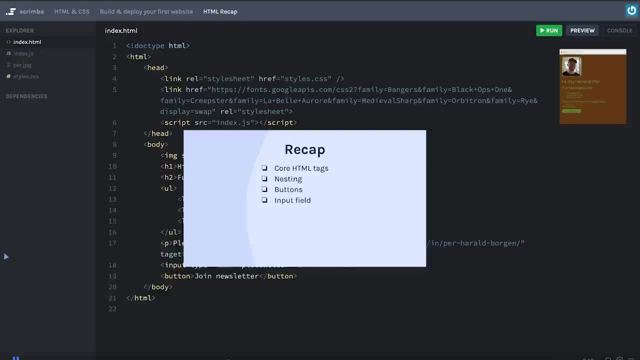 structure, And you learned about the buttons and input fields. And then you learned about the tags, which again are inside of other tags, creating this tree like HTML structure. And you learned about the field, which are two tags that help us make our website interactive, so that 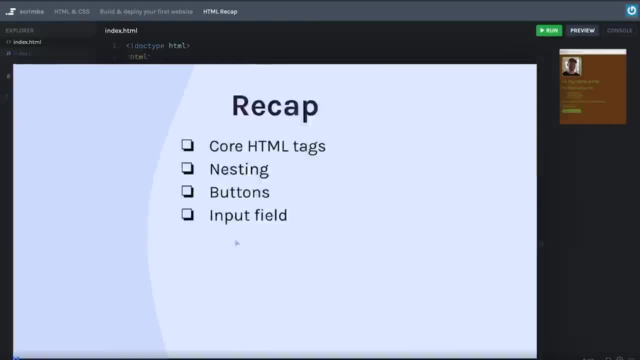 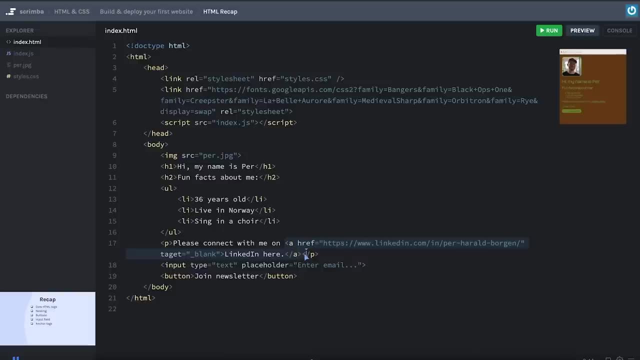 users can perform actions on our website. We also learned about the important anchor tag, as that is what allows you to create links in between different websites or internally on a website, in between pages. Another thing which we had to look at was the document structure. 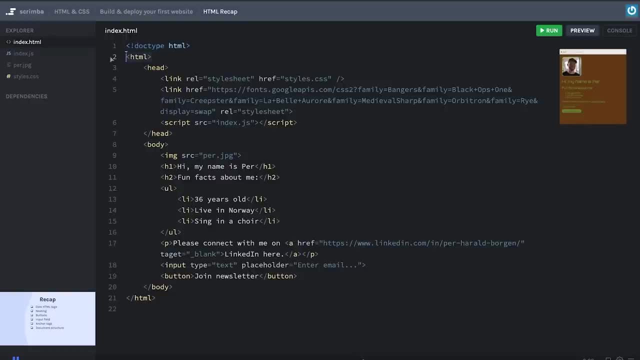 because a proper HTML document requires a doc type, an HTML tag, a head tag and a body tag. And then, of course, you learned about lists, both the unordered lists you can see here, and also ordered lists. And then, at the end, we did something super cool, which 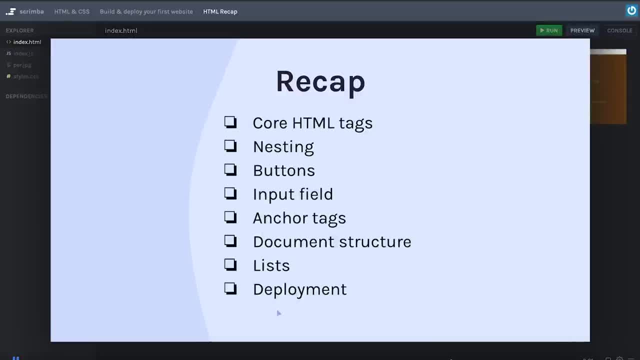 was to deploy our website using Netlify so that it lives out on the World Wide Web. So at this point you might be a little bit overwhelmed. that's totally okay. feel free to take a little break now, And when you return back you are going to learn about CSS, aka cascading style. 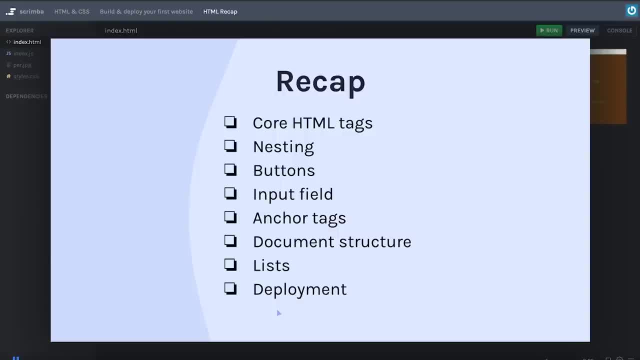 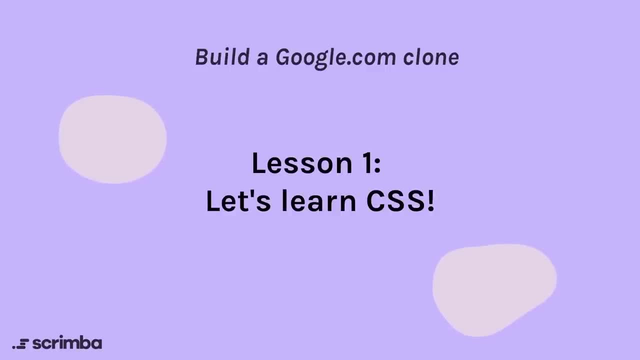 sheets, which is a tool we use in order to make our websites look good. So that is going to be a lot of fun. I'm looking forward to see you in the next section. Welcome to the second section of this course, where you are going to graduate from HTML. 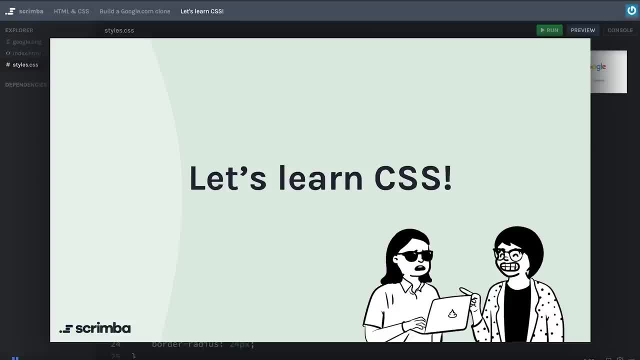 into the world of CSS, or cascading style sheets as it stands for. This is super exciting, because now you'll be able to make your sites look beautiful as well. So the main project of this section is actually the googlecom homepage, Because this time around you are. 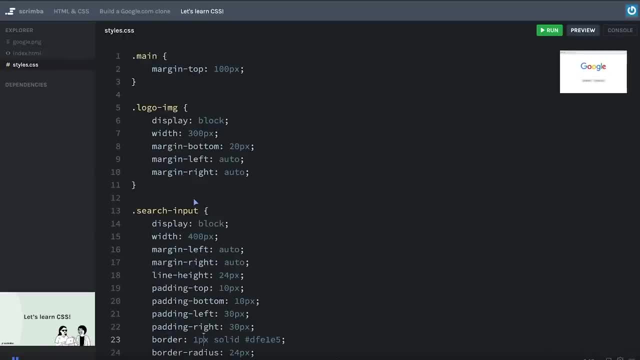 going to write the CSS as well, And this probably looks a little bit freaky, but it's not, So let's get started. Welcome to the second section of this course, where you are going to graduate from HTML, which is a tool we use in order to make our websites look good as well. This is going. 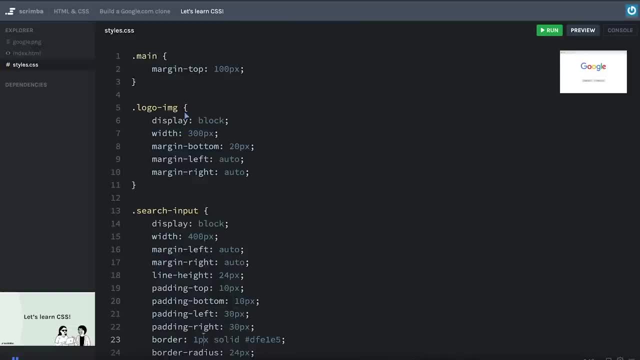 to be a lot of fun. I'm going to take you through it step by step And actually, before we get going with Google, we're going to get you familiar with the syntax here and have some fun destroying wikipediaorg. So it's going to be a lot of fun and we have no time. 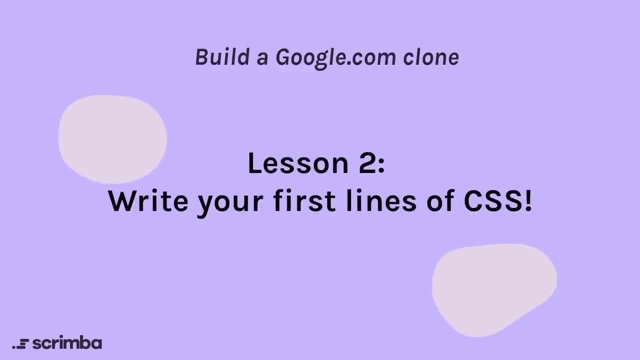 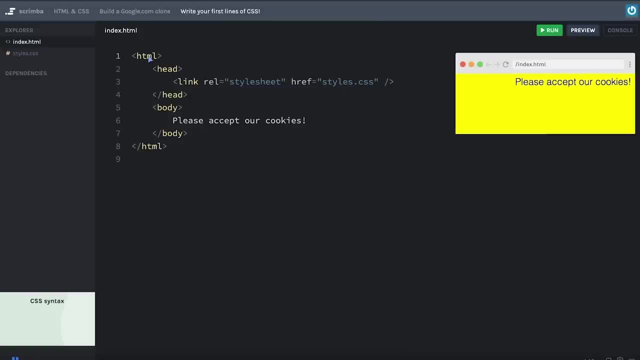 to lose. Let's just get started. Okay, so let's get you writing your first lines of CSS straight out of the gate. As you can see, here we have an HTML file which has a body that please accept our cookies as text directly in the body tag And that is rendered here. 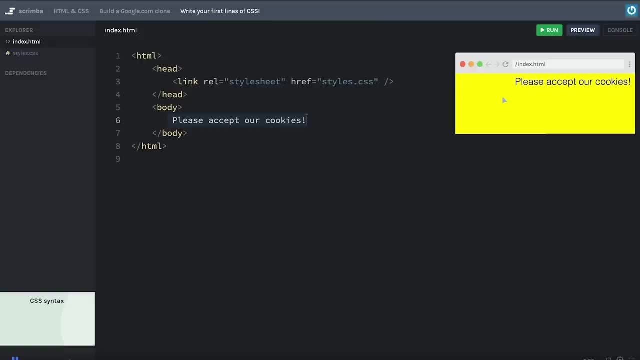 in the mini browser. However, as you'll notice, the style doesn't exactly look like default browser styling, And that is because we've added this line here which says link, meaning it's linking to something, And what kind of relation does this link has to our HTML? Well, 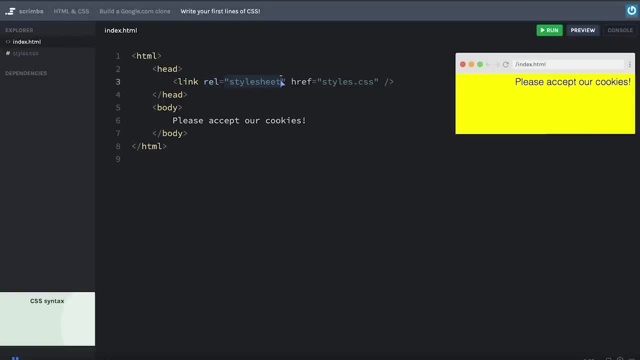 it's rel style sheet. it is a sheet that contains styles. And where does this sheet live? Well, that is dictated by the href attribute, which you probably recognize from anchor tags, and it's pointing to styles dot, CSS. And lo and behold, in our file system we have a styles. 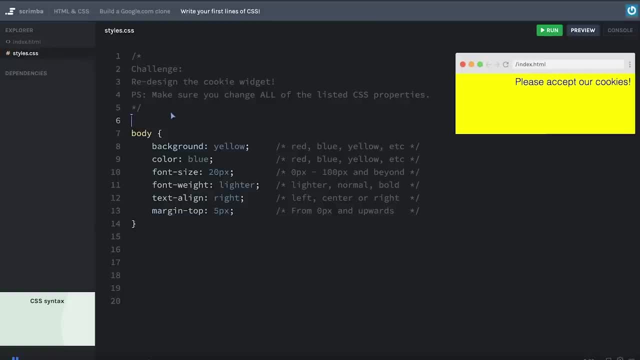 dot CSS file, And there we can see a few lines of scary looking codes you've never seen before, perhaps. however, don't worry, we're going to go through this. So what happens here is that this CSS code is being pulled into the HTML file by this line three here and then. 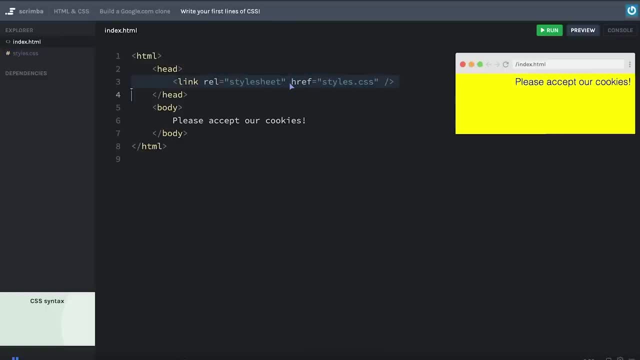 it is applied to the website when it is rendered. So if we were to comment out this line three here and rerun the example, it'll look very boring like this. So let's undo. that doesn't exactly look great now either, But it's at least some styling, although this cookie widget 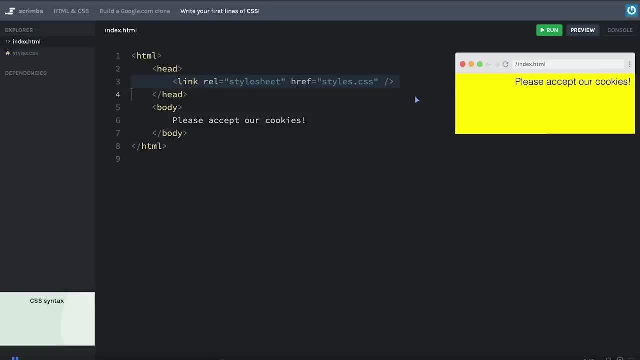 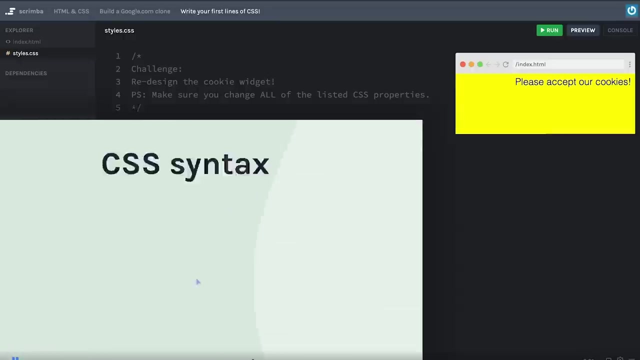 is a little bit weirdly designed, in my opinion, which leads me to your challenge. you are going to redesign this cookie widget by changing the values inside of this body selector. And now you might ask: well, what is a selector? Okay, let's go through that, Because that is the 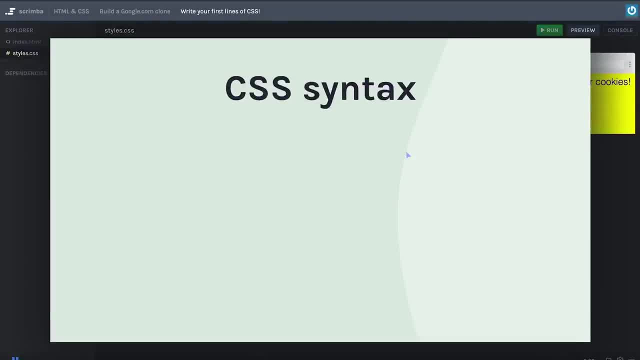 basic CSS syntax you need to know in order to solve this challenge. So CSS works by selecting certain elements on the page, that is, HTML elements, and then styling them however you want, And the element you select is what you start with. So let's start with when writing a CSS rule. Here we are selecting the body, that is the 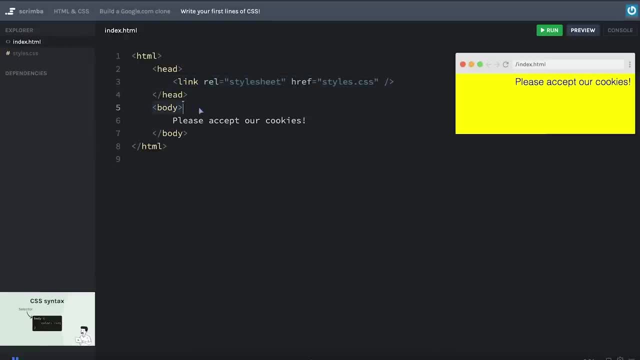 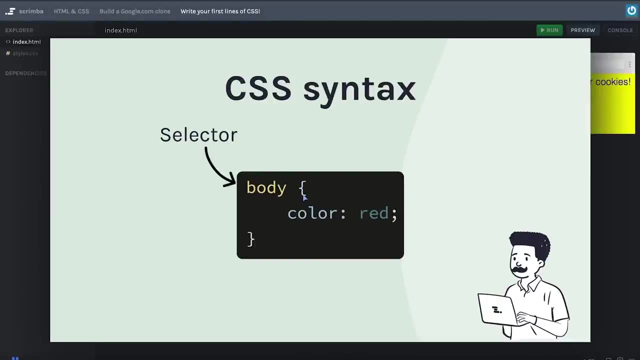 exact same thing we're doing here. And what's our body? Well, that is this tag right here. then, in order to apply some specific styling to the body tag, write an opening curly bracket and a close curly bracket, And then, inside of those brackets, we have something called. 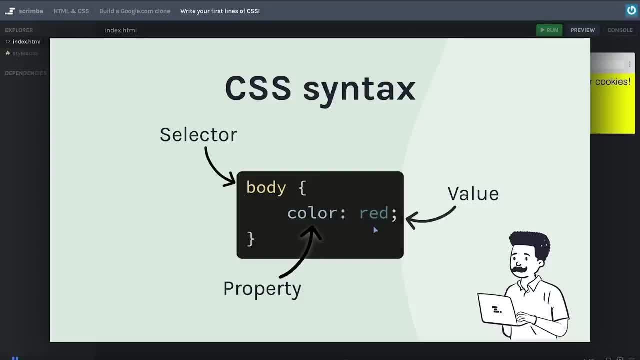 a property, which in this case is color, and the value, which in this case is red. So here we're saying that the color which is actually text color- That's what color means here- the text color in the body should be red. So if I now 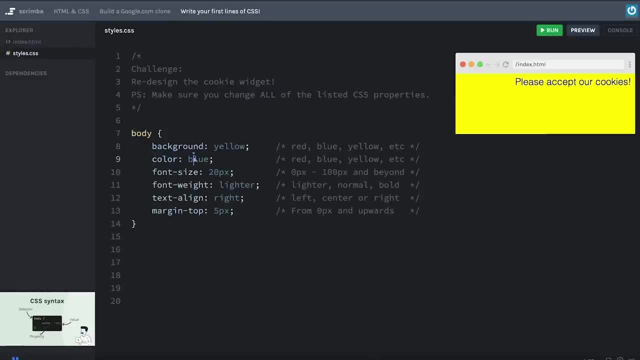 change the color property from blue to red. you can see in the browser, we have changed the text inside of our body to red, because if we head over to the HTML, this text is indeed inside of our body. Now, as you might have noticed as well, the property is followed. 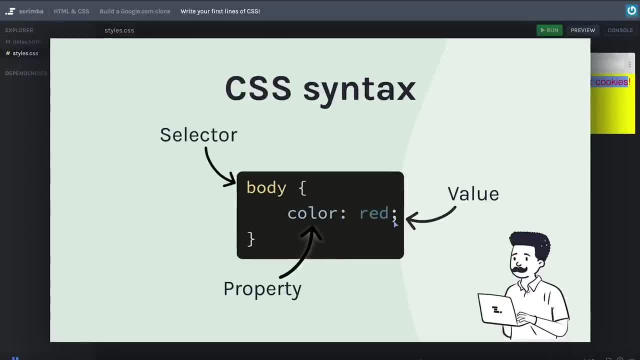 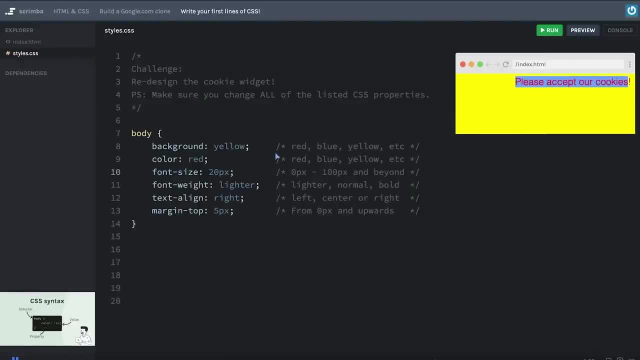 by colon and the value is followed by semicolon, And you have to have that notation, Otherwise you'll break the example. So what I want you to do now is redesign this cookie widget, make sure you change all of the listed CSS properties. That's background color font. 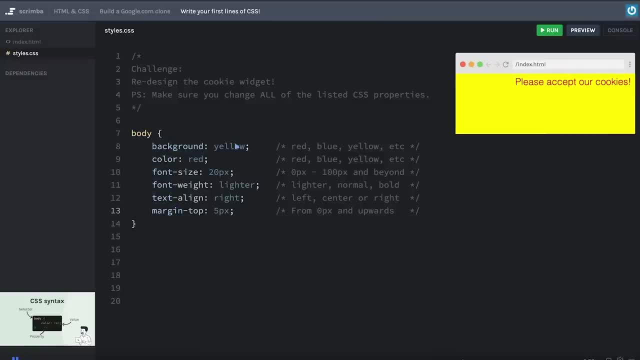 size, font, weight, text align and margin top And what you'll change it to is up to you, But I've given you the hint of what kind of values the properties expect here. in the comments On the right hand side you can see comments in. CSS is done with this star. 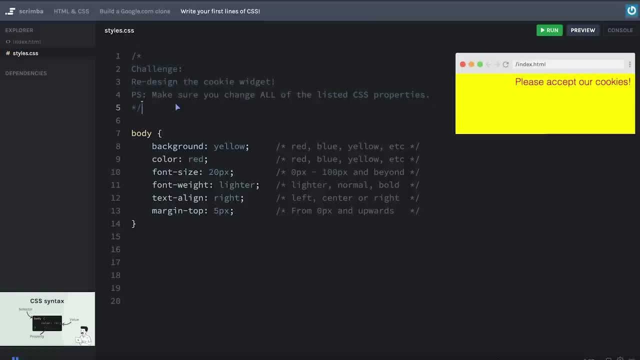 and slash character. So the grayed out text, as in with the HTML, is not interpreted by the browser. It's just help text for you in order to solve this challenge, And I'm intentionally not giving you any more information about what each of these properties mean, because 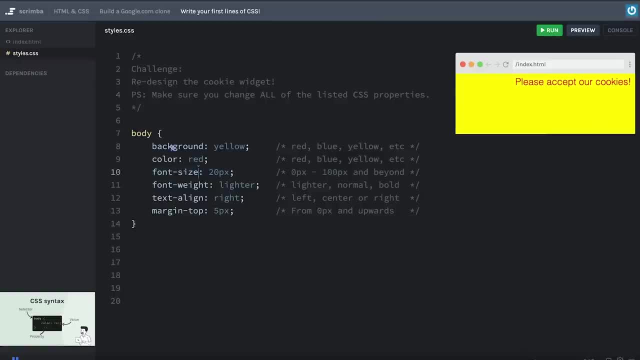 I think they're pretty self explanatory, So I want you to experiment with changing them and draw your own own conclusions as to what, for example, the font size does to the styling on our page. And then, once you've done this, once you've redesigned the cookie widget, move on to the 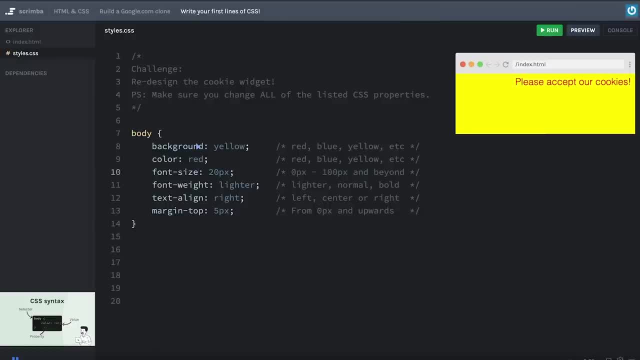 next scrim, And then I will show you how I would do it as well. Good luck, So really good job, writing your first lines of CSS. That is no small accomplishment. Now I'm going to show you how I would design my cookie widget. So I want my widget to have: 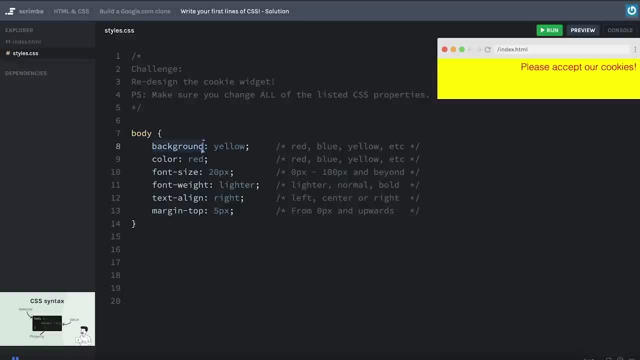 cookie colors. So, for my background property, which is what sets the background color of the body which fills up the entire browser, at this point I'm going to choose a color called saddle brown, like that, And you might wonder: well, how do I know that saddle brown? 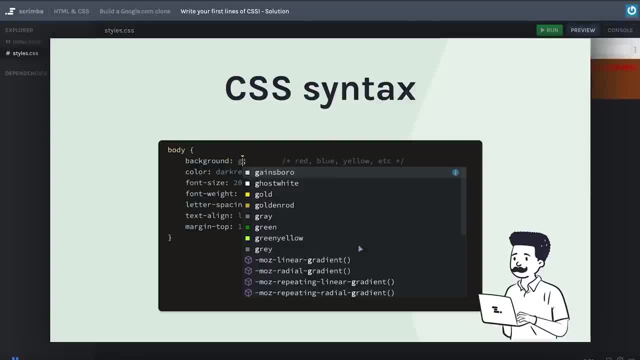 is a color that CSS supports. Well, you might have noticed, as you wrote CSS values, that VS code, our editor starts suggesting values for you as you start typing. So that is how I found saddle brown. This suggestion box here isn't recorded by scrim by itself, So you won't see it in recording. 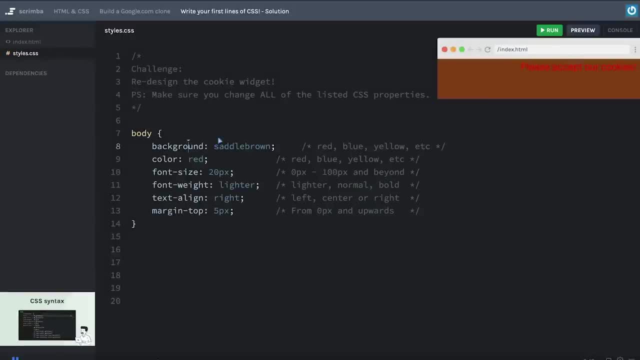 but you will see it as you interact with the code yourself. So we have the background. Now let's move on to the color. Here I don't have red, I want to have something a bit more cookie ish, And it just happens to be a color called chocolate, like that, starting to look. 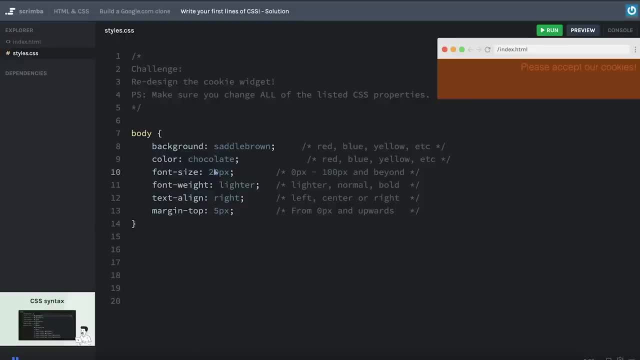 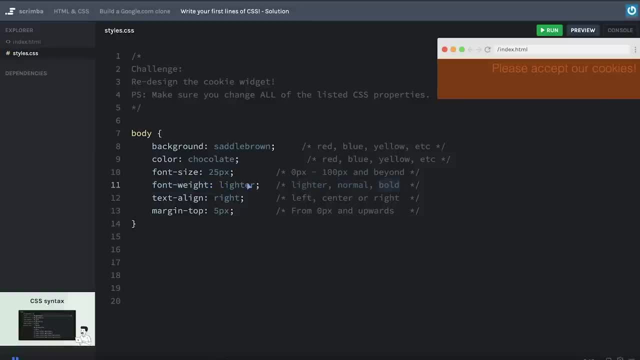 and set that to 25.. Okay, so I'm going to go ahead and set that to 25.. Alright, so over and over it one, you can start to see the color parties and the other colors over and over. Some of them have more color. You can have a different color. I have red. llama yellow and a navy blue and a navy blue and a navy blue, And I can turn it over to a green base to make the talk, creating looking like a pink. Now let's go ahead and click on Open Email, Airег and I have all of our articles here. obviously you can jump. 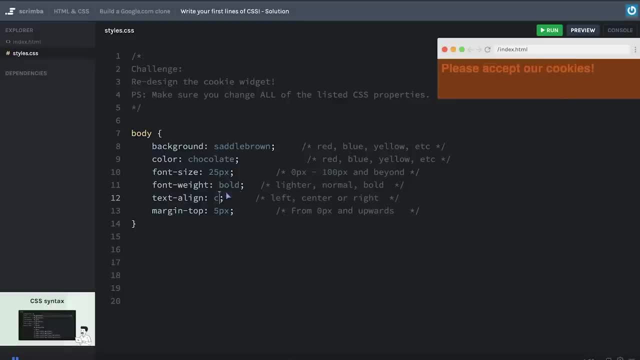 in the keep you in my chat. Hello everybody, welcome back to temasほی and the next. nice, it is pushed all the way to the right hand side. Let's center it for this time, which means that we only have the margin top left- And that is also a pixel value- as the font. 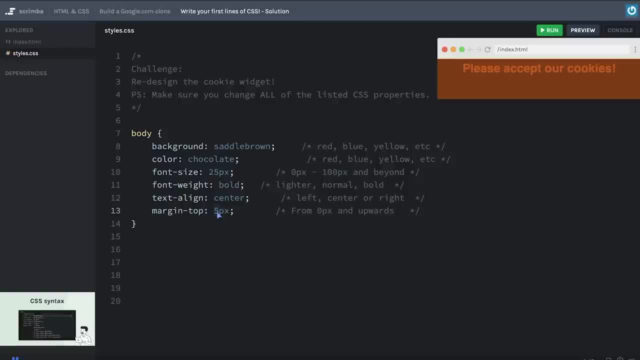 size was, but it's set to five pixels. Let's remove that. Let's bring it down to zero and see what happens. You can see the text jumped up a little bit And now there's no spacing in between the top of the browser and the text itself, So it adds margin. that is spacing. 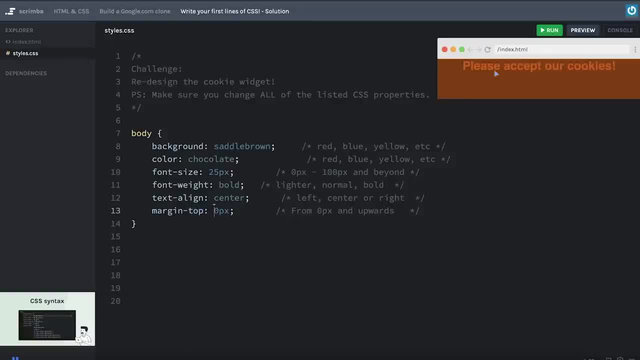 to the top. So this means that we can use this in order to push the text down to the middle of the browser, kind of centering it vertically. Let's try, for example, 20.. Not fully centered, Let's do 40.. Yes, that looks really good. Now, before we move on, there's 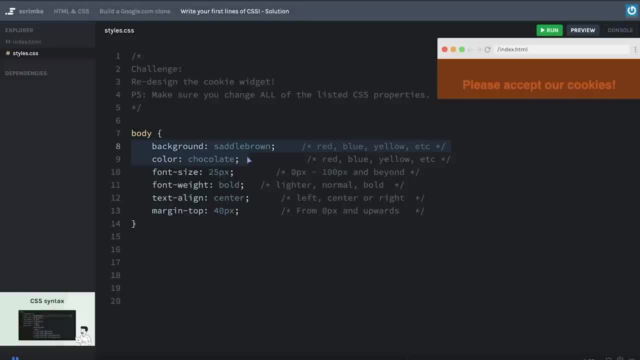 one thing I want to mention, which is that normally, when you deal with colors in CSS, you likely won't see these plain English descriptions of colors. Instead, you'd rather see is something like this: So this weird six character long expression with a hashtag in front of it, and this is: 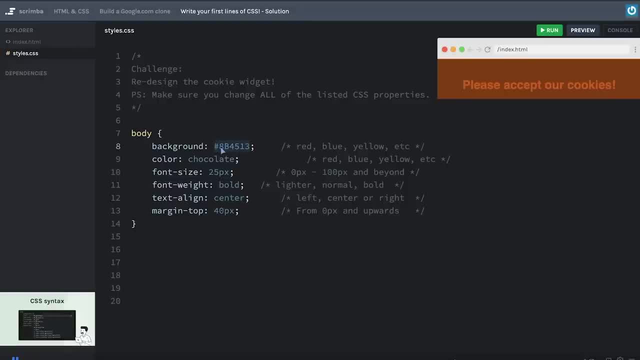 called a hex color code And that is a description of the color. It's a recipe for how much red, green and blue this specific saddle brown color consists of, Because, as you can see, nothing changed in our browser. I did this, But if I change the recipe- for example changing 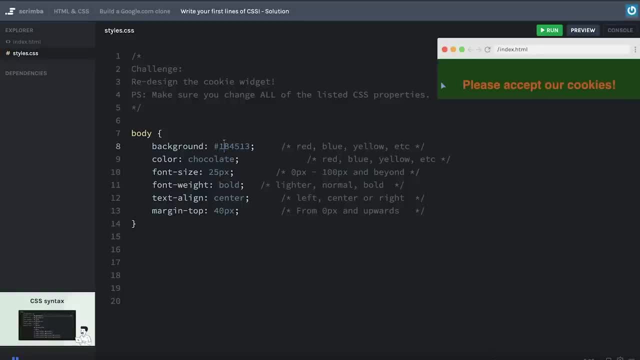 this eight to one boom. you can see that the color is suddenly completely different. Now we're not going to go into how these hex color codes work on the inside. That's outside of the scope of this lecture And it's certainly not expected that you remember. 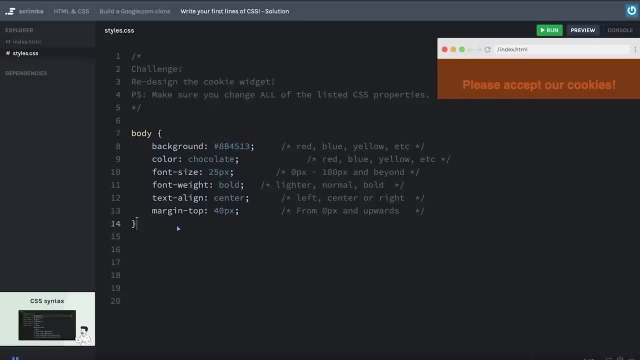 what kind of colors the different hex codes refer to. So now you might be a little bit confused and overwhelmed about all of these properties. Don't worry about it, you're not expected to remember everything right now. I just wanted to dip your toes into the water. 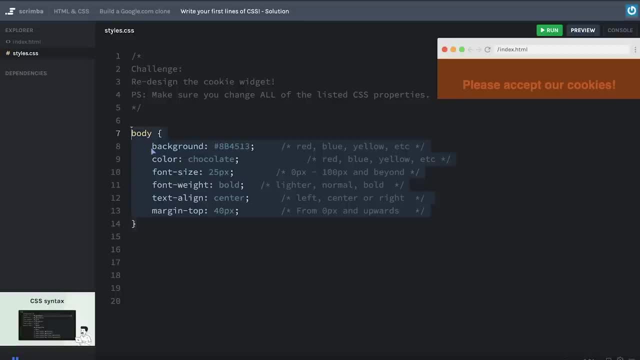 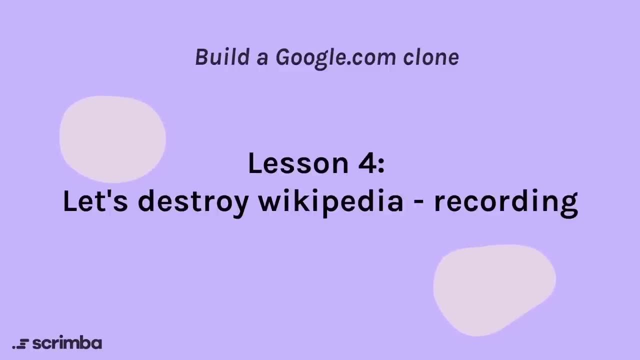 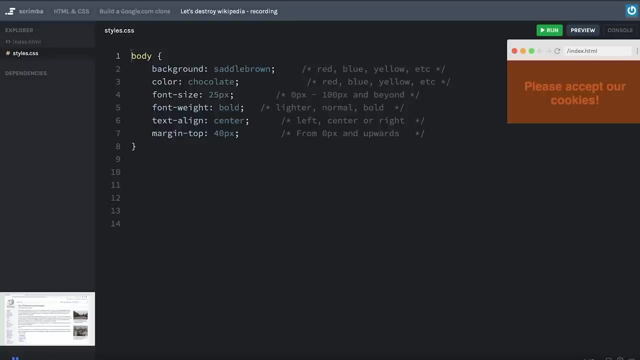 so that you are exposed to them, And then you'll certainly get plenty of practice with all of these properties later down the line. So let's just move on. Now that you know enough CSS to be dangerous, let's use your newly acquired superpower in. 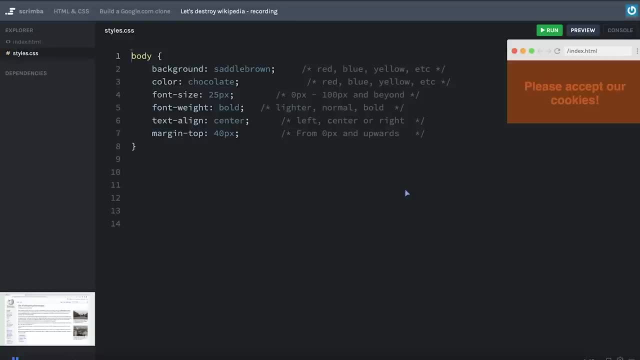 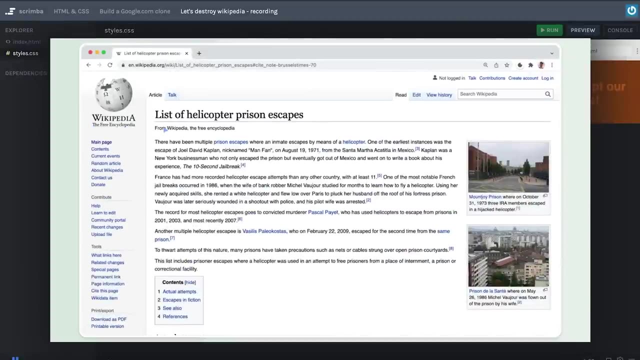 order to destroy Wikipedia, And for that we need a Wikipedia page, And about the coolest one there is is this list of helicopter prison escapes. I mean, oh my god, how insane is that? So click this image and you'll be taken to this article, And then I'll show you step. 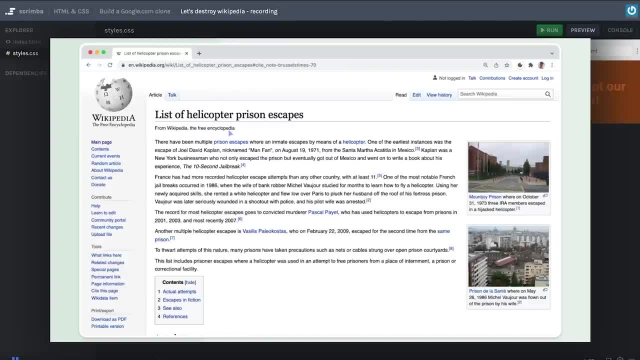 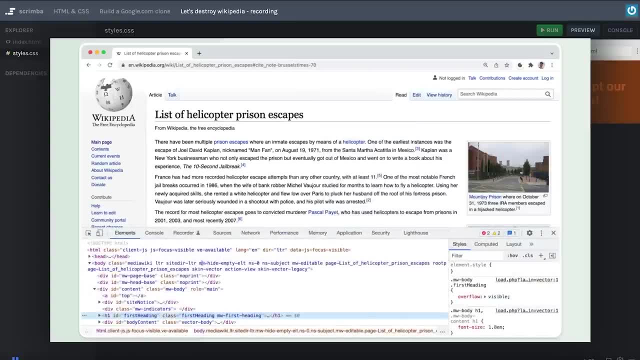 by step how we can destroy it with CSS. So the first thing you need to do is to right click. that'll open this menu where you can choose inspect And once you click that, the dev tools will open. then choose the icon in the far left, as that allows you to use. 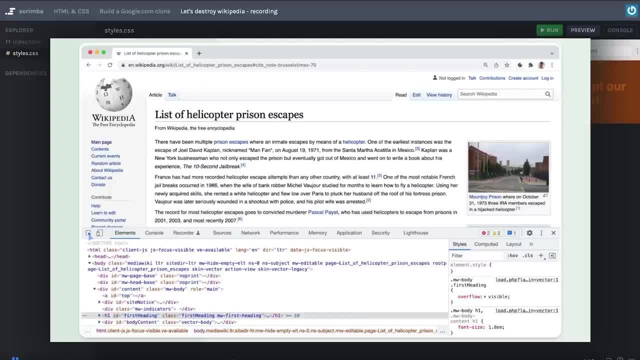 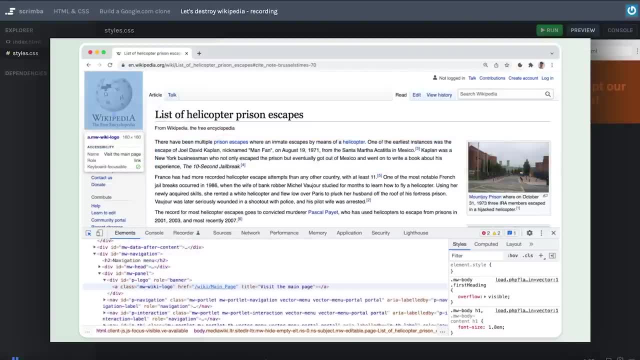 your cursor to select elements on the page, So that when you hover over an element like this one, you'll see that the dev tools selects it for you. So if you move your cursor over to the logo, you'll see that one selected, And if you move your cursor over to the main, 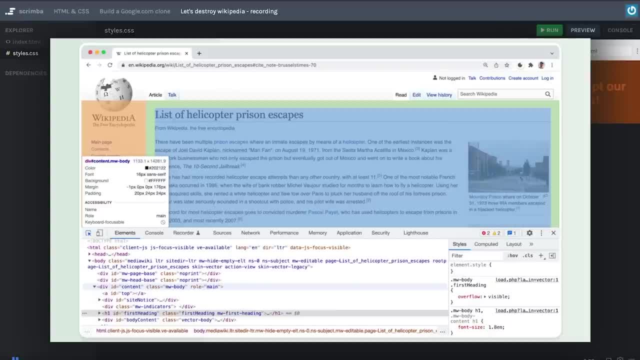 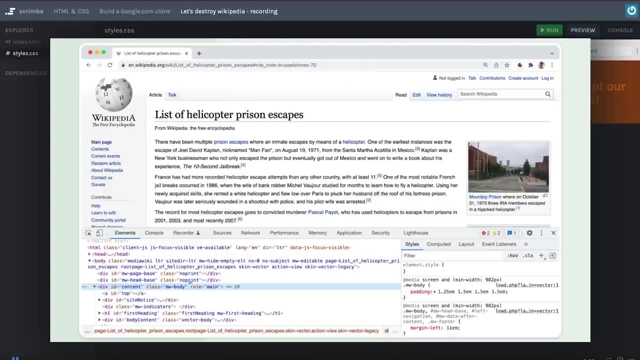 part of the screen here you can see. it selects the entire article. Once you're on that selection, I want you to click, because that'll select the specific HTML element here in the elements tab And don't worry about all of this you. 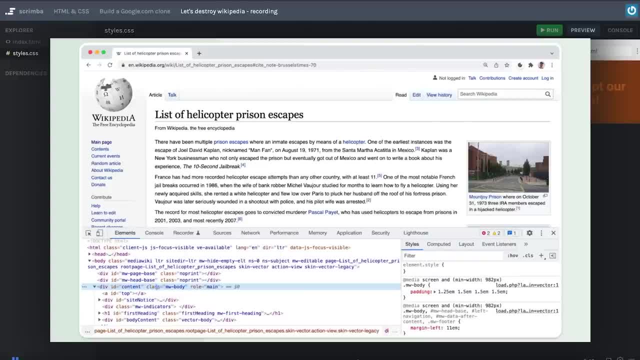 do not need to recognize the tags and attributes and everything you see here. what I instead want you to do is head over to the right hand side, where you see element dot style, click there and you'll be able to actually apply CSS directly to this page. So you can for. 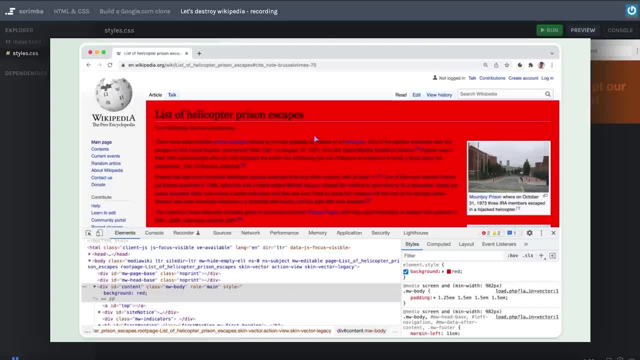 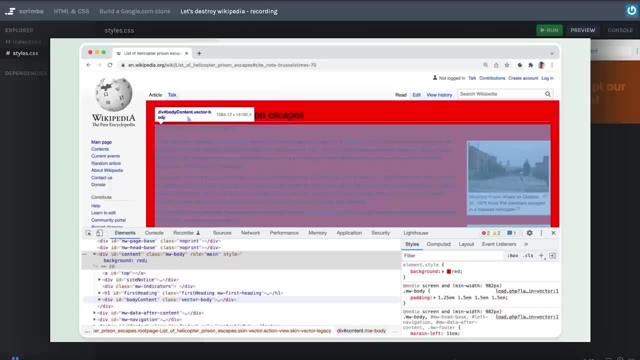 example, write background red and boom there, we have really ruined this article. Then if you select another element on the page from this body- content element- you'll see that the content element. here you can do the exact same thing. click on the element style And. 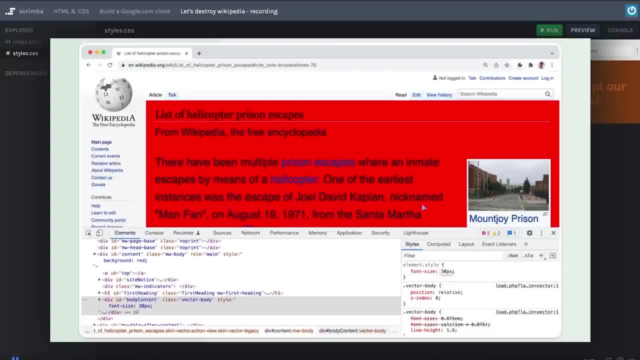 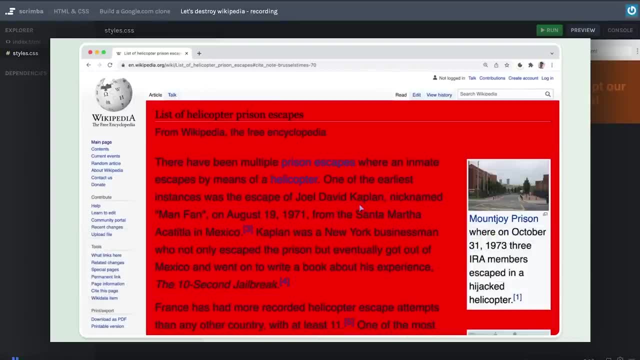 now, for example, right font size and 30 pixels. And there you go. Now you can click on the x icon in the far right corner here, And then you can read about these helicopter prison escapes, with a really bad background and huge text, if that's what you prefer, So feel free. 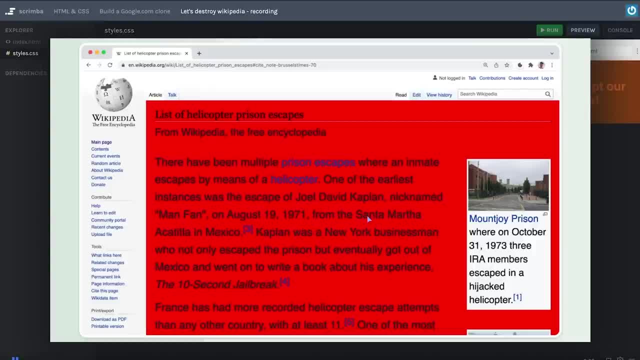 to spend an hour in this article, and then I will see you in the next scrim. Okay, so now it's time for you to go to the next screen. Okay, so now it's time for you to go to the next screen. Okay, so now it's time for you to go to the next screen. Okay, so now it's. 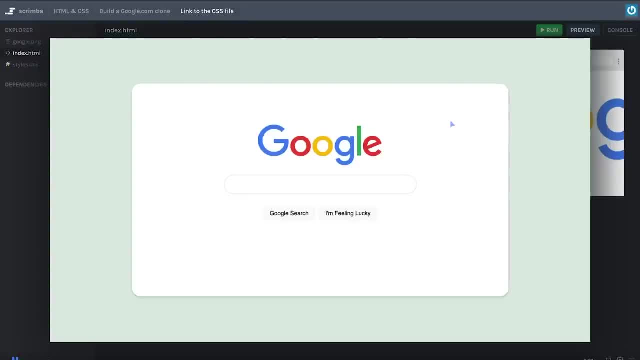 time for you to get again build the googlecom homepage, But this time around you're also going to write the CSS, so that you'll understand everything that goes into building this elegantly designed search engine. As you can see, I've set up the basic skeleton here in the HTML. 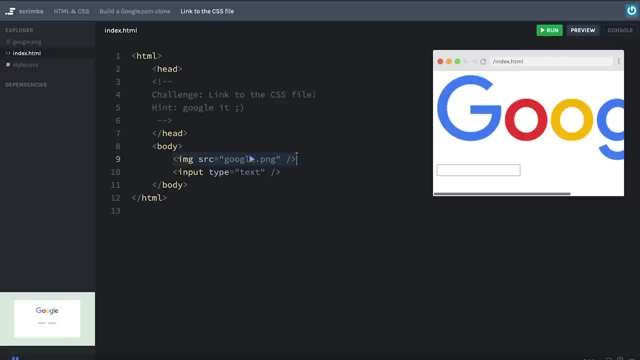 file for you. in the body tag we have an image which is pointing to the google dot pilgrimage, which lies in the same directory as our index HTML folder appear, And we have an input type text which is our search field, And we're only going to start with these two elements. 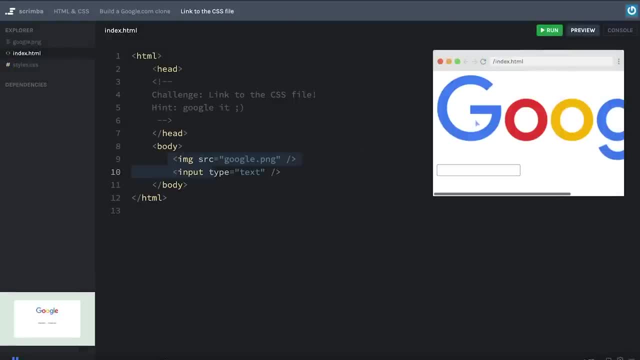 and then later move on to the buttons. Now, as you can see in the mini browser here, this looks horrible. It has no styling, So the logo is far too large. the input field doesn't look very good. In short, there's a lot of work to do here, But before we can start writing CSS, 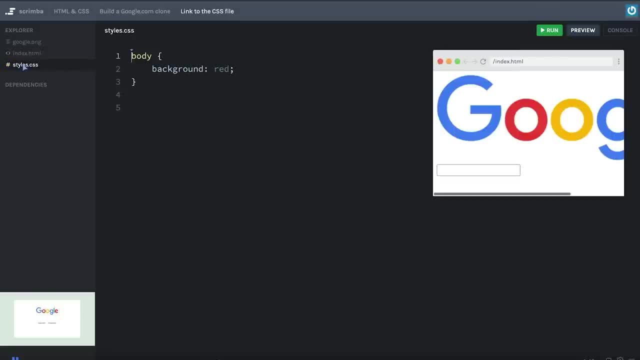 you need to link to the CSS file, because he I have a style CSS here which just sets the background of the body to read as a way of testing whether it is actually linked to the HTML. Currently it's not. you are going to have to link to the CSS file on your own And, if you remember, 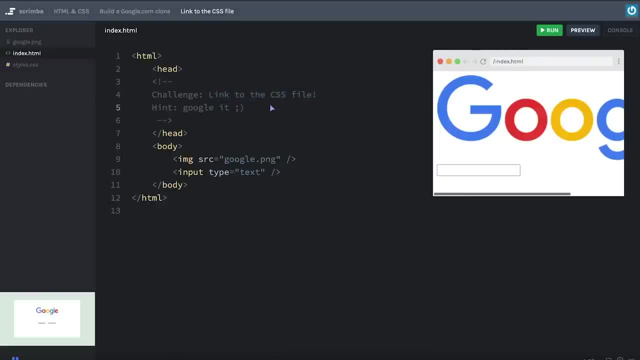 a couple of scrims back. I showed you how to do that, though please don't look back at that scrim in order to solve this challenge. Instead, Google it, because I do that almost every single time. I have to link from an HTML file to a CSS file, So you should not be ashamed for Googling. 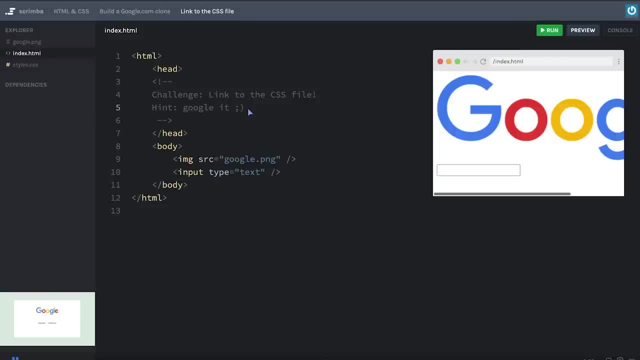 such a quote, unquote, simple thing. Instead, just do that right now because it's important practice, And then when you come back, I will show you how I would do it as well. Okay, hopefully that went well. Now let's have a look at how we can solve this. So I would simply: 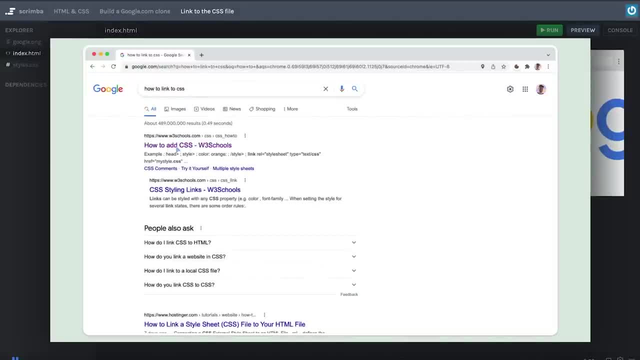 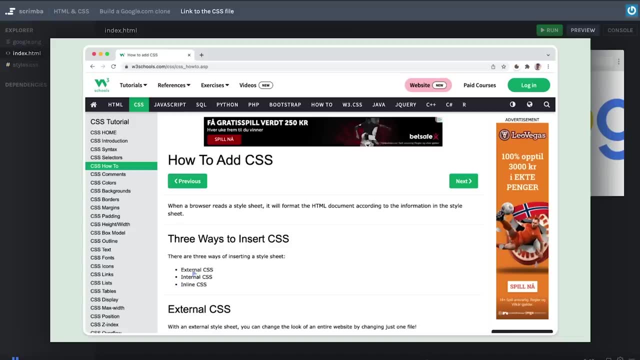 type how to link to CSS into Google and click at the top result. This happens to be a w three schools article. Here you can see that there's a few different ways you can import CSS into the HTML file, But we're only going to worry about the first one here, called external CSS. 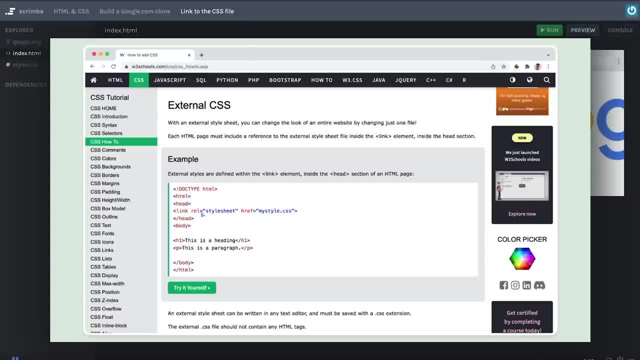 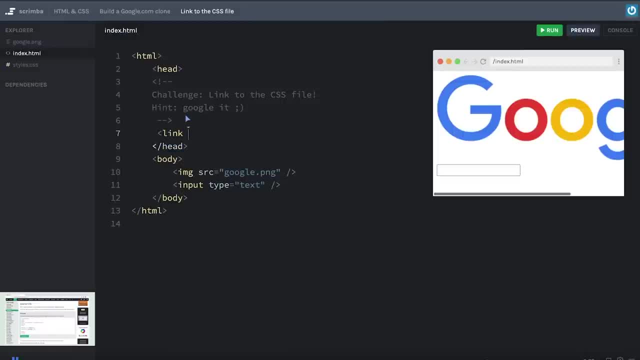 As you can see, if we scroll a bit down, what we do is we type link rel equals style sheet and href with a pointer with the CSS file itself. So we'll do think: well, equals, I'll sheet. href equals styles dot CSS. 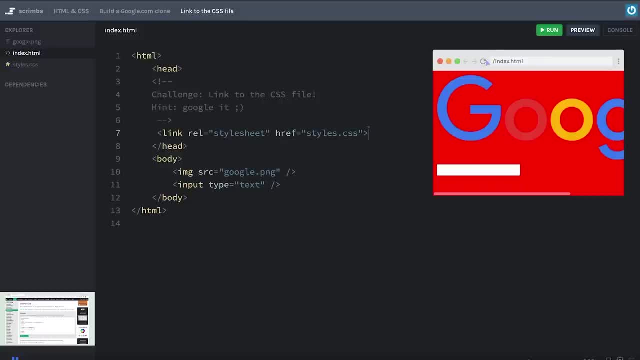 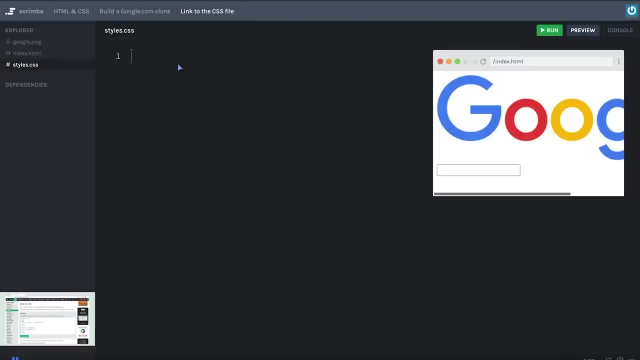 and then closing it. And if we now refresh the browser, boom, there we go. It is red, looking horrible. So we can remove that so that it looks white again. But now we know that we have linked the CSS file to the CSS file, And now we have linked the CSS file to the HTML file, And 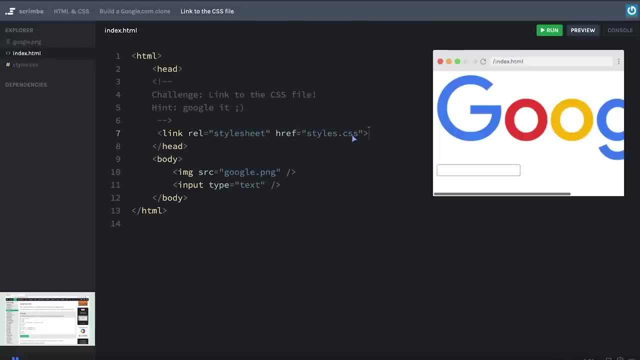 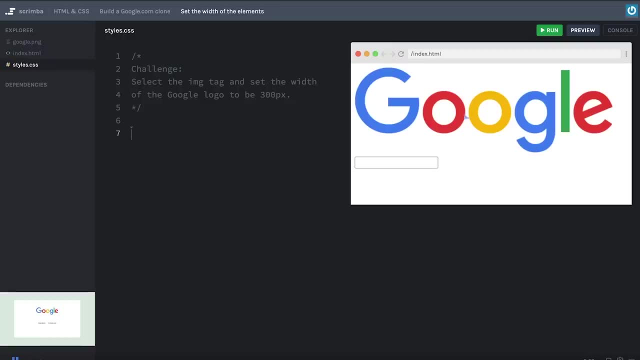 then we can go ahead and put the CSS file into HTML together. So now we're going to put the CSS file in the HTML file together, So we are ready to move on and start styling our page. The first thing we want to fix in our example here are the widths of the elements, Because 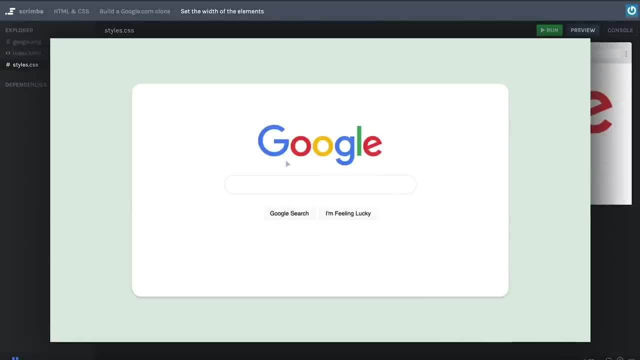 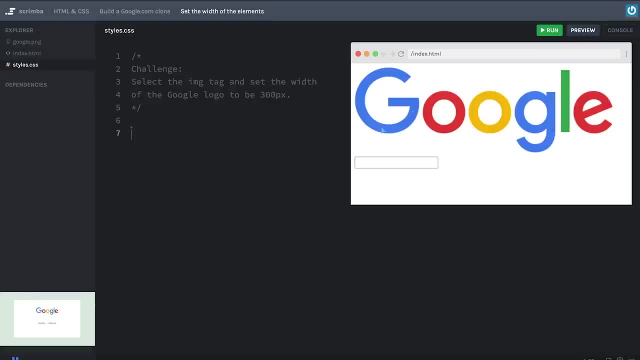 if we compare it to the finished sign, you can see that the input field is meant to be wider than the logo. However, in our example, that's not the case. Quite the opposite, actually. the logo is much wider than the input field, So we need to shrink the logo and then. 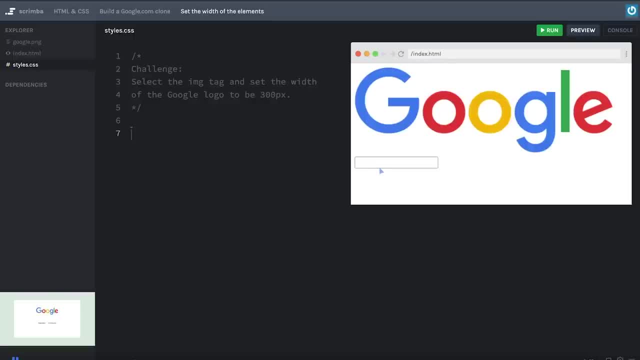 make the input field wide enough. Now, if we want to compare this, we can put in the inside of the logo and then make it wider than that wider. So I'm going to start and do one of these and then you will do the other. I happen. 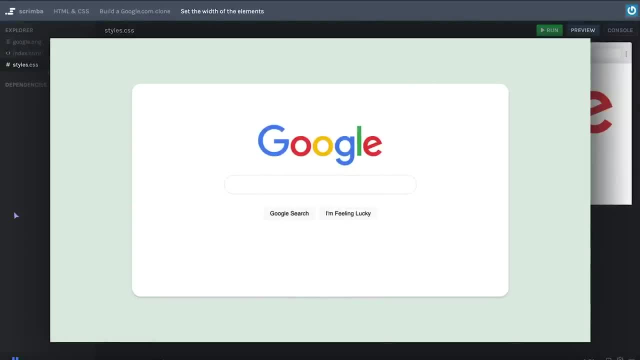 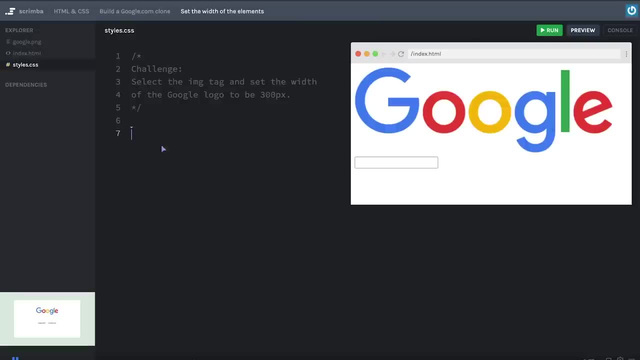 to know that the width we want to have on this input field is 400 pixels. What I'm then going to do is target the input field using the element name and create a CSS selector, just writing input. then open and close curly bracket. then simply write width and 400px. 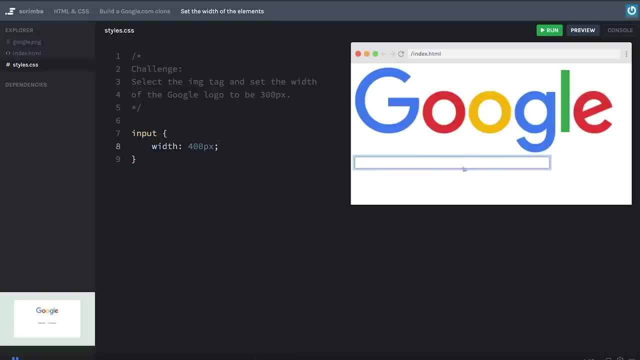 And boom, there you can see, suddenly the input field widened quite a lot And, as you might have noticed, we're using this pixels value here again, which we've used a couple of times already actually, And if you're a little bit confused as to what a pixel is, 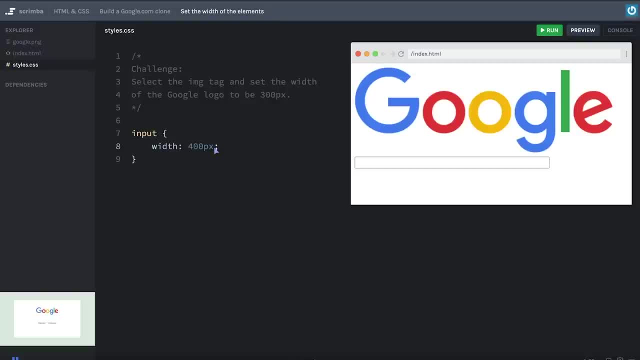 you can think of it as the smallest unit of space that our screens can render. So a pixel is just a tiny square, so tiny that we actually need 400 of them stacked up besides each other in order to get a width of this size. 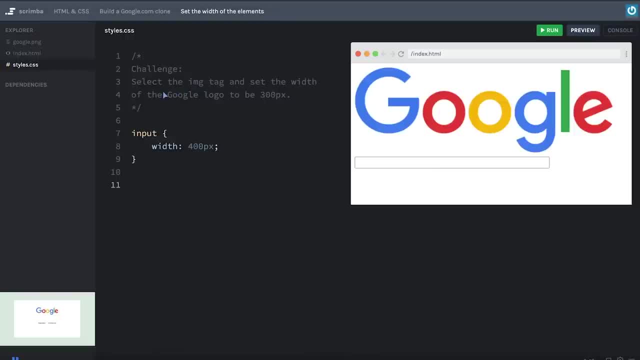 So with that, I want you to fix the width of the Google logo, select the image tag and set the width of the logo to 300 pixels. Go ahead and do that right now, And then I will show you how to do it as well when you return back to the scrim. Okay, let's do this. I'm 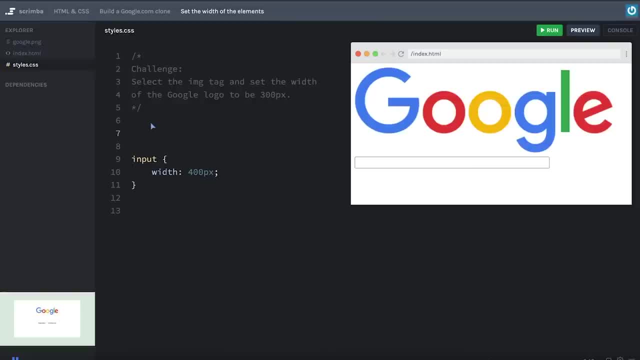 gonna break this down into a few lines So I get some space above the input field and then target the IMG L element to the image element, open up the curly brackets and do with 300 pixels like that. Ooh, we're not quite yet at the finished design, but the ratio between the logo and 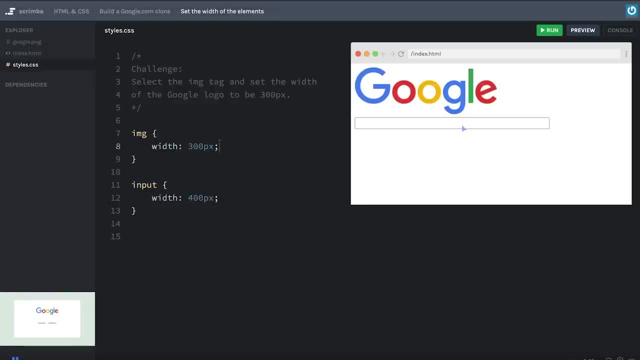 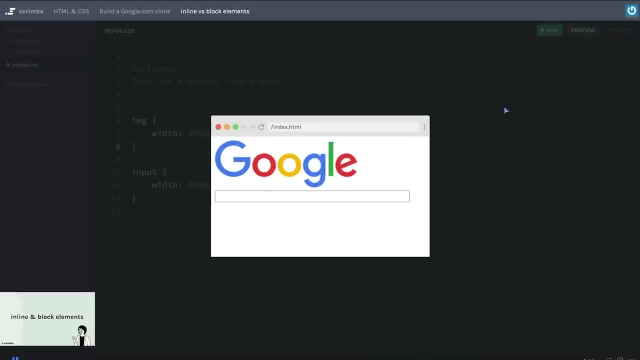 the input field is now a lot better. Great job, Let's move on. Okay, I've discovered a problem with our Google site, which is that if we make the browser really wide, you can see that suddenly the items stack up besides each other, And that's because we've disabled. 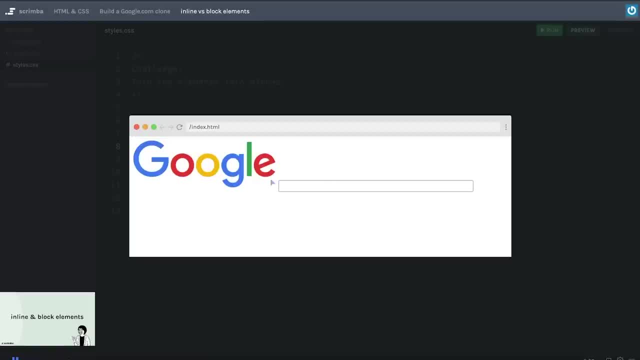 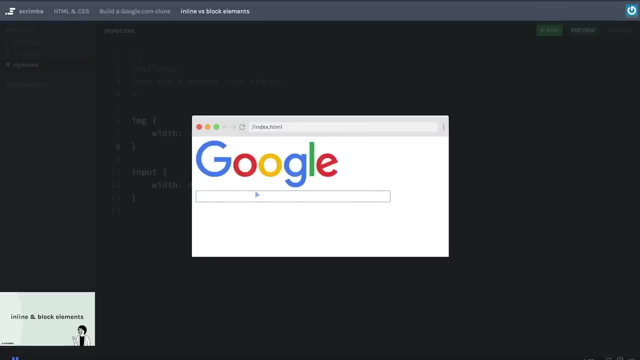 the image element, And the image element is now a very different image element Now, when guides each other on the same line, And that's obviously not the kind of behavior we want. we want them to always be stacked on top of each other And in order to fix this, you 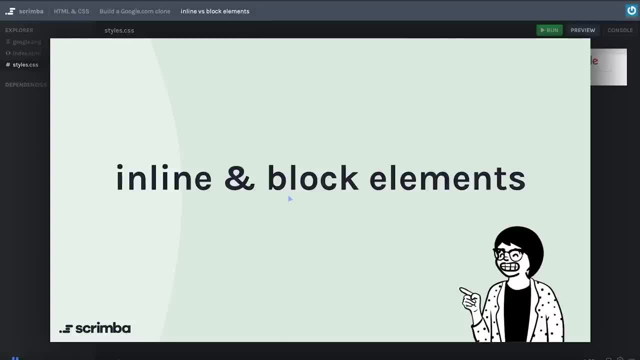 have to learn about inline elements versus block elements, And that's best understood through the lens of an example. So let's say that you, for example, have a collection of things you want to showcase. you could be like George Franson, for example, and collect. 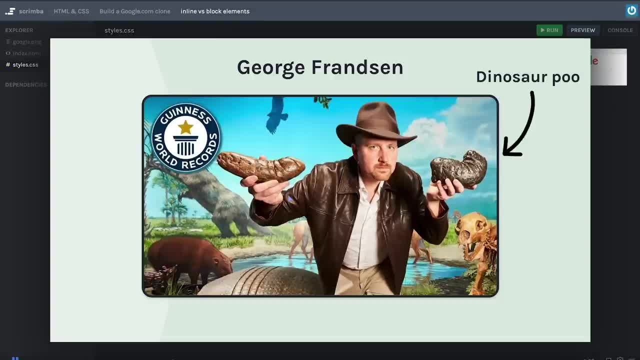 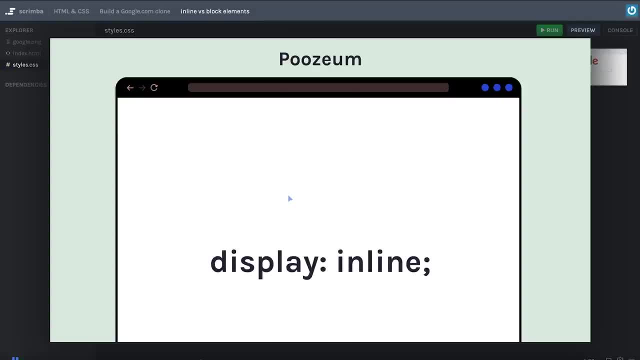 dinosaur poo. he actually has the world's largest collection of fossilized feces And naturally he wants to exhibit them in a museum. And if he were to use display in line on his images they would stack up besides each other like this, So kind of like in a line: 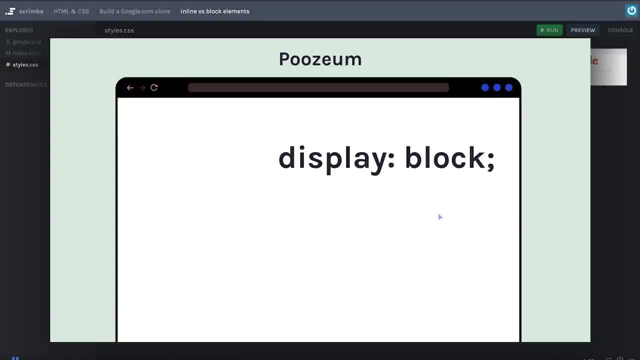 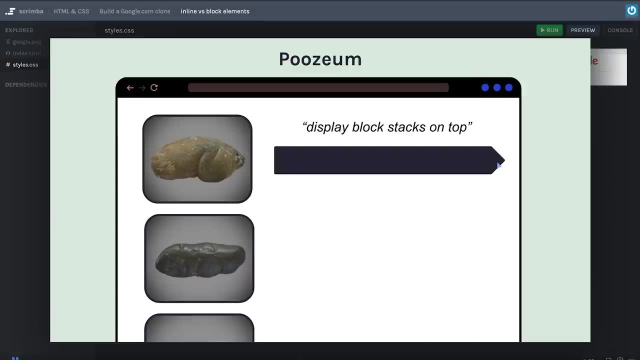 horizontally. However, had he used display block on his images, then they would stack up on top of each other. So rule of thumb is display block stacks on top. Another way to look at this is that the block level element locks out the rest of the available horizontal. 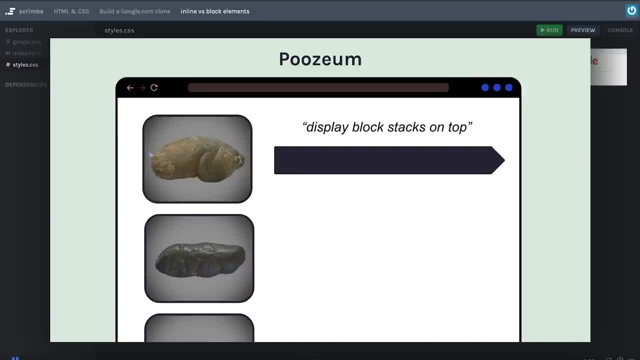 space So that nothing else can be placed there, And that is regardless of how wide this images. the content itself display block requires control over all the horizontal space in its given container. So when this block image is placed here and you add a new image, it 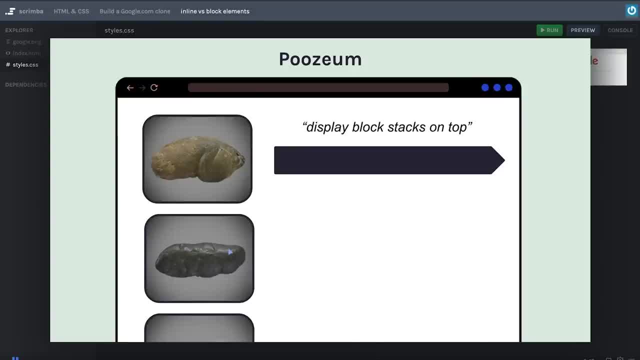 would have to be placed underneath the previous one, And if it is display block as well, it'll block out the rest of the available horizontal space, and the next image have to be placed below that one again, and so on. So the solution is obviously to turn these elements into blocks. 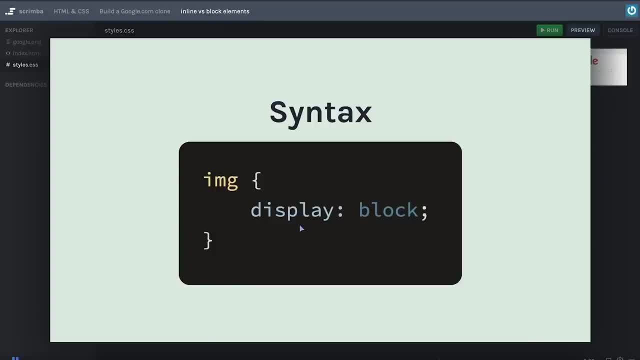 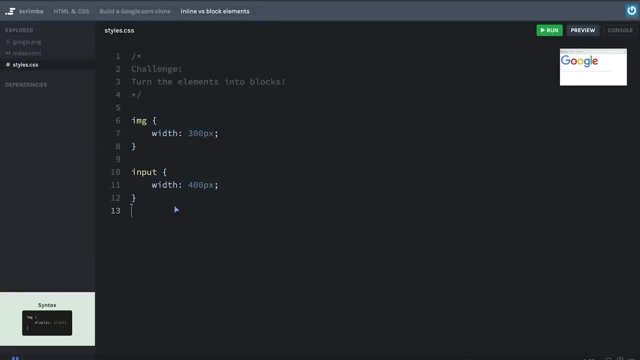 And I'm just going to give you the syntax here. This is how you write it: display colon block. Go ahead and do that for both of these And observe what happens to the example when you make the browser wide. Good luck, Okay, let's do this. So I'll do display block up here And the same here. If we look at 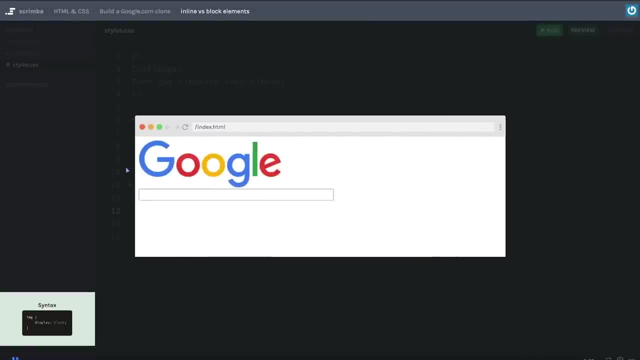 the browser, seemingly nothing has happened. However, if we now make it wide, you can see: yes, no matter how wide this image is, it's still going to be placed on top of each other. No matter how wide the browser is, these will always stack up on top of each other. 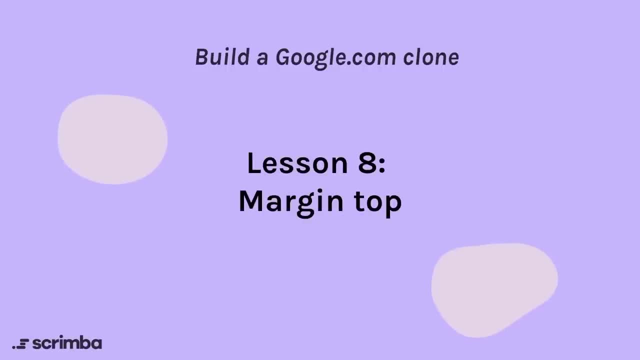 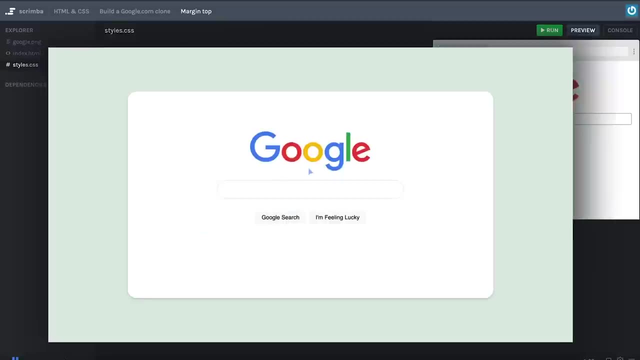 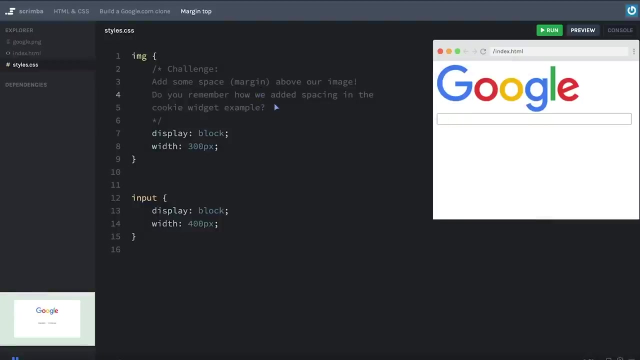 So great job, Let's move on. The next thing we need to fix is the lack of white space above our Google logo, Because if we take a look at the design here, we want quite a lot of space in between the top of the browser and the logo, And I'm not going to tell you how to add that, But if you can, 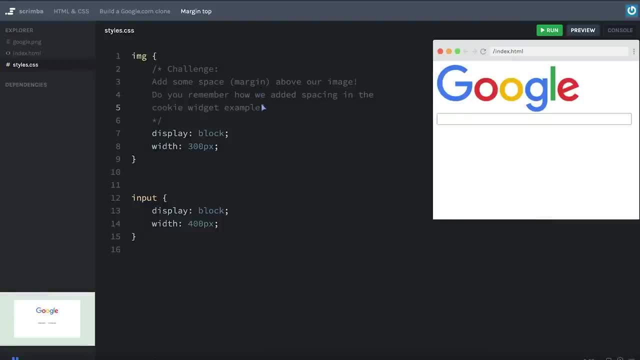 think back to the very first scrim in this section. we added some space above the text in our cookie widget, And that specific space is called margin, or margin top to be specific. So your job is to add some margin on top of our image. Right here you can start on line seven, So there. 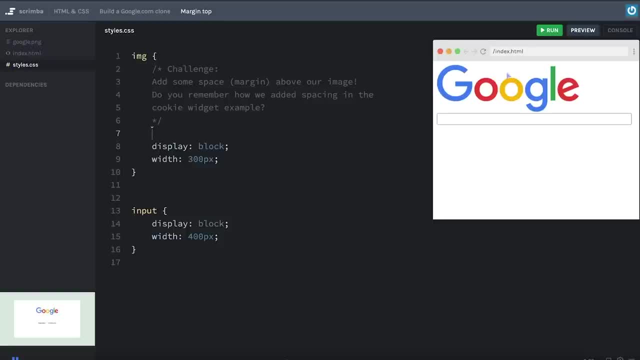 are example here: gets some breathing room, some white space above the logo and the input field. Go ahead and give this one a shot, And then I will, of course, show you the solution when you return back to me. Okay, hopefully that went well. If not, no worries. I really 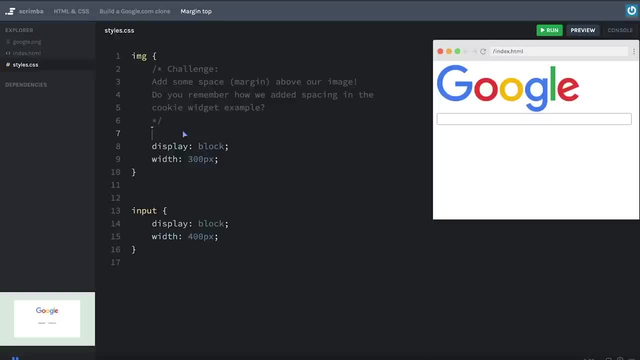 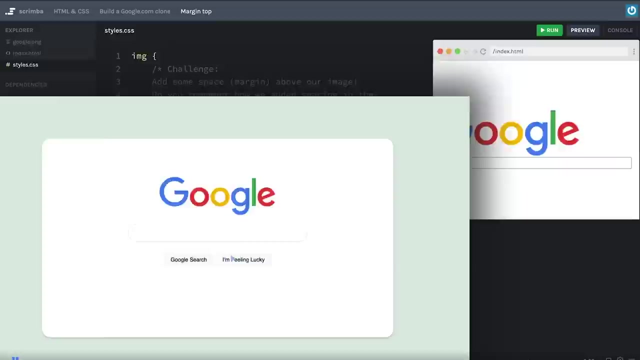 pushed you out on thin ice here, So it's completely okay if you didn't remember that. the property is called margin top And what you add there is a pixel value, So, for example, 100px, And there we go. We've now added a margin on the top of our image, And while we're still quite 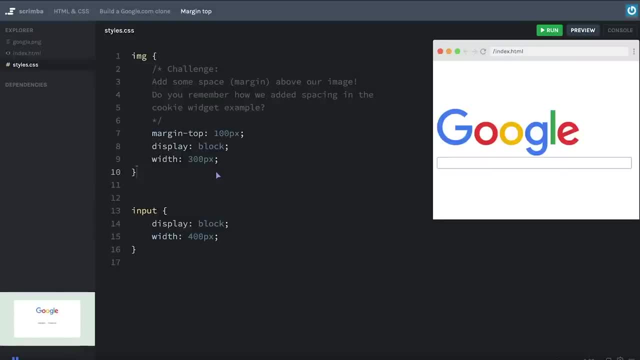 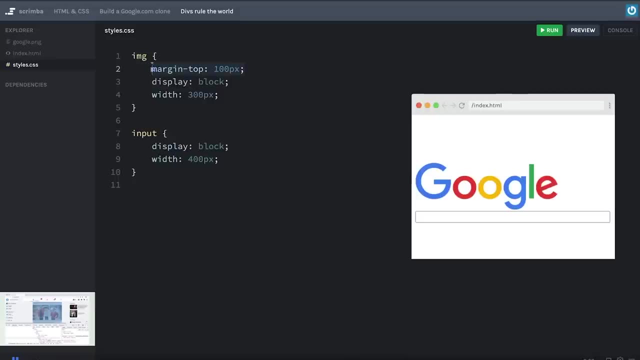 far off from our provided design. here we are getting closer. Great job, Let's move on Now. while it totally works to add the margin top, directly on the top of our image, we can also add a margin on the top of our image. So we can add a margin on the top of our image. 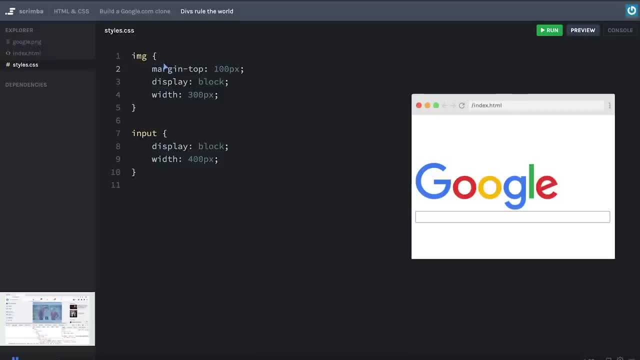 And while we're still quite far off from our provided design, here we are getting closer, So we have a margin on the image here. we'd most likely not see professional developers do this, Because what they do instead is wrap these two elements in some kind of container. 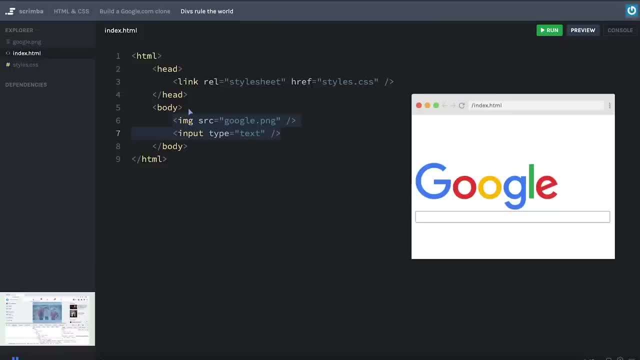 and then control the positioning of these elements indirectly via that container. And in order to do this, you have to learn about the div. I'm going to create an opening div and then indent these two And then a closing div below here. Now, if we run this code, seemingly 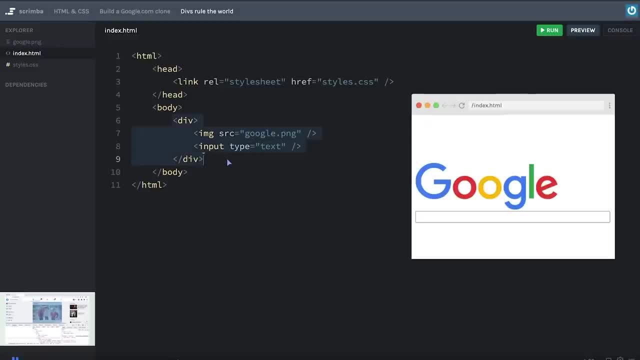 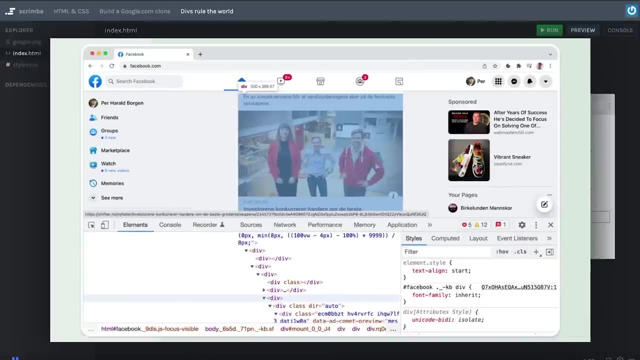 nothing has happened Because the div actually does very little in itself itself, though it is indispensable for web developers. Just to show you how important it is, Let's take a look at Facebook and my timeline. Here I've opened up DevTools and 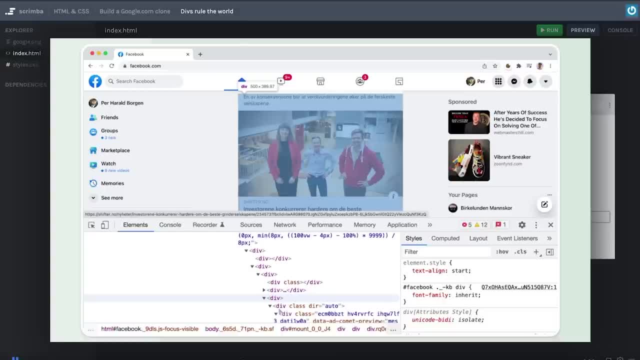 inspected one of the timeline items And you can see it is actually a div inside of a div, inside of another div, inside of yet another div, inside of a div, inside of a div. who divs really do rule the world, So it's important that you learn about them And the way we'll 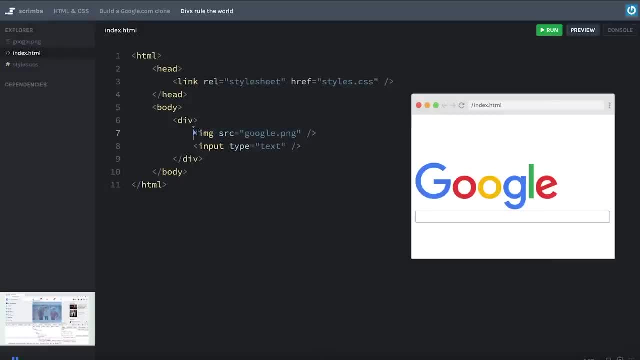 use this div now is by removing the margin top styling from the image and then add it to the div itself. And the reason this is important is let's say that, for example, Google decides to create a video here instead, or a interactive doodle or some kind of game. 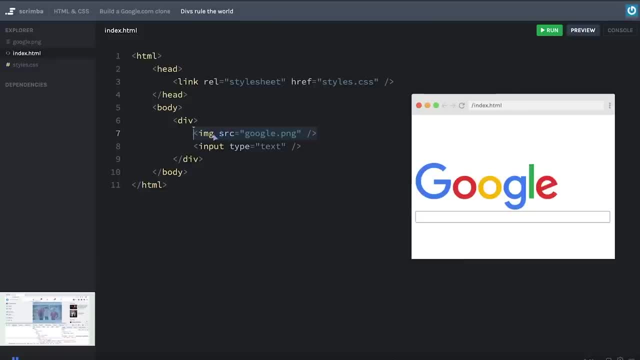 they often play around with the Google logo. Well, if so, it's a really bad idea that it is the image itself that controls the margin from the top of the browser and down to the content, because that image might be removed, So a solution that will get you into trouble in the future. So what we'll do here is we'll. 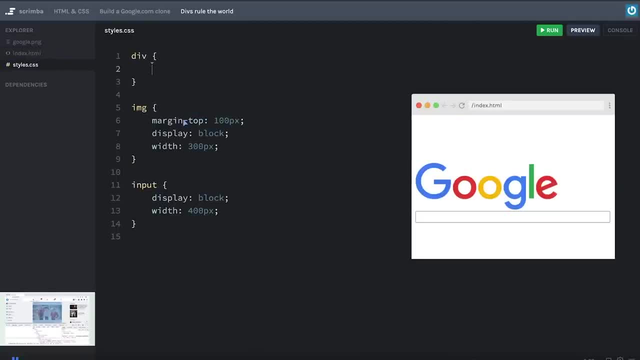 simply instead target the div and then remove the margin top from the image and boom, it has popped up. Now we lost all of our whitespace, But if we add it back to our div we are back at the design we started out with. seemingly nothing has changed, But, as you know, we have. 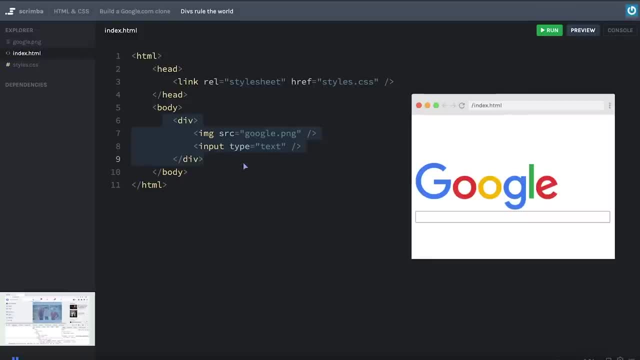 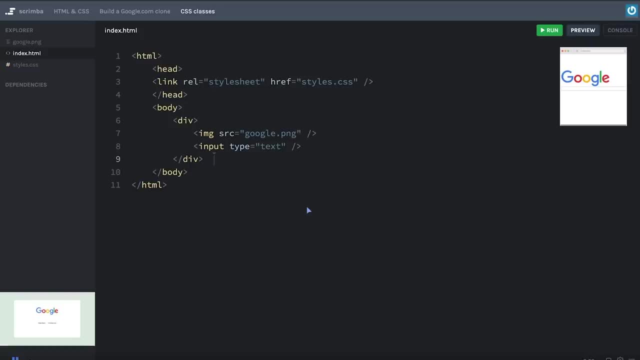 a better HTML structure. So we have definitely made good progress here. So with that, let's move on to the next trim. The reason you need to learn about classes now is because our current setup, where we simply have the elements like this and then selecting the elements, 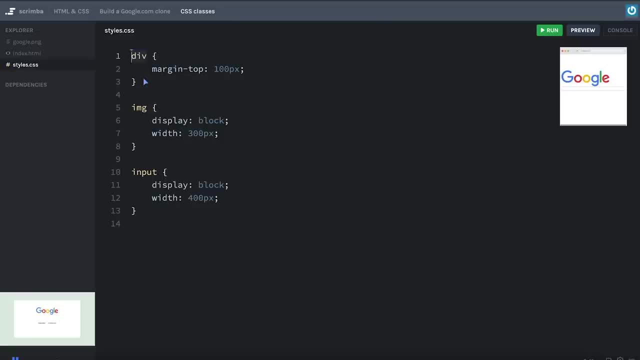 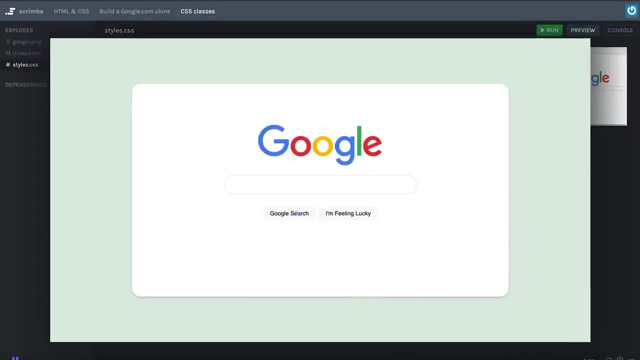 using the element selector in CSS will give us bugs down the line, Because when we add the two buttons beneath the input field, we'll actually wrap these two in a div as well, And let's see what happens at this point. What I'll do now is simply add a div to the 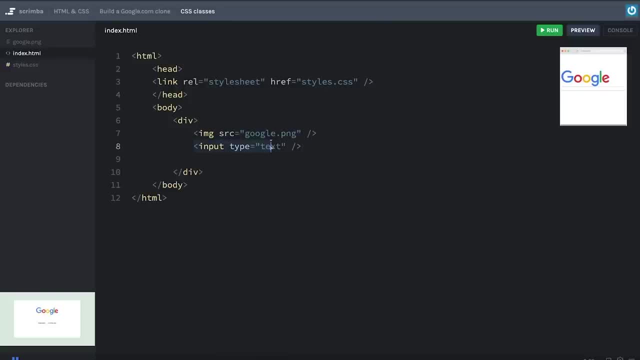 input field And then we'll add the HTML for these buttons down here beneath the input field. So it is a div with two buttons inside of it, And then you can see we are closing that div- the inner div- And then we are closing the outer div. Let's run this code And oh, 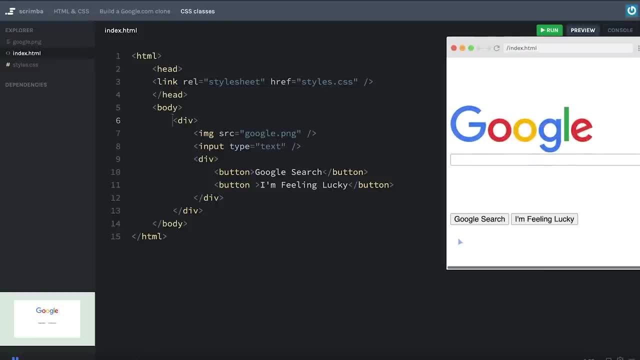 wow, What you can see is that the spacing between the input field and the buttons is totally off, And that is because our CSS element selector here selects any div it can find and applies the margin top to it, So it doesn't just select the first one, but it can select. 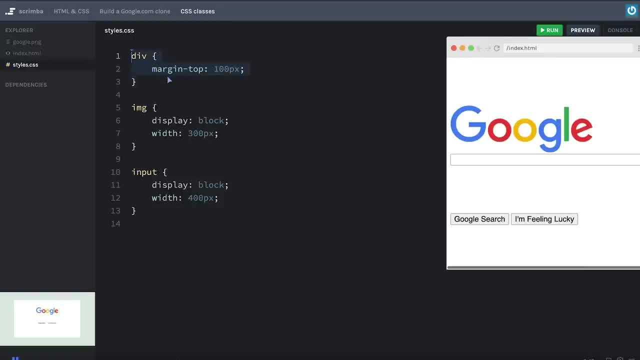 1000s of devs. So this is a very generic solution and likely not something we want to use, as we want to have multiple divs with different types of styling in our HTML element. So let's now instead fix this by doing the following: All right class equals then, for example: 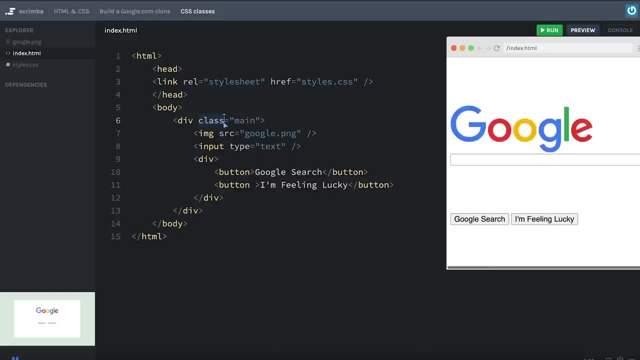 main. this here is an attribute called class, So it's built into HTML And this here is the name I'm giving my class. I want to call this div my main element, And now the way I select that in the CSS is by, instead of just writing the element name. 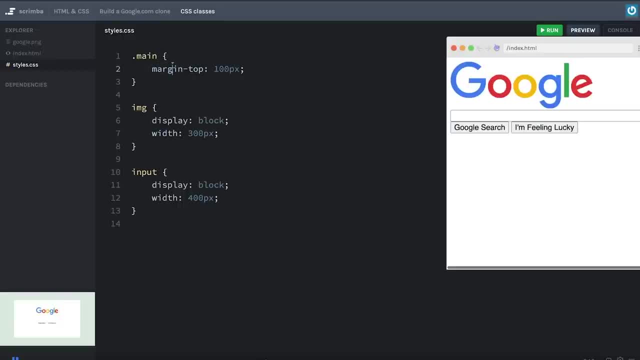 simply doing dot main like that. Now, if I rerun this code, you can see now the margin top is only applied to the outer div, our main class, and not to the div which wraps the two buttons. So that is exactly what we needed. 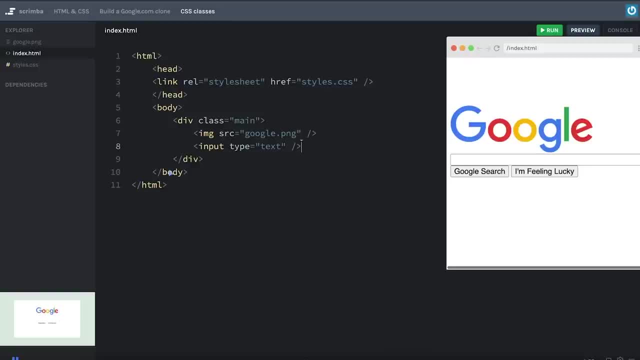 I'm going to remove these two buttons here because we don't want to deal with them just yet, And then I'm going to give you a challenge. First, you're going to add a class to each of these two elements, that is, the image and the input. you have to decide what you will. 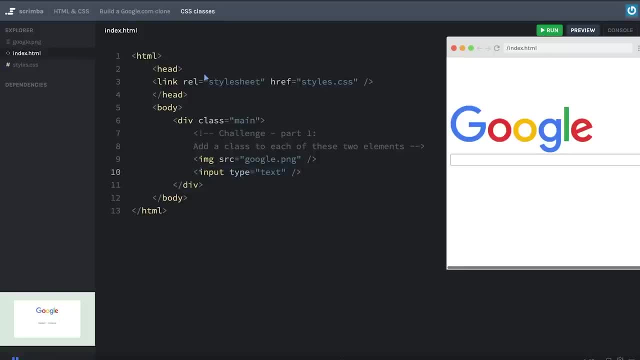 call the two classes, but make sure to give them different names. And then you're going to, in the CSS, replace the element selectors with class selectors. So that is the IMG selector here And obviously the CSS class selectors. you're going to replace them with as the ones you. 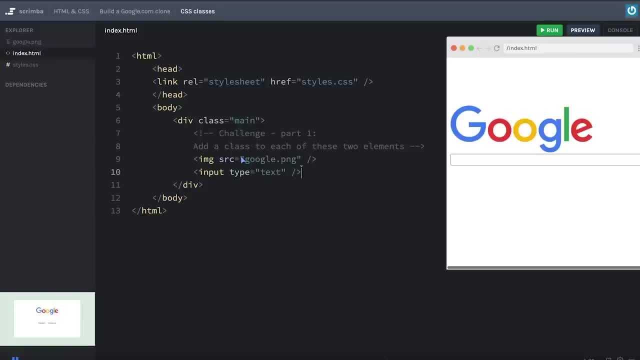 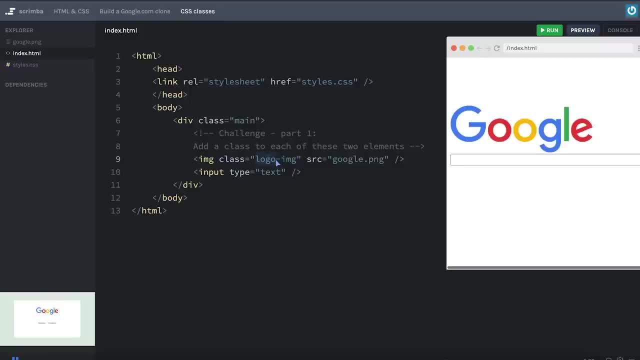 equals. So here I'm using a Convention where I'm first giving my class a descriptive name And then using a dash, and then specifying the element as well. This is an IMG element, but it could have been, for example, an SVG or something else. Now, I don't expect you. 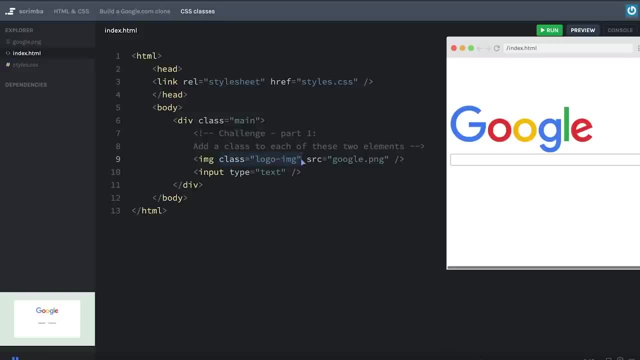 to have followed the same convention. there are plenty of CSS conventions and it doesn't matter at all what you use In your example. you can call your classes whatever you want. Okay for the input, we'll do. class equals search back Input, like that. So we've now. 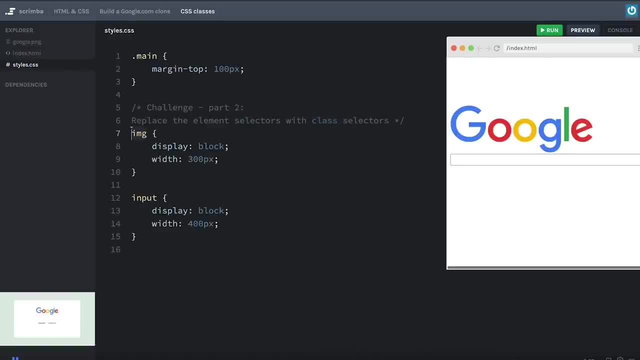 called our first class. let's just go ahead and call this class equals. Now I've already that. Okay, let's move through the CSS, then I'll replace this with art. Now you can see it broke the layout because this styling now is not applied to any element, So we need 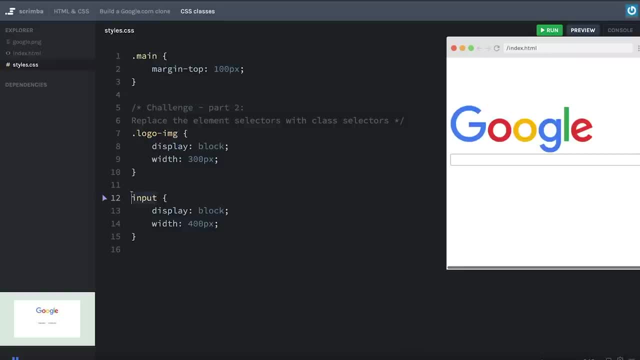 to do logo dash IMG, like that, And here do dot search dash input, And there we have the exact same example. didn't change at all, But we now have a more flexible solution that scales better. So great job solving this challenge. Let's move on. 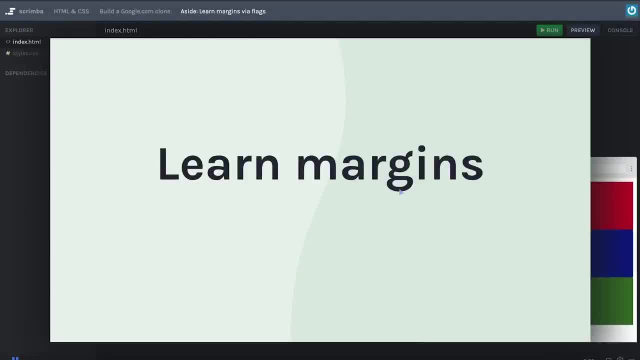 Now it's time to take a closer look at margins, And you've already dipped your toes into this, as you have used margin top, So you might have some intuition about what margins do. However, now you're going to learn it properly through creating flags with CSS, Because flags 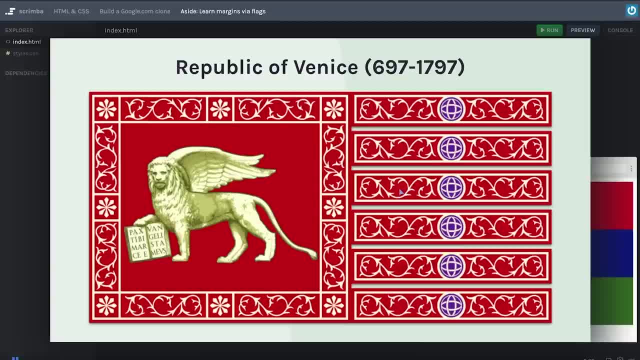 are just awesome. I mean, take a look at this flag here, for example, from the Republic of Venice, a state which existed for over 1000 years in Europe, And it contains, of course, a flying lion holding a book. What's more natural than that, Or this one, right? 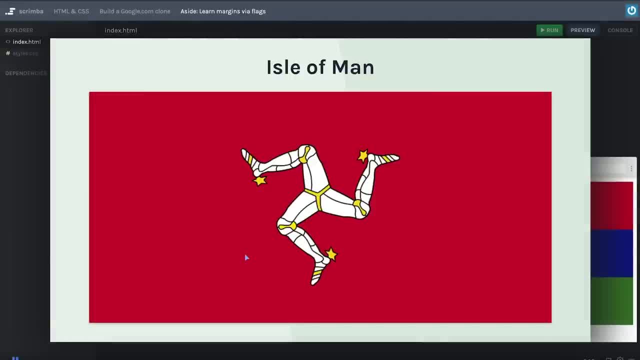 here for the Isle of Man. I mean, have you ever seen a more creepy creature than this three legged thing right here? Imagine having that thing running after you. That would not be fun And this flag would be really hard to create in CSS actually. So we're not going. 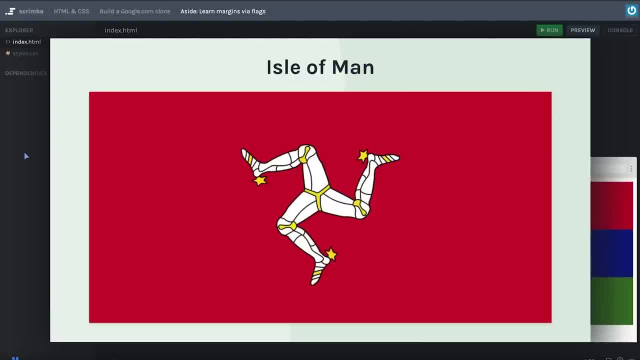 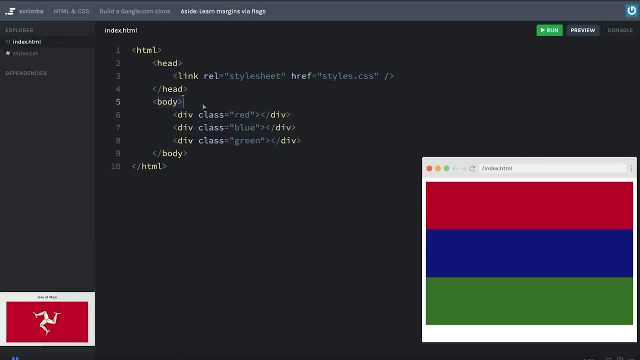 to create this, this one. we're going to start off at a much easier level with just some very simple shapes, So let's have a look at those. actually, here is what we're going to work with. As you can see, there are simply three divs inside of the body tag And each div has a class red. 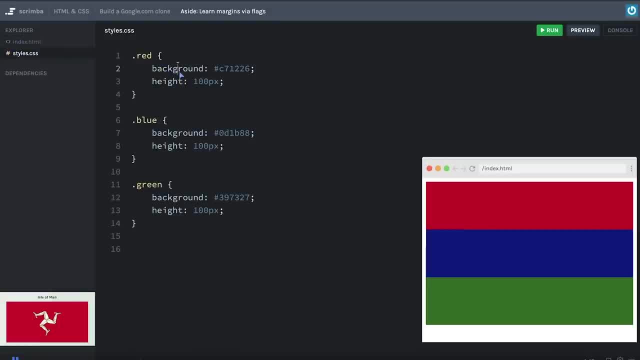 blue or green. If we check out the stylescss, you can see that these three classes apply a background color to each of the elements and sets the height to 100 pixels. And here we have the result: three rectangular boxes that are stacked on top of each other, And 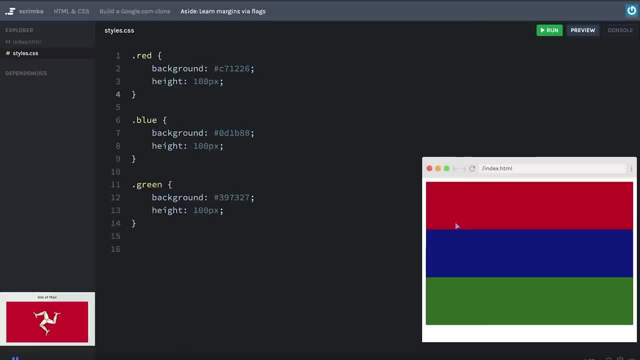 that tells us that these are display block, because display block stacks on top. there's one thing that bothers me here, And that is that we have a little bit of white space around the three items. Why is that? Well, actually it's because our browser is trying to help. 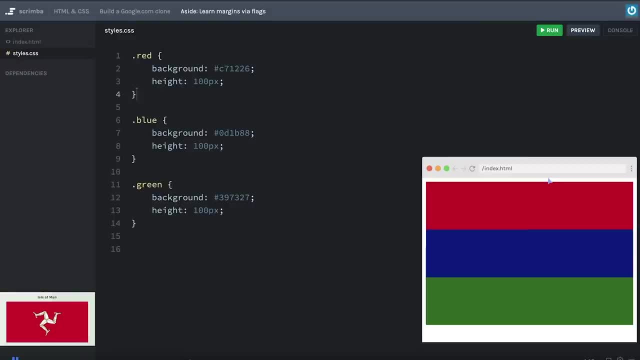 us here. It's assuming that we want a little bit of space around the body tag so that these three don't touch the edges of the browser. So what's actually going on here in code is that the browser targets the body and sets a margin of eight pixels. you notice, when I added this, nothing. 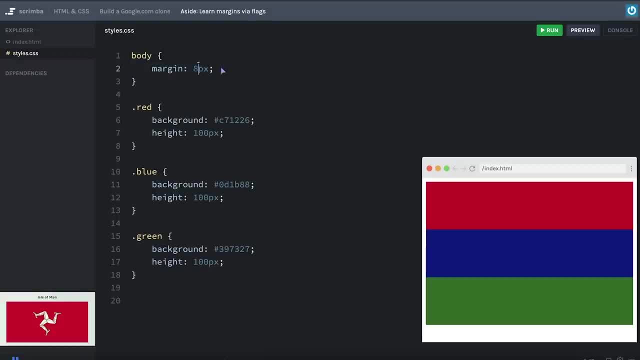 changed. So if I remove this it's still the same meaning that this style here is applied automatically. So that means that margin is actually the space around an element. Because now if we change this to zero, boom, there you can. 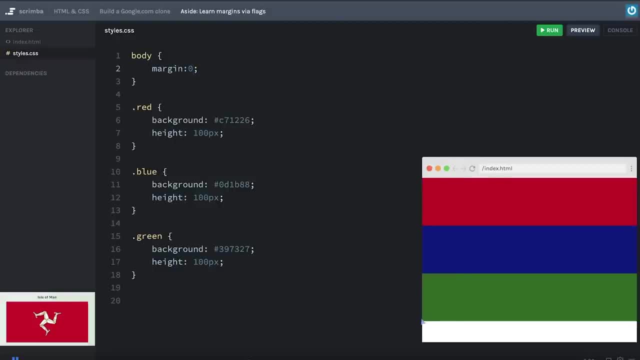 see, suddenly our divs touch the edges of the browser. Now here at the bottom they stop after 300 pixels, since we've told them to. So this margin zero here seemingly didn't change anything at the bottom, because the bottom contains whitespace anyway. if we make 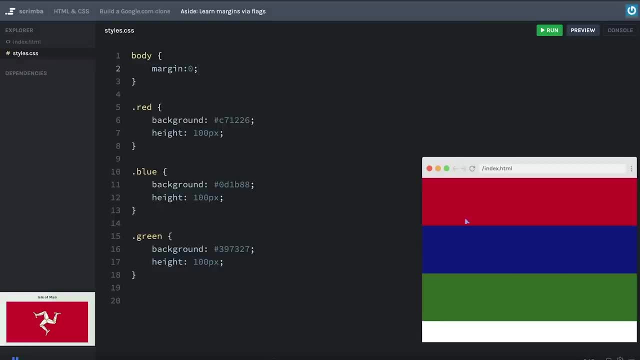 our browser tall enough, But anyway, that's a digression. Let's get it back so that the browser is completely filled up with these three items. And now let's play a little bit around with margins. So what do you think will happen if I add a margin top of 10 pixels? 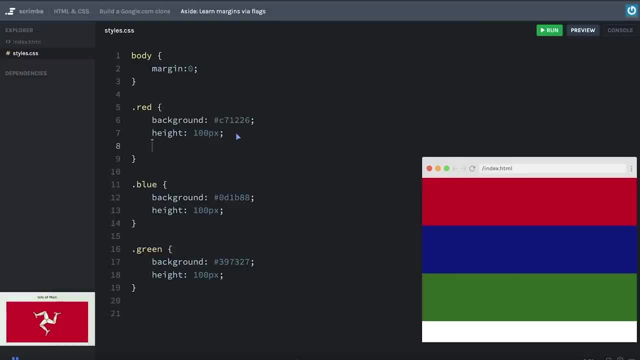 on the red here. Take a guess. Okay, margin top: 10 pixels. boom, it added 10 pixels on the top. what do you think will happen if I add margin left 10 pixels as well? Let's try it. Okay, so it added 10 pixels on the left hand side. it's only on the red side. 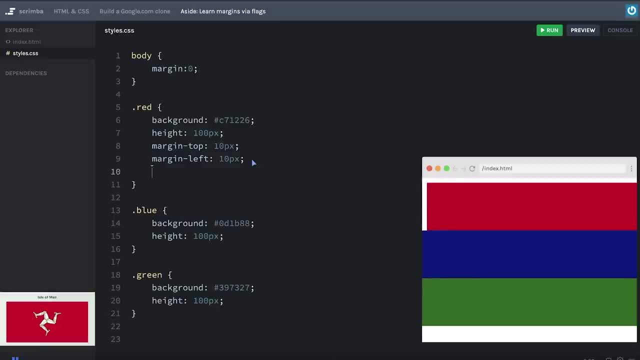 red rectangle, not the blue or green rectangle. Likewise, if I do margin and pixels, that's 10 pixels to the right hand side as well. If I do 100, it eats up almost a third of our red rectangle. Okay, so now it's your turn. I want you to add 100 pixels of margin. 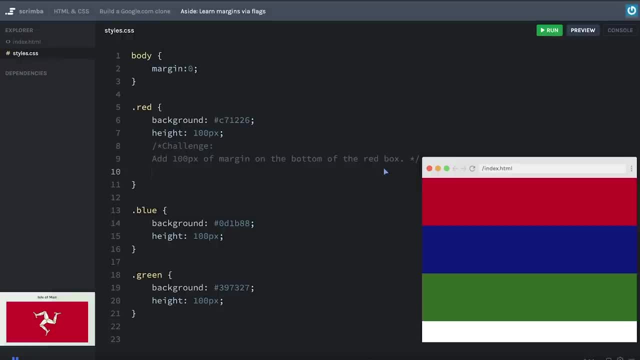 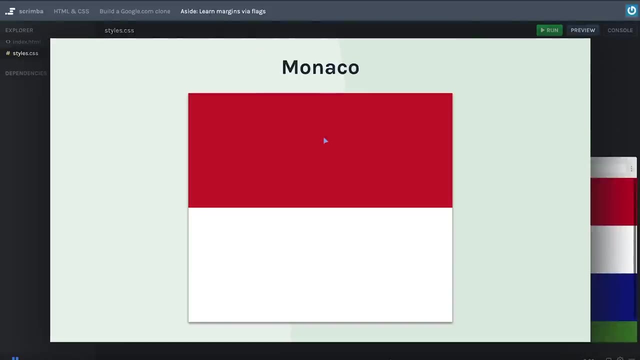 on the bottom of the red box. So go ahead and give that a shot right now. Okay, if you did margin bottom 100px like that, I want to congratulate you because you just created the flag of Monaco. really good job creating your first CSS flag And. 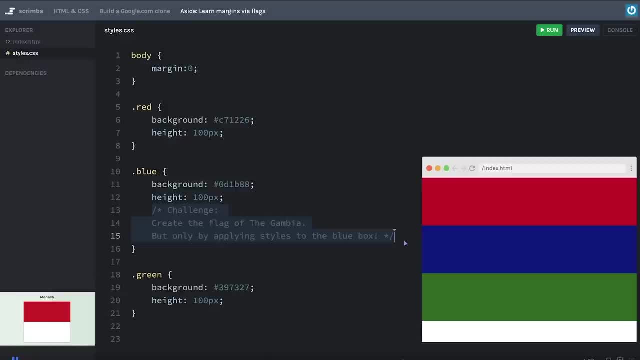 now let's do that yet again. Here is your challenge: you are going to create the flag of the Gambia, And here we have that flag. However, there's a catch: You can only do this by applying styles to the blue box, So by adding margin to this. 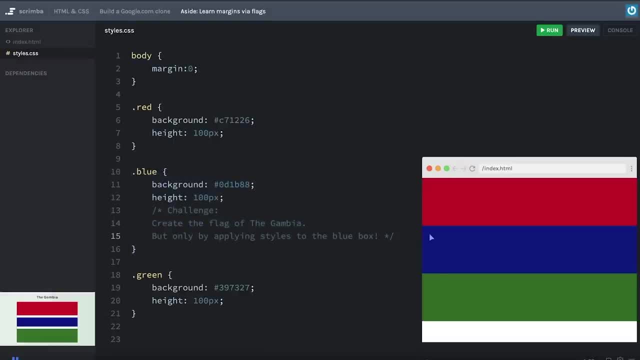 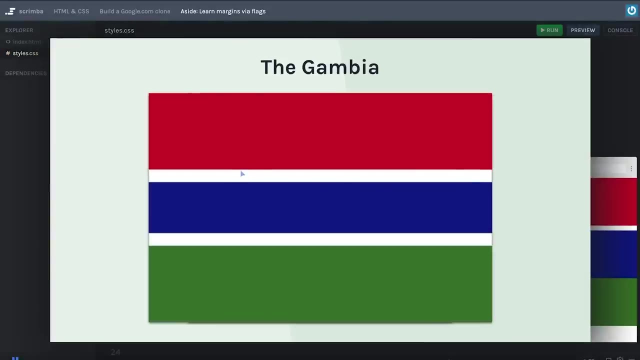 CSS rule right here. So go ahead and give that a shot right now. Okay, hopefully that went well. The way to do it is by doing margin top. Let's try 10 pixels and see. Actually, I think we want our white space to be a little bit more than. 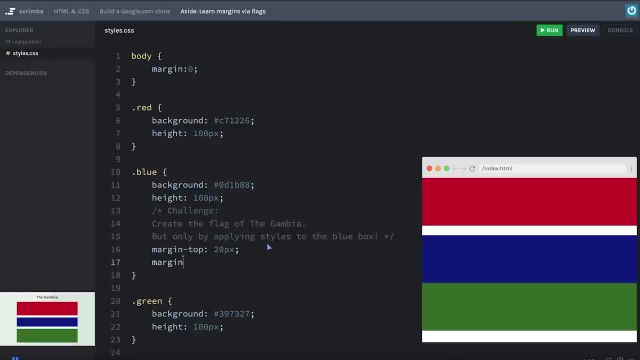 10 pixels. So let's do 20 like that, And then margin bottom as well: 20 pixels, And there I think we have 10 pixels. 10 pixels, And there I think we have 10 pixels, And there I think we have 10 pixels. 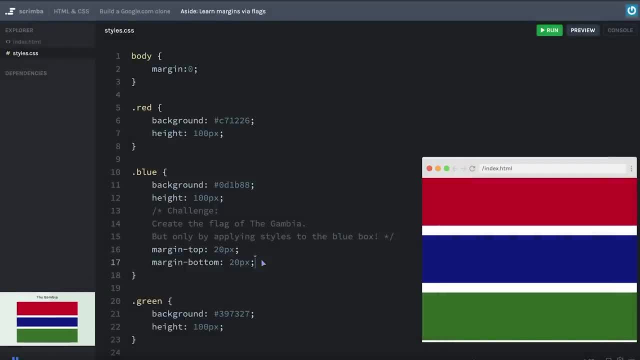 10 pixels, And there I think we have 10 pixels. And there I think we have 10 pixels. And there I think we have a pretty good flag for the Gambia. Now, before we move on to our Google project, there's one little weird thing I want to tell you about margin. 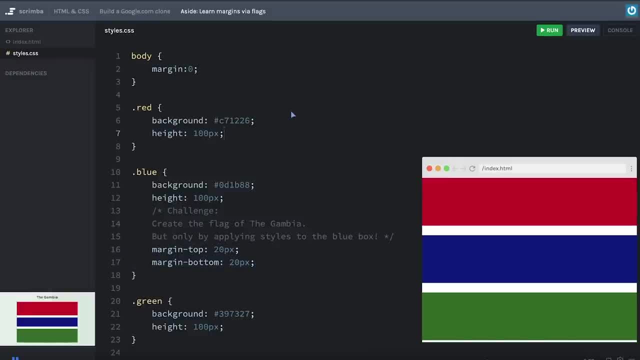 top and bottom. Because what do you think happens if I add, for example, margin bottom of 15 to this red element here? Well, according to my logic, the margin right here would be 35 pixels, because we added 20 pixels on top of the blue, and if we add 15 at the bottom? 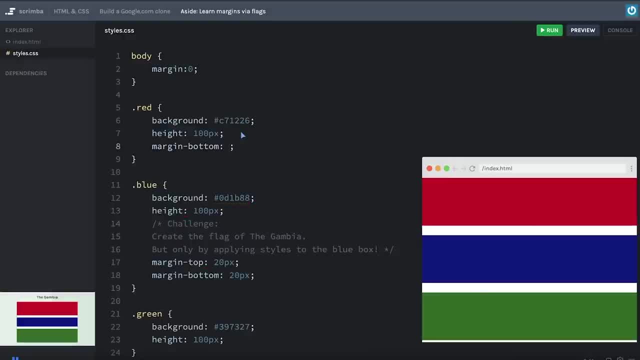 of the red one, that should be 35 pixels in total. However, now that I added this, nothing happened, And that is because margin top and margin bottom will, in many situations, collapse into each other, So that as long as this margin is smaller than this, this will take precedence, And it's only when this one becomes larger. 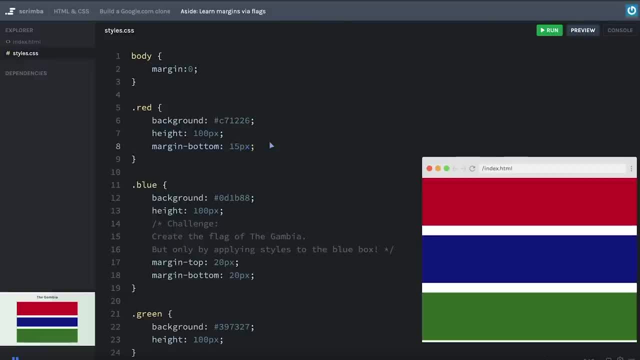 for example, 25, that it will kick in, So let's take it back to 15.. And to make things even worse, there's actually scenarios where this doesn't happen. However, digging into that is outside of the scope of this lecture. I just want you to be aware of it, Because 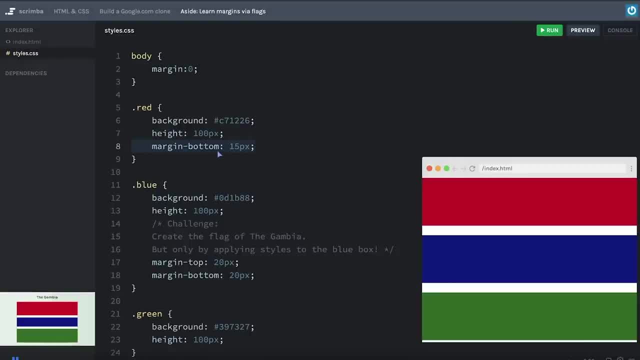 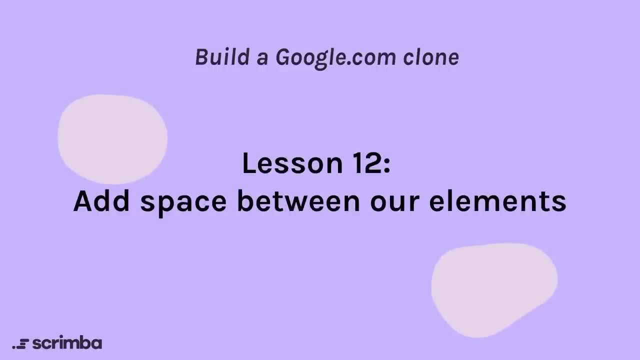 if you're suddenly in a situation where your margins don't seem to add up is probably because of so called collapsing margins. Okay, with that, let's move on. Okay, we're back at our Google project. I want to give you a quick challenge. I want 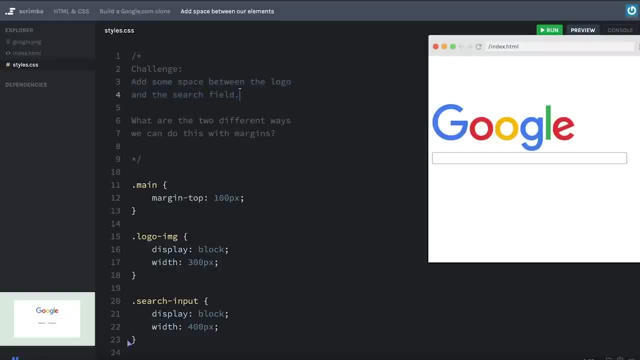 you to add some space between the logo and the search field Because, as you can see here, there's some spacing in between the elements in our design. However, in our project now they are crammed together. There are two ways you can do this: using margins. 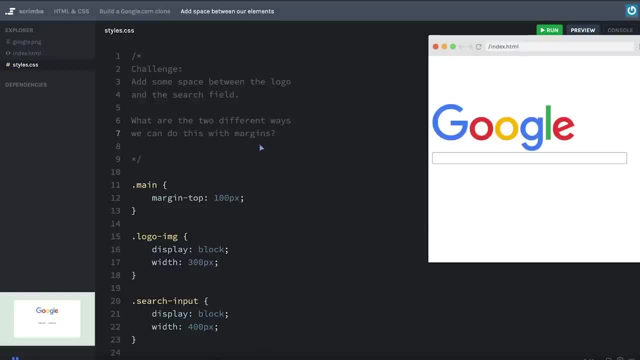 And I want you to think about which two ways that is and choose one of them. Go ahead and do this right now. Okay, hopefully that went well, let's do it. So you can either add a margin bottom to the logo or you can add a margin top to the search field. I'm going 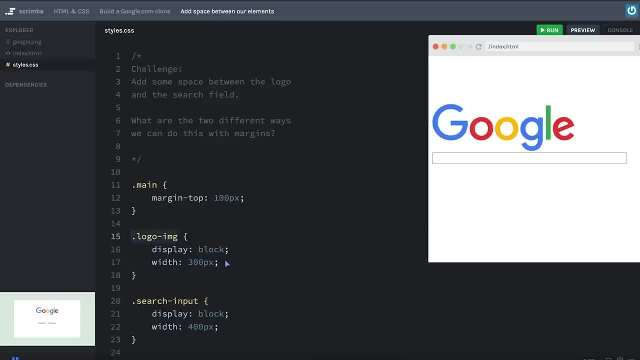 to go with adding margin bottom to the logo, As I think either way is as good as the other at this stage. margin bottom, and how much do we want to add? Well, let's try 20px. And yeah, as you can see, we've got some spacing. 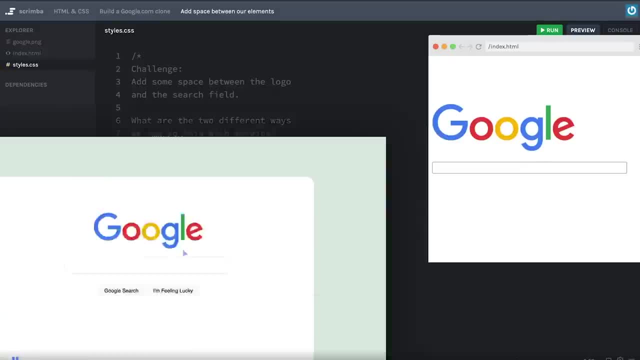 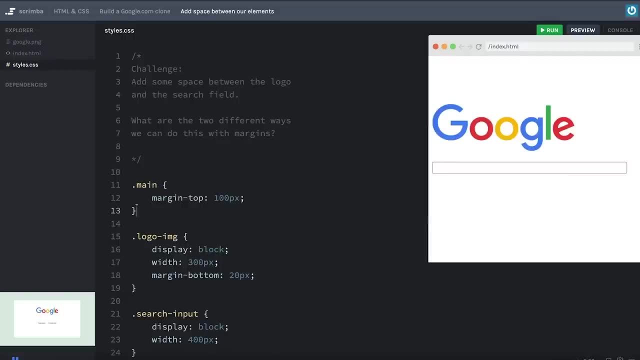 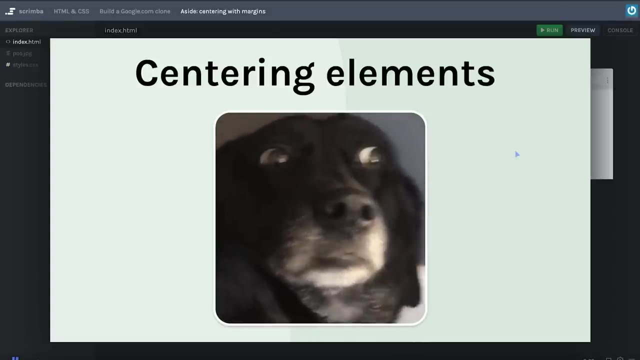 the bottom of the G is not touching the top of the input field, And if we compare that to the example, I think it looks more or less the same. So great job, Let's move on. Okay, now you are going to learn about centering elements in CSS, And that is a scary topic. 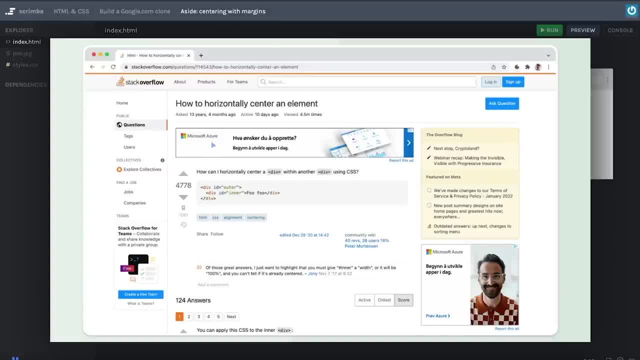 for a lot of developers. So scary that this stack overflow question about how to horizontally center an element has been viewed 4.5 million times. So if you think this is a little bit confusing, you are in very good company, So don't worry about it. So, with that in mind, 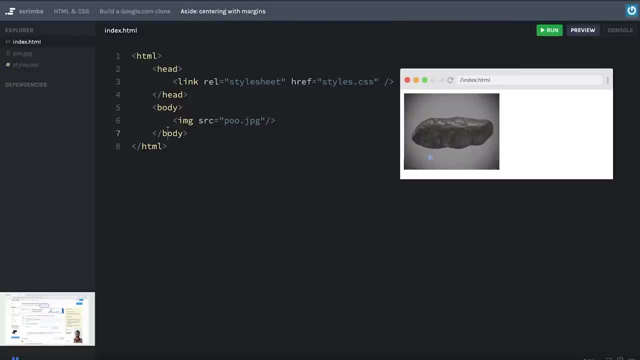 let's move over to our example. you are going to center this dinosaur pool. As you can see in the CSS, it has just one property set at this point, which is a width of 200 pixels. That is because the image is. 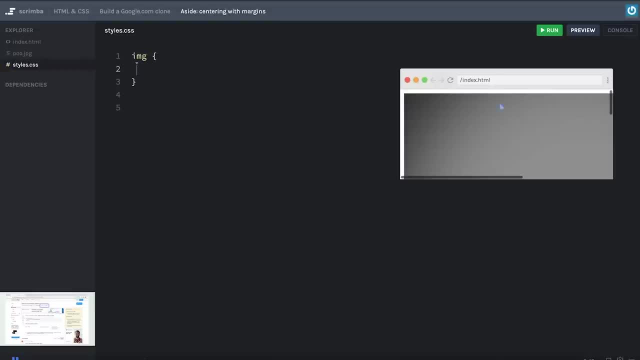 so wide originally that if I don't set that with, it'll just take up more space than we have available. And setting the width of it is actually an important thing in order to center it, because there are three things that need to be in place when we are to center. 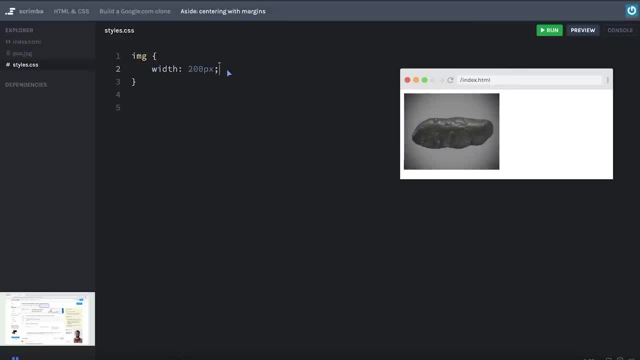 elements with the technique you are about to learn, with margins, And these three components are: first, the element needs to be displayed block, because how is an element supposed to center itself if it doesn't command full control over all the horizontal space, If it's display inline and allows other elements? 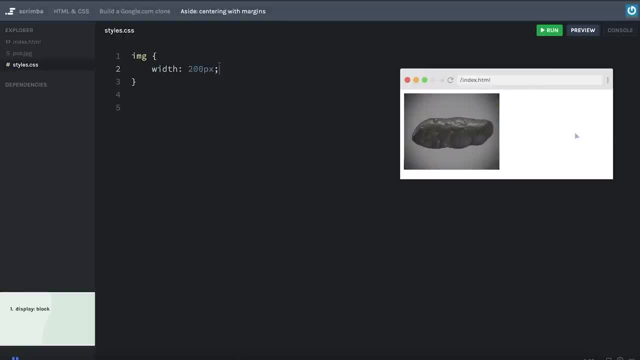 to stack themselves besides the element, well then it won't be able to center itself because that space now is busy with other things. So in order to center this pool, it needs to control all the horizontal space, So it needs this, a block like that. Now, that didn't change anything, But under the hood. 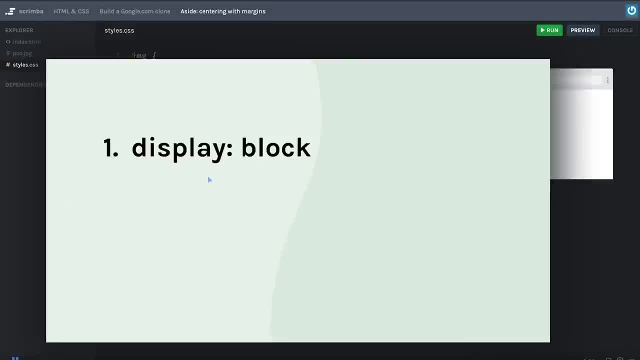 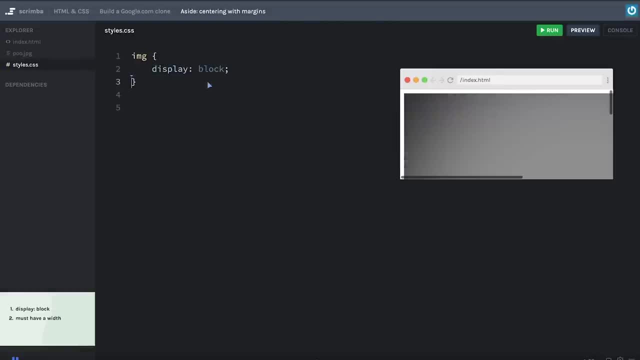 the pool now controls the full horizontal space. Okay, the second part is that it must have a width, And that is what we've done here already, Because how is this item supposed to be centered inside the browser if it is wider than the browser itself? That's often. 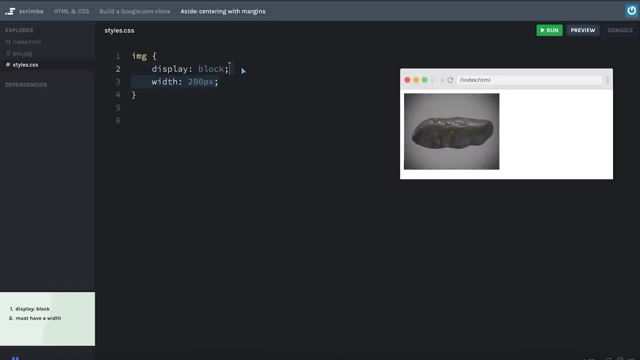 what happens with either large elements or with some HTML elements who just naturally actually expand to take up all the available space in the block. So we have to make sure that our element has a width And finally we set the margin on the left hand side and 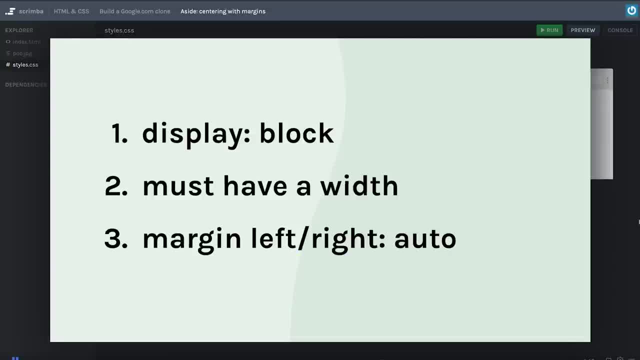 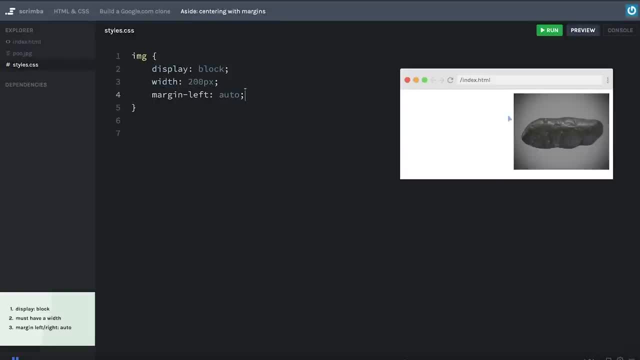 the right hand side to the value auto. Let's just do that Margin left auto. Oh wow, Now it pushed the poo all the way to the right hand side, Because auto here means take up all the available space, And since this is a block, 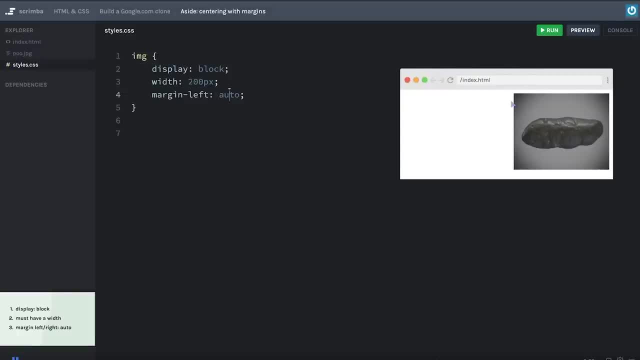 element. the available space is all the space that's left after the poo has taken up its 200 pixels. So just ate up all of this space and turned it into margin. However, at this point margin right enters the party margin right and says: I want the available space. 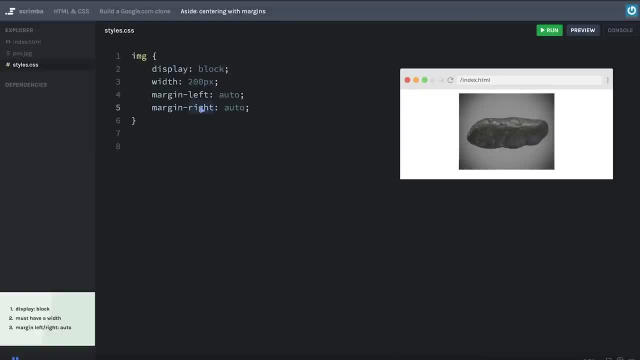 as well, And at that point the margin left and margin right goes into a discussion and decides: well, actually this: there are two of us here pushing on each of the side of the element, trying to get all of the available white space. 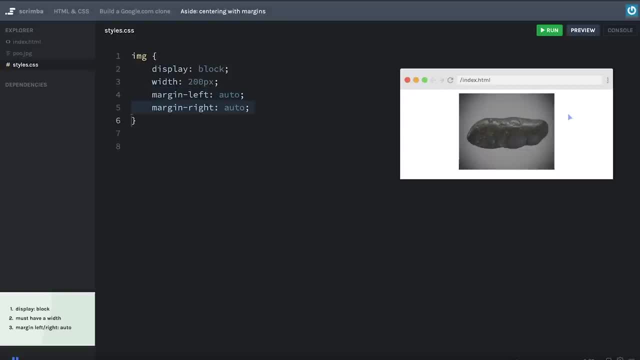 So let's just divide it evenly amongst both of us, And the result? well, it is that the item is centered. So that was a long explanation of centering with margins. If you feel confused, don't worry about it right now. All you need to do is remember these three conditions and 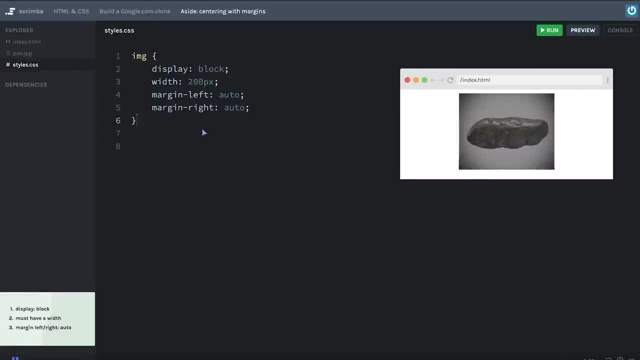 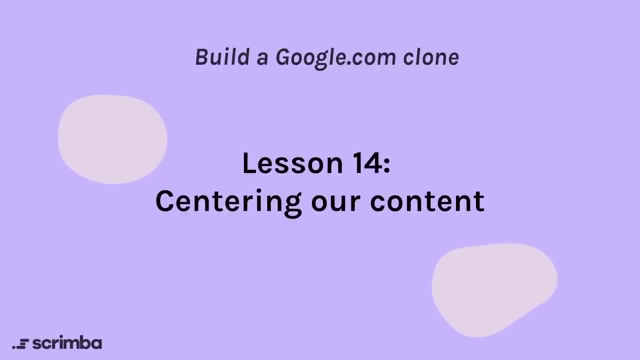 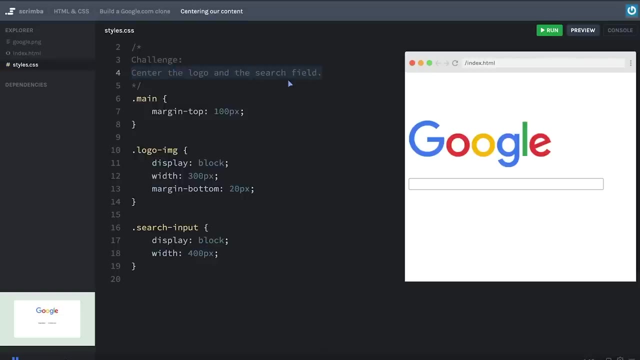 just be aware of the 4.5 million other developers who are in, or have been in, the same boat as you. Let's move on to the next script. Okay, Okay, We are back at our Google project. Now your challenge is to center the logo and the search. 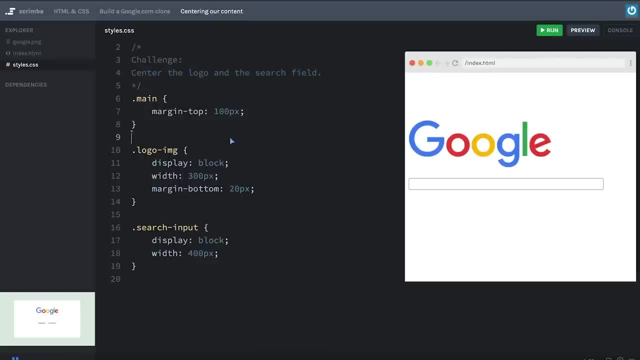 field using the technique you just learned. So go ahead and give that a shot right now, And then I will, of course, show you the solution afterwards as well. Okay, as you hopefully remembered the way to center an element which is display block. 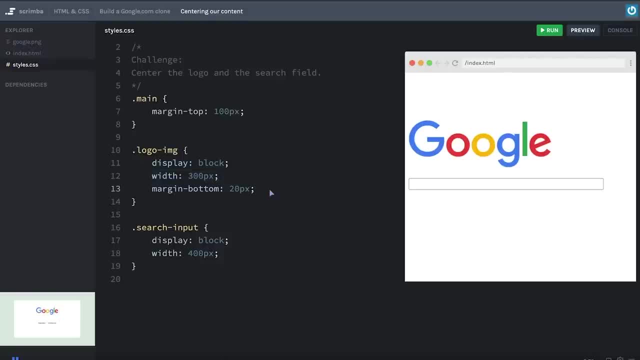 and has a width is by adding margin left auto and margin right auto. So let's do that. So margin left auto And, as you can see, that pushes the logo all the way to the right hand side because the margin left set to auto and it takes up as much space as it can. We'll. 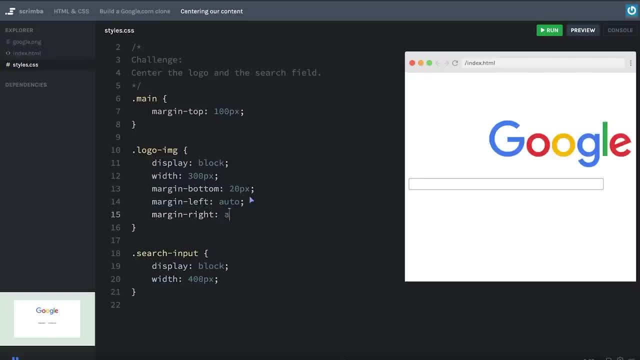 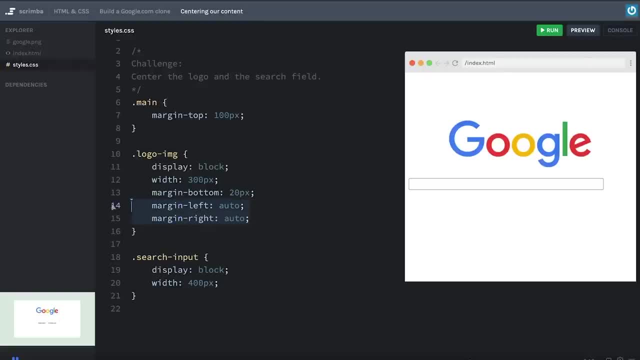 Our element is centered. So now what we can do is be super lazy and copy that code and paste it in down here and boom, our input field is centered as well And our project is starting to look a little bit like our finished design. So this is super cool, Let's. 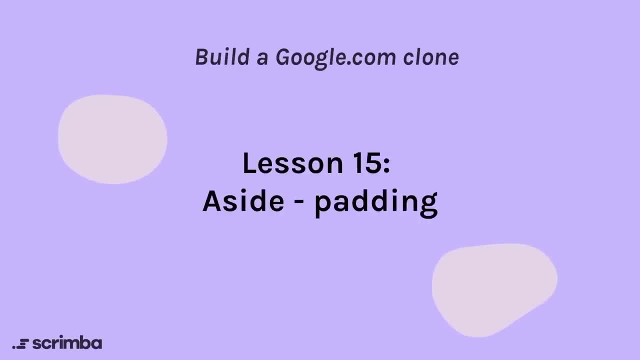 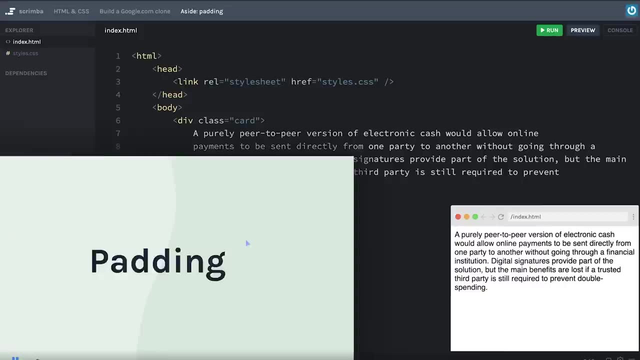 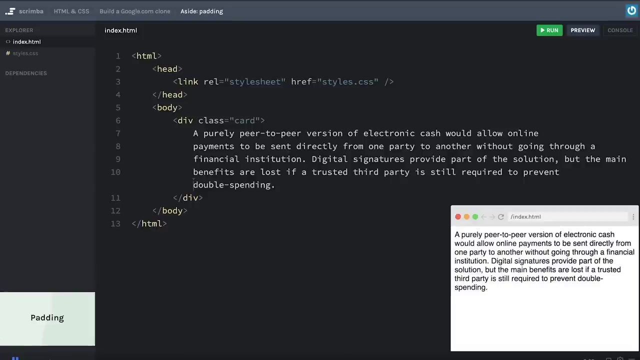 just keep up the pace and move on. We need to take a little step back and learn a new CSS concept, which is the close relative of margins, called padding, And we're, of course, going to learn that through the lens of an example. 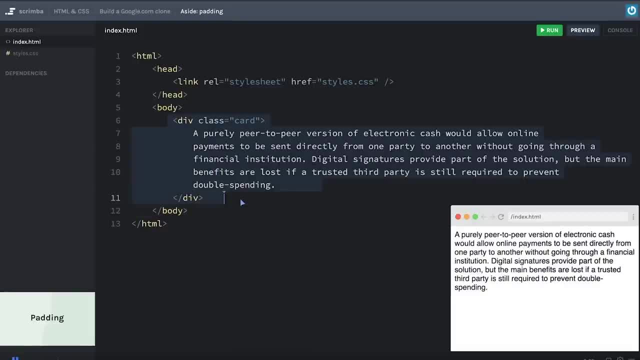 So here I have just a simple div which contains a little bit of text, or specifically the two first sentences in the white paper behind Bitcoin. And, let's say, we want to turn this into a nice looking card that people can read. If so, we'd probably create a class and call it card Then. 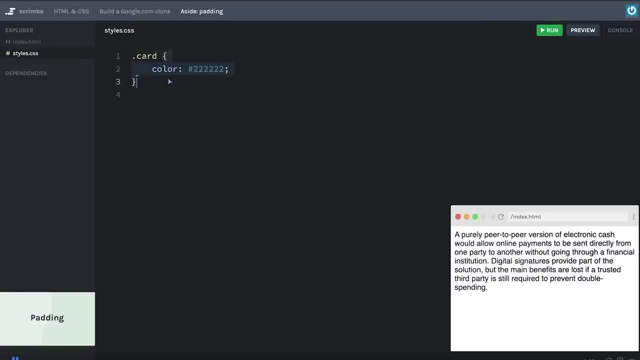 of course, in the stylecss we'd select that card and apply the styling. As for now, it just has one property set, which is the color that we've set, to a shade of black that isn't pure black, but a little bit softer, so to speak. That is because, by default, the browser uses pure black. 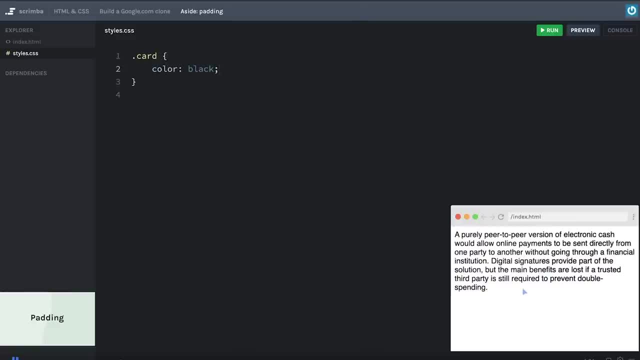 as the text color and pure white as the background color. And as a rule of thumb, you never want to have pure black on pure white, because that's not a pleasant experience for the eyes, So instead we went for this. But that was a digression. Let's move on with turning this into a nice looking card. 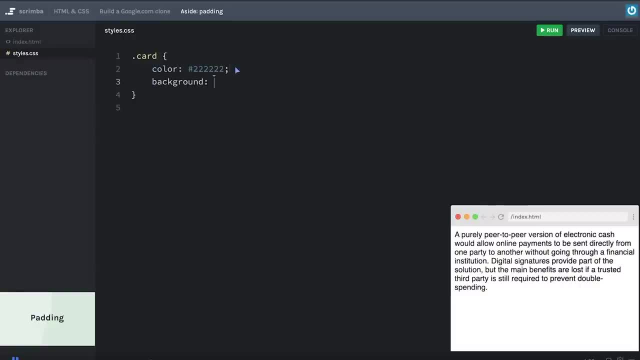 So a card needs a background color. So let's just do background light gray, for example, like that. And we also don't want our card to be full width because, as you remember, divs are blocked by default and take up the full width if you don't specify any width on it. So we're going to do. 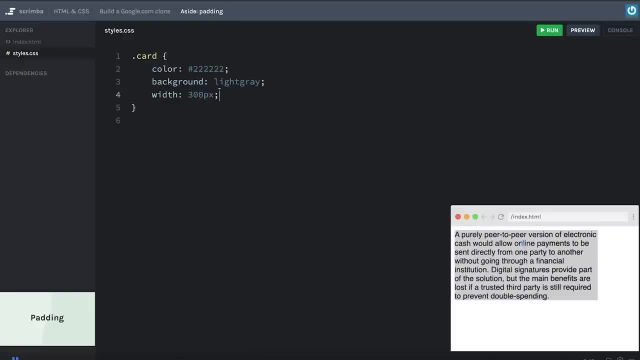 with, for example, 300 pixels, like that. And then we also want some space above the card. That is, of course, margin top. Let's push it 50 pixels down from the top And finally, it should be centered. So let's do margin left auto and margin right, Like that. Okay, so now we have 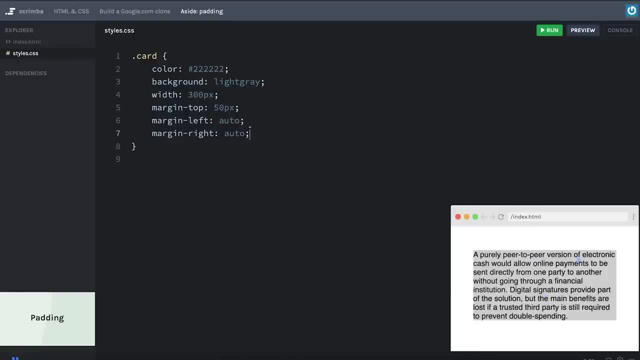 something that looks at least a little bit like a card. But there's one problem here, You can see: the text is crammed all the way into the edges of the, which doesn't look particularly good, And that is where padding comes into play. So now I'm just gonna apply the padding by doing padding and for 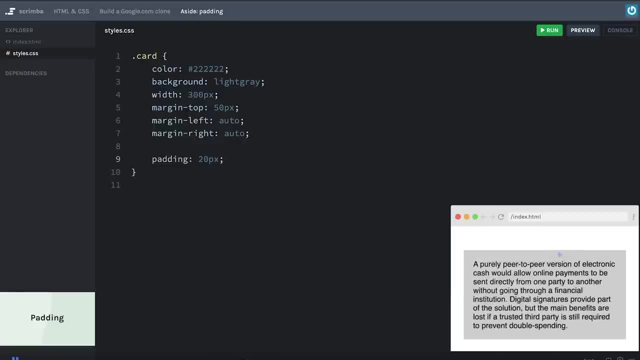 example, 20 pixels like that. As you can see, that created a little bit of space, basically some breathing room in between the text and the edge of our div container here. And if I do 50, you can see it's even more breathing room. 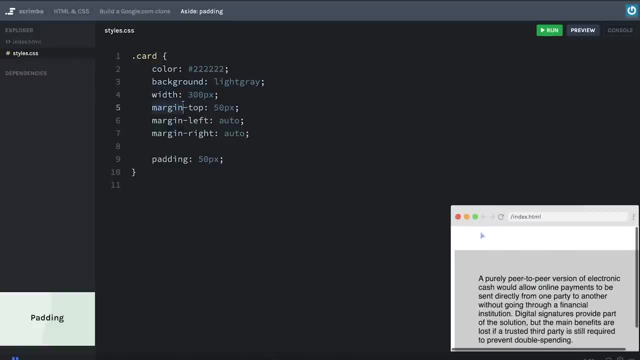 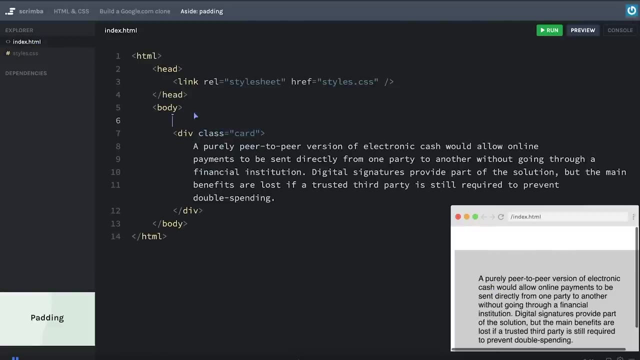 So worse, margin, add space on the outside of our div. the card which we've selected here, padding- will add space on the inside in between the content and the edges of the container or the div. So margin kind of lives up here And down here if we are to visualize. 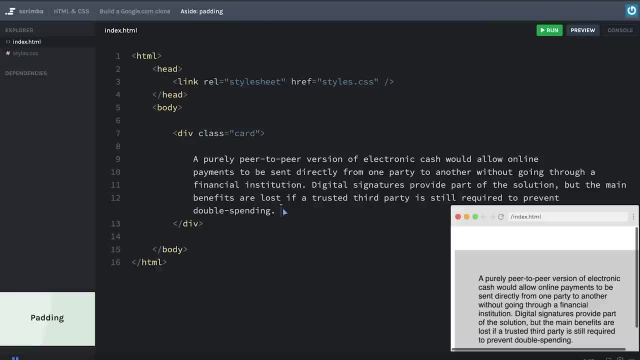 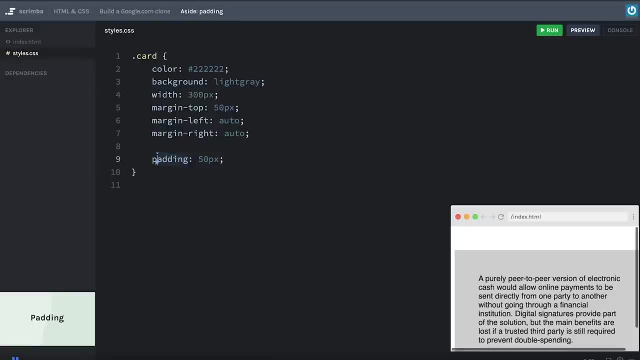 this in our HTML. we're padding lives on the inside of our element. that is here and here. And now you might wonder: well, why did I just write padding, whereas for Martin we're specifying each of the sides? And well, you can do exactly that on padding as well. This: 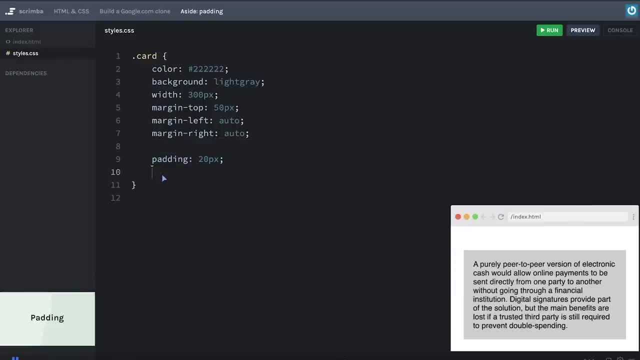 padding 20 pixels right here is the exact same thing As writing The following: padding: top 20,, bottom 20,, left 20, and right 20.. So with these four lines we can actually delete this one up here. then we have the same convention as we're using. 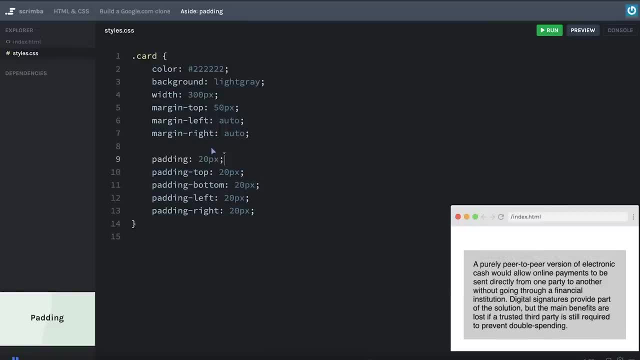 with margins. it's just that you can use padding 20 pixels like that if all of the values are the same. it's basically a shorthand, And now that we have all of them written out we can play around a little bit with it, perhaps at a hundred pixels on the left hand side. 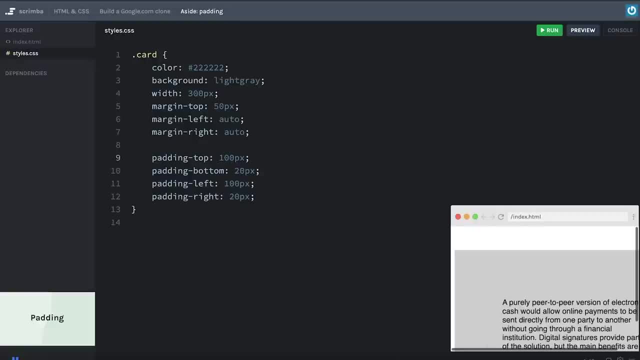 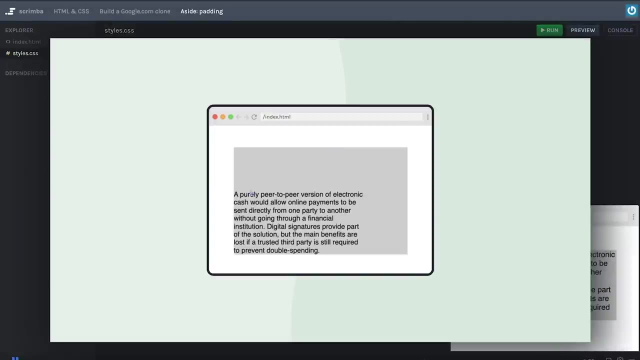 looks really weird. And a hundred pixels on the top as well, And suddenly our card does not look very good. But let's get it back. And now I want to give you a challenge. I want you to add padding to make our card look like the provider design. And the provider design is right here. you. 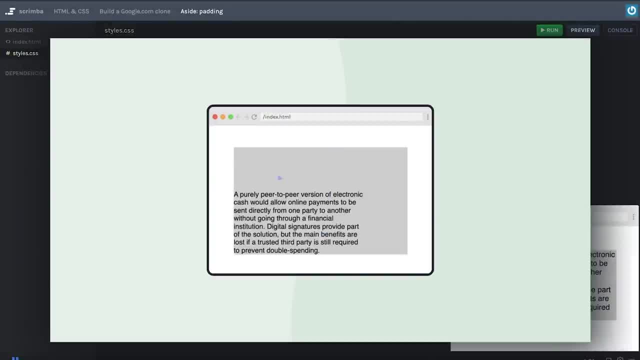 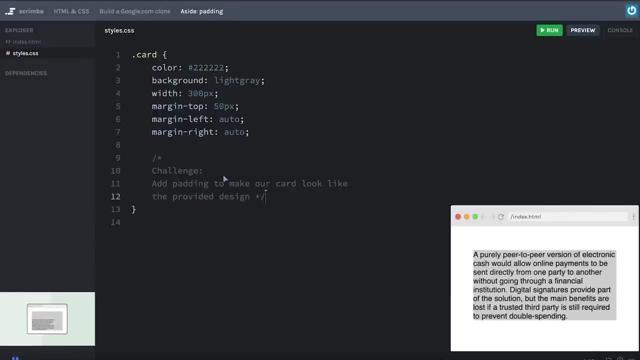 can see, it's a completely broken card, as we've been ruthless about our padding And I've actually removed all of the padding rules from the CSS, as I want you to build some muscle memory writing padding. So go ahead and make this card look like the provided design And 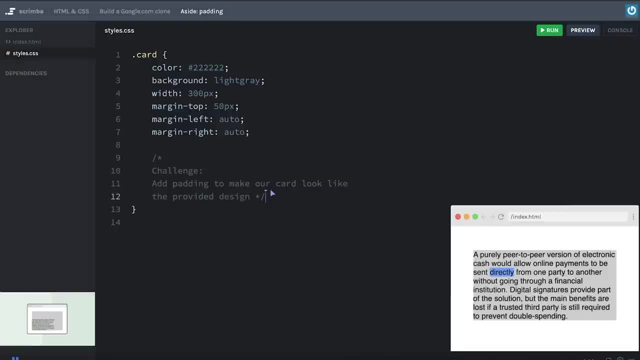 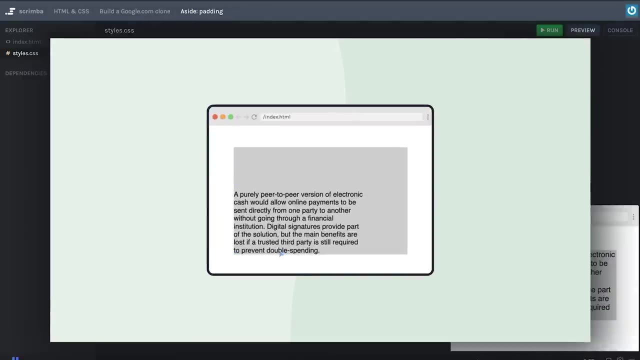 I'm going to make this card look like it does in the slide and then return back to me once you've done it. Okay, hopefully that went well. If not, no worries, let's do it together. As you can see here, it's completely crammed into the bottom left corner, which means that 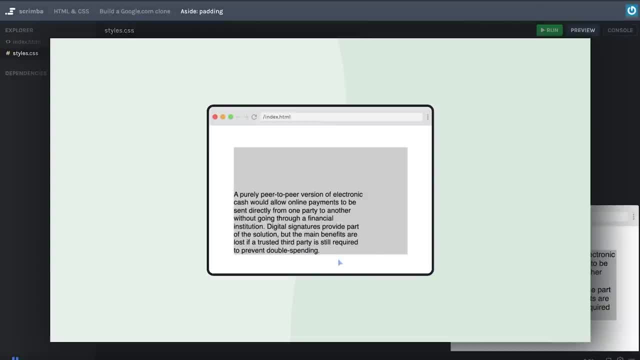 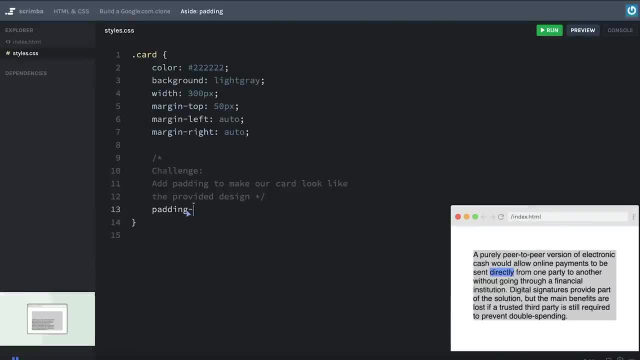 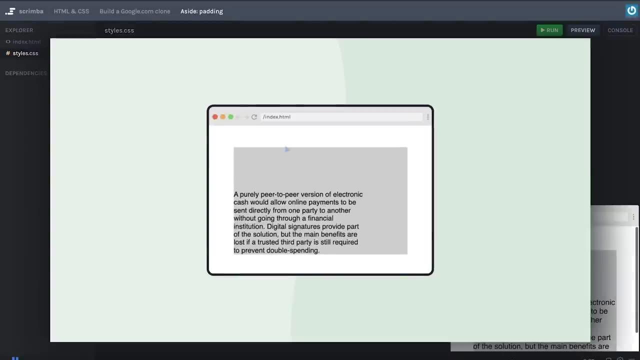 it doesn't have any padding on the left hand side or any padding on the bottom, but a ton of padding on the top and a ton of padding on the right. So I'm just going to go ahead and do padding top 100 pixels, something like that Seems pretty much what we have. 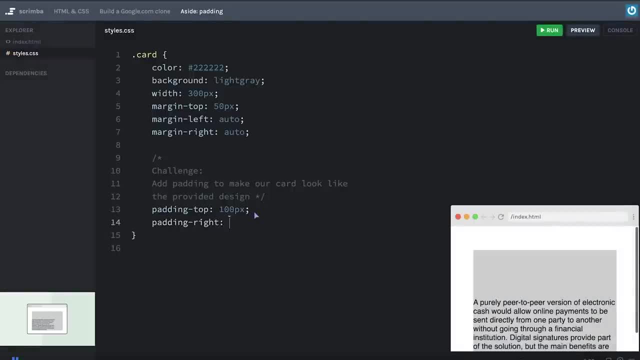 in the design as well, And then do the same padding right, 100 pixels, like that, And to me that looks actually pretty much like our design. I don't need to write padding bottom or padding left. now though I could do it. I could do padding autumn, zero pixels. 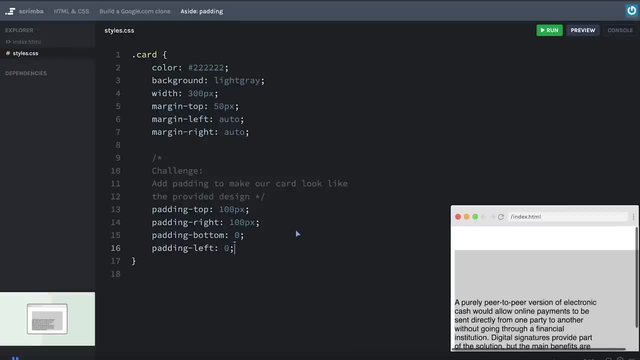 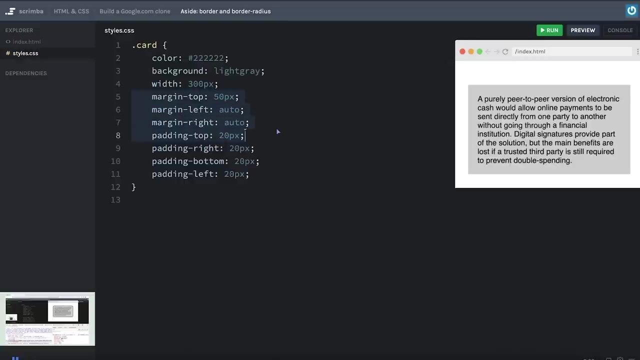 or just zero, And padding left zero as well, though that didn't change anything, So it's actually not needed, because, by default, the padding of a div is zero. So, however, you solve this great job, Let's move on. So now you've learned about controlling the space on the outside. 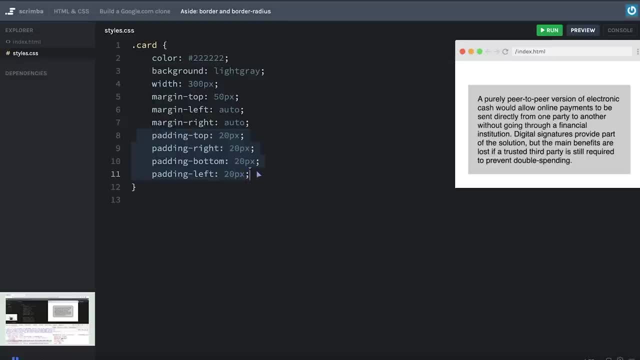 of the element with the margin and on the inside of the element with the padding. But wouldn't it be nice if we could also control the border in between the margin and the padding? And it turns out we can through- you guessed it- the border property. Because if I write the border here and then specify 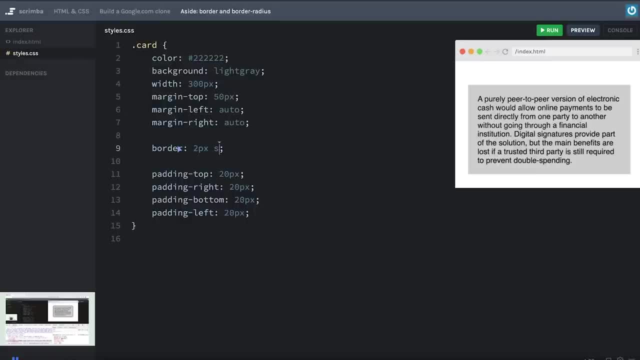 for example, two pixels thickness, solid in shape and then color red. you can see, then we get a border which is on the outside of the padding but on the inside of the margin. And if we change any of these three values here, 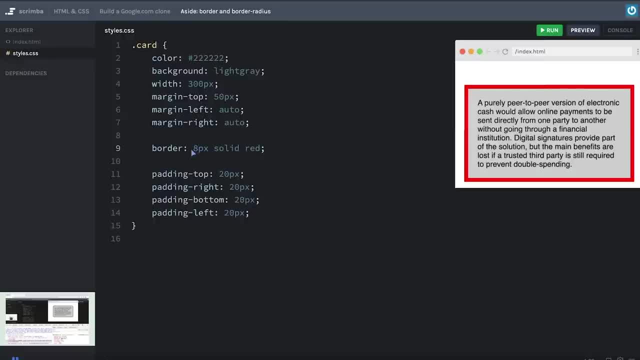 it'll update accordingly. So let's try eight pixels with instead. you can see it's much thicker. Now, instead of solid we can do audit like that- pretty weird. And instead of red we can do, for example, FFF, white in hexadecimal, or just write white like that. 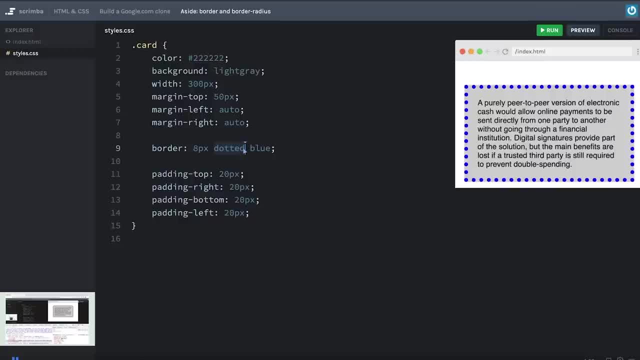 or just blue, So it's a little bit clearer Now. there are many types of borders, But in 99.9% of the cases you want to use solid like that, And also very often you'd want to soften up these corners, And you can do that with. 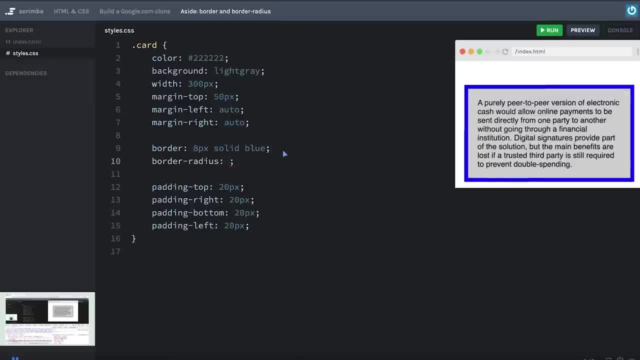 the border, Adius property, an area. specify a pixel value, for example 30 pixels, and boom, there you can see, we have this much softer corners. If we crank this up to 100 or 1000, it stops at some point, because then the edges have simply turned into half circles. 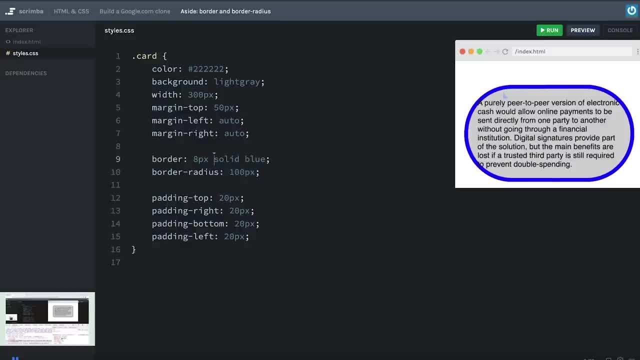 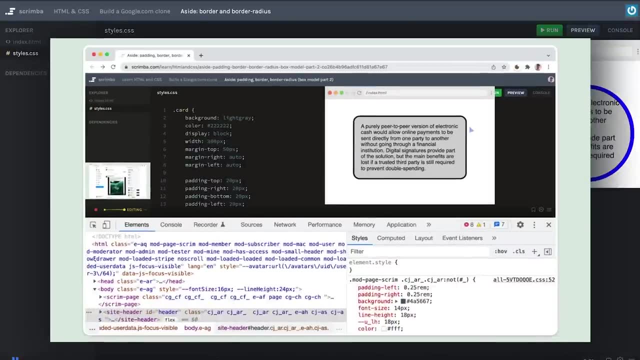 So at some point, there's no use going any higher Now. this looks pretty bad. So what I want you to do now is fix it up so that it looks like this, And I'm not going to give you any of the values I've used here, just a little hint. I took an already existing 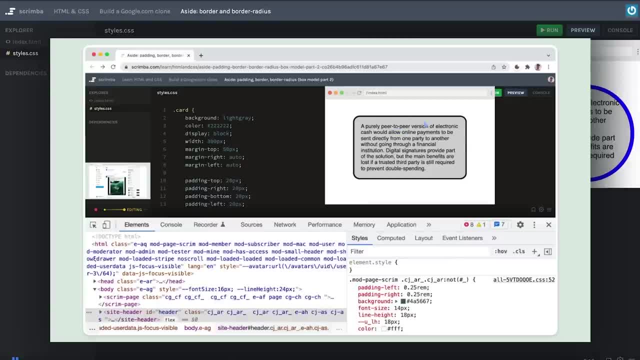 color in our box and use it for the border. So that's a common web design trick to reuse colors and not have too many different colors. So if you think this is pure black, you are wrong, So go ahead and change the values. 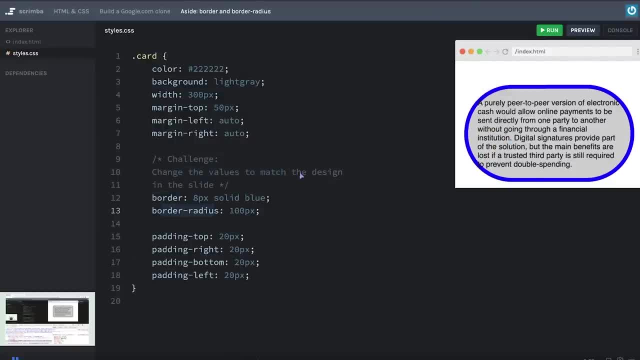 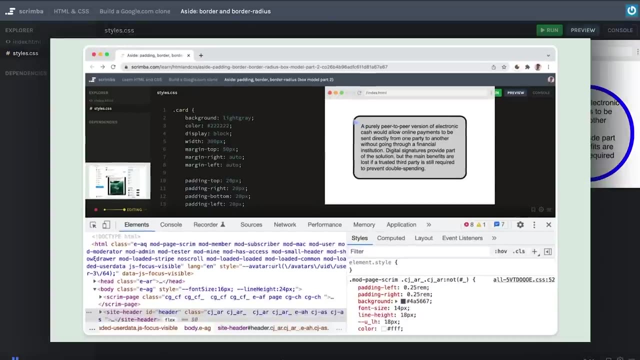 Of the border and border radius, so that our example here matches the design I've provided in the slide. Good luck, Okay, hopefully that went well, So let's start with the border. eight pixels here looks a bit too thick for me, So let's try for instead, like that. I. 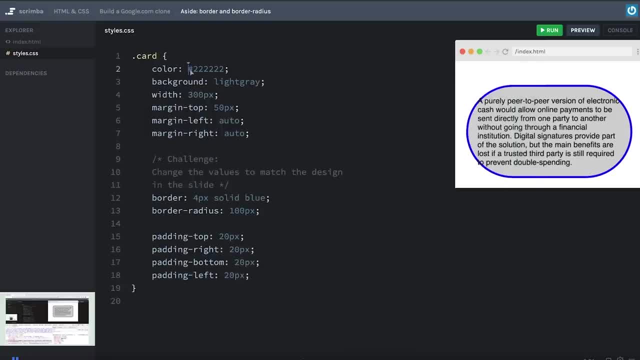 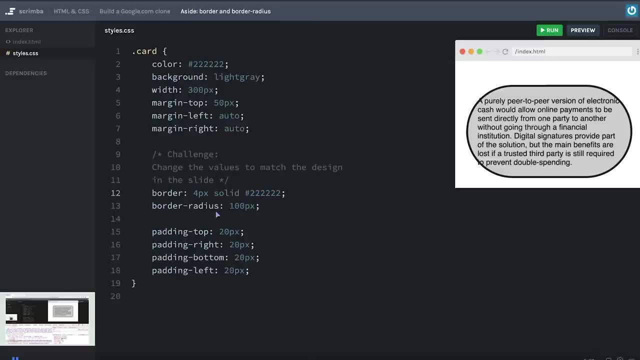 think that matches better. Yes, And the color I gave you a hint was just the blackish color we have for our text like that, And the border radius is much smaller. Let's try 10.. This still looks a little bit rounder, So let's try 20.. Yes, there I think. 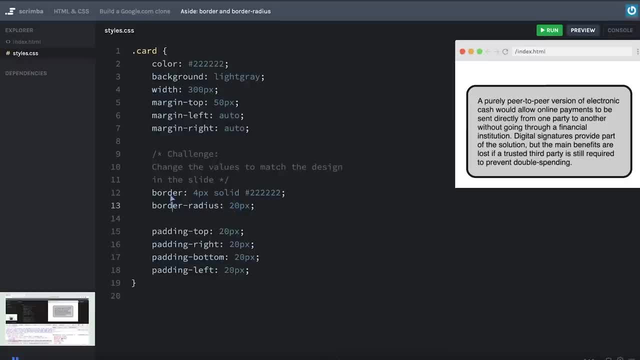 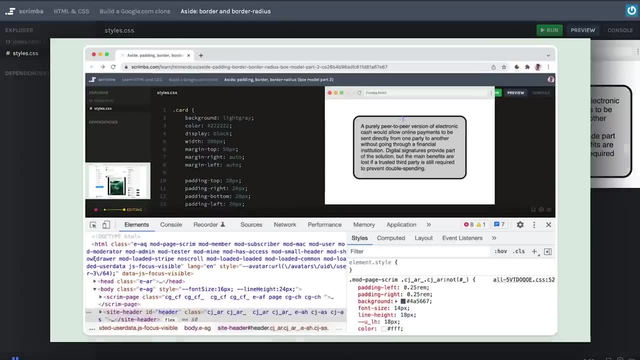 we got it, Great job. Now cool thing to do in order to inspect the margin, border padding and size of the element in general is to open up the dev tools, which can be done by writing, right clicking on the nav bar here and then clicking inspect And then this dev tools. 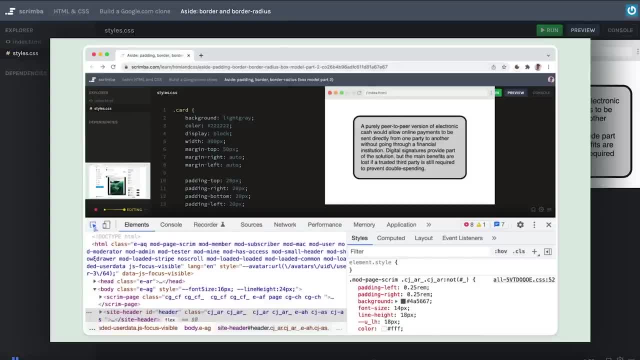 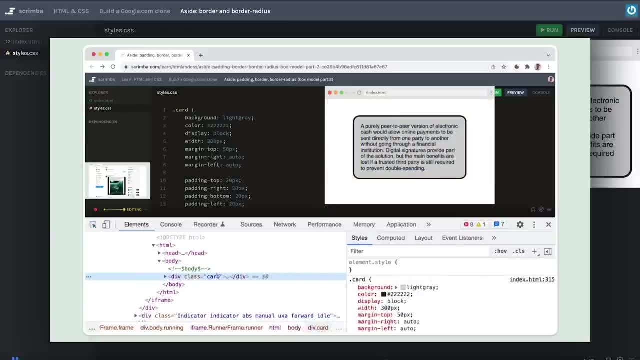 panel will open here. clicking on the select icon on the left hand side And then hovering over the element, finally clicking at it There, you will see that we have selected the element in the elements tab And under the styles tab you can see the styling we. 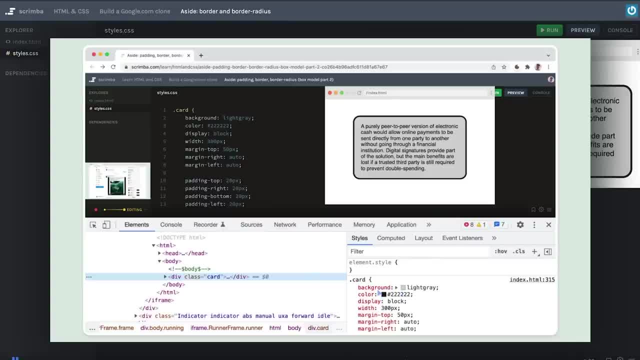 have applied using CSS. So here you can actually modify them if you want. But we're not going to do that right now. We're going to scroll down And verify that our margin, border and padding are correct. So if I hover over the margin, 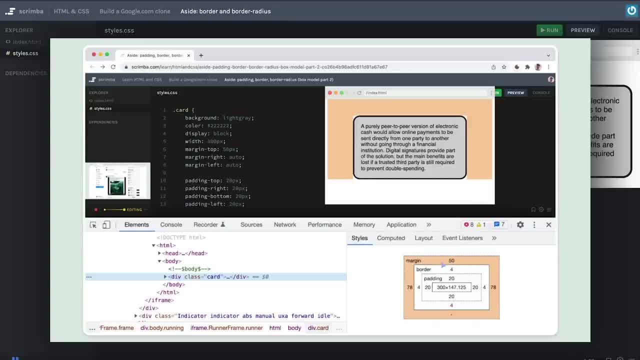 here. you can see up here in the mini browser. it is marked in orange And the values are provided down in the box here. If I move over to the border, you can see that border is now selected in the browser And it's indeed four pixels as we code it up a minute ago. 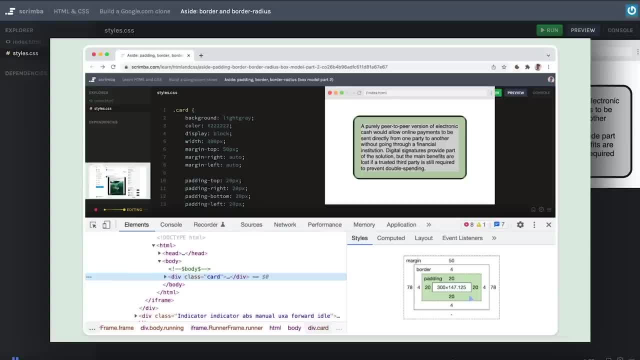 If I move over to the padding, you can see that is also indeed, 20 on each side, just as we want it to be. And finally, if I hover over the center, here the content is highlighted, and the content of this dev is just as we wanted it to be. So we have selected the content. 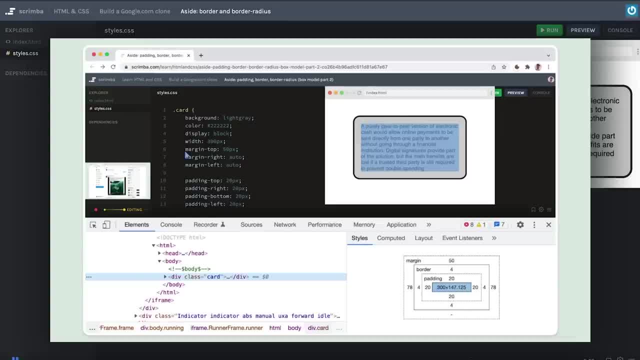 And then we move over to the margin. here you can see that our margin is now selected And the text- And, as you can see, it is 300 pixels wide, just as we set it as. so it's working as expected, And the height is dictated by how many lines of text. are two sentences required? 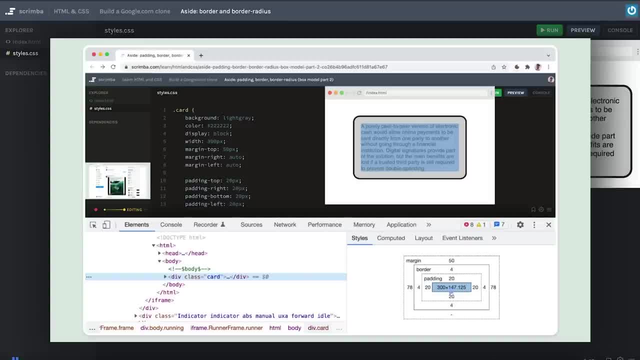 So using this technique of inspecting an element and its sizing properties like this is a really good way of debugging if something, for example, looks wrong, because it gives you an ability to verify if the numbers here match up with what you've tried to write in your CSS. So 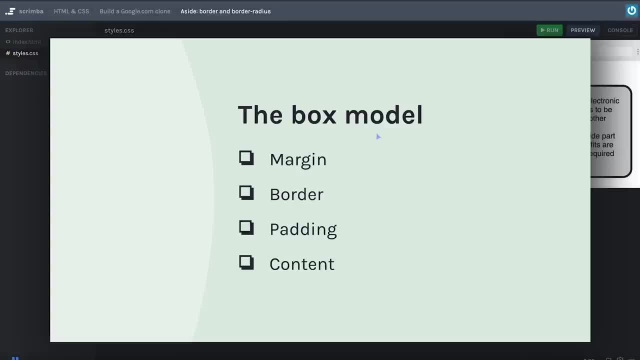 now that you've learned all of that, I want to tell you the name of this, And it's actually called the box model And, to be honest, I've never really liked this word. it sounds more complex than it is. in my opinion, it's just spacing around the elements, a border spacing. 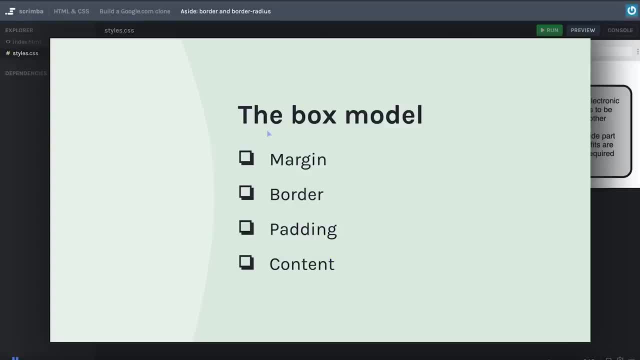 on the inside of an element and the content itself. But in web development we call this the box model, So you'll probably hear this name come up from time to time, but you shouldn't fear it. you know exactly what it is And you've used all of the properties in the box. 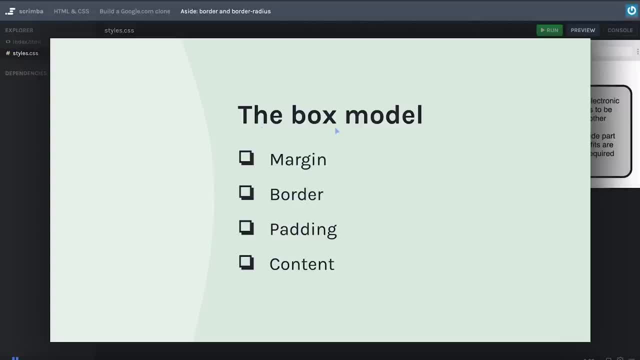 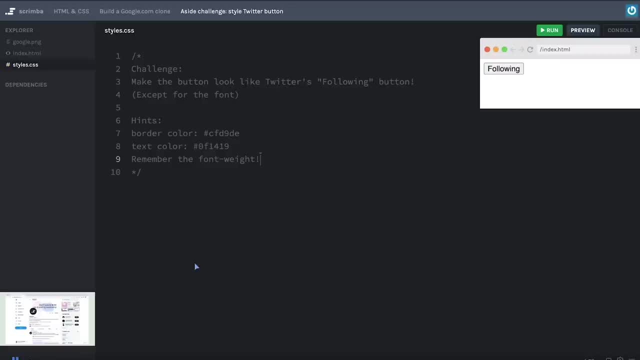 model, So don't worry about it. Actually, a new box model practice in the next trim. I'll see you there. Okay, now you are going to create a really neat looking button, namely the following button on Twitter: let's zoom. 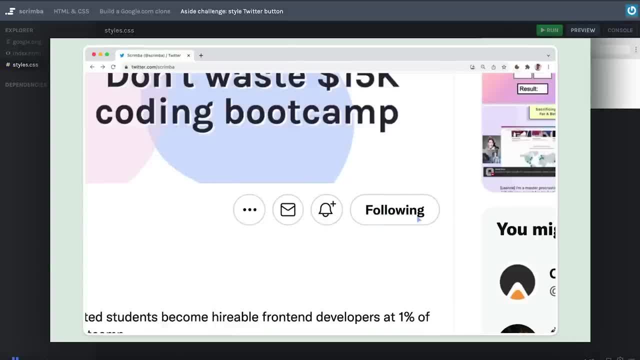 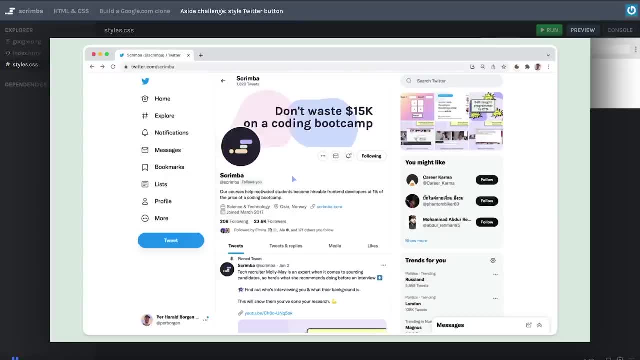 in a little bit And here you can see it. this is the button. you see if you already are following someone and we zoom out again. this is the scrimball Twitter profile. you should definitely just click this image and follow us, because we share a ton of useful 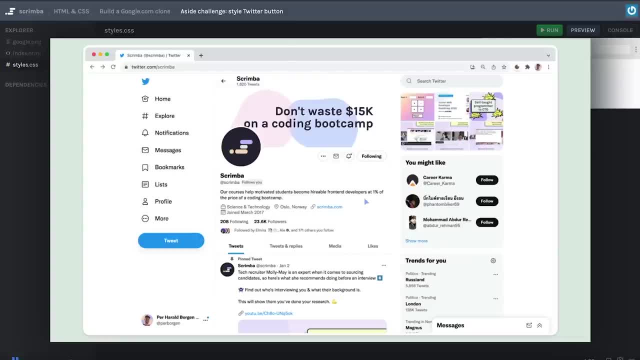 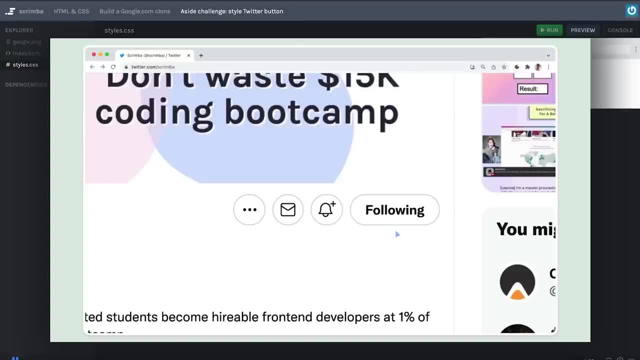 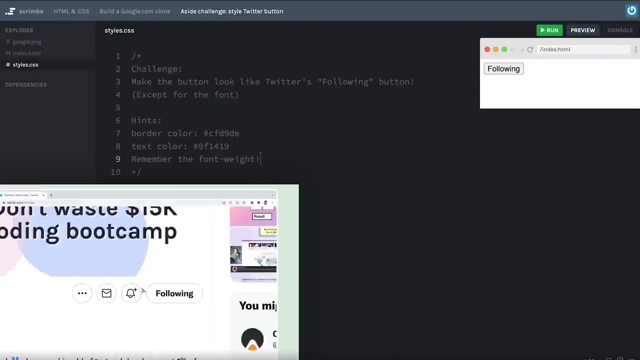 tips and tricks and career advice for aspiring coders Here, So it's definitely worthwhile. Anyway, now you are going to use the things you've learned about padding border, border radius and so forth in order to make this button right here with the ugly default styling, look exactly like this, Or not, exactly As we're. 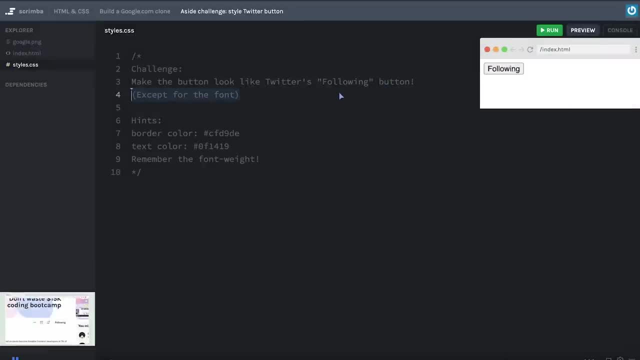 not going to worry about the font- it is a little bit different- But other than that, you should try to make it look identical. I've given you some hints here. For example, the border color is this hex color right here And the text color is this hex color And. 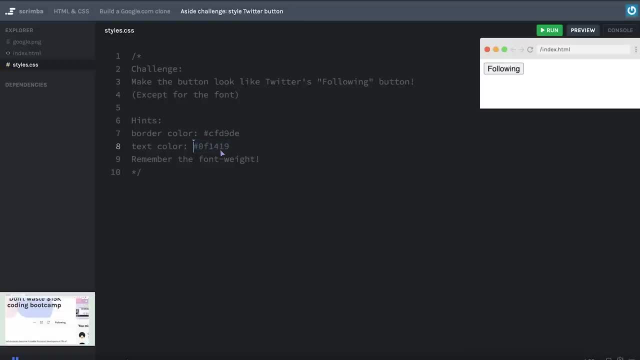 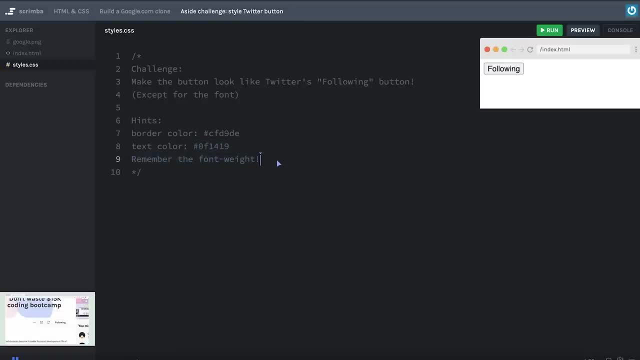 to adjust the font weight, And I don't think you've done that ever since the very first scrim where you wrote your first lines of CSS. So you might have to look back so that you figure out how to adjust the font weight, Or you can Google it up to you. Anyway, just 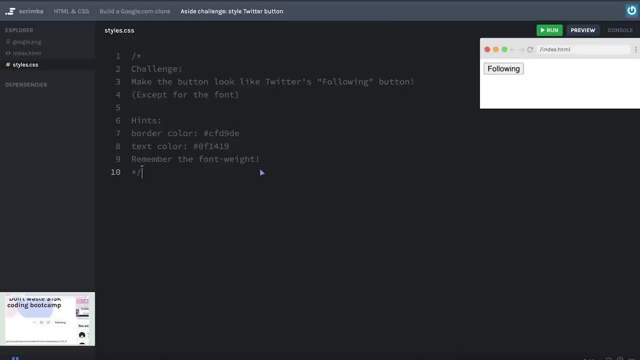 go ahead and give this your best shot, And if you at some point get stuck or don't know how to do it, no worries, we are going to do it together afterwards as well. Good luck, Okay, hopefully that went well. let's do it together. I'm going to target the button. 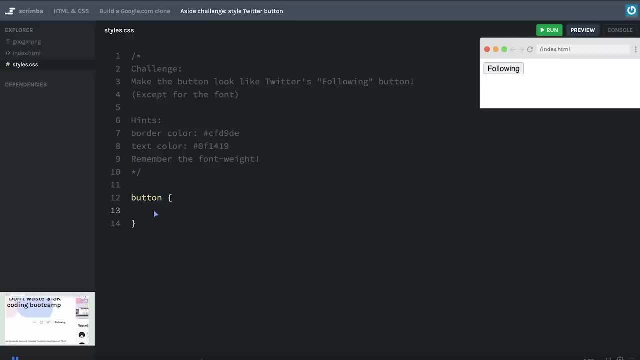 just using an element selector like this. And now let's pick the low hanging fruit, namely the ones we've gotten here already, For example by doing color, then copying this color right here. Okay, that didn't change much, at least not visibly. then let's do: 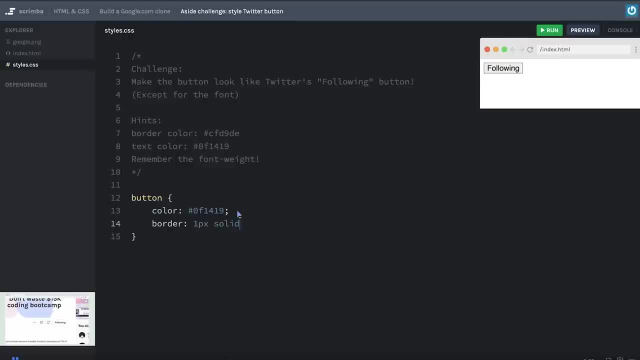 border And I'm going to start with one pixel solid And then the border color right here, like that. Okay, so it looks a little bit different now, But not quite this. One thing we can clearly see is that this image has a white background. 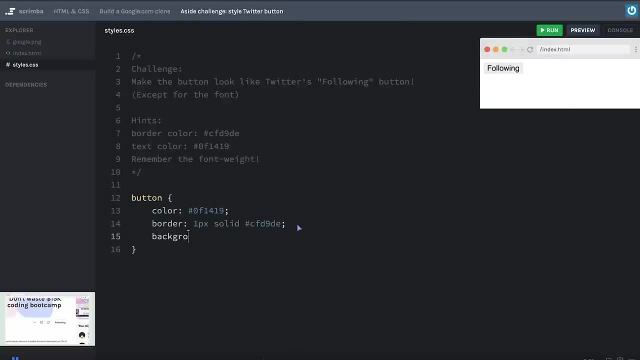 whereas ours is still a little bit gray, So let's do that as well. Background White: Okay, yes, But our button is much more crammed. There's too little padding, Whereas here you can see, we have a little bit of padding on the top and the bottom and actually quite 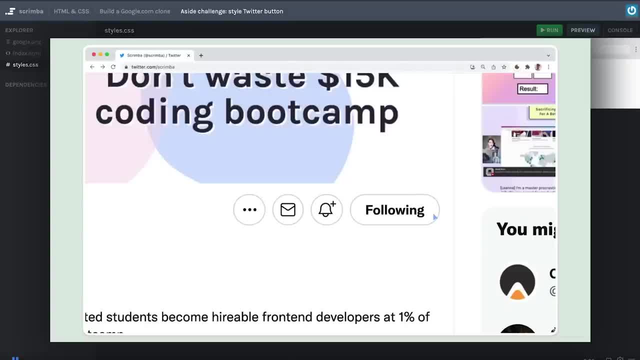 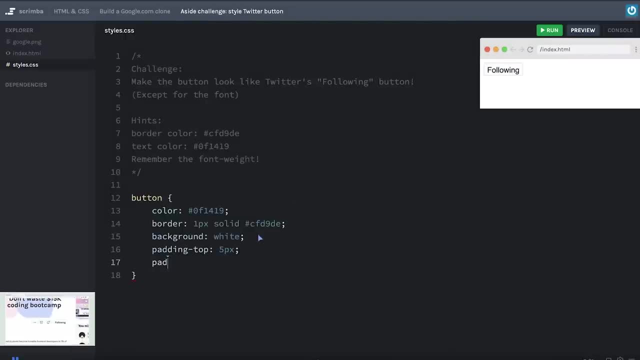 a lot of padding on the left and right hand side, And that's actually a little design tip right there. What you'll often see is that buttons have more padding on the left hand side and the right hand side and they have above and below. So let's try padding top five pixels, for example, padding bottom five pixels. 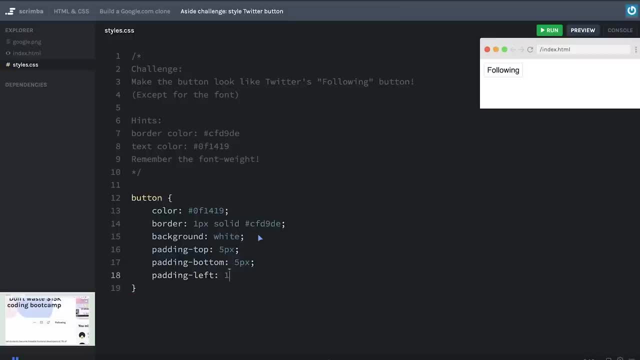 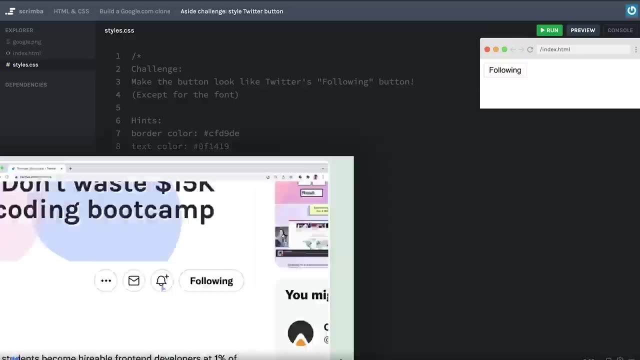 And then we'll try left 10 pixels and right 10 pixels as well. How does that look? Not too bad, but actually, yeah. well, we can see this is a bit less padding than now, But actually it looks like this button has even more, So we've added half as much on the top. 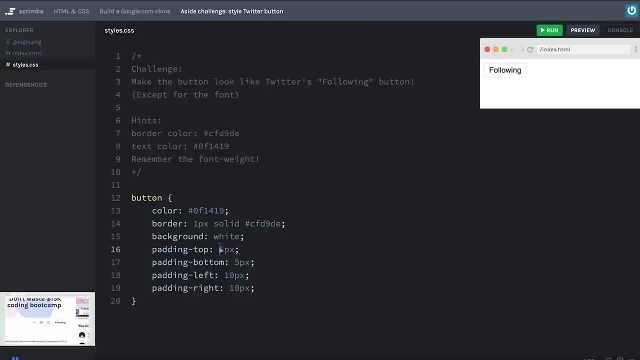 and bottom, as we have on the sides. So let's crank up both of these a little bit. I'm going to select both of these and do eight top and below, and select both of these and do 16 left and right. Yeah, I think that's more like it. Now, one thing that definitely is remaining: 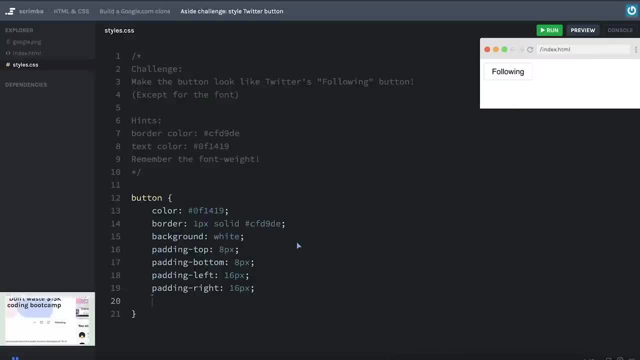 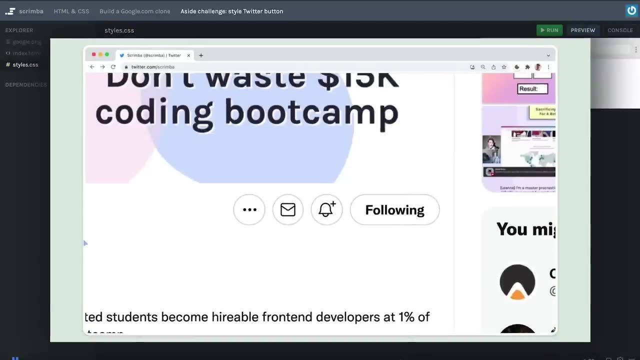 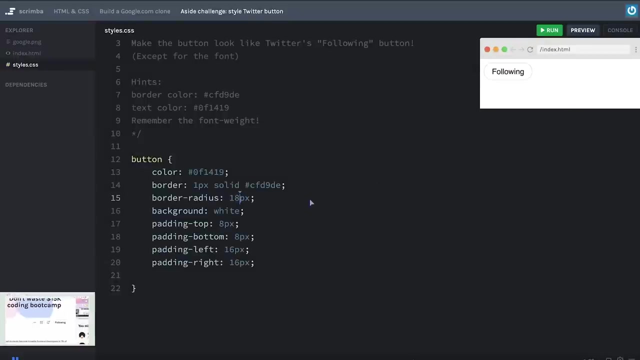 is the rounded edges here. So that is the border radius added up here, with the border 10 pixels. It's a little bit round now, but not as round as the Twitter button, So let's do 16.. Yeah, more like it. Can we go higher? Yeah, I think we can go to 18.. That looks. 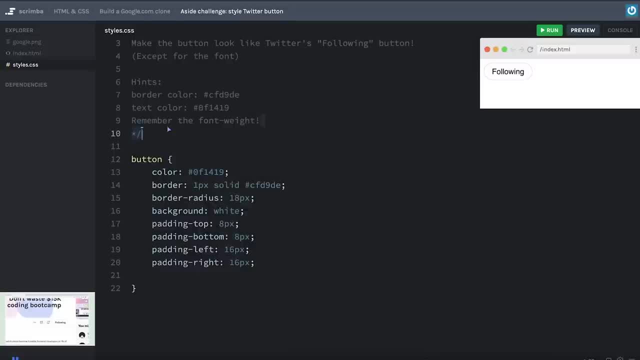 quite good to me If we compare it to this one. And then, finally, we needed to remember the font weight. font weight: bold like that. That looks a lot better. I think the final adjustment I want to make is adding even a little bit more padding around it, Because now that I 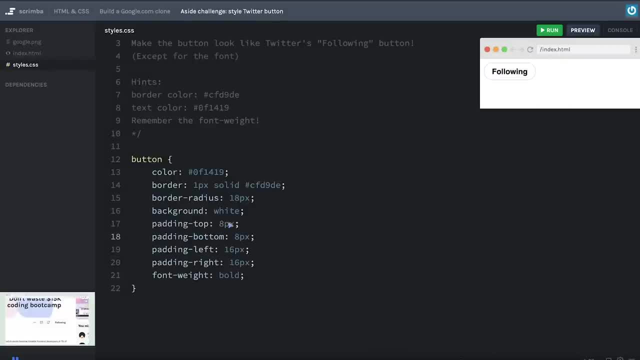 look at it, it feels like this is a bit more spacious. So here we are really in the nitpicking area. But let's try 10 on both of the top and bottom And let's try 20 on the left and right. And what's interesting now is that since the box now has grown in size, because 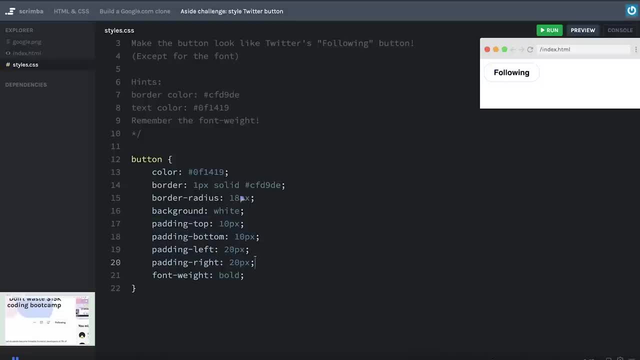 it's affected by the padding. the border radius can also be cranked up a little bit. I think actually we can do 20.. Now, Yes, because the bigger a box, the bigger the padding. The bigger a box is more pixels you need to add in order to get this fully soft looking. 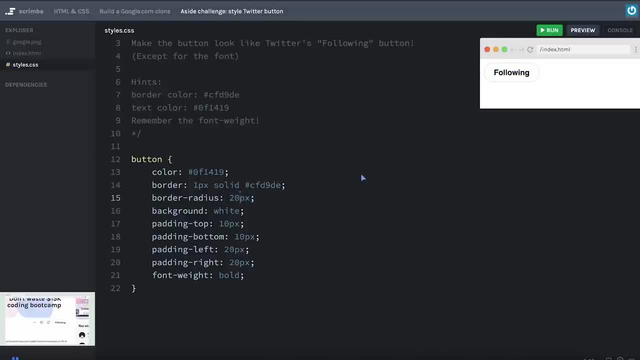 button which essentially has two half circles on each of its sides. So looking at the example and comparing it with ours, I think we have reached our goal, And if your values are different than mine, that does not matter at all. you're actually creating the button of a huge public. 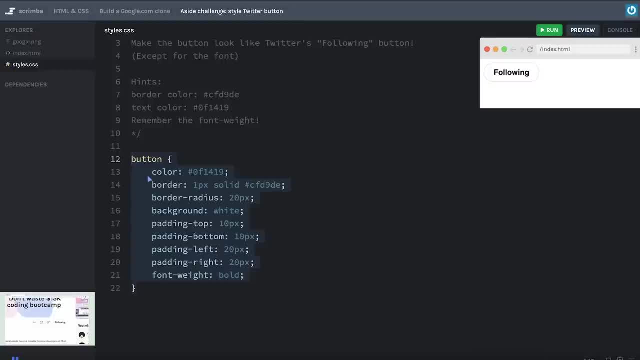 company. here you're just learning basic CSS, So it's totally not expected that you create buttons as neatly as Twitter does, Because they probably have a team of developers and designers working just on this profile page. So, however it went, be proud of yourself and get ready to move on with our Google project. 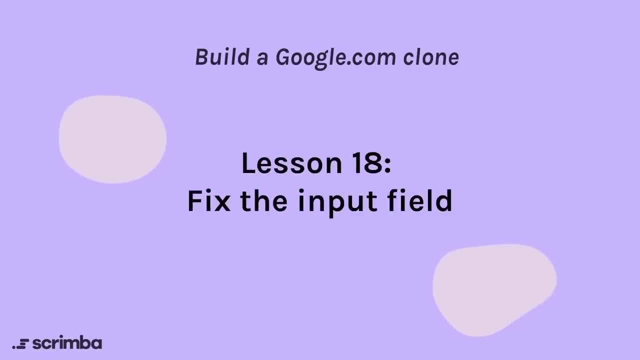 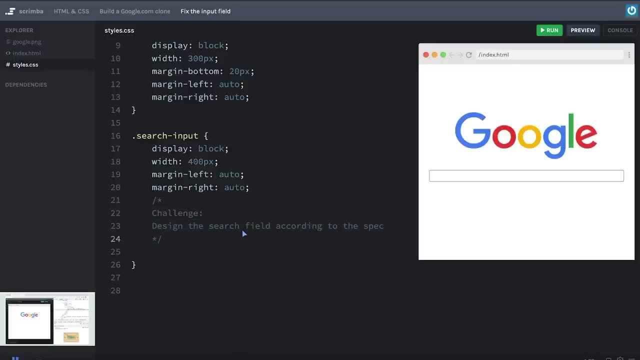 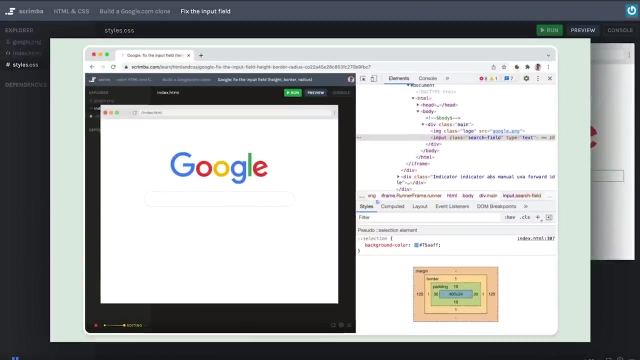 I'll see you in the next grip. Okay, we are back at our Google project And now you're going to fix the design of our search fields And you're actually going to get a design spec and the proper walkthrough of how I want it to look. So here I've opened up the dev. 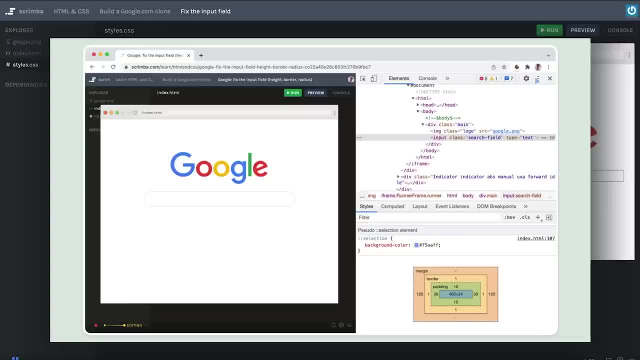 tools. I'm actually on the right hand side as I want to inspect the box model of this element with you, And if you wonder how I managed to stick the tools to the right hand side here, just click these three icons. If you're in Chrome, then you can choose the. 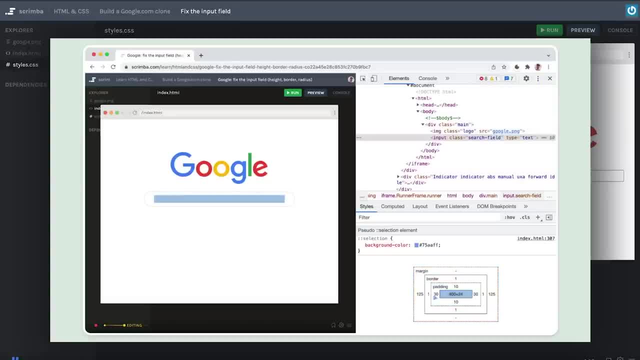 dock side. So let's move on down here to the box model of the input field And if I hover over the content in the box model here, you can see that it says 400 pixels times 24 pixels And you can see the content is marked in blue. 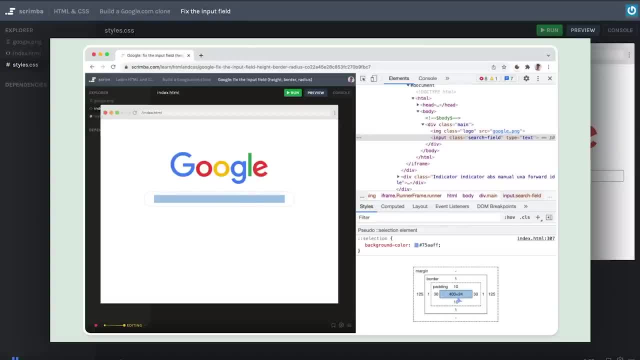 In the mini browser here. That means that our width is 400 pixels. We know that because we set ourselves here and the height of the content should be 24 pixels. Okay, let's move on to the padding. by hover over that you can see is green and it's highlighted in green. 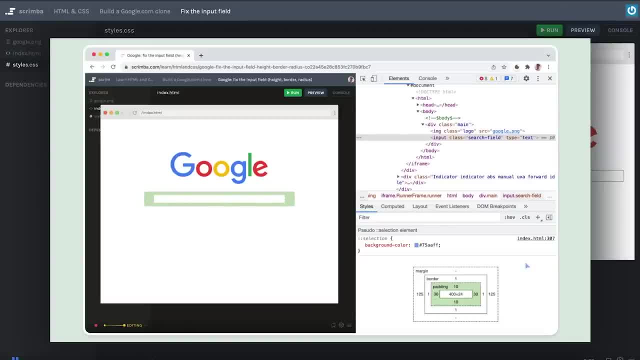 in the mini browser, the padding at the top and the bottom are 10 pixels, as you can see down here, and the left hand side and right hand side have 30 pixels each, And then if we move over to the border, you can see that it's simple. 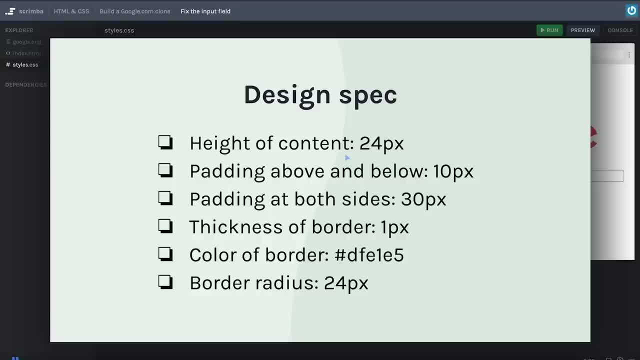 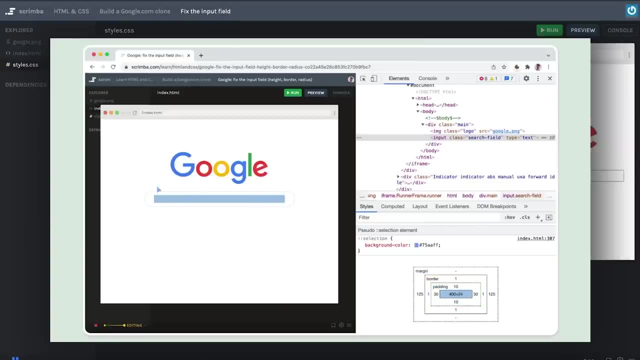 It's actually one pixel all around. So here is your design spec, given to you by your hipster designer down in the bottom right corner here. height of content: 24 pixels. But do remember that that is actually the height of the inner box here, not the height of the total input. 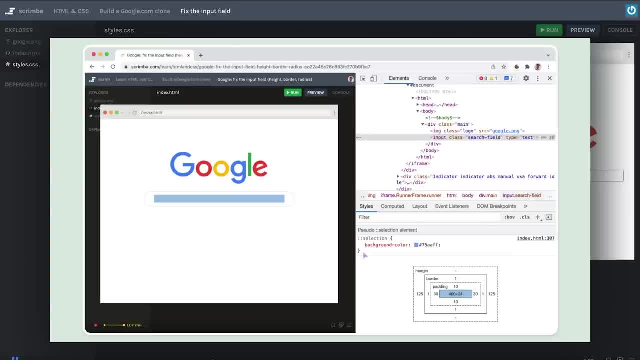 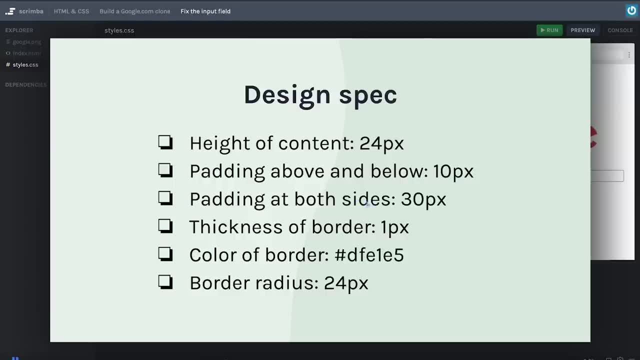 field, as that also contains the padding and the border, but the height property should be 24 pixels, the padding above and beyond, as said, 10 pixels. right and left hand side, 30 pixels. Because of border, one pixel. the color of border is this And then finally, also the. 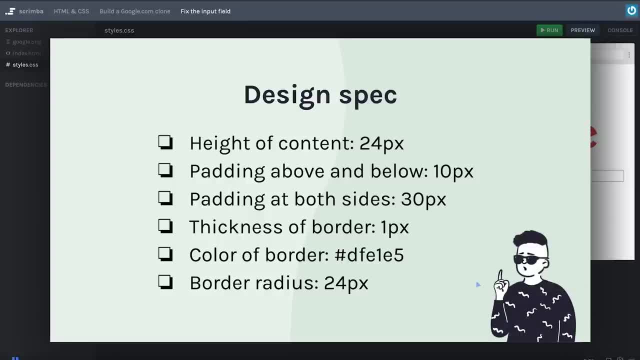 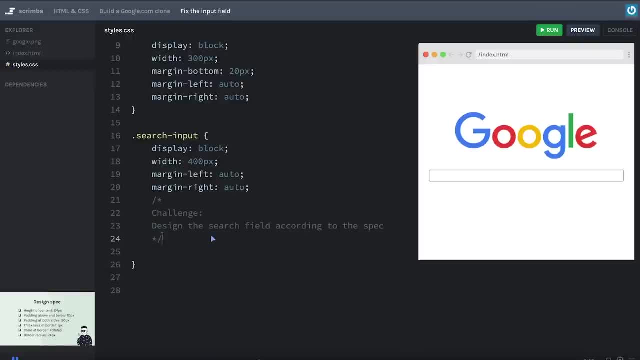 border radius is also a value that our designer has been kind enough to give to you, So take this design spec and implement it using CSS. Okay, hopefully that went well. If not, no worries, we'll do this together right now. So, starting with the height of 24, there. 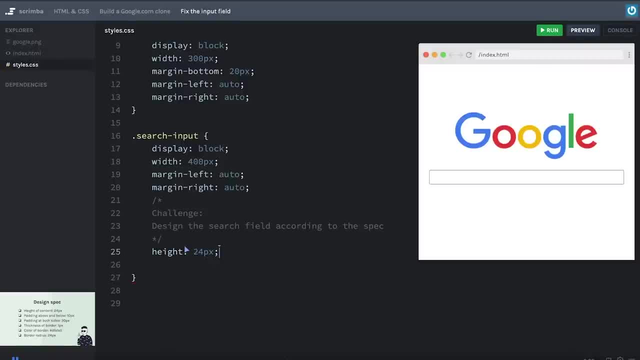 I'm going to just write 24 pixels Like that. Okay, so it became a little bit taller. Now Next step is the padding. top and bottom was 10 pixels, So padding top: 10px. Autumn was also MPX, like that. Okay, the padding. 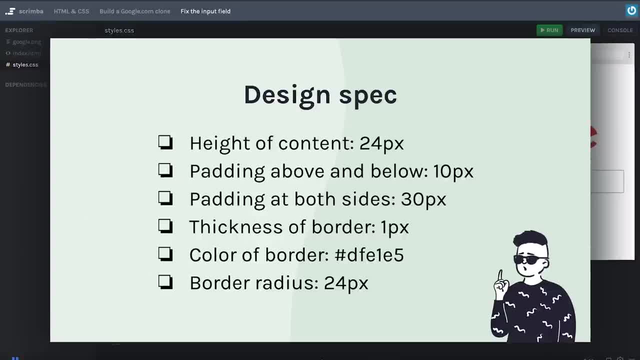 left and right hand side were 30 pixels according to the spec. So let's implement that like that And then we'll move on to the border: one pixel and this hex code right here. So I'll do border And here we have to provide it with three values. 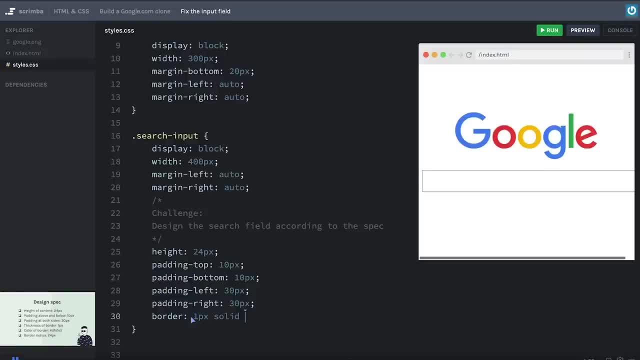 So one pixel, it is going to be solid, and the color is the F e, one e, five like that, looking pretty good. The final thing, then, is the border radius, And that should be 24 pixels according to the design, And look at this, it is starting to look really professional. 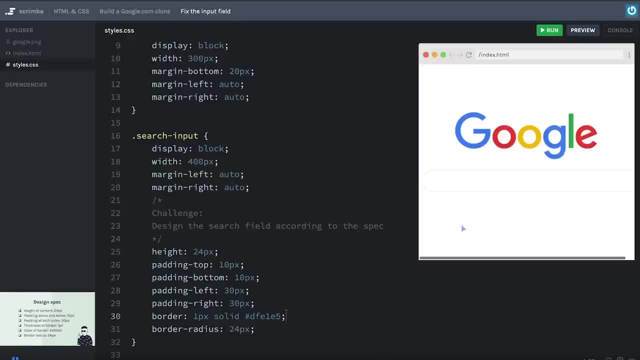 So really good job if you did this challenge And if you did a couple of mistakes, no worries at all. Actually I also did a little mistake here, according to best practices When setting heights for improvement Input fields, because actually I want to show you that this height of 24 pixels here. 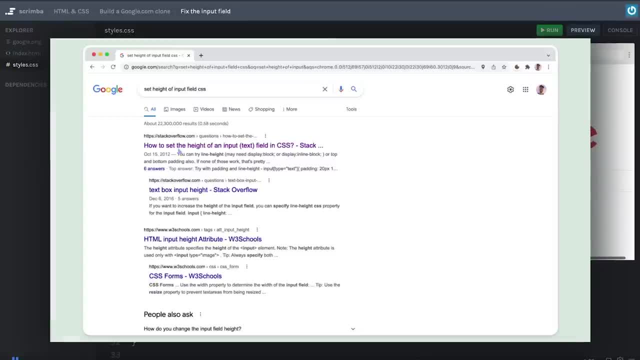 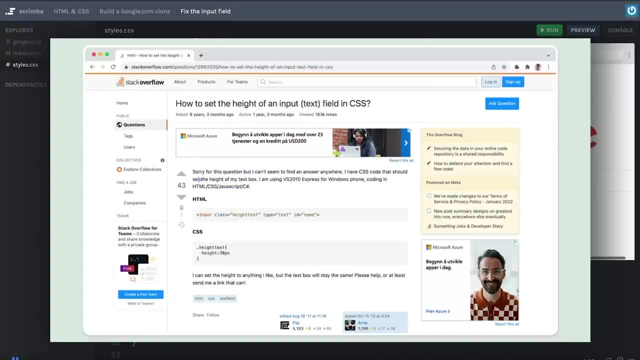 is actually not the way we want to do it, Because if I Google, set height of input field CSS and then click the first link, that is a stack overflow question, And here you can see someone who's been having problems with this, So they've asked a question about it. 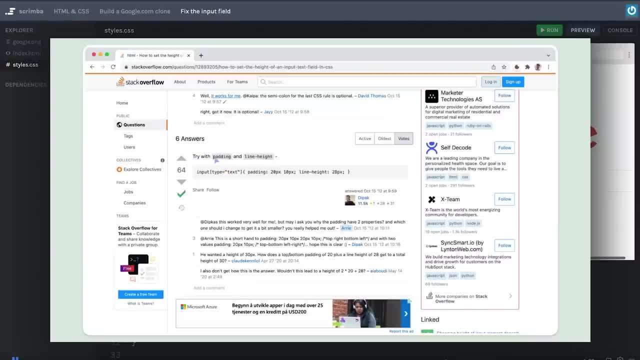 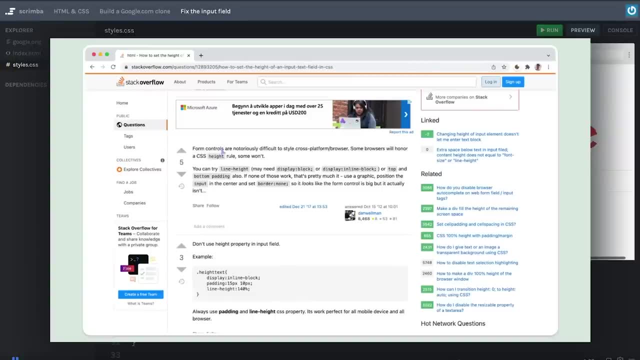 If we scroll a little bit down, you can see that people are saying: try with padding and line height, line height- that's not something we've used. We scroll a little bit down you can see that Some browsers will honor a CSS height rule, some not. So it seems to be a little bit difficult. 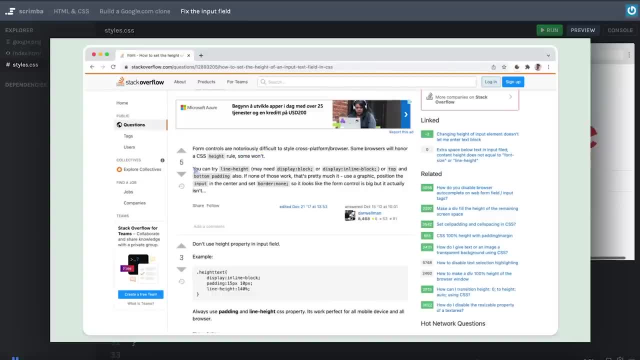 to use height for the input field, And this person's wall suggests line height, And likewise with this third person here. So I'm going to trust the wisdom of the crowds here and use line height instead, Like that didn't change anything. But we are using a property. 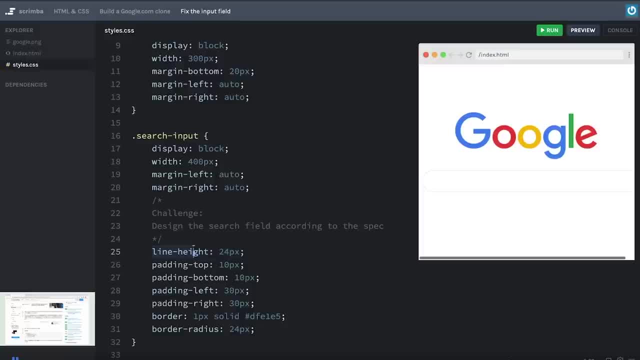 that more browsers apparently will honor, And line height is actually just the height of one line of text And since that is everything we have inside of an input field, it's just one line of text. that'll be the exact same thing as setting the height of the inner content of the input field. 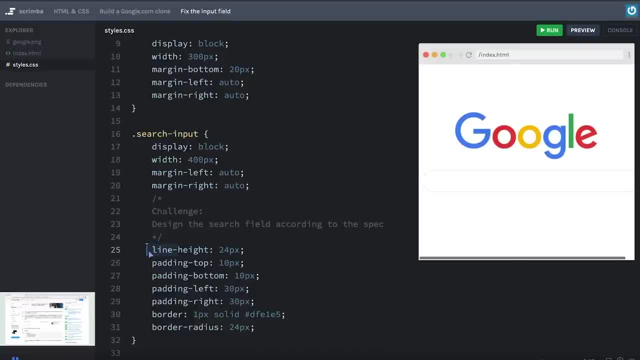 So if that was a little bit confusing and you prefer to just use height, that's totally fine as well. It's more important that you are using what you're comfortable with that and that you are doing it the 100% correct way according to conventions. So just use whatever you want. I. 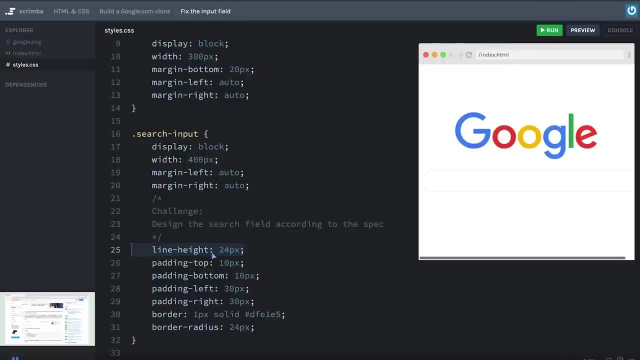 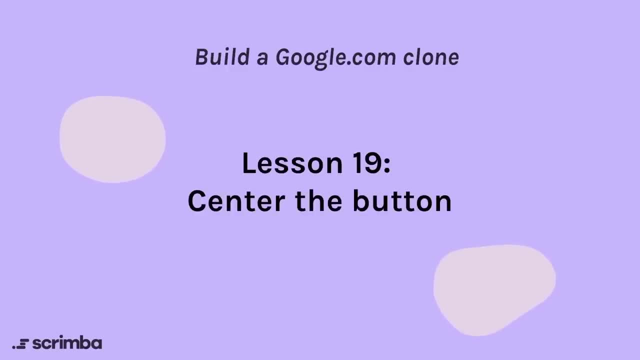 just wanted you to be aware of the fact that this is the recommended way according to Stack Overflow. With that, let's move on. Okay, now we're going to add the first button to our Google project, So I'm going to head over to. 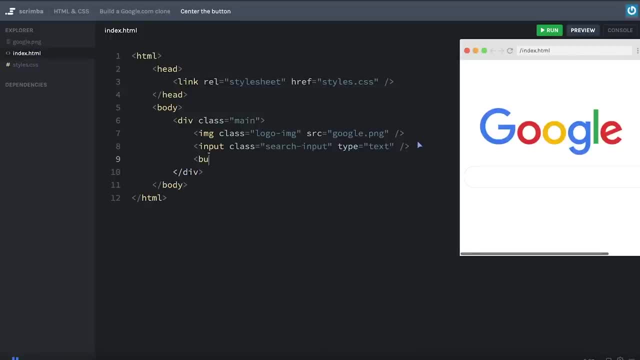 the HTML And here beneath the input field, I'm just going to type button like that And this will be the Google search button. So there we have. it doesn't exactly look good, But don't worry about that. Now I want to give this a class as well And a class name you'll often see used for. 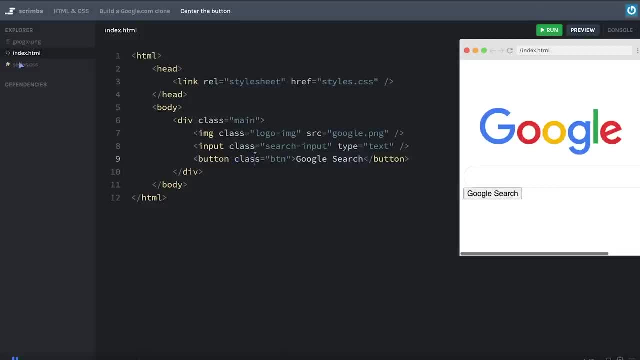 buttons is simply B, T and like that. Okay, now that we have that, I want you to center the button and add some space above it. So go ahead and use the class selector to select this button and solve this challenge. Good luck. 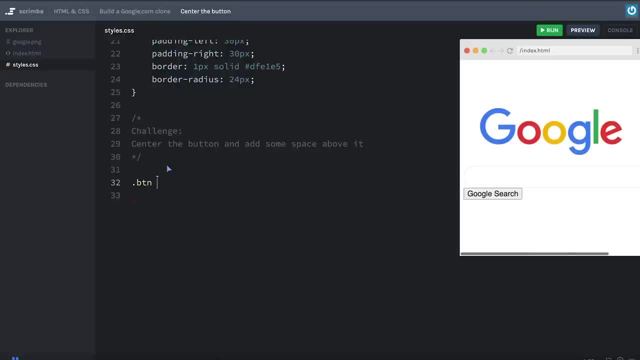 Okay, so what I'll do is do dot vtn To select the button here. you might have been tempted to simply do margin left auto and then margin right Auto. However, that doesn't seem to do anything. Why is that? Well, if you remember the 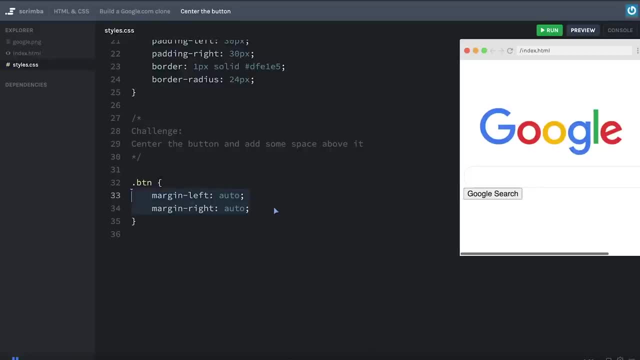 criteria you needed in order to use this technique to center elements. one of them was that you need your elements to be display block, whereas buttons are actually display inline by default. So if we do display block, boom, there we go, the button is centered. And now you might ask: well, what? 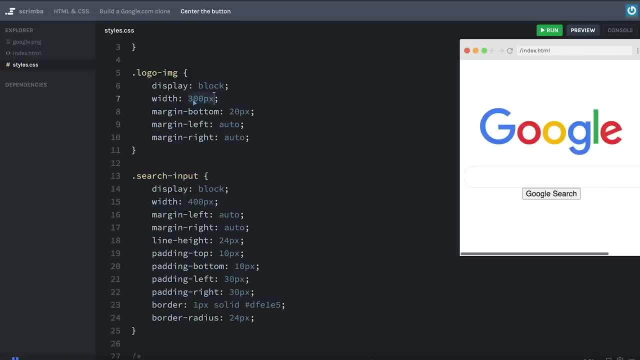 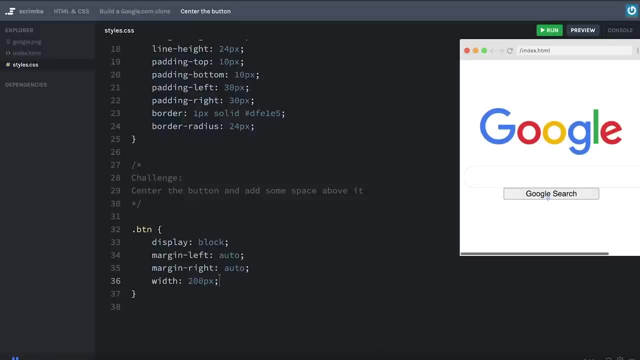 about the width. we also set the width on the input field And the logo. Well, we could do that as well with this one. let's do with 200 pixels, for example. However, it's not needed, Because if we remove the width, you can see that it still has a width. 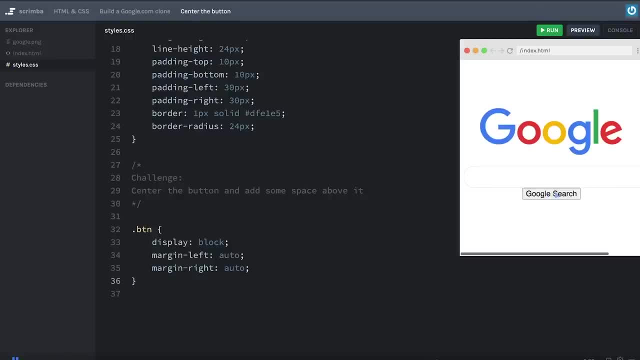 which is certainly not full width across the entire page. So it kind of has an implicit width without us setting the width. So, even though it is a criteria that your element needs with in order to use this technique here, in order to center it, you don't necessarily have to set the width. 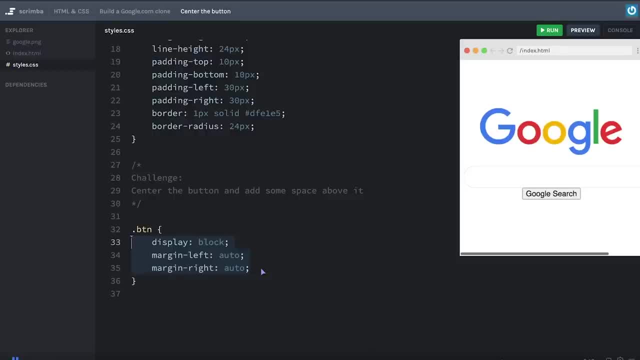 yourself If the element already has some kind of width, so it works perfectly fine, just doing display block and margin left right, auto in this example. Finally, we are going to add some space above it, So let's do that. I'll do margin top and do, for example, 30 pixels. Yeah, looking pretty good. 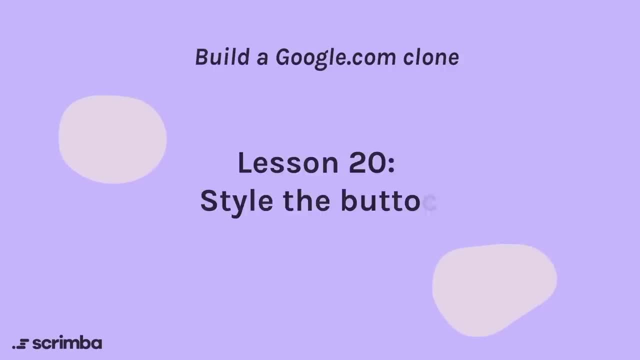 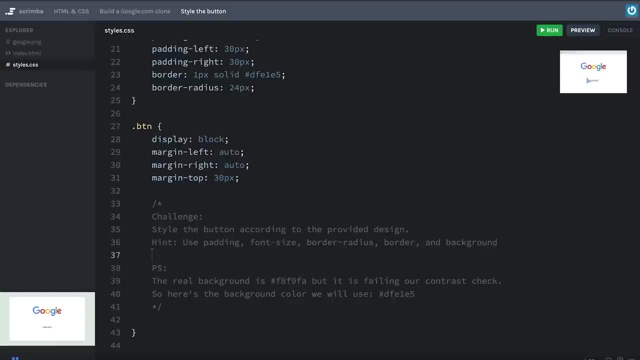 Great job solving this challenge. Let's move on Now. we are going to style the button in our Google project Because, as you can see, this is how our button currently looks, But this is how we want it to look, So we got to do a bunch. 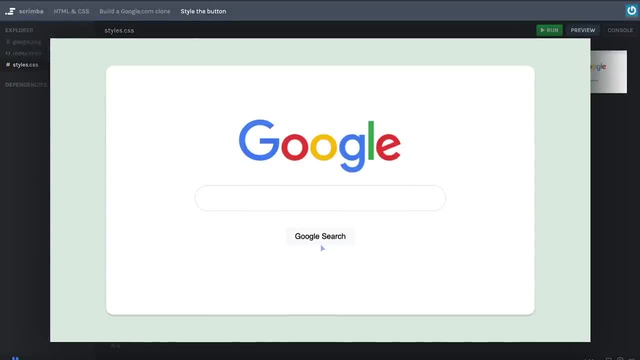 of changes. However, there's one thing I want to change actually on this googlecom homepage, because notice how low the contrast is between the background color of the button and the background color of the entire website. It's hardly possible to see that there's any difference, And that's not. 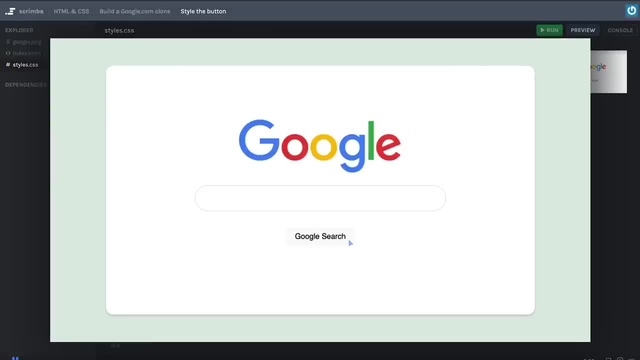 good, because it reduces the accessibility of the site and makes it hard for people who are visually impaired to use it. Actually, to prove this, let's take these two colors- the light gray here and the white- and put them into a contrast checker online, For example, this one right here on user. 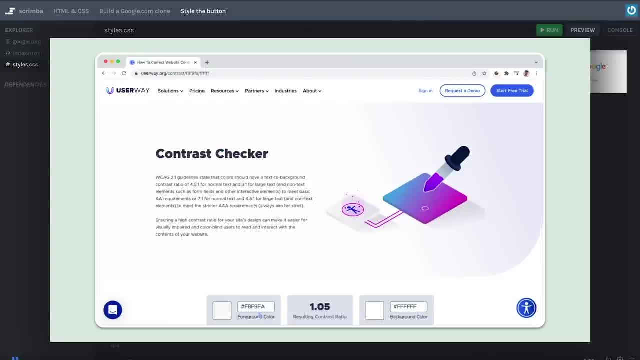 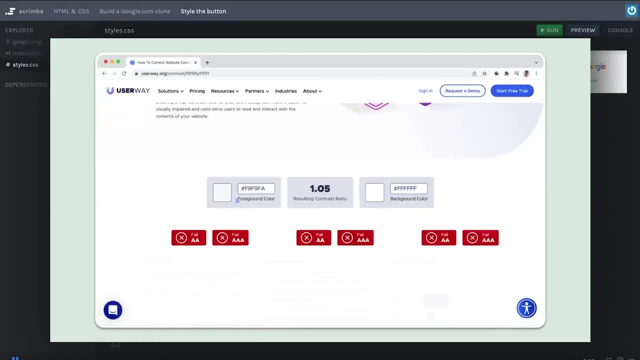 rateorg. They have this nice little contrast checker where you can paste in the foreground color and the background color and then get a contrast ratio. And this f8, f9, f- a hex color- is the one that Google is using, And if we scroll a bit down, you'll see that Google indeed fails. 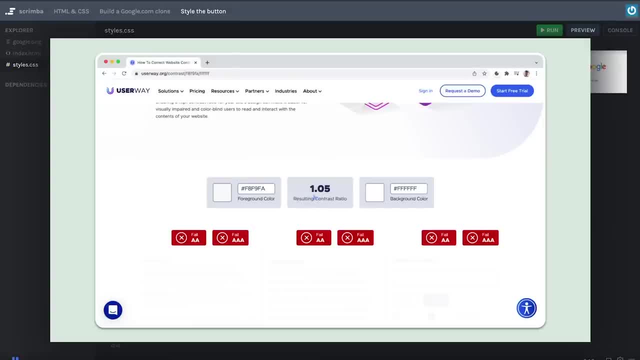 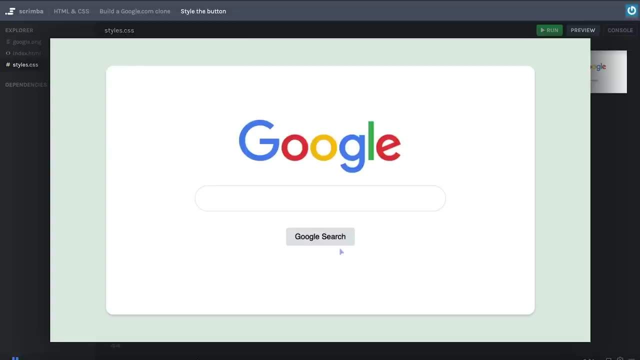 Miserably on this test. complete failure. The ratio is 1.05, though it should have been 4.5 or more. So not good Google. So what we will do instead is change the background from this to something like this: Here you can see, it's much easier to see that it is indeed a button, So even 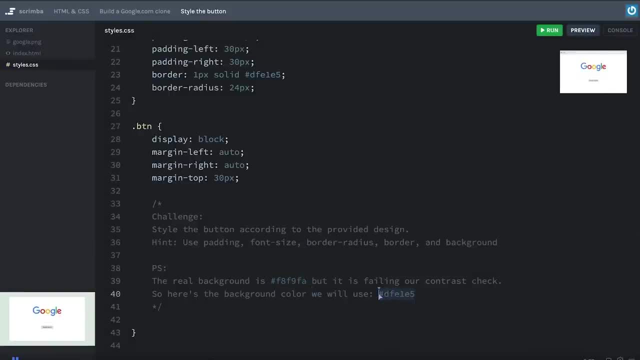 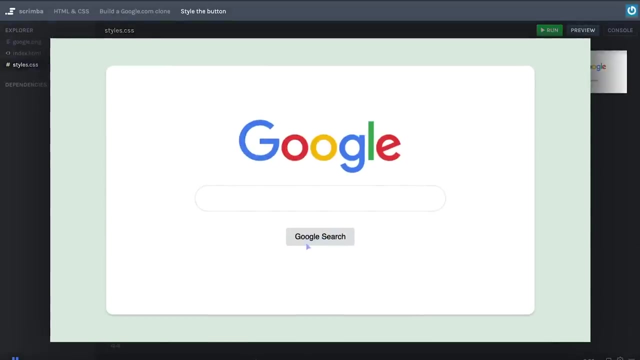 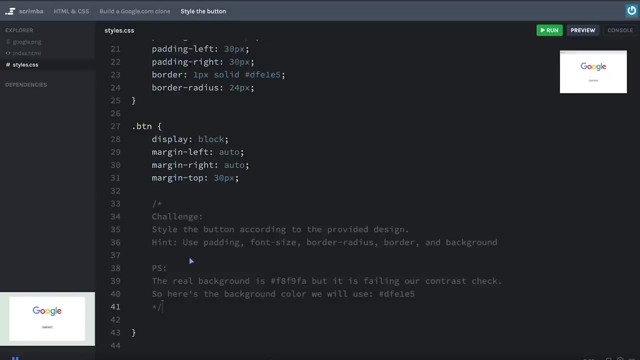 though, the real background color is this one right here. we are going to use this one right here, So, with that in mind, I want you to style the button. of course, that is, go ahead and do this right now, and then I will show you the solution afterwards as well. 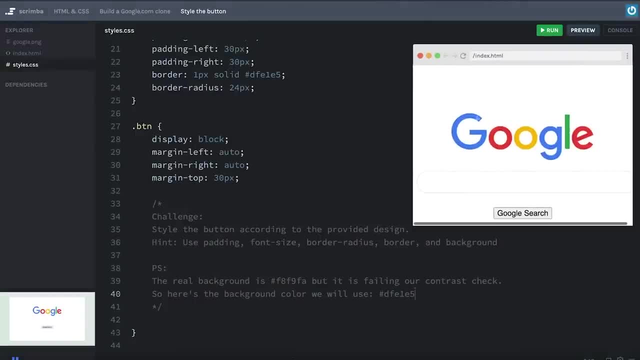 Okay, let's do this. I'm going to bring up the example here, have it on the side so that we can see how it develops, And then start with the background color, as we have the value for that one down here. Round like that. Okay, next I will try to see what is the. 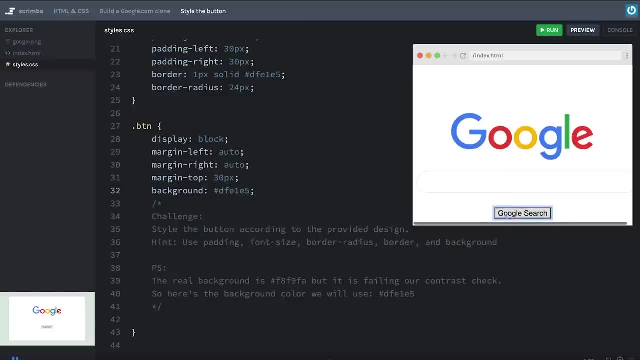 most apparent difference between this button and this one right here. Well, the border is certainly different. This button does not have a border at all, Whereas this one has got has a border, So let's just remove it. border None like that. Okay, good, Now we 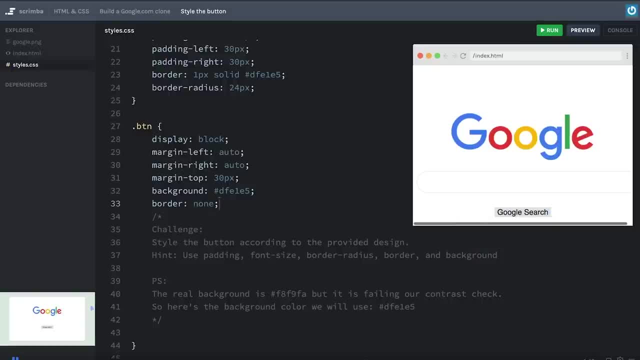 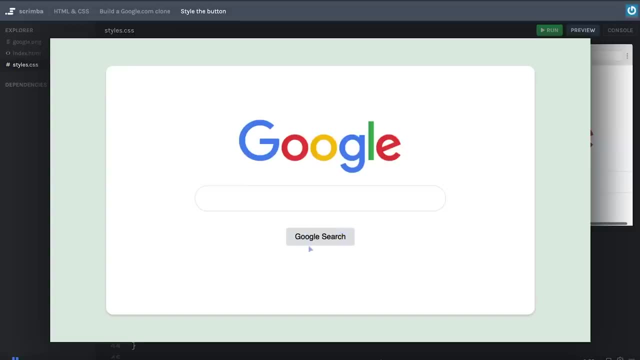 can see that the text is much more crammed into this box than it is this one right here. So that is the padding. And also you can notice that there's more padding on the left and right hand side than on the top and bottom. So I'm going to try to add, for example, padding. 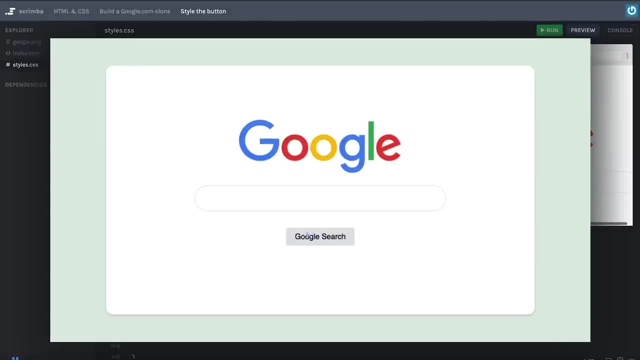 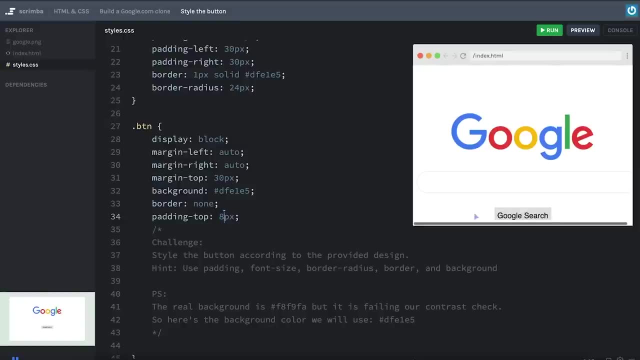 top five pixels. Yeah, it actually looks like this one here has more than five pixels, maybe because this space is still pretty crammed, So I'm going to do, for example, eight. Yeah, I think that is more like it. I'm going to give that on the bottom as well, Like that? 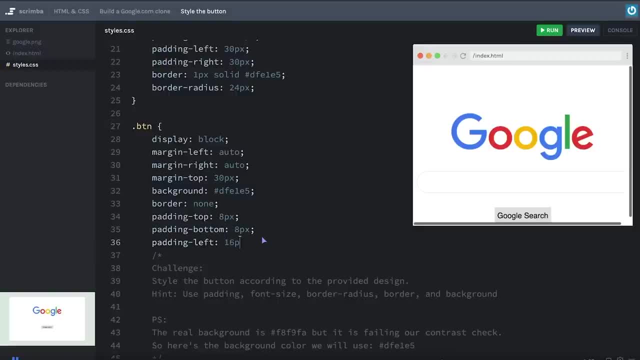 On the sides. we're just going to try the double padding: left, 16 pixels, padding right, 16 pixels, And you know what? I think that button and our button looks pretty similar in size. So next up is the border radius, because you can see, this one is totally rectangular versus this one has softer corners. 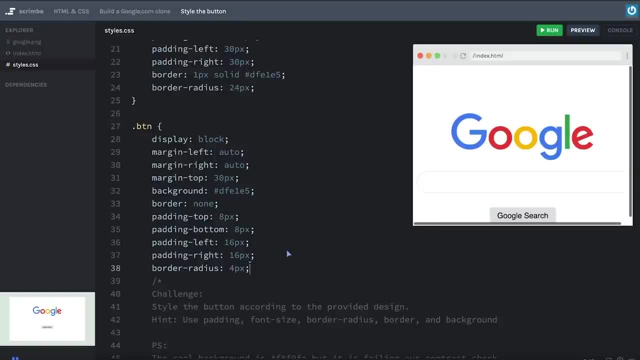 So I'm going to do border radius something like four pixels. So that is pretty good. The final minor adjustments I'm going to make is reduce the font size ever so little from what it is here down to what it is here. I mean it's almost identical, But I happen. 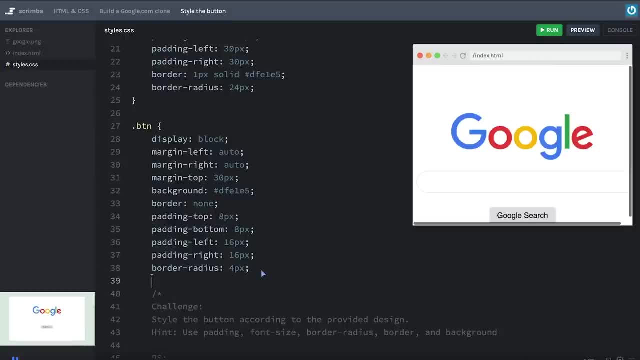 to know that this one is indeed 14 pixels. So I'm going to do font size 14 pixels, And then I'm just going to have to do a few more adjustments. The last thing I'm going to do is reduce the width of the button as well. While I'm done with the unmute button, I am going to increase the width of the button by one. next to that, I just want to make sure that you're paying attention to the list of values that I've chosen, and how many I've chosen, So let's quickly go ahead and reviewing. 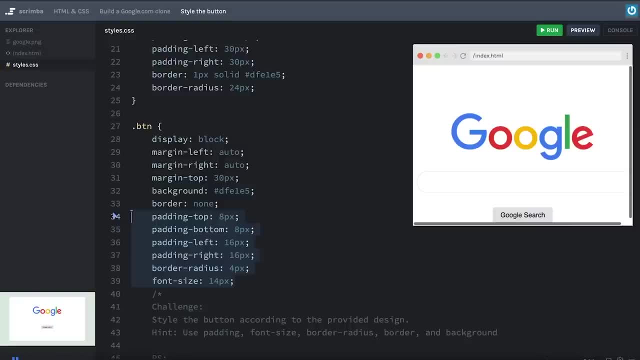 the list of numbers. Then we can see that I have more than five pixels And we can see that maybe it's like the last one. And then I have the second button and the third one, And now we have the third button, And then we have the fourth button. 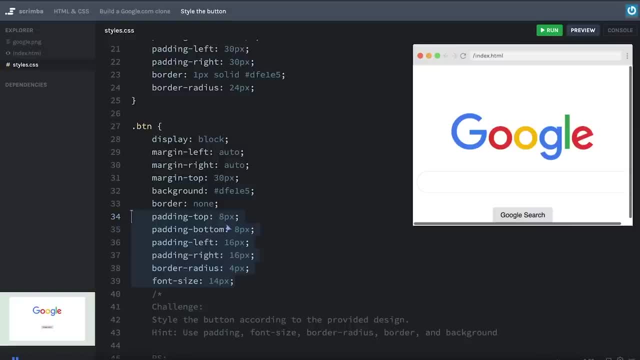 And in the end, I still have 12 pixels. So we're going to have about three and a half pixels here, And then we have something we call the 0.6. range, basically. So, regardless of how your example ended up, good job reaching this far. 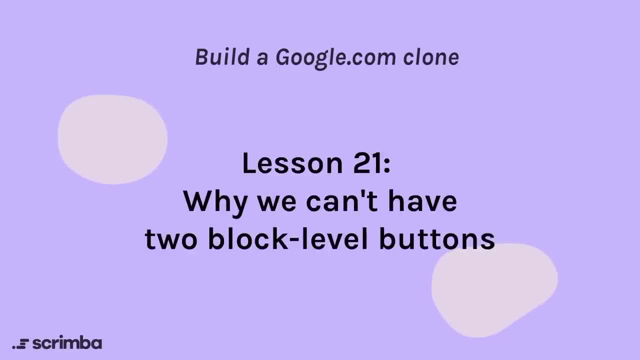 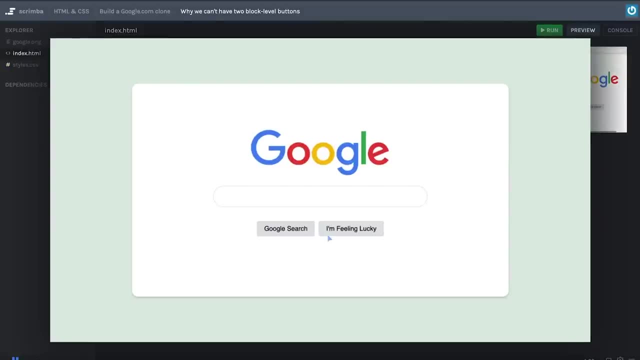 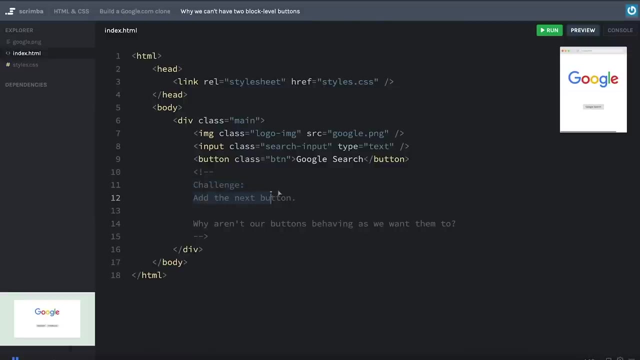 let's just keep up the pace and move on. Now we are going to add the second button to our Google project- this- I'm feeling lucky button right here, And I want you to do that on your own first. So that's your challenge: add the next button And do remember to give that. 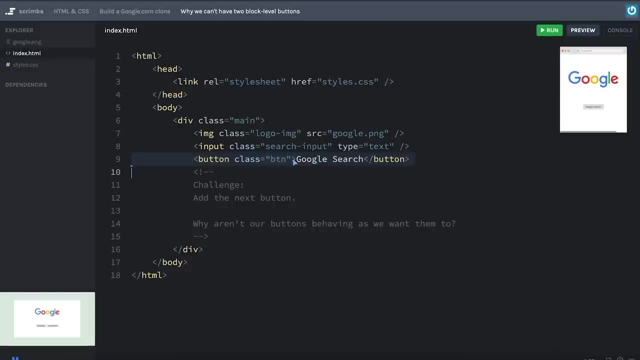 button a BTN class, so that it's styled as our search button. And once you've done that and executed the code, I want you to take a look in the mini browser and ask yourself: why aren't our buttons behaving as we want them to? Because, as you'll see, there's something. 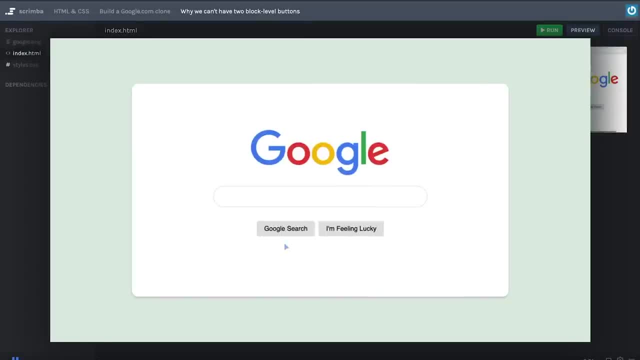 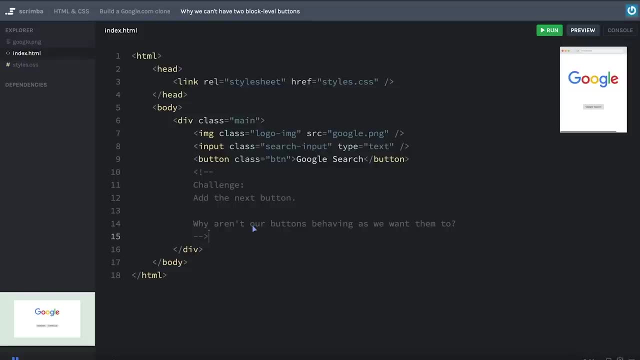 wrong with the layout, at least when comparing it to this layout right here. So go ahead and do that right now And try to think of why our layout is wrong, And then I will do it as well when you return back to me and explain what's going on. 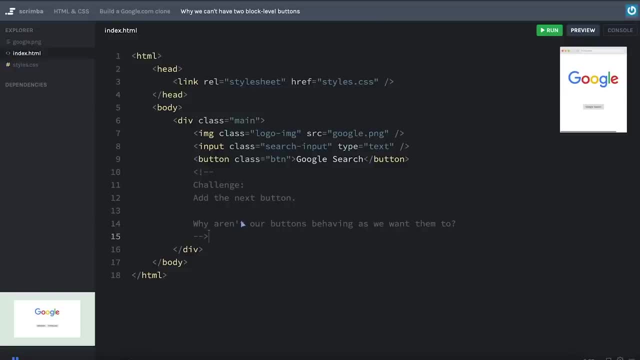 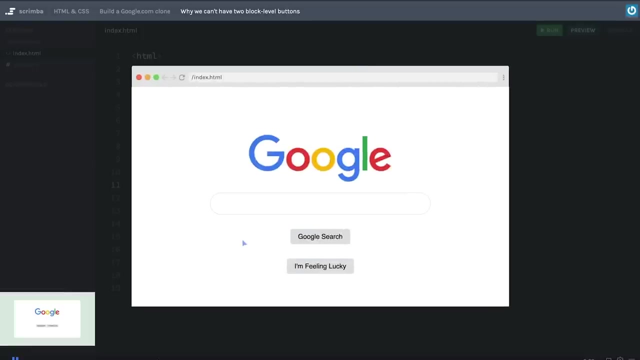 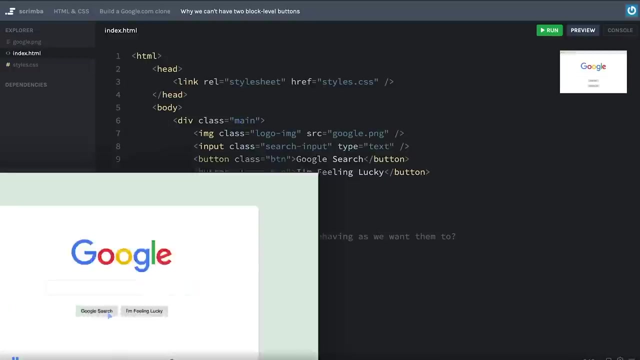 Okay, let's do this. So I'm lazy, So I'm just going to copy this one like that And, right, feeling lucky, run the code And, as you can see, the buttons are now stacked on top of each other. Hmm, what we can do in order to figure out what's going on here is actually: 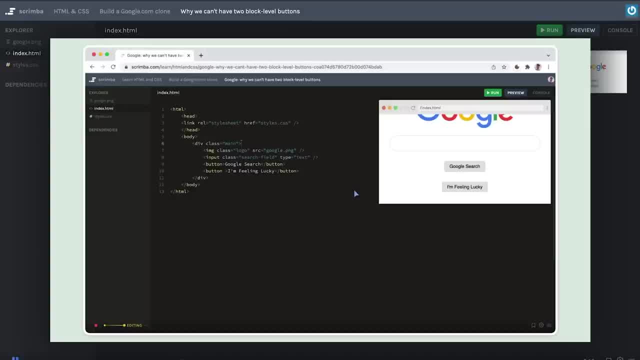 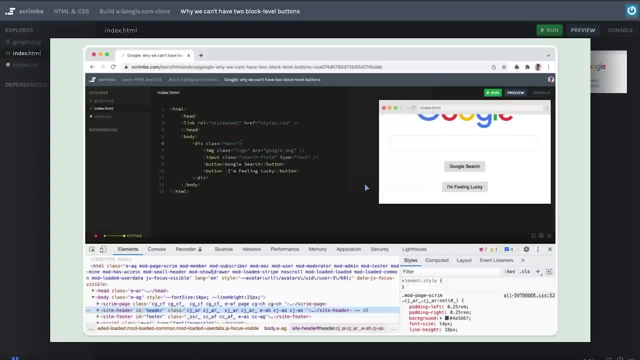 use the built in dev tools in the browser, which you've seen a few times. So let me show you this debug session using slides. I'm going to right click in the nav bar and then choose inspect, open up the elements tab and then click on the selector. 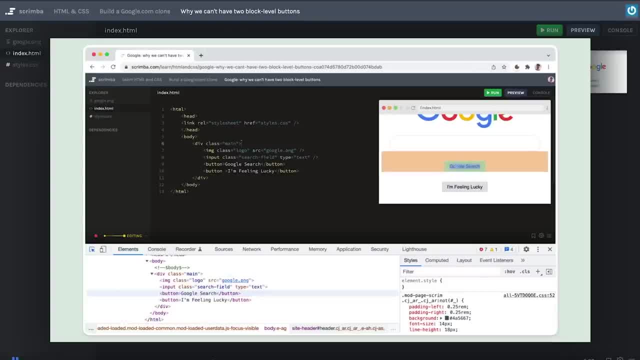 icon here so that I can select this button by hovering over it And then down in the styles tab. I can scroll down until I see the box model for our button And what you'll notice is that our button is taking up all the available space on the left hand side. 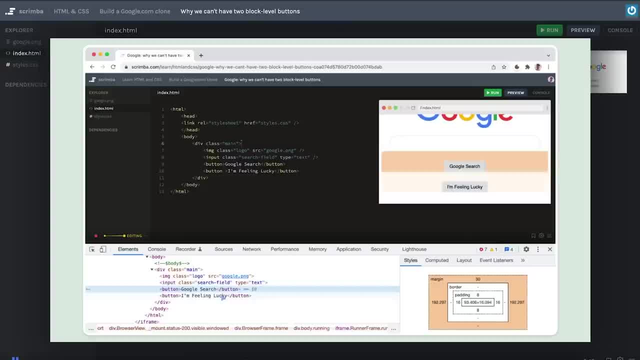 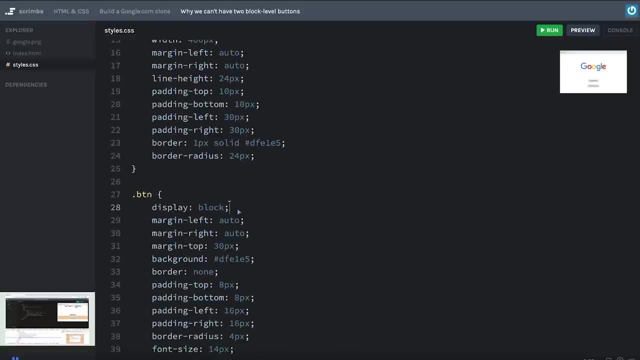 and the right hand side And if you scroll down to the second button you can see that that button is also doing that. that is because they are display block, Exactly this line right here, If you remember from previous lectures. display block kind of takes up all of the available space on. 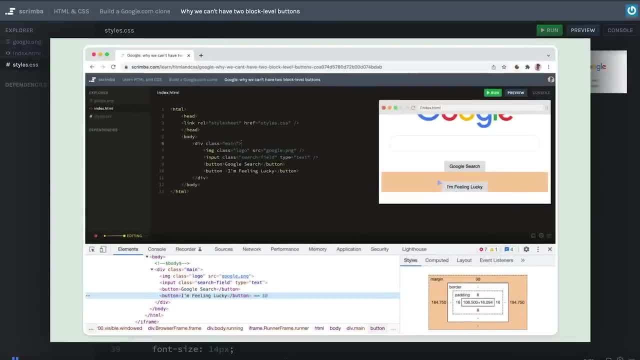 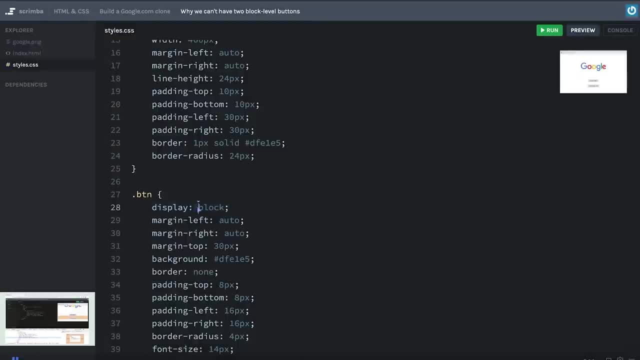 the horizontal axis. So, as we said earlier, display block stacks on top. we aren't able to get the layout we want if our buttons are display block, And then you might be tempted to do: well, let's just remove the display block. 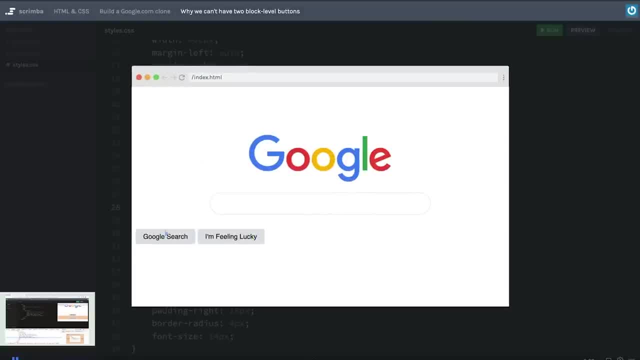 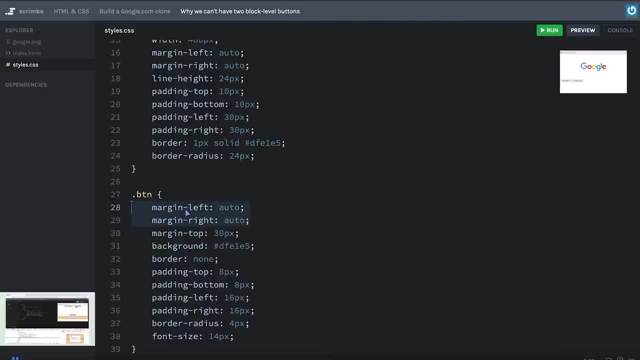 If we do, they will be on the same line. Yes, they are now inline elements, but they will just be crammed all the way to the left hand side because margin, left, right, auto doesn't work. If you remember, from the lecture about centering, you learned that display block. 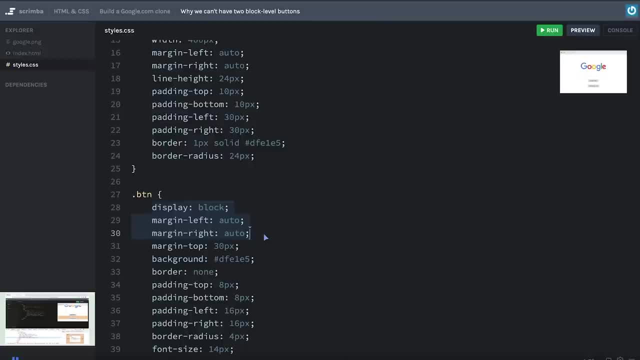 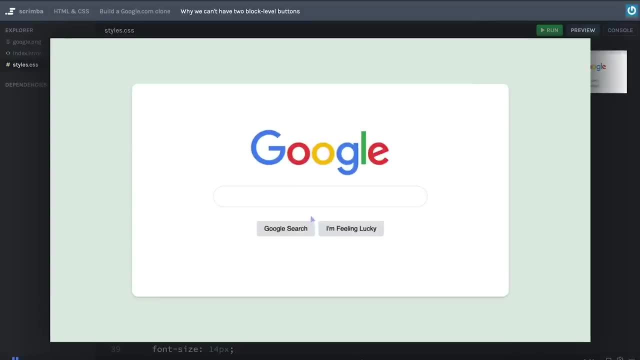 and margin, left, right, auto works together in order to center something. you can't have just one of them, which means that in order to go from this layout to this layout, we have to use a different technique for centering The elements, And there's actually two ways we could do this. There's the simple and inflexible. 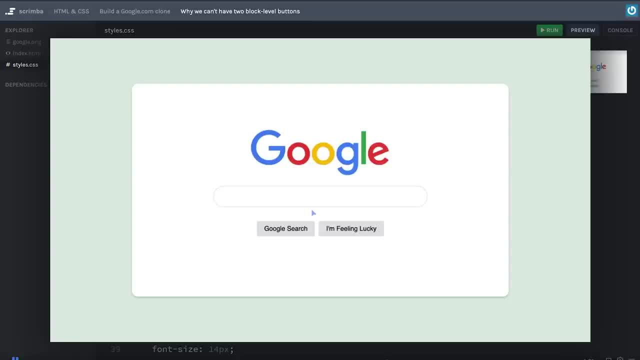 way using text align. And then there's the slightly harder but super flexible way using flex box, And since you're going to use flex box several times throughout this course, I want you to get familiar with it right away. So in the next scrim we're going to talk. 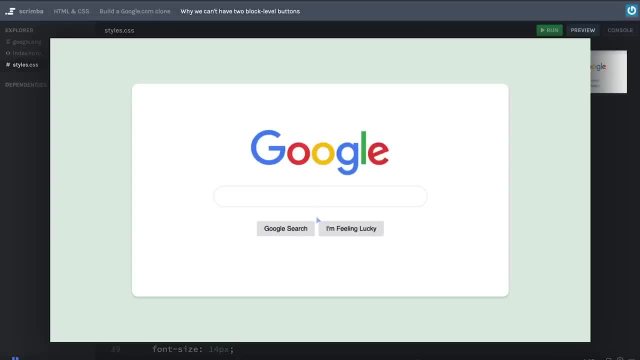 about flex box. But before we do that, I just want to show you the simple way as well, so that you've seen it, because, as you might remember, from one of the very first scrims in this section, something called text align, in order to align our text either to the left, right or center. 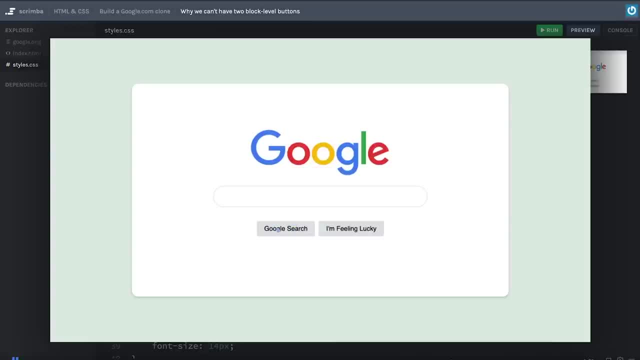 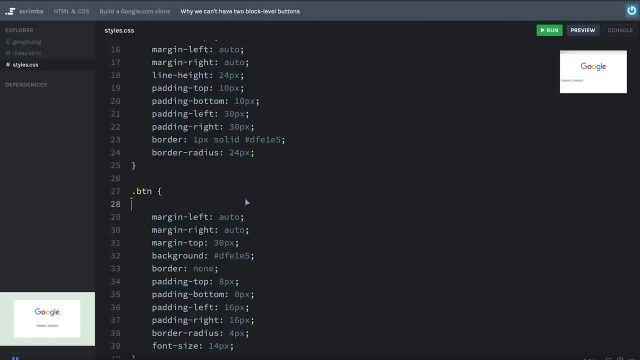 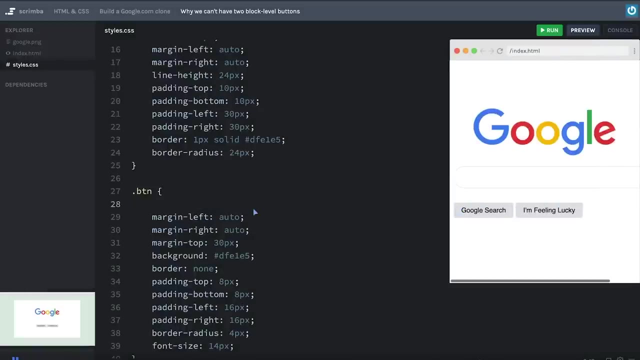 Now, the text align property actually works on all inline elements, not just on text. So what we can do is remove the display block from our buttons. As you know, that turns them into inline elements and they are crammed to the left And, as inline elements, only take. 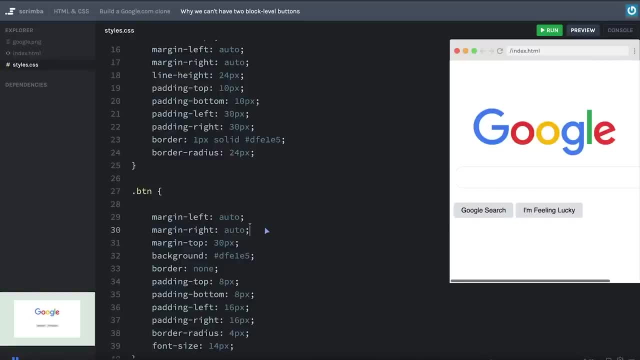 up the available space they need according to their content. there is no available margin to use, So auto here, which basically means take up whatever available margin there is, serves no purpose. So we can remove both of these two as well as you can. 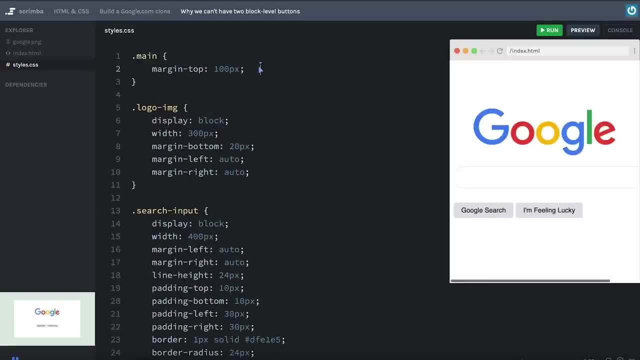 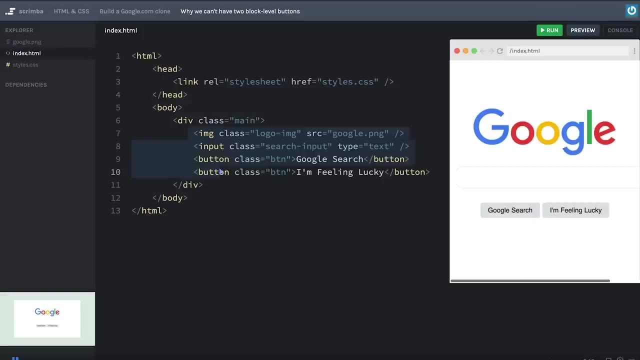 see, it made no difference. And then we can move up to the main, the parent. we'll do text align center, like that. and boom, both buttons are now centered. So here we have told the container, the main element, all inline elements inside of it, should align to the center. And 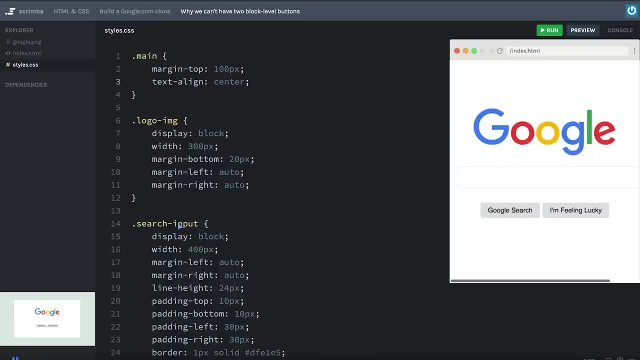 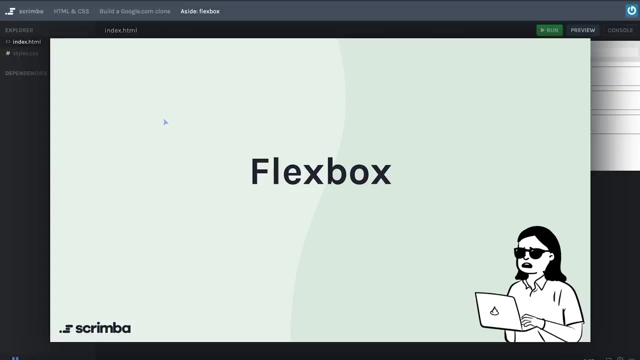 we can move the main element to the center. So that was the easy button, flexible way of doing this. Let's, instead of using this technique, move on to do it how the pros do it: using flexbox. Flexbox is everywhere. Let's just have a look at Twitter, For example, here: 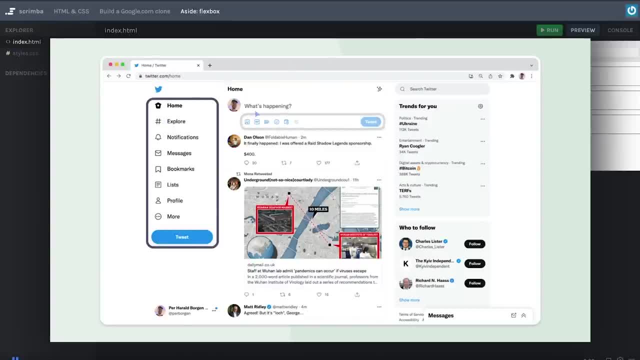 the menu on the left hand side is created with flexbox, as with the tweet options menu and the timeline itself. And guess what? these trends for you and who to follow? it's created with- you guessed it- flexbox. So this is something you need to learn. Let's imagine that you have a e commerce. 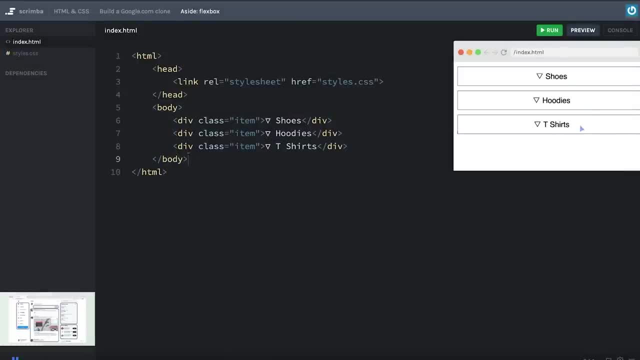 website, which you can see here, that sells shoes, hoodies and t shirts. well then, you'd probably have a navigation menu like this one, where users can click and then probably open up a sub menu or something like that, As you can see, the items stack on top of each. 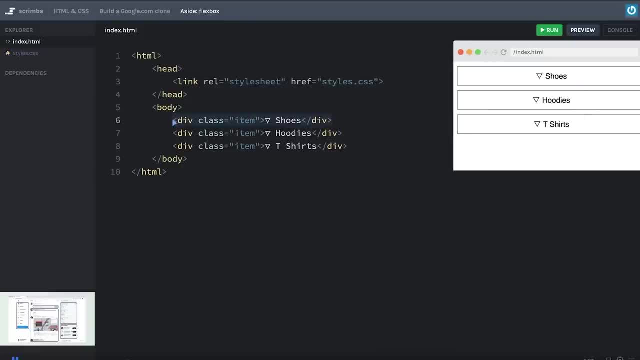 other. that is to be expected, as these are devs, and devs are display block. they want to take up all the available space in the width. And if you're wondering how I styled these, we can head over to the stylescss And just have a quick look at that, you can. 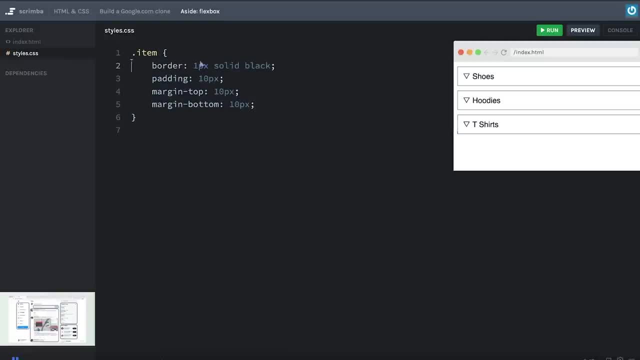 see, I've aligned the text to the center inside of all the items. had not done that, would have been aligned to the left. Also, there's a border, as you can see. there's some padding on the inside and there's some margin in between the elements. Now the question is: 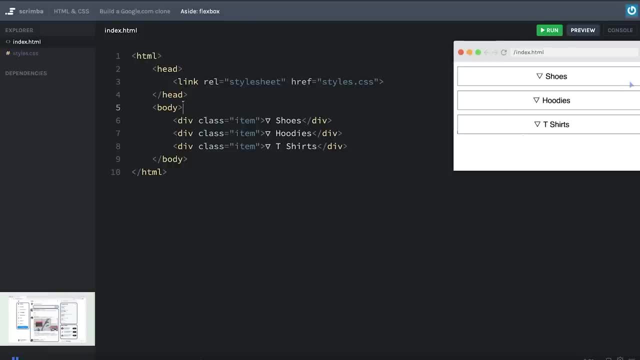 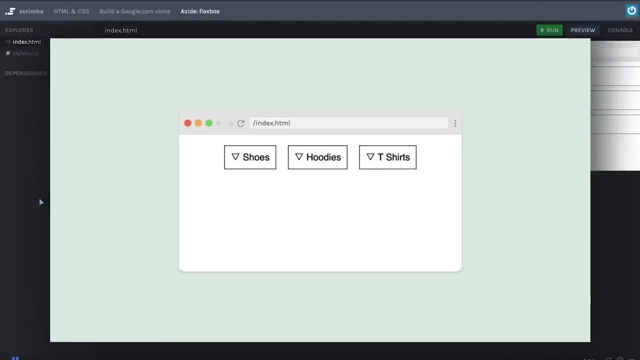 what if I, instead of this vertical layout, wanted a horizontal layout, which is more common for so called navigation bars, So something that looks like this: Well, this is where flexbox comes to the rescue, And in order to turn this into a flexbox layout, 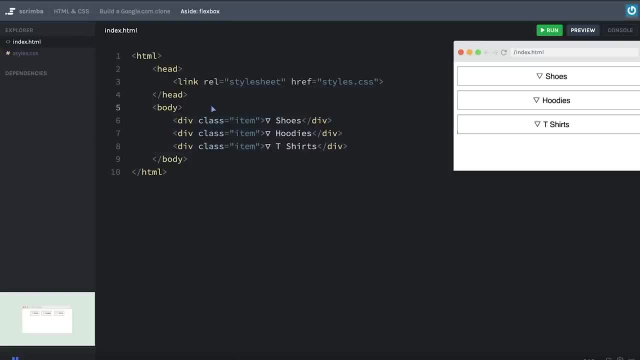 I would first have to wrap these three items in a container, because a flexbox layouts always consists of a container and its direct children, So let's wrap it in a div And give this a class of, for example, nav dash wrapper like that. If I run this now, nothing happens. 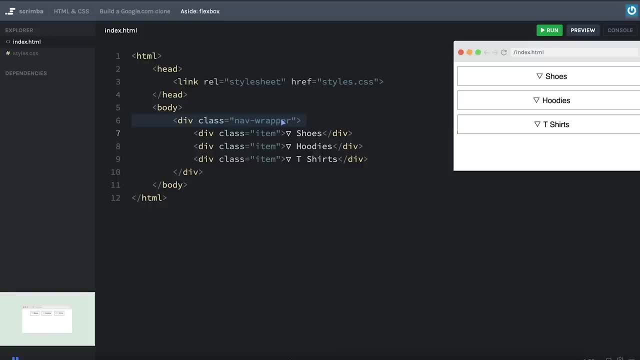 Because this, as you know, are invisible unless you give them any styling or content. So let's head over to the stylescss And now target the nav wrapper like that In order to turn this into a flexbox container. all I have to do is write display flex and boom suddenly. 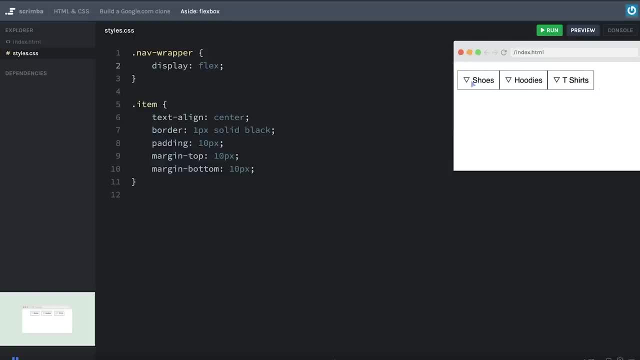 we have forced our three divs into one row. Now this layout flows from left to right along the horizontal axis, And that is pretty significant, given that these items were displayed block by default. But flexbox, as powerful as it is, overrides that and forces them on to one. 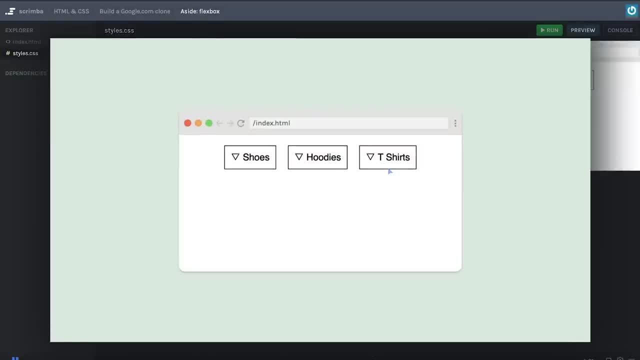 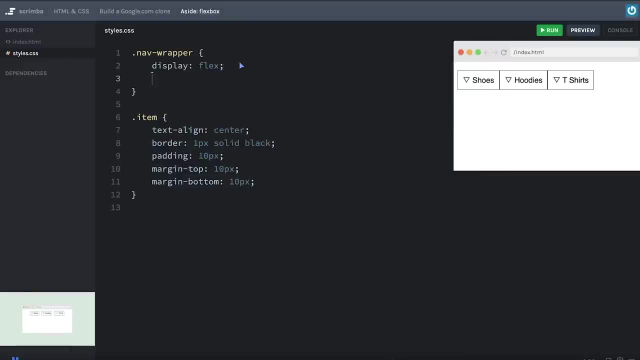 line. However, we haven't got quite the layout we want yet. As you can see, it's centered And there's also some space in between the items. Now let's start with the centering, because flexbox now has control over these items and can decide where along the main. 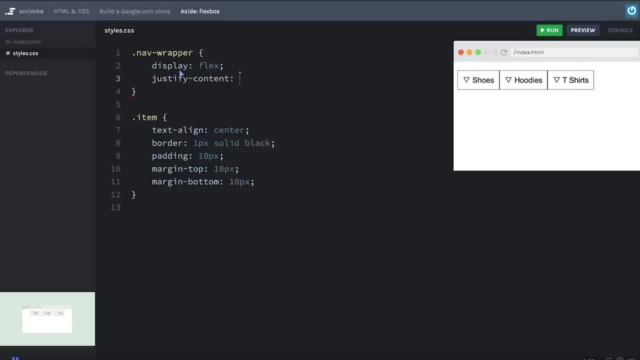 axis they should be positioned. So we can do justify content- that is a little bit of a weird name for a property, But that's just how it is- And then set that to center. like that. Now all of the items are centered. Final step is just to get some spacing in between these items And that is done with. 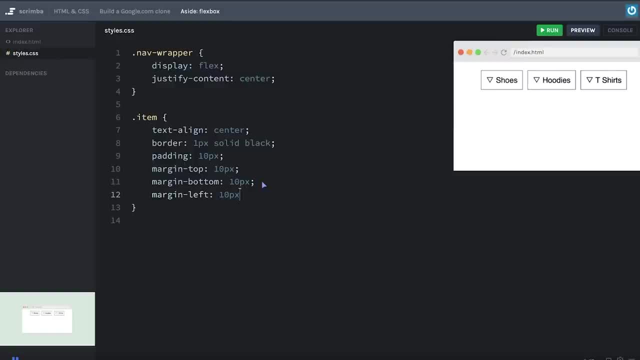 our good old friend margin through the margin left, let's do 10 pixels And let's add the same thing on the margin right, Like that, And there we have the layout we wanted. Now, a final cool thing I want to show you is that we can do, for example- and here as well, that'll. 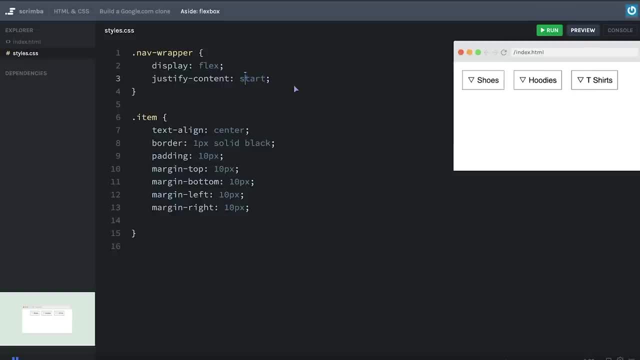 push it all the way to the right hand side or start at the beginning, Or alternatively, you space dash around. That's pretty cool. Now we've distributed all the white space around each of the items And another one is space between. now all of the available space is between the items. 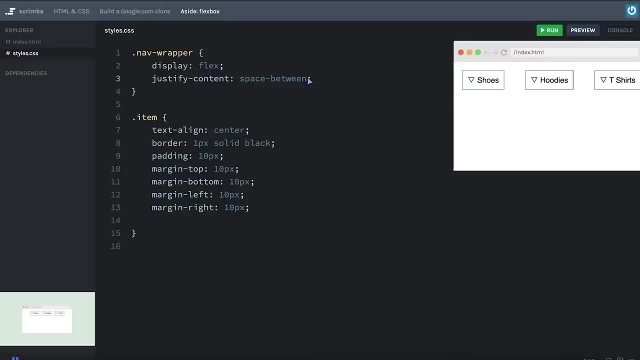 So they're spread out like this. Now we are getting ahead of ourselves here. I just wanted to demonstrate this to show how powerful flexbox is. what you are going to work with is the center here. So with that, let's return back to our Google clone. 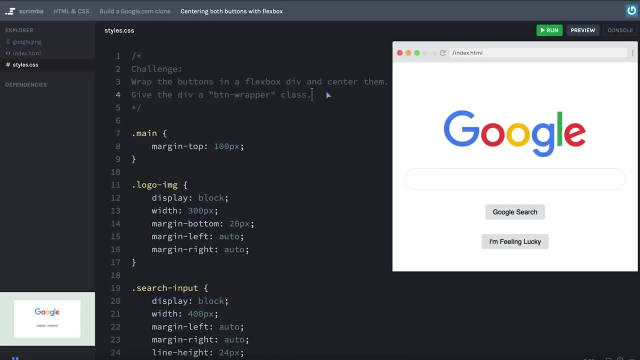 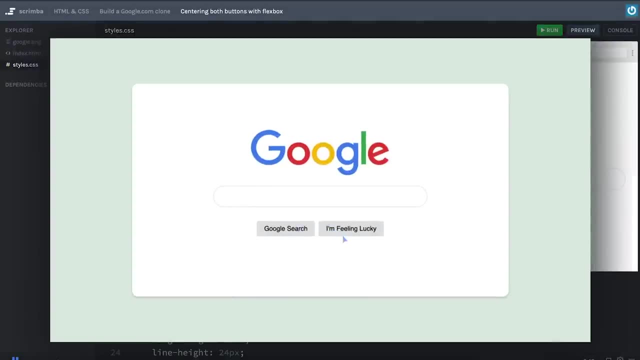 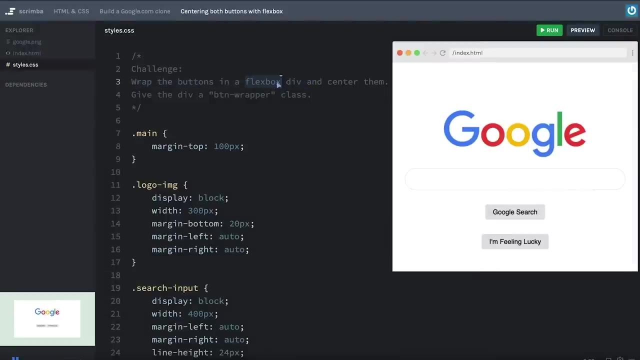 Okay, we are back at our Google project, And now your job is to center these two buttons besides each other, meaning getting to this layout right here, And the way to do that is, of course, using flexbox. So you'll wrap the two buttons in a flexbox div and then center them. And then also, I want you to 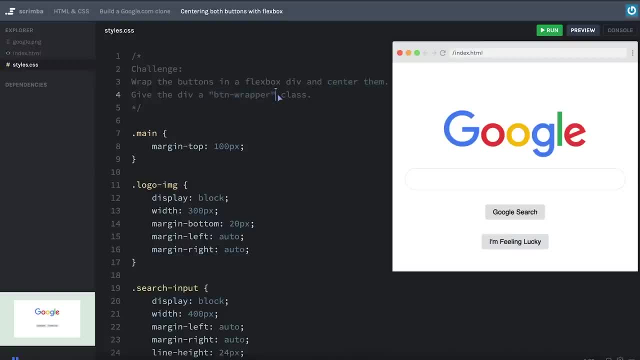 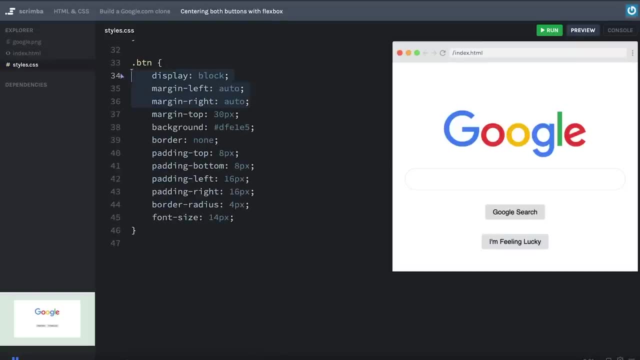 give the div a class of BTN dash wrapper, So you'll need to modify both the HTML and the CSS here Now, before you start. I'm going to remove these three lines here, because they are solely there in order to center our buttons using this display block and margin. 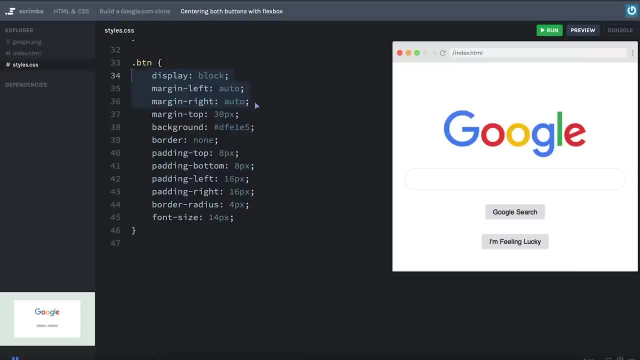 left, right auto technique. However, now we're going to use the flexbox technique, And we don't want to use both techniques at the same time, because that'll just be confusing, as they will affect each other. So I will remove these lines, And now you're left with this. 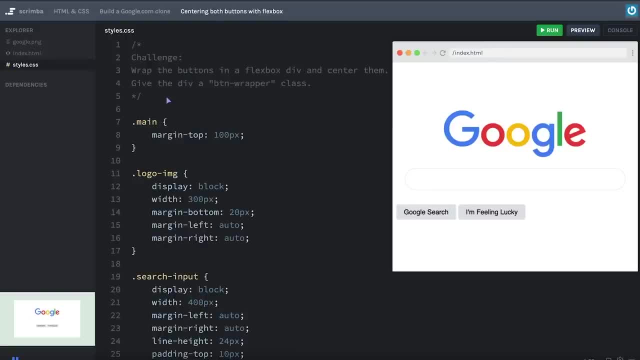 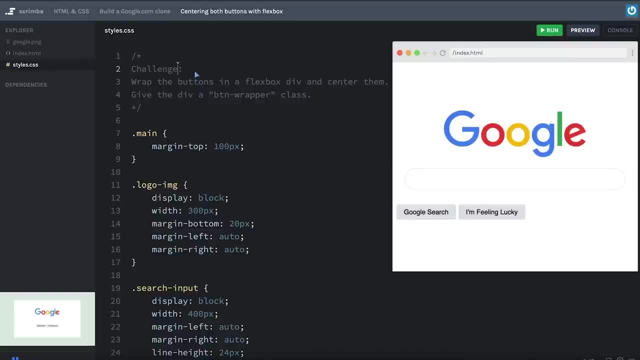 left aligned layout here. So please take over here, do this challenge and then return back to me when you've done it, Or when you feel like you've done it. You need some guidance. Good luck, Okay. hopefully that went well. If not, no worries, We'll do it now together. So I'm 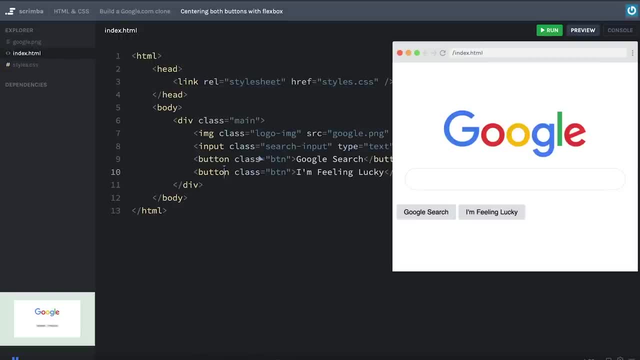 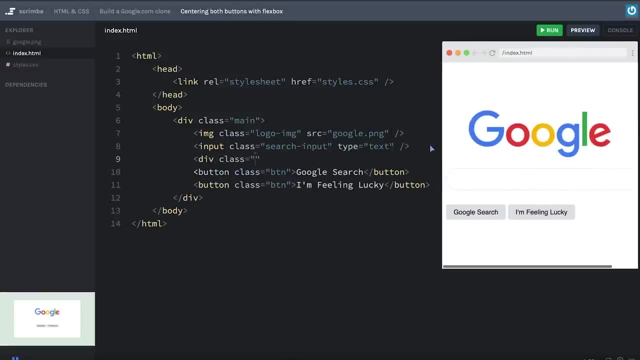 going to start with this flexbox div that we want in our HTML. it should wrap our buttons and only our buttons. So we want to start it up here. if class of BTN dash wrapper, I'm going to indent my buttons, Then end the div down here. So now it is simply wrapping our two buttons, If I run this code. 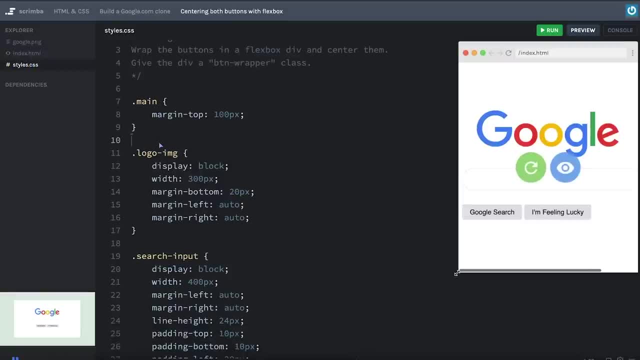 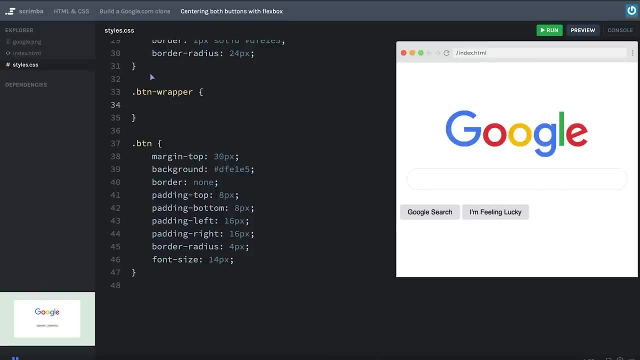 seemingly nothing has happened. But under the hood we have the button wrapper which we can target using BTN dash wrapper like that, And then we can do display flex. that's turned our div into a flexbox And now we can use the justify content and do center. 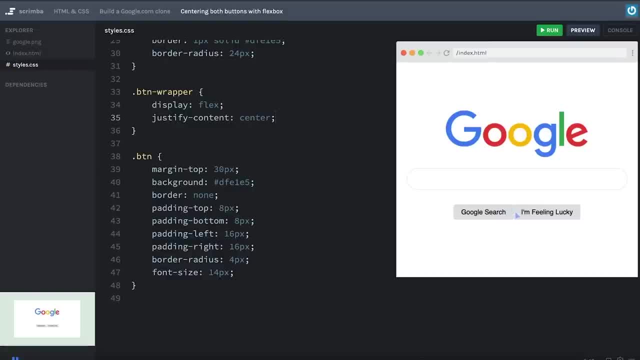 like that, And here you can see both our buttons are centered. However, they are totally crammed into each other Now there's no margin in between them. So in order to fix that, we want to add a little bit of margin left and right to these buttons. So I'm going to do. 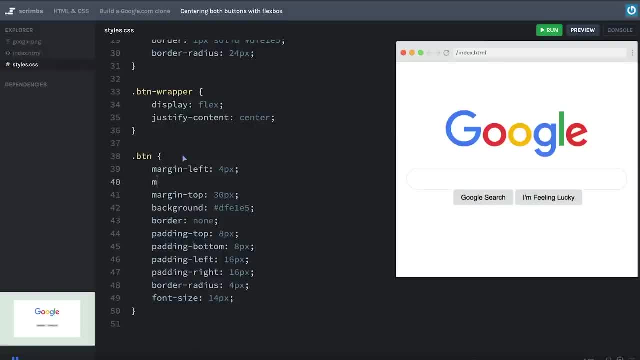 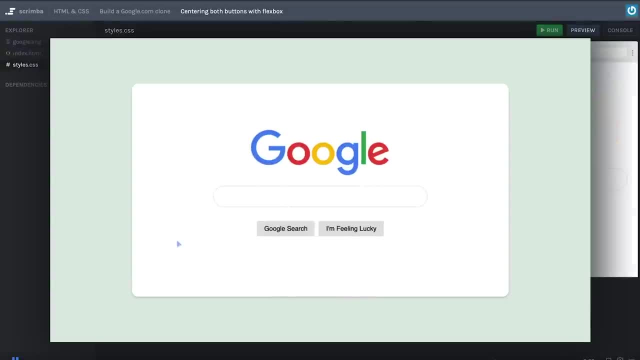 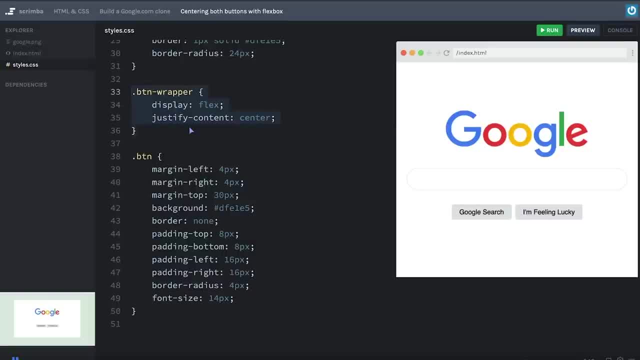 also, if you're a little bit confused about flexbox, that is totally okay as well. we're going to work with that several times throughout this course. you'll get more opportunities to practice this. just feel proud that you've at least dipped your toes into flexbox as. 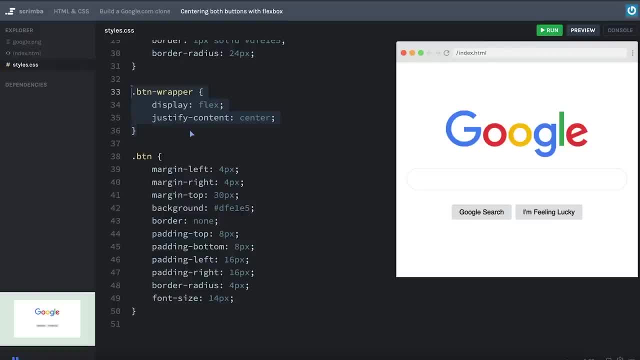 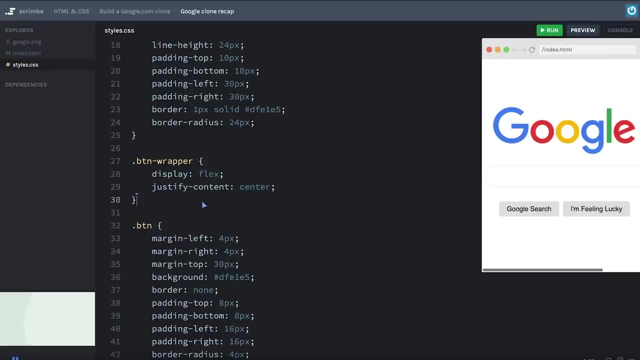 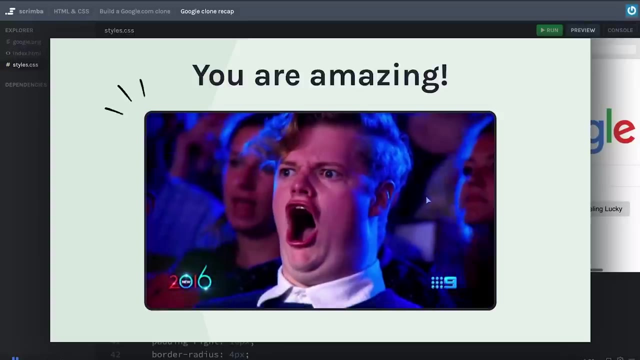 that is a super important tool for any front end developer. So great job, Let's move on Now. there's one final thing I want you to know, and that is that you are amazing. Okay, because you have taken your very first step into the world of CSS, And that is more than most. 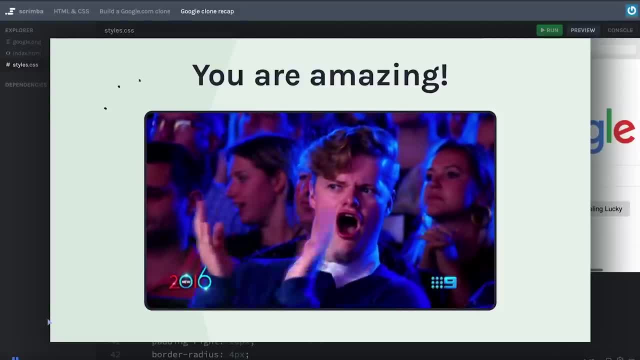 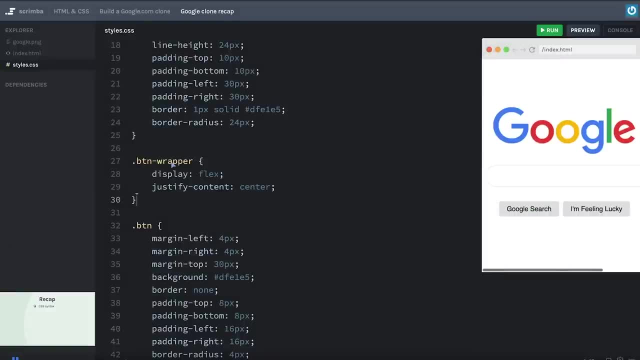 people ever do. So take this moment to feel great about yourself. And also, let's take this moment to recap what you've learned. Starting out, you learned about the CSS syntax. that is how you select elements and also use properties and values. And then you learn the key concept about inline. 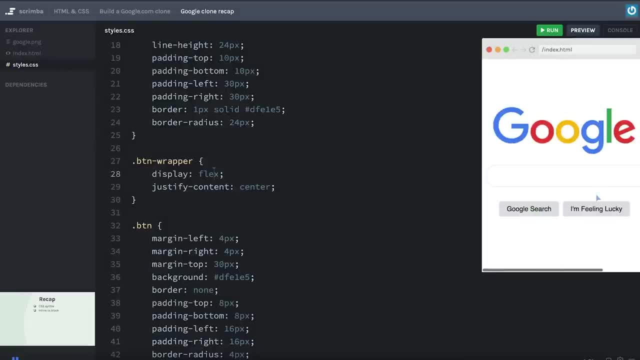 elements versus block elements. So block elements stacking on top of each other, like these two, and inline elements standing kind of in a horizontal line, like the buttons here, Moving on. you learned about margins, which is how you create white space outside of elements. 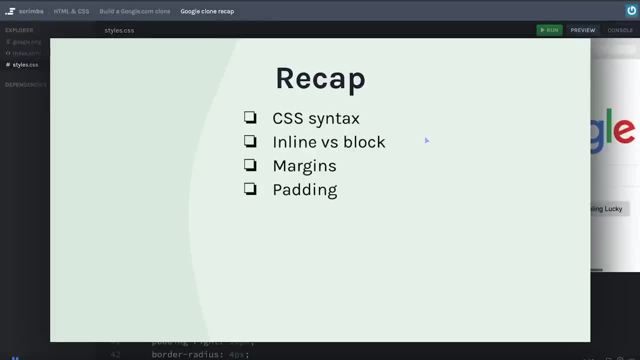 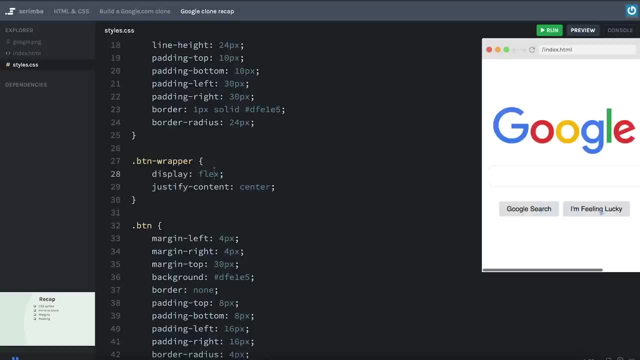 for example, above the Google logo here, And you learned about its close cousin, the padding, which is how you create space on the inside of elements, for example in between the text and the edges of these buttons. Also, borders is what is between padding and margin, And we use that. 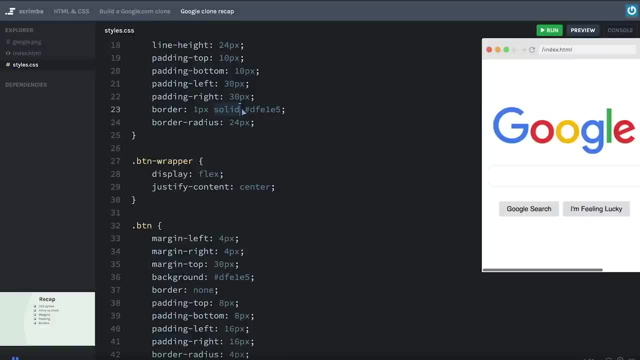 on the input field. here we decided its thickness, its type and color and also the radius of the corners. So we didn't want to sharp edges, but rather soft, circular edges, which we achieved with this border radius property. What we also did was take a closer look. 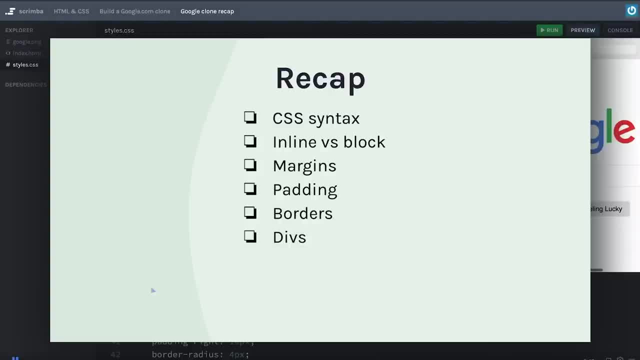 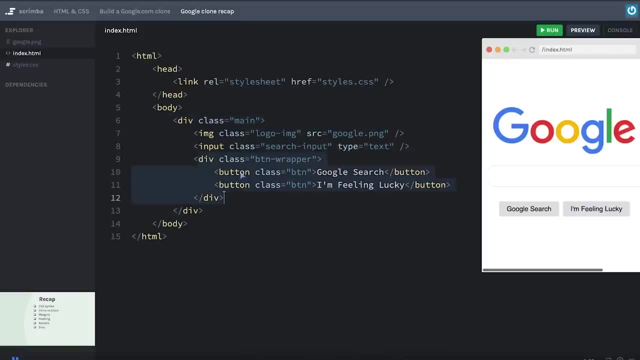 at the div tag, which you saw briefly in the HTML section. This time around, though, you actually created two divs, one to wrap the entire project and another to wrap the buttons, And we had to separate those from each other, So you had to learn about classes. That is the attribute you set, like. 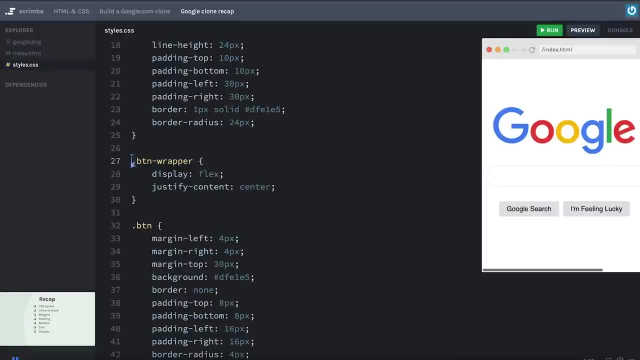 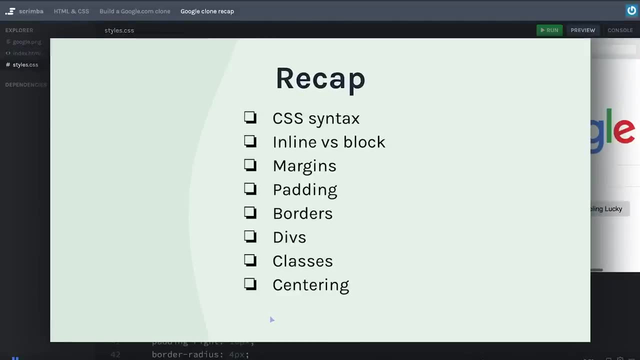 this And you select by using the dot notation in CSS. Also, a big thing is centering in CSS. you learned three different ways of doing this, And the final way you centered elements was through the use of flexbox, a super powerful tool that all front end developers need to be comfortable with. So you have learned a. 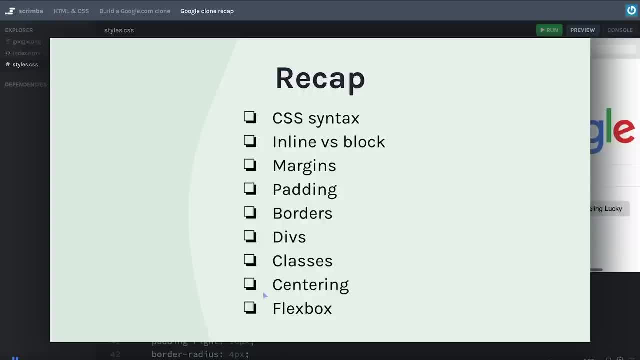 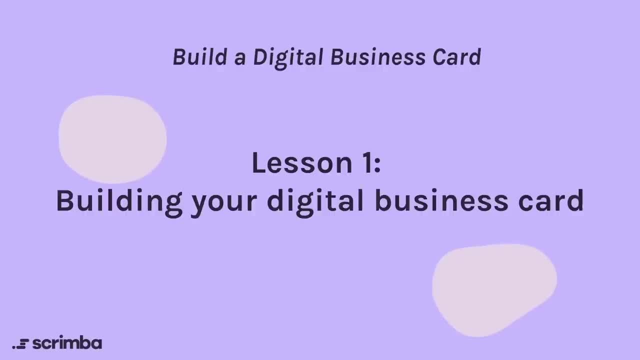 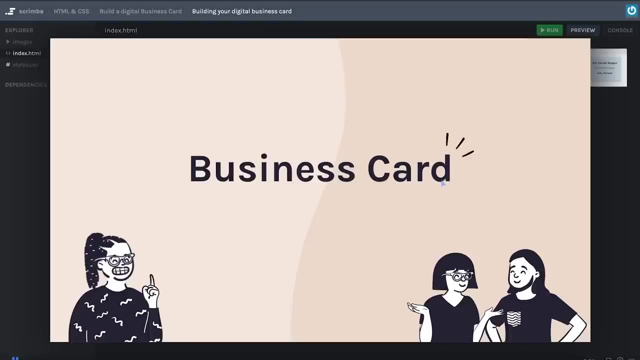 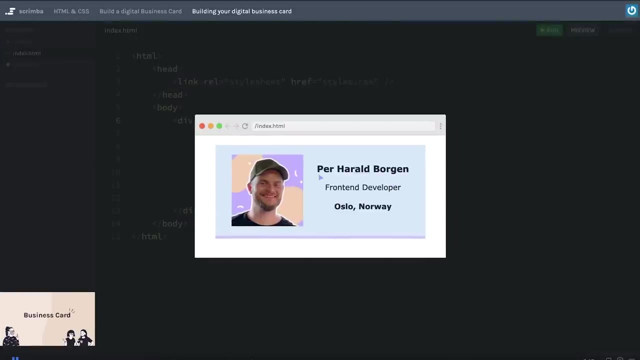 lot. Now I think you should take a little break. you have to digest these things, recharge, and then I will see you back here when you are ready, in the next section. Welcome to the second CSS section of this course, where you are going to build a business card for yourself, And it's going to look more or less like this, though you're going to personalize it, make it your own, not only with your own information, but also with a beautiful color palette of your choice and a font that you like. So you are going to level up your design skills as well as your CSS skills, meaning that this is going to be a lot of fun. So let's just get started. 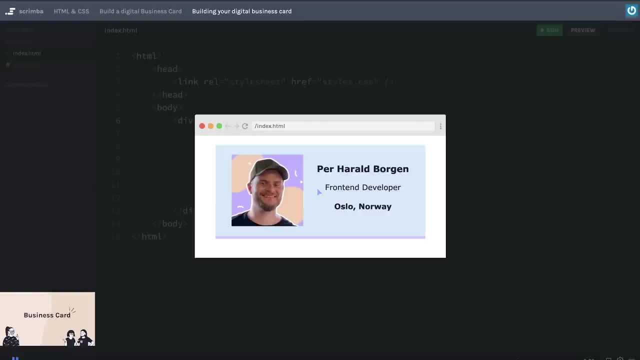 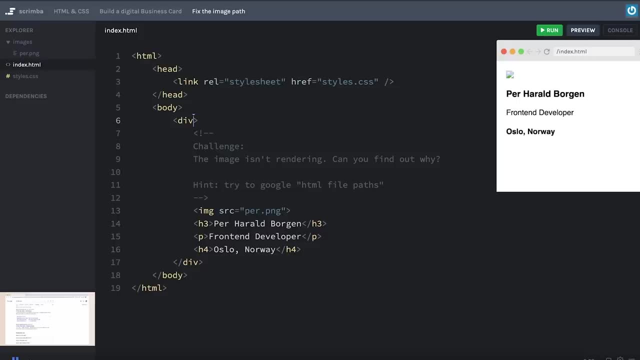 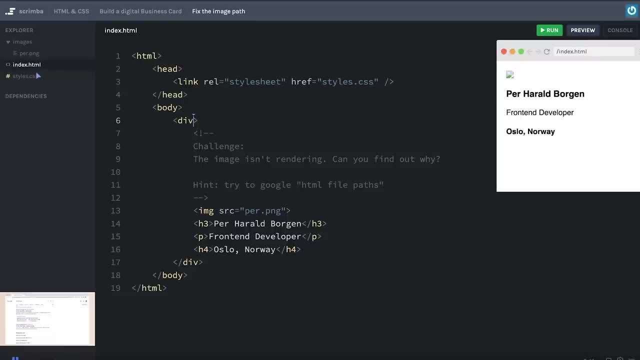 As you can see in the file system, here we have an index HTML file, also a styles dot css file And finally we have an images folder which contains my avatar. it's a PNG file called pear dot PNG. Now, starting with the HTML, it's just a very simple setup with the HTML tag and then the 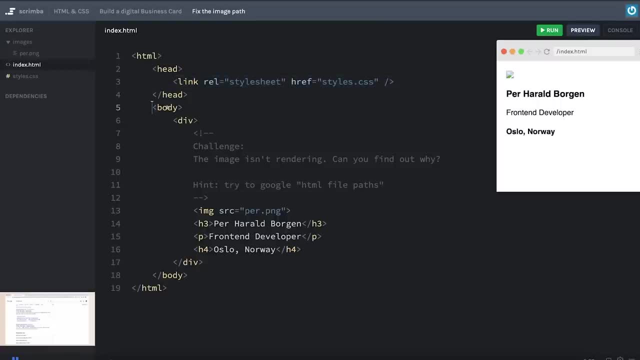 head tag which links to the styles dot css, the styles dot CSS. As for the body, it has one direct child which is a div, which will work like kind of the container for our business card, And inside of that div we have an image tag. 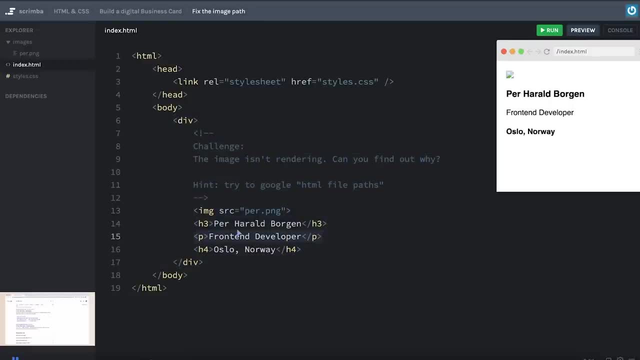 we have an age three with my name, we have a paragraph with the title and an age four with the location. Moving over to the CSS, we only have one rule here. we're setting the margin to 20 pixels on the body And if you remember how this works when we're not specifying either margin, 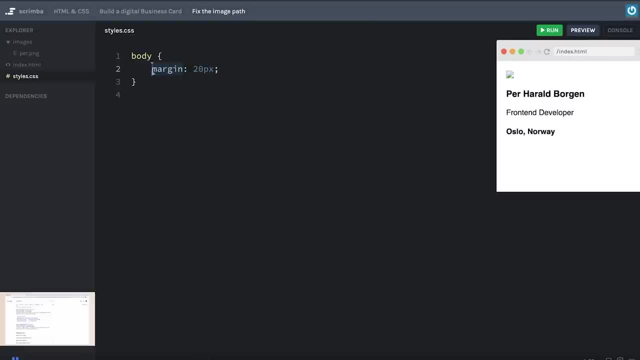 top margin, bottom, left or right, just setting the margin. in general, these 20 pixels will be added on all four sides- on the top, on the left, bottom and right- And that's simply because I want to avoid that these elements touch the edges of the mini browser. So there's a problem though. 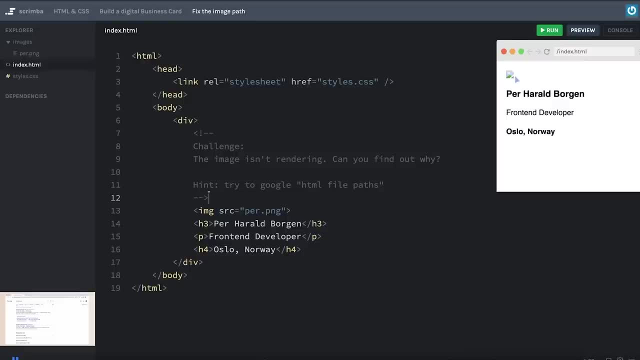 as you can see, the image isn't rendering properly. it's just an icon. that is, as far as I can remember, not how my face looks like, And the problem is in the image tag. So I want you to try to fix it. 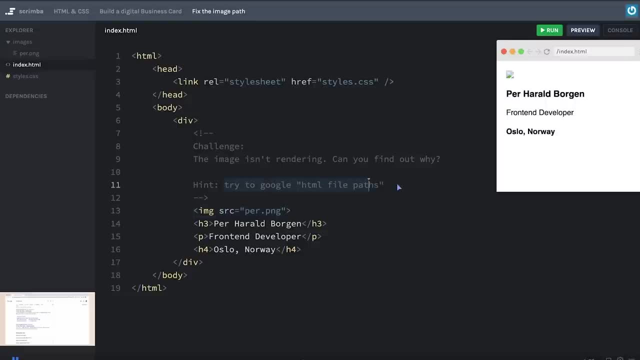 And I'm not going to give you any more hints, rather than, if you're stuck, try to Google HTML file paths. that should help you. So go ahead and give this one a shot, And then I will show you how to solve it as well when you return back to me. Okay, let's do this. Let's take this string. 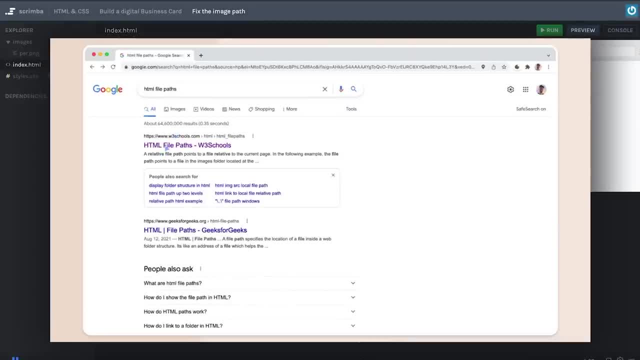 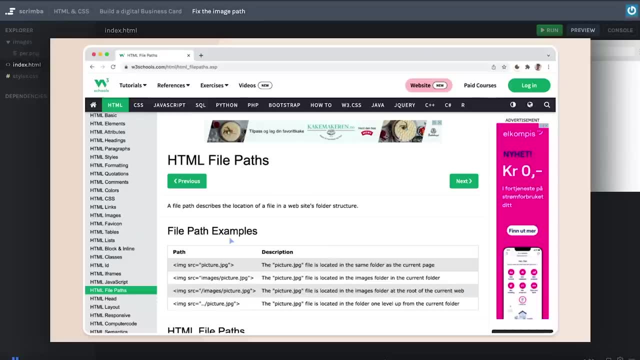 right here and paste it into Google. There you can see that the top result is a w three schools article. Let's head into that one. Here you can see file path examples. Let's zoom in on this one. And if we have image, source equals picture dot jpg, which would be the same as we have here. 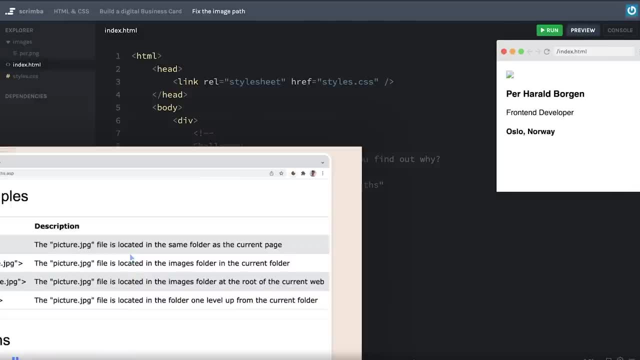 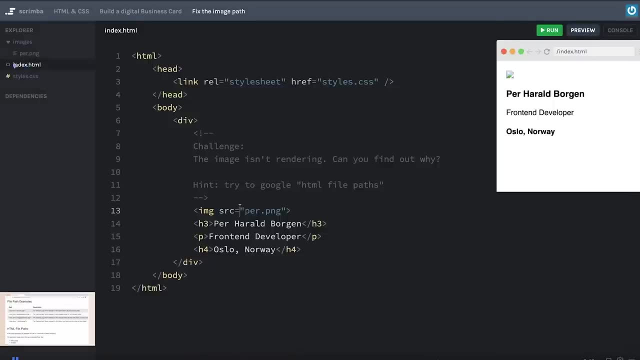 although our image is called pear dot PNG, that means that the file is located in the same folder as the current page. Well, is that the case? now? looking at our current page, index dot HTML, you can see that the image is not located in the same folder as the index HTML, because the image 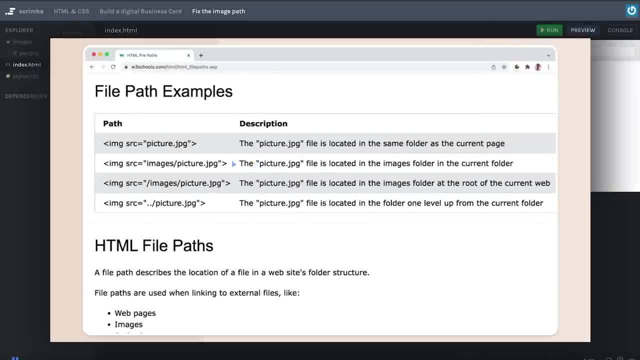 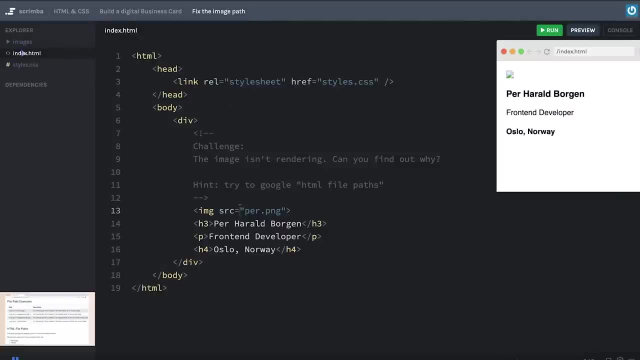 lives inside of the images folder. So what we then might need is something like this, where we do images slash and then the picture name. Here it means that the picture is located in the images folder in the current folder. That looks correct. The images folder is in the same folder as index dot. 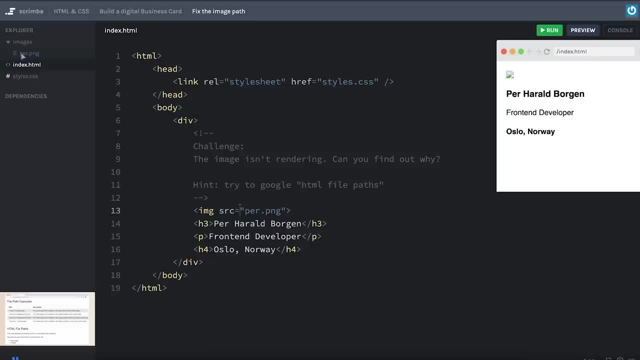 HTML And the headshot of me is located inside of that images folder. That means that we can try to do images like that slash. run the code. Oh, there we go. We have my avatar imported and are ready to move on to the next trim. I'll see you there. 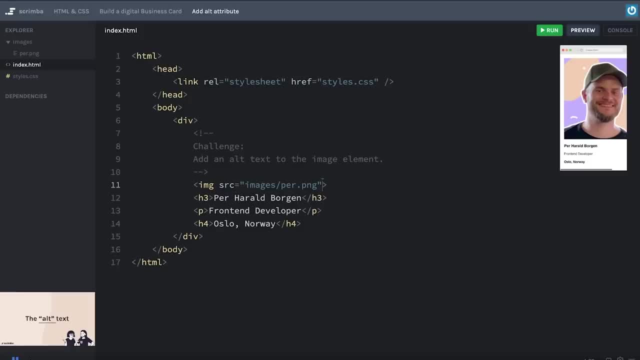 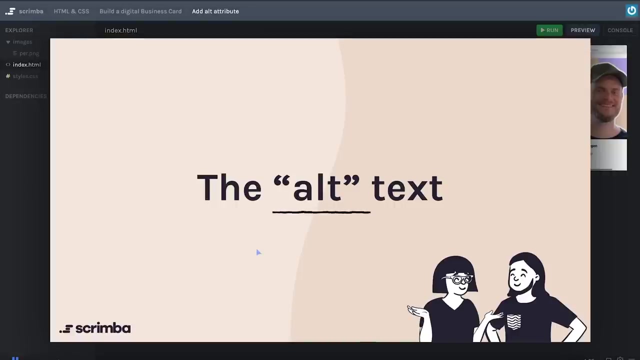 Okay, now we're going to do a little bit of housekeeping here, because this image element actually has a serious flaw, because it lacks an important ingredients that all image tags should have, which is called the old text or the alternative text. That is simply an attribute that 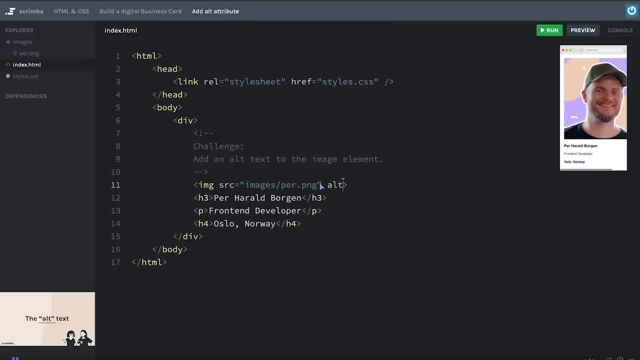 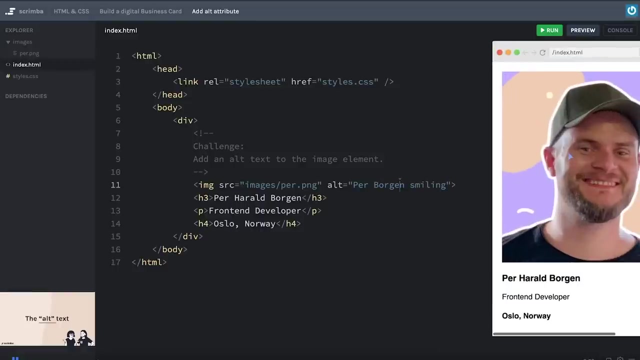 is written like this: alt equals, and then, inside of quotes, you are to write a description of the image. So here we go. description of the image. So here it could be, for example, pear Borgen smiling like that. However, if we run this code now, you can see that seemingly nothing has changed. 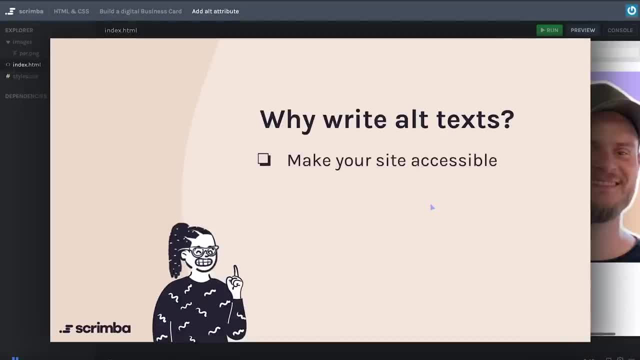 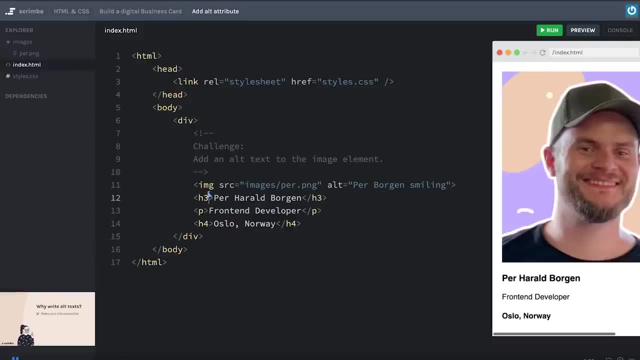 So why do we all write these alt texts? Well, first of all, it makes your site accessible, Because imagine that a person who is visually impaired or who is blind is trying to visit your website. In that case, they would use a screen reader which goes through the HTML. 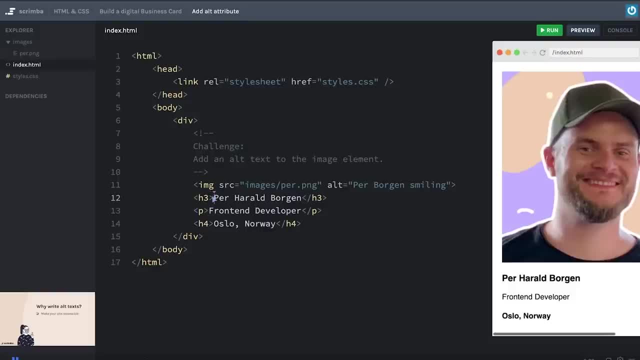 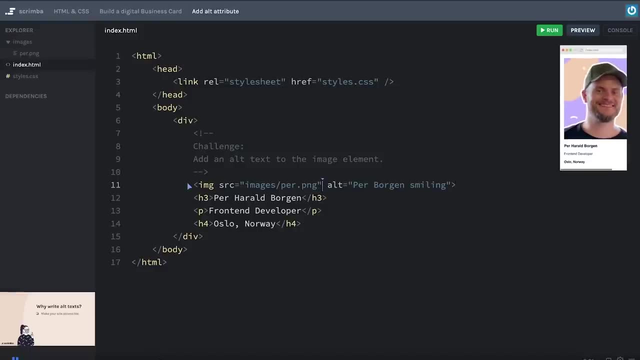 and reads it out loud to the user. And as for the h3 tag, it would be simple for the screen reader to read out loud what that says, because that is text. However, for an image like this one, you need to add an old tag to describe the image so that the screen reader 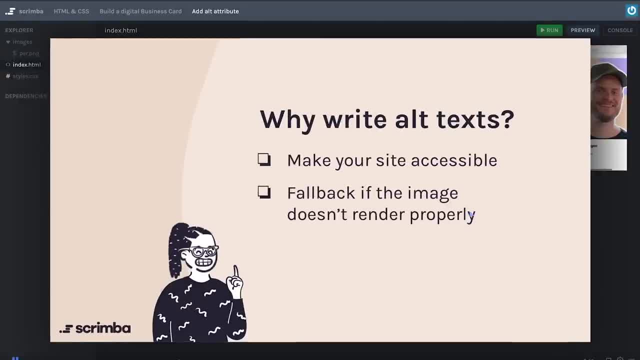 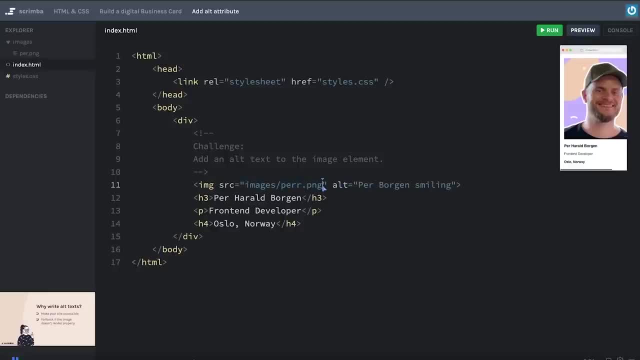 has something to read out loud. And secondly, this also works as a fallback if your image doesn't render properly Because, let's say, you have a spelling mistake in the source attribute, for example an extra R. Well, in that case. 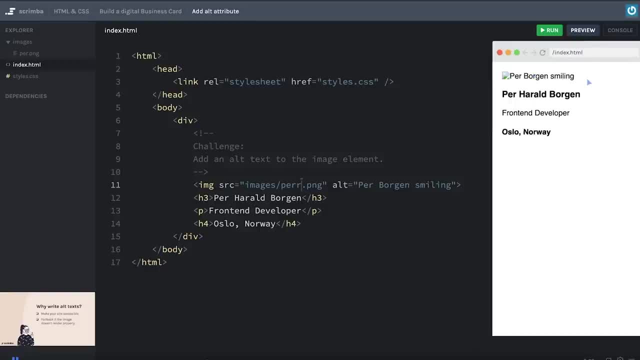 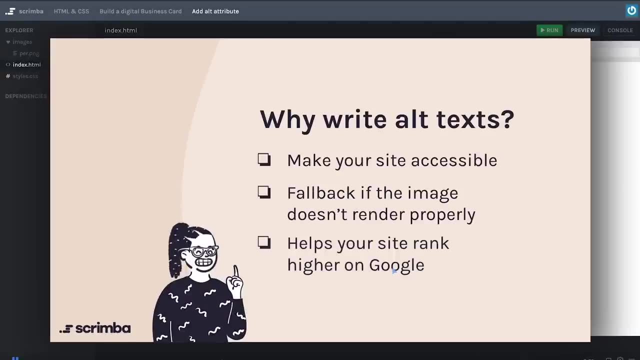 the image won't render, but the old tag provides as a backup so that the user seeing this can kind of understand what was at least supposed to be there. And finally, writing old texts will help your site rank higher on Google, meaning you get more search traffic And that. 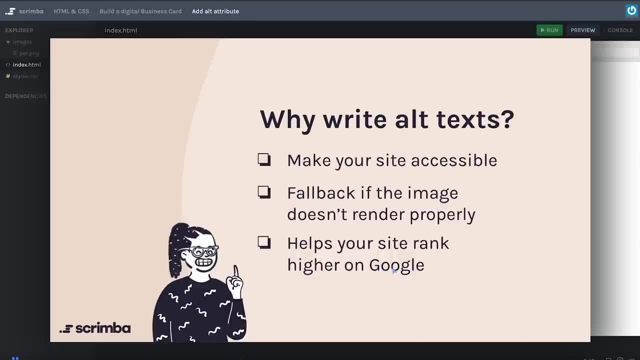 is because the old tag most likely provide important metadata about the image so that Google knows how to use it in a search results page, And if your site is not accessible, it might be punished in the form of ranking lower. So, with that in mind, let's start by. 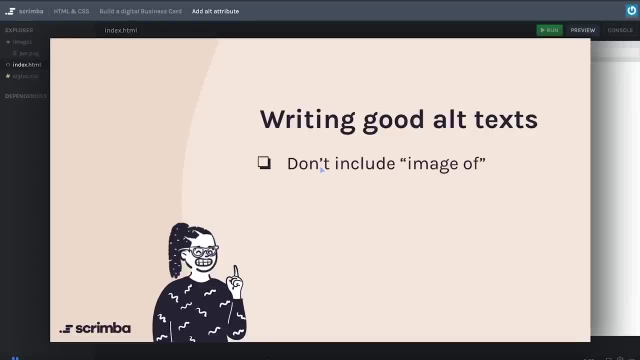 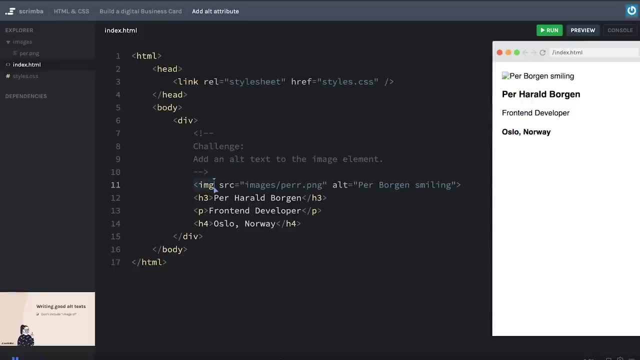 seeing some of the features of that. Let's start by looking at how to write these old texts, And the first thing you need to know is that you should not include, for example, image of, because that's simply not necessary. This screen reader knows that it is an image because it is an image tag. Secondly, should 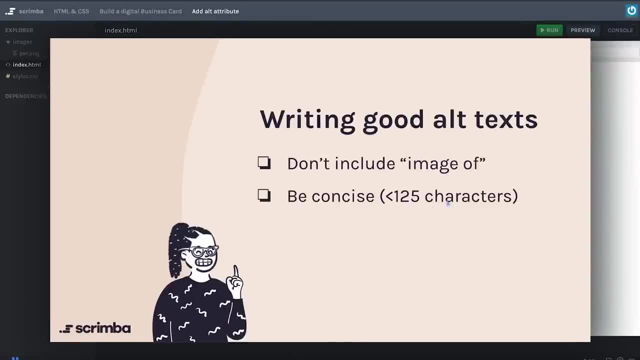 be concise, meaning less than 125 characters, because a lot of screen readers will cut off after this limit has been reached. And finally, a trick you should use in order to come up with a good old text is: imagine that you are describing this image to a person, or you are. 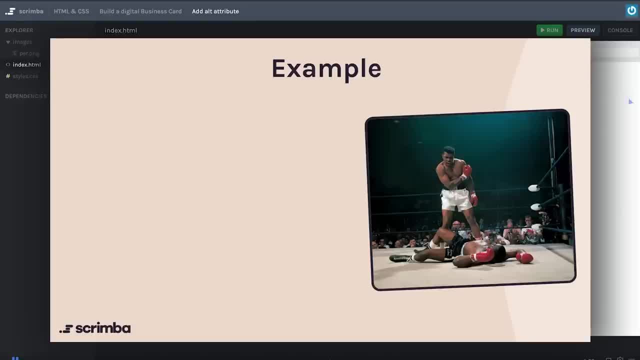 over the phone, So let's try to do that with an example. Here we have an iconic image of Muhammad Ali in a boxing match, And one way to write an old text for this could be just a boxing match, but it would actually be a pretty poor way of describing it, because there's 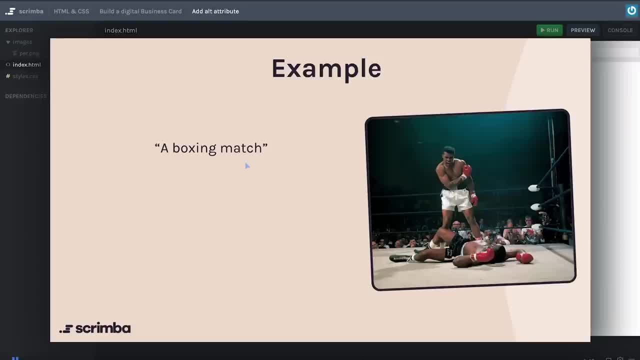 so much more going on here. you have plenty more characters you can use in order to describe it, So a better one would be two boxers in the ring, one line down and the other standing up. That's a good factual explanation, But we're not quite there yet because it isn't. 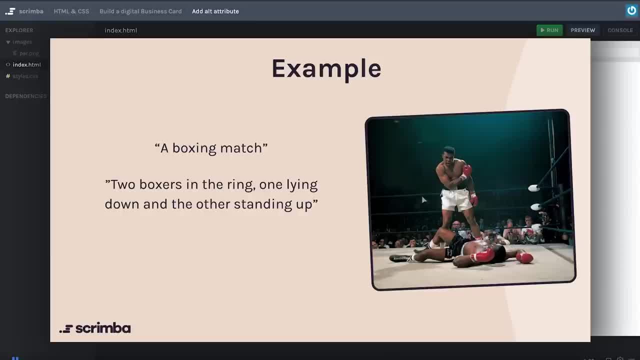 actually describing this iconic moment when Muhammad Ali knocked out Sonny Liston. So if you were to describe this over the phone, you would probably understand that this description is pretty shallow. So what I would rather write as an old text for this image would: 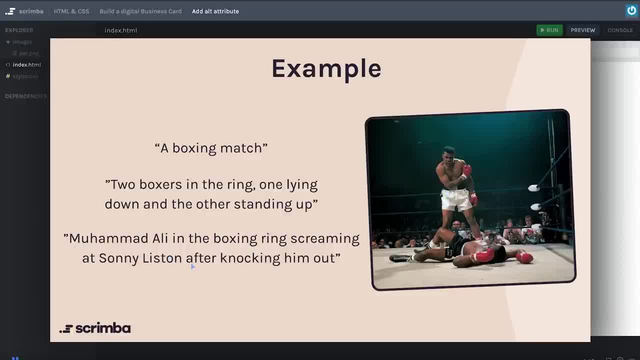 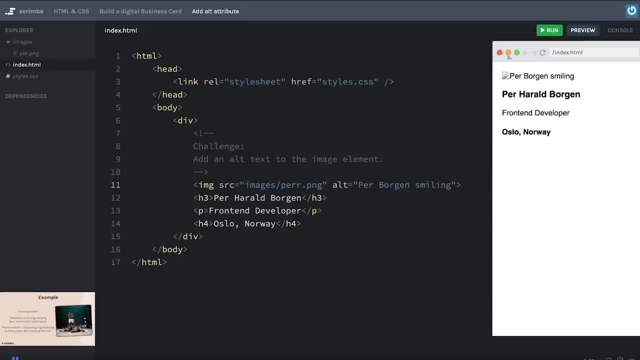 be Muhammad Ali in the boxing ring screaming at Sonny Liston after knocking him out. That, in my opinion, properly describes the intent of this image, what the person who has decided to show this image on a website is trying to convey. So, with that example in mind, I want you to write what do you think is an appropriate? 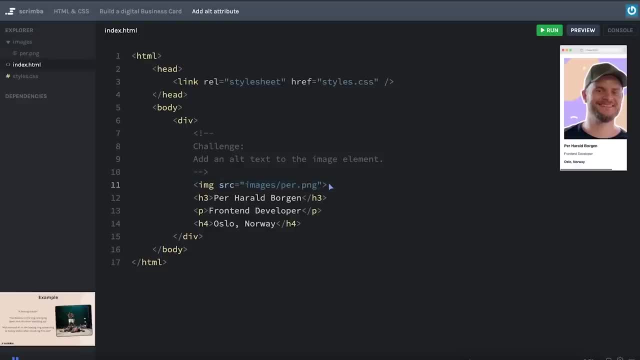 old text for this image. go ahead and do that right now, And then I will show you what I would write when you return back to me. Okay, let's do this. We'll do alt equals quotes. And here I would use my name, here, Harold Borgen, And you can see I'm smiling and I'm 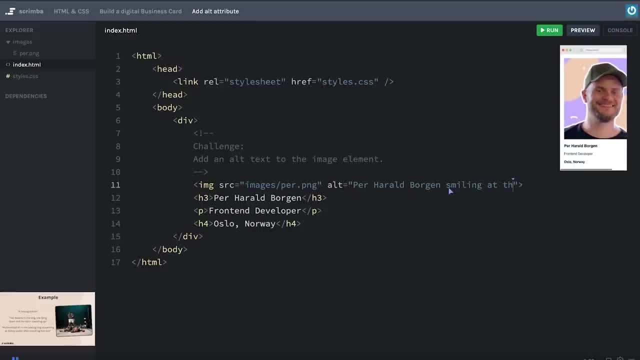 looking at the camera. I think that's important, So I'd write smiling at the camera. Finally, the background is really playful and colorful, So I want to include, for example, with a color full background like that. So if yours was a bit simpler or shorter, don't worry. 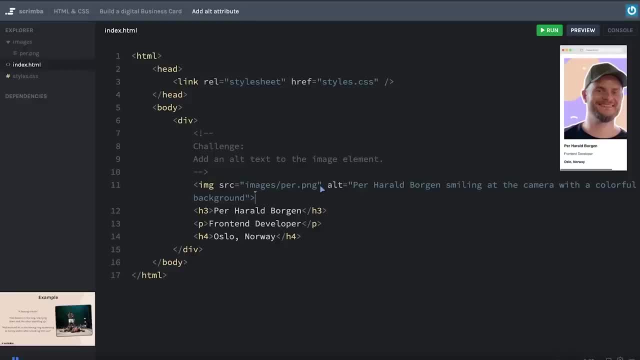 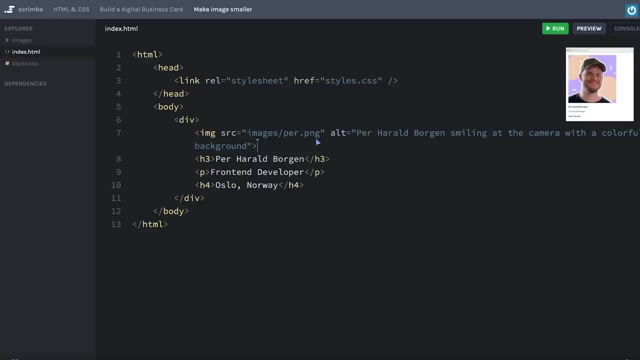 about it. The most important thing is that you add an alt text and do as best as you can- And actually plenty of developers never add this. So just by adding it, you are actually separating yourself from the image, From most other beginners. So with that, let's just move on. The next thing we're going to 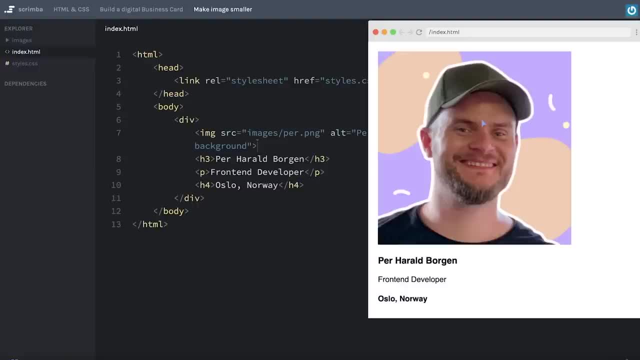 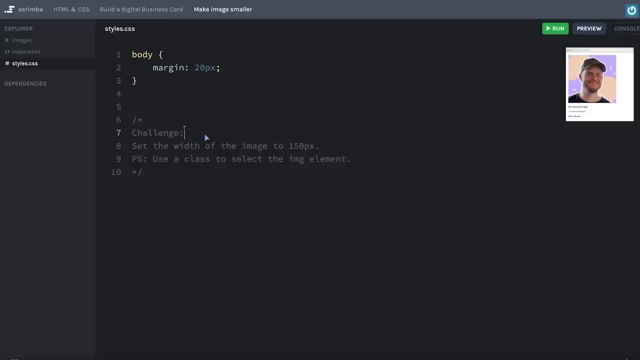 do is shrink this image to a suitable size for our business card, because as it is now, it is far too big. So I want you to head over to the styles dot CSS, and solve this challenge. you are to set the width of the image to 150 pixels And you need to use a class to select. 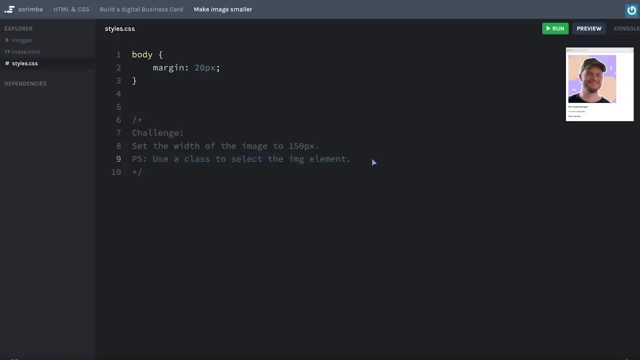 the image element. So go ahead and give this a shot right now. Okay, hopefully that went well. Let's now do it together. So first we need to actually create the class that we are going to select from the CSS. So let's head over to the HTML. 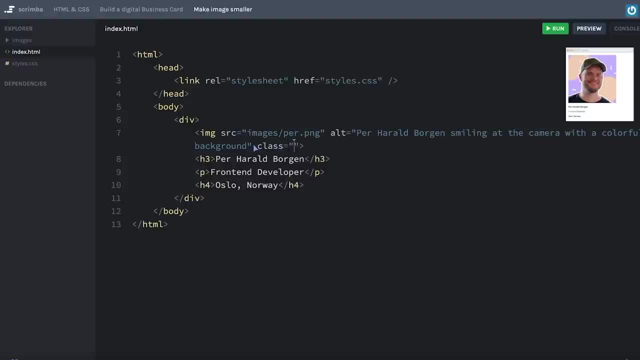 file. Here we'll just do class equals And I'm going to call this one an avatar like that. Actually, now that we have three of these on the image element, I think for readability purposes it works well To break the. 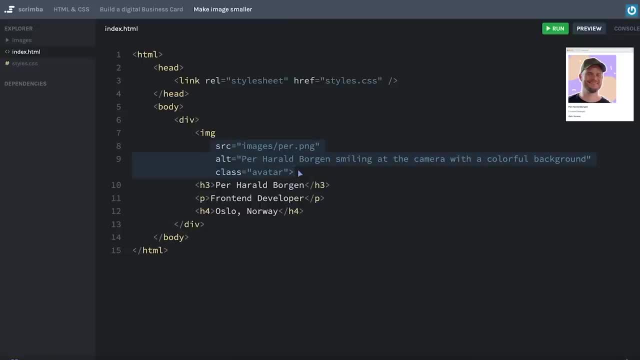 into three lines. I think this is a little bit easier to read. then I'll head over to the styles, dot CSS and target the class of avatar And reset the width to 150 pixels. Now rerun the code. There we go. So great job solving this challenge. Let's move on. 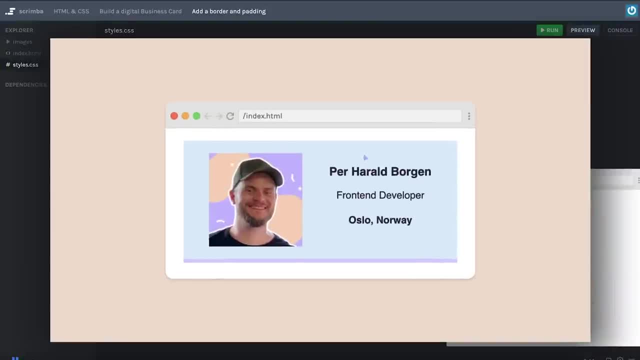 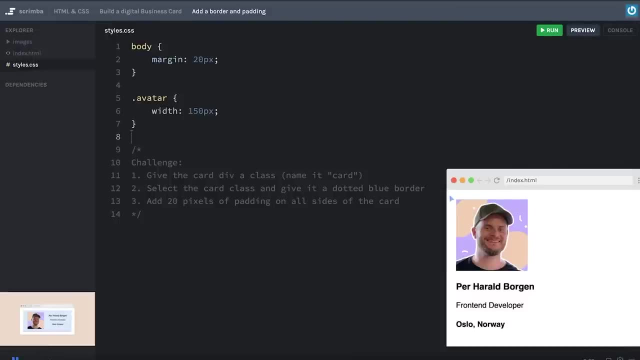 Okay, now you're soon going to start building the layout of this card. However, right now, the card kind of blends into the background. there's no separation between the card and the background, So I want to add a little helper style in order for us to more clearly separate the card from. 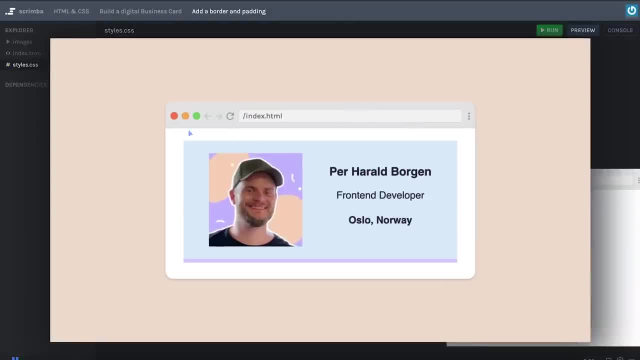 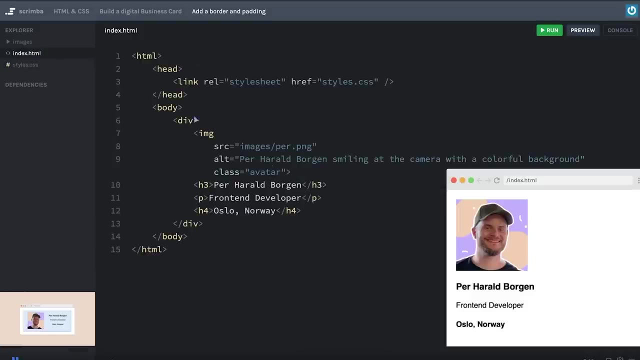 the background, And for that we need to grab hold of the outer element of the card. And can you take a guess what kind of HTML element you think should wrap the entire card? if you guessed a delle, that is correct And heading over to the HTML, you can see we are. 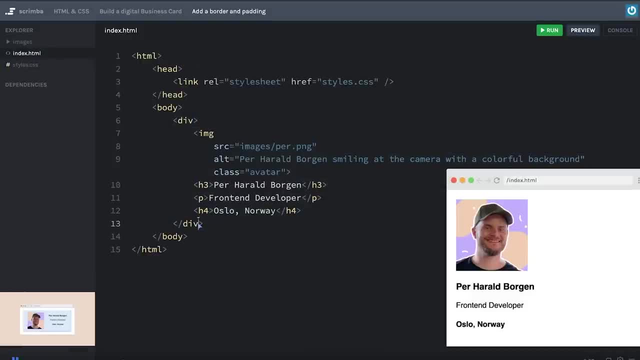 actually already wrapped up. Thank you, mapping the entire thing in a div. So here we have our container div, or card div, or whatever we want to call it. So what I want you to do now is to first give that div a class. 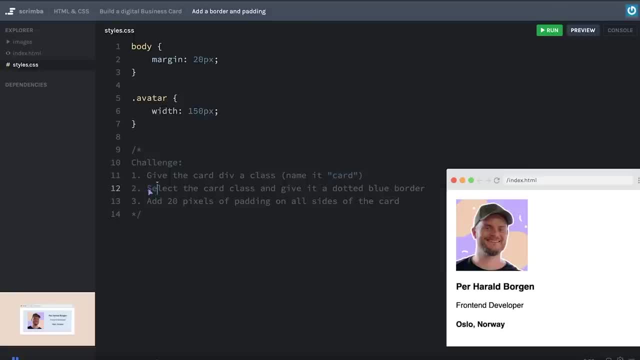 And actually I think you should call it card, And then I want you to select the card class in CSS and give it a dotted blue border. This is our helper styles. it will give us a little blue border around the element so that we can see how our card div kind of behaves. 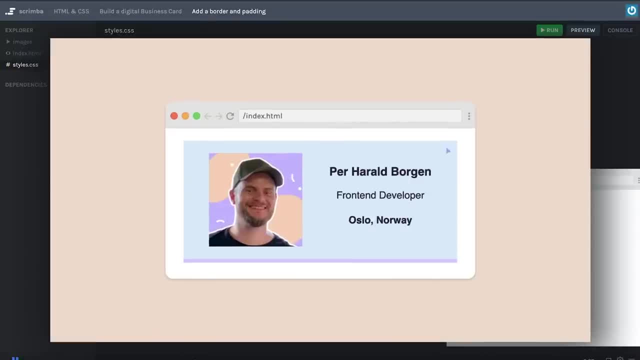 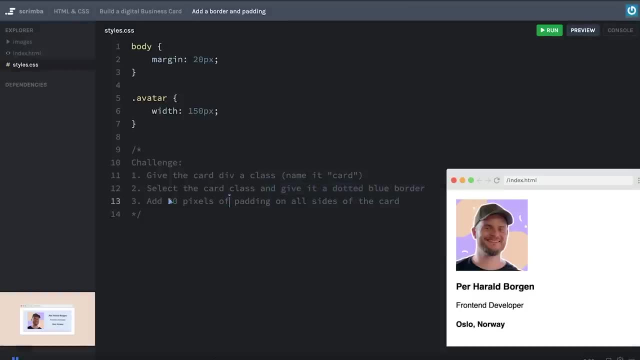 And also, as you can see from the design here, none of the elements touch the edge of the border, So it seems like there's some padding in play here. Let's just add 20 pixels of padding on all sides of the card as well, So go ahead, solve these three challenges. 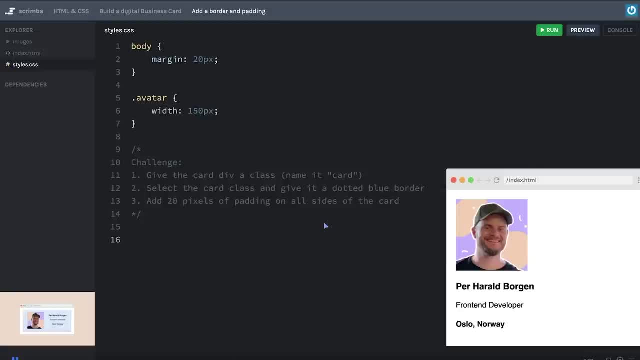 And then I'll, of course, show you the solution as well. Okay, let's do this. So first we need to give the card div a class. I'll head over here and do class equals card. I'll run this code so that we have this class in. 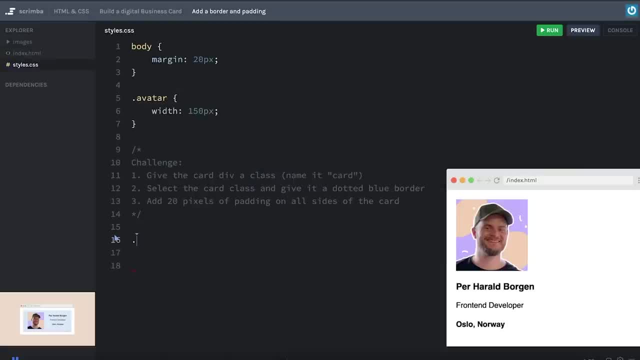 the DOM. The next step is to select the class by doing card And then adding a border. you remember from previously. that is done through the border property, which takes three values, the first one being the thickness of the border. I'm just going to set it to one pixel, the. 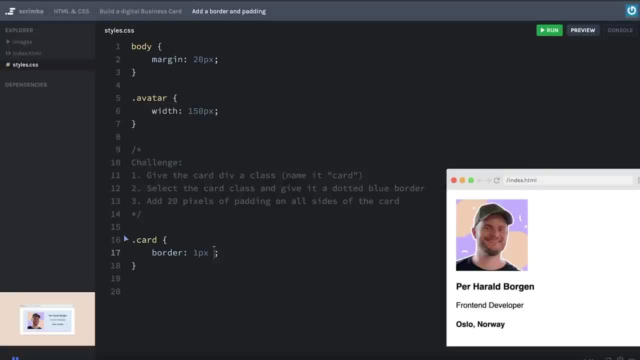 second being the quality, for example, solid or dotted or dashed or a few others, And we're going to use the dotted one And the color will be blue. And there you can see, boom, we have a border around our entire card, And this will make it a lot easier for us. 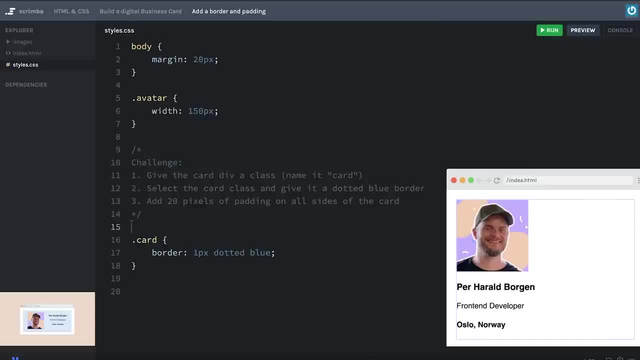 to work with the card now that we can see it clearly on the page. Finally, we want to add 20 pixels of padding because, as you can see here, the elements touch the border on the sides and we don't want that. we want some space. So we'll do padding 20 pixels, like. 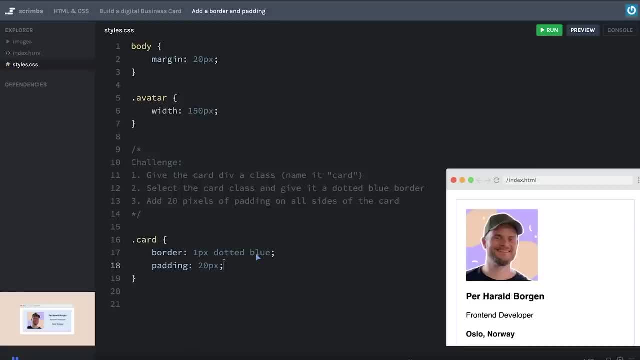 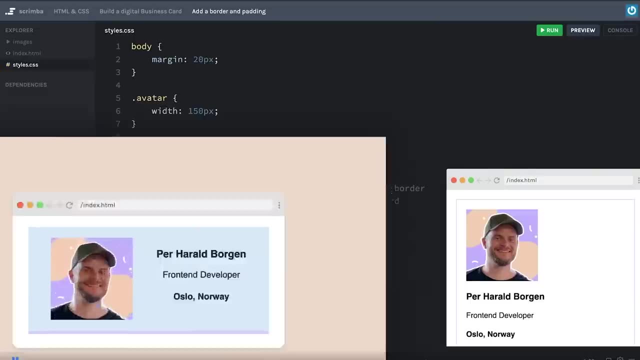 that, And there we go. We have solved the challenge. With this in place, I think we're ready to start moving on with fixing the layout And, as you can see, on the finished design here there's a big difference between this one and our current one, And that is that the current 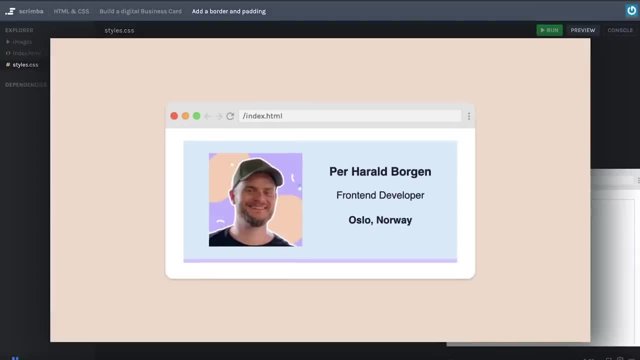 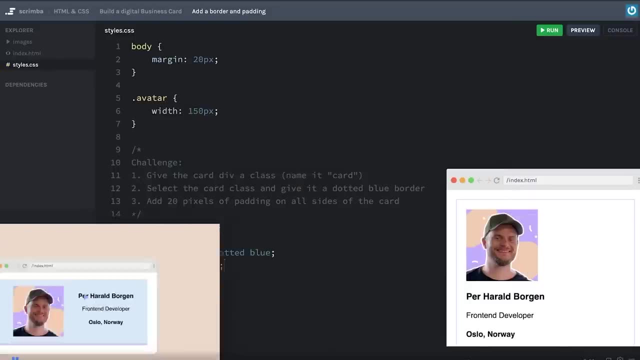 one is vertical, whereas this one is more horizontal, So they stack up differently. We want the image on the left hand side and the text on the right hand side, not everything on top of each other. So basically we want two columns: one for the image and one for. 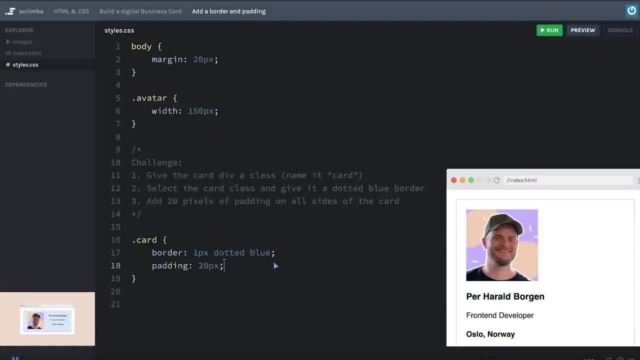 the text And, as you might remember from previously, flex box helps us create columns. So let's now just experiment by adding display flex to the card And let's see what happens. Oh, wow, Okay. so what happened there? it actually turned every single element into. 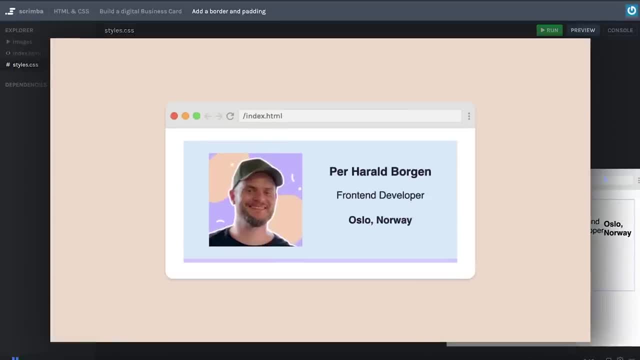 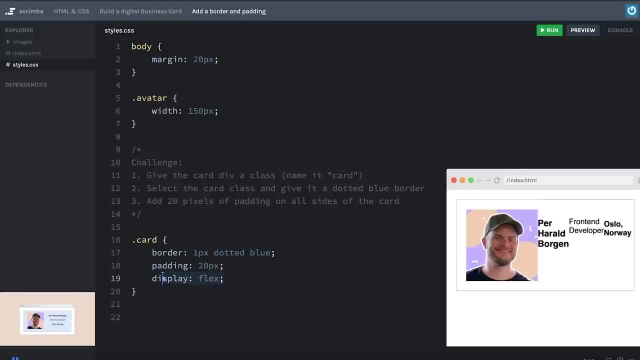 a column in itself. That's not exactly what we want here. So display flex isn't the entire solution. So what we're going to do now is to go out on a tangent, learn a little bit more about the text, And then we're going to go ahead and create a new element And 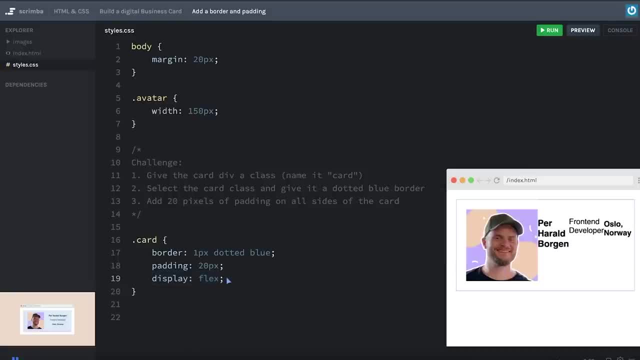 let's do that in the same way for the other two, And we want to make sure that we have this flex box concept in CSS and then return back to this business card project once we're ready to build a layout like this. So let's move on and learn more about flex box. 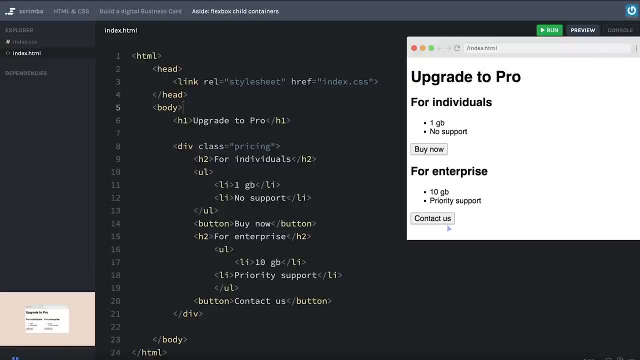 Okay, so let's say that you've built some kind of software as a service and now you want to sell it. then you might have a page like this, where people can upgrade to pro and they can choose the individual plan which gives them one gigabyte and no support, or 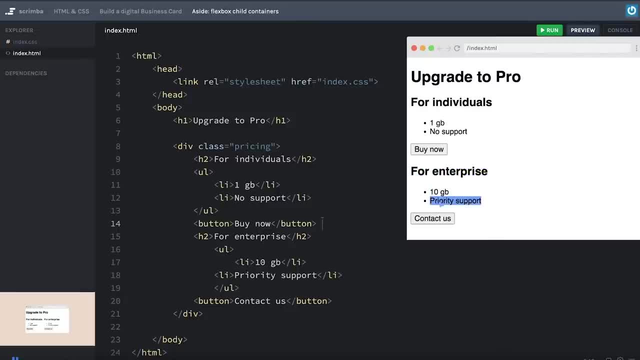 the enterprise plan. Okay, so first let's say we want to go over here and when we go back to the interface which gives them 10 gigabytes and priority support. Now, I've purposely not given any design to this example, as I wanted to make it as easy as possible to grasp, But hopefully 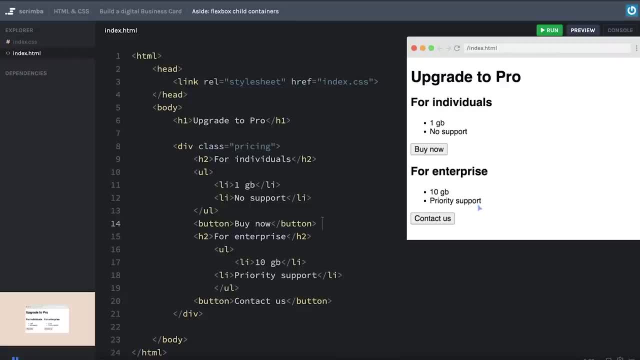 if you are to create a pricing page, you'd make it look a lot better than what we have here. So you can see the HTML right here for the entire pricing layout. I've wrapped it in a div And I'm using an h2 unordered list button and so on. Now let's say that you instead, 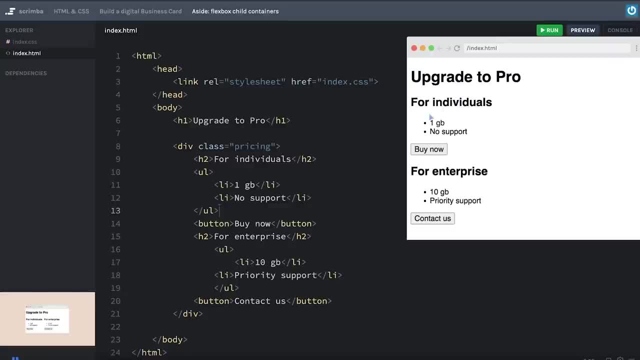 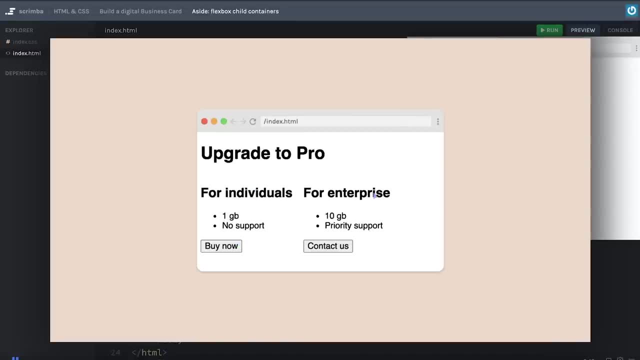 of having this one column layout here where everything stacks on top of each other. you want this two column layout where you have the individual plan at the left hand side and the enterprise plan at the right hand side. Well, if so, we know that flexbox will. 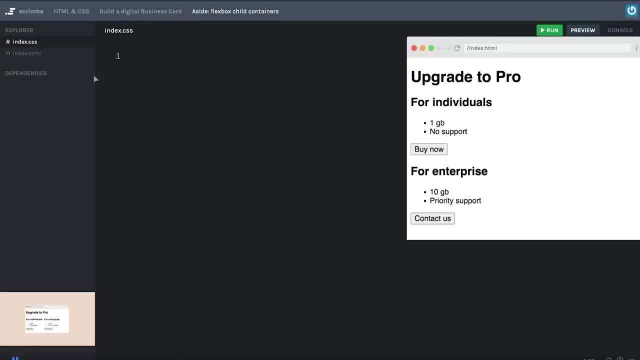 help us create columns, But if we try turning our container is the div with a class of pricing into a flexbox, you'll see that it'll break the layout, just as we saw in our business card example, Because what's going on here is that flexbox takes every single item. that is every single. 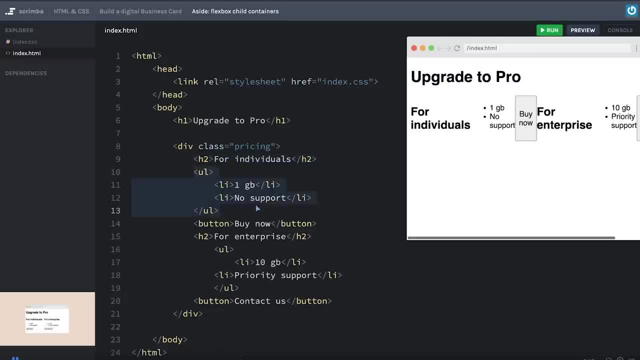 direct child and turns it into a column in itself. So we get a column for the h2, for the unordered list, for the buy button, for the h2 again, and so on, And this is obviously not what we want. It's far from this two column layout right here. However, there's one hint. 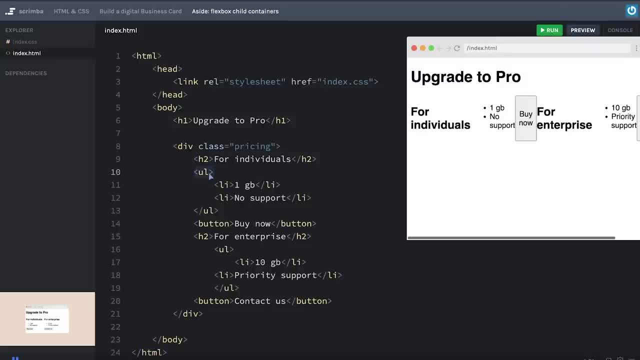 to be drawn from this example, And that is that you check out the unordered list here, see that it has two children of itself, Li elements, And those two are not their own columns. They are in the same column, stacking on top of each other. So it 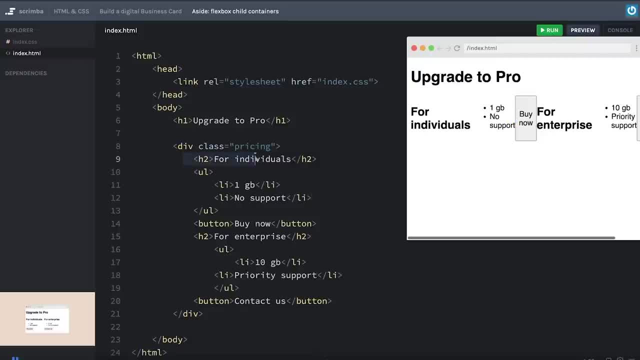 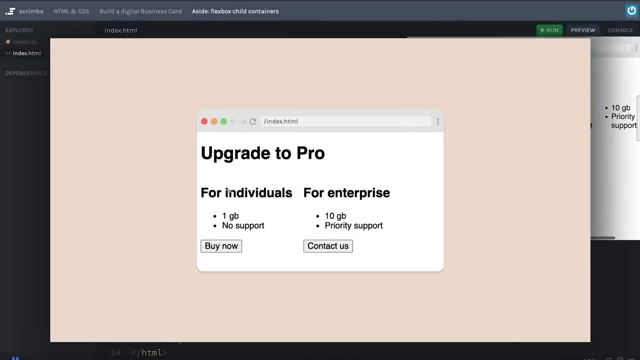 seems as if flexbox only turns the direct children into their own columns. So the direct children are the h2 here the ul the button, but not the list items, And once we know that, we can use that knowledge in order to get to this layout. 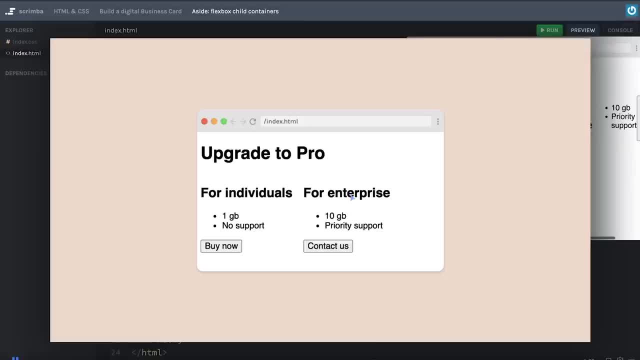 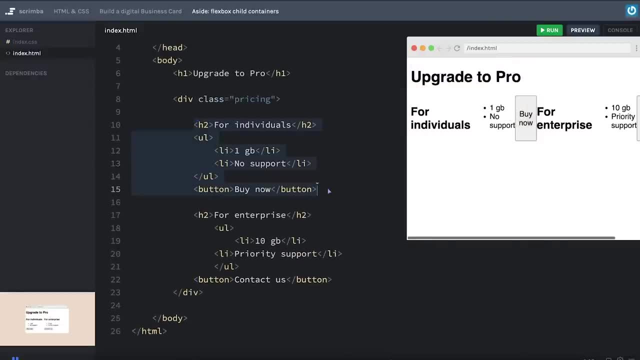 This layout has two columns. that means that our flexbox container should have two direct children, not six as it has now. And how can we achieve that? Well, we want this group to be inside of a direct child of this container And we want this group of HTML elements to 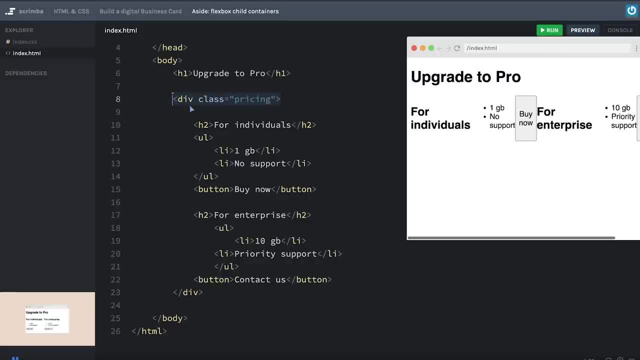 also be inside of another direct child of the flexbox container. So what we'll simply do is we'll wrap both of these inside of a div like that And we'll indent it for readability purposes. Let's try to run this code having wrapped one of the two. 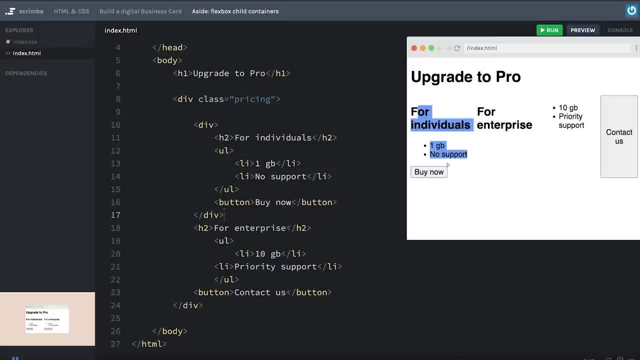 groups into its own dev, And there you can see, the four individuals plan now stacks up just how we want it, But the rest of the layout is still broken. So we need to do the same thing down here Like that, run the code And there we go Now- our flexbox container. 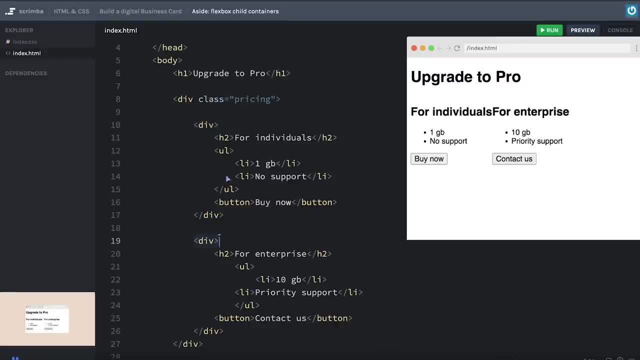 actually only contains two items- this div and this div- And it doesn't care about what's inside of both of those children. it only cares about its direct children, And the result is that we get the layout we wanted here, at least in terms of having two columns. There's still a problem with lacking space in between these. 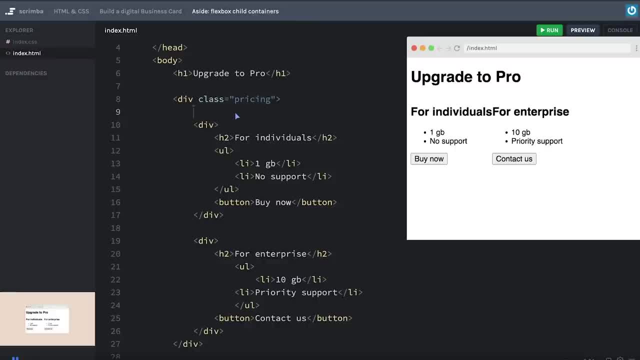 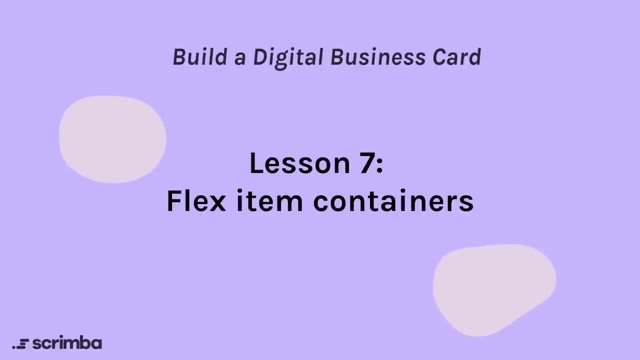 two children, But we're not going to deal about that right now. For now, I'm going to send you back to the business card example so that you can use this to improve our layout. Okay, we are back at our business card example. Now. the thing we need to do here is to find: 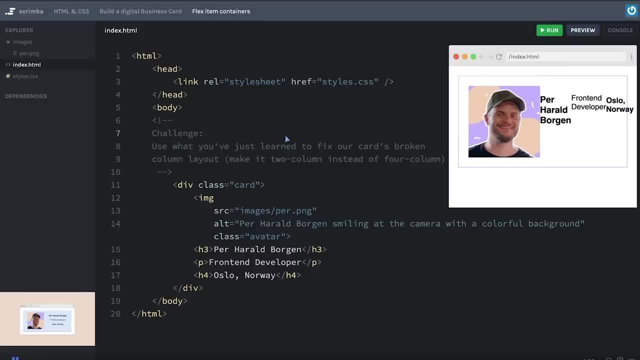 Okay, we are back at our business card example, And now I want you to use what you've just learned in order to fix our cards: broken column layout, because you are going to make this card into a two column instead of a four column, which it is now as the image name, title and. 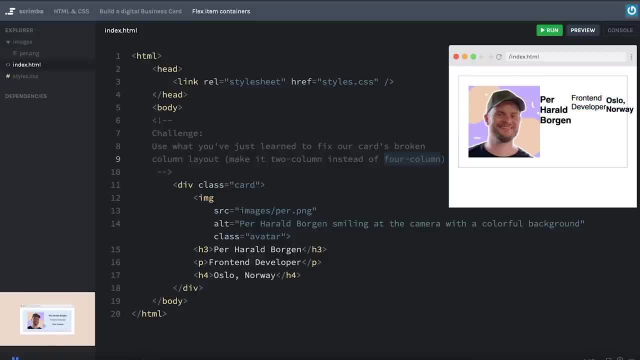 location at four different columns, But instead we want two columns, one for the image and another one for the text elements. So this challenge is solved in the HTML. as you know, we already have a display flex on the card, And the only thing you need to do is one change. 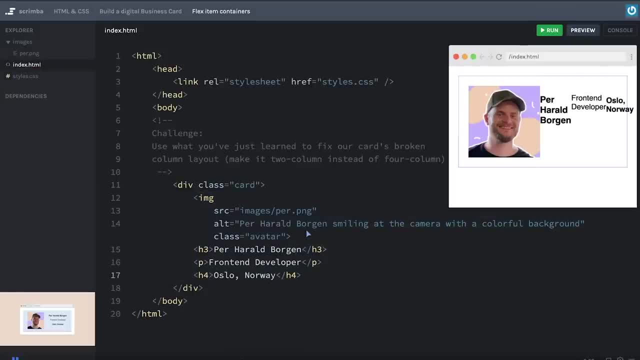 inside of our flex box. So hopefully you're able to do that. go give it a shot And then I will show you the solution as well. Okay, hopefully that went well. let's do it together. So the problem is that flex box. 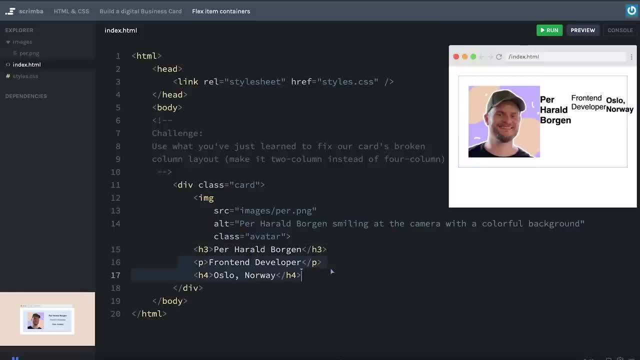 treats each of these elements as a single child and thus each of them get its own column. However, we only want two columns, So we want these three to be governed by one flex child, So we need to wrap them inside of a div 12.. We'll do like this: open the div and then close. 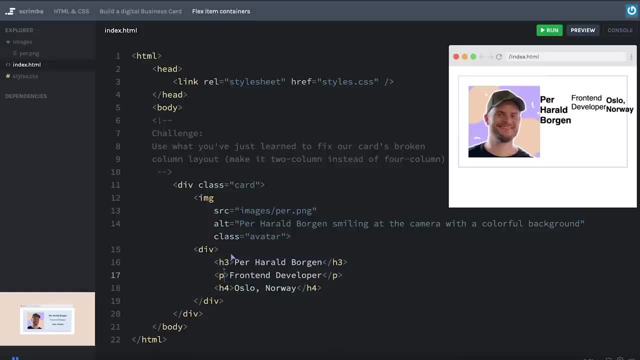 the div down here And we'll indent these so that we get some better readability. Now you can see, the flex box only has two direct children: this one and this one. That means that we should get two columns in our layout, And yes, we do. Brilliant, Of course there's. 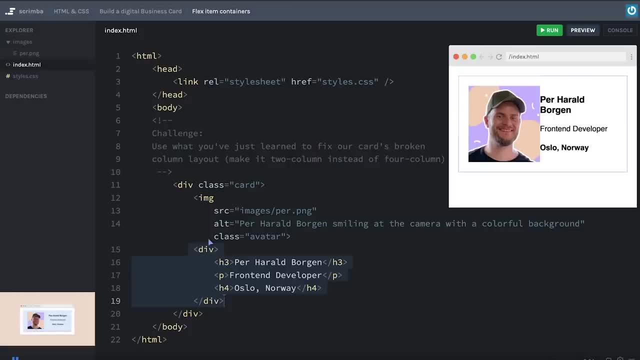 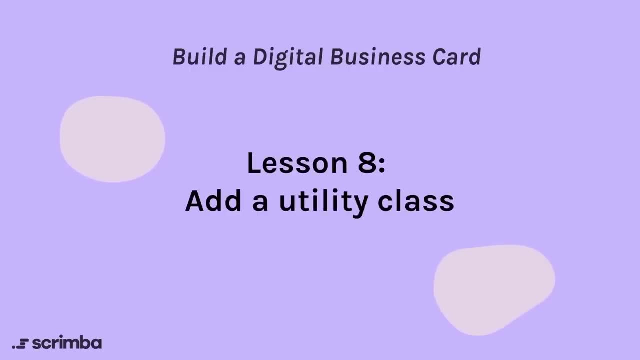 a long way from this design to this design, But we are making great progress here, So let's just keep up the pace and move on to the next scrim. Okay, I think. looking at this example now, I gotta admit that I'm pretty pleased with. 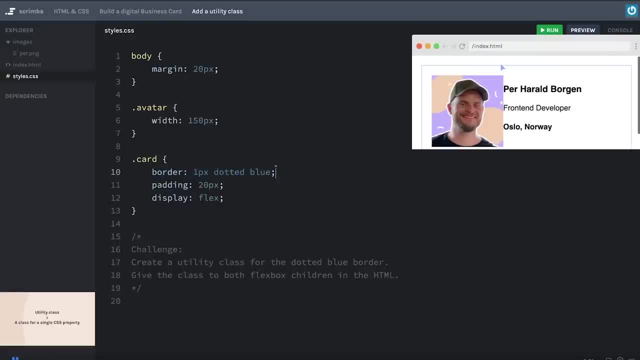 this border, one pixel dotted blue here. I think it serves a very nice purpose, which is to highlight for us how our card is being laid out on the page. So wouldn't it be nice if we could use that exact technique on other elements on the page as well, For example: 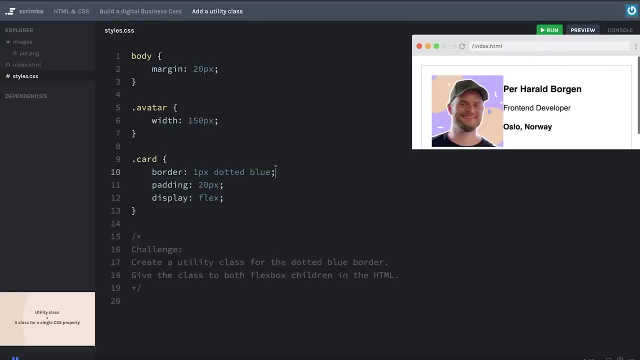 we can see that we have this border one pixel dotted blue here, And then we can see that we have this border one pixel dotted blue here, And then we can see that we have this border one pixel dotted blue here, And then we can also see here, for example, the children of 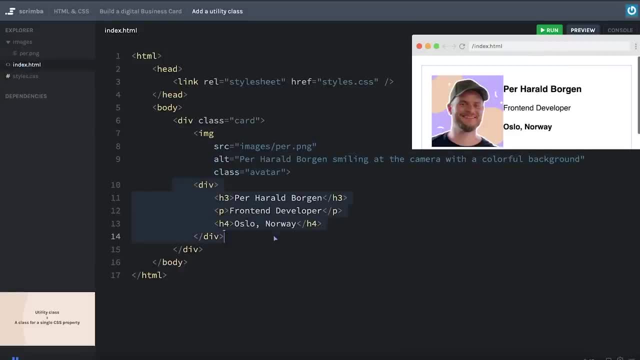 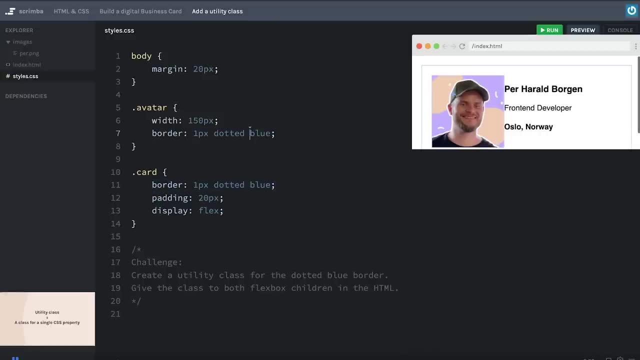 the flex box container, that is, this image right here and the div tag. that would have been really neat, And we can do that by, for example, just copying this one and adding it, for example, to the avatar either. The avatar is got that blue border as well, However. 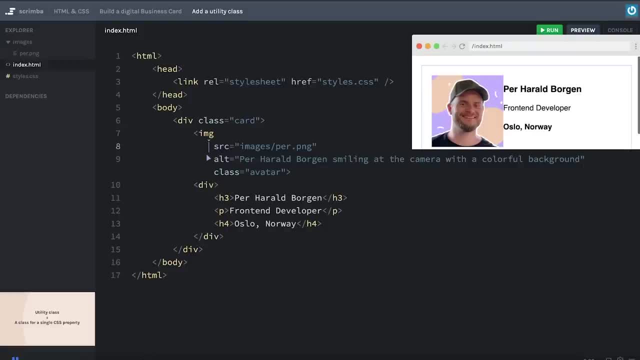 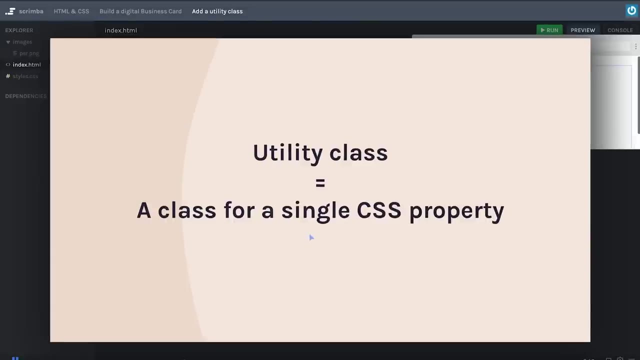 wouldn't it be neat if we in our HTML could just quickly apply a class to any element, for example this one, and it would get the same thing as well? So, basically, the argument I'm making is that we should create gated class for this blue border, And what that is is a utility class, aka a class that only. 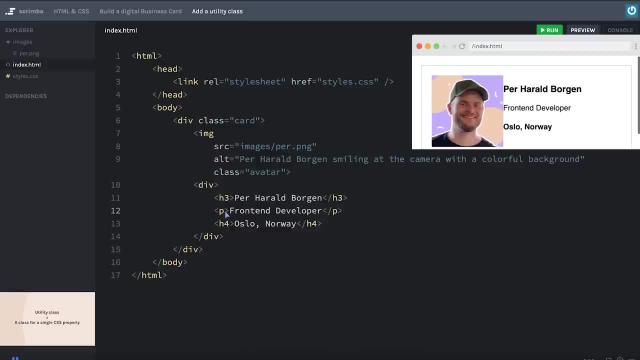 sets a single CSS property. So let me show you how this would work. Let's say that we, for example, want a class to make our text italic. then we'll simply do class equals italic. like that, If we run this code, nothing has happened because the class hasn't been. 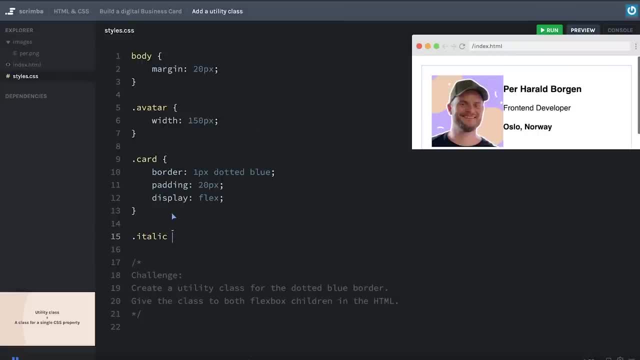 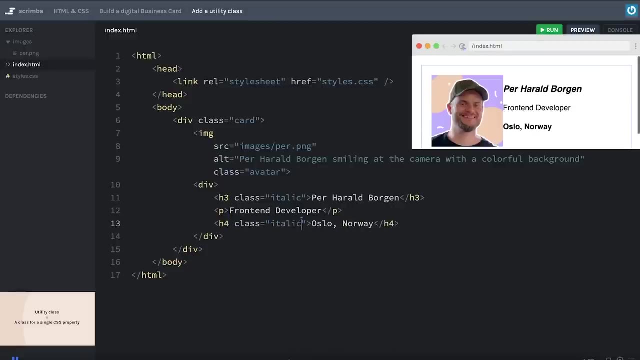 created yet. But here we can create the italic class and do font style italic, like that, And now you can see the name is in italic. Now if we want to reuse this, we can just do class italic here as well, And the code and the location is also italic. And if we 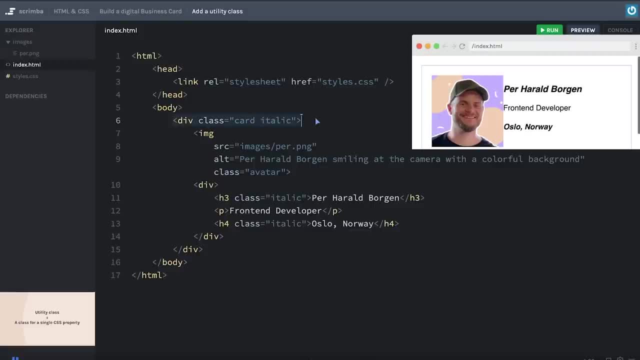 want the entire card italic. we can even add the class here up on the container element itself, run the code And now this has been inherited down To all of these elements And if you're a bit confused about what I'm doing here, it. 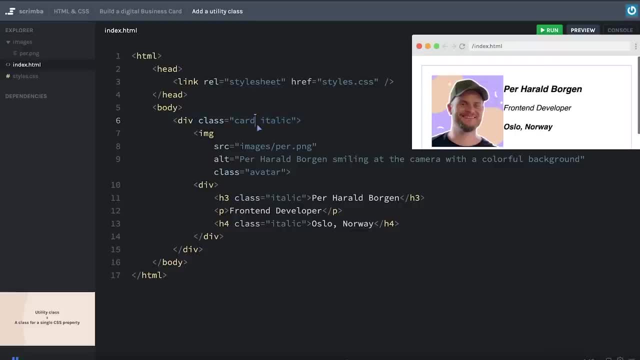 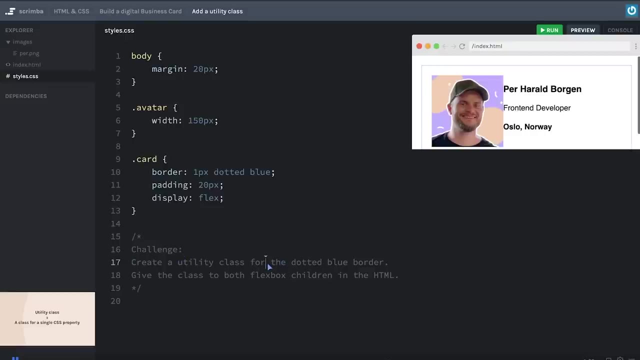 is simply adding two CSS classes to a single element. Do that simply by adding a space in between the two classes. Okay, let's get rid of these like that And delete this one as well. Now what I want you to do is create a utility class for the dotted blue border. 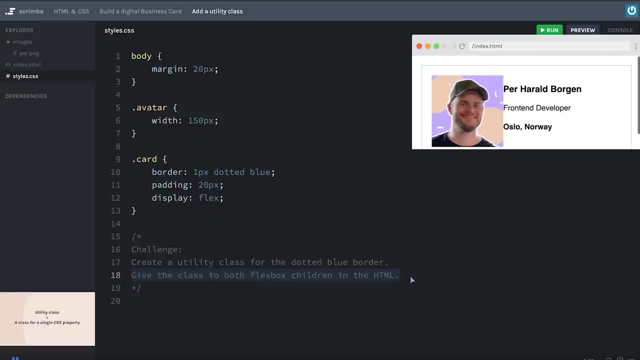 This is the styling we have here. And then give the class to both flexbox children in the HTML. That is the flexbox items you can see here and here. And also I think you should give the same class to the card as well, so that you can remove this line 10 here. So go ahead. 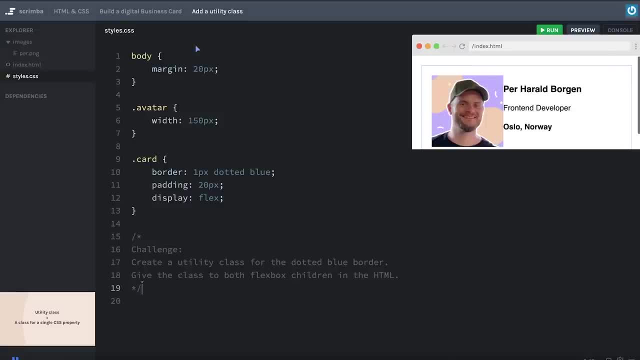 and give this one a shot, And then I will show you how to do it afterwards as well. Okay, hopefully that went well. Let's start out by creating the class All right, border, blue hair, And then inside of it, I'll just cut this away and paste it in here, So I'm 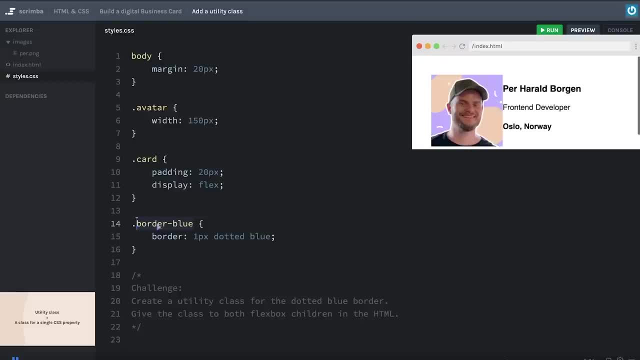 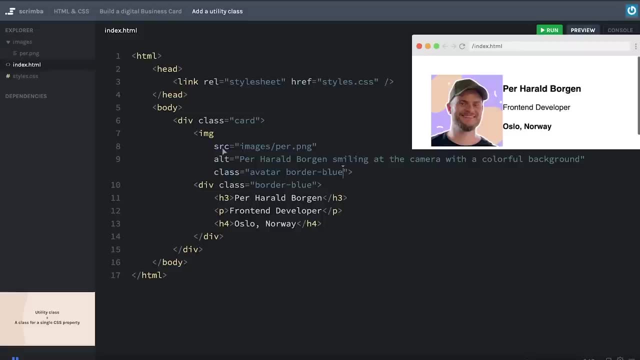 going to go ahead and paste it in here, And then I'm going to go ahead and paste it in here instead. Now we have a utility class for blue borders. I'll copy it and add it to this flex item And, as a second, as to the image element, we run this code. you can see. 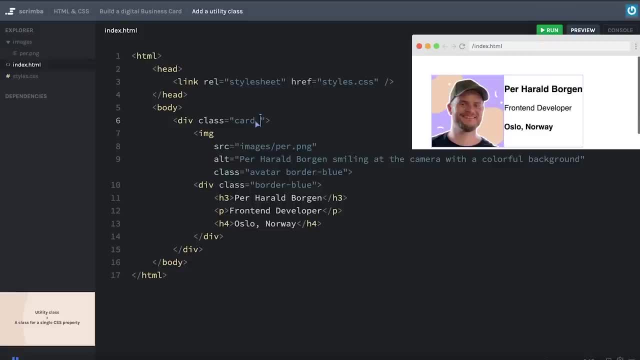 now both of these have the blue border around them. Let's also add the border blue class to the flexbox container. run the code and boom. there we go. Now we have an even better overview over how our elements are laid out, Okay. 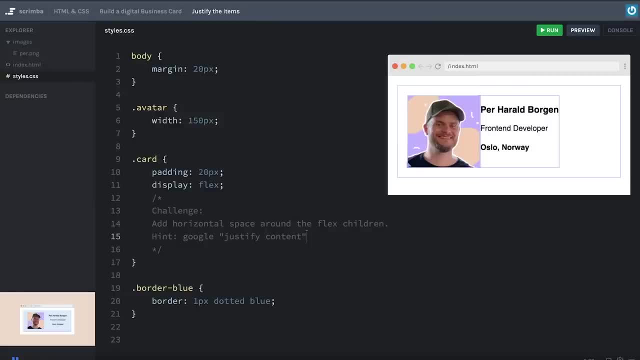 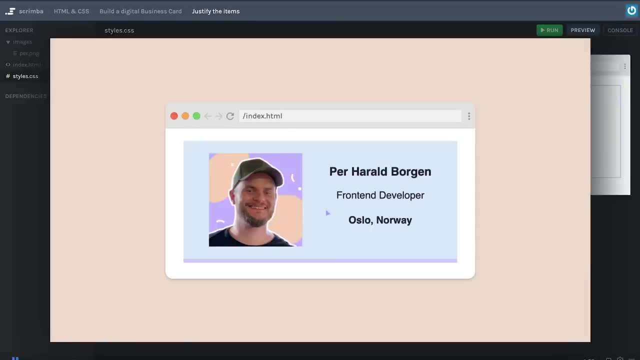 with these blue borders around the flexbox, children, it's pretty easy to see that our layout is pretty far from how we want it to be, Because here you can see in the card that there's some space in between the two elements, Whereas in our example they're completely. 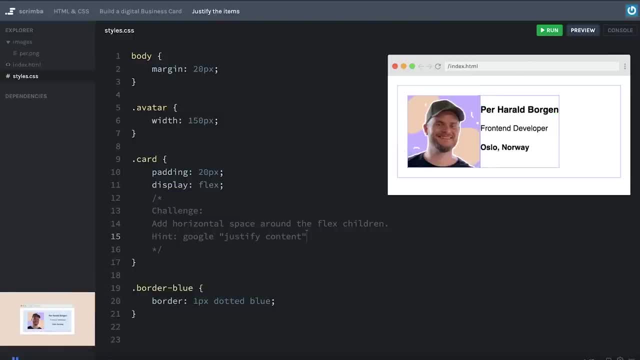 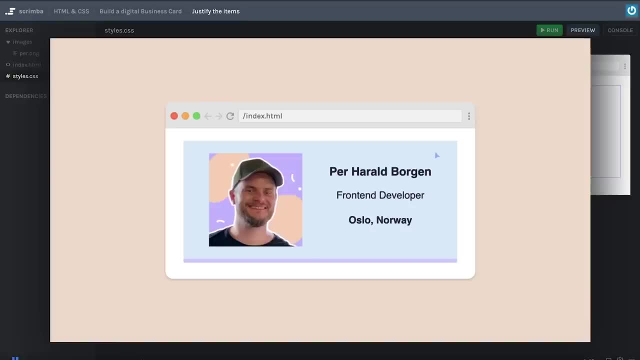 crammed together and also pushed all the way to the left hand side, Whereas here they're kind of spaced out. there's some space on the left hand side in between the element and also some space on the right hand side, So they're kind of spaced out in a nice way. 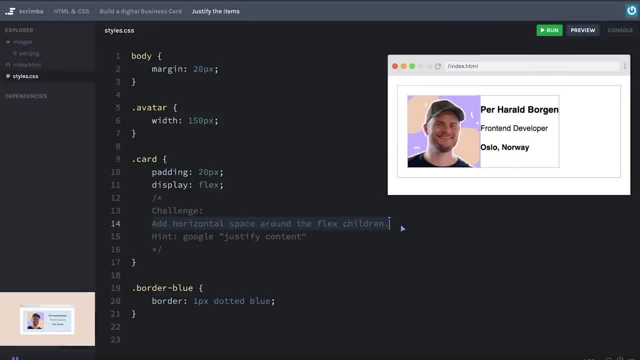 And now I want you to add to that horizontal space around the flex children. There's a flexbox property that does this, and you've seen that property before. However, you might have forgotten it. if so, then Google justify content and you might find the answer. I'm not going to. 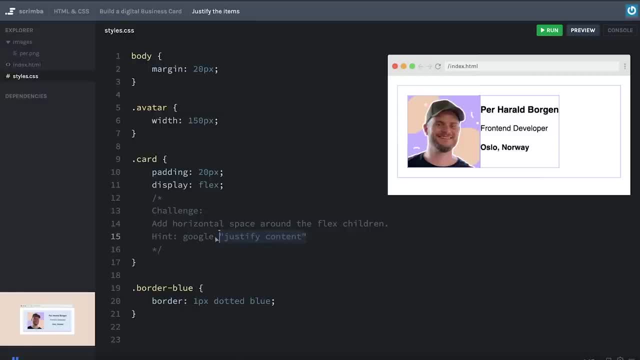 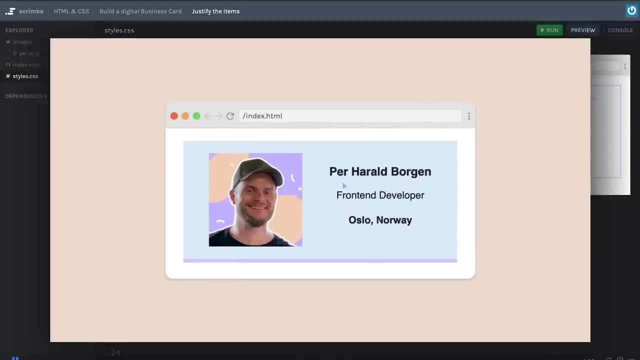 give you any more hints than that, Because if you have forgotten about it, it is a great practice to Google it. Then, once you've figured out the answer, go ahead and add the horizontal space so that our example becomes a little bit more like this layout. And just so you. 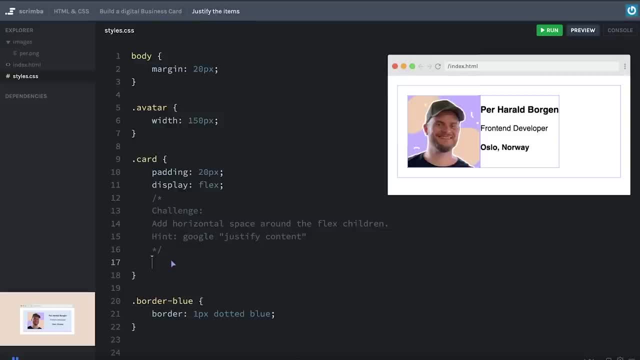 know you only need to add one, One property for this, not multiple. So give it your best shot And then I will show you the solution afterwards as well. Okay, let's do this. So the property is called justify content- a little bit of a weird name, I agree, but that's how it is And here we can use. 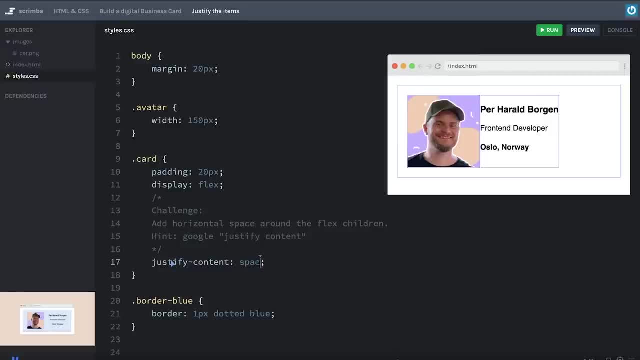 a range of different values, And the one we're looking for is called space around, like that. And now you can see, both elements Now have some space around them, And also we can do space between. then all of the available space will be between the two items, Or we could even do center, as you've seen before. 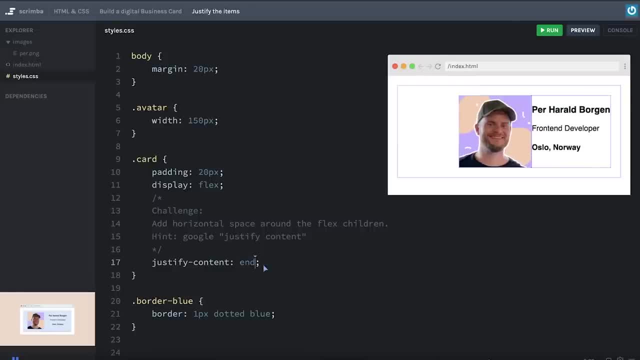 then there's no space in between them, but both of them are centered, And end pushes it all the way to the end And start keeps it at the start. So this is a super powerful property And we want the space around value for it. 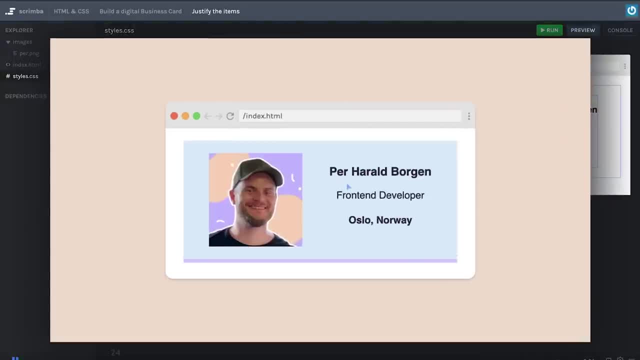 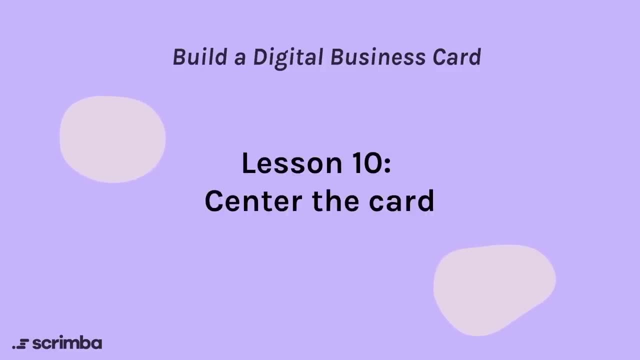 As you can see, it's a at least getting closer to the layout we have in our finished design. So great job, let's move on. Okay, time for a new challenge. you are going to set a fixed with on the card and then 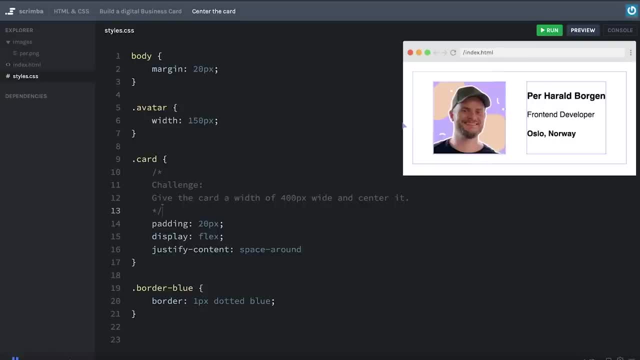 center it on the page because its behavior is a little bit weird right now. As you can see, if we enlarge in the screen, the card gets enlarged as well, And that makes the spacing between the elements look super weird. the aspect ratio becomes very different from. 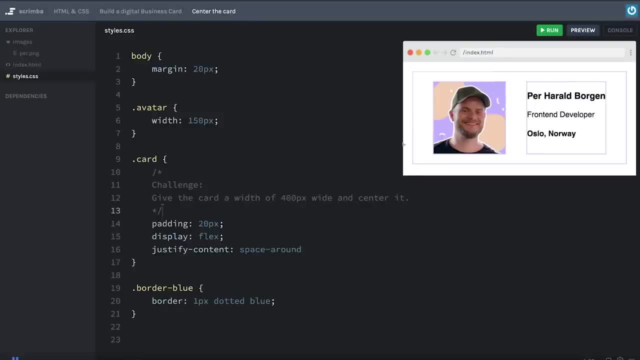 a business card, So we don't want that. instead, we want the width to be 400 pixels, So it should be a fixed with, And then we also want the card to be centered on the page. Now, one thing I want you to notice when I enlarge in this is that the card is a display block. 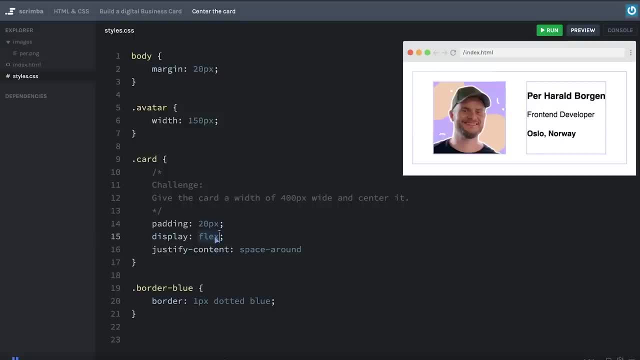 even though we've set it to display flex. So that means that Flexbox containers by default are display block And hopefully you remember from previously that display block takes up all the available space. Thanks for watching in the horizontal axis And there's also one of the three ingredients you need in order. 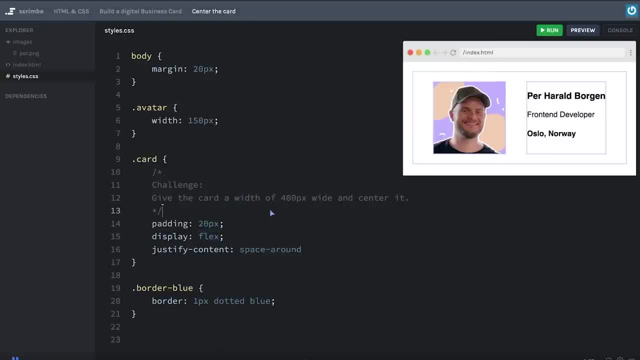 to center an element using margins. So hopefully you remember from the Google project how to center block elements. So go ahead and give this one your best shot, And then I will show you the solution as well when you return back to me. Okay, let's do this. I'll start by setting the width to 400 pixels, like that. Now you 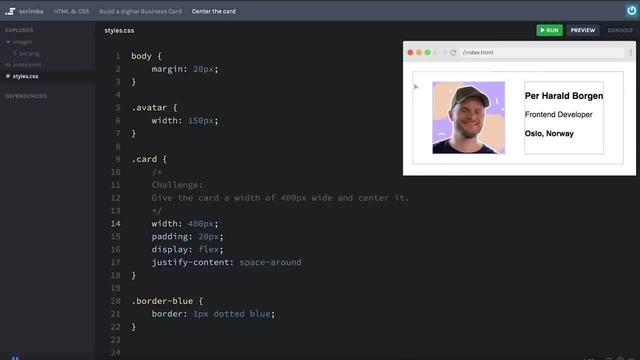 can see if we enlarge in the screen, the card is stuck to the left hand side of the website. So in order to fix that and instead center it, we'll use margins And hopefully you remember that we'll do margin left and set that to auto. that pushes it all the way to the right. 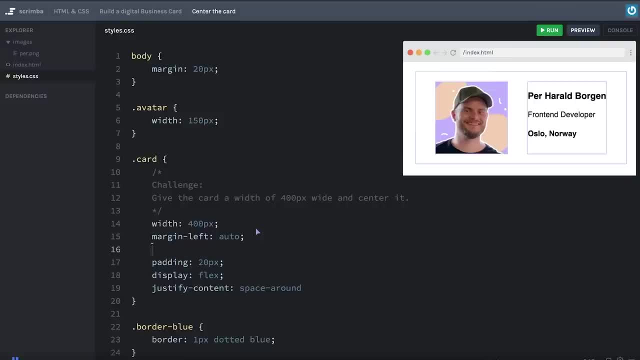 hand side, because all of the margin is now on the left hand side. But then, in order to even it out and center, it will do margin right as well and set that to auto. And the result of having an equal margin on the left hand side and the right hand side is that the card is centered. So great job. 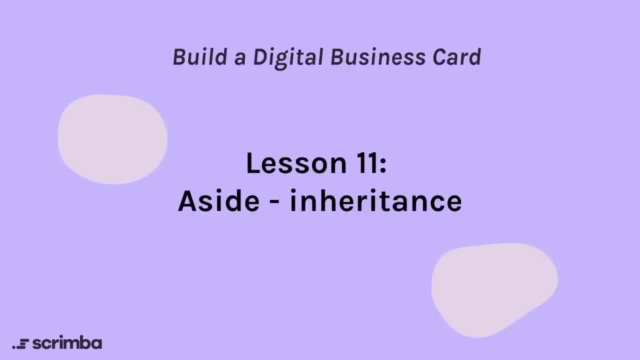 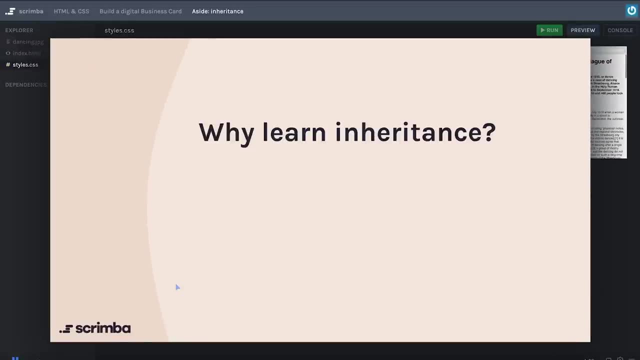 on solving this challenge. Let's move on. Okay, now let's talk a little bit about CSS inheritance. And why is that important? Well, CSS inheritance allows you to write so called dryer code, And dry hair stands for- don't repeat yourself- meaning that with CSS inheritance. 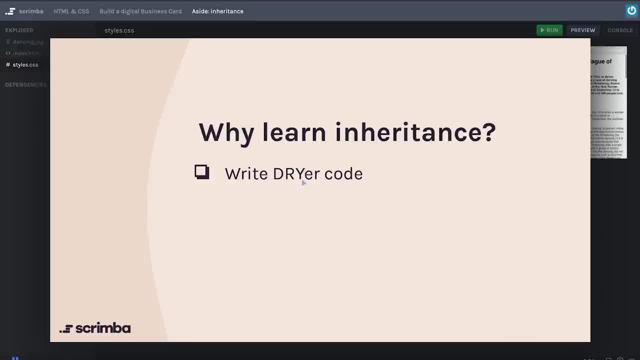 you can write less code though still receive the same result, And that's a good thing, Because less code means a smaller surface area for bugs, And that also means that you will be a more efficient developer. So let's have a look at how CSS 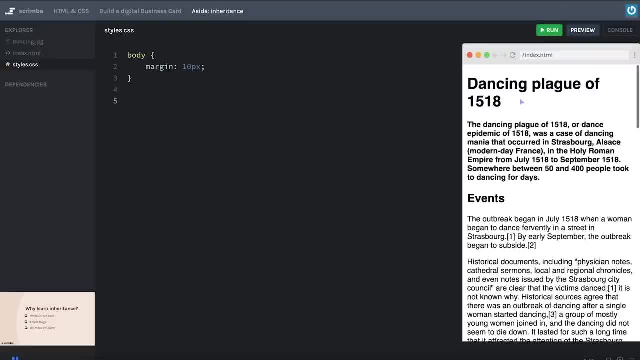 inheritance works in practice. Here I've pulled in a Wikipedia article in our mini browser, a really wacky article about a dancing plague that happened in 1518.. In modern day France were either dozens or hundreds of people took to the street and danced for days without 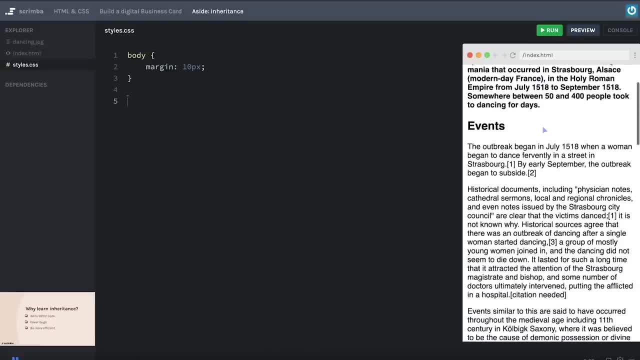 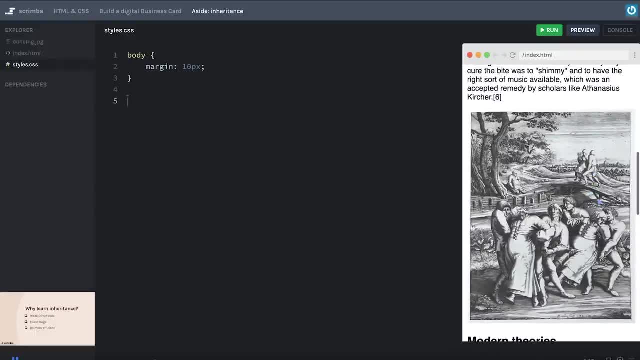 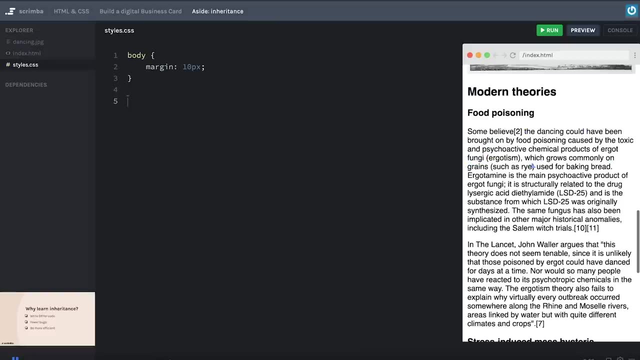 no one really knowing reason. So this is really weird, but properly documented from multiple sources And here is an illustration. I have no idea what caused this dance epidemic, But I think the modern theory about their grains being poisoned by fungus that gave them the same high as you. 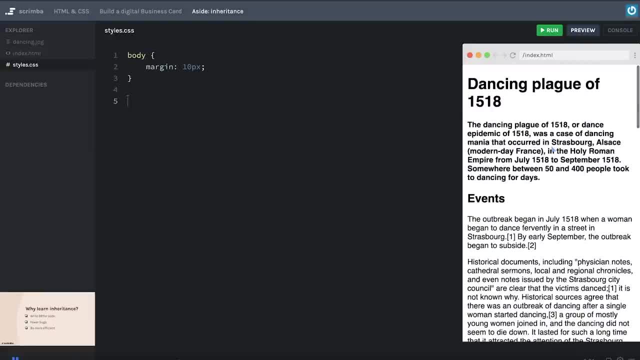 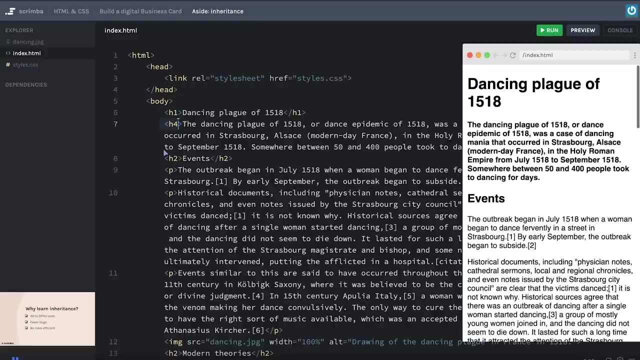 get from LSD sounds pretty reasonable. Anyway, let's not get too far into this rabbit hole. What I want to do is use this article in order to show you how inheritance works. So if we head over to the HTML here, you can see that we are using a bunch of different tags: h1,. 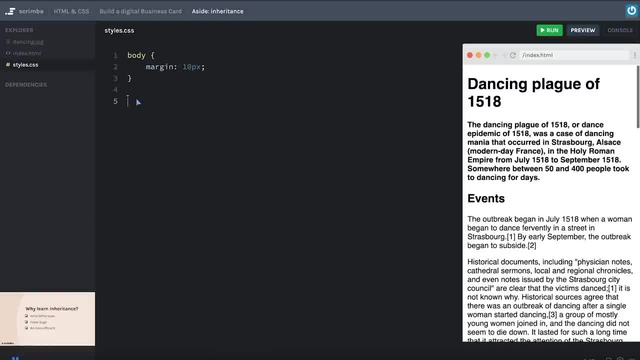 h4,, h2, paragraph and so forth. And let's now say that we want the text in this article to be aligned to the center and not to the left side. Well then, a very poor way of solving that would be to target the h1 first and then do text align center, like that, And then the 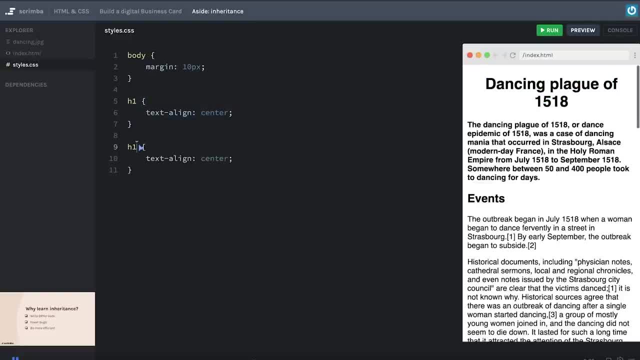 center is text, And then copy that. we can do the same for the h2. And there, you see, the h2 is centered, And then we can do it for the paragraph, like that, and so on and so on. However, this is: 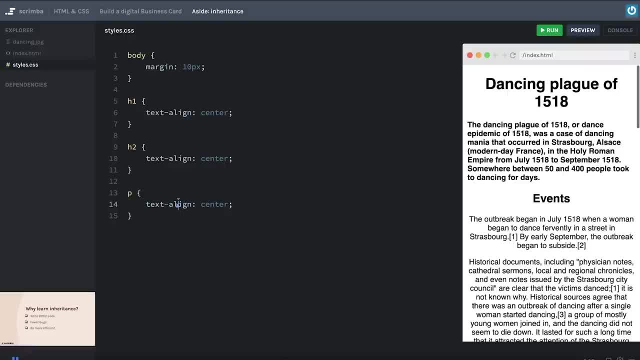 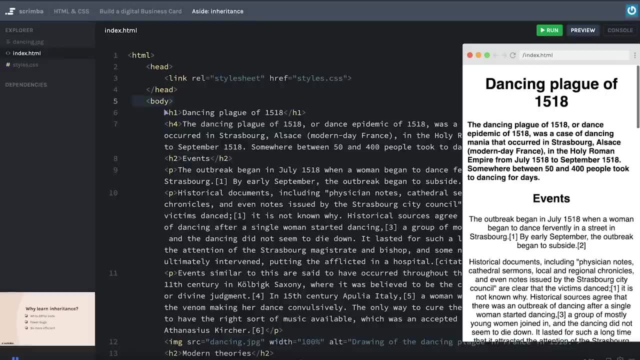 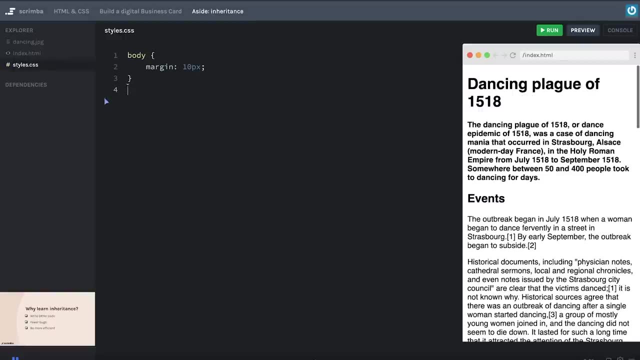 not a dry. we are repeating ourselves a lot here, And it's not necessary, Because since the h1 and the h4, and all of these live inside of the body, they will also inherit some properties from the body tag. So what we can do instead it's just delete all of these. Now it's back. 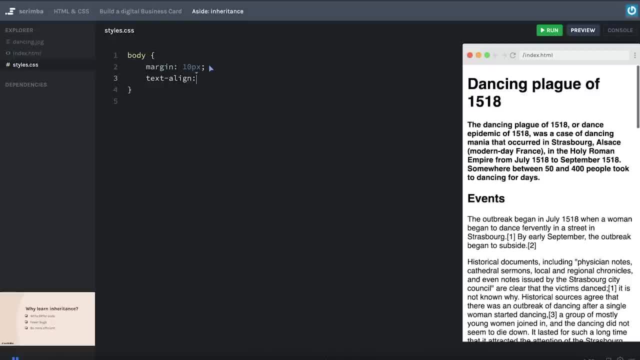 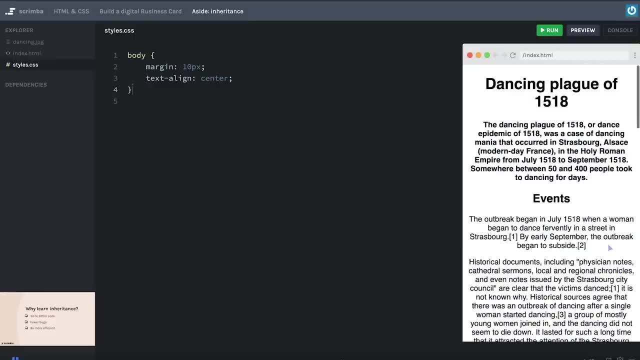 to left align, And then here we can add text: align, Enter like that. Now all of these elements inside of the body are centered. So as simple as that. however, there's only a certain set of properties that are inherited, And actually, 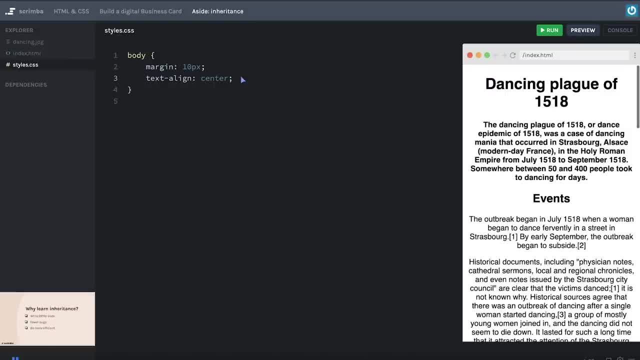 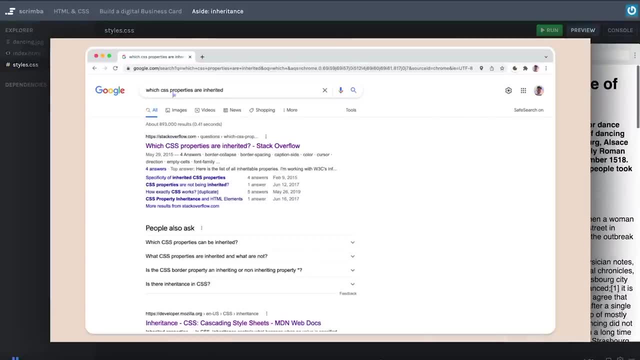 most properties are not inherited. So then you're probably wondering: well, how do I know which are inherited? Well, let's do what we always do when we are unsure of something when we're coding, We'll Google it. which CSS properties are inherited? Here's a Stack. 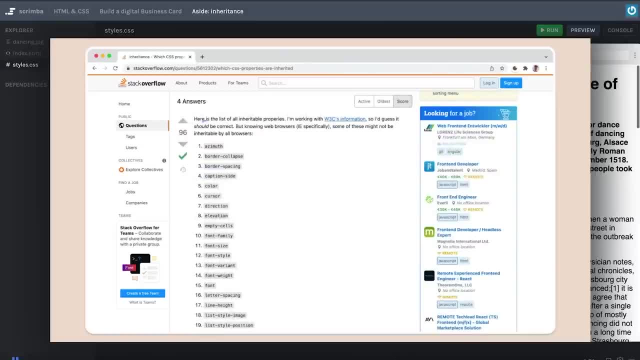 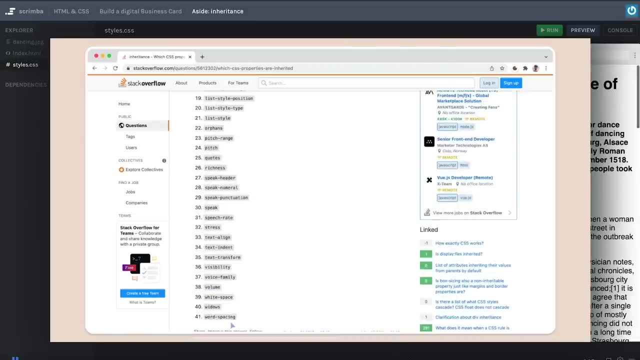 Overflow question And scroll down to the first answer. You can see here is a list of all inheritable properties. you can see it's down to 19.. If we scroll a bit down, down to 41. in total, that is quite a lot. However, you only need to care about very few of these, one of them being the text. 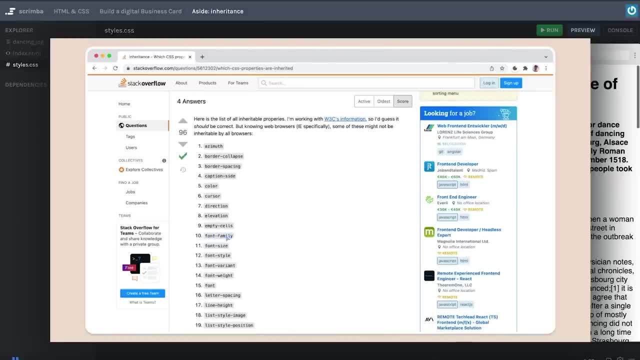 align that you just saw, and the others being the font properties, So font family, font weight, font size and so on, And finally also the color. Other than that, don't worry about any of these At this point. you're going to look at the text align and you're. 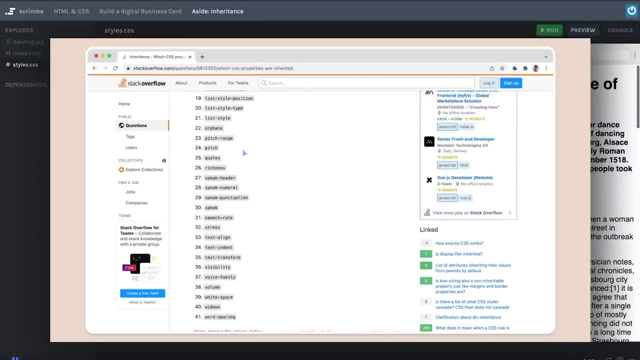 going to look at the font size, and you're going to look at the font size and you're going to learn some of them later. But, to be completely honest, there's a ton of CSS properties here I have never heard about before. I recorded this scrim. Okay, now it's time. 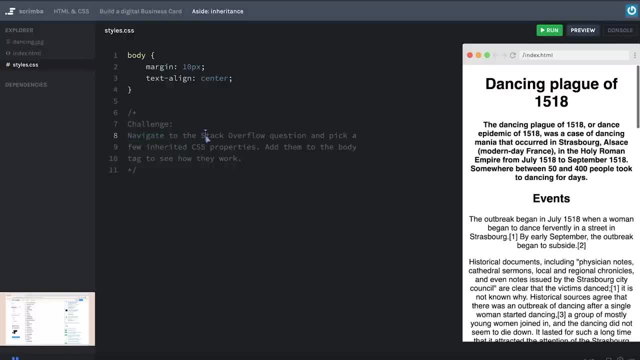 to get your hands on the keyboard. So I want you to navigate to this Stack Overflow question- this one right here- and then pick a few random inherited CSS properties and then add them to the body tag up here to see how they work. You probably have to Google them to figure. 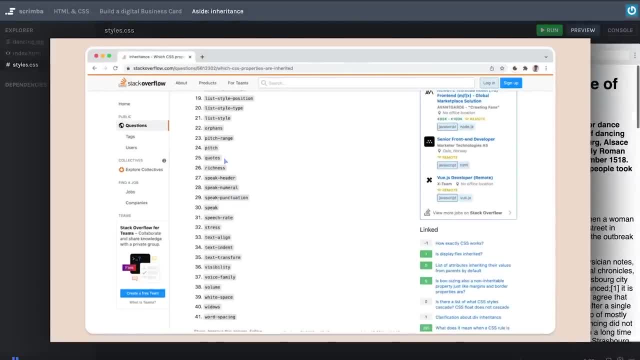 out what kind of value you should set to the properties, But that's also just good practice. Now, some of these is to warn. you are meant for screen readers or audio for, for example, speech rate and volume and stuff like that, So they might not result in any. 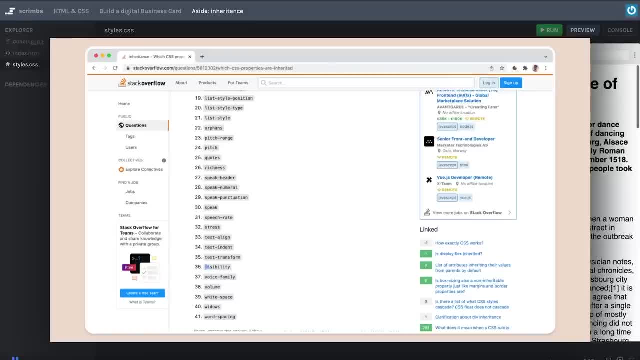 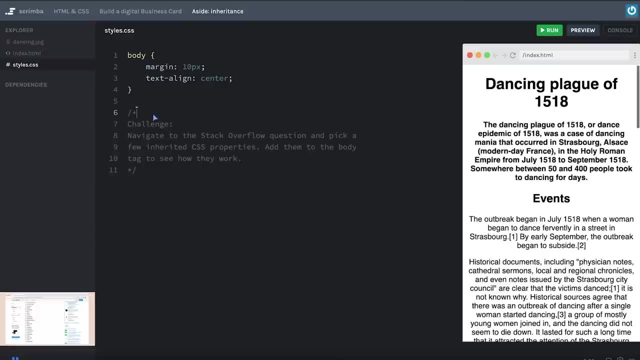 visual change on the page. others will, So just pick a few, try it out, see how it works. In order to experiment a little bit, you can click on this image to get to the Stack Overflow question And then, when you have experimented with a couple of properties, I will see you. 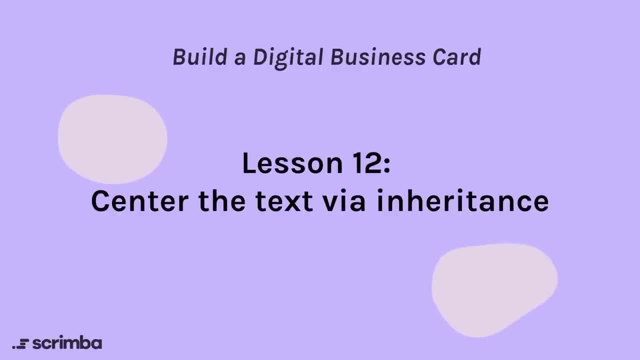 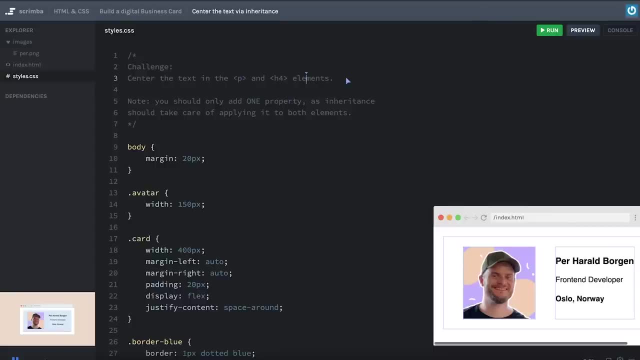 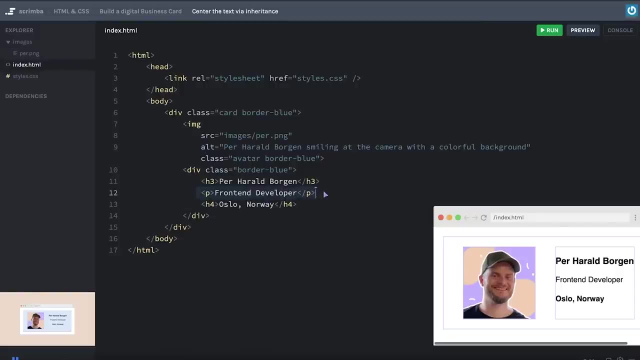 back in the next scrim. Okay, now it's time for a challenge in the business card project, because you are going to center the text inside of the paragraph and the age four elements, And that is the paragraph right here which has front end developer and the age four right here. Because, as you can see, 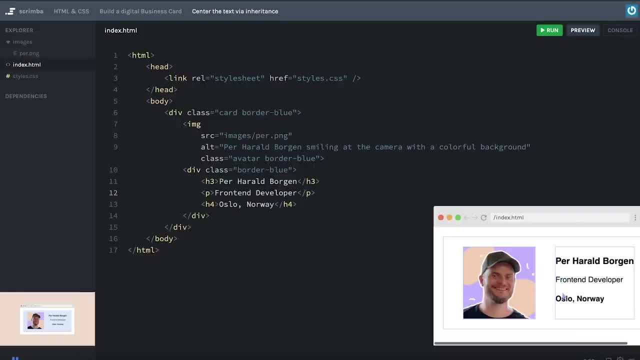 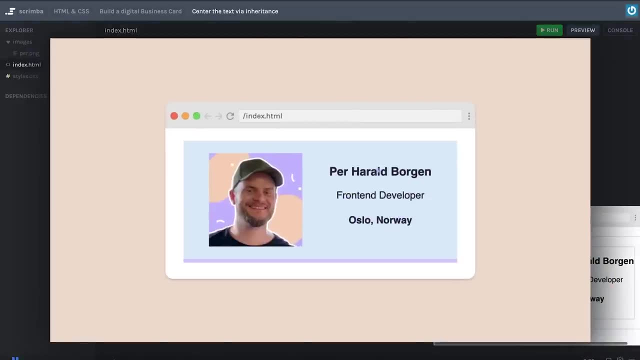 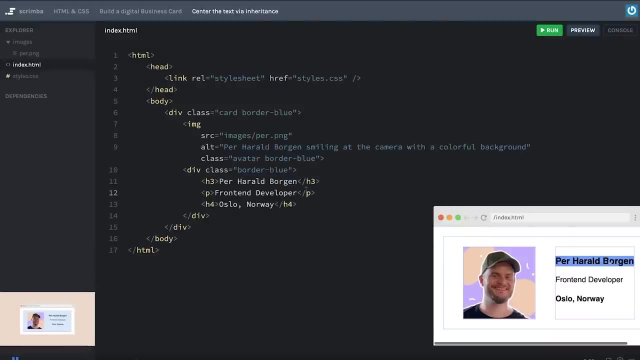 both of those elements are now crammed all the way to the left hand side, whereas in our finished design they are aligned at the center of this flex children directly underneath the name page. And if you're wondering why we're not caring about centering this one, is because it takes 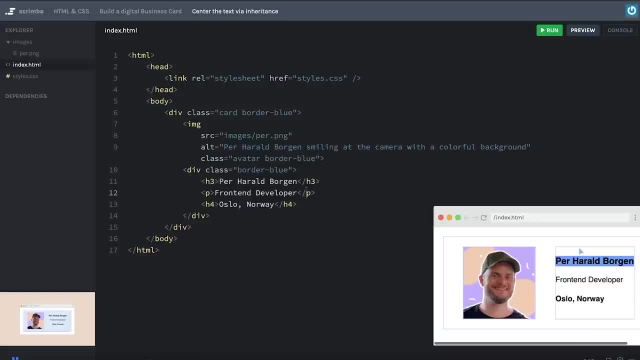 up the full width of the container, So you can't center or left or right align it, because it takes up the full width. Anyway, it is the element that actually decides how wide this container should be. So you will only see the paragraph and the age for change when. 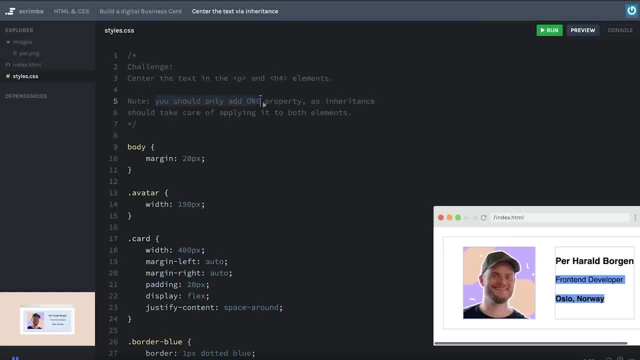 you fix this And the way you should do it is by only adding one property and then have inheritance take care of applying that property. So I'm going to go ahead and add one property to both elements. So you're only going to write one line of code. I'm not going to tell you where you should add that line of code. 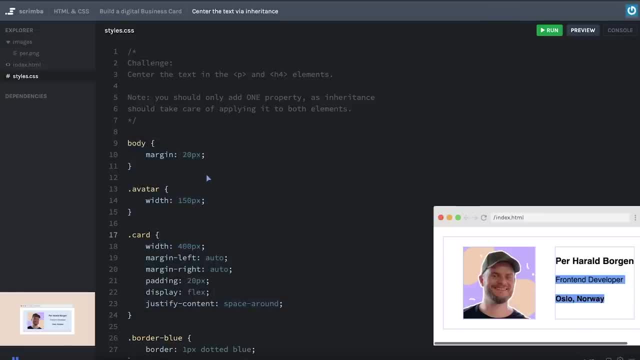 you have to figure that out on your own, And I'm also not going to tell you what the property is called or the value you'll give it. but you have seen it before So hopefully it's not that foreign to you. So jump into the code and try to solve this challenge now. 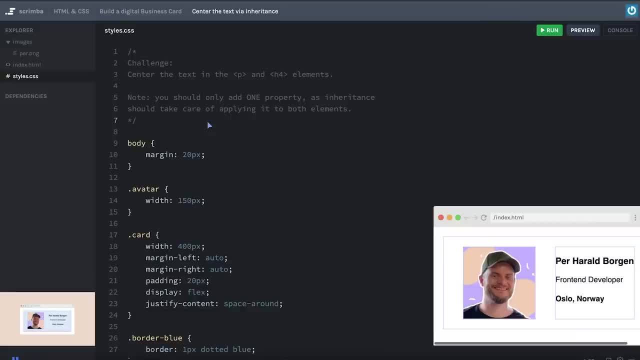 Then, of course, revert back to me when you want to see my solution. Okay, hopefully that went well. Now we're going to use the text align property and set it to center, But before we do that, we need to decide which element we should target with that property. 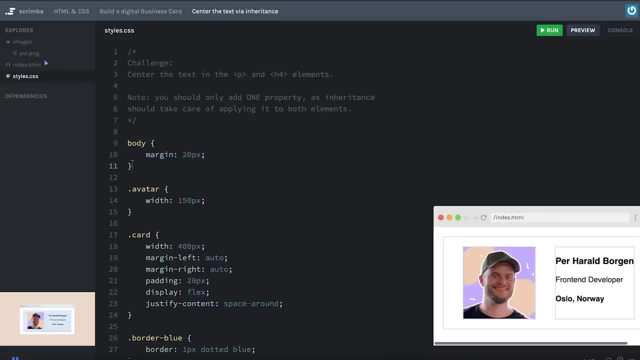 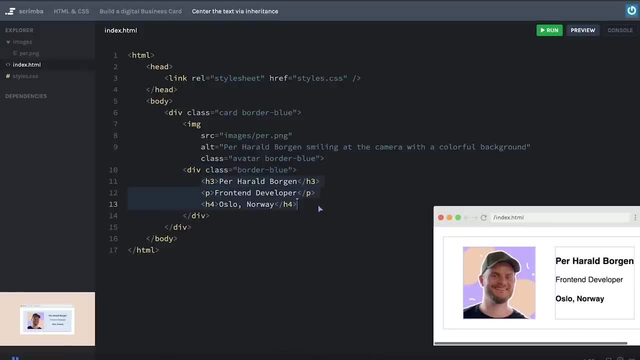 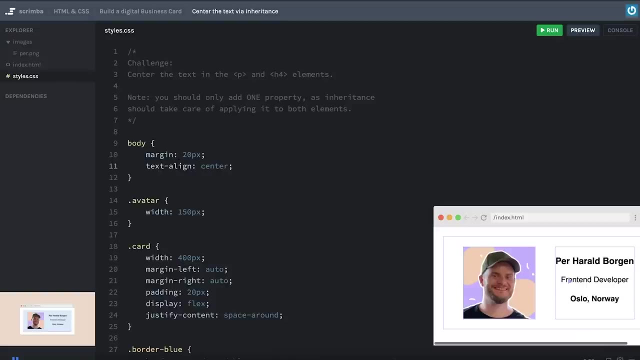 Should we add it to the entire body, for example? if so, it will inherit down from the body into the card and then into our flex children right here. And then finally, to these elements as well. that works perfectly fine. We can actually try it. text align, center and boom. 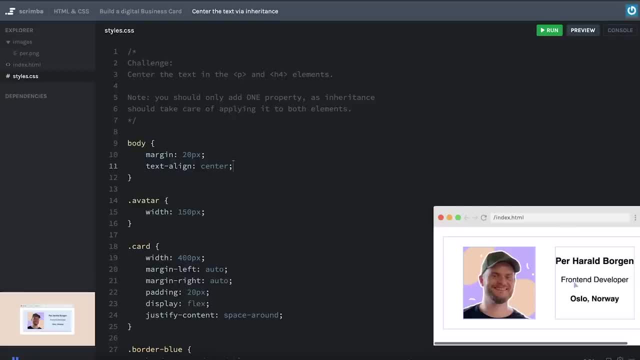 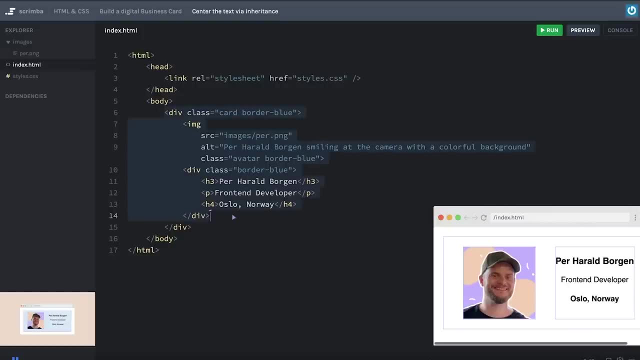 these two are now centered. However, imagine that this card is a part of a bigger website. If so, we've now centered all text inside of the body, which is where all of the HTML, both now and in the future, will live. Well, this might have second order consequences. 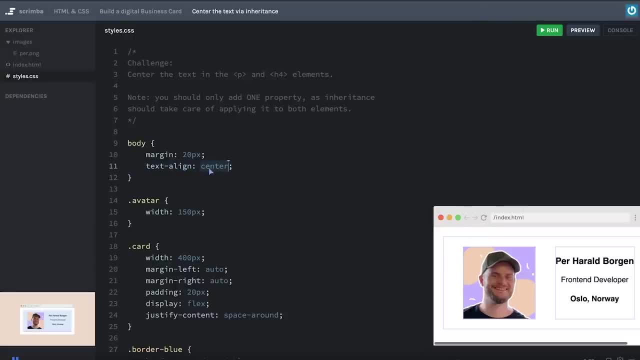 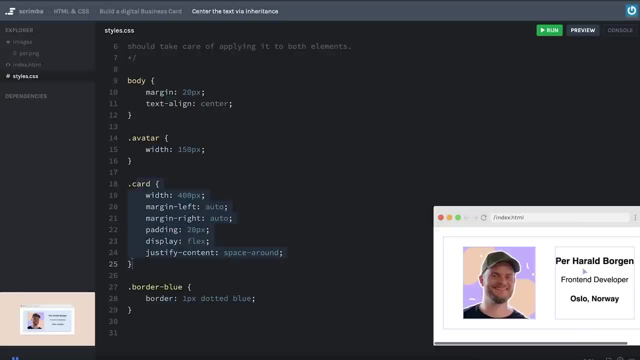 perhaps we want to have a nav bar with a title that isn't text align center, but rather text align right or left. So actually I think it's better to scope this to, for example, our card. we at least know now that all the texts we currently have in our card should. 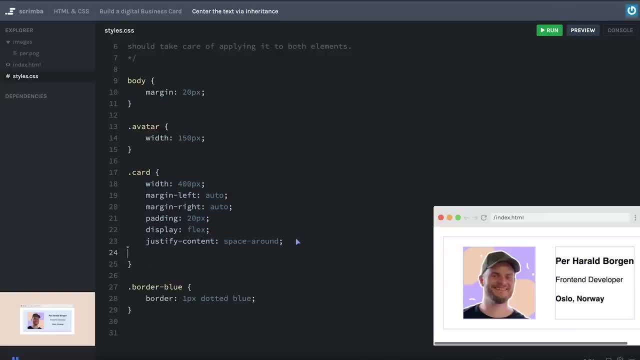 be aligned to the center. So let's do that Instead. let's just remove it from the body and paste it in here And now. we're not causing any unwanted second order effects outside of the card. So this is, in my opinion, a better solution. But if you added it to the 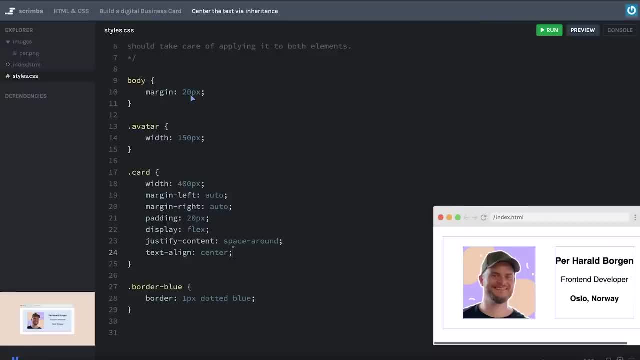 body. that is a perfectly valid solution as well. So don't feel that you did a mistake in coding. there's always plenty of ways to solve things And there's rarely one right answer. There's just consequences for whatever choice you make. So really good job doing. 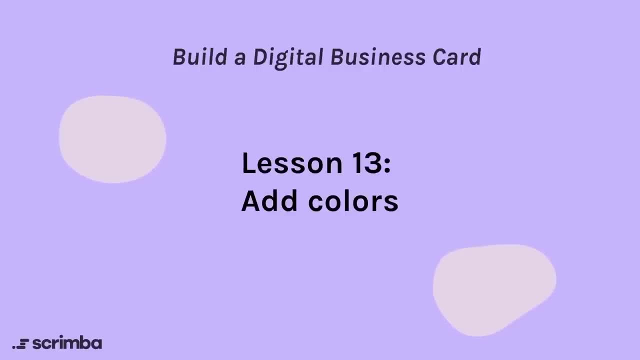 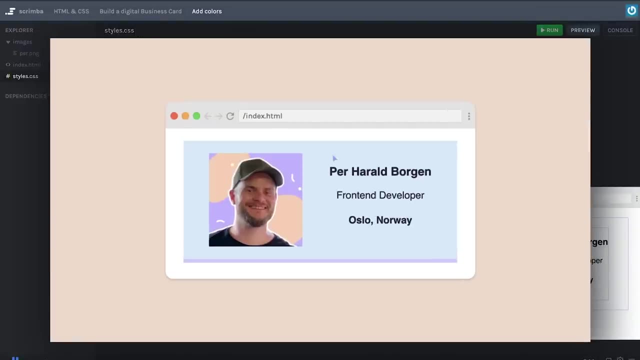 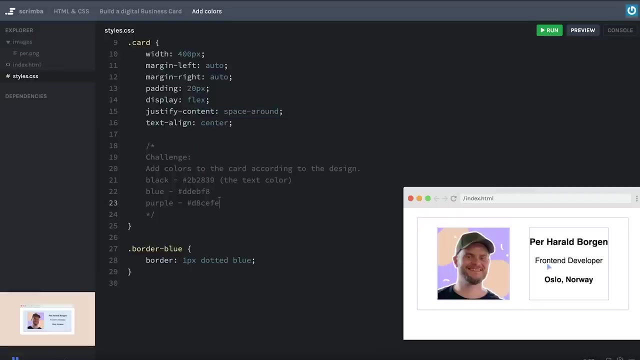 this, Let's move on. All right, now the fun stuff remains, which is adding colors according to the specified design here. So this is a really rewarding little challenge that will make a ton of difference, as you'll go from this boring white layout here to a nice colorful layout. So you're 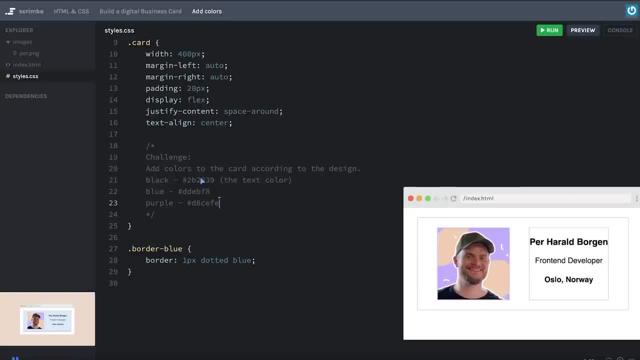 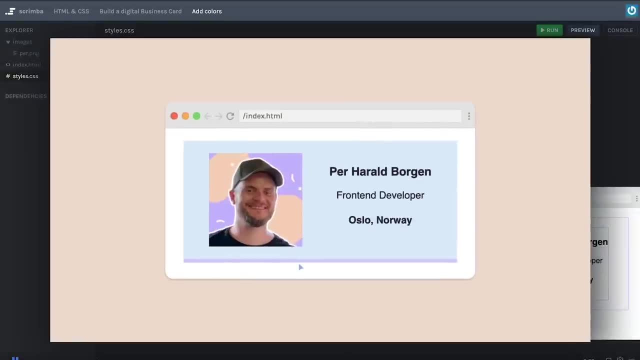 going to add these three colors. As you can see, I've added the hexadecimal values for each of the colors: the black, the blue and the purple. The purple is the border at the bottom here. The blue is the background color, Of course. and then, finally, you might wonder: well, what's the black? Well, that is actually. 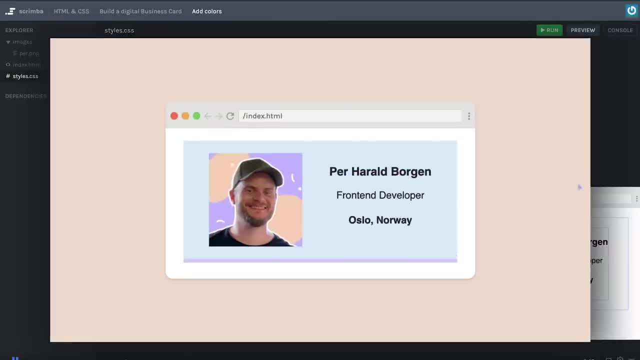 the text color, as the text here isn't pure black, as it uses this shade of black instead. Now you might wonder: well, how do I create this order at the bottom here? I've only learned how to create borders around an entire element previously. Well, the way to solve any problem. 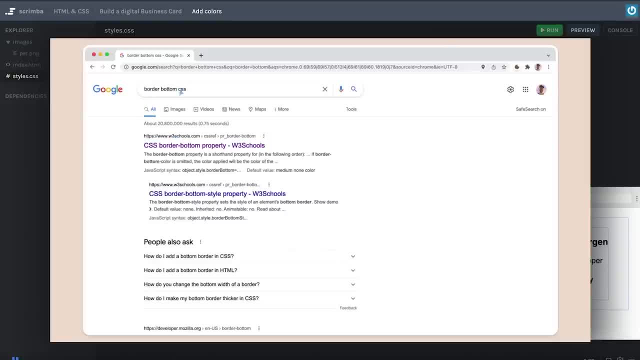 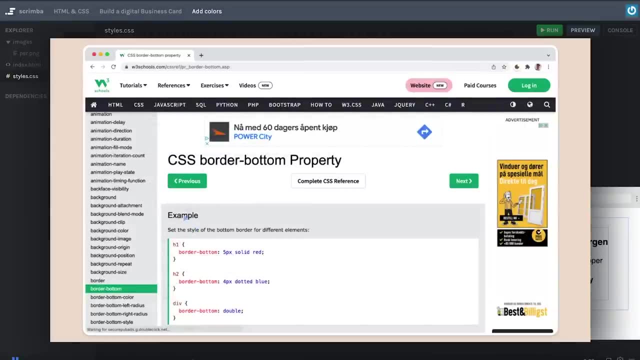 when coding is to Google it. So let's just write border bottom CSS in Google. There you can see a w three schools article. click in on it And here it has some code examples which we can zoom in on. set the style of the bottom. 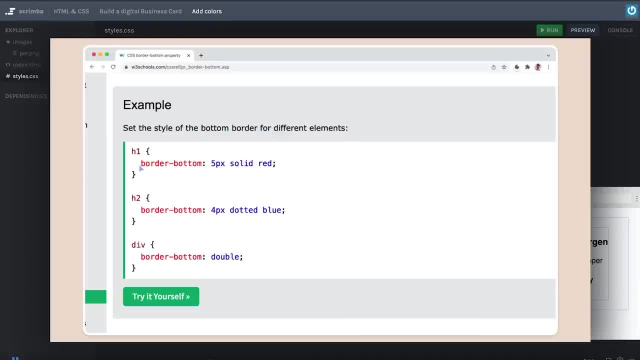 border for different elements, And here it shows us how to set the border bottom. So we do border dash bottom and then, for example, five px solid red. Well, that's exactly how we'd set the border itself, except that we would omit this dash bottom in the property. 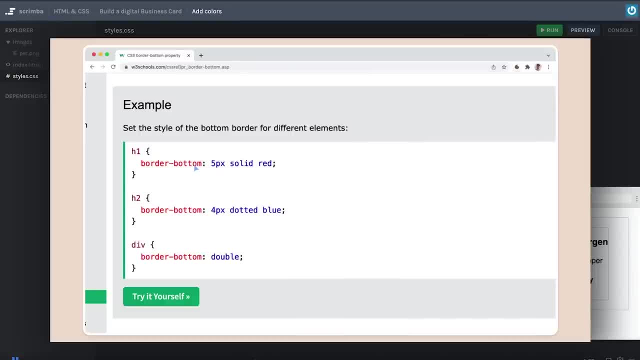 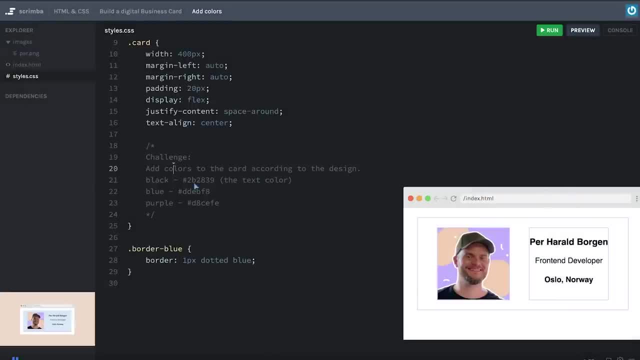 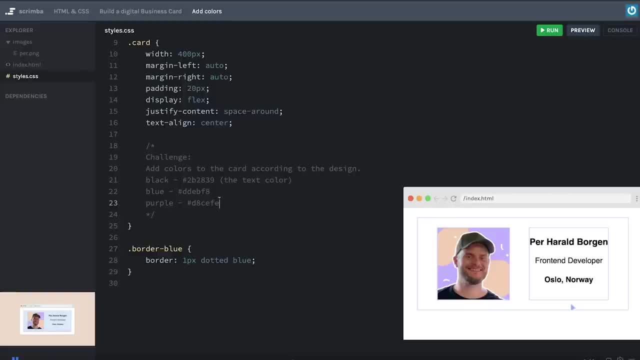 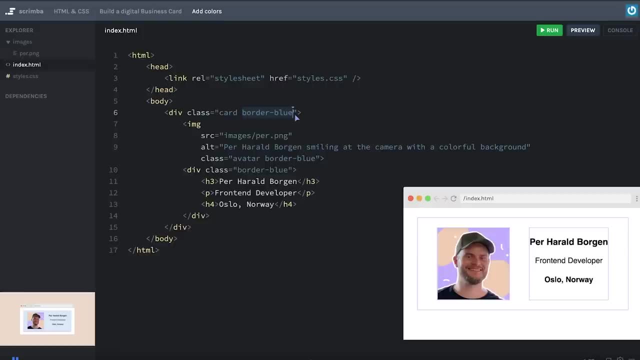 it to you is to remove these blue borders here because we don't need them anymore. So let's head into the HTML. I'm going to mark the border blue. utility class: we've added do command plus D that enables you to select multiple instances of whatever you've highlighted. 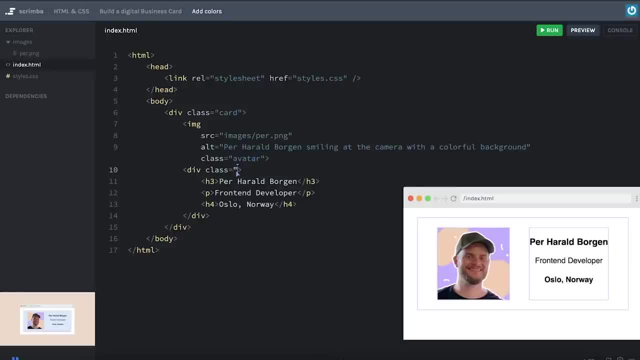 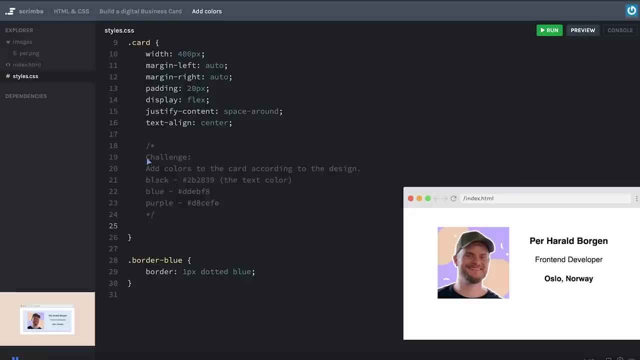 And then boom, I'm going to remove it like that. Then also, we don't need any class in the div. But this flex children anymore And the code, our borders are gone. I'll leave this for now, in case you want to add it back in. But now it's your turn. Go ahead and try to solve. 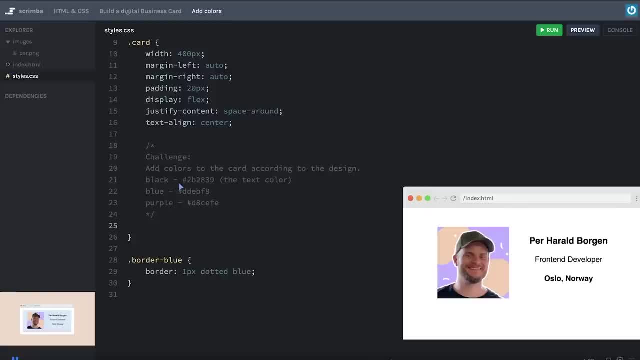 this challenge And then, of course, I will show you the solution when you return back to me. Okay, hopefully that went well. Let's now do it together. I'm going to start with the blue background first. that'll make the biggest difference, So I'll do background. 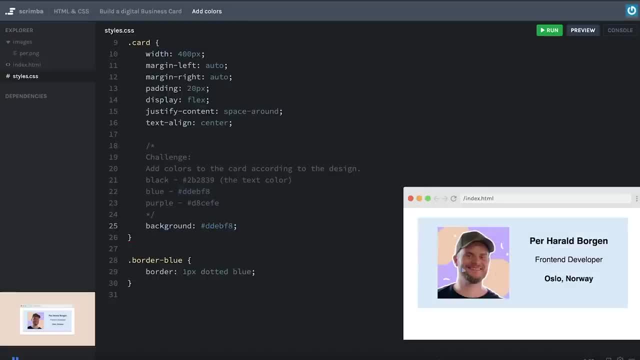 Thank you, And then I'll copy this hex value like that. Very good, Then I'll do the text color is color and copy the one right here. Yes, not as visible as the previous change, But something surely happened. We're now using that shade of black for the text. And finally, the purple. 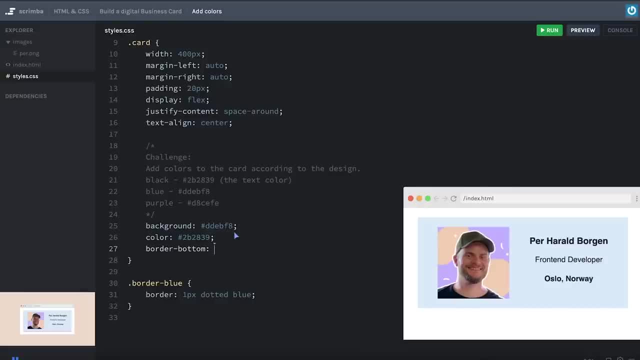 border bottom will be added by doing border dash, Adam. And then let's try two pixels And we want to use solid, then the purple color. Okay, we can see a three. So let's add a thin border at the bottom. Let's have a look at the design. It looks like it is. 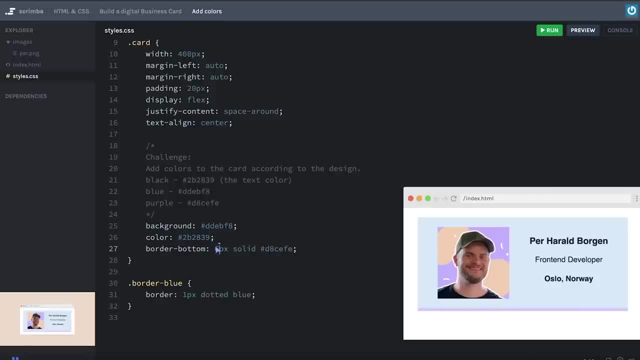 definitely thicker here, So let's crank it up a little bit. For example, six pixels- Yes, that looks pretty good to me actually. So really good job reaching this far. you are very close to the end right now, So let's just keep up this great pace and finish up. 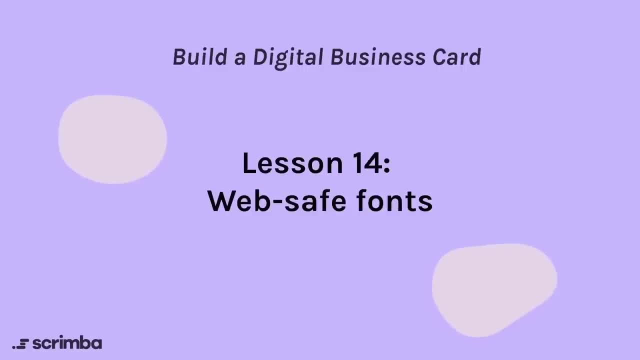 this project over the next few scripts. Okay, now I want to talk a little bit about the fonts, Because fonts are actually really useful, So let's go ahead and do that. So let's go ahead and do that. Okay, now I want to talk a little bit about the fonts, because 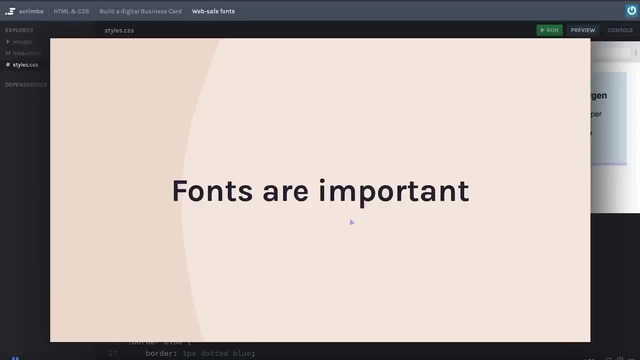 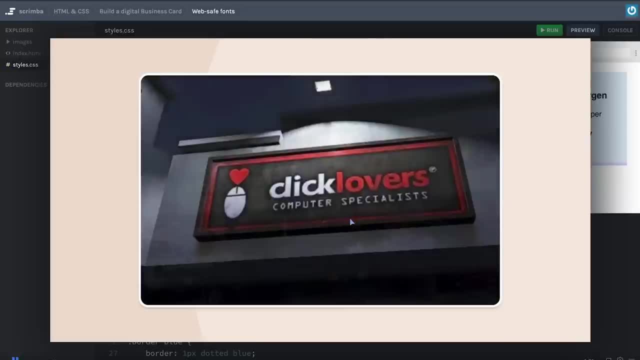 fonts are really important. Let's say that you, for example, have created a computer specialists company called click lovers. Well, you might want to think about which font you choose in that case. Or if you're the owner of the Megaflix shop, you should also think carefully. 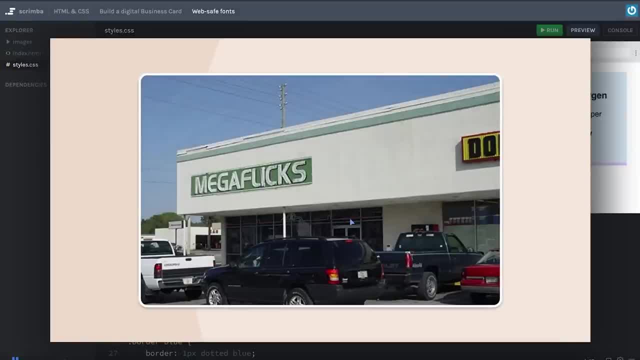 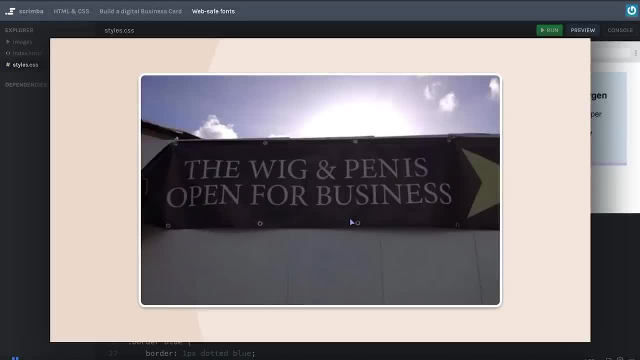 about which font you choose. Finally, if you are the head of the wig and pen Association, make sure that your font spaces out words correctly. Now, these are, of course, extreme cases and they're all on prints. you'll rarely see cases as bad as this on the web. But fonts. 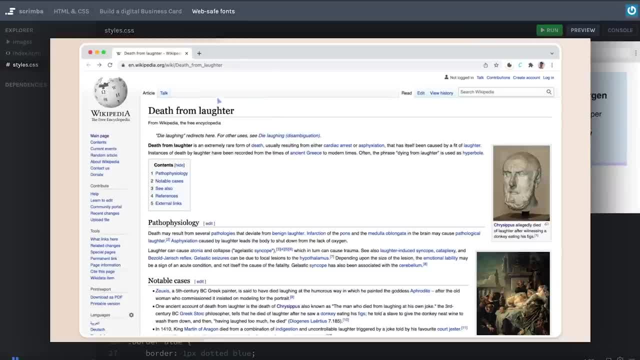 really matter online. Let's take Wikipedia, for example. here is a random article about people who have died from laughter. As you can see, Wikipedia has this very serious, nice font. But if we change that to something like Comic Sans, you can see the text gives a whole different type. 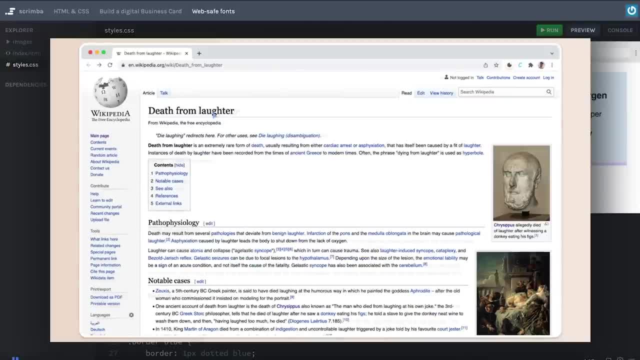 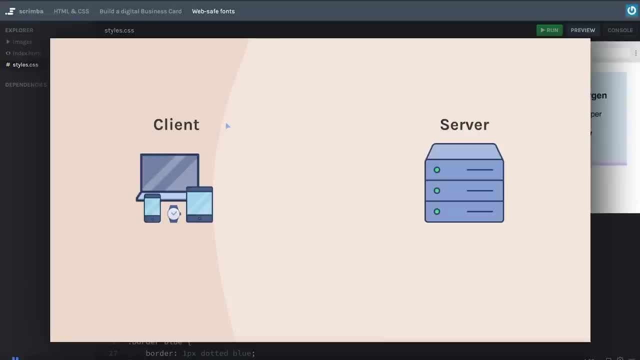 of association. it went from being very serious like this to being more like a comic book. So when you are building projects, it is important that you choose a font that kind of suits your project. So let's move on to look at how it works technically under the hood, Because 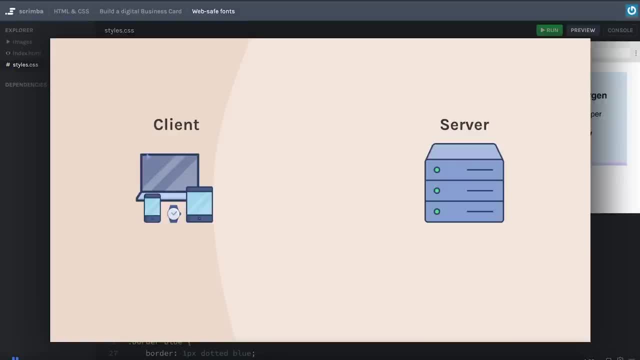 when you visit a website, for example, scrimblers, you're going to see a lot of different fonts. So let's move on to look at how it works technically under the hood, Because when you visit a website, let's say scrimbacom, You visit it via a client that could be your mobile tablet, desktop. 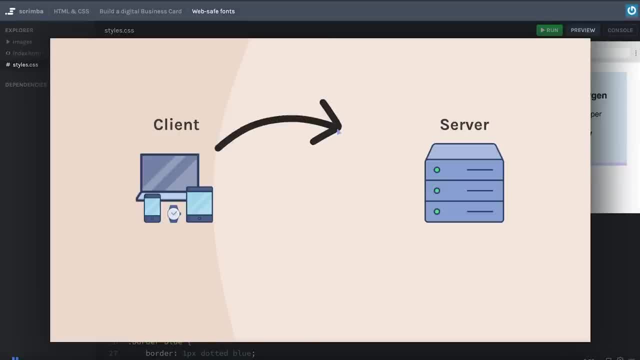 or whatever. What happens is that when you type www dot scrimbacom into the URL bar, it sends off a request to scrim boss server And then the server says, Yeah, okay, You want to visit our website. Yeah, of course, Here you go, And it takes everything you need. 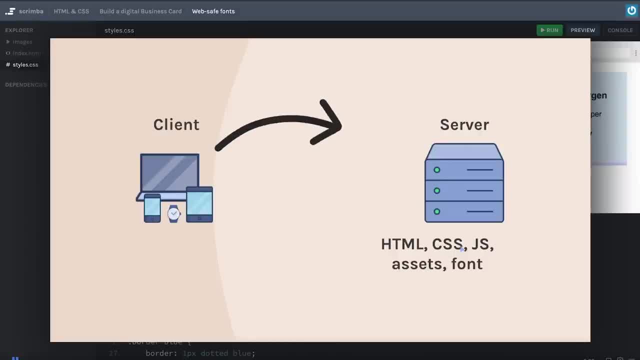 in order to run the screen by in the browser. that is, the HTML, the CSS, the JavaScript, the assets, which can be images and videos and so forth, And then also the recipe for the font, and then it sends that back to the client. However, for some websites they won't send you. 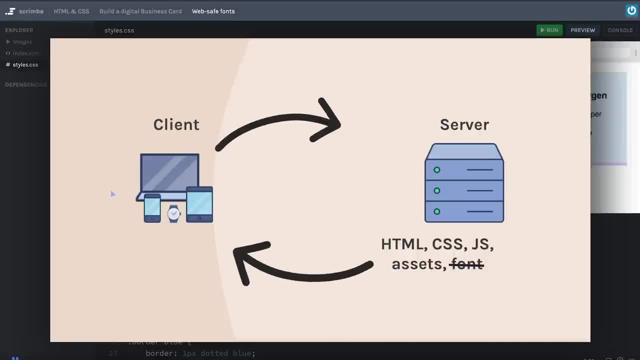 the recipe for the font over the network, because they will instead, on the website, use a font that most likely is already pre installed in your clients And that is also called a web safe font, meaning that the recipe for rendering that font exists in most clients. 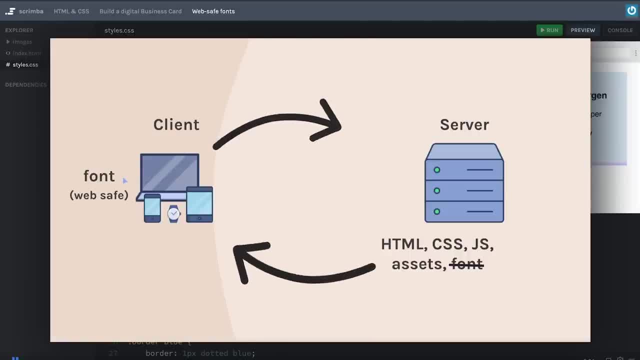 Now, of course, there might be some clients that don't have that specific font, But in almost all cases it's safe to use one of the web safe fonts without sending the recipe for it over the network. So what are these web safe fonts? Well, here is an article on v3 schools where you can 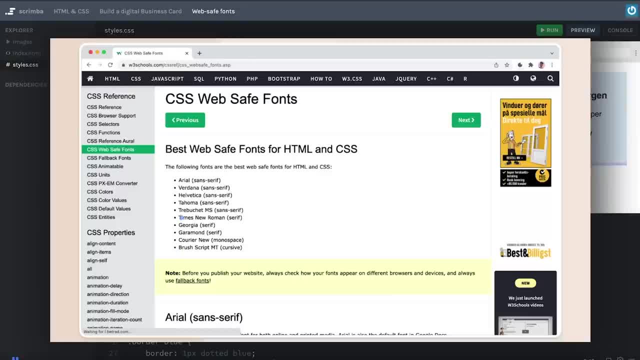 see all of the web safe fonts for HTML and CSS, So when you're using these, you don't have to send the recipe for the font over the network. Now for our digital business card, we're only going to use web safe fonts, But later down the line you'll also learn how to pull in external fonts, so that 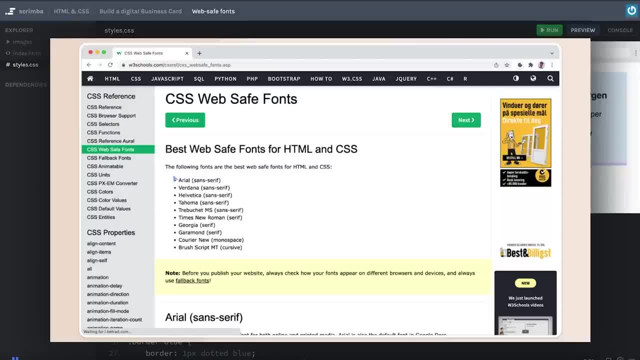 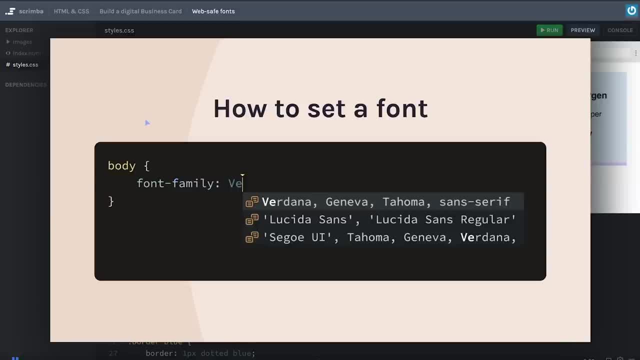 you can go outside of the internet, And that's where we're going to focus on today. So let's take a look at these 10 fonts, as they don't really give you a lot of flexibility. So, with that in place, let's look at how you actually use a font in CSS. So, in order to set the font, 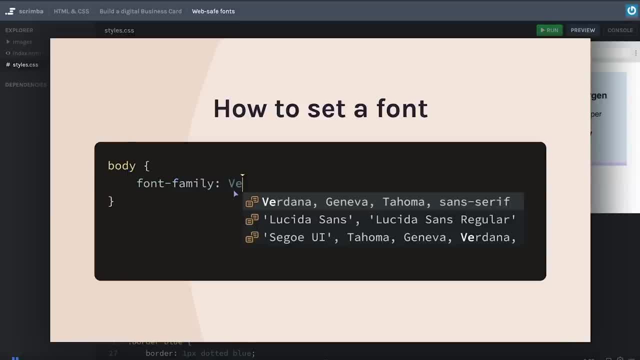 you first target normally the body and then type out font family and then the name of the font. And here you can see we've typed V, E And that triggers vs code, which is the editor powering scrim bar to come up with suggestions for you. You can see it doesn't only suggest Verdana. 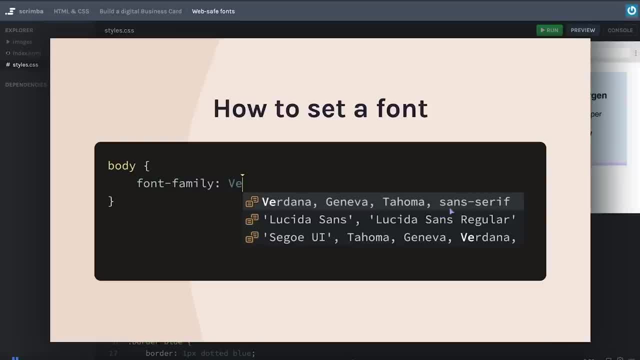 which is the font we want. It also adds a bunch of other fonts after it, All separated by comma. So if we hit enter now, boom, then we've added what's called a font stack, And what this means is that if the browser finds the Verdana font installed, it finds the recipe. 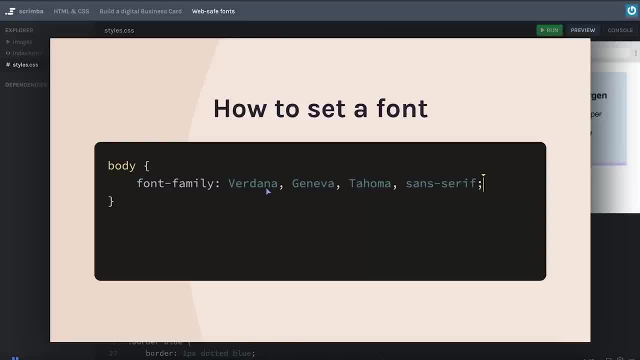 for that font, well then it will use it. However, if it can't find it, if Verdana isn't installed in the client's computer, then it'll try to find Geneva, which is a pretty similar font. If it can't find Geneva, it'll jump on and try to homa, And if it can't even find to homa, it says: well, 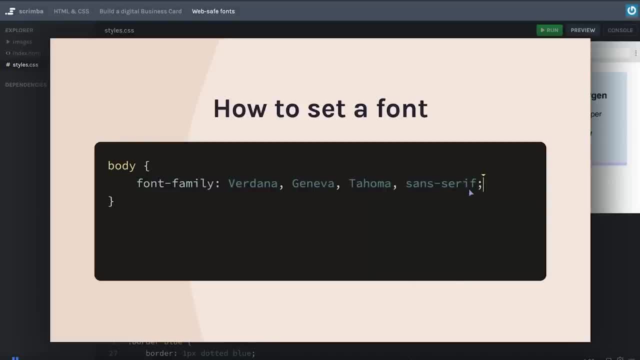 give me any sans Serif font. and sans serif is a category of fonts. So here it's just saying: give me any font from this category. And there are mainly two categories: and serif and serif. Here you can see an example of both of them. Serif fonts contain these decorative strokes: 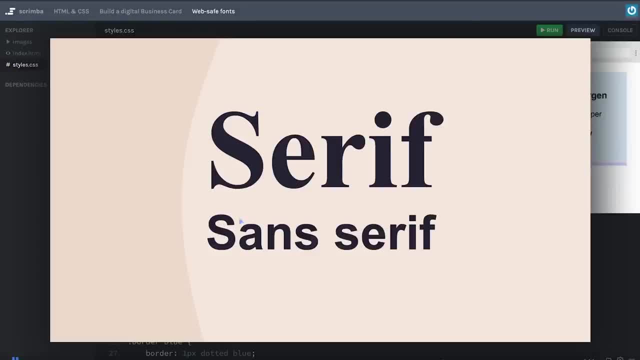 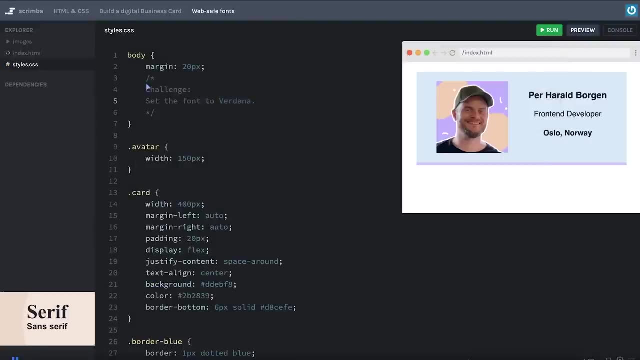 at the end of the letters. you can see here, here, here, whereas sans serif is without those decorative endings. So sans then means without or not, or something like that. you get the point. Okay, that was a lot of theory. Now it is your turn. you are going to set the font here. 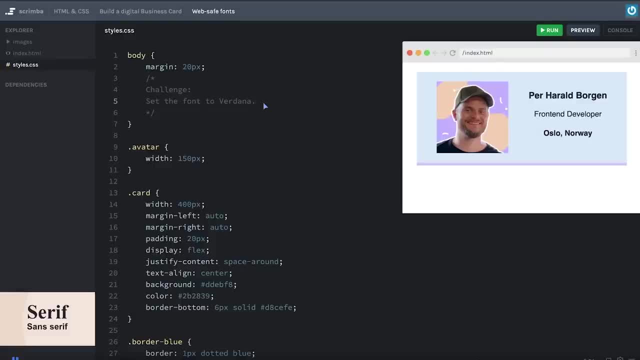 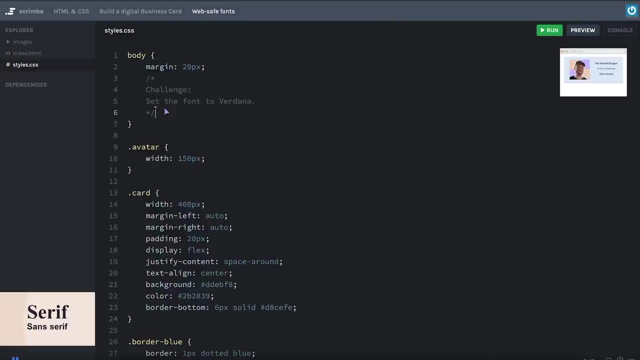 to Verdana And also make sure to remember to get the entire font stack so that we have backups in case the client doesn't include the Verdana font. So go ahead and do that right now. Okay, hopefully that went well. what you'd want to do is font family colon. start typing. 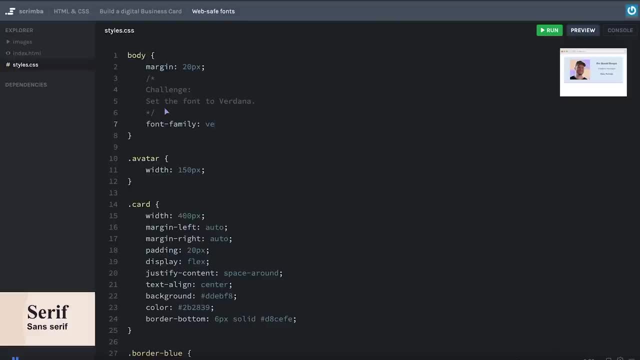 and then the editor suggests The entire font stack. though you won't see that now because the scrim bot DOM recorder doesn't record it, However, I can see it, So I'm just gonna hit enter And boom, the editor suggested this entire font stack. with me. we have changed the font. Let's verify. 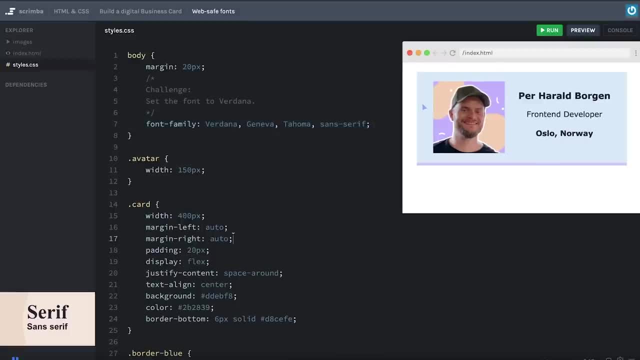 that by removing it, Boom Yeah. that's different from this, So really good job. We've actually now completed the design for our business card. However, there's a little issue with our code, because this is how noobs write their margins: 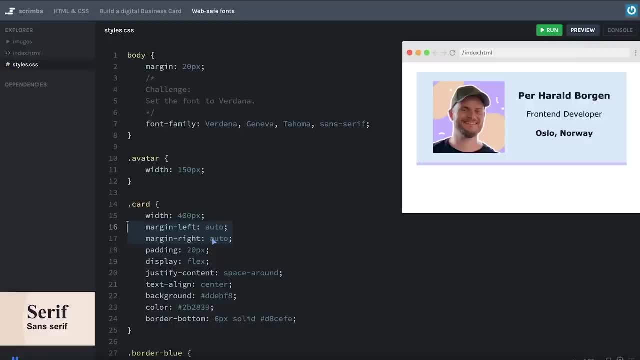 And I want to teach you how to do that. So let's go ahead and do that. Let's go ahead and do that, And I want to teach you how the pros do it. So let's move on to the next scrim, where you'll learn exactly that. 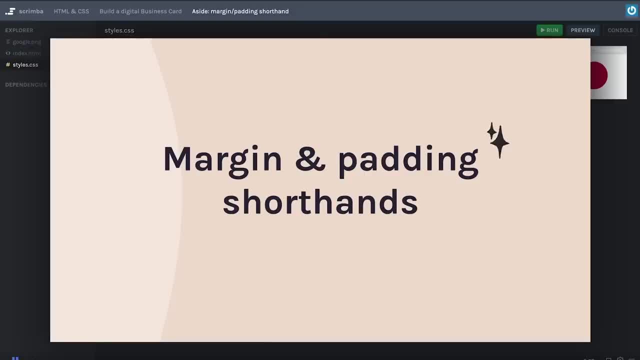 Okay, now it's time to learn about the short hands for margin and padding, And you've actually been exposed to one of them already, which is that if you have the same value on the margin top, right, bottom and left, you can reduce those four lines into one margin: 10. 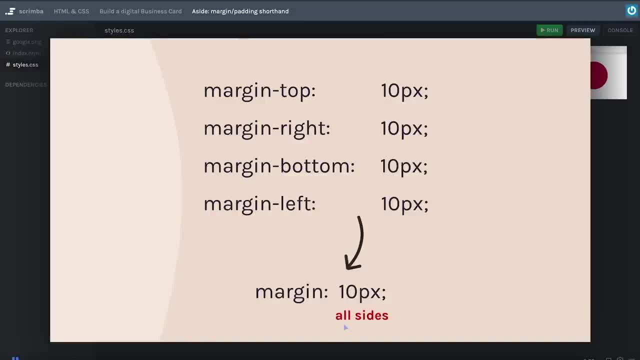 px, then the browser will take this 10 px and apply them to all sides, So these four lines are identical to this one down here. Now the question becomes: what happens when you have four different values, for example 10, px 20, px 30 and 40?? Well, if so, you 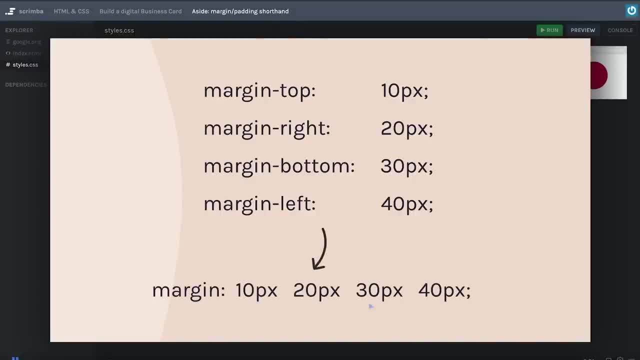 have to do like this: margin and then 10 px, 2030, 40.. So the first one is margin top, the second one is right, the third one is bottom and the fourth one is left. So now you're probably thinking: well, how can I possibly remember this order? And the trick is to think: 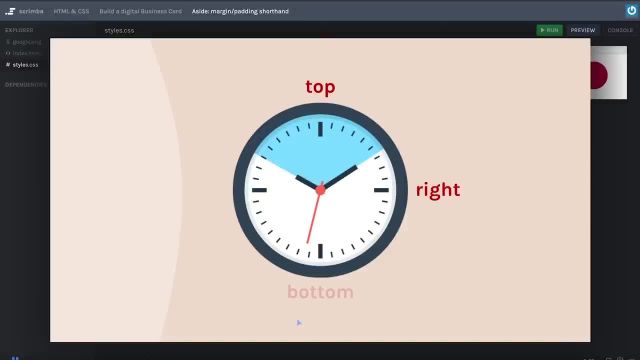 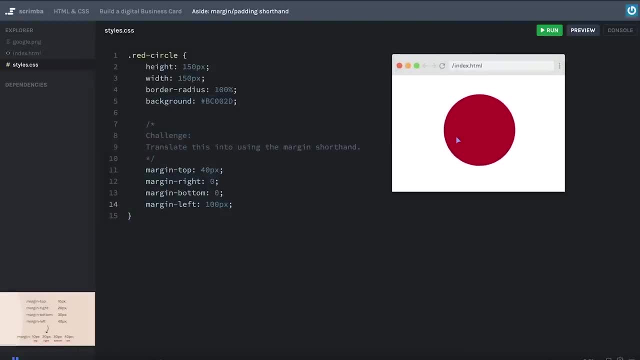 of the clock: it starts at the top, then goes to the right, then goes to the bottom, then goes to the bottom and then goes to the left. So, with that in mind, I want you to improve this code here, which creates the Japanese flag in CSS, Because, as you can see, this: 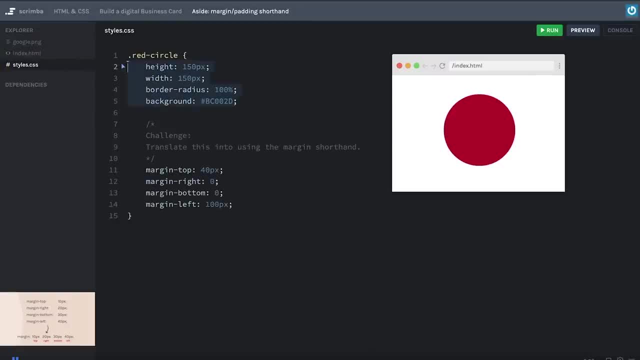 red circle here, which is a div, has a few styles applied up here, But down here we've used the non shorthand way to set the margins, setting some margin on the top so that the circle is pushed down. nothing on the right and the bottom, but 100 pixels on the left. 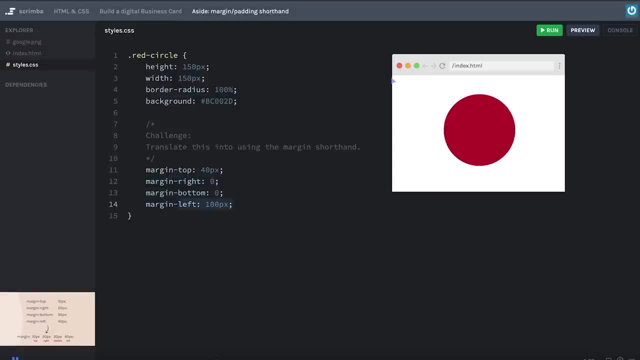 so that it's pushed to more or less The center of the screen, given that the screen is as wide as it is right now. So I want you to translate this into using the margin shorthand instead. go ahead and do that right now. Okay, hopefully that went well. I'm going to actually comment these. 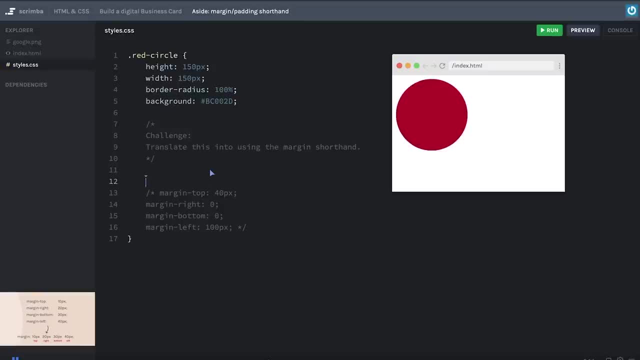 lines out. Now you can see the circle is up in the left corner. And then I'm going to do margin, starting at the top should be 40 pixels, then the right side And zero pixels, and the bottom should also have zero pixels And then the left side. 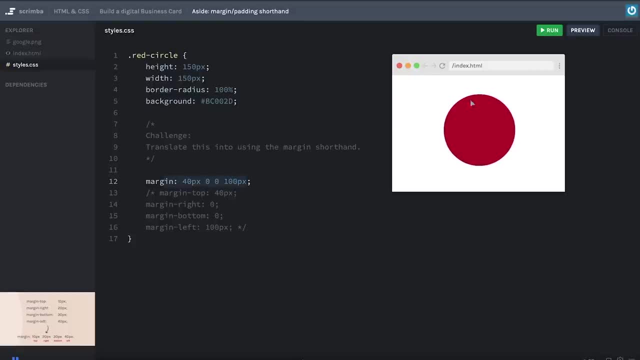 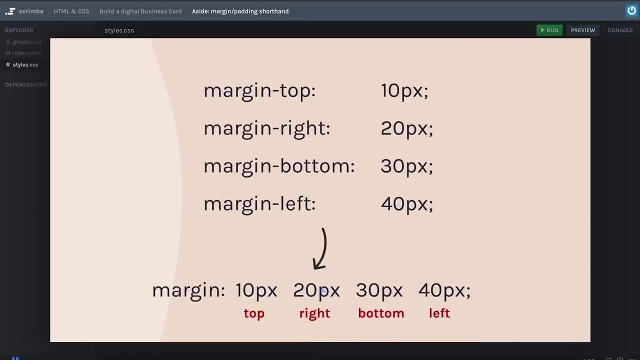 which should have 100 pixels. And there we go, we are back at the exact same layout. So great job if you manage to solve this. Now there's another scenario I want to teach you about as well, which is if we have top and bottom as one value, and right and left. 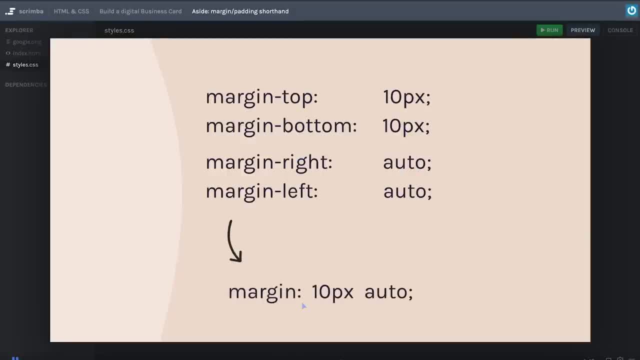 as another value. if so, you can actually reduce it to margin. and then only two values: Here you do 10.0.. 10px and auto, because 10px is top and bottom, auto is left and right. So the way to think. 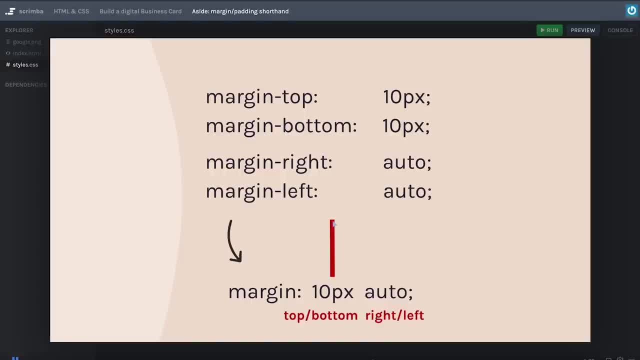 about this is that the first value controls the vertical line, the y axis, and the second value controls the horizontal line, also known as the x axis. So, with that in mind, let me change this a little bit. I'm going to go back to the funky way of writing this And 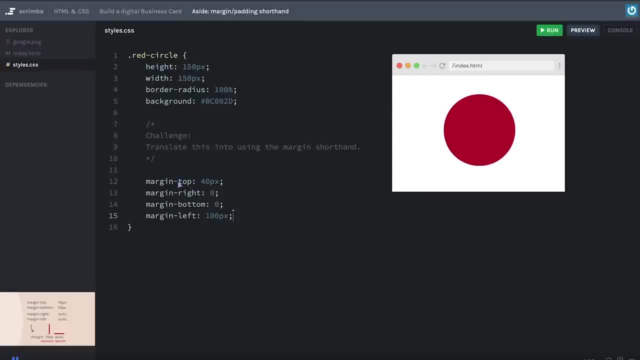 I'm actually going to improve it a little bit, Because if we want to center the circle, we shouldn't hard code a margin left, because that'll only work on this circle, because that'll only work on this screen size. When we do like this, it's not centered anymore. 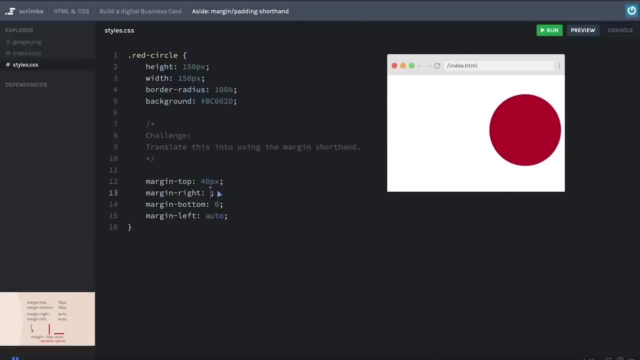 So let's instead use the better technique of using auto on the left hand side and the right hand side, And also just to make sure that no elements are allowed to appear directly underneath our circle. I want to add 40 pixels to the margin bottom, So now I'll make it. 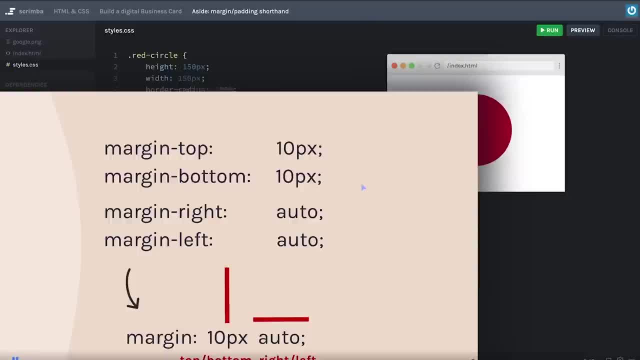 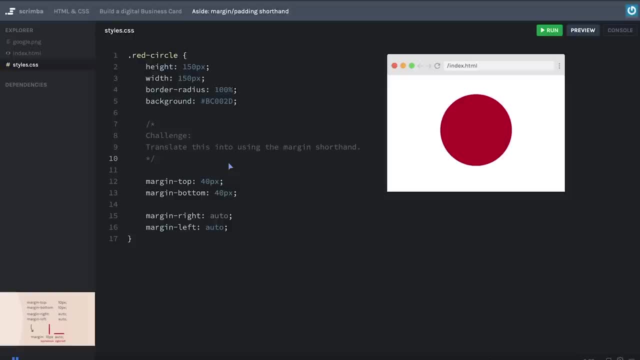 a little bit easier for you and separate these two. With this in mind, can you reduce these four lines into two? Okay, let's do this. I'll comment out these And if you're wondering what shortcut I used for that, I'm using command plus k plus C, but that is on a Mac keyboard. I'll comment. 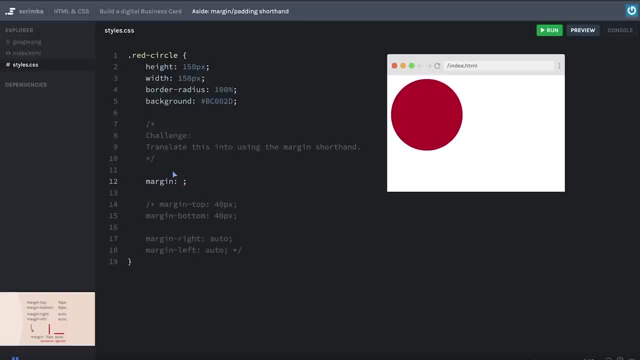 this out. Then I'll do margin. First we'll set the vertical axis. it should have 40 pixels at the top and the bottom, So that is 40px. And then we'll set the horizontal axis, which is auto like that. 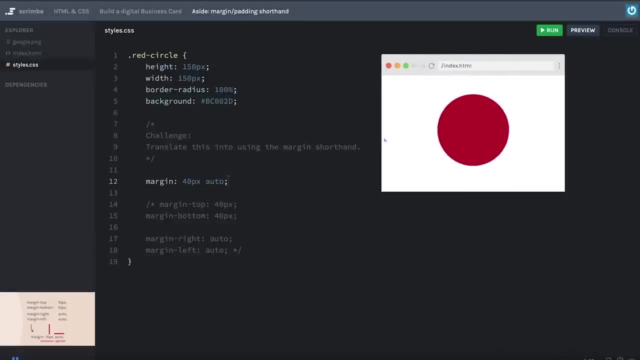 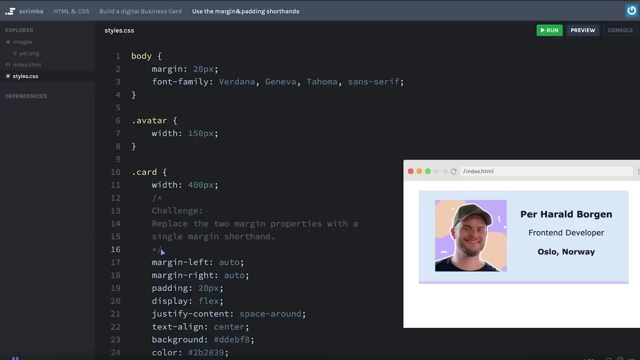 And boom, there we go. We have it centered, at least horizontally, regardless of how wide the screen is, And we have reduced four lines into one. So great job, Let's move on. Okay, now you're going to take what you've learned about the margin, shorthand and use. 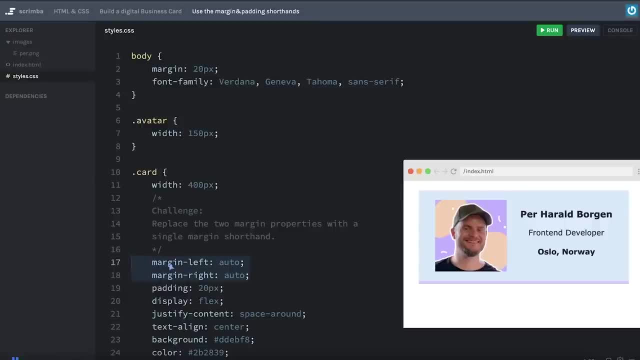 that in order to reduce these two lines into one. So we're going to replace the two margin properties with a single margin shorthand And, of course, after you've done that, the card should still be centered. So go ahead and give this one your best shot. Okay, let's do this. So I'm going to start. 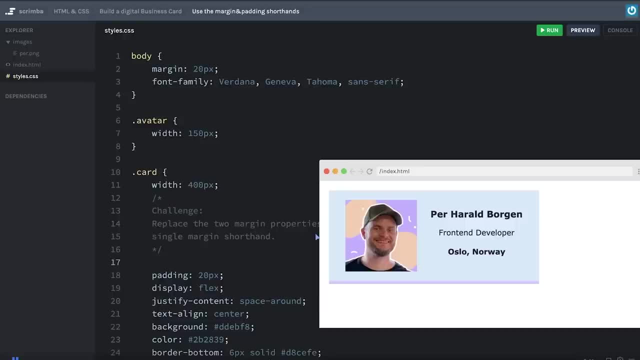 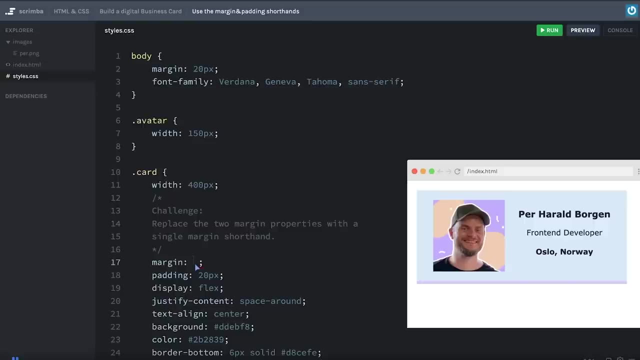 by removing both of these. Now you can see the card is aligned on the left side. So, in order to fix this, we'll do margin And then the first property we'll set will be the vertical line, meaning margin top and margin bottom, because we're only going to set two values. 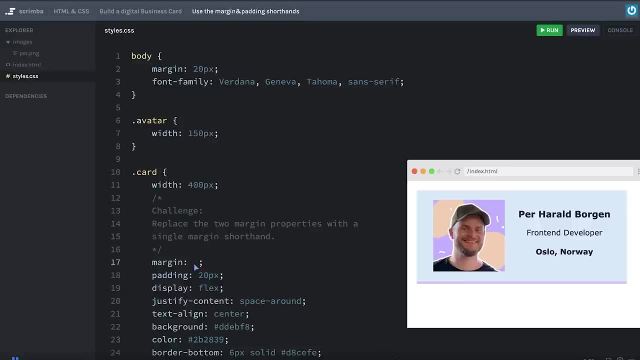 To do that, each of the value dictates two sides, either top, bottom or left right. So we'll set zero as the first value. That means margin top zero and margin bottom zero. Then for the second value, which dictates the horizontal margin, meaning left hand side and right hand. 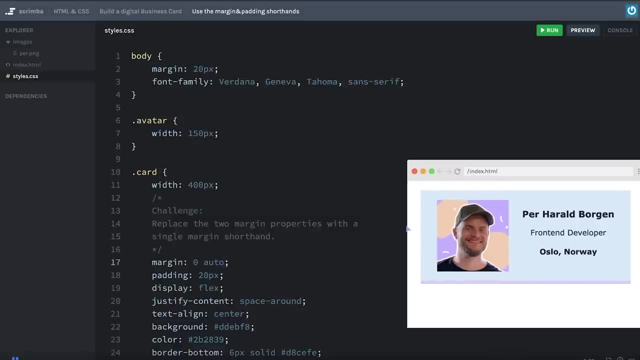 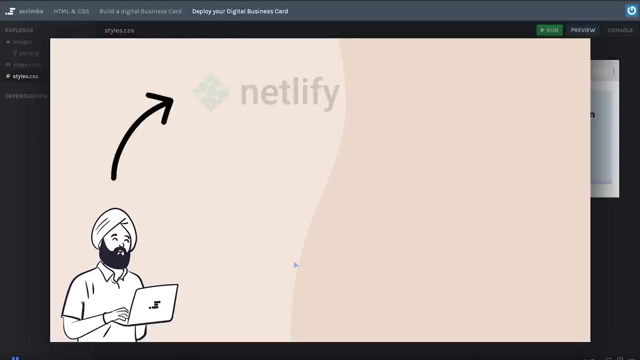 side. we'll set, of course, auto. And there you see, now the card is still centered and we have reduced two lines into one. So great job solving this challenge. Last time we deployed a project, we first added our code to Netlify, which then again. 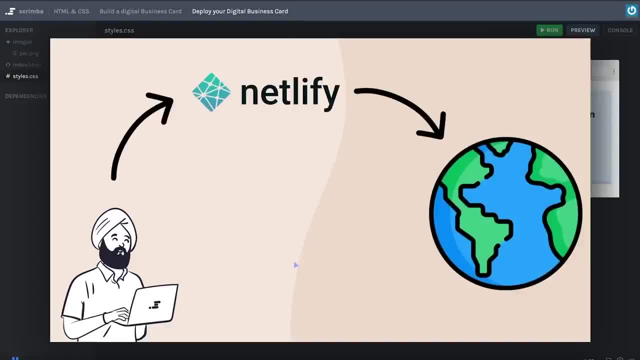 took care of deploying our project to the web. Now, while this works perfectly fine, the way the pros do it is to go via an intermediate service and step called GitHub, and then let GitHub take care of sending off the codes Netlify so that it's deployed to the web. 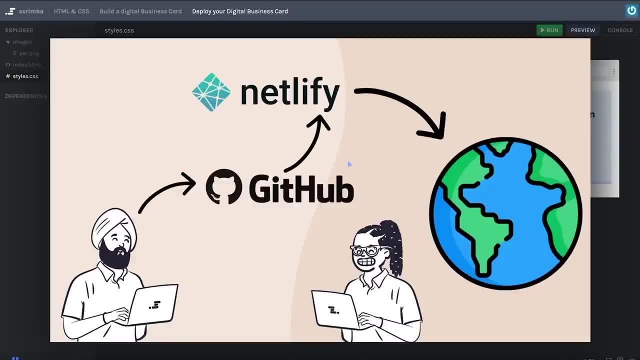 And the reason you want this kind of architecture is because GitHub allows you to collaborate on your code with other developers. So now we are going to deploy your business card using this technique. The first thing you need to do is head over to GitHub. If you're watching this course on a scrim buy, you can just click. 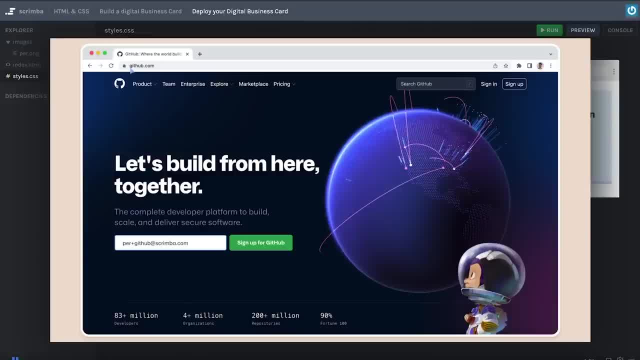 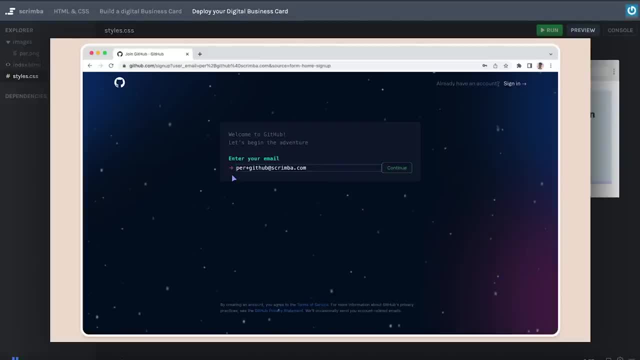 on this slide right here, But if you're following us on YouTube, just head over to githubcom And you'll get to the exact same page. Once you're there, I want you to click at the sign up button. that will open up a form where you have to add your email, create a password. 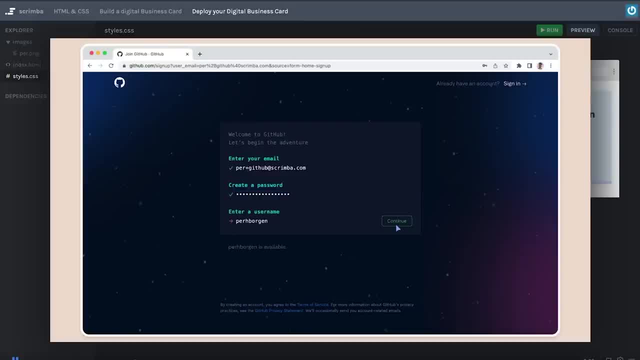 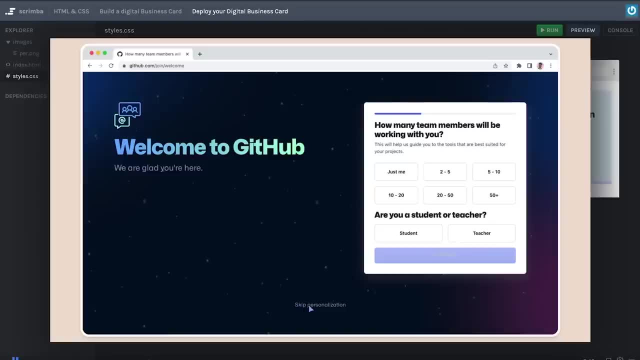 and also choose a username. Once you've done all that, click the Continue button, which then sends you to this onboarding screen where you can add a little bit of information about yourself, or just click on the skip personalization option If you are impatient. once you've done this, you'll see a dashboard. yours is probably. 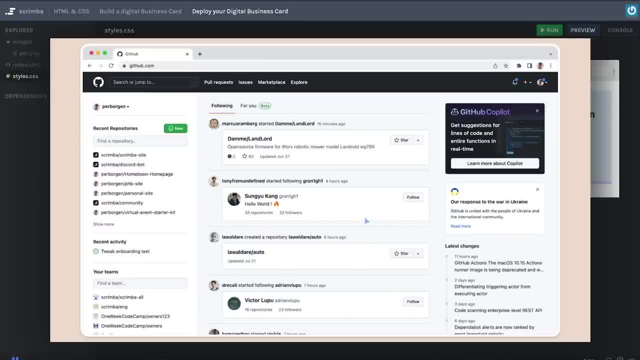 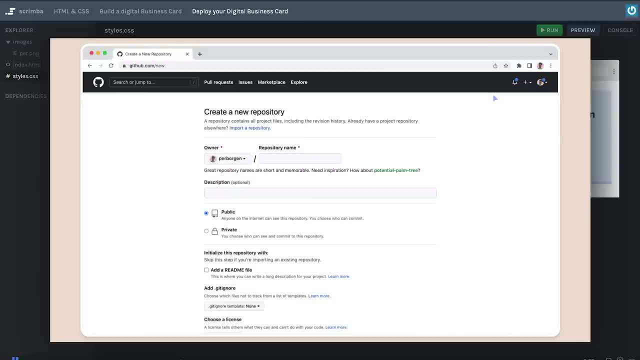 not as filled with information as mine, though that doesn't matter. What we're going to do now is click on the plus icon in the top right corner. there it opens up a menu where you are to choose new repository. the repository is the backbone of any software project. This 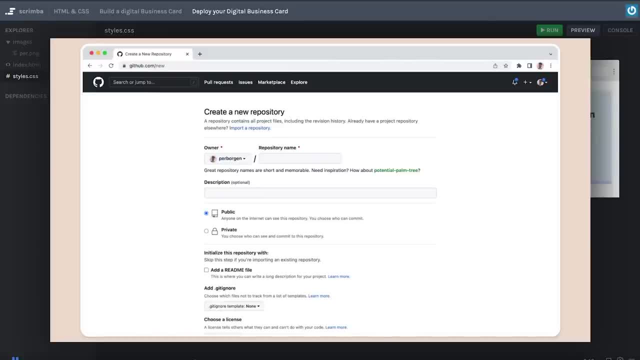 is where you'll find all the project files, And GitHub, along with the git protocol, takes care of your business credentials and security for your project. we're going to talk a little bit more about GitHub in this video of tracking all the changes that has been done to the repository from its birth, though. 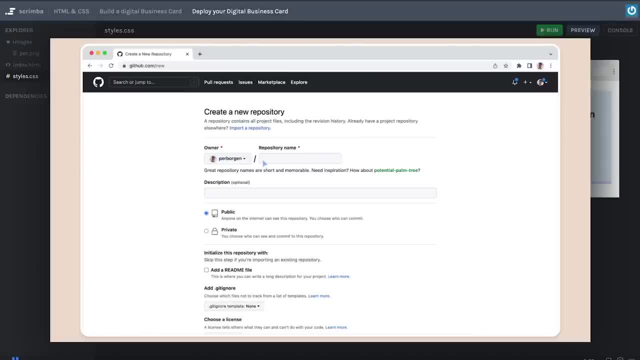 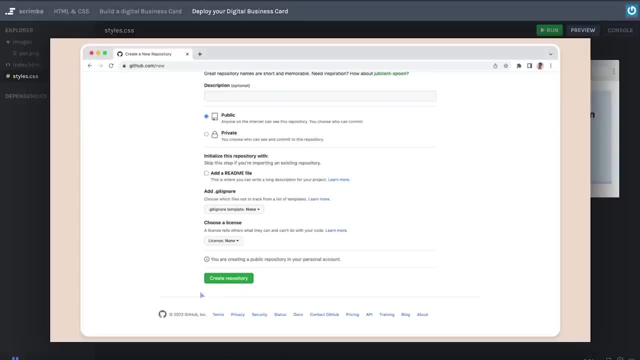 we're getting ahead of ourselves right now. we are just going to give it a name which you type in here in the repository name field, like that. I'm going to call it business card And then I'm not going to touch any of the options here, I'm just going to scroll down. 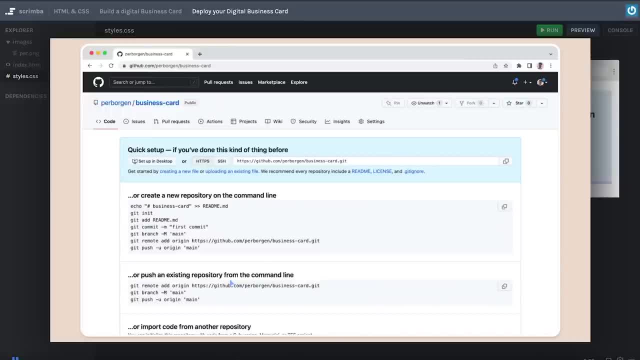 and click Create repository. And there we go. Now we have to upload our files. we can do that in many different ways. Right now, we're just going to do the very simplest one. So what I want you to do is click on the uploading an existing file link right here, as that'll. 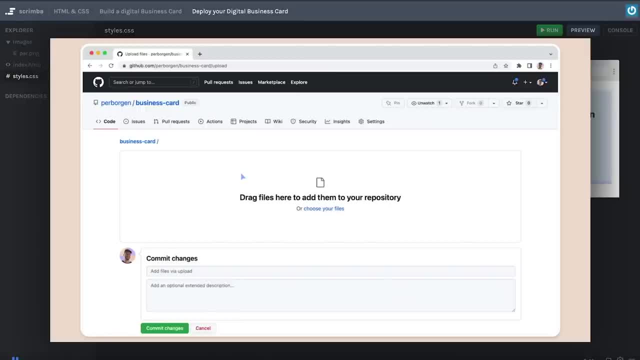 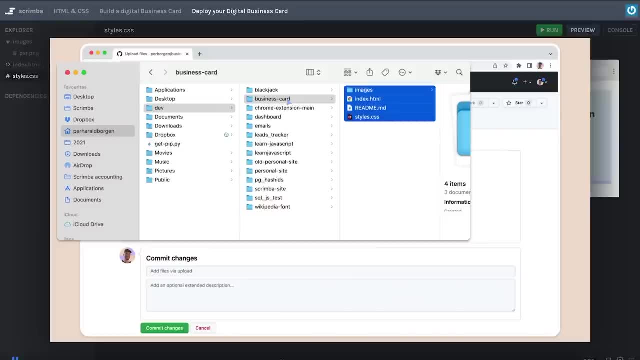 take you to a drag and drop field quite similar to what we saw at Netlify. earlier Here I want you to open up the business card folder which you created on your local computer in the previous scrim mark all of the files and then just drag and drop them into the 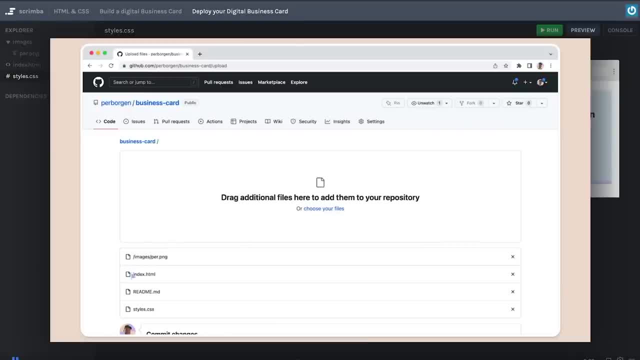 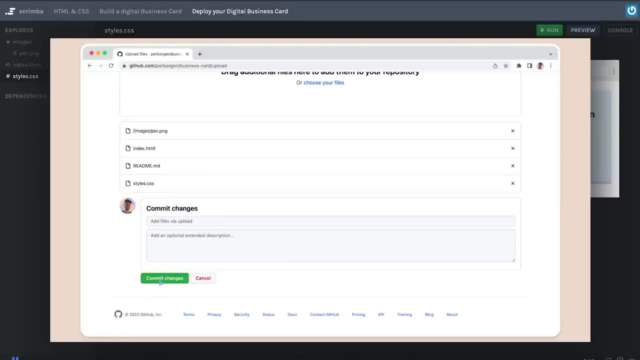 rectangle at GitHub. Once you've done that, you'll see all of your files listed. just scroll a little bit down. And then we have to do something called commit changes, which might seem a little bit weird And complicated, but don't worry about that. right now I'm just going to go with the recommended. 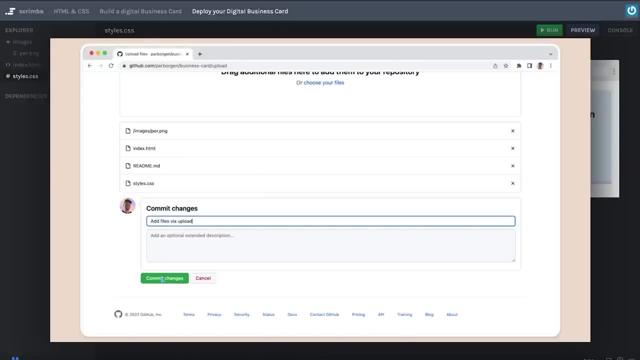 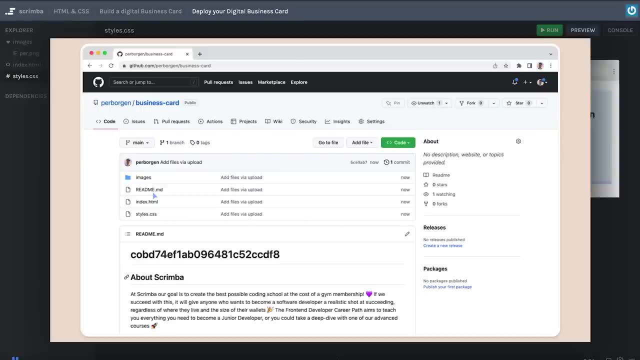 text: add files via upload and then hit commit changes. And boom, there we go. we have a repository on GitHub which includes all the code we need for our business card. Now, if you were to collaborate with other developers on this project, they would push their code. 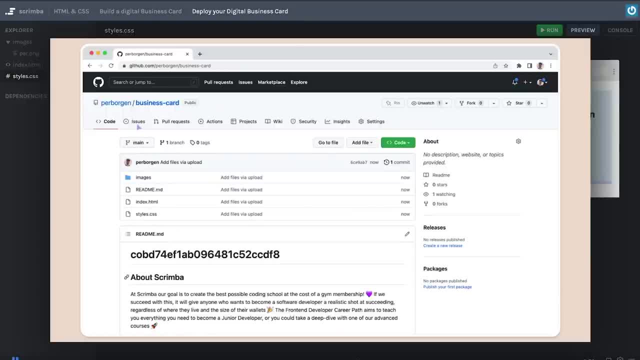 up to this specific repository And you would also probably create issues for tasks you want to do and work with something called pull requests, which is when you want to pull requests and then merge someone's changes into the code base, And there's also a ton. 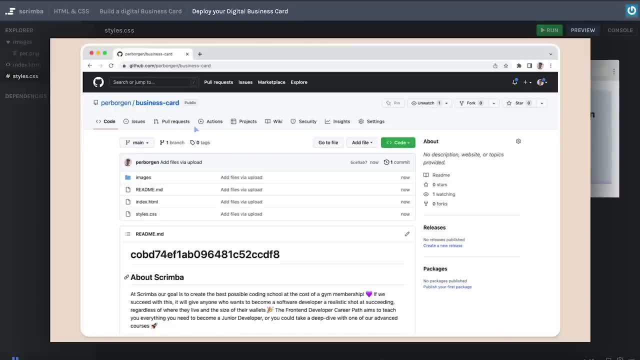 of other things you can do here, But we're not going to worry about any of that right now, Because the only thing we want to use this repository for right now is as an intermediate step before our deployment. So let's head over to Netlify and make sure you're logged. 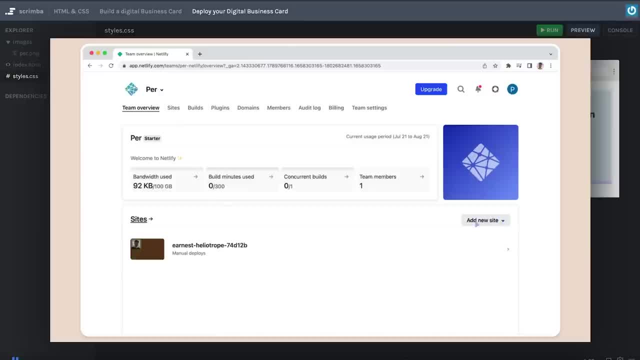 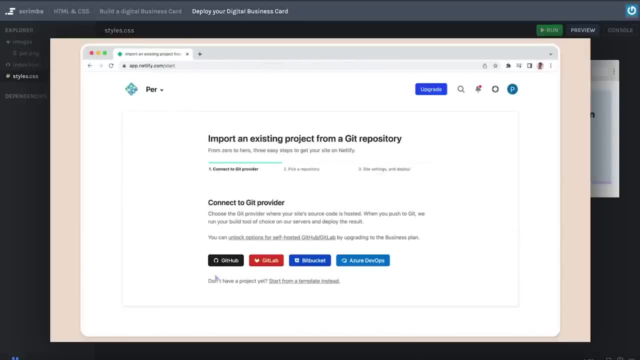 in so that you see the previous project we deployed, And right besides it you can see this button called Add new site. click on it and choose import an existing project. Here you're able to choose GitHub. click on that And it'll open this pop up menu where GitHub asks where you want to install Netlify, Because 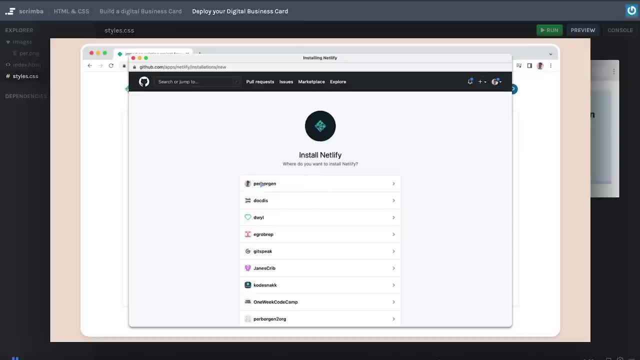 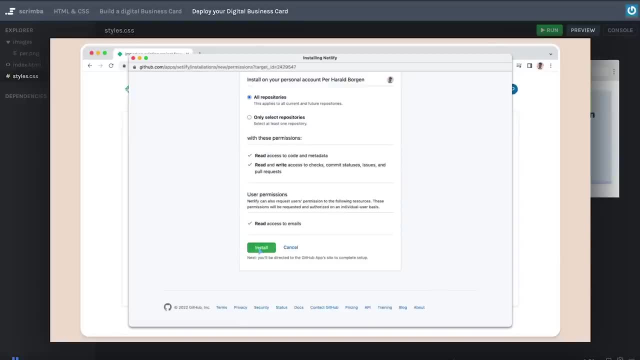 that's what you're doing. Now we're installing Netlify on our GitHub profile. click on your GitHub username, in my case Pierre Borgen, And here I'm just going to leave all the settings as they are. scroll down and hit install, And there we go. Now you can see. 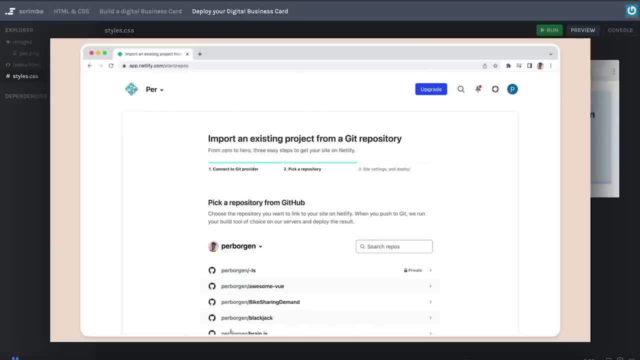 that Netlify has pulled in your GitHub profile and has your repositories listed. I have a bunch of repositories, So I'll have to search for the business card. I'll write the business and there we can see it. When I click on this repository it is imported into Netlify And here I can adjust some settings. but I'm 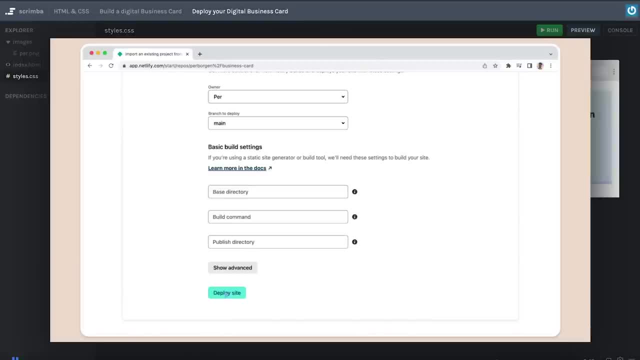 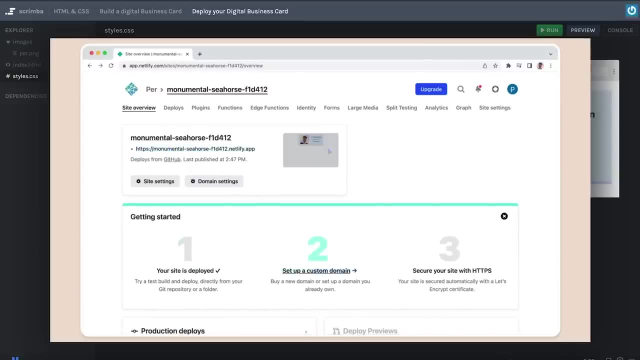 not going to do any of that. as usual, just scroll down to the bottom and hit deploy site, And there we go. The deployment is now in progress, So we'll have to wait a little bit And then, once this image turns into a screenshot of your site, it is deployed. So clicking 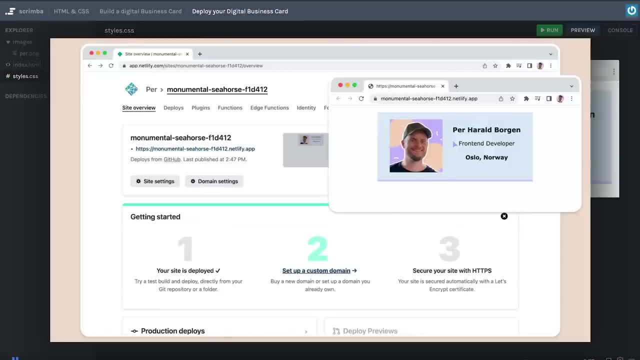 on this link will open up our business card. Really good job, though I hope your business card looks a lot cooler than this, As you were to personalize it in the previous scrim. actually, to prove to me that you add a personalized this, I want you to head over to Twitter and 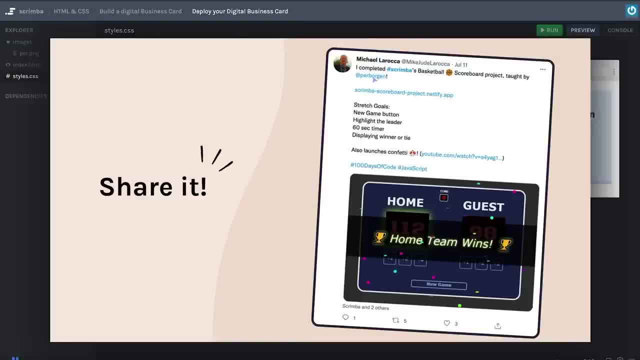 share your deployed business card. do as Michael Rocca does here And mention me if you want to, alongside a link to your project and perhaps even a screenshot of it. that would be super cool. So go ahead and do that right now, And then I'll see you in the next scrim. 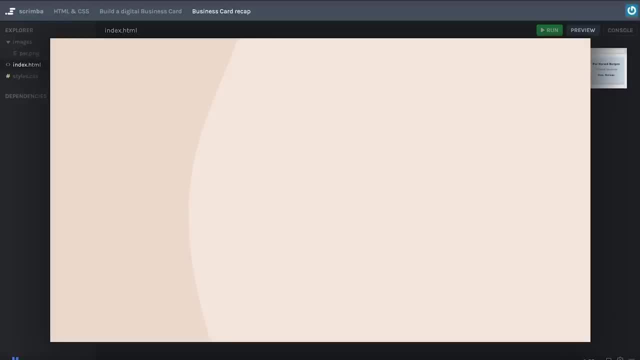 Woohoo, you've just completed the business card section of this course. That is very well done. Now let's go ahead and see what it looks like, Just like you saw in the previous done. Now let's have a little look at what you've learned. Starting out, you learned about: 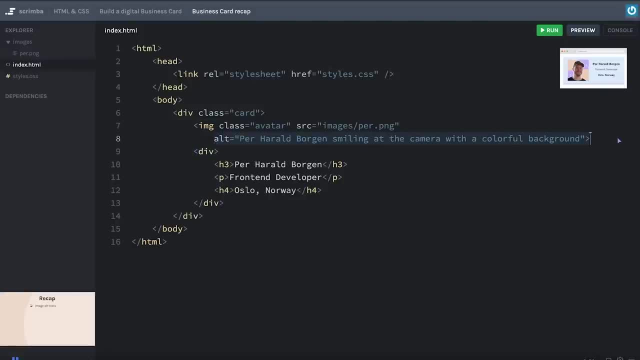 image alt text, which is a really important HTML attribute that makes your sites more accessible. Next up, you learned about flex child containers, which means that we took this flex box layout here, the card, and made sure that it only had two direct children. So that is one container and two. 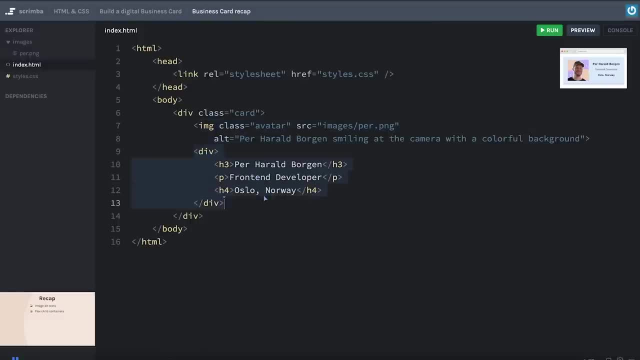 flex items so that these two stacked up besides each other on columns. However, we wanted the content inside of the second column to be on rows And for that reason we had to turn this flex child into a container in itself, so that these three could stack on top of each other. You also learned: 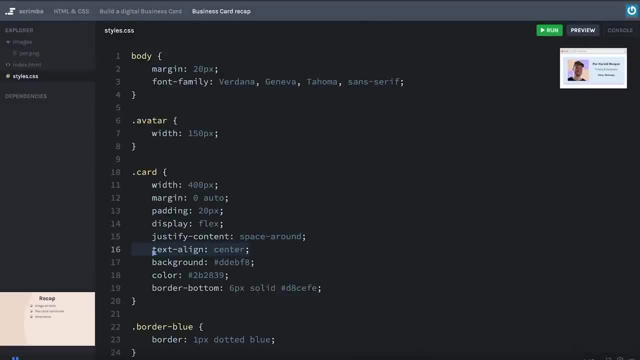 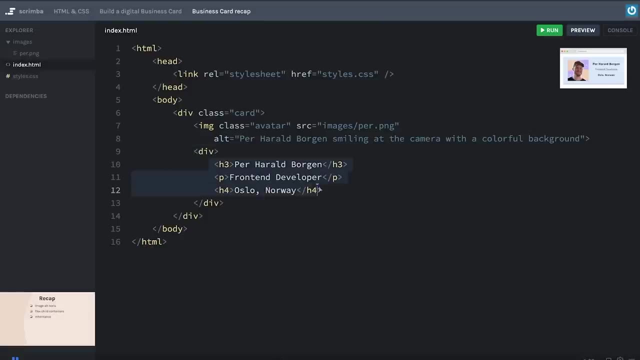 about inheritance, for example here with the card class, where we set the text line to center and that propagated all the way down from the card via the div and down to its grandchildren, the text elements that contain the data for the business card, And also you learned about shorthand. 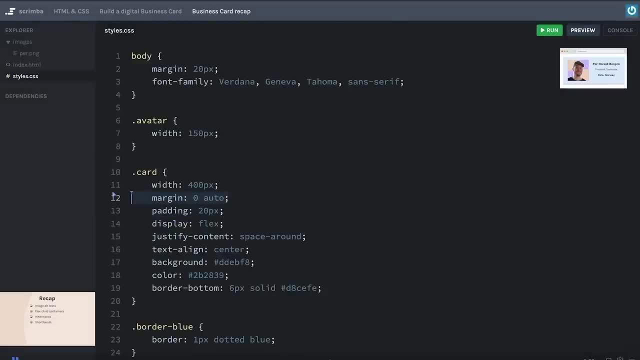 more specifically, the margin And padding shorthands, where we, instead of specifying each margin like the top, left, right and bottom, we just use shorthand zero auto to set zero on the top and bottom and then auto on the left and right. And then you learned about web safe fonts, which are these fonts that you can use? 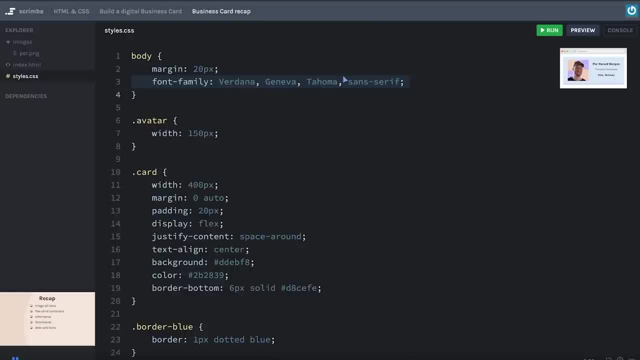 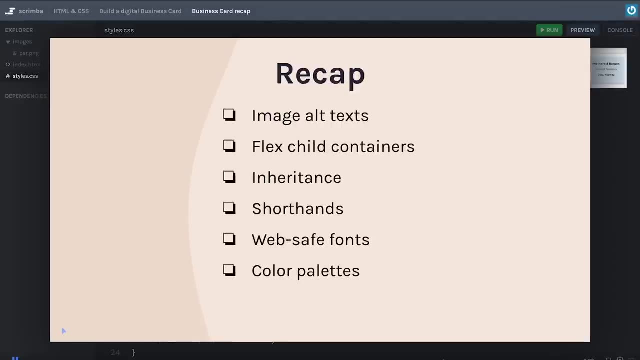 pretty much without worrying about whether or not they are installed on the user's computer, because in the overall majority of cases they actually are, so they are safe to use. And we took a look at color palettes, which is critical to know about, as colors often make or. 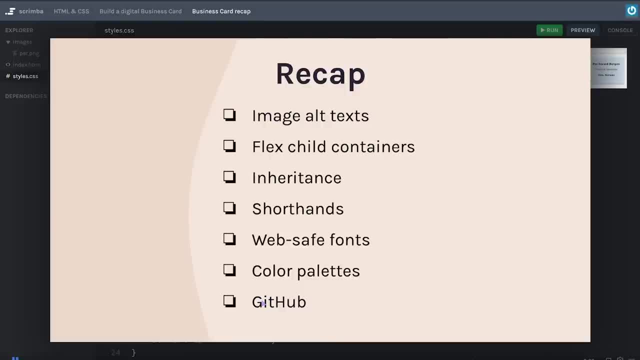 break. And then, finally, you learned about GitHub and how to create a repository for GitHub and use that as an intermediate step when getting your code from your local computer and up to the World Wide Web via a Netlify deployment. So this was a lot of things to learn. 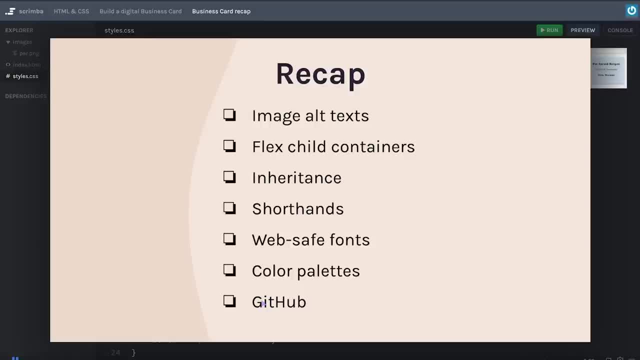 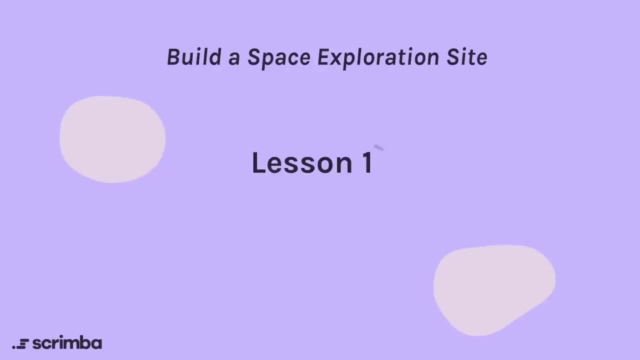 I can totally understand if you are a little bit overwhelmed. now take a little break and let these concepts mature in your mind, And then I will see you back here when you are ready to move on with the course. Welcome to this section, where you are going to. 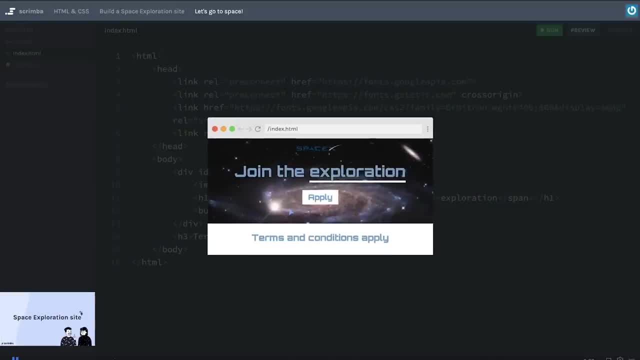 build a space exploration site. Here is the example you're going to build. As you can see, it has this super neat background image that animates and that really breathes life into the site. We're also using Google fonts to pull in this custom space ish font right here, And we're 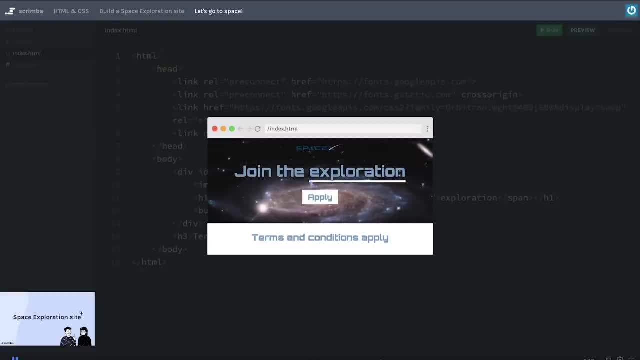 doing a lot of interesting things with some subtle text shadows. this underline and more So. there will be plenty of new things to learn, in addition to reinforcing HTML and CSS concepts you've previously learned. So that's a great lesson for you, And if you have any other questions, feel free to reach out to me on the 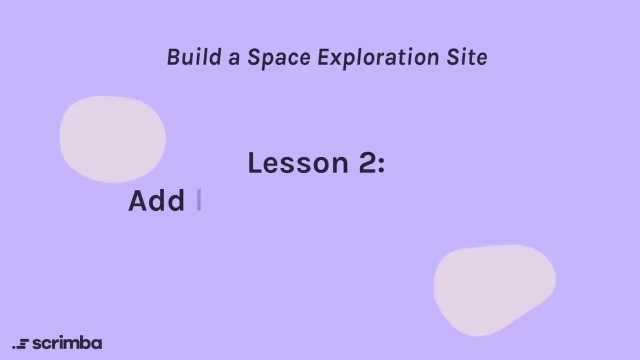 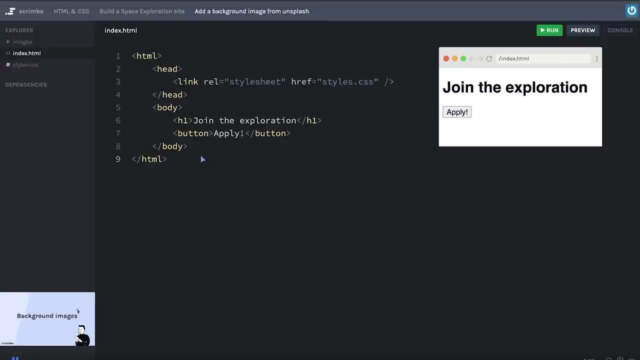 chat And I'll see you in the next one. I'll see you again in the next video. Bye for now, So let's launch into this section. Okay, let's get started building our space exploration site. As you can see, I've set up a basic HTML structure for you here. it is very simple. 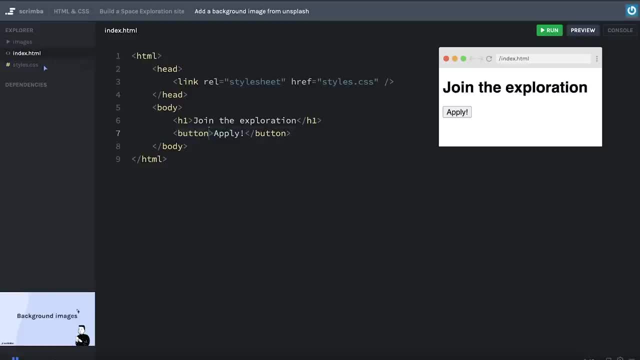 as the body simply contains an h1 title and a button. as for the CSS, there is no, as we are going to add that now. So the first thing we're going to do is fix the background here, because we don't want the white background. we want to have an image of the universe in. 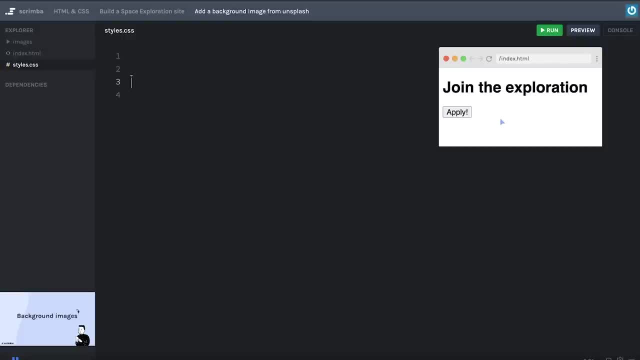 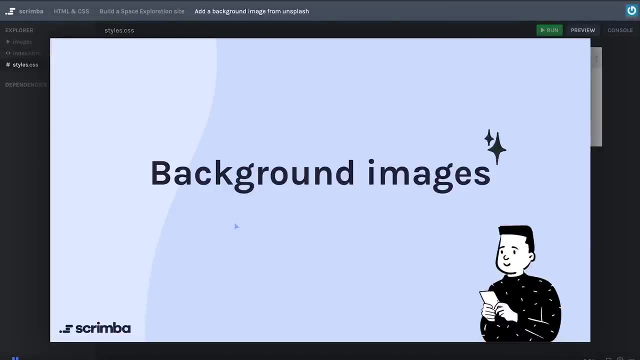 the background. Later down the line we're going to change that to an animated image so that it looks like a video playing in the background, which is even cooler. But as for now, we're just going to do a standard background image, as we're going to work on this for a 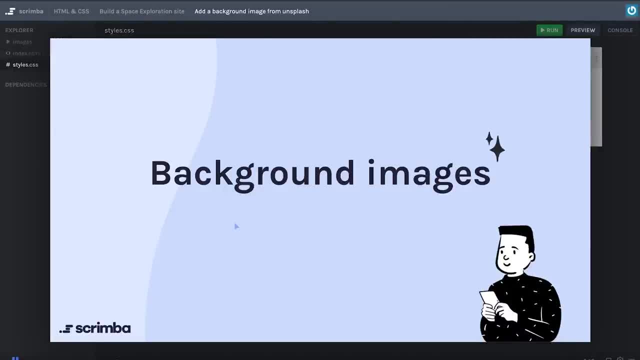 while, And I don't want to have an animated image looping in the background as we work, as I think that's a little bit annoying. So let's start out with just a static background image, And just so you know, background images is something different than how you've used. 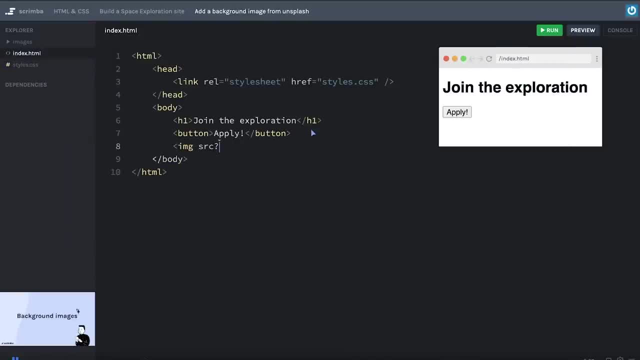 images up until now where you've done IMG, SRC, some kind of JPEG Like that, instead. background images are not in the HTML, they are added in the CSS file And I've talked about that. let's just find a cool background image and then deal. 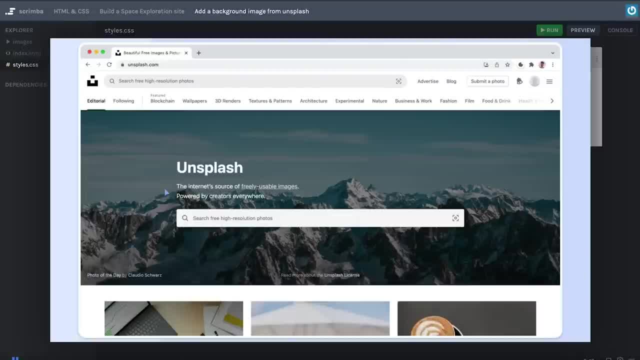 with how to implement it into our app, And the service I prefer to use for finding cool images for your web design is Unsplash, Because the quality of images here are really good, So they will take your web design to new heights And you can use them freely however you want. 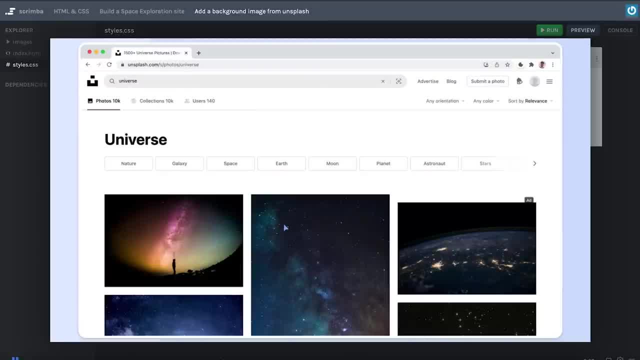 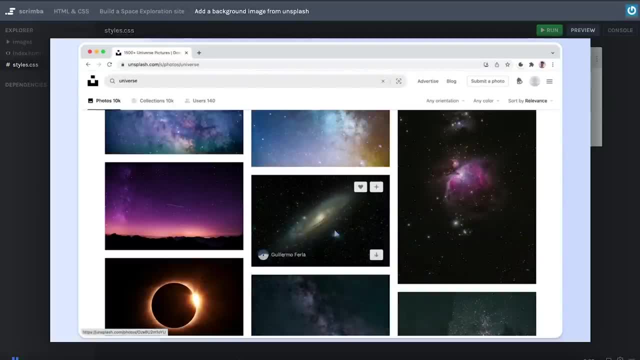 So if I search here for universe, we'll get a ton of nice images. Let's scroll a bit down, As you can see. there's plenty of good candidates here, But I think this one is particularly nice, So I'm going to. 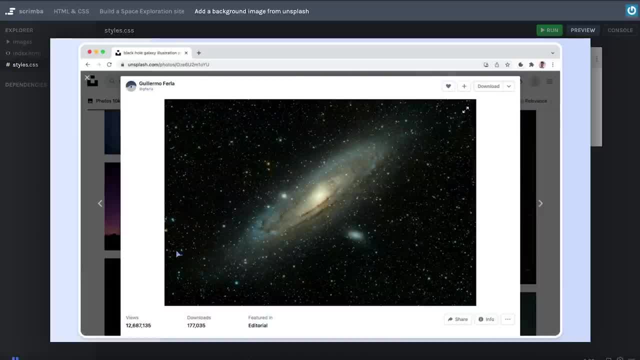 click in on it. it is created by Guillermo furla And you can see it's really popular, have over 12 million views already. Now, if we want to download this, you can click on the icon up here and download it- range of different sizes, And I've actually done that. 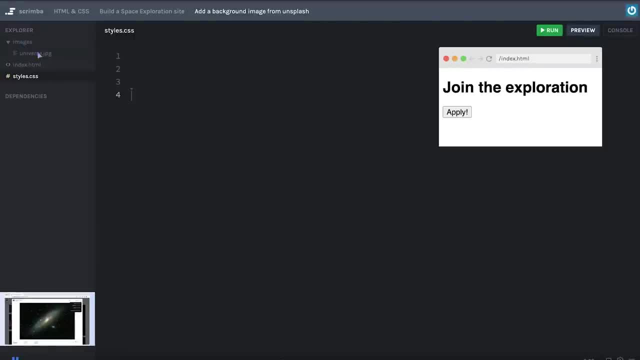 and placed it here in the images folder. So here you can see: universe dot jpg. So let's see how we can add this to our app. What I'm going to do is target the body, because we want the image to span across the entirety of our page, So we need to add the background image to the body. lose the background. 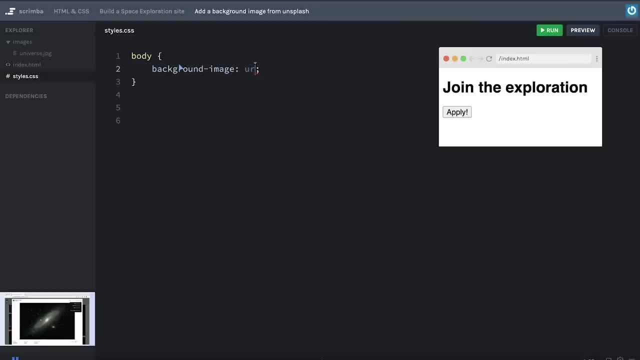 image property. Here we'll utilize something called a CSS function. Don't worry about why it's called a CSS function. Just remember that the way to do it is by writing URL open parentheses and then, inside of the parentheses, you refer to the image source, just as you. 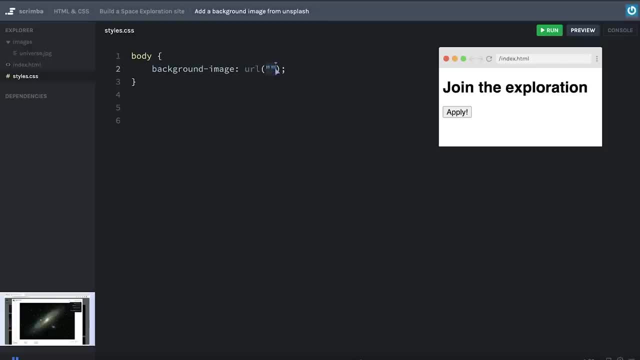 do in the image with the IMG. It is using quotes, So inside of the quotes we'll write the path to this exact image. And the way we do that is first by navigating to the images folder. So images, then the slash, going into the folder using the uni verse of JPEG and boom, there we go. Suddenly. 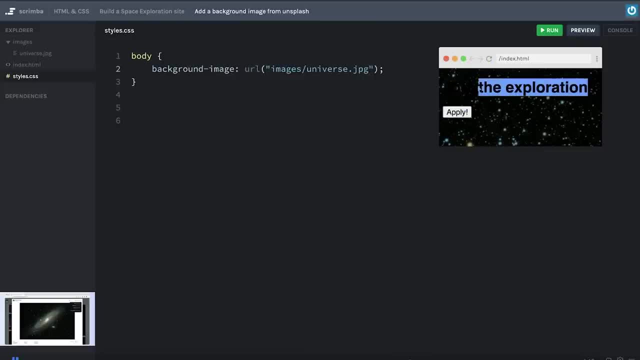 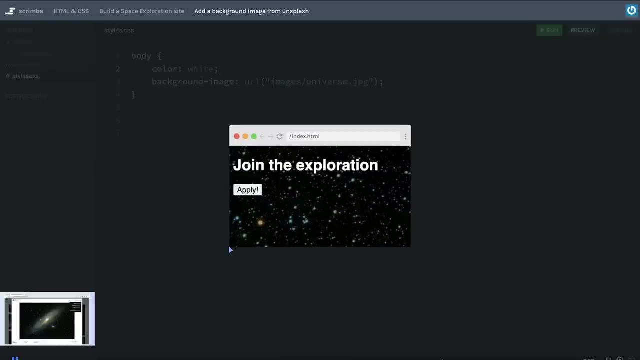 our background changed. However, there's a couple of problems here. Our h1 is now almost invisible, since, by default, the text is black and the background is very black as well, So I'm going to change the color To white. like that much better. Also, this image is 1000s of pixels wide, whereas our 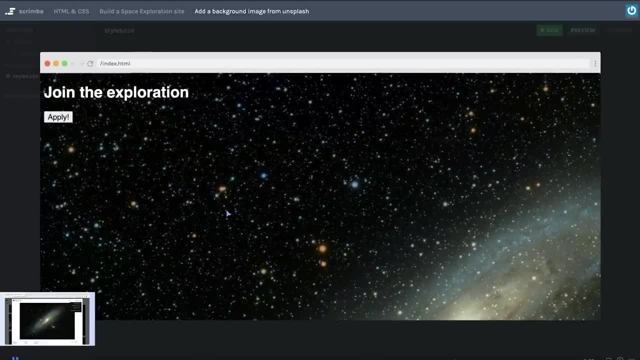 browser is not that wide, So notice that if we make it super wide, we still only see edge of the galaxy, more or less the center of the image. So what we need to do is shrink our browser down to like a couple of 100 pixels wide, which is what we want, And then make. 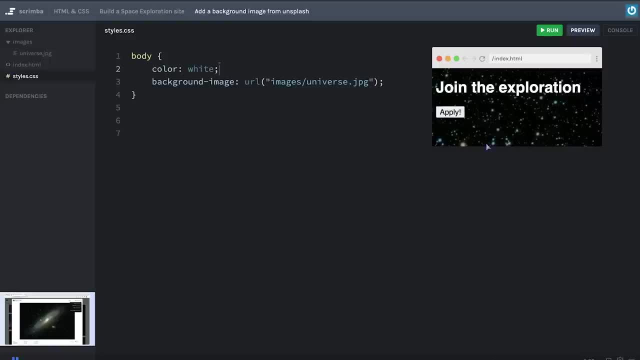 our background image shrink so that it's squeezed into the width of this browser, And if we do that, as background size and the value cover, boom. there we go. Now the width of the background image is exactly as the width of its container, which again is exactly. 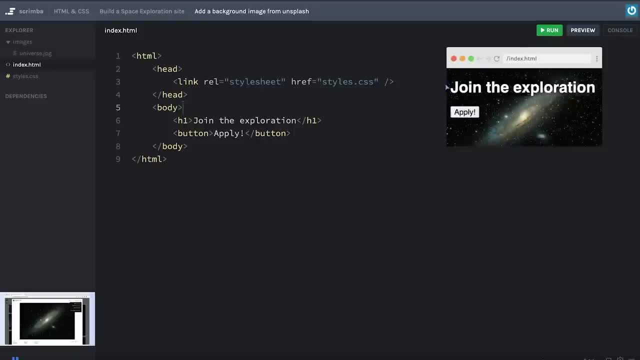 as wide as the browser itself, meaning that the browser and the background image has the exact same width, And that looks pretty good. I'm not going to give you a challenge on how to do this right now, as you'll get plenty of practice Using background images. you're. 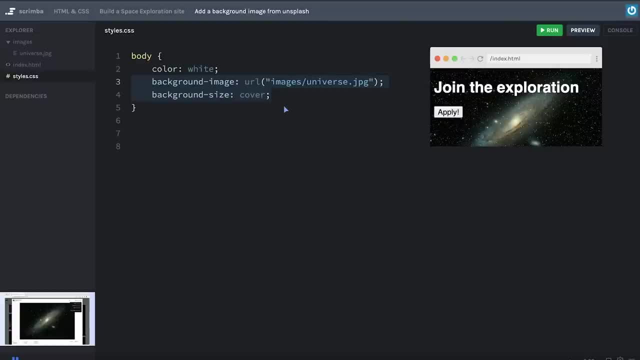 going to get a lot of practice using background images, So I'm going to give you a challenge on how to do this right now, as you'll get plenty of practice using background images later in this course. So with that, let's just move on to the next scrim. 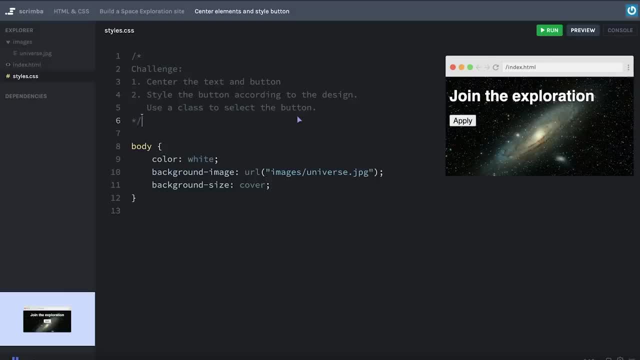 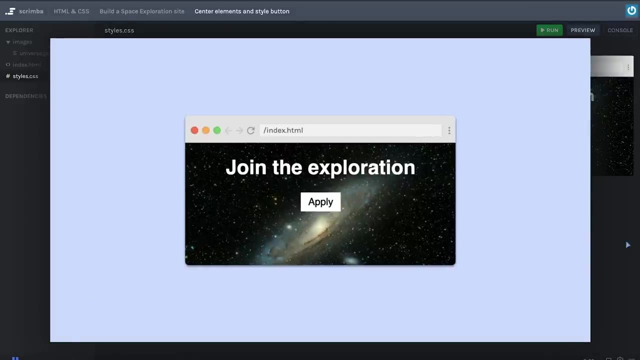 Okay, in this two part challenge, you're going to improve the design of our app. First, I want you to center the text and button and then style the button according to the provider design, And that is found here in the slide. As you can see, the button is slightly different. 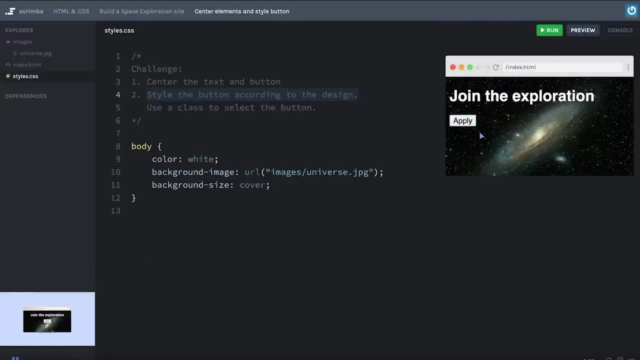 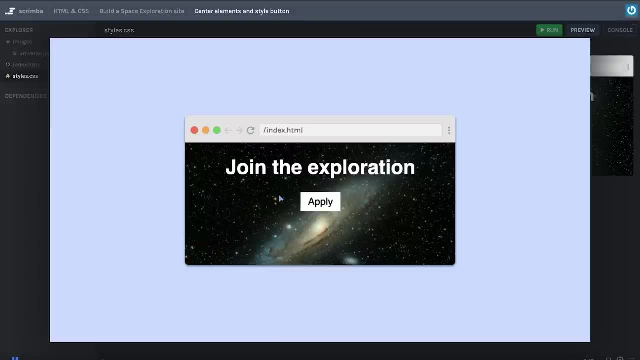 from how it is right now, Not too different, But certainly it has some CSS properties applied- And I'm not going to tell you which, because this is a good way for you to train your design eye. When you design the button, I want you to use a class in order to select it, So not. 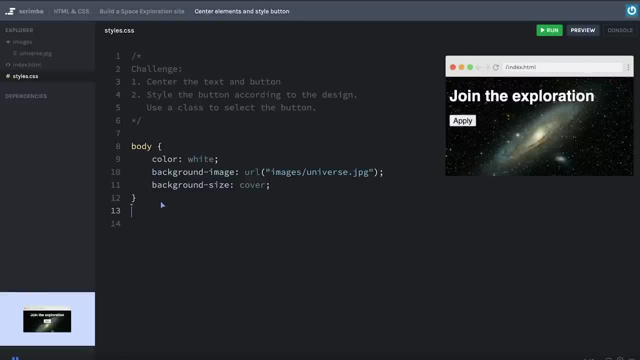 just using an element selector, like we do here. So go ahead and give this a shot, And then I will show you the solution as well when you return back to me. Okay, let's do this. First we got to center the text on the button, And here you can use. 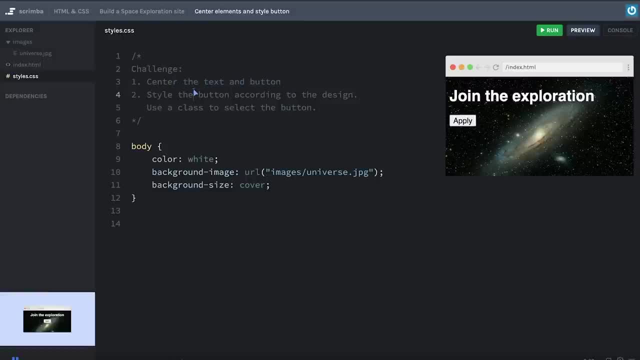 a range of different options. First, we're going to create a new class called class options, either using margins or flex box or text align. you've learned plenty of ways to center elements. Now I'm going to choose the easiest one, which is to apply a text. 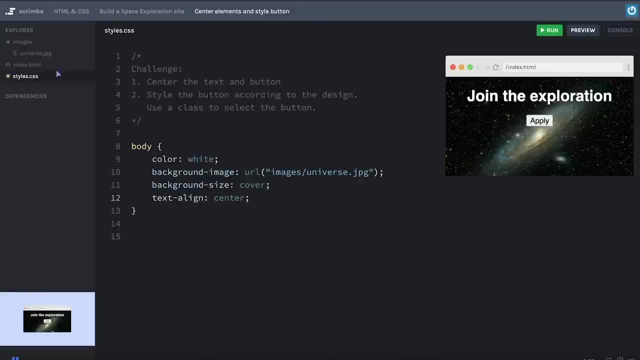 align center in the body element because, as you know, this centers not only the h1, but also buttons. Okay, with that out of the way, let's move on to the button. First, I want to give it a class, And I think BTM is a good class name, So let's add it to the 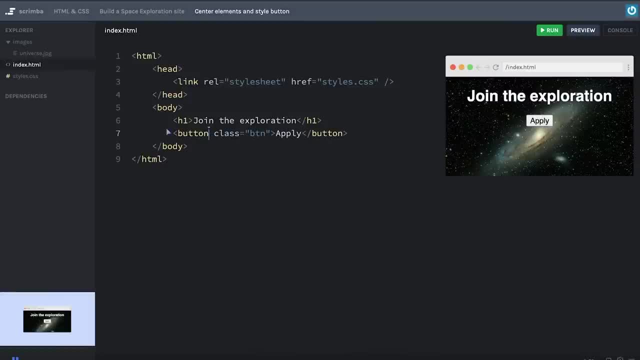 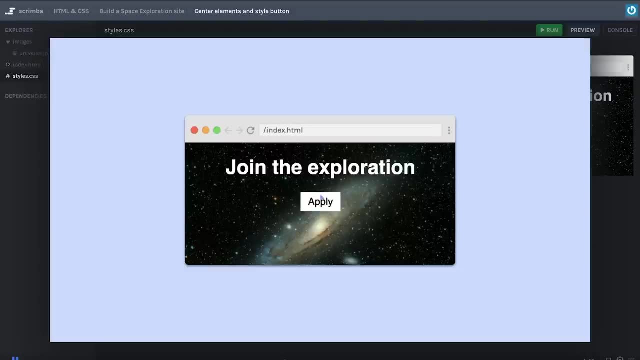 HTML as well, like that and run the code. So we have it applied in the DOM. Now let's have a look at this design. The first thing that is apparent to me is that this button has more space around the text. as you can see here, it's a bit more crammed, So that 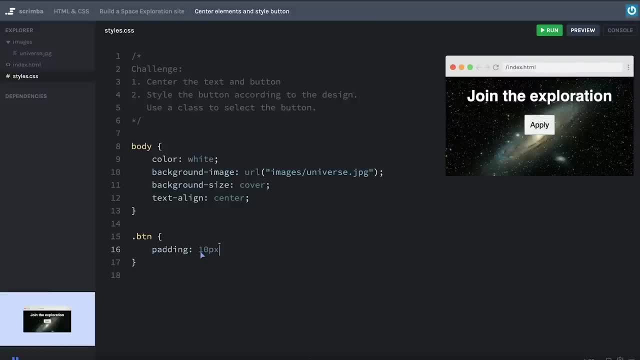 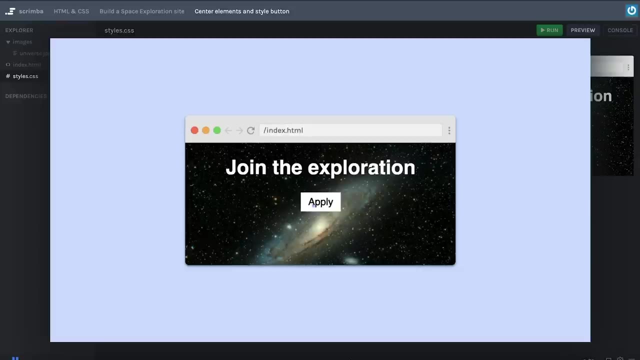 is the padding property. Let's write 10 pixels just on all four sides of the padding. Having a look at this button right now, you can see that this one is a bit more rectangular versus this. one is a bit more squared now because in this design here there's more. 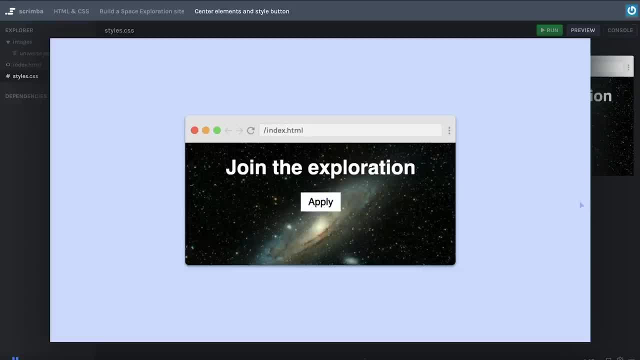 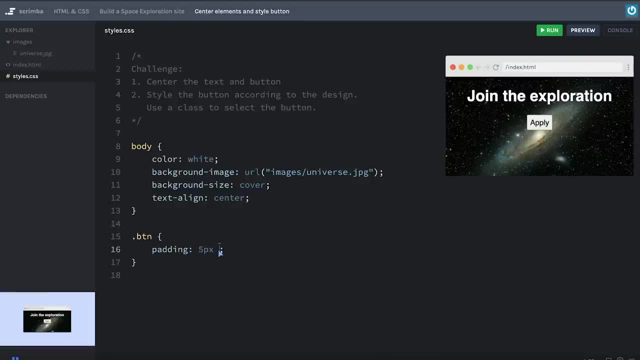 space on the left and right hand side than the top and bottom, And if you remember the short time, we can do this by, for example, starting with five pixels on the top and bottom and 10 pixels on the left and right, And that looks much better. Maybe it's a little bit. 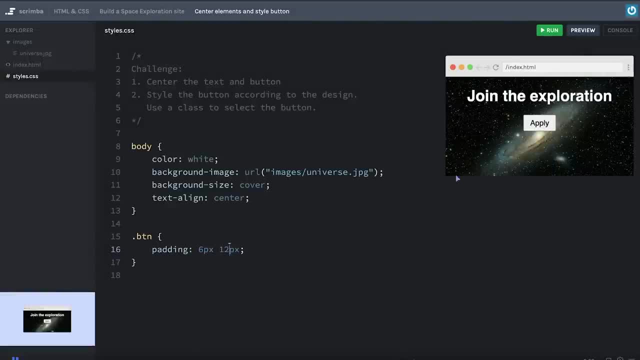 higher, So let's do six and 12.. That looks pretty good to me. Now let's go to the next one. And this one is a little bit more complicated, So let's go to the next one. And this one is a little bit more complicated, So let's go to the next. 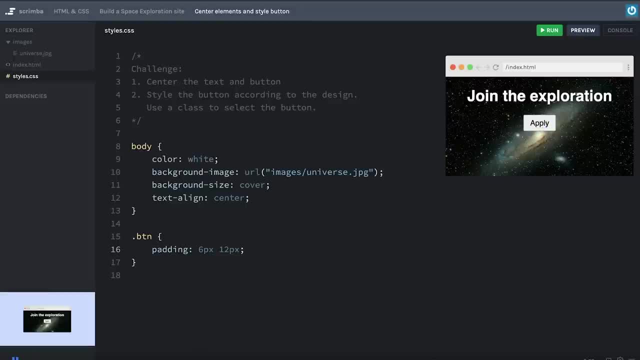 one, And this one is a little bit more complicated. So let's go to the next one, And this one has a white background color. Now, the next thing I want to change is the background color. It's not totally apparent, but actually this one has a white background color, whereas 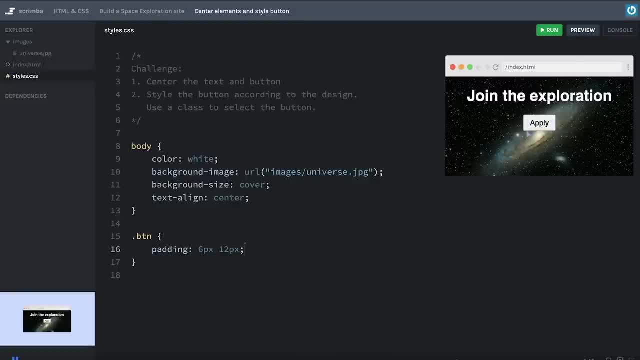 this one has the default button background color, which is a bit grayer. It's not that easy to see because of the background. here it looks pretty white compared to the black background, But it is actually not entirely white, something you'd know if you worked. 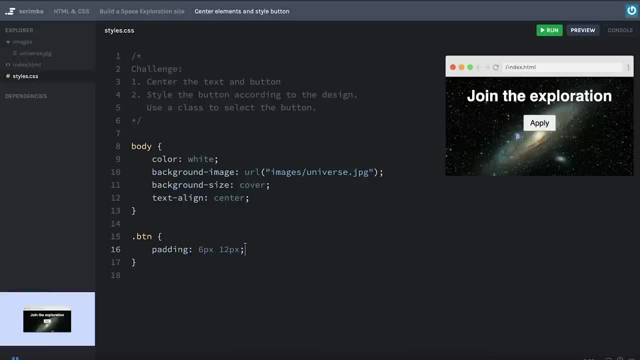 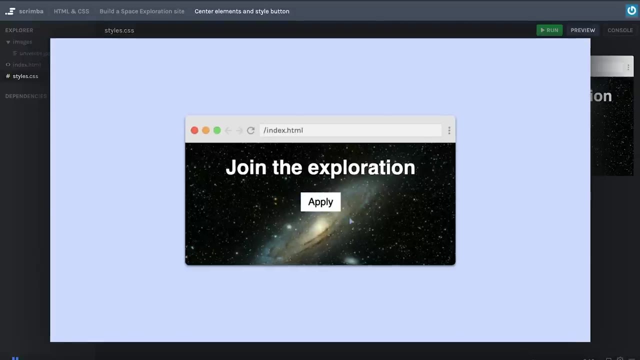 with buttons in HTML for a while, as they always have a default gray ish background color background: white, So like that. Okay, now it suddenly became apparent that it also has a border in this default styling First. that's not the case in our provided design, So let's do border we can. 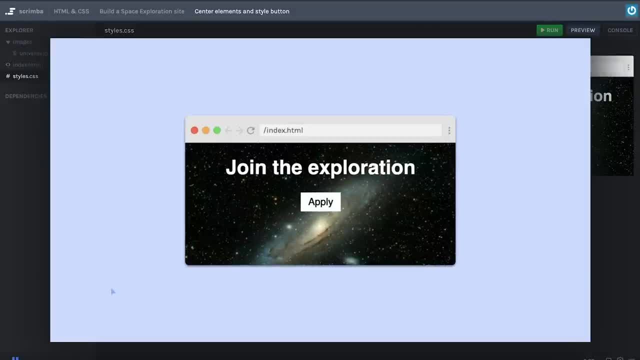 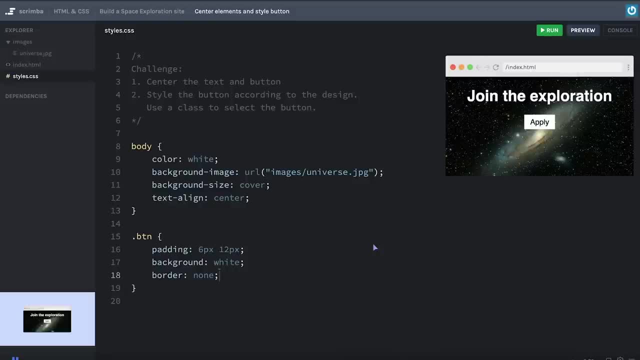 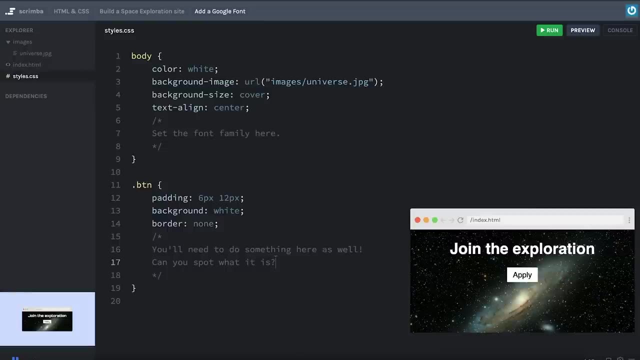 do none like that, And with that, it looks like we have completed our design, as these two look identical as far as I can see. So really good job, Let's move on. Okay, now you're going to get a new superpower in your tool belt called Google fonts, And that is. 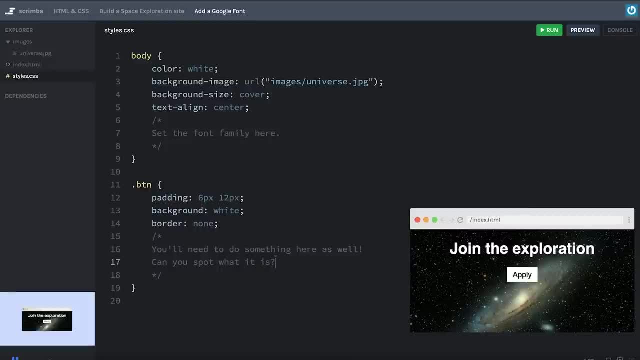 a service that gives you access to over 1000 different high quality fonts that you can use in your projects, And the reason you need to learn about this now is because the font we have here isn't good enough. In my opinion. it is a little bit boring for a space project. 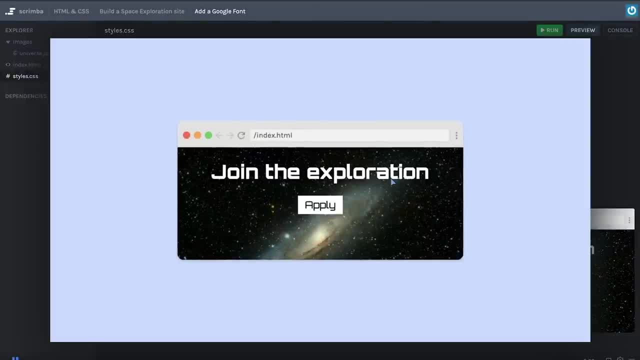 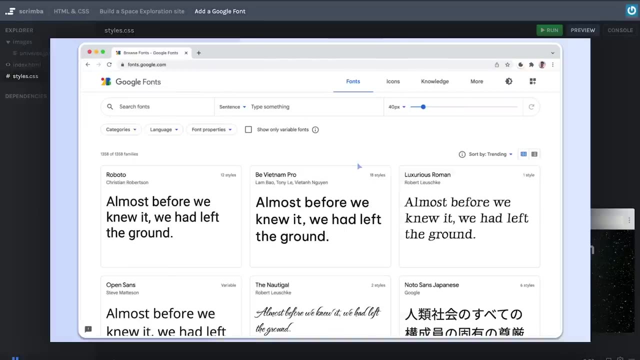 What we want instead is something like this, which looks a lot more sci fi ish. However, this font isn't one of the so called web safe fonts- You'll learn about earlier- which is already installed in most operating systems. This is a very custom font, So we have to use Google fonts in order to bring it into our project. 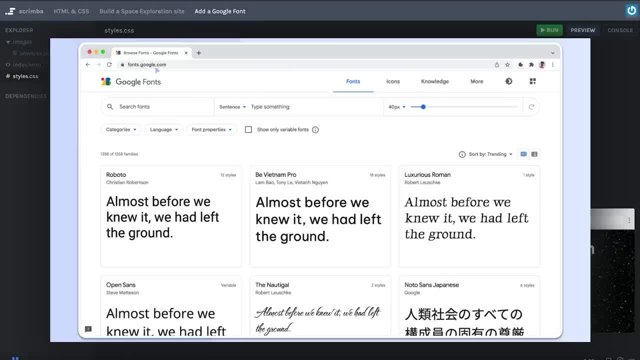 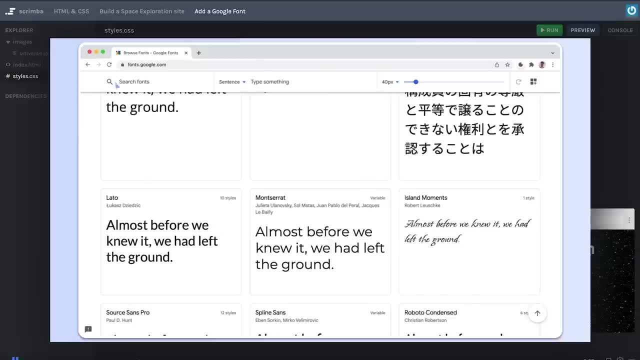 And here you can see the Google fonts interface. it's located at fontsgooglecom And if we scroll a bit down you can see it contains a range of very different fonts. Now it has a search feature up in the top left corner, but it's actually not that good, To be honest. 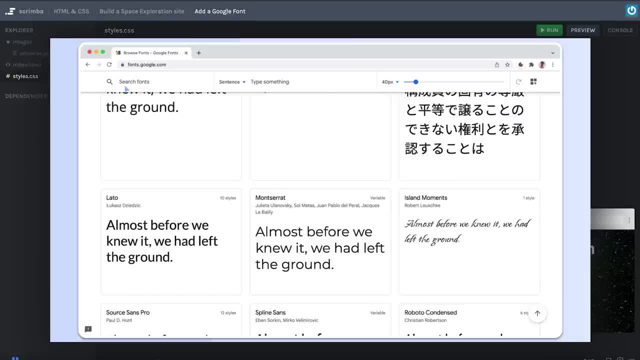 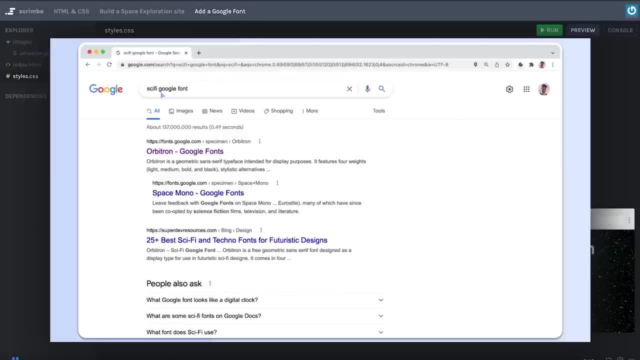 it's better to just use regular Google search when searching for Google fonts, So let's do that instead. The way I found the font we're going to use now is just by googling sci fi and then Google fonts, And then Google suggested this Orbitron font. So 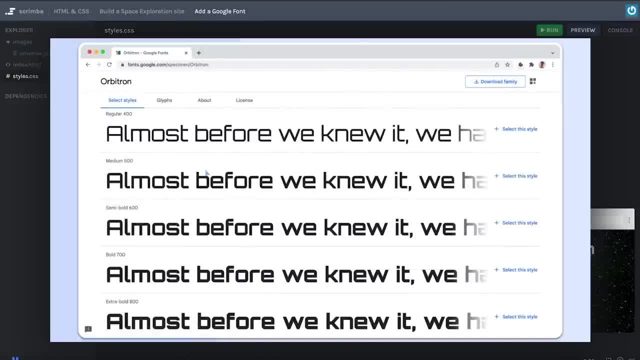 if we click into it you can see here it is. If we scroll a bit down you can see we have to choose specifically which styles we want. So I'm going to choose this 400 regular style by clicking on select this style like that And you can see the panel on the right hand. 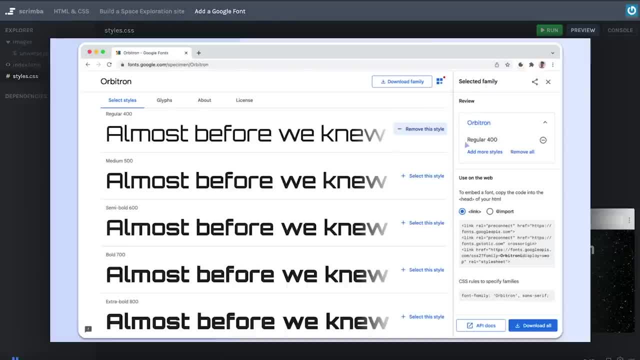 side, And it is clear that we have chosen the Orbitron font and the regular 400 font weight. Also, let's click on this extra bold in case we want to bold some text on our site, And there we have that one as well. Now, if we want. 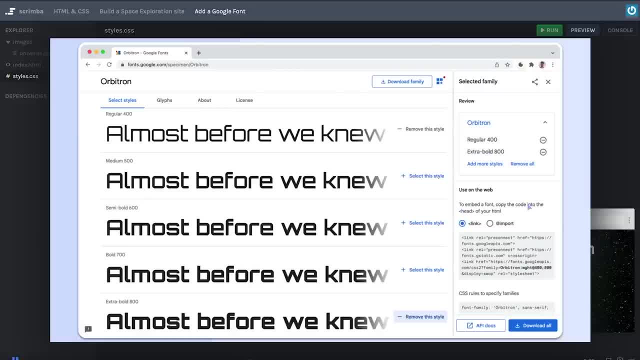 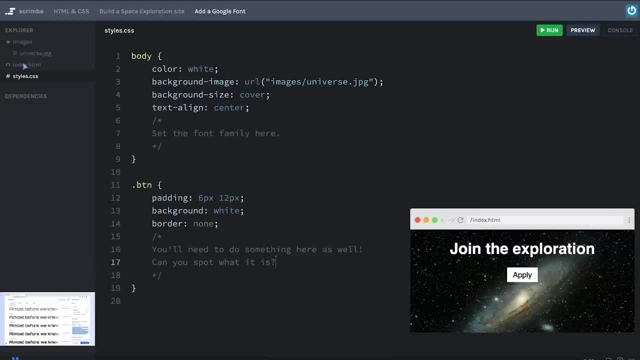 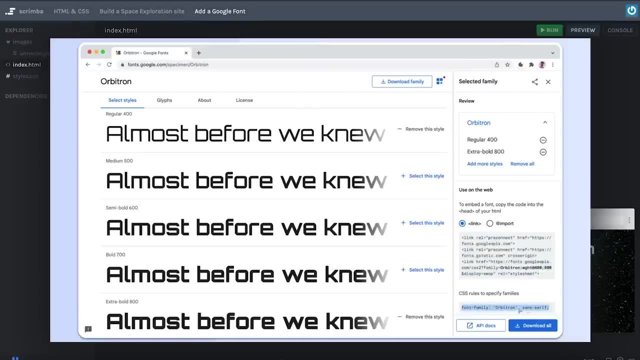 to use this on the web. we can embed it by simply copying a piece of code into the head of our HTML- And that is the code you want to copy- and then paste it in exactly here. Next up, we also have to specify it in our CSS, And that's done by pasting this line: 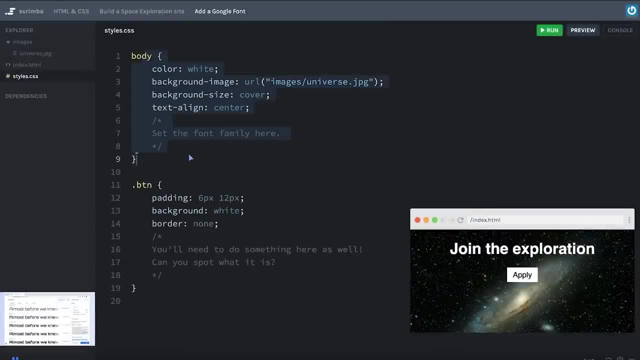 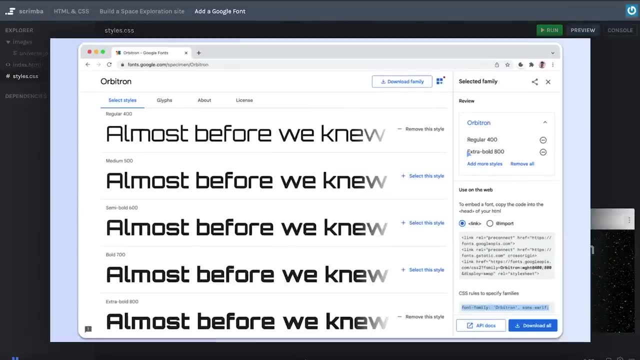 into our CSS, for example, in the body tag. I'm not going to do this for you, though. scrim bar is all about you doing things on your own getting your hands on the keyboard, So now I want you to head over to Google fonts, fetch the Orbitron font in these two styles and 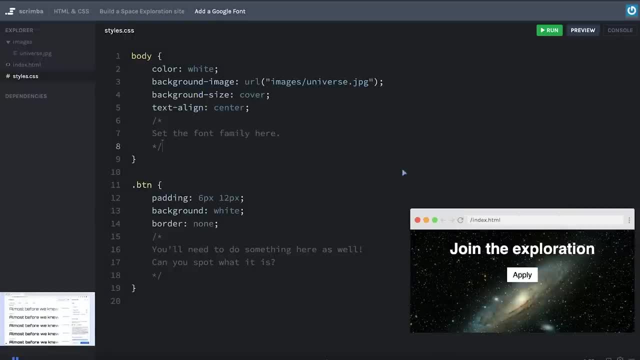 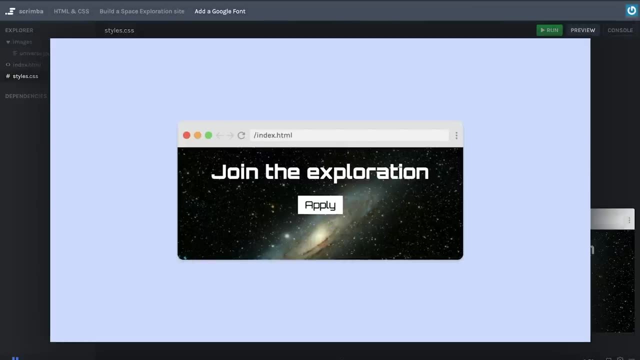 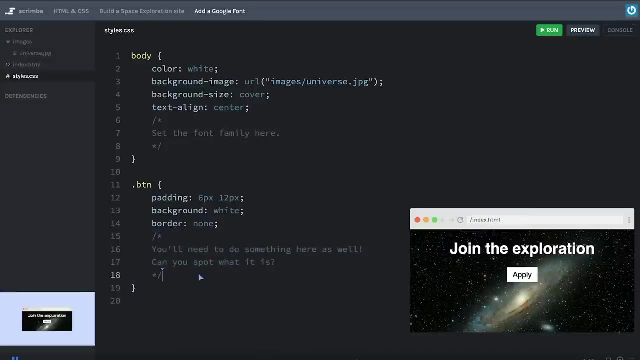 then do whatever you need to do in order to make the Orbitron font render properly on our site. I'm going to leave you here with this screenshot, because make sure to compare this design with what you get in the mini browser, Because there might be something you need to do down in the BTN selector And hopefully, 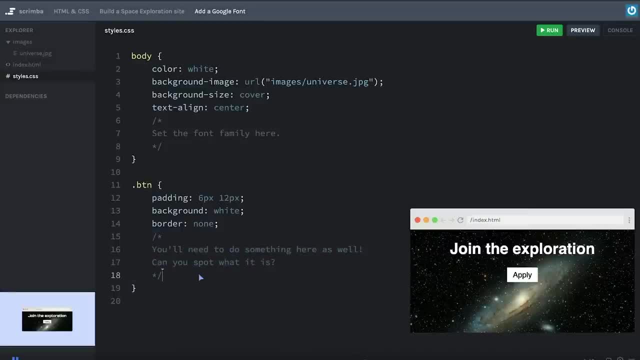 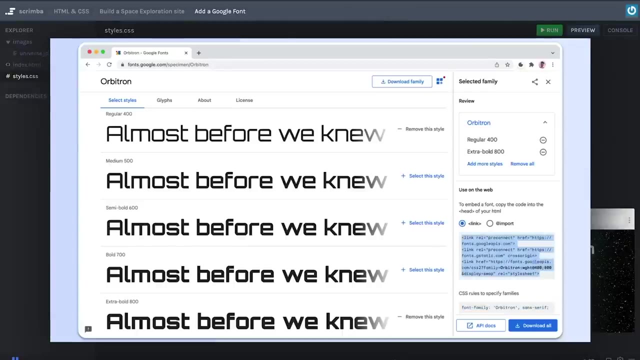 you're able to spot that. If not, no worries, because I'll be here showing you the solution when you return back to me. Good luck, Okay, let's do this. So first we're gonna take this snippet of code right here and then paste it into our HTML like that. then need to run the code so that it is implemented. Okay, we're done, Let's get started. And here we're going to run the code, And if you're interested in this search, you can do the following here. So this is our code, it's our HTML Hunters, And then you can see that this 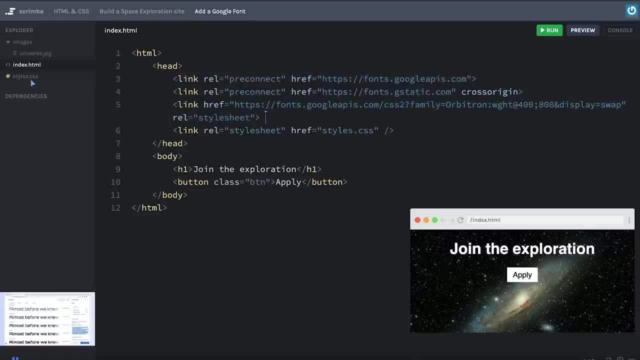 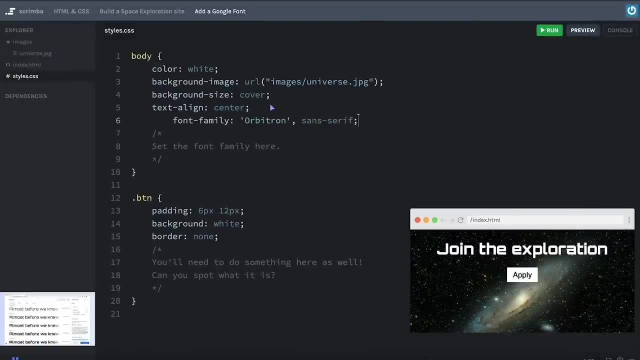 will be installed. I've added all of my links here. We're going to go here and then do this. We're going to so that it is imported into our project And then next up it is the styles which we're going to set here. let's copy that line of code and then simply paste it in right here. 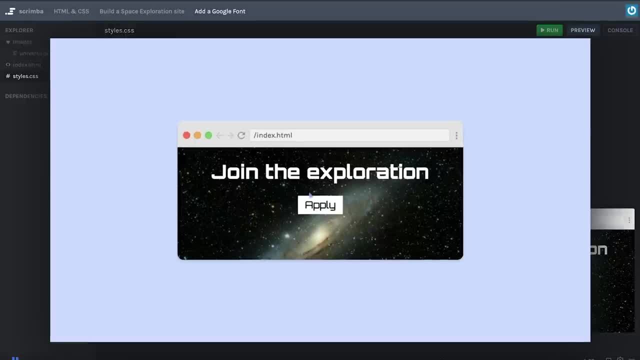 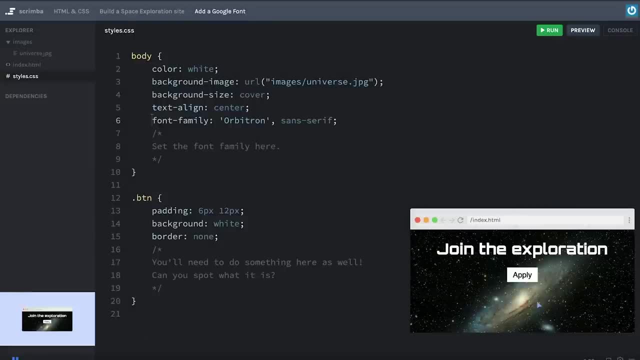 And boom during the exploration now looks like our project right here. However, this one also has the orbitron font applied to the button, But we don't have that. we still use that boring old font that we had previously. Why is that? Well, that's actually because 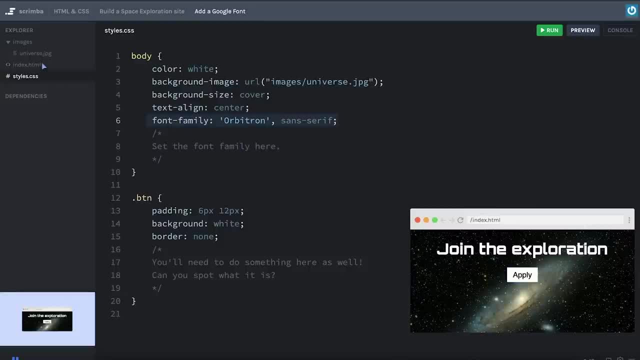 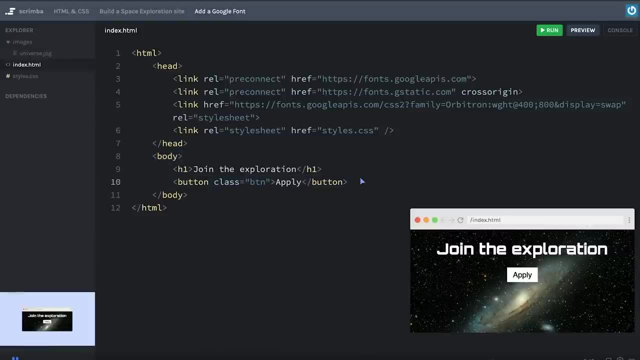 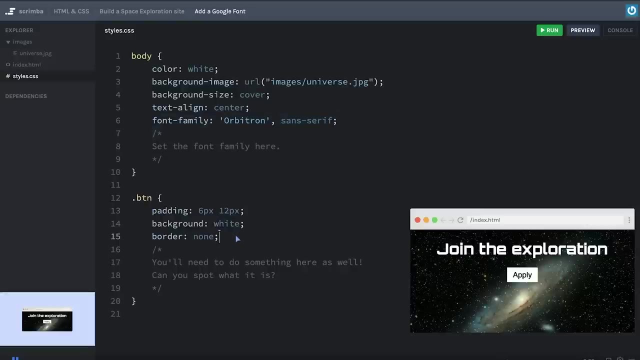 buttons don't inherit font families. So here the H one has inherited the font property from body, but the button has not. So what we need to do here is specifically tell the button to have this font family, And we can do that in two ways. One way is through using 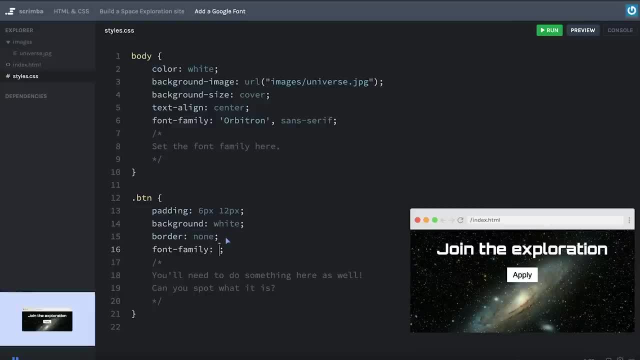 a CSS value you haven't learned yet, and that is the inherit keyword. As you can see now, it does inherit from the body, but only because we've specifically told the button to do exactly that- What I'm assuming you did instead, which works. 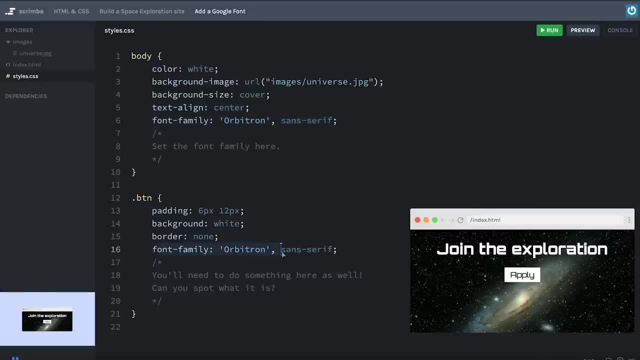 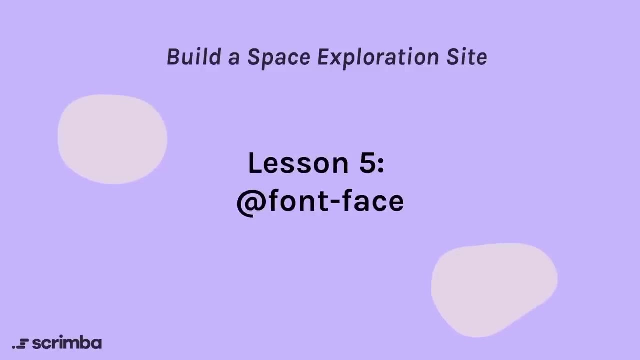 perfectly fine, as well as simply to paste in the font: family orbitron on the BTN class. As you can see, that also works well, So hopefully you were able to spot this. If not, no worries, It was just a little gotcha I left here. Let's move on to the next scrim. Before we move, 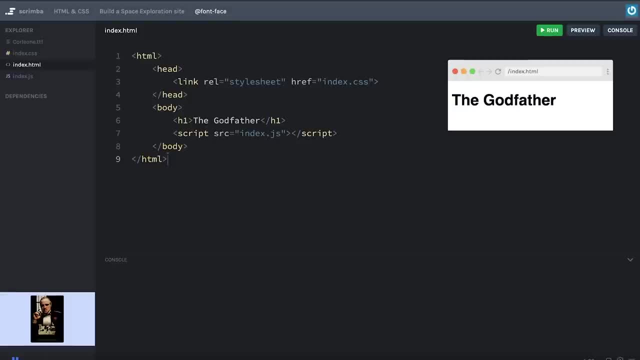 on from the subject of fonts, there's one more technique I want to teach you, Because in some cases, Google Fonts might actually not be enough, And that's typically the case if you want very specific fonts. For example, let's say that you are building a Godfather website in honor of the 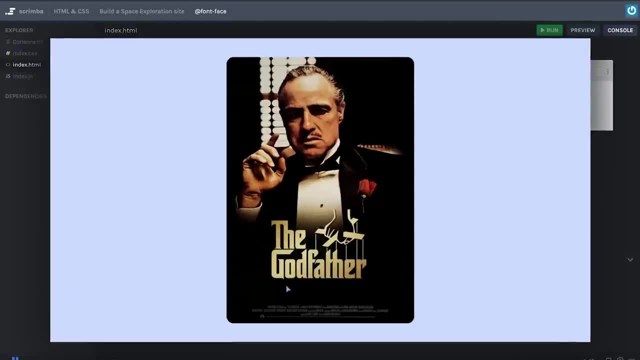 classic film. Well, in that case, you'd probably want to get a hold of the real Godfather font, though Google Fonts doesn't host that one because it is simply too specific for them to care about, So you'd most likely have to find this font somewhere on the World Wide. 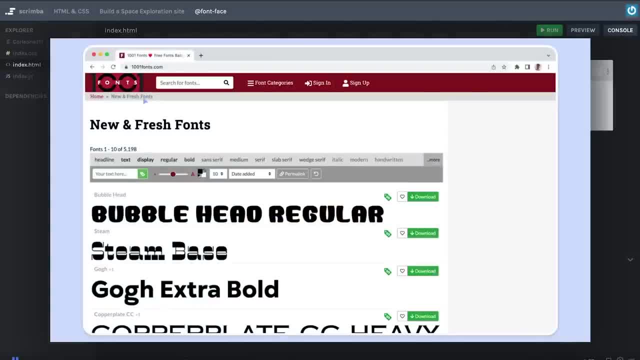 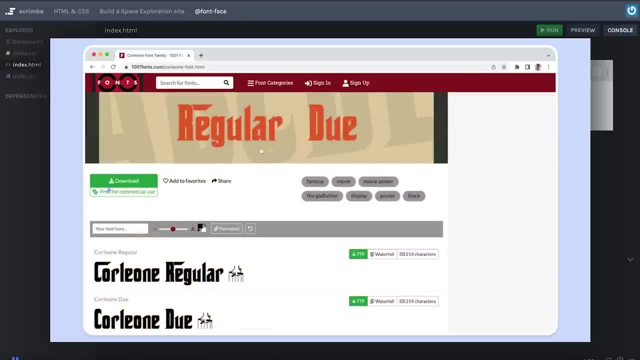 Web And there are great services. for this example, a thousand and one fontscom And there if you search for Godfather, they actually have it, So you can click into it, scroll a little bit down and click download. So what you then did is kind of downloaded the recipe. 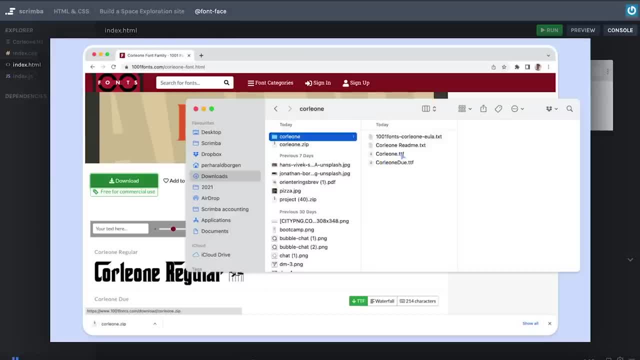 for the font, And if you open up the folder you got, you'll see a TTF file. that's a file format for fonts. what you then can do is simply drag and drop that file into your file system, like I have done right here. you can see I have the Corleone dot TTF file Now. 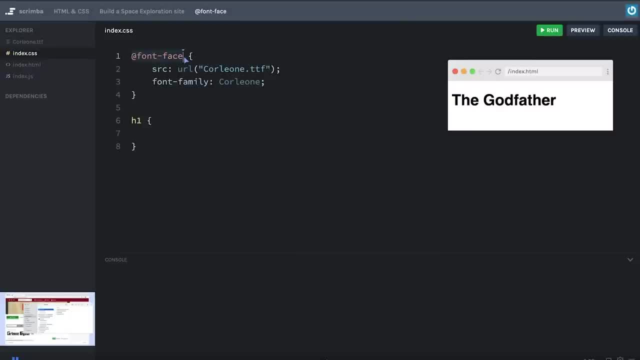 what I can do is use the add font face rule in CSS, So simply writing an app and then font dash face, and then open up the curly brackets and write two properties: the source, which should use the URL technique pointing to the TTF file, which I'm doing right here, And also I need to tell CSS what name I want. 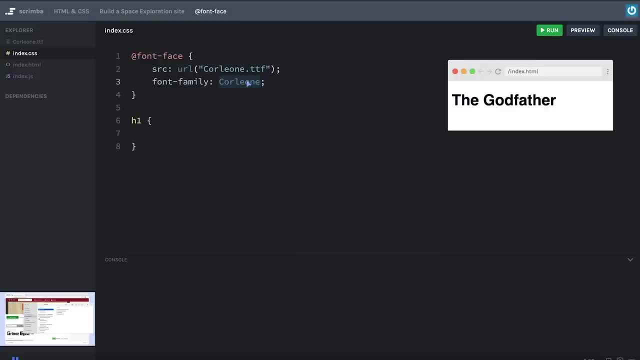 to give this font in my style sheets And I'm just going to choose Corleone for now, but I could have chosen whatever name I wanted. Now I'm able to target the h1 and use this font family, So I'll do font family. 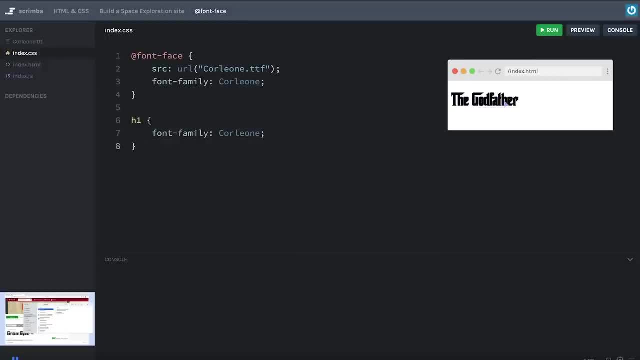 Corleone. And there you can see, I have the godfather font, So I'm off to a great start on my tribute page. So now what I think you should do is actually try and do this yourself. find a random font online, download it so that you get a hold of the TTF file drag. 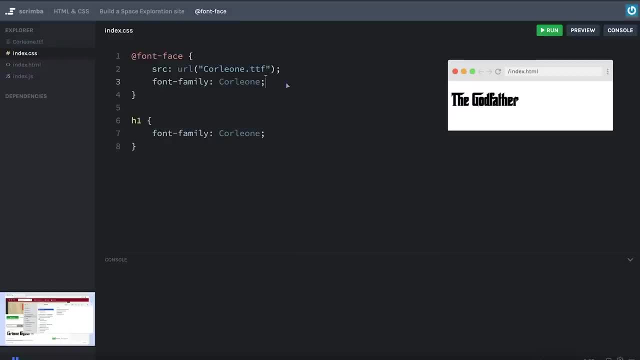 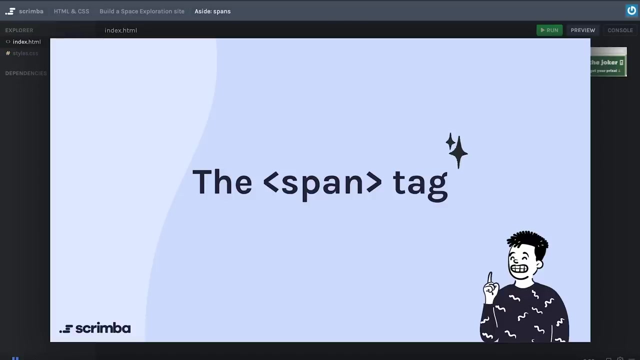 and drop that TTF file into the file system here on scrim bar and use the add font face property to make that font available in your style sheets. Once you've done that, I will see you in the next scrim. Now learn about the span tag, because in the next scrim you are going to create an underline. 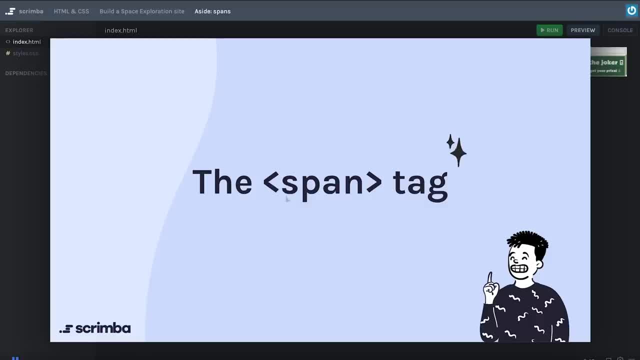 under the exploration word, And in order to achieve that, you need the span tag. So let's take a little step back from our space exploration site and learn all about this awesome tag. The example we're going to use in order to learn the span tag is of banner ads. You've 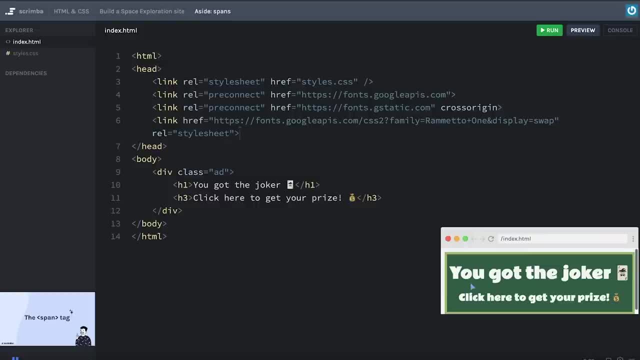 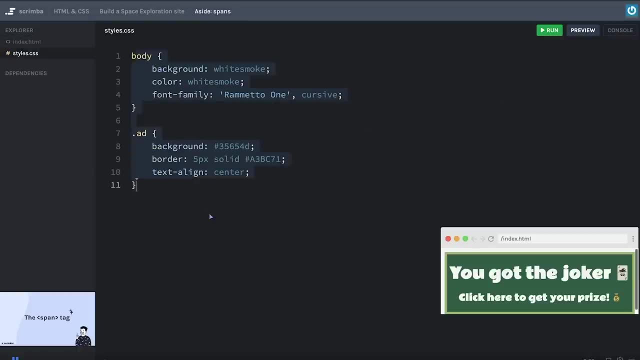 probably seen these before. you've browsed the web, for example, on new sites, And many of these are actually so called HTML five ads work. they're built using HTML and CSS And it's actually a little bit sad how many clever developers in this world who are spending. 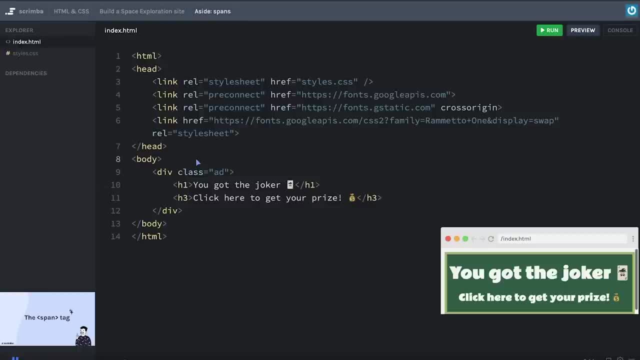 all of their time and their best years and getting more people to click on these ads through making them more invasive, more eye catching and more targeted. But that's the name of the game, So we just have to accept it, And you are now going to do exactly that. 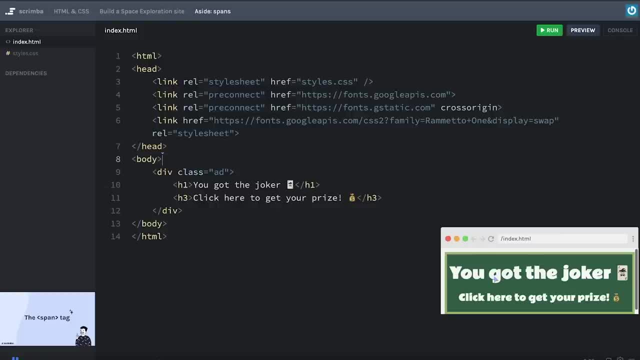 you are going to make this ad more eye catching, So that's hopefully more people are going to click on it and visit our scammy casino. So how do we do this? Well, looking at the HTML, you can see the div wrapper has a class of add which sets the background color border. 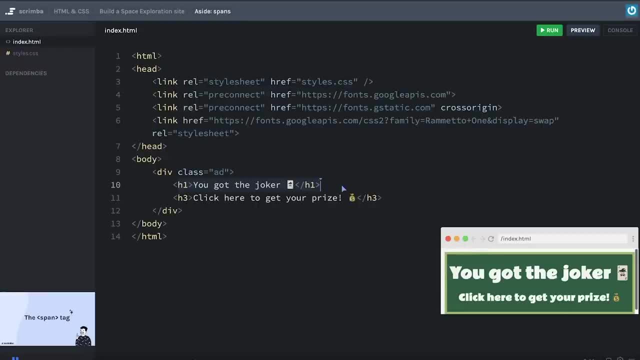 and the text alignment inside of this green rectangle. And there are two elements inside of the ad, that is, the h1 and the h3. And it says: click here. So what we want to do is make this hair word pop out more. So how do we do that we can't target the h3 itself? 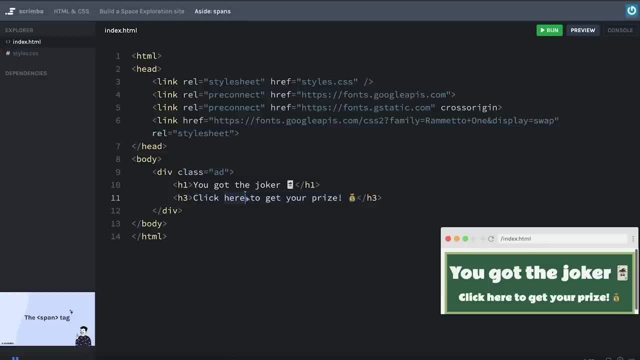 because that'll style the entire sentence. we only want to style this word, And this is where spans come in. Here we can write span like that, open the tag before the word and close it directly afterward. If we now run this code, seemingly nothing has happened because spans are invisible. 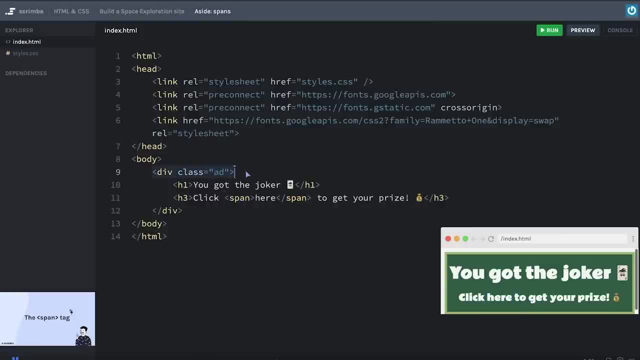 unless you give them styling. So they're kind of like the div, as divs neither provide any styling, unless you give it to it specifically, Although the difference is that spans are in line whereas divs are block based. So to demonstrate that, if we change this to div, what would happen to run the code? 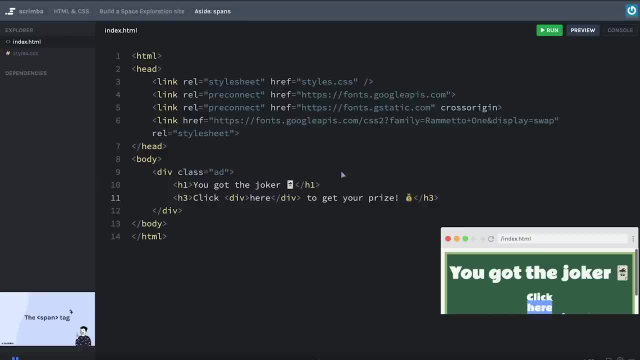 is that it would break the hair word onto a new line. because divs are display block, they take up all the available space into width, where spans do not do that, only take up the space they need in order to make room for this content. What we now can do is give. 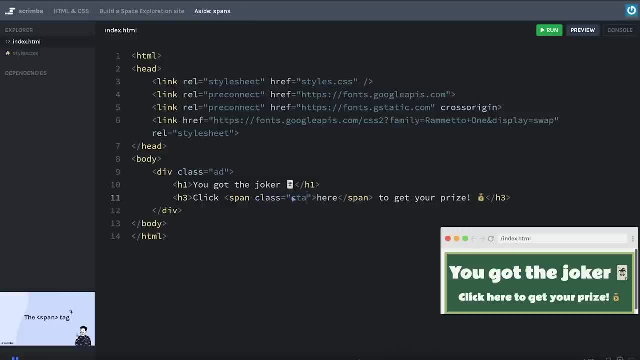 this span, a class. I'm gonna call it CTA, That's short for call to action, As that's normally what these kinds of at the center of our CSS script items, which we know for installation of Lしました variable, which comes from настand, there's a discuss upper. 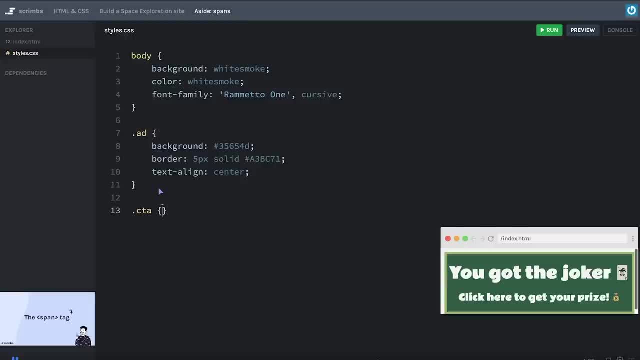 are called, And in the CSS we'll do CTA. Let's just see that it works by doing color red. Yes, There we can see. we have now only targeted the here word. This doesn't look particularly good, though, So let's instead do something that makes it look a bit more. 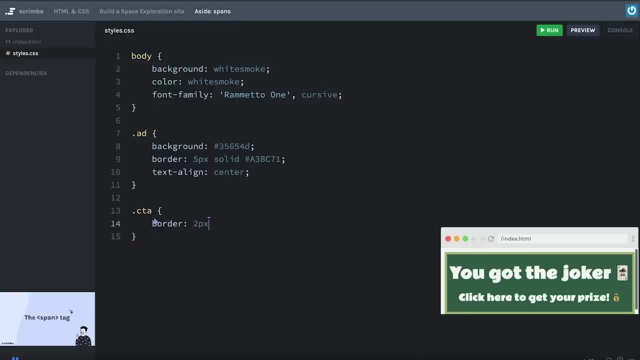 like a button. For that we'd need a border, in my opinion, for example, two pixels, and we want it to be solid. And here let's steal the color from the border around the ad so that we reuse it a little bit. I think that can look nice. Yeah, okay, Here you can see. 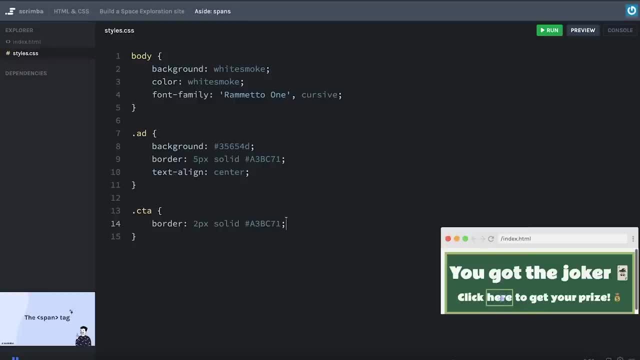 that it's added a border around. the word is very crammed on the left and right hand side, So let's try to add some padding. Let's just do five pixels or something. Actually, I think we can do five pixels on the top and 10 pixels on the left and right. Yeah, that looks much. 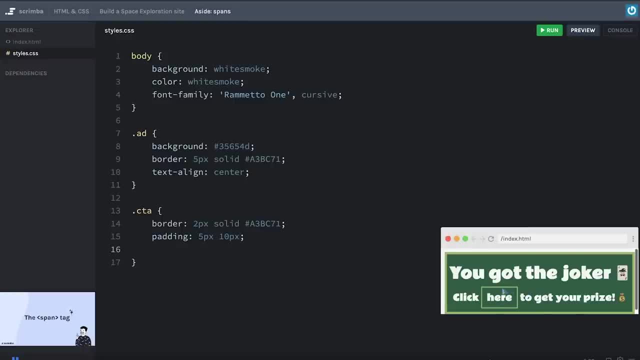 better And then to make it pop out even more so that it doesn't blend into the overall background we have on the ad itself. So I'm going to do background Now. I happen to have a nice brown color here which I think looks decent with the other. 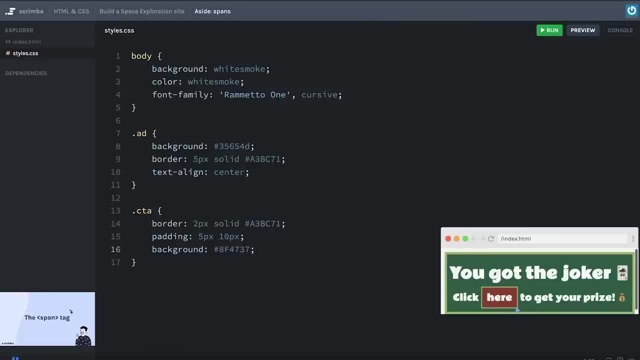 colors here, So now it is a lot more easier to see that you are going to click here on this thing that looks like a button as it stands out more, And hopefully we have increased the click through rate with 0.02%, And those made our boss really happy, So great job. 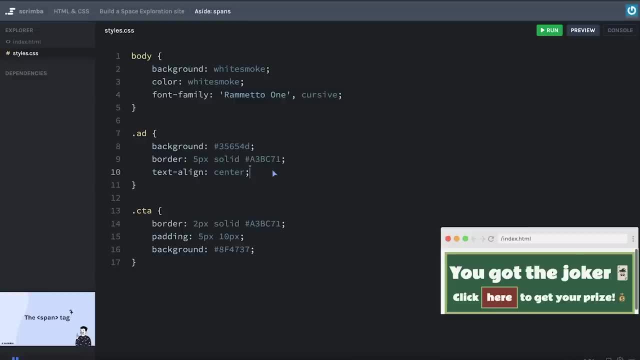 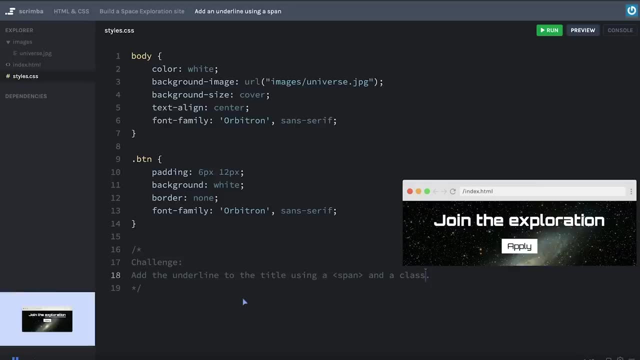 Now that you've learned this, let's return back to the space exploration site and put your new skills to the test. Okay, now you're going to create this neat little underline under the exploration word, And I want you to do that using a span and a class. As for the specific design of the 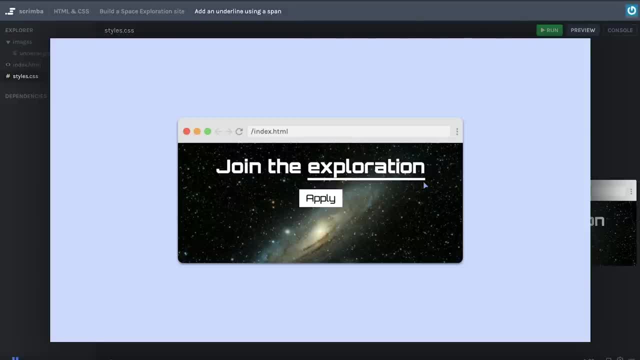 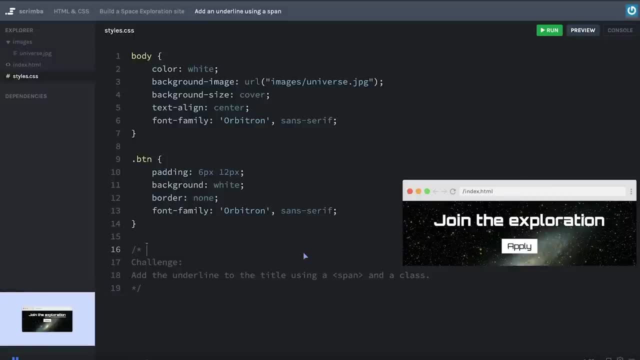 underline and what kind of CSS property you are to use. that is something you'll have to figure out on your own, So go ahead and give this a shot. Good luck, and I'll see you on the other side. Okay, hopefully that went well. Let's do it. I'm going to start with adding this span to the 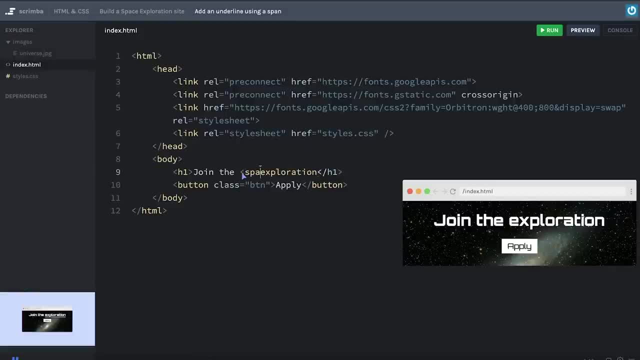 HTML. it should wrap the exploration word So span, like that. And then I'm going to give it a class. I'm going to call this class underline, because it'll only have one job and that is to give the exploration word the underline. So this class is something we've talked about. 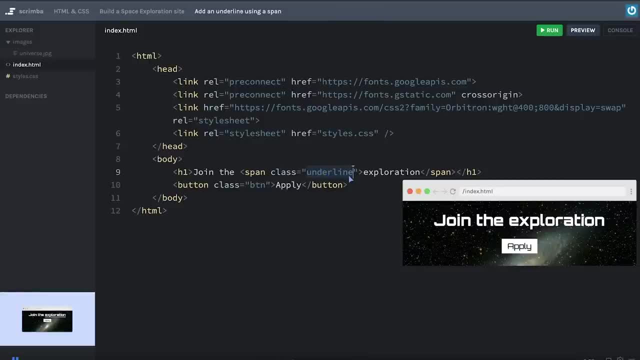 earlier. it's a utility class. it only has one job and that is setting a single CSS property. So if we run the code now, nothing has seemingly happened, But we do have this in our DOM, meaning we can select it in the CSS. we'll do dot under. 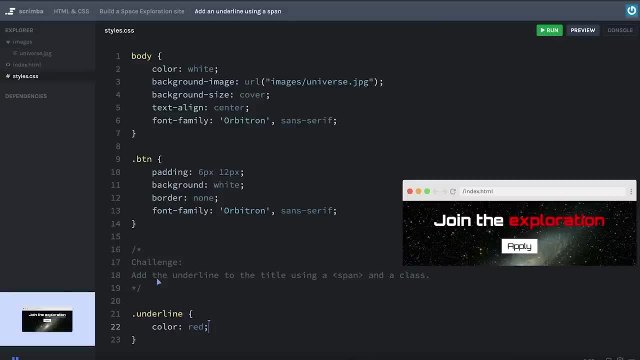 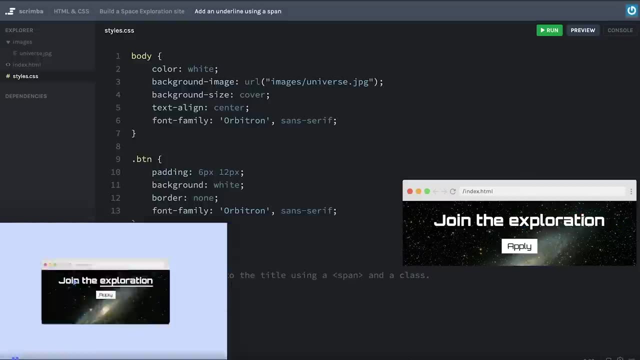 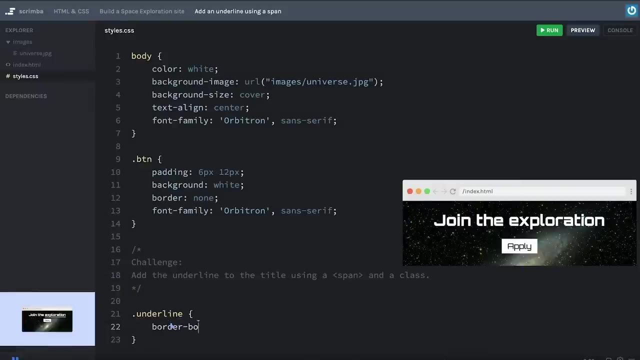 line like that. Let's just try and set the color to red to see that it works. And yes, it does indeed work. But that's not the effect we want. we want to set the underline. And what is this underline? Well, it's actually just a border bottom. we do border bottom. 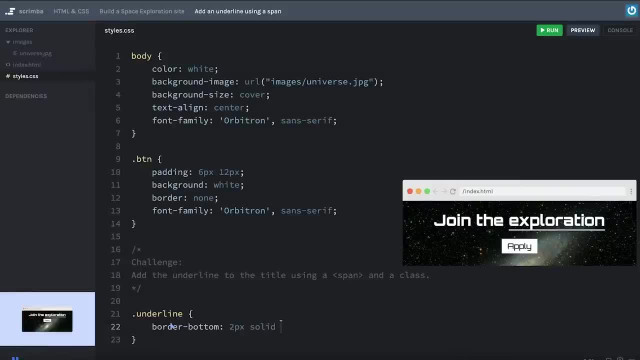 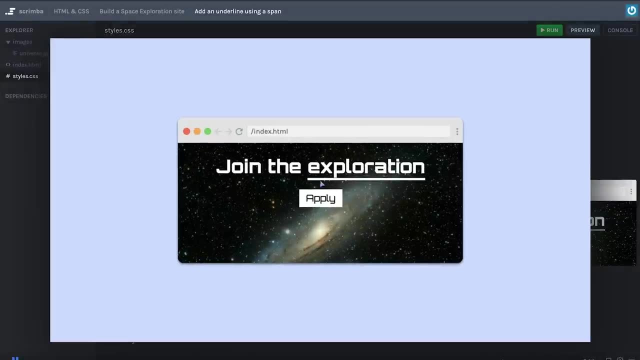 like that: two pixels solid White. you can see. yes, we did get a border under it. However, this border looks a little bit thicker, So I don't think two pixels is the correct thickness I think we want to. 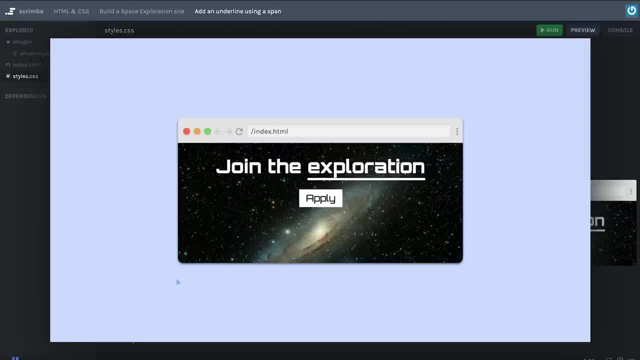 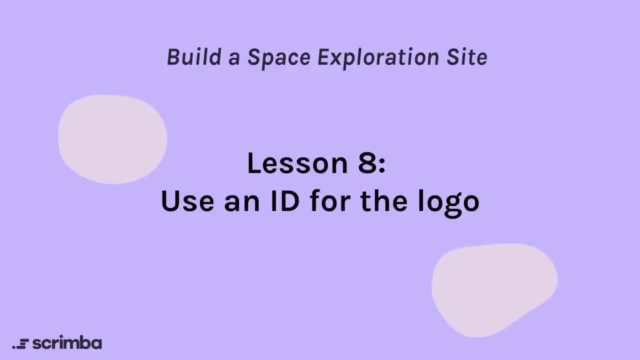 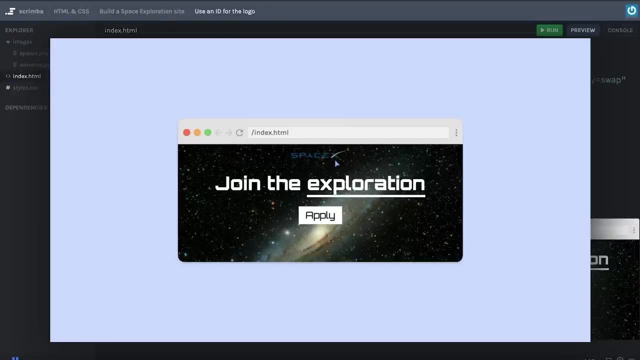 have something like four. Yes, that looks pretty good to me. So we have solved this challenge and we are ready to move on. Okay, now we are going to add this SpaceX logo at the top here, And while you're adding it, you're going to learn a whole new. 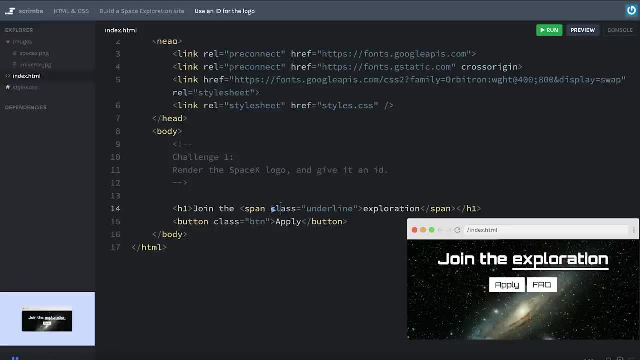 concept in HTML and CSS, namely a close cousin of the class attribute, which is called the ID attribute. And the way to use it is simply by writing ID instead of class. But now you're probably wondering: why would we use this ID? Well, if we now try to rerun this code, you 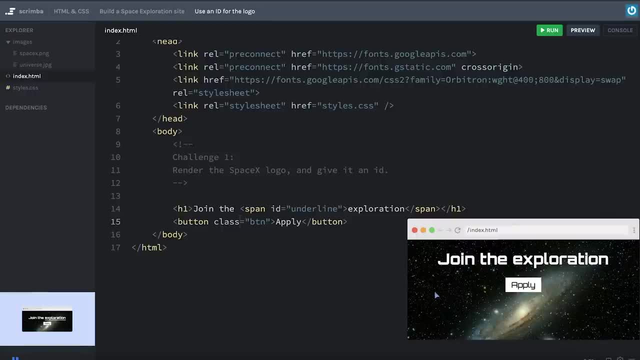 can see that our underline is gone, And that is because, when you are using an ID like this, you have to refer to it in the CSS, Not by using it in the CSS. you have to refer to it in the CSS, not by using it in the CSS. 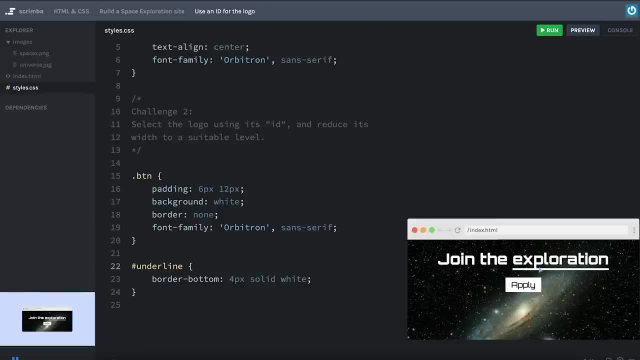 But instead by using a hashtag There. you can see now our border bottom is again applied to our example. So now you're probably wondering: well, why would we want to use this? it just further complicates things by having both IDs and classes to worry about. And the thing 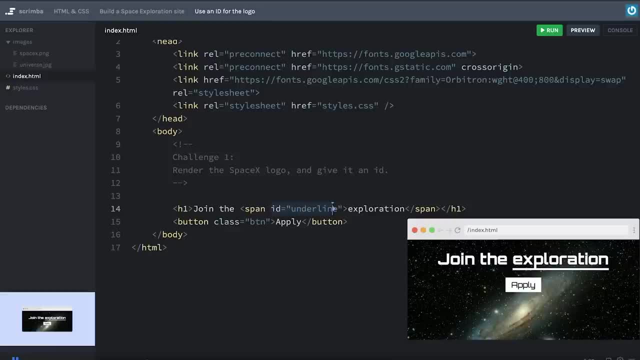 is they serve two different scenarios. you should use an ID if you know that your element is unique and you'll only use it once, So ID of underline should only be applied once in this entire document, Whereas class is something you can reuse again and again. it's meant for usage, So 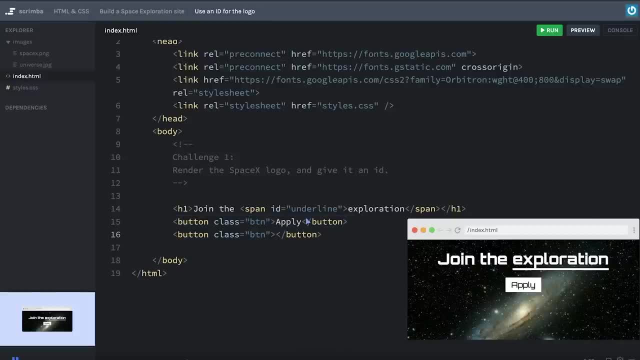 if you, for example, wanted a button here that also said, for example, fa queues, then a class is what you use in order to make sure that this button has the same styling as this button. But if you did that with IDs and turned the BTN here into an ID, this would. 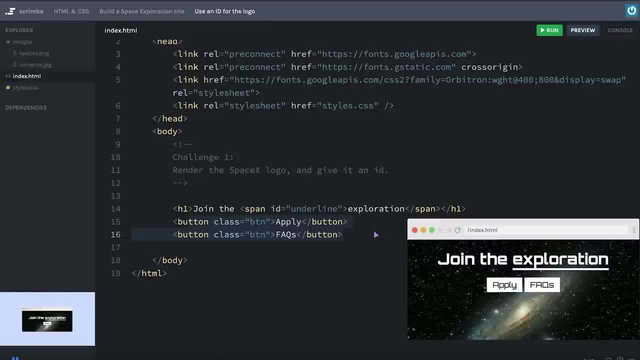 be invalid. HTML browsers are very forgiving, So it probably would work Technically, the styling would be applied, but you just shouldn't do it Now. as for this ID of underline here, I actually don't think it makes sense to use an ID, Because this underline here could perfectly. 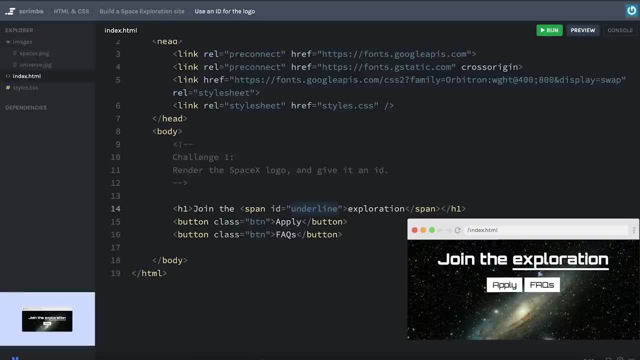 find be a part of our design system and also be applied at multiple other sections and paragraphs throughout our entire page as we build out this space exploration site. So I want to have the freedom to be able to reuse this later as well, even though I'm only using 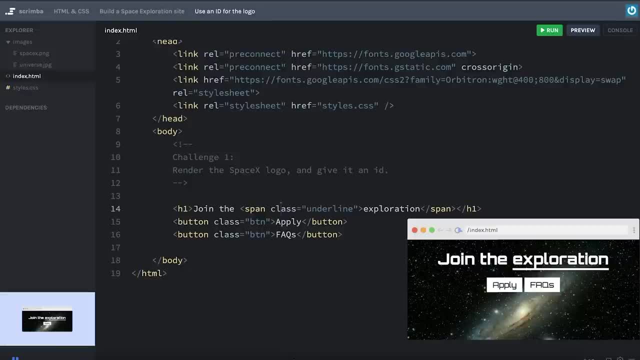 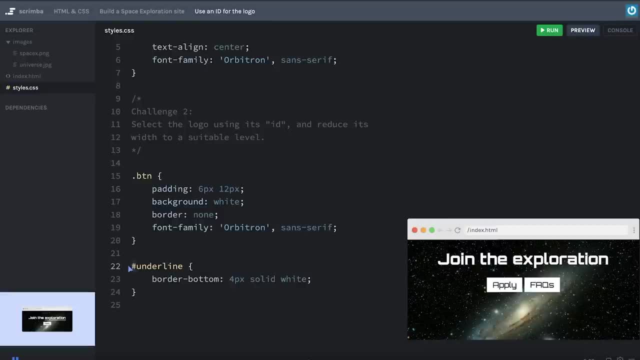 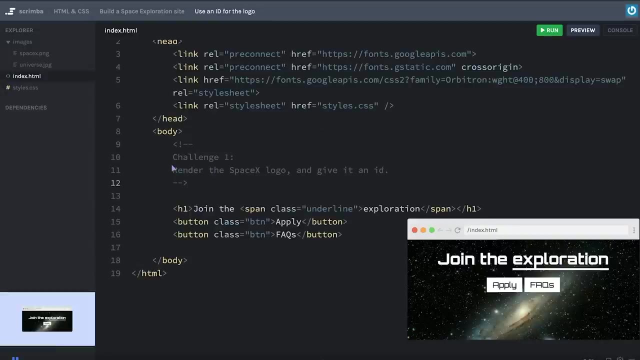 it once now. rerun the example- now it's not applied- And then go from the ID selector to the class selector in CSS by replacing the hashtag with a dot, and there it is applied. So that was a long intro. The reason for that was that I want you to render this SpaceX logo you. 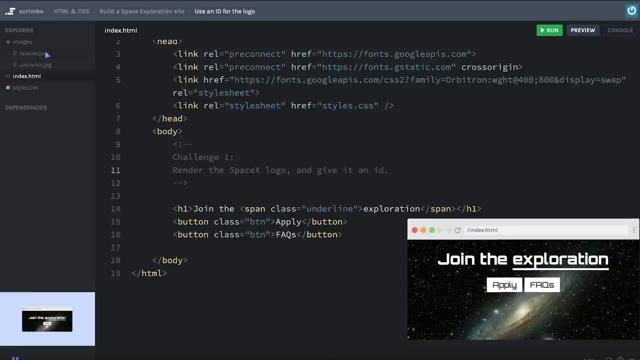 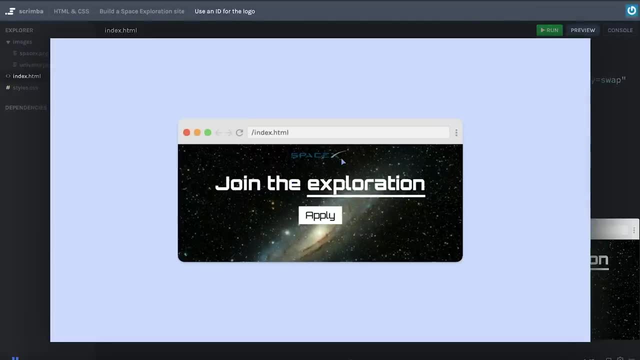 can see. I've added the SpaceX dot PNG image file up here And then I want to give it ID, Because this SpaceX logo at the top here is most likely unique. we probably don't want to have multiple entered SpaceX logos at this size. So this is kind of our main logo And you can give. 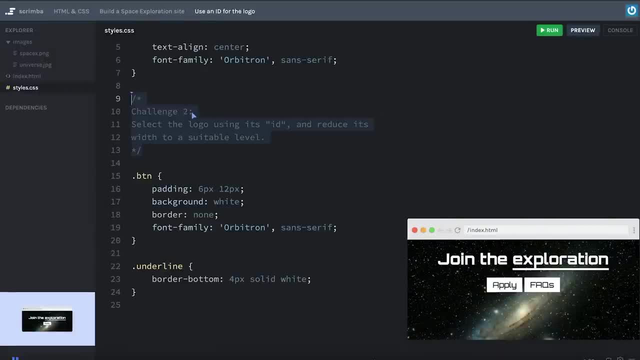 it that ID main logo. Then in the CSS, you need to select the logo using whatever ID you have given it And then, as you'll see, you'll have to reduce its size. That's why you need this CSS rule right here, because it is far too big this image. Finally, I'm 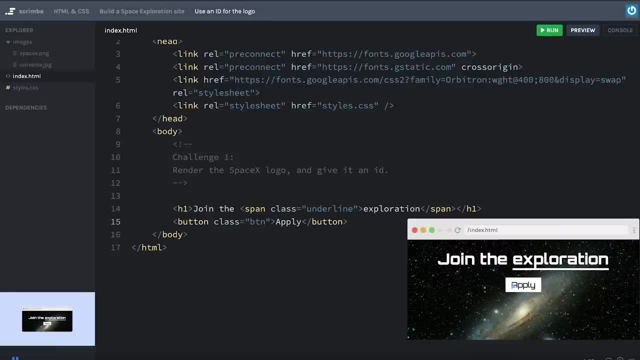 going to remove this faq button so that we're back to our original design. Now it's your turn. take over and try to solve this challenge. Okay, hopefully that went well. let's do it. We're going to render it using an IMG tag. 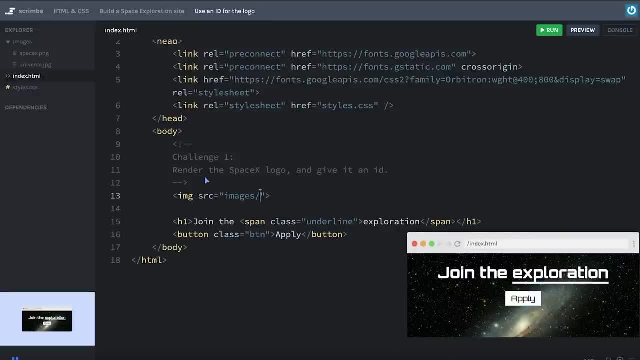 And the source will be first images and then slash SpaceX dot PNG Like that. if we run this, you can see: Oh wow, haha, That is not exactly what we were looking for. It's far too big, this image, So we need to save this image as an image. Here we go, Go-ahead, save. 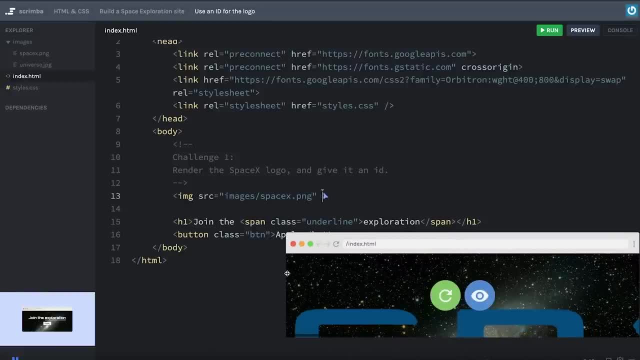 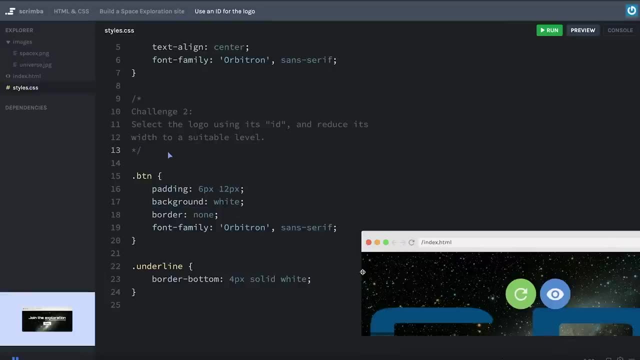 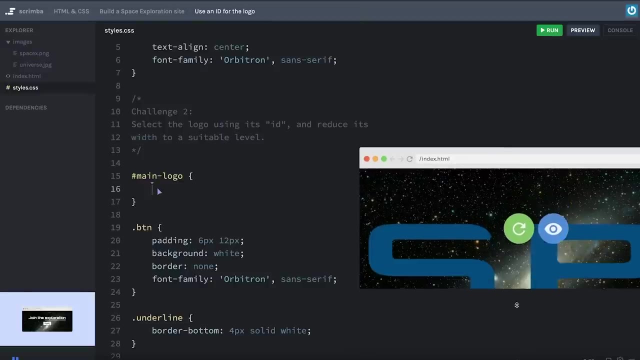 we have to reduce its size And to target it, we're going to use an ID And I'm going to call this main logo like that. Now, if we head to the styles of CSS, we'll do hashtag main dash logo, And here we have to reduce its width. So let's try with, for example, 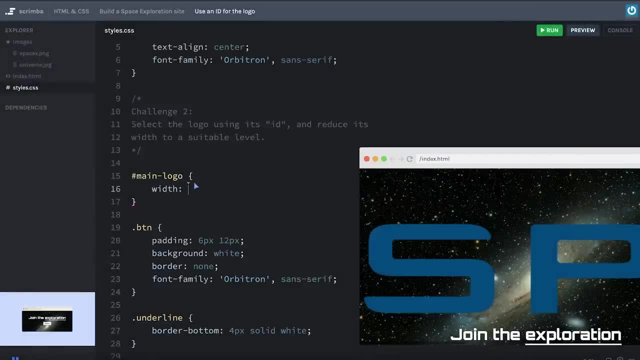 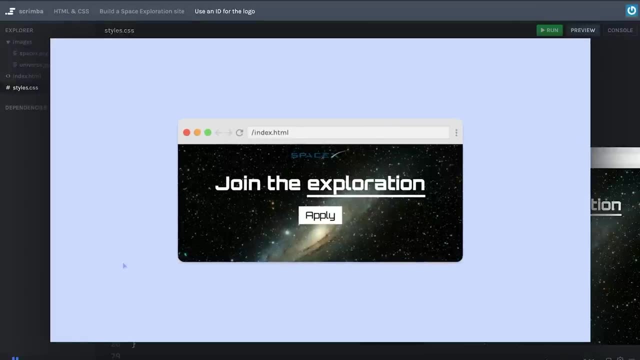 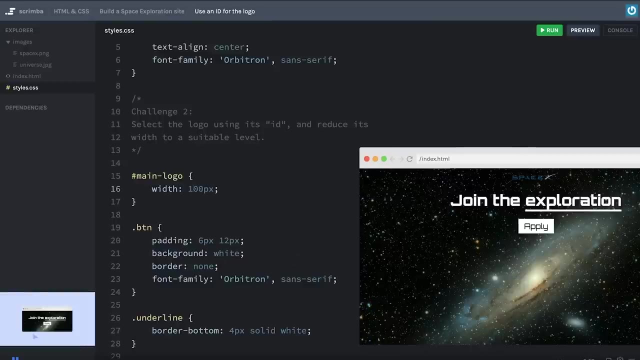 perhaps this is 200 pixels, I don't know. Let's try 200px I got. Oh, that was a bit too large in my opinion, So let's reduce it further to 100 pixels And, yes, that is much more like our design, in my opinion, looking pretty good. So with that we have. 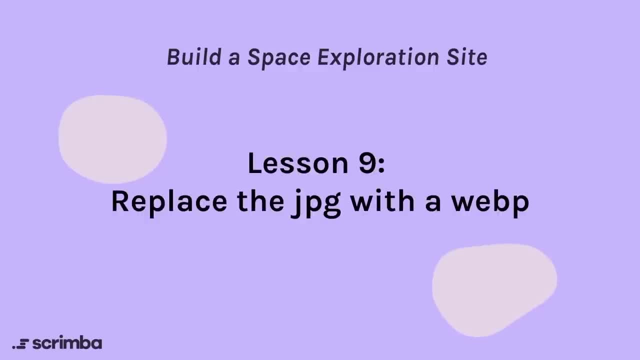 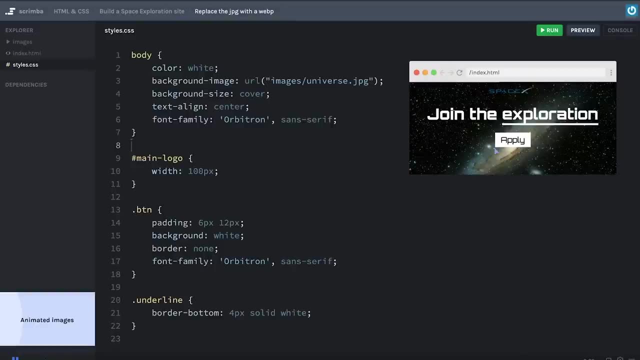 solved the challenge, Great job. Now we're going to breathe some more life into our example here, Because it works fine with this static JPEG as the background image. but wouldn't it be a little bit more interesting if we added a little bit more depth to the image? 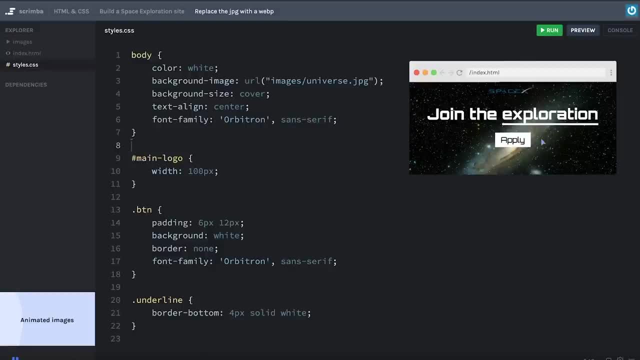 Yeah, that would be a lot cooler if it was animated, So you could see the stars flying around. And in our images folder we now just happen to have a file called galaxy dot web p. What's that? Let's just try to replace this universe JPEG here with the galaxy web. 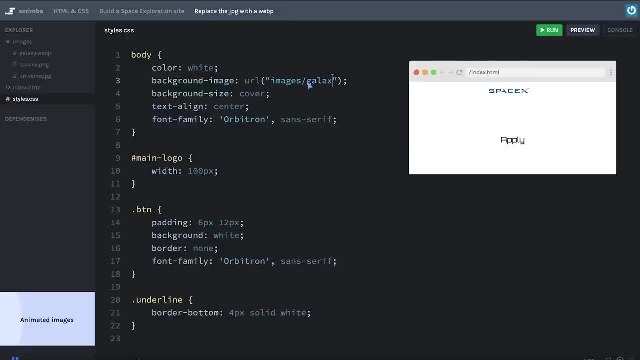 p file. So I'll do galaxy dot web p and boom. the galaxy web p is an animated image in which you see a bunch of stars around the galaxy, And to me this looks a lot cooler than what we just had Now you. 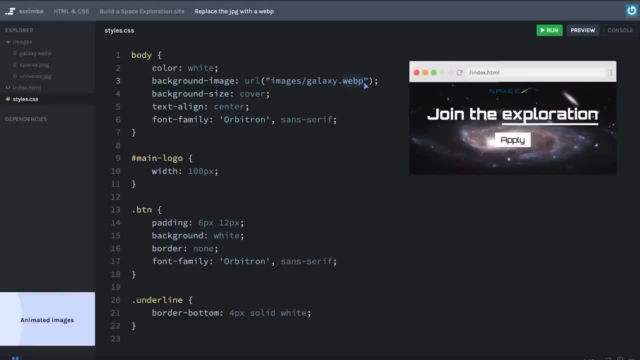 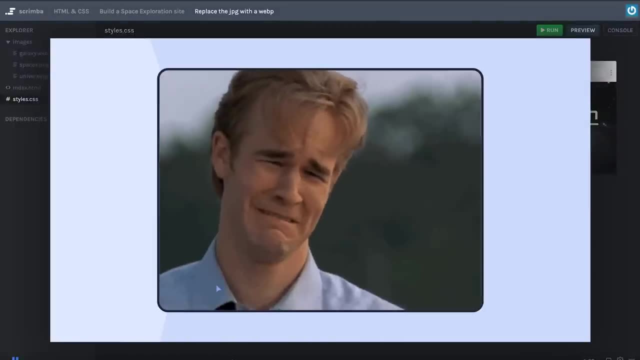 might wonder what this web p here is, and that is just an image format pretty similar to so called gifts GIF, And gift is what you recognize from all over the web in animated images like this one right here, which you've probably seen before. So web p is used exactly. 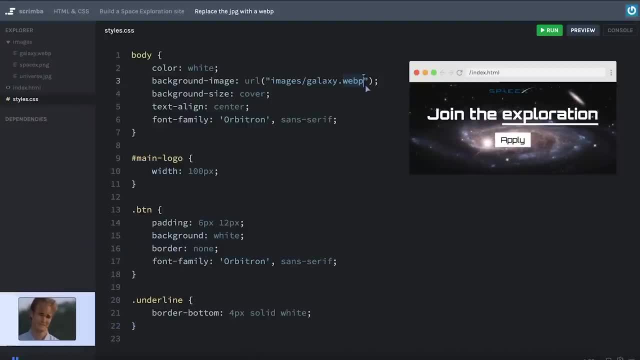 as gifts are on the web. However, it has a better compression So it's more compact and doesn't use as much data as gifts When they're sent from a server to a client. So we want to use web p where we can And 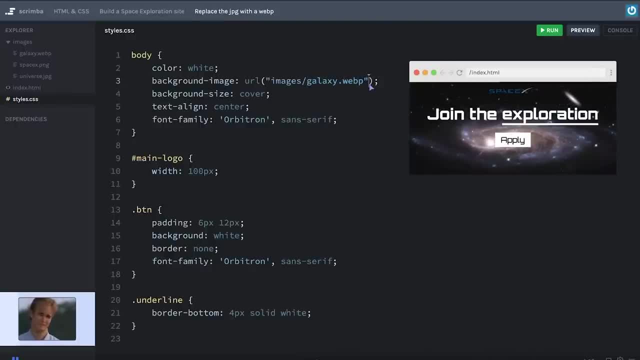 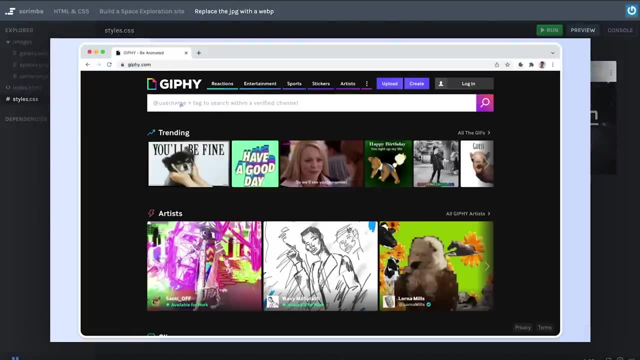 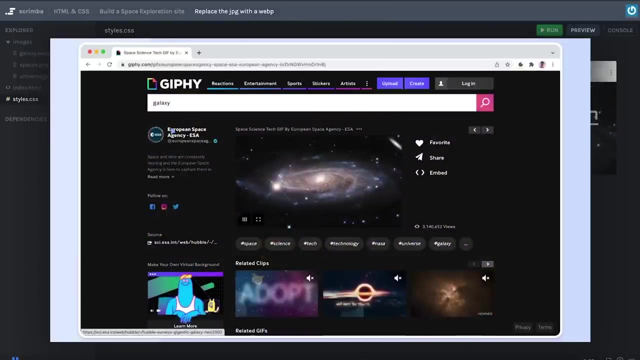 now you might wonder: well, where did you find this galaxy dot web p image? that is on a site called GIPHY That is a search engine for gifts. So I just navigated to it, searched for galaxy, scrolled a little bit down and found this neat looking galaxy GIF here created. 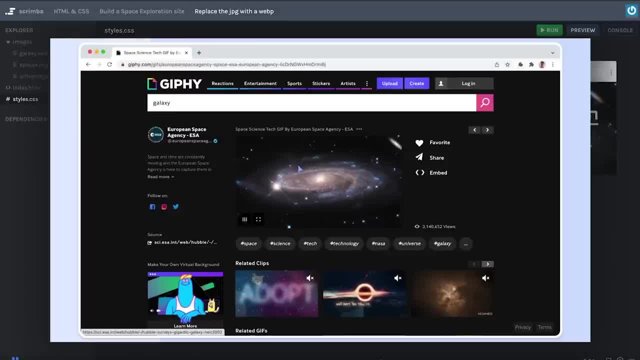 by the European Space Agency. Now this is a slideshow, So you can't see that this is GIF is now being animated, but it actually is, because I just saved this image to my local computer and then uploaded it to the images folder right here. Now, if you want, you can. 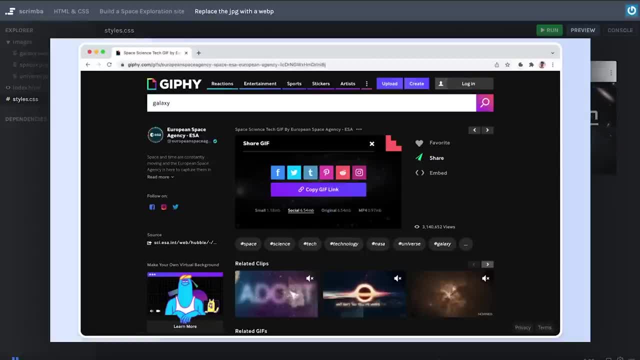 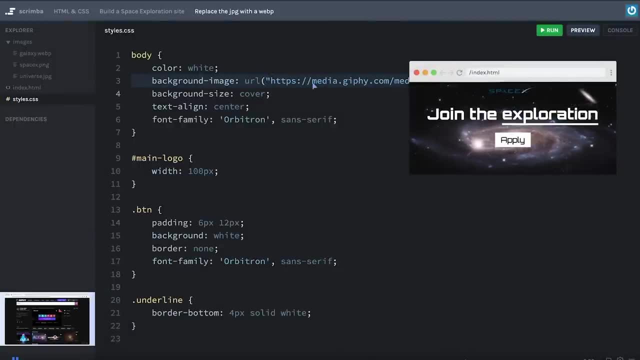 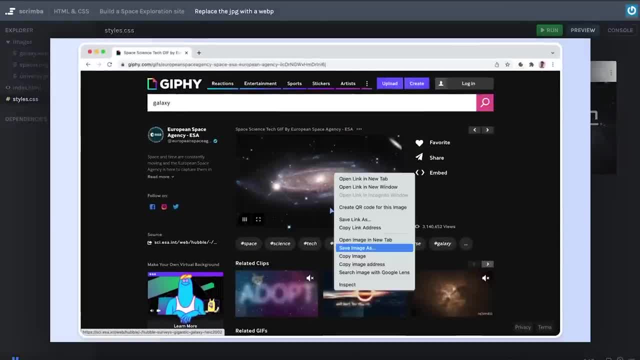 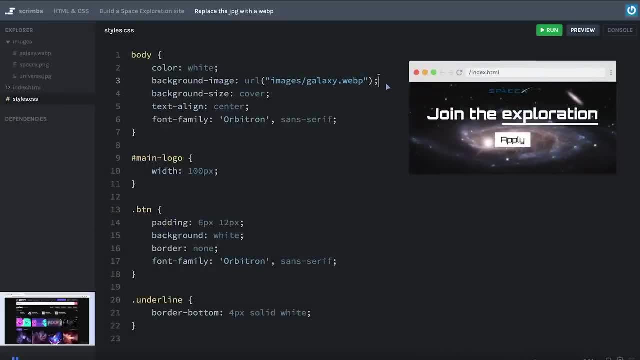 Let's lakes, and I think you should head over to the fee, search for a few images and just paste them in right here and see how that affects our example. just so you've gotten familiar with using GIPHY and pasting external URLs into the background image property in. 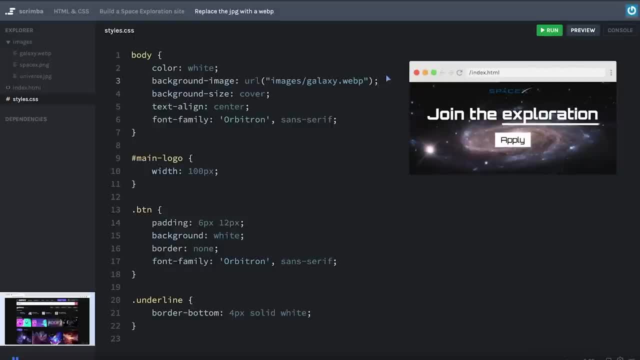 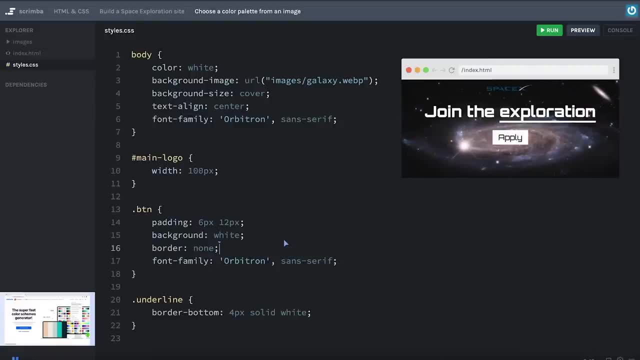 CSS. So go ahead and do that, And then I will see you in the next skrim denvercom. One thing I like to do when working with images as backgrounds is to fetch colors from lookups from the image and use it in the design, because that can often look pretty cool. So let me. 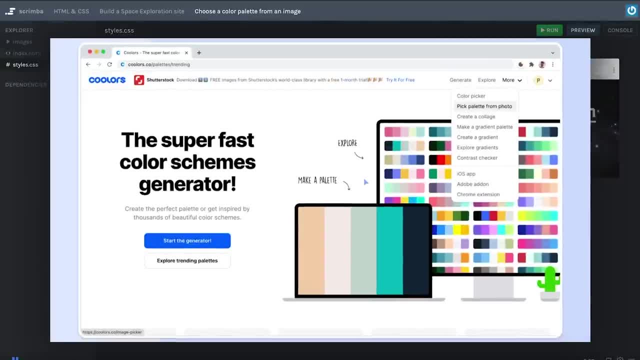 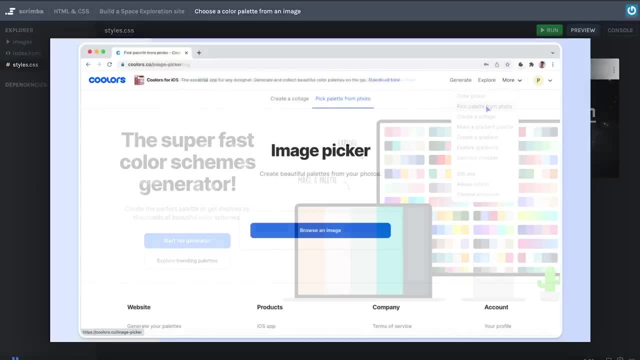 show you exactly how to do that. We can use coolers, the service you're already familiar with, because if you click on the more option in the navbar, you can choose pick palette from photo. that'll take you to this image picker where you can choose an image by clicking. 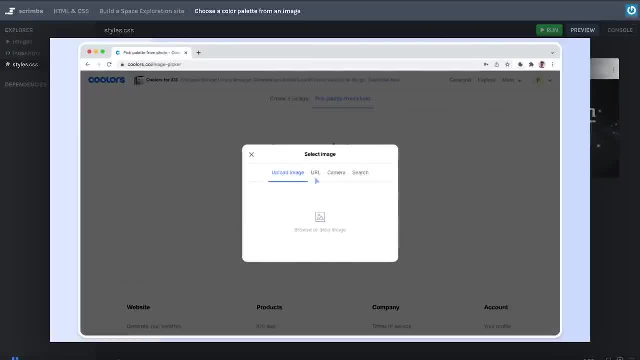 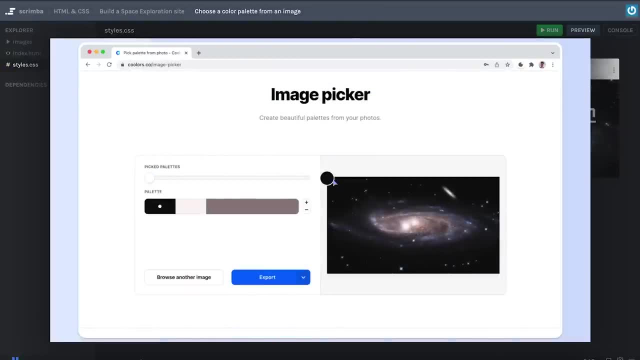 on the browse an image and either upload the image or paste a URL to it. Once you've done that, you're taken to this nice tool where you can either drag and drop this picker around on the image until you find the color you like, Or you can use this range input. 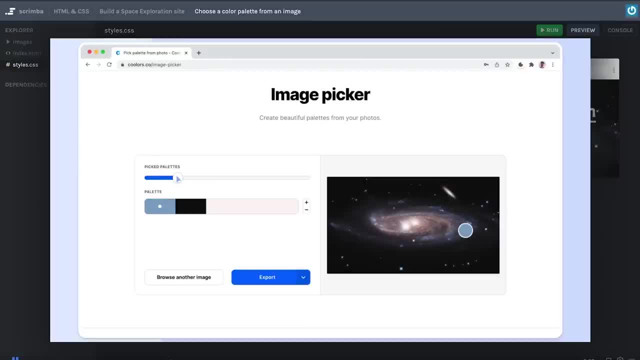 here is that will automatically try to find interesting colors in the image for you, And then it generates a palette, as you can see right here. Now let's say, we like this palette, then we'll click Export and save palette and we have it in our dashboard. Now it only 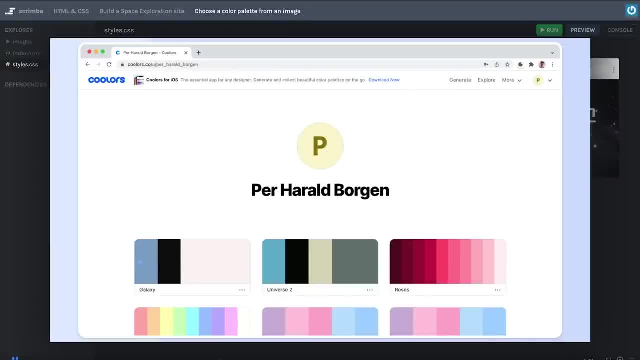 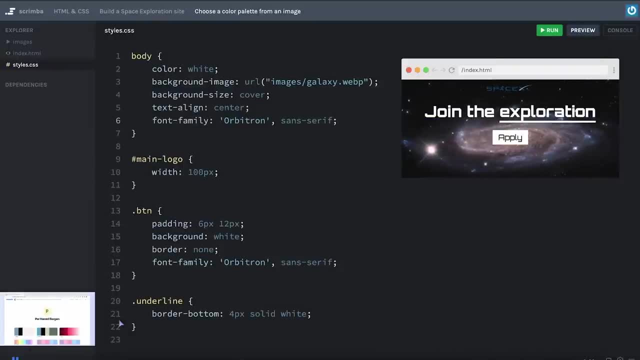 has three colors, but that doesn't matter. I'm only going to use one of these, that is, the blue one, because I think it would be cool to use this blue color as the text color on our site. So I want the h1 and the button text to have that bluish color, And the way 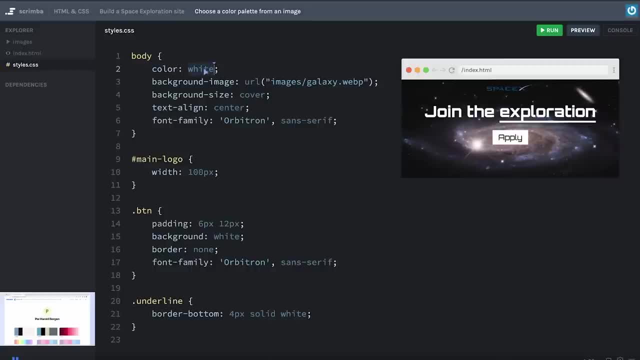 I'm going to do that is change the color of the body here, because that is where the h1 gets its color from. it is the only element inheriting from the body at this point, So I want to do like that. this is the hexadecimal value I got from coolers And, as you can see, 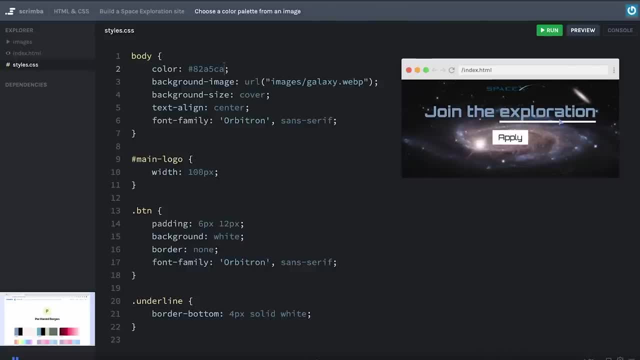 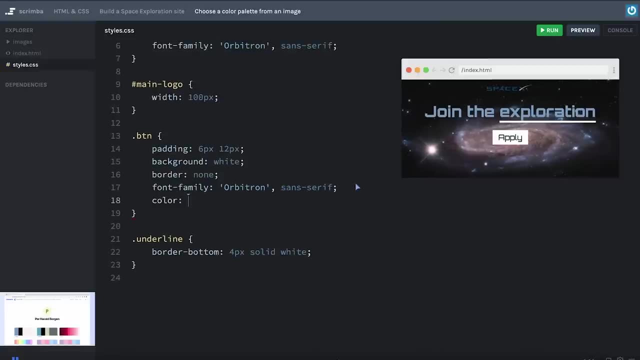 I think it looks pretty cool. And also, let's keep the underlying white, because I think it makes sense to have that in a different color. Now, moving on to the button, we'll do color and paste it in again, And there we go. Now, here I. 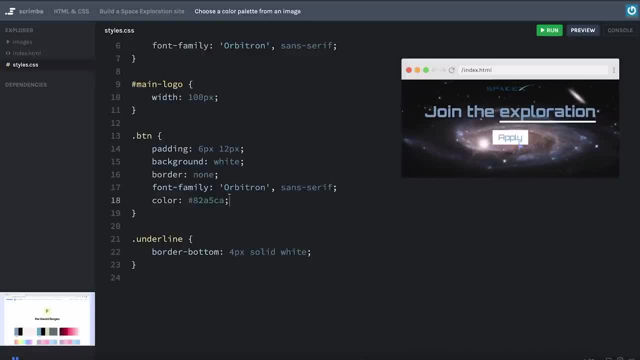 think actually this apply text could be a bit clearer, because the contrast with the background is just okay at this point, Because with this blue color I think the thin letters became a bit too thin. Now, a final thing I want to do with this apply text here is: 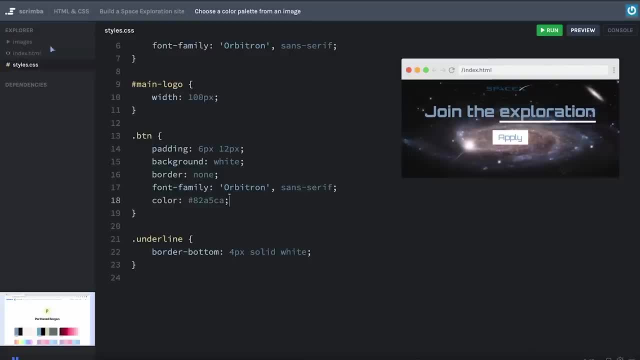 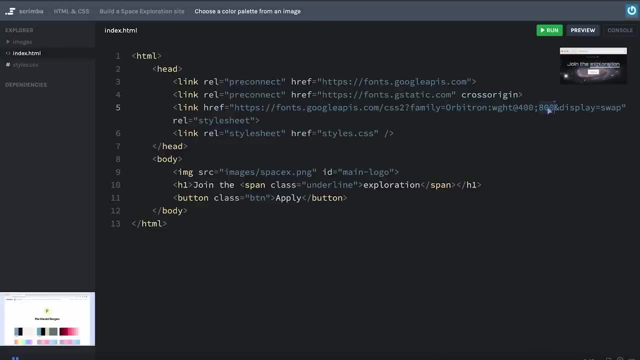 make it a little bit bolder, make it stand out a bit more, And luckily we imported not only the regular font weight with the Orbitron font family but also the 800 font weight to the extra bold. So what we can do now is actually do. 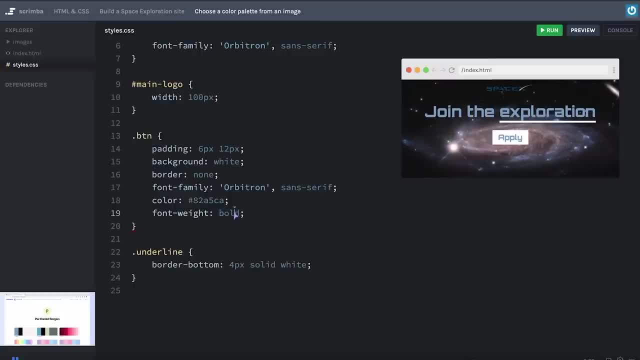 font weight And then just bold, and there you can see it actually bolded the text. or we could use the value directly, which is 800.. That'll give us the exact same result, as the font weight property can both take numerical values and named values. So the numerical values range from 100, 200, 300. 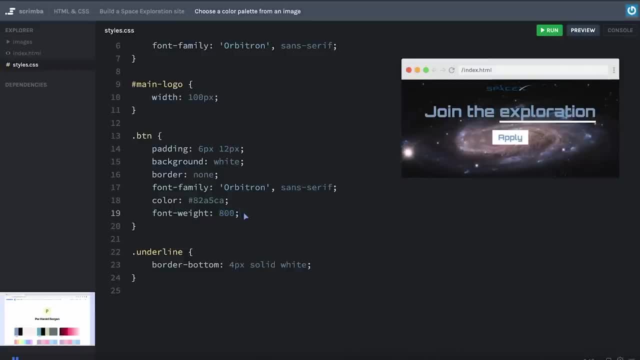 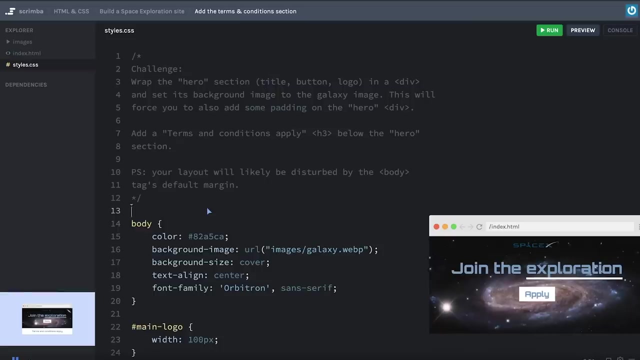 400 and so forth up until 900.. And the named values are, for example, normal, bold and so on. So we imported 800.. So let's just write 800 here. With that, I think our example looks pretty good. So let's move on. 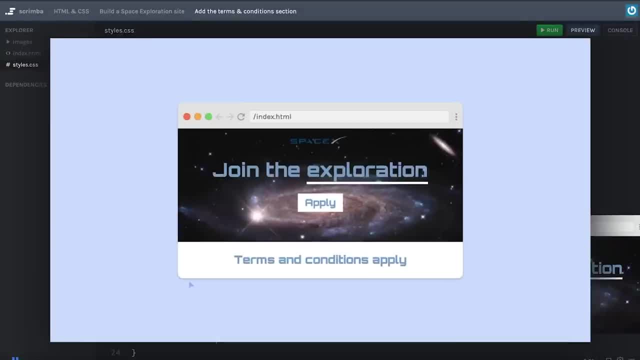 Going to space is definitely a risky affair, So I want to add this terms and conditions text underneath the main section of our site. However, I don't want to add this: This is scrimball. So you're going to do it, of course, but I'm going to give you a set of detailed. 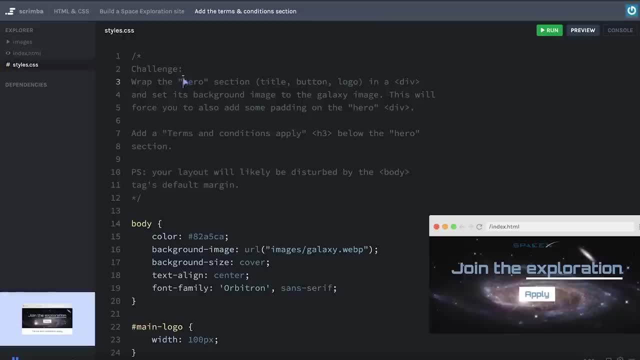 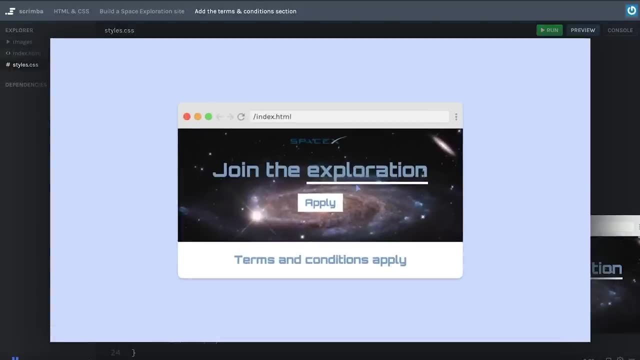 instructions so that you know how to go about doing this. So you're going to start with wrapping the hero section in a div And the hero section is the one you can see on top here. it's very often called a hero section and web design, And it's probably called that. 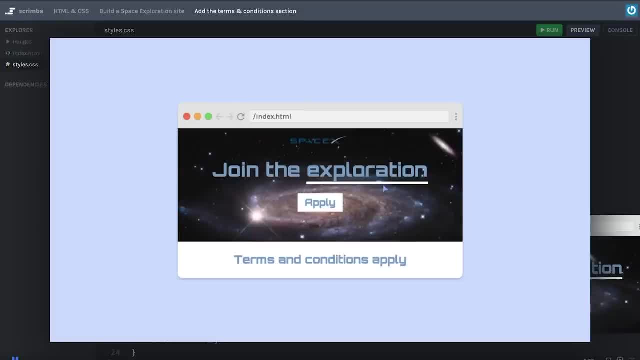 because kind of serves as the user's first glimpse of the company and the offering and has this kind of prominent place towards the top and it usually extends full width, So it is kind of the hero of the website. So in our case it is these three elements right here: the logo title. 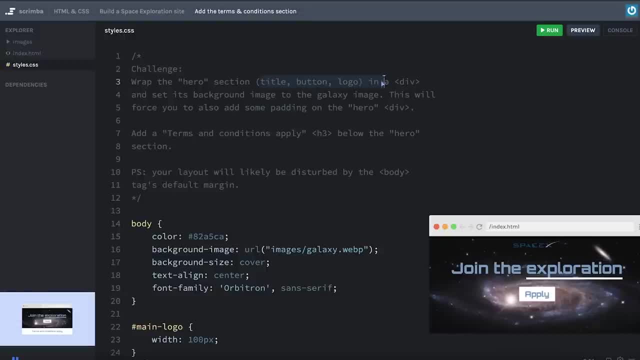 and the call to action button, And those should all be wrapped inside of a div. And then I want you to move the background image, that is, the animated galaxy image, from the body and over into this div. Now, as you do that, you'll notice that you'll have to add some. 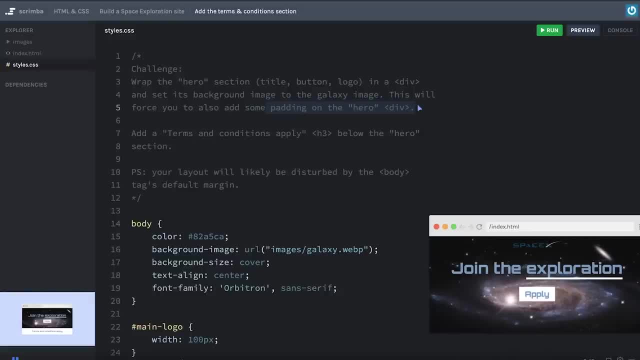 padding to this hero div, as it'll look really crammed. If you don't add that, Then I want you to add the terms and conditions apply in an H3 below the hero section, And then, finally, a problem you'll probably come across is that the body tag has some default. 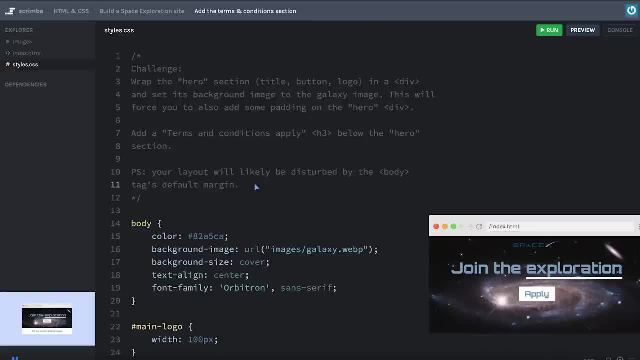 margins, which right now doesn't bother us, but which will become apparent once you change this layout. So go ahead and give this one your best shot, And when you return back to me, I'll show you how to do it as well. 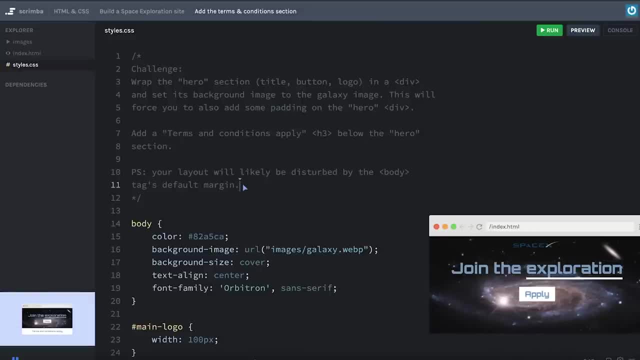 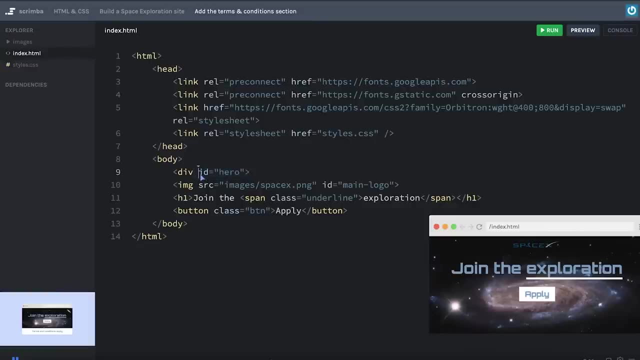 Okay, let's go. I'm going to start with the hero section, div. I'm going to add it right here. I'll give it an ID of hero. it is unique, so it's okay to use ID. Then I'm going to indent this end and run the code, and seemingly nothing has happened. 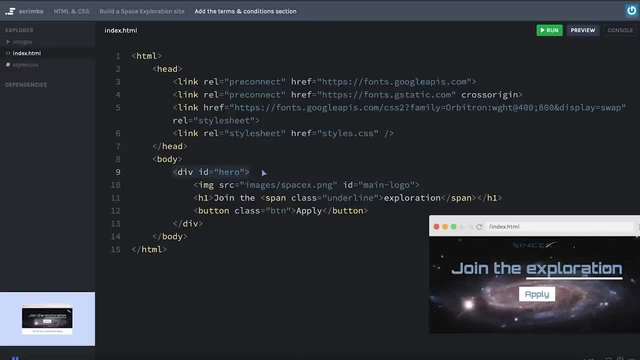 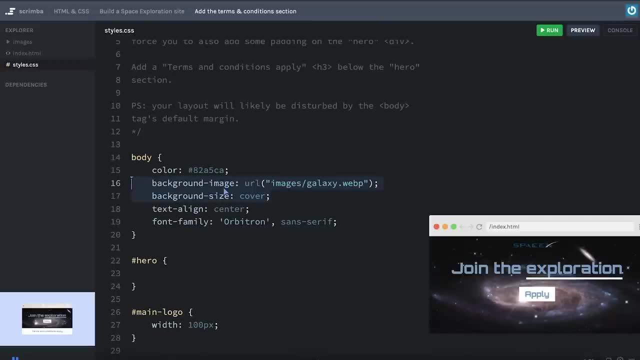 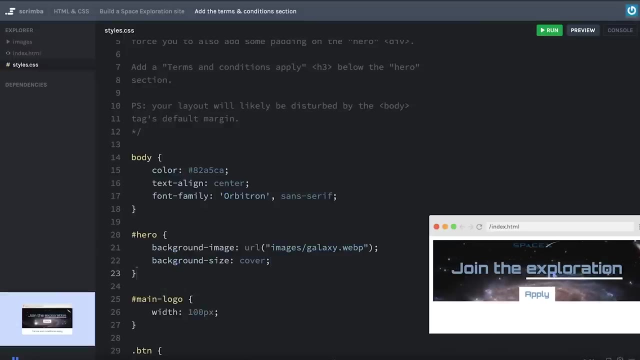 Because, as you remember from previously, devs don't have any default styling to them. So what we need to do is target the hero and then move the background properties from the body To the hero, And there we go. As you can see, it doesn't look particularly good Now, as 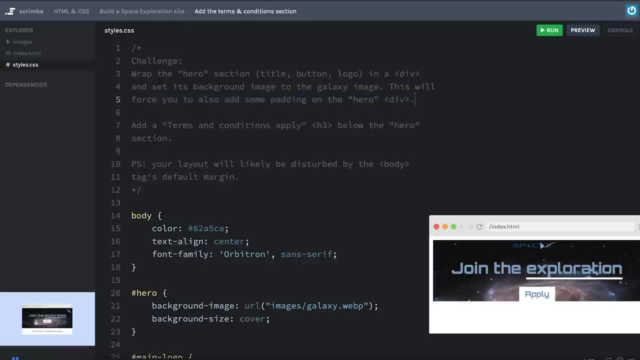 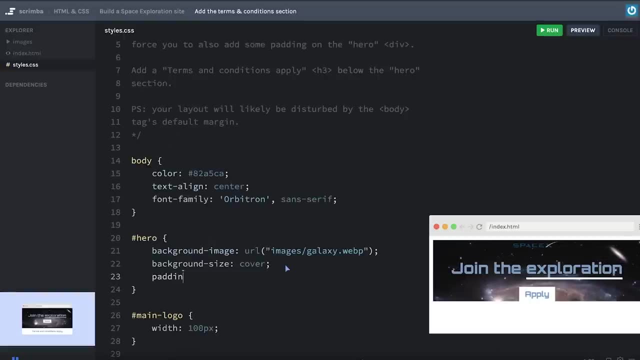 I said we will be forced to deal with the padding in the hero, because you can see, here the logo is really crammed all the way up to the top and there's no space underneath the button. So let's add padding And on the top, maybe we want 10 pixels like that. Yes, 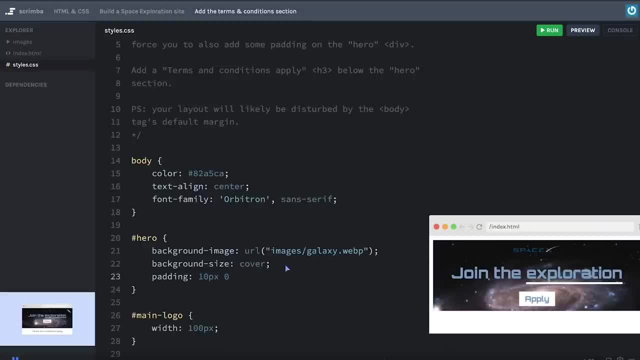 On the right hand side we don't need anything for now, But on the bottom we want a lot of padding. maybe we'll do 40 pixels Like that. then on the left hand side don't need anything either. So here we have the 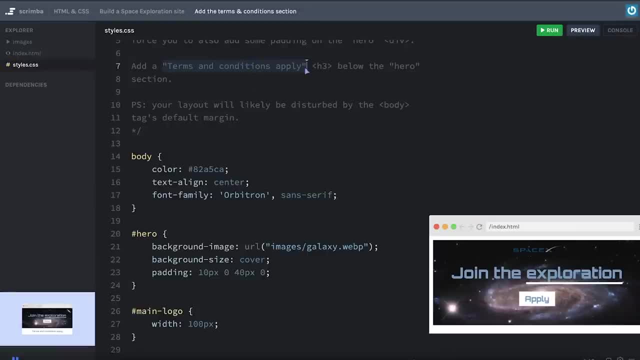 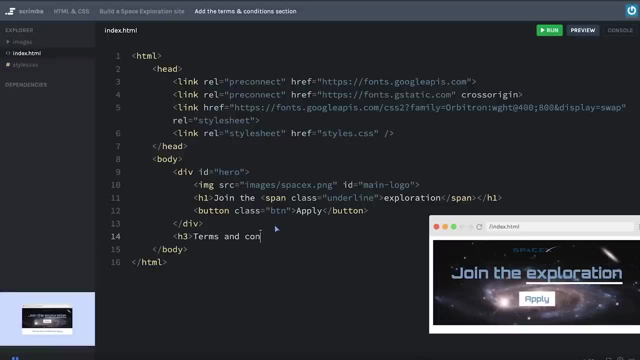 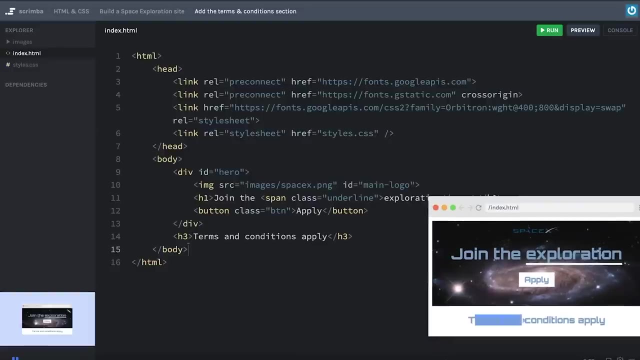 padding. Now let's add the terms and conditions apply: h3 below the hero. That's just like this: adding an h3,, terms and conditions apply. like that from the code. And there we go. it has already the color we want, since we have set the blue color as the text color. 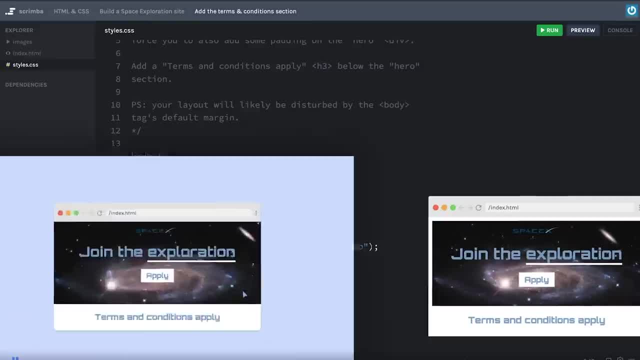 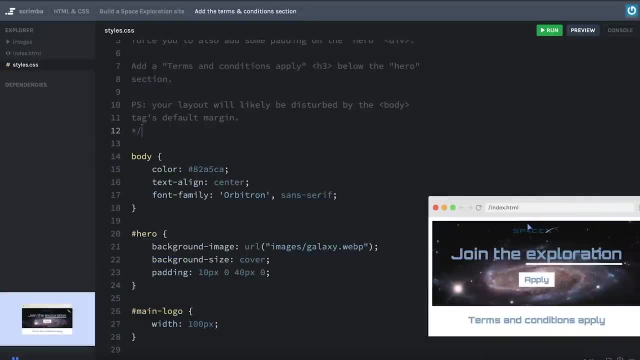 on the body, So it inherits the color property From the body. However, as you can see, are still not quite done, because something has happened with the margins on the site, or at least the margins of the body has become more apparent, because now the entire body isn't filled with the background image anymore. 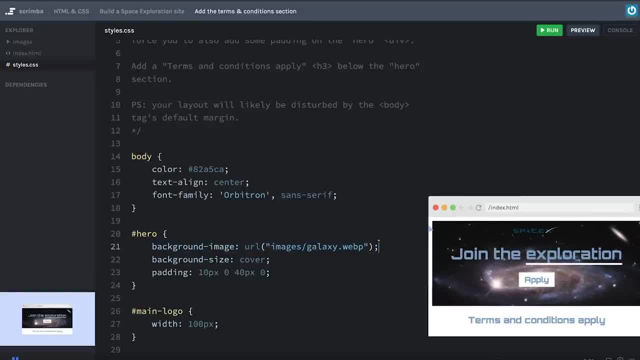 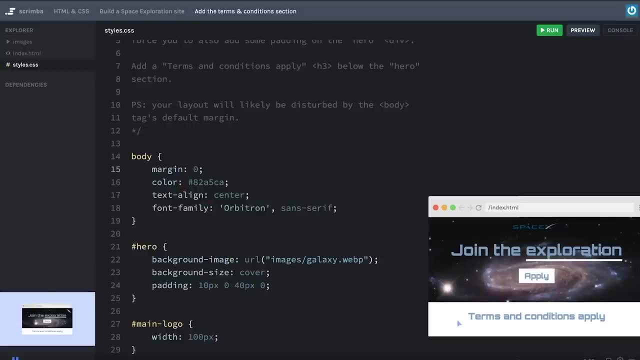 So we're suddenly noticing that the body has some default margins on all sides. we don't want that, So we're going to neutralize that by doing margin zero. and boom, there we go. we have completed the challenge. Now there is one more thing. 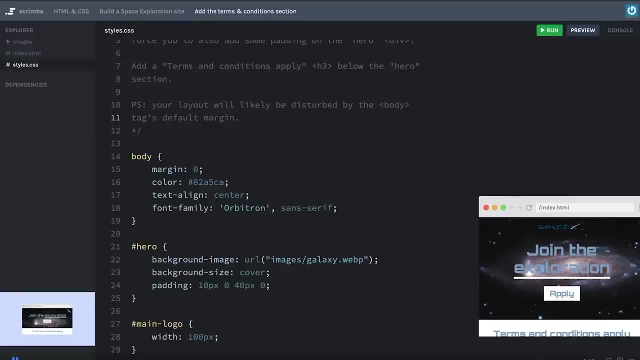 Which is a little bit problematic, which is that if you watch this on a mobile, for example, so that the exploration word is located directly over the galaxy, the readability sinks quite a bit because the text color blends in with the background. And we will fix that is by 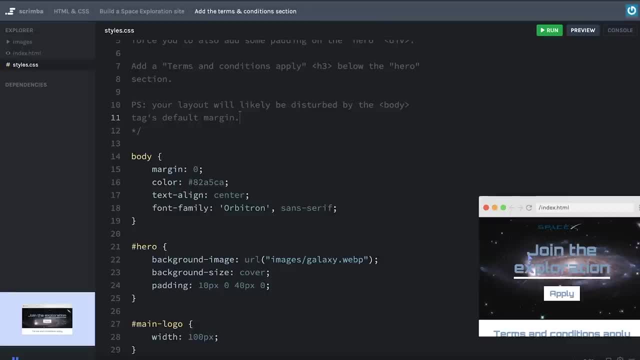 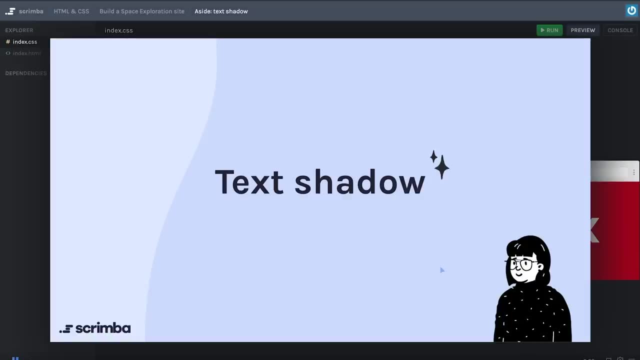 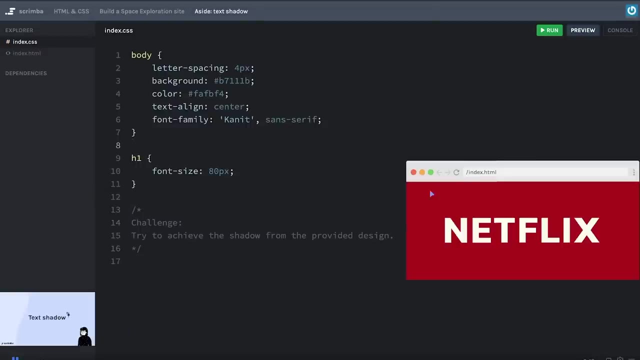 using a shadow technique on this text. So now you're going to learn exactly that Text shadow is a really nice tool to have in your web design toolkit, as it can make your designs much better. So here I've created a very simple imitation of the Netflix logo with the red background. 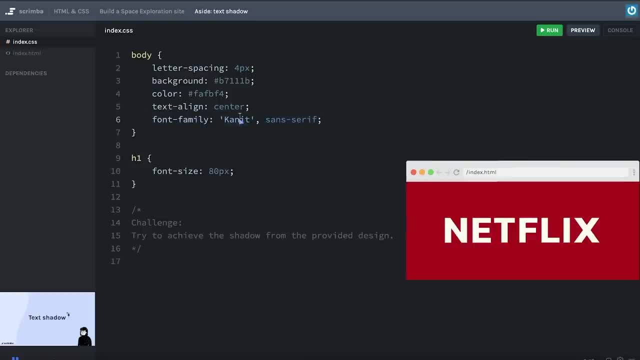 and white text. As you can see, I've pulled in a font which kind of looks like the Netflix font. it's not really the same, but it's close enough And it is an H1. And I've set the font size to 80 pixels. Now, what if I want to have a black shadow like this as that? 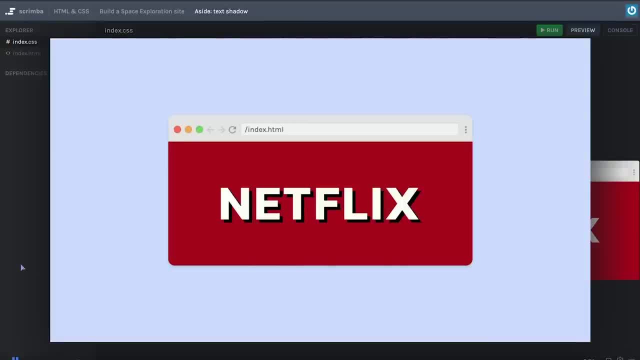 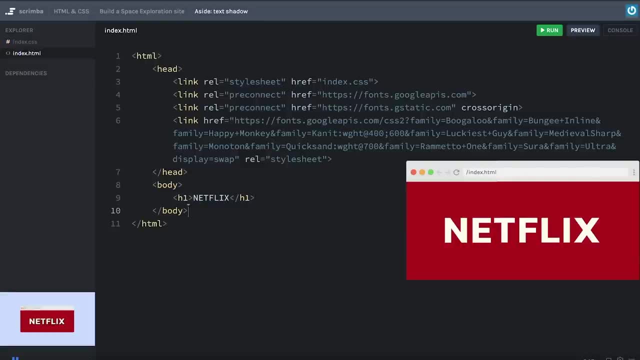 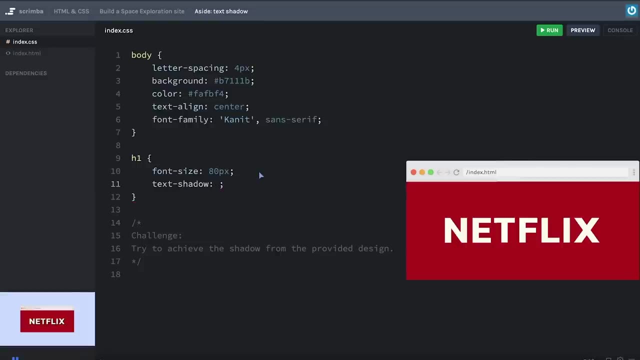 makes it look even more like the classical Netflix logo. I can achieve that by on the H1,, which is the element, And that includes the Netflix text. as you can see, here I can add a property called text dash shadow, which must contain three values. So just bear with me here as I'll. 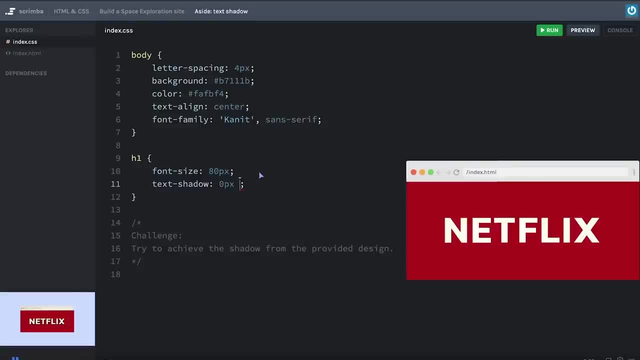 write all three of them out and then I'll explain it. I'll do zero pixels, zero pixels, black, and seemingly nothing happened. That's because I first wanted to show you the third value here. black, that's pretty simple, That's just the color of the shadow And, as you can, 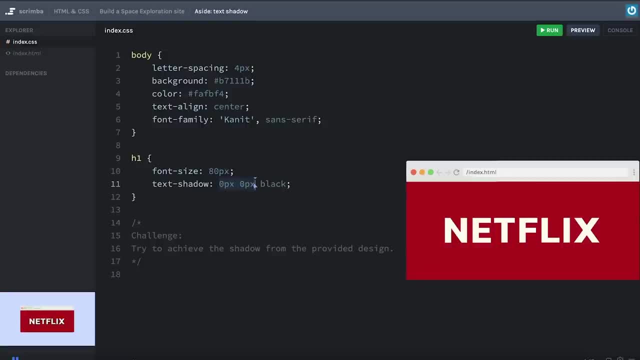 see here it is black. Okay, Two other values dictate the offset of the shadow on the horizontal line and the vertical line. So if I add, for example, five px here, you can see that now the shadow appeared it's as if it's sticking out to the right of the letters five pixels If I do the opposite. 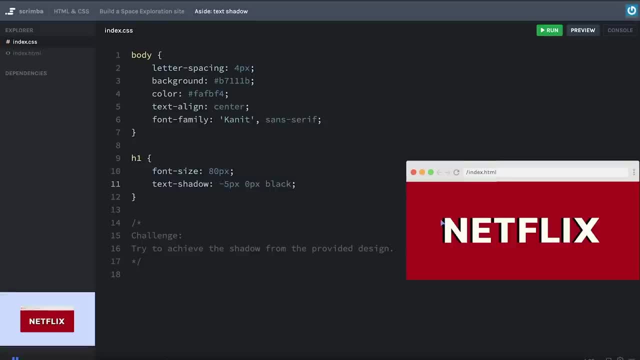 minus five pixels, it'll stick out five pixels on the left hand side. As you can see, there's no shadow below and above, because that's dictated by the second value. So if I turn this back to five and on the vertical one do, for example, 30,, then you can see that. 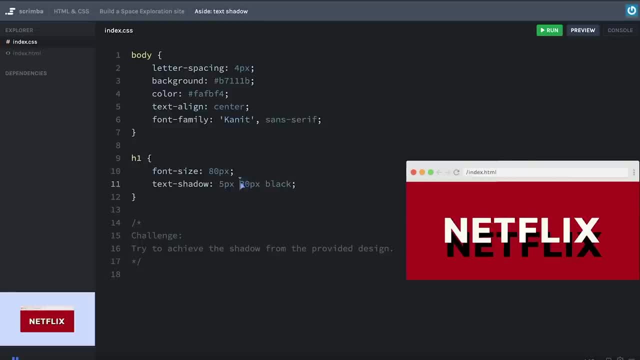 the shadow got pushed far too much downwards. If I do minus 30, it's pushed upwards. If I do five pixels, it's pushed only five pixels downwards, which looks pretty good. actually, It is indeed the design we were looking for. So some rice here. the first value is how. 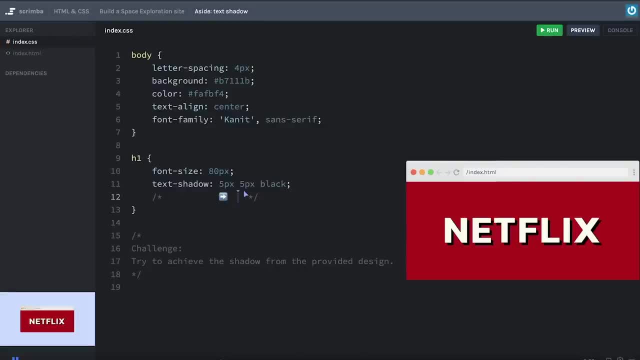 many pixels you want to push the shadow to the right. The second value is how many pixels you want to push to the right, And then the next value is how many pixels you want to push the shadow to the left. So this was to summarize here. the value here means: and here in one. 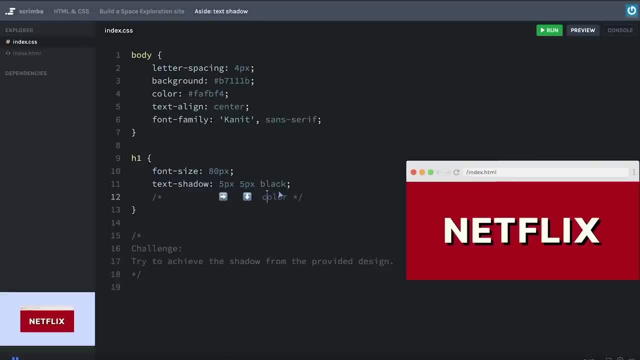 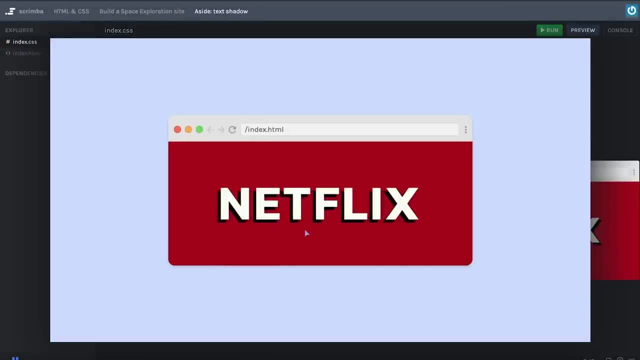 how many pixels you want to push the shadow downwards. And the third is the color. So what I want you to do now is try to make the shadow look like this. As you can see, now it's on the left hand side and below, like as if the sun is shining from the top. 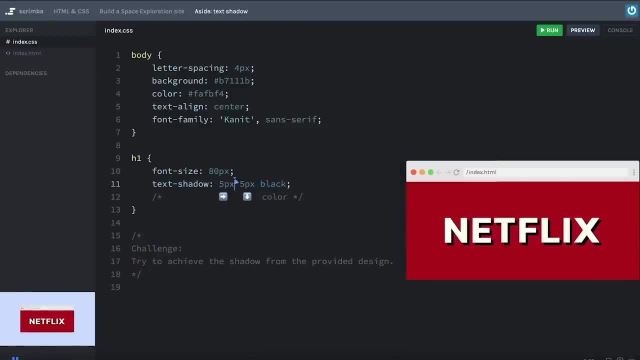 right corner. So take a guess at how you need to change this line 11.. Here, in order to get that effect, go ahead and do that right now. Okay, hopefully that went well. what you need to do is basically put a minus in front of. 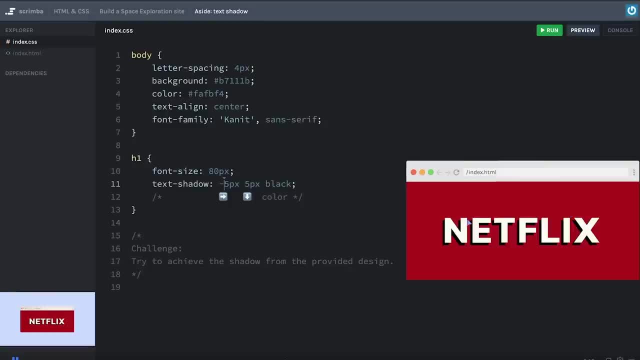 the first value. like that that shifted the shadow from being on the right hand side of the letters to the left hand side. Okay, changing it back again. Now I want to teach you body. fourth value you can add to the text: shadow property. 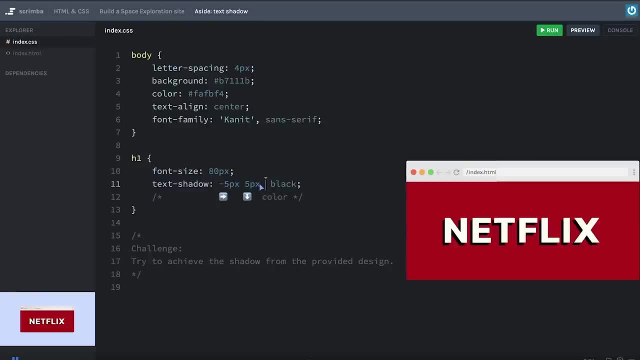 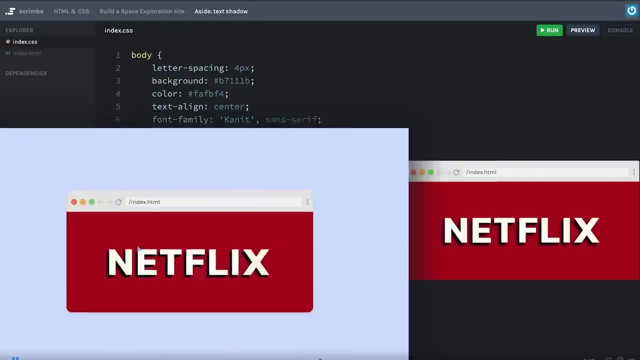 And that is the text shadow property. And that is the text shadow property And that is the third pixel value. So here you can also write, for example, five px. And what happened now? if we compare what we have here right now with how it was before we added? 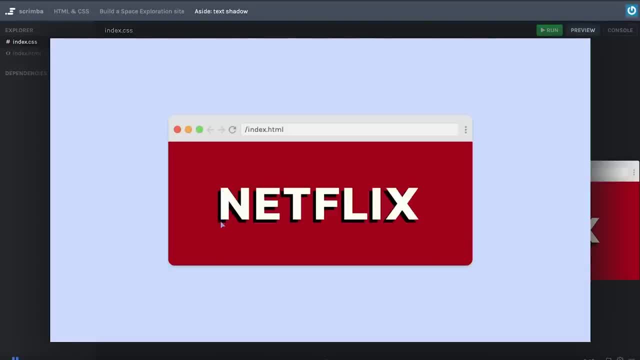 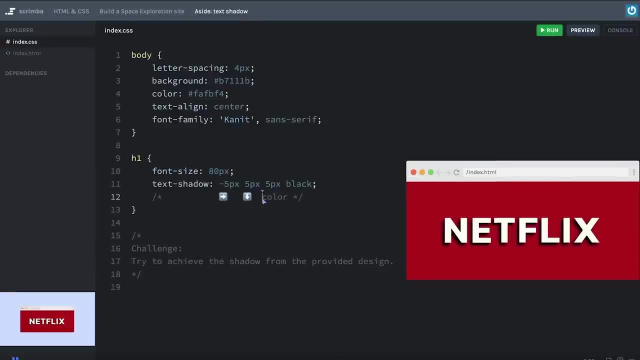 that value. you can see that previously the edges of the shadow were sharp, there was no blur, Whereas here they're kind of fading over into the red color behind it, And this is called lure. If we reduce this one to zero again, the edge is sharp again. Now, if we 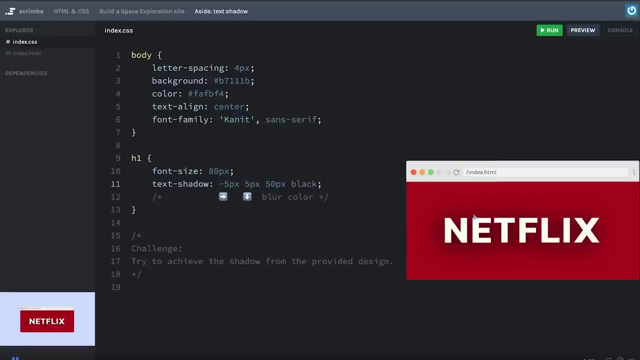 do something crazy like 50, you can see that it is so blurry that it just looks a little bit like background is a little bit dirty. So let's get it back to zero again here. What I want you to do now is try to achieve this shadow. Go ahead and give that a shot right now. 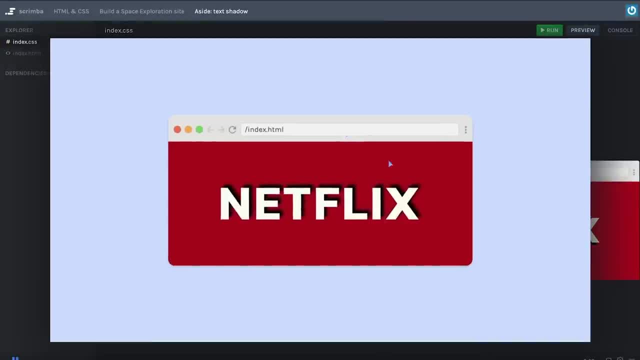 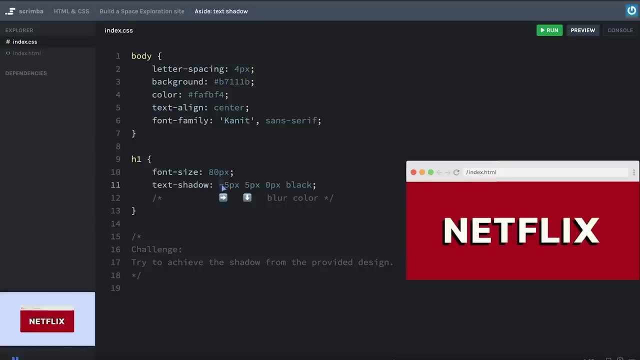 Okay, hopefully that went well. Let's have a look. You can see the shadow is above and to the right of the letters. Let's fix that first. To have it on the right of the letters, we need plus value on the first one. we want to push it to the right And we're going to 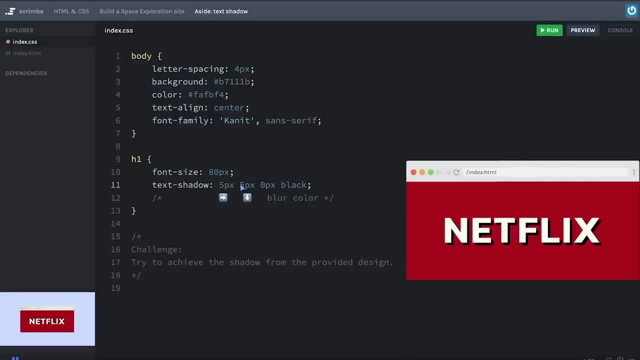 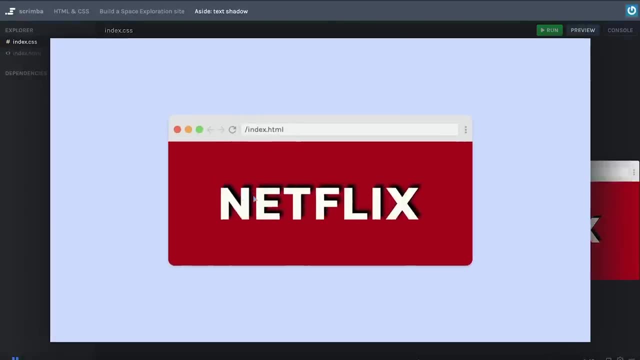 have it above, as we don't want to push it downwards, As we're doing with this value, is we want to minus it, pushing it upwards like that? And now the only difference is that this is a lot more blurry, whereas this is completely sharp, So let's try five pixels. 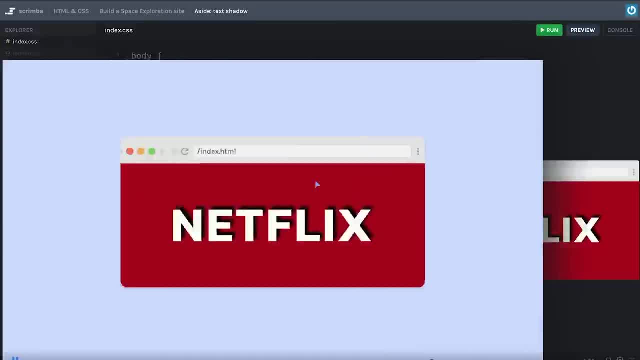 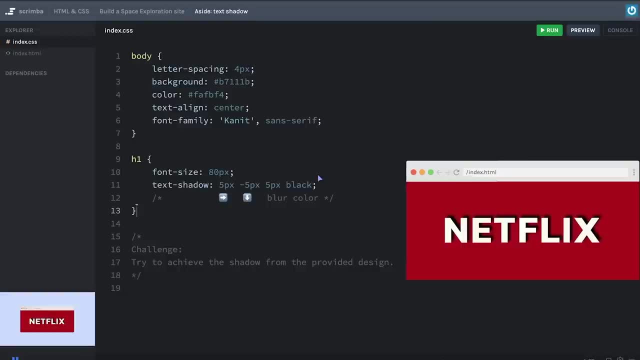 here as well And boom, there we go. That looks pretty correct to me, So great job doing this challenge. before we move on, I have just a final trick I want to show you, which is a little bit of a hack but super useful, Because let's say that, for example, the background here, 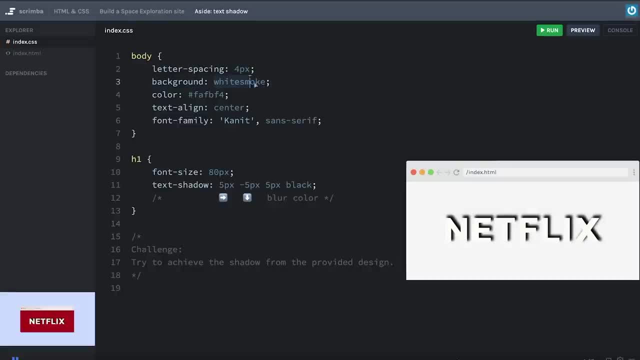 was white smoke instead of the red color, And white smoke is a very white color with just a little bit of gray in it. As you can see, it looks really bad Now. we can hardly see the letters. we can clearly see the shadows If we now set zero pixels on the two. first, 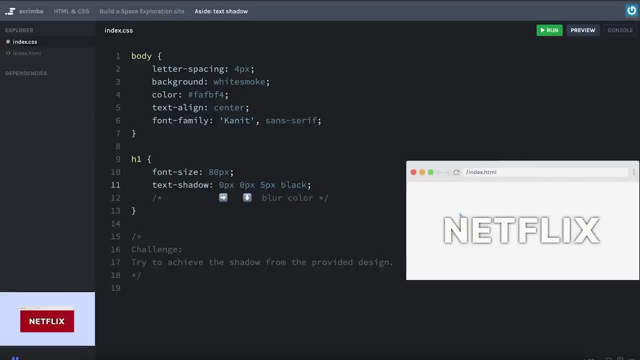 values but keep the blur. well then, suddenly there's no shadow, but there's just a glowing effect around the letters, making them visible, even though they are in almost the same color as the background. And if we make this smaller, for example one, you can see the line around. 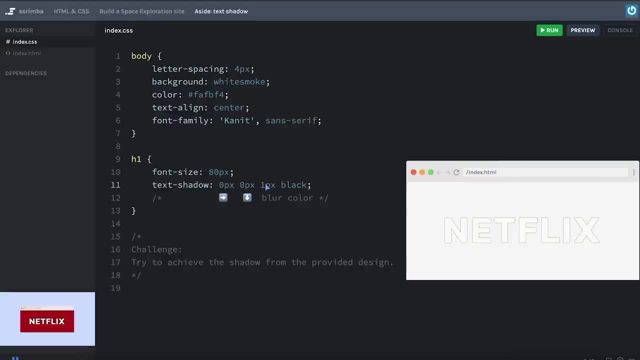 the letters look a little bit sharper since it's very little blur. Now, if we do like 20, each letter gets a lot of blur around it and thus making them visible. So that is a little trick to use, Normally, with small values on the blur in order to make your text stand out a little. 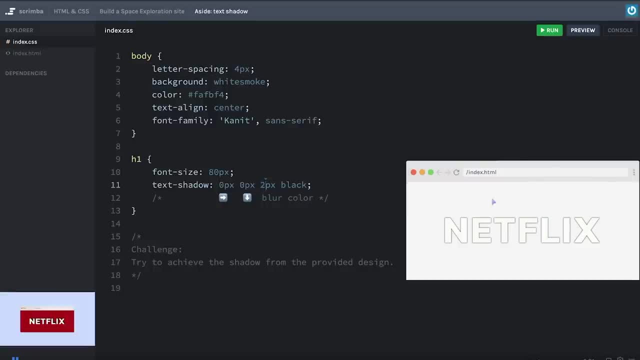 bit more in the situation where your text color and your background color is a little bit too similar, And this is very relevant if you have a background image in which the contrast between that image and the text color is a little bit too weak, So then you'd use 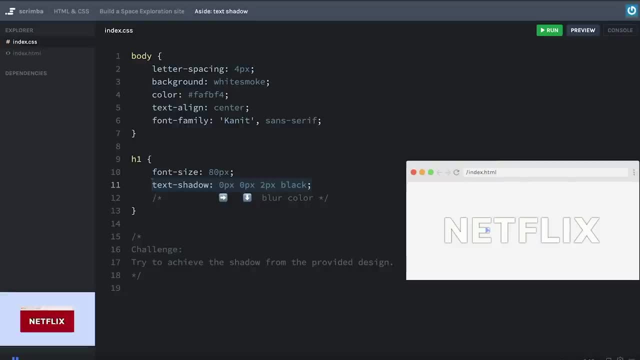 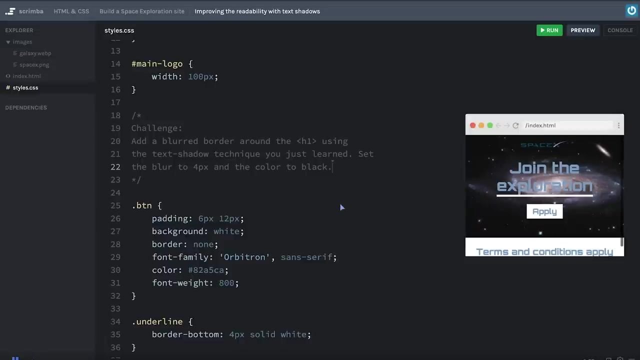 this hack to make your text stand out despite the similarities between your text color and the background image. So that was quite a lot about text color, But now you know it. so we are ready to move on to the next scrim. Okay, now we are going to fix this problem of the text blending too much into the background. 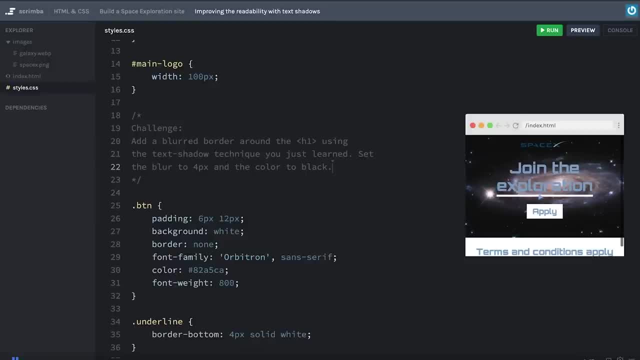 when it is broken into two lines and thus are located exactly over the galaxy in the background image here, because the readability is a bit too low now in my opinion, And I want you to fix that by adding a blurred border around the h1 tag using the technique you've. 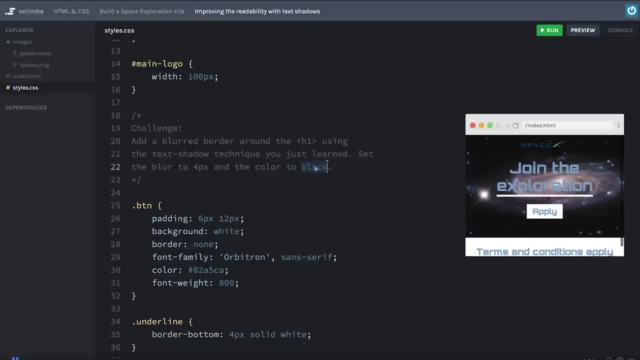 just learned you should set the blur to four pixels and the color to black. So go ahead and do this right now, Then I will show you the solution as well when you return back to me. Okay, let's do this. So first we need to select the h1.. And we've been really good. 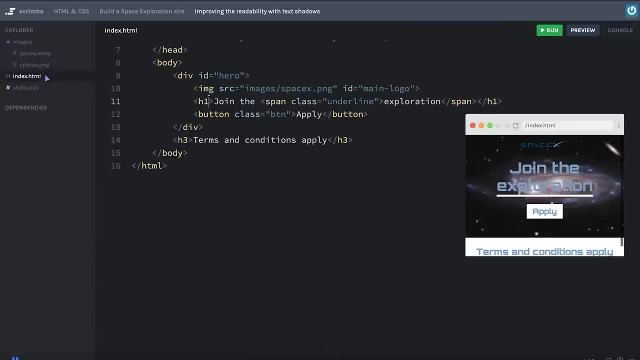 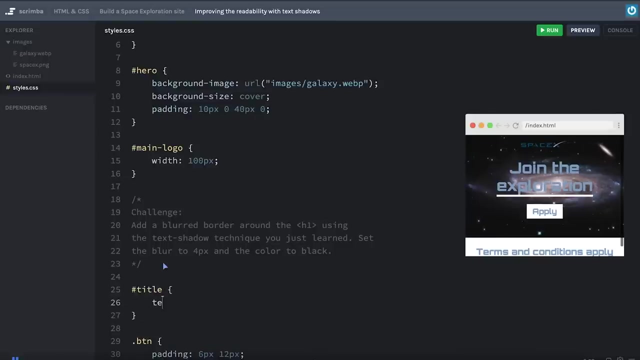 at using IDs and classes here. So instead of just selecting the element, I'm actually going to give this one an ID of title. We probably only have one title on the page, So running this and navigating back into the CSS file, I can select the title, And then I need to use the text shadow property. 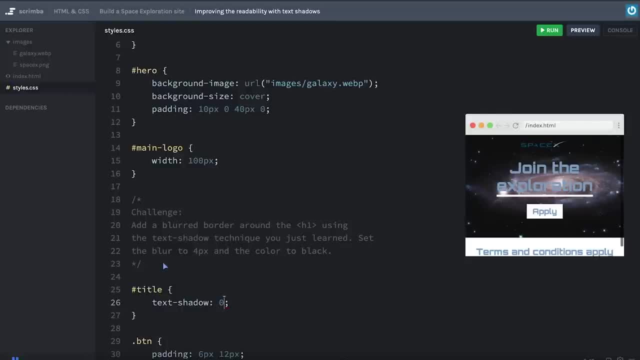 We want both the horizontal offset and vertical offset to be zero pixels. We're not actually doing creating a shadow here. the effect we want is more of an outline. So then, without any offset, but four pixels blur, it'll blur a black shadow ish effect around the entirety. 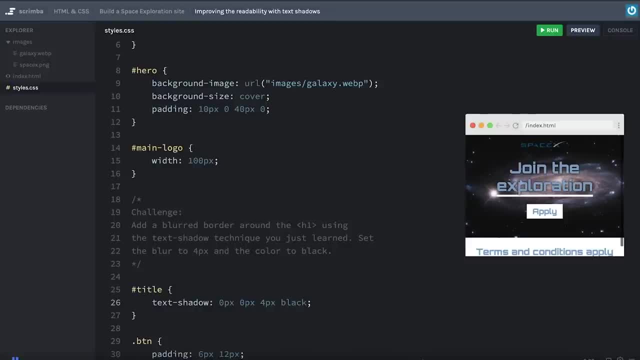 of all the characters. So if you look at it now and look closely, there is a slight blurred black border around the letters. It's not that easy to see, But if you now look at this while I comment out that CSS rule, you'll see the difference. So keep looking at the exploration word And 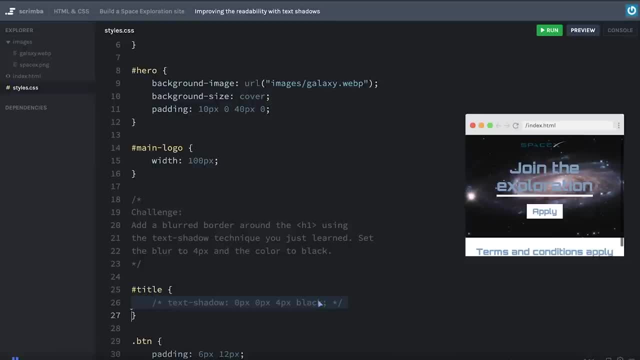 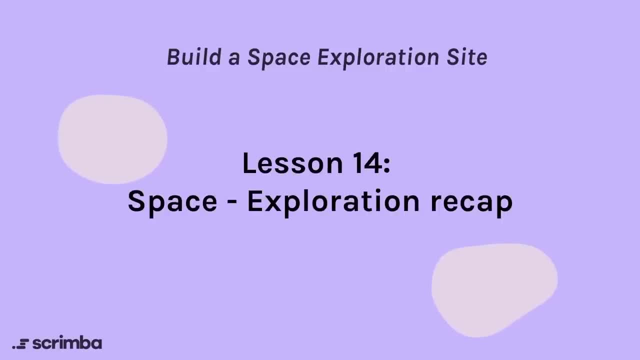 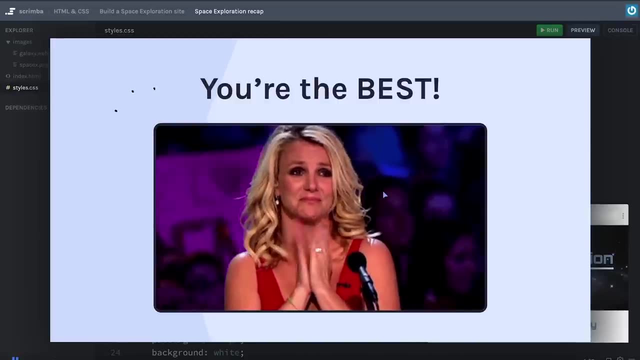 So now the readability is a little bit better. Great job Now. I'm not sure if you're aware of this, but you're the best because you've completed this section, And that is very well done. Plenty of people who have started this section has never completed it. You're not. 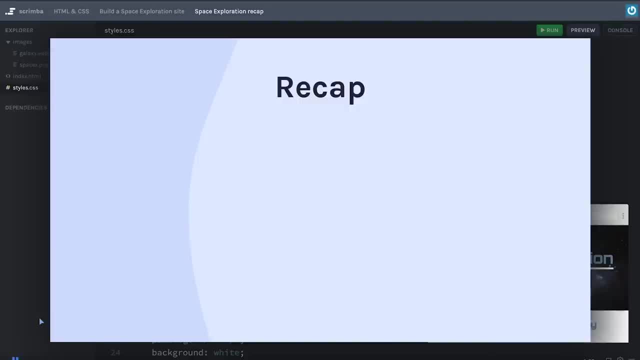 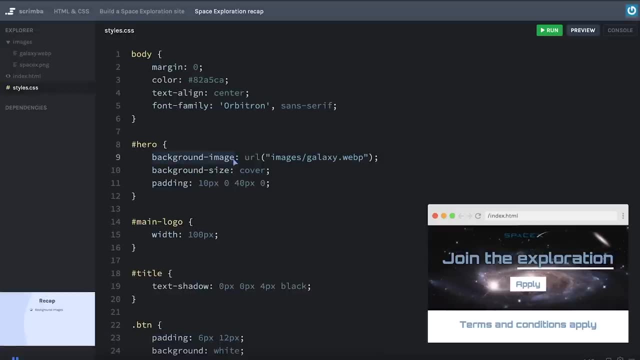 like them. So I am really proud of you, And let's take a quick look at what you've learned. Starting out, you learned about background images. More specifically, you learned about the background image property and the URL function, and also the background size property. 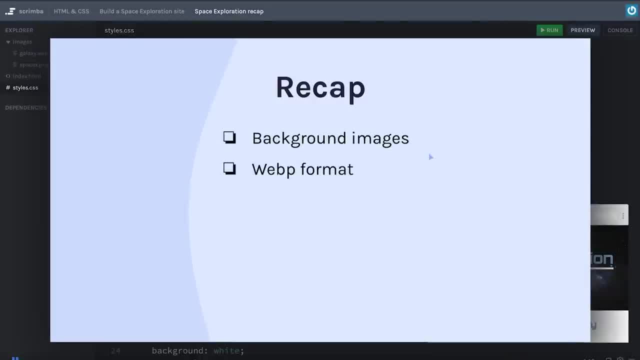 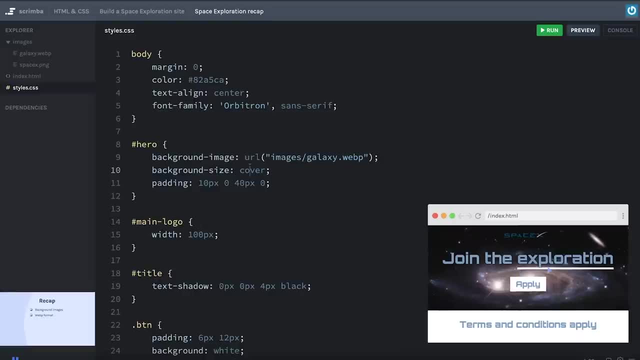 in CSS and setting that to cover. We also then used a web P format in order to get this animated image in our hero section, which is super cool and really breathes life into our website. And then you learned about Google fonts. we imported them up here in the head. 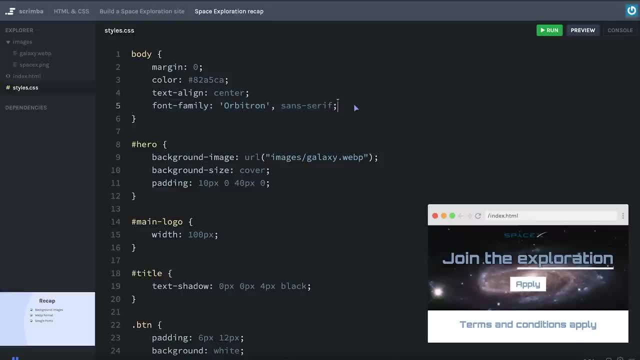 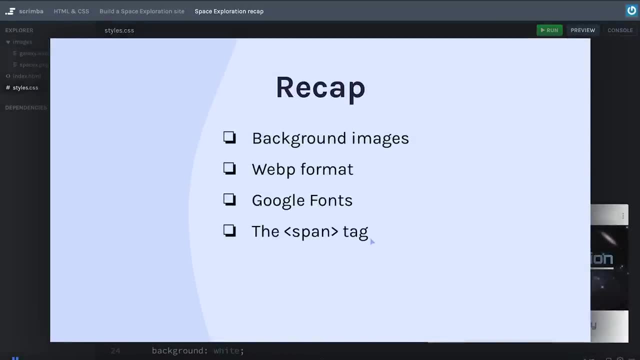 section, and then you set the font family like this. fonts do so much for the design of websites, So this is an important thing to know as a web developer. And you also learned a new HTML tag, which is the span tag, which you can see right here. it is what allowed. 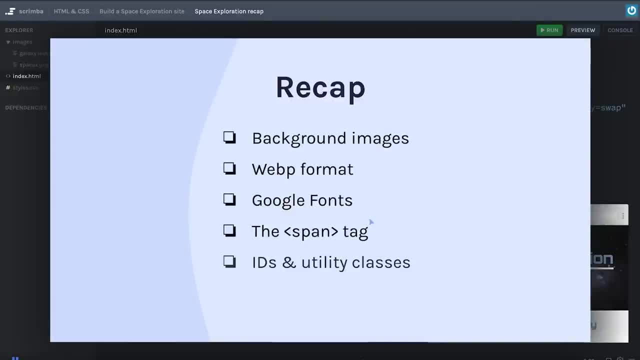 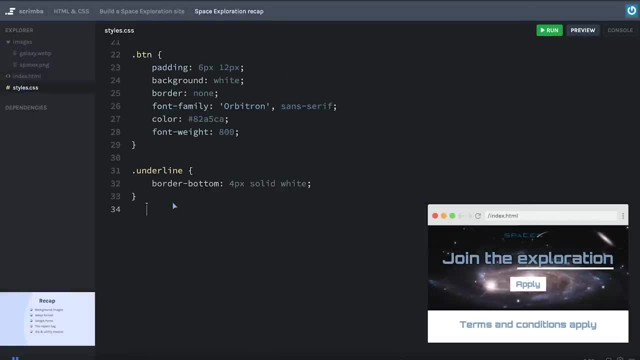 us to create this underline under the expiration word, which you did in combination with a utility class, the underlying class, which only has one job and that is to set the underlying whatever element it's applied to. And then also, we learned about IDs, which is another. 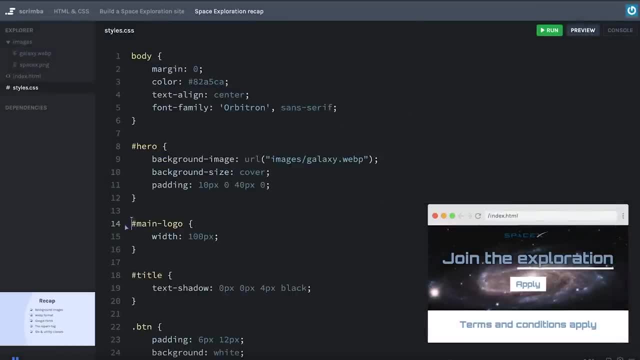 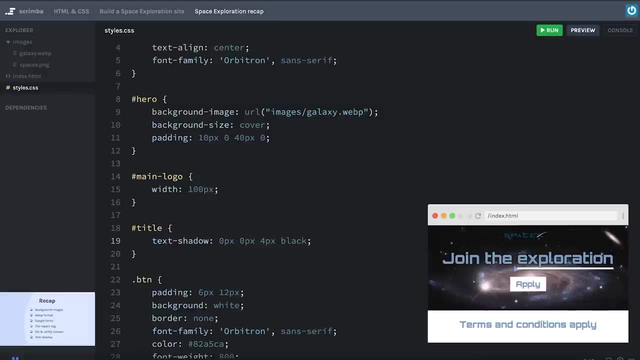 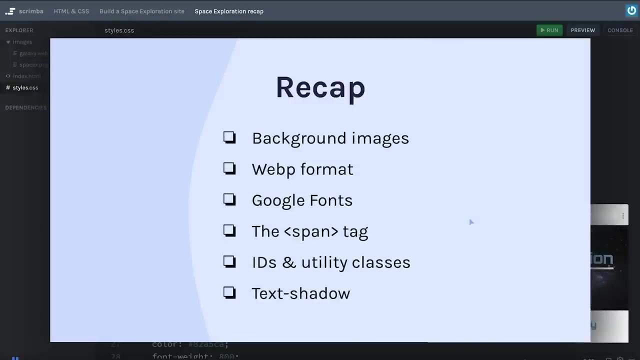 attribute in HTML that you target in the CSS using a hashtag. And at the very end, we did a really cool trick with the text shadow property in order to make the readability of our title here a little bit better. So you've learned some key concepts in this section. now is the time for you to get up, stretch, maybe get a cup. 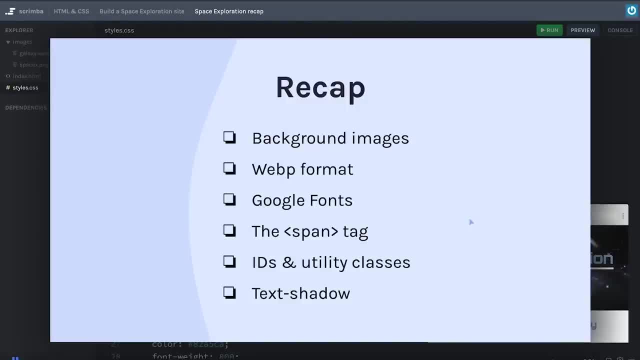 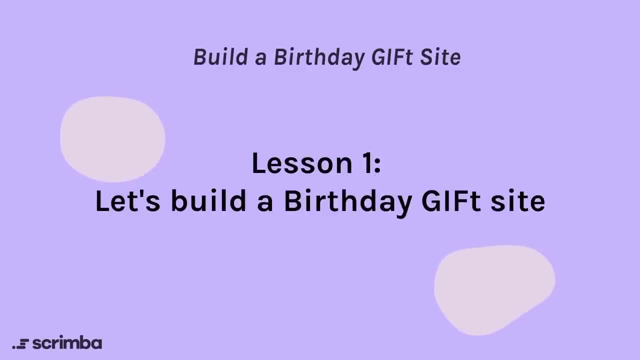 of coffee or whatever you prefer to recharge, because be sure to do exactly that, And then I will see you in the next section. Welcome to this section where you are going to build a birthday gift site 00, 00, and it is a really. 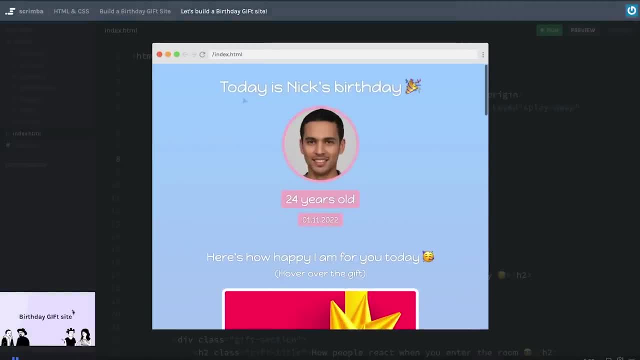 just so cool, because this site is something you can use for whenever a friend or family member of yours has a birthday. So what you do is basically add their information to the header here, And then we have these gifts. So, for example, this one saying here's how: 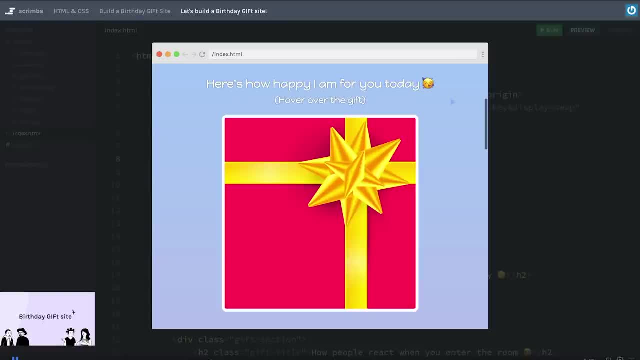 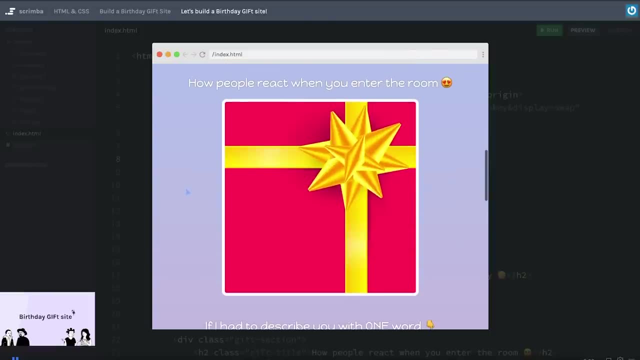 happy I am for you today, And when the birthday boy or girl hovers over the image, they will see a nice gift that makes them feel truly appreciated. Going down, we have other gifts. how people react when you enter the room. Oh, this is meant to make them feel really. 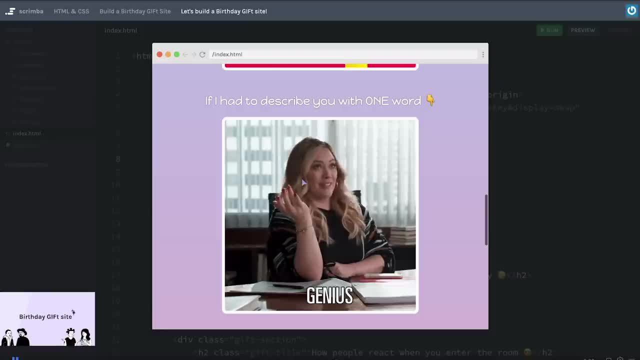 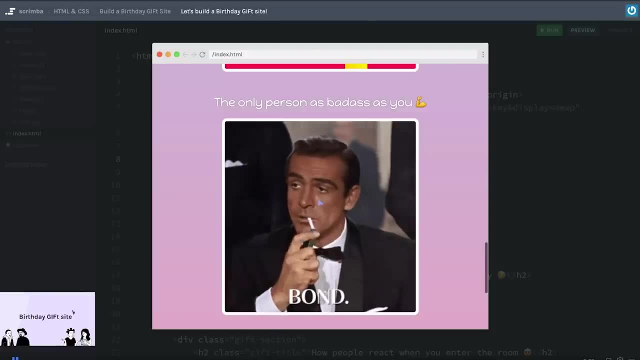 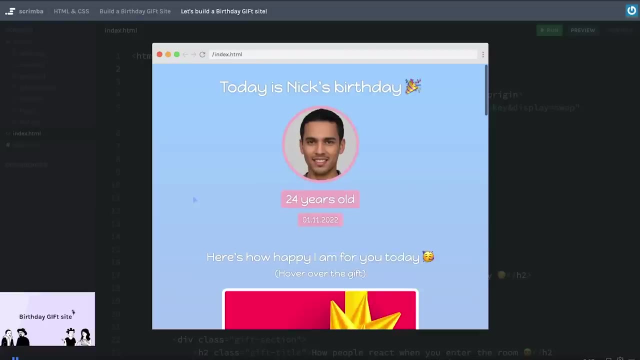 good looking And here, if I had to describe you with one word, genius, so you make them feel really smart. Next up, the only person as badass as you is, of course, James Bond, and then rounding it up with a little toast, So hopefully you have someone special to send. 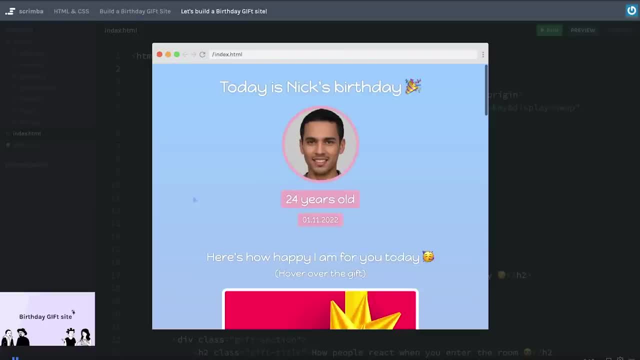 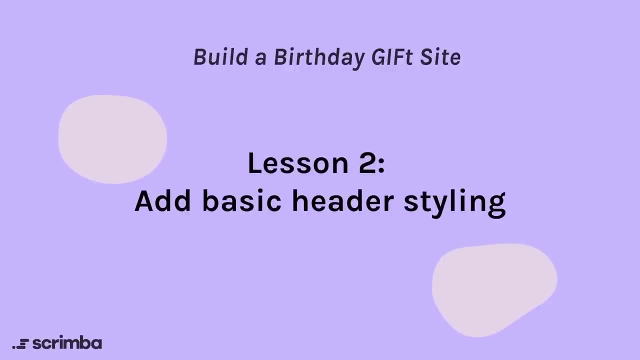 this site, to like Nick here, for example, who, despite being a computer generated image created by an AI, also is one of my favorites, My best friends. So I am looking forward to make Nick happy on his birthday. Let's just get started with this section. Okay, it's time for your first challenge. what you're 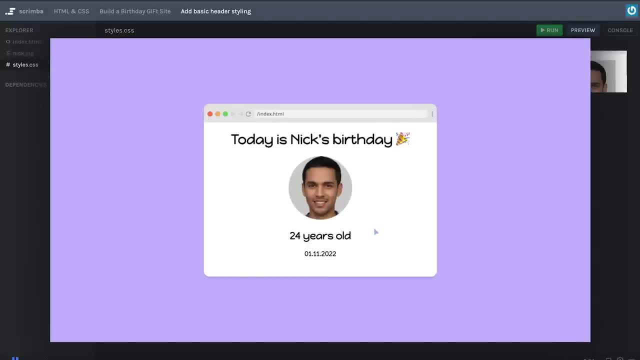 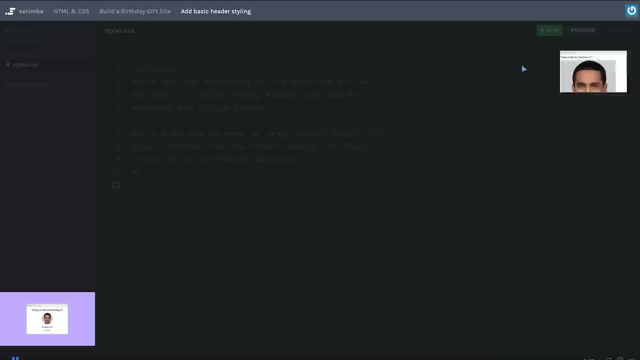 going to do is create this basic design here for the header of our app, And it's pretty far from what we got right now. As you can see in this stylescss, we have no styling at the moment, So our site looks pretty dull. You can see. everything is left aligned and 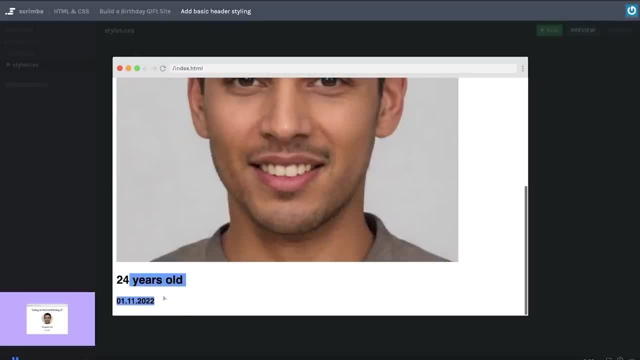 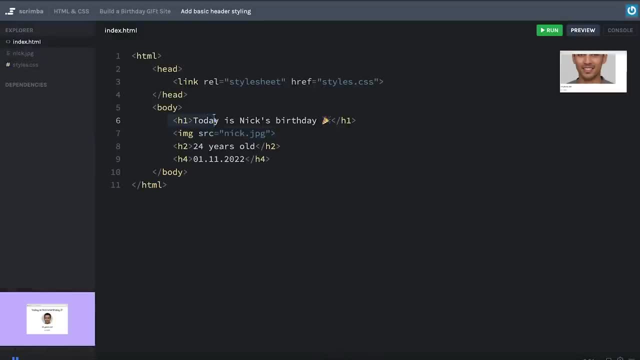 inside, And then we also have the background image here So you can see it should look like this. We only see of the белорусов in the background. You can see how we have added the little white lines there. The bottom edge of Nick is far too large, Plus, we're lacking. 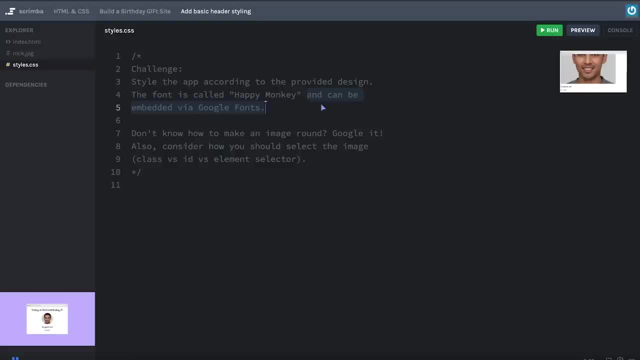 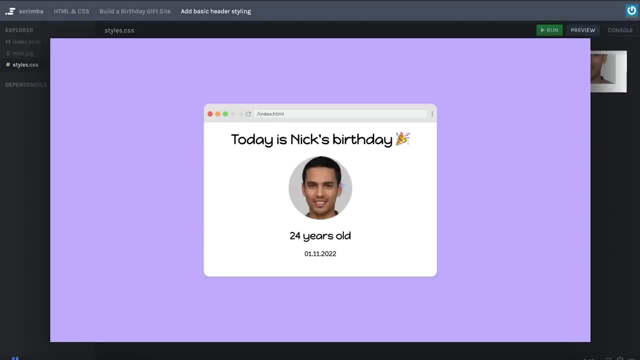 the appropriate font. taking a look at the HTML here, it's just a very simple structure with an h1, an image tag, an h2 and an h4 inside of the body. So nothing special there is right now. So you will have to figure out how to make an image round. And yet again, 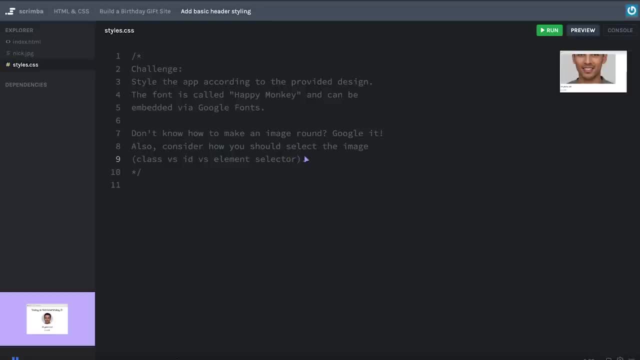 you'll find the answer if you google it. Finally, I want you to consider how you should select the image. So should you use a class selector, an ID selector or an element selector? you can use any of them, But I want you to think about it and try to figure out what you think. 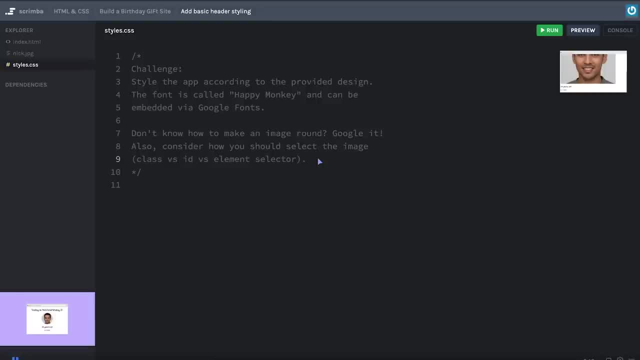 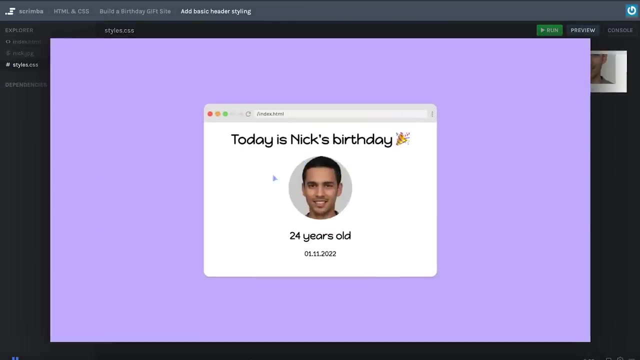 makes most sense. Go ahead and do this right now, And then I, of course, will show you the solution when you return back to me. Okay, hopefully that went well. Let's do it together. I want to start with centering everything, And for that I'm going to do body, then set. 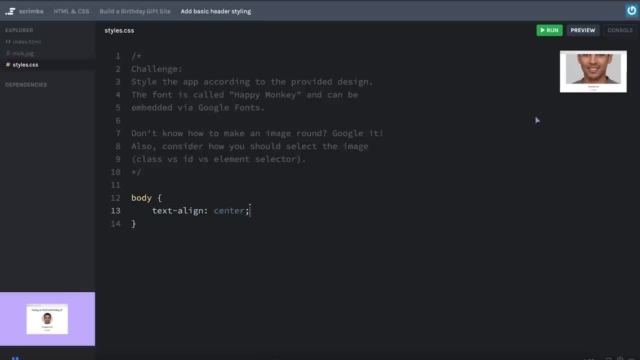 the text line to center like that. See that, indeed, centered our elements Next up. I want to fix the image. It is here And I think it makes sense to use an ID selector here, because this is kind of the main image of our birthday boy And 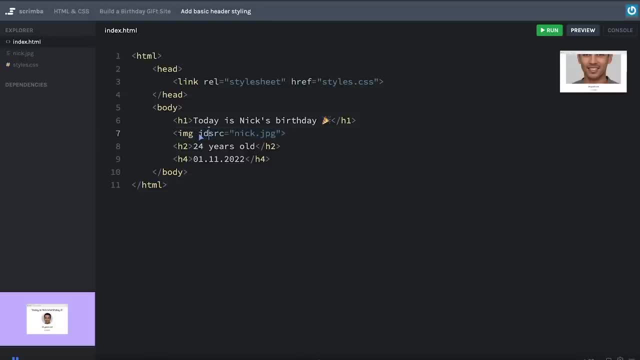 I don't think we'll duplicate it across the page, So it is unique, meaning we can use an ID. So I'll do ID equals. and then BFF for best friend forever, because Nick is my BFF. Please don't make fun of me because my BFF is a computer generated image, But that 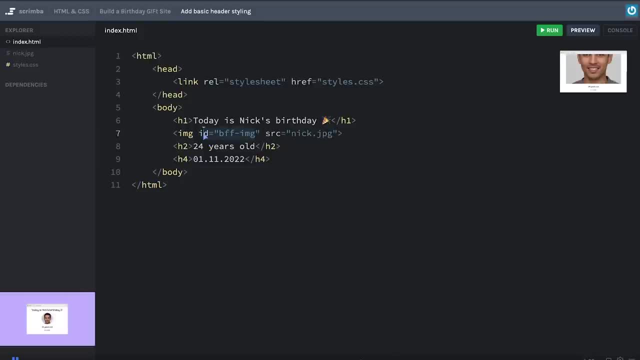 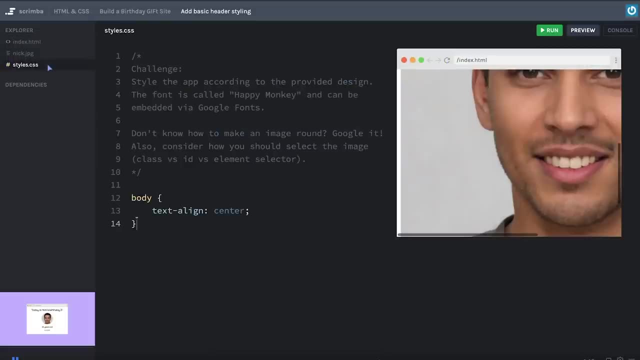 is just how it is, And then I'll do dash IMG just to make it a little bit easier to understand what it is based upon the ID name. Then I'll run the code So that that is applied to the DOM And, heading over to the styles, I'll do hashtag, BFF, dash. 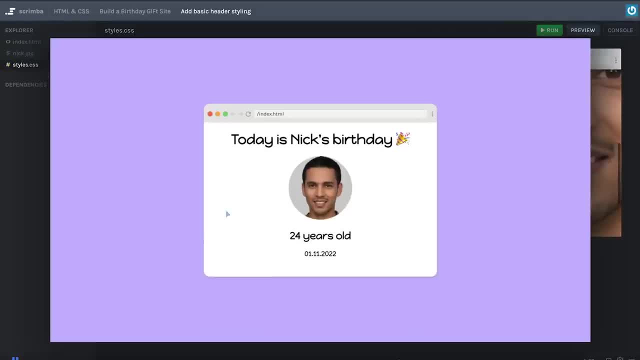 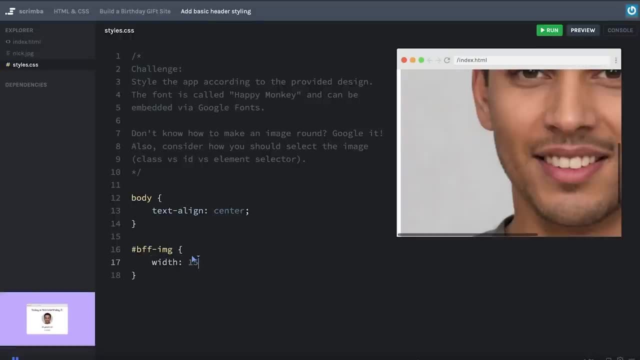 IMG like that, And first I want to fix the width of it. it's far too wide. This looks more like 100- 200 pixels, So let's try with 150 pixels like that. Yes, that is pretty much what we're looking for, And hopefully you figured out how to make an image round. 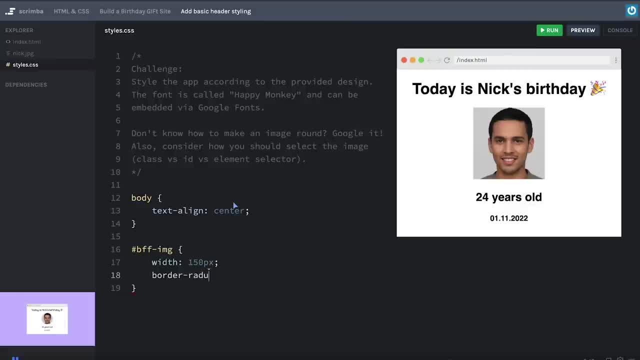 And the way to do it is to use the border radius property, which you've seen a couple of times by now, And the maximum border radius an element can have is 50%. And boom there, it is completely round Alright. the final part is to add the Google font. the happy. 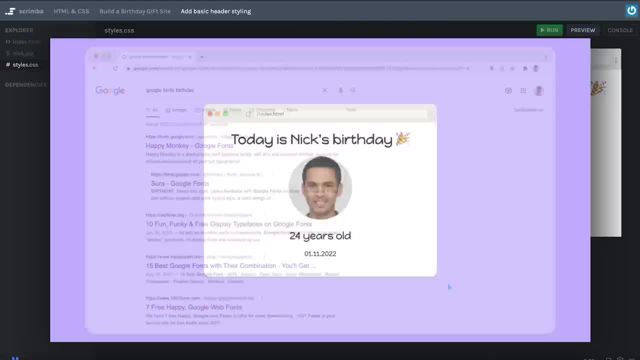 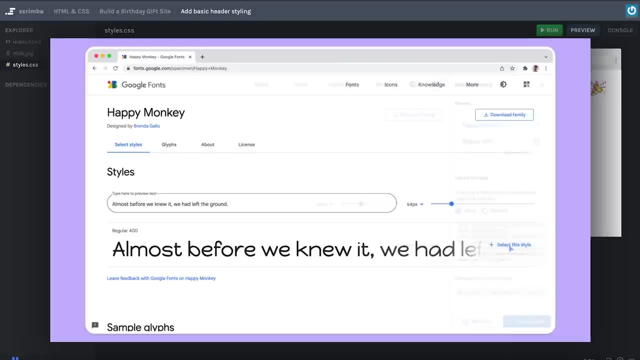 monkey font. That is a very birthday ish font. Actually, I found it just by googling Google fonts- birthday. then happy monkey was the top result. Clicking into that, we'll select it by clicking select this style And then we'll copy the links here so that we can embed. 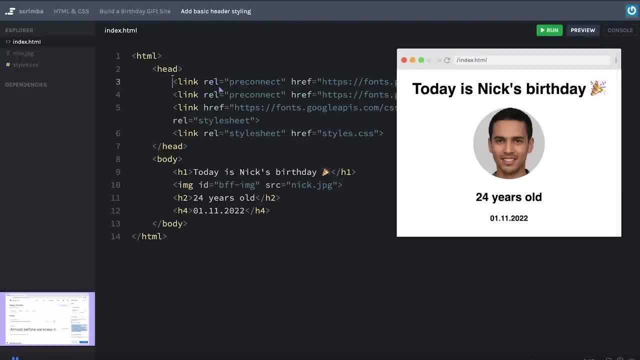 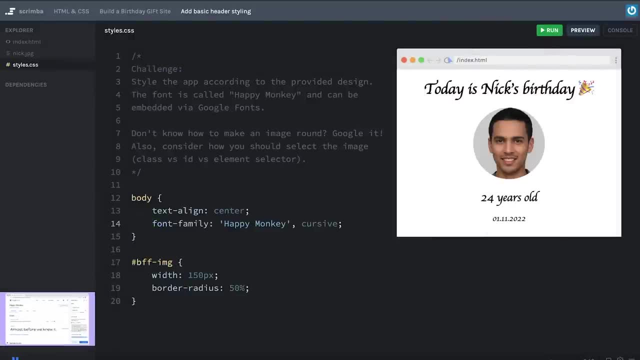 it into our project. I'll paste that into the head of our project, then copy the font family rule, so that I can paste that directly in as well. Now I'll have to rerun so that the font is embedded. And yes, there we go. That is, as far as I can see, exactly the design we were looking for. 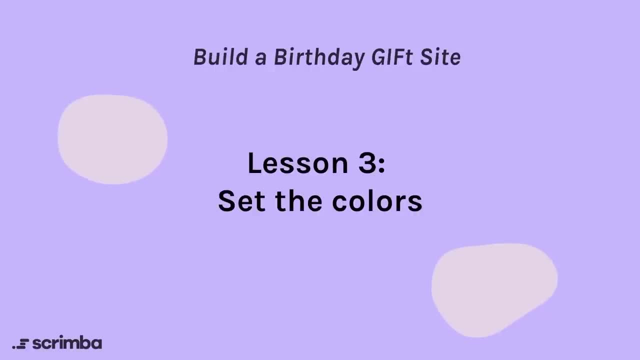 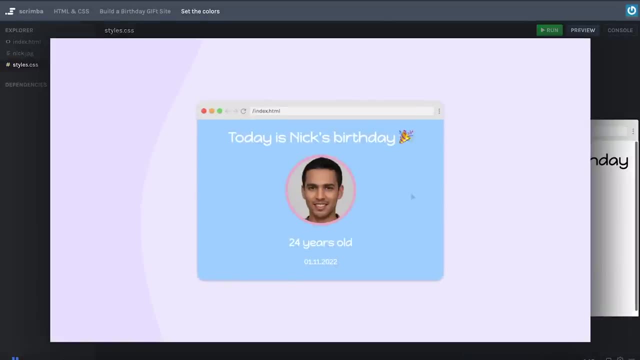 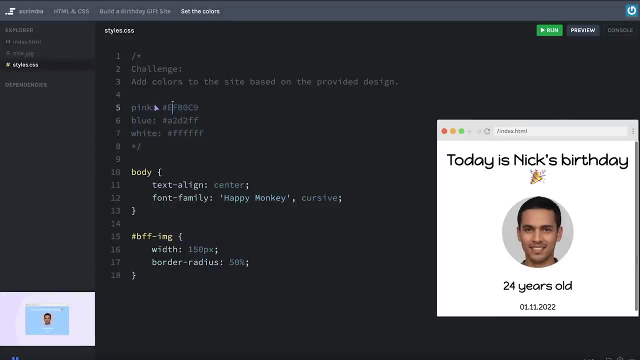 So great job, Let's move on. Okay, your next challenge is to colorize the app, because I wanted to look like this, with a nice blue background, Pink border and white text And, as you can see, I've provided the hexadecimal values. 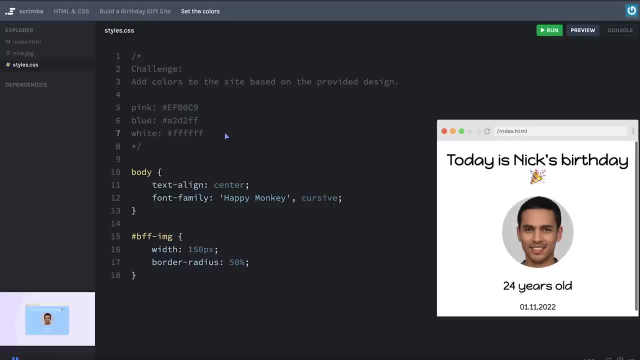 for the pink, blue and white colors here. So your job is simply to figure out where you need to add these and what kind of CSS properties you're going to use. Go ahead and do this right now. Okay, hopefully that went well. Let's do it together. I'm going to start here in the body. 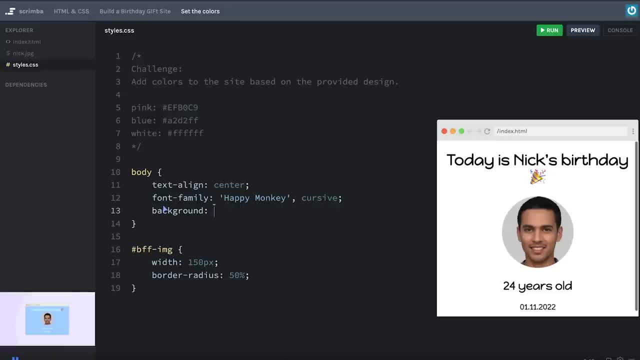 taking the blue hexadecimal value and setting it as the background of the body. Boom, there we go. Next up, we want to set the color property here to white, just just six F's after each other, Like that. Now that is inherited down. 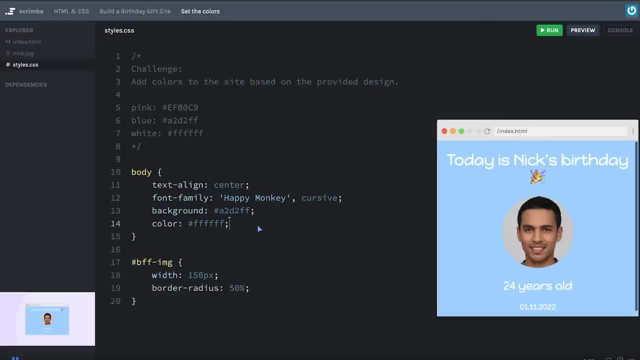 from the body into all of these. Okay, final step is the image. As you can see, it should have a border around Nick and it should be pink. So here we'll use the border property And let's try six pixels. 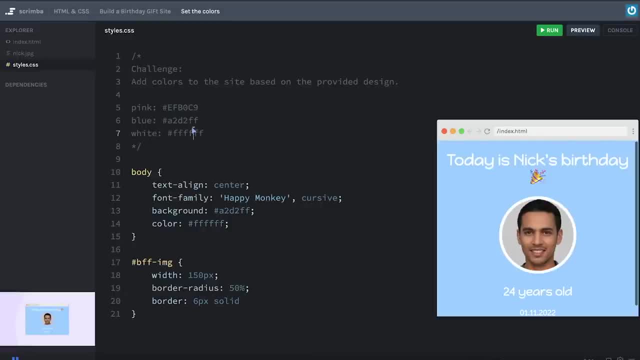 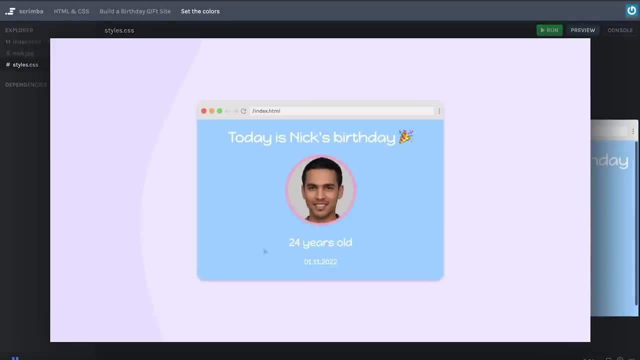 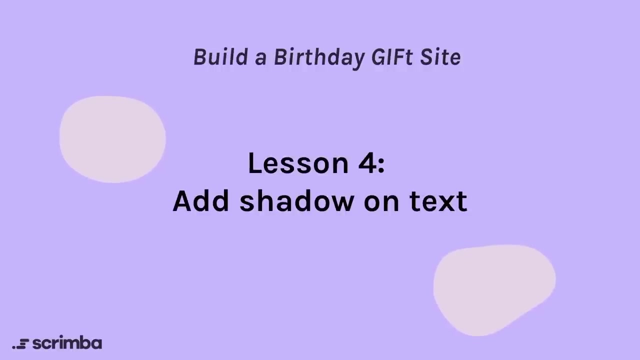 Because it looks pretty thick. it should be solid. Then we'll copy the hex value from pink and paste in right there, And actually that looks about right to me. So great job, Let's move on. There is one problem with our site at the moment, which is that if we run these two, 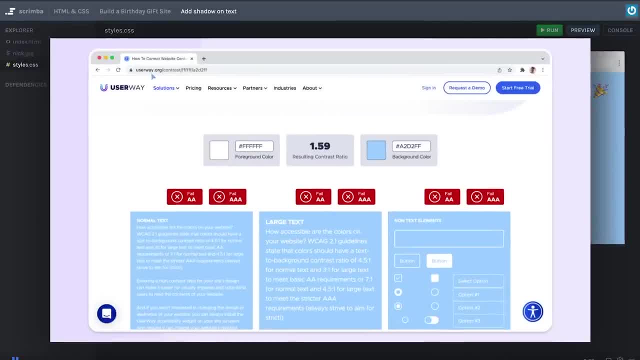 colors. through a contrast checker, for example userwayorg, you'll see that our accessibility actually fails Because the contrast ratio is too small. So what can we do to improve this, given that we want to keep the colors we have? what we can do is use the trick you learned in the 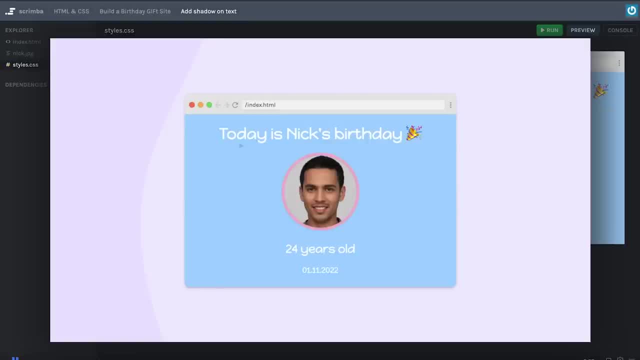 space exploration section. Because pay attention to what happens to this text If we add a thin black border around the text using the text shadow property. So this is without the text shadow property And this is with it. As you can see, the text now stands out more. 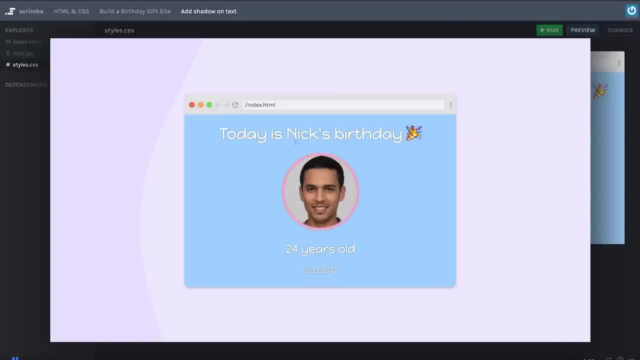 as the black contrasts Well with both the white and the blue background, and it's also pretty subtle. So the text still looks white, but it's just a little bit more visible And in my opinion, I think the readability here is pretty good. So what I want you to do now is write the CSS for this exact technique. 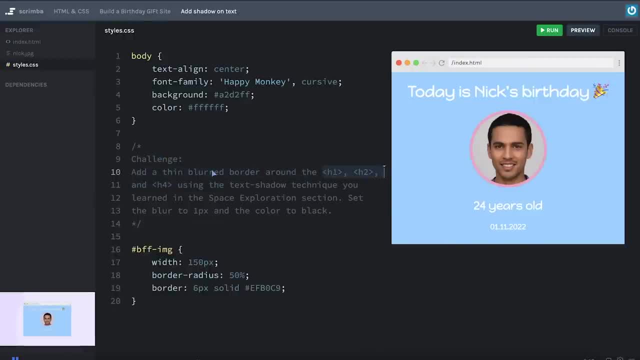 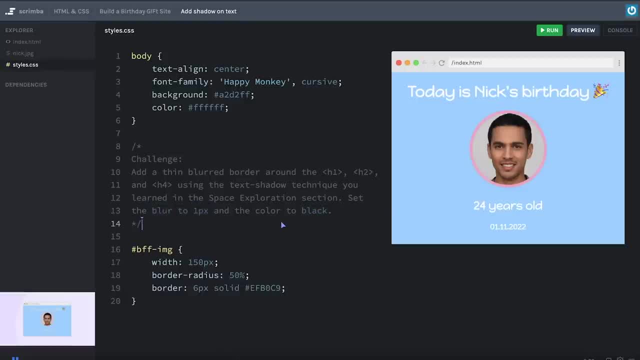 Okay, so let's go ahead and do that. So let's go ahead and do that, And if you don't remember how to do that, give it your best shot, And then I will, of course, show you the solution as well when you return back to me. 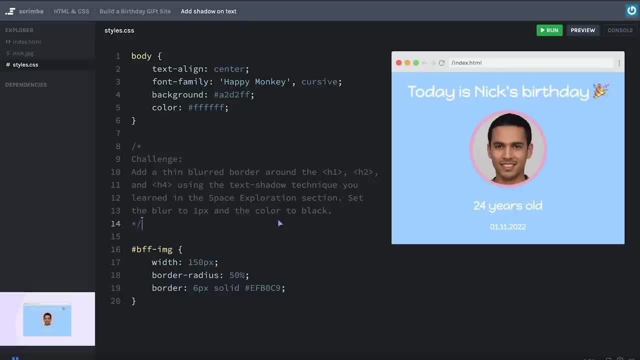 Okay, let's do this. So let's start with the h1 here, And here I'm just going to use an element selector, as we'll have a lot of h2 and h4 throughout the site And I think we want all of them to have this style, so there's no point separating it into a class. So text: 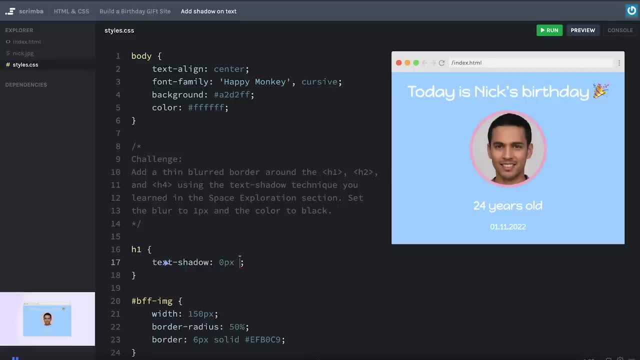 shadow, setting the first two values to zero pixels, since we don't want any offset vertically or horizontally. but the third value, the blur, should be set to one pixel, and then the color is black And boom, there we go. we have that thin outline which improves. 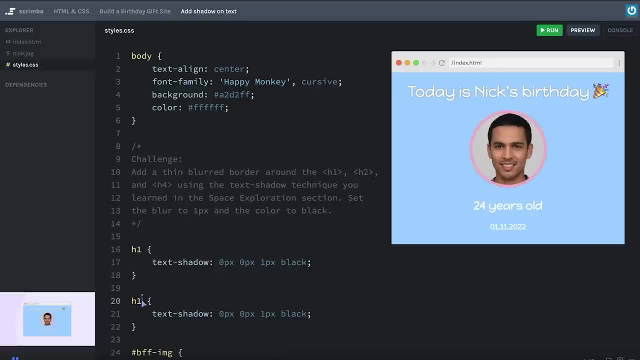 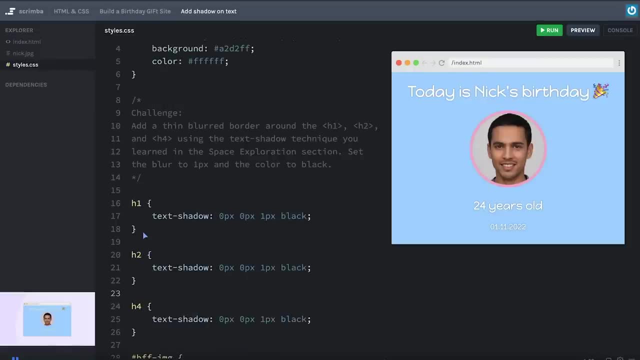 the readability, And now you probably did something like this. I added a whole new rule for the age two and yet another one for the age four, And if you did that is completely fine. That is how I expected you to solve this challenge, But I do want to show you. a little trick which allows us to reduce all of these into one line, And that is simply by using a group CSS selector, where you simply add multiple selectors on one line. So what you do is, instead of just writing h1,, you write h1,, comma h2.. Now we can delete the. 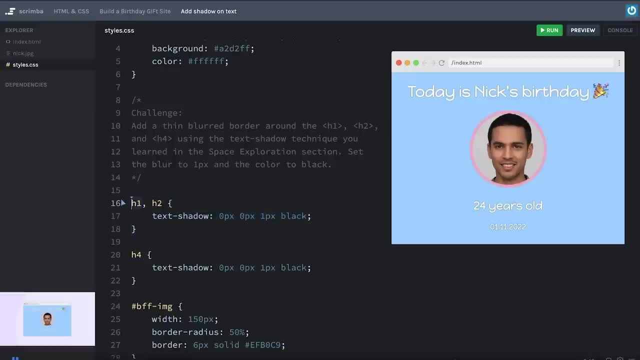 h2. Because this rule is applied to both the h1 and the h2. And likewise we can just add the age four here as well. Like that. Now we can remove all of this. As you can see, the thin border is applied. 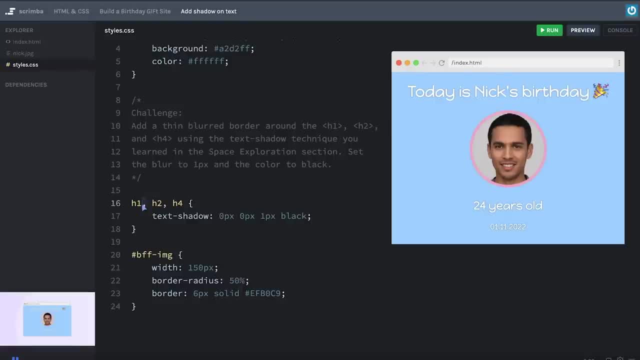 to all of the elements. Now, it is really important that you actually use a comma here and not just added like this: this means something entirely different And we're not going to learn about that right now as it's outside of the scope of this section. So make sure. 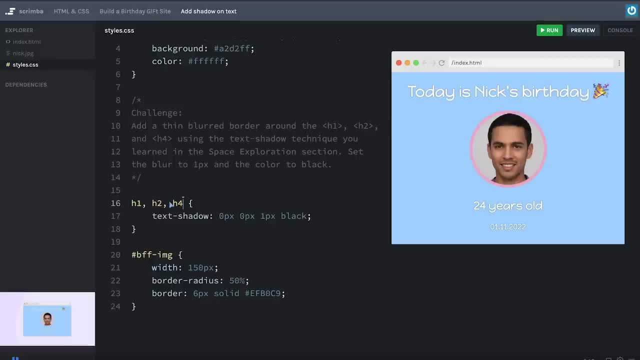 you have the commas And then you can use this technique, And I happen to know that we also want this text shadow to be applied to our h3 elements down the line and also our paragraphs down the line. So I'm just going to add them here so that we don't have to think about this as we add. 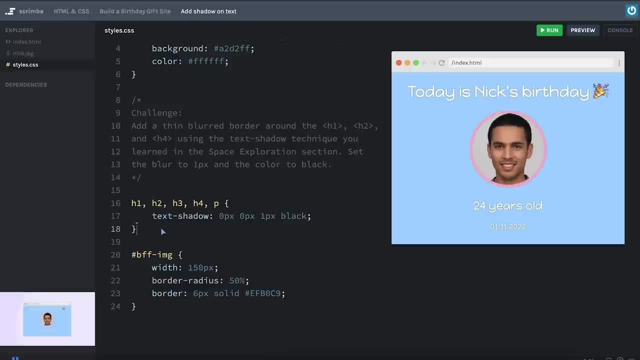 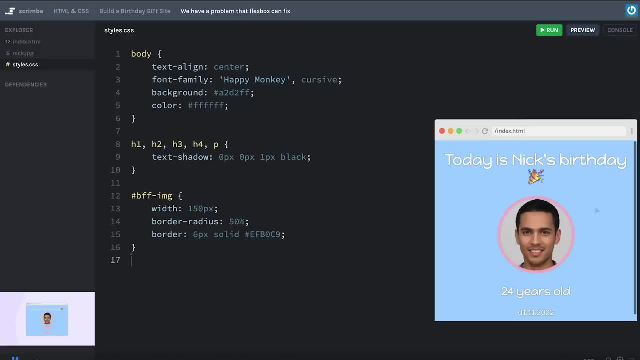 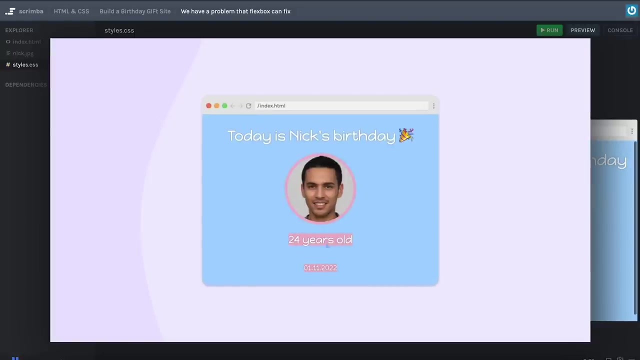 new elements to our site later down the line. So great job, let's move on Now. we want to take this pink background that we have around the image and apply it behind the h2 and the h4 element so that it looks like this. So let's try the most intuitive. 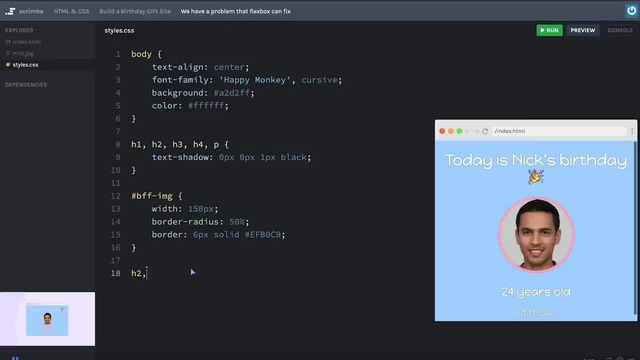 approach and see how that works. That would be to target the h2 and the h4, I'm going to use this comma selector here to target both simultaneously, as we've done up here, And then we'll set the background to this pink color right here. However, as you can, 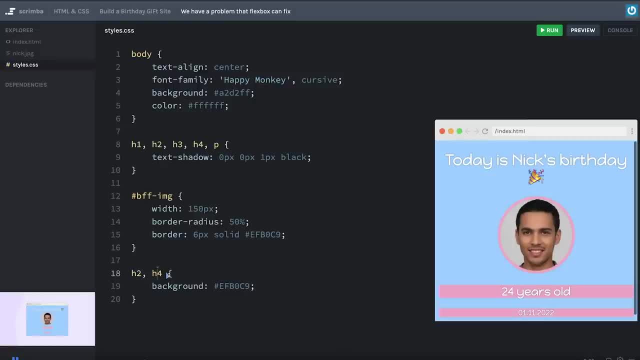 see, that did not give us what we wanted, Because heading elements like h2 and h4 are by default display block, So they take up all the available horizontal space. So let's then try to turn them into display in line and see what happens then. Ah, that did not work well either, Because 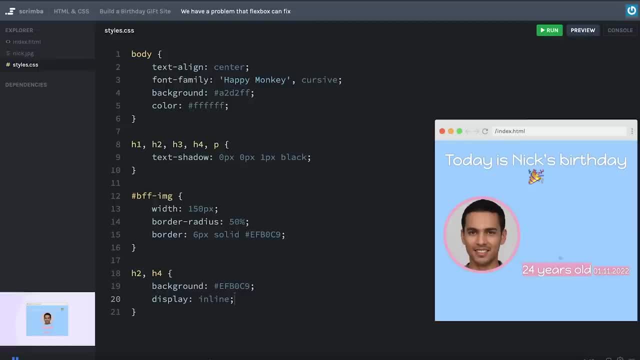 they're in line. they're actually narrow enough to be on the same line and actually jump up to the line above with the image, which also is display, in line. So let's remove the display in line as well, And the way to actually solve this is to use a technique. 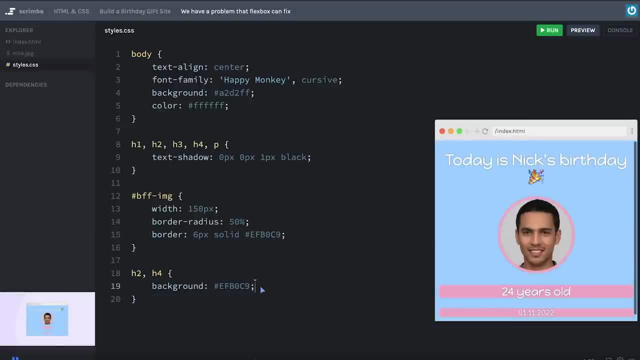 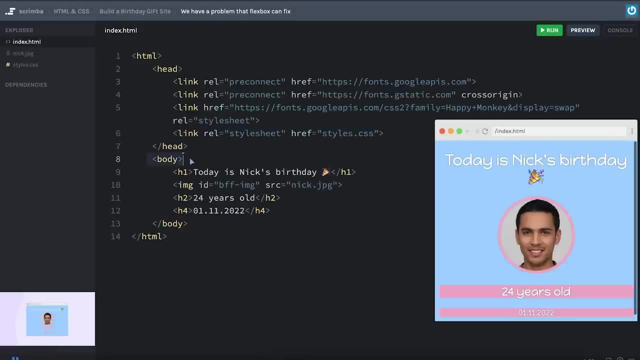 you haven't learned yet. Now I'm just going to show it to you fast, And then we're going to take a closer look at how it works in the next script, Because what we can do is head into the body, which is the container element for these two and for all of our elements. 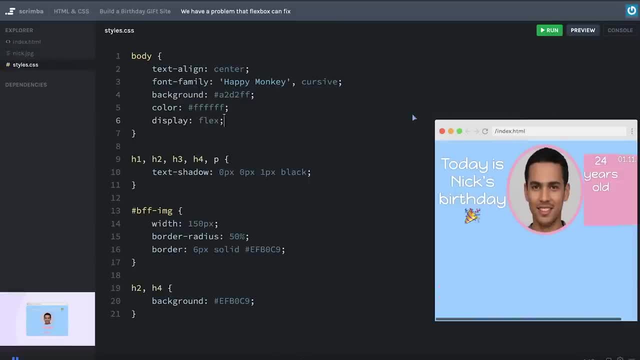 actually and do display flex. That's back things up on a horizontal line, turning every element into its own column, But we can change that by doing flex direction. Now is set to row by default And that might sound a little bit confusing, since I've always said that flex box turns every element into its own. 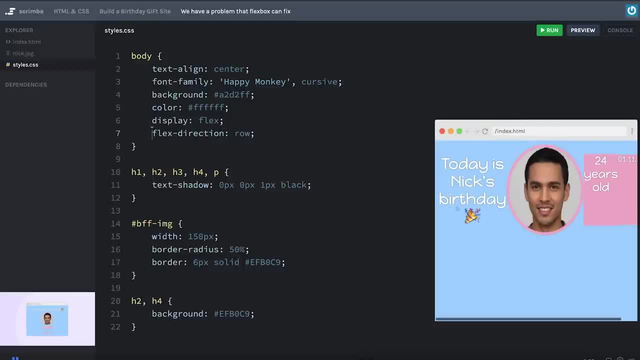 column, And yes, it does that. However, what it also does is make sure that all of the elements are in the same row. So that is why it's called flex direction row, because rows go from left to right And you can see there's only one row from left to right, And then 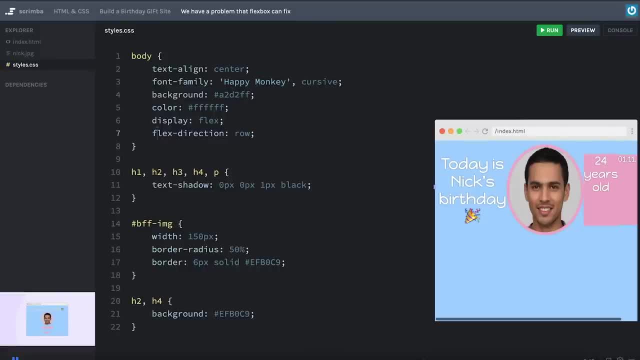 you can see here, we have a row from left to right here- which becomes even clearer if you do like this- and all the elements are inside of the same row. Now, in order to flip this, we can simply change row from column like that. Now all of the elements are stacked. 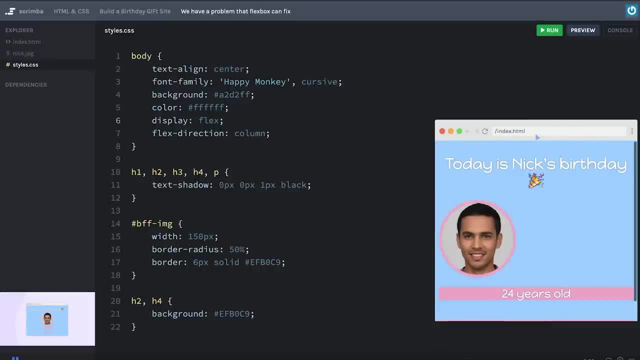 on top of each other, again in one column, because a column goes from top to bottom, So this is just one column. Now, with that in place, we can use another CSS property in that flex box give us, which is called align ash items, and set that to center and boom. 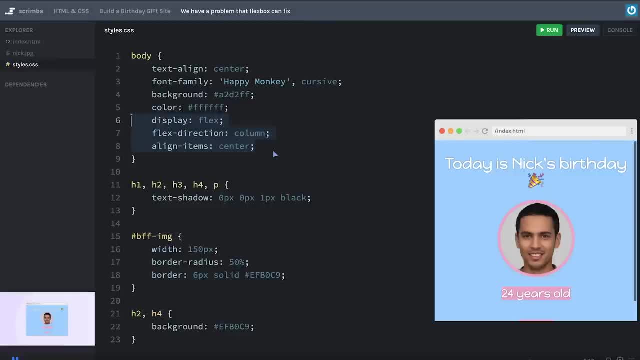 there we go Now. this was probably pretty confusing And you were not meant to understand this right now, which is why we're going to take a little digression here and look closer at how flex box works And then return back to this example, where you will code it up. 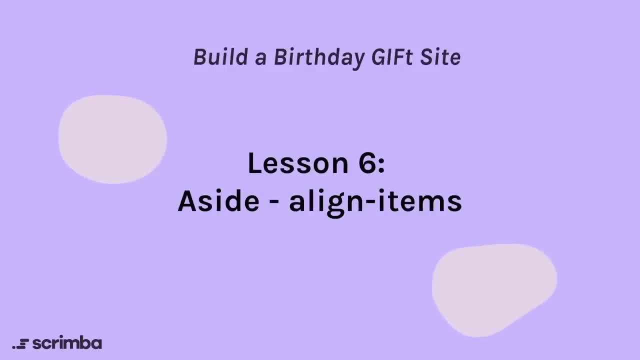 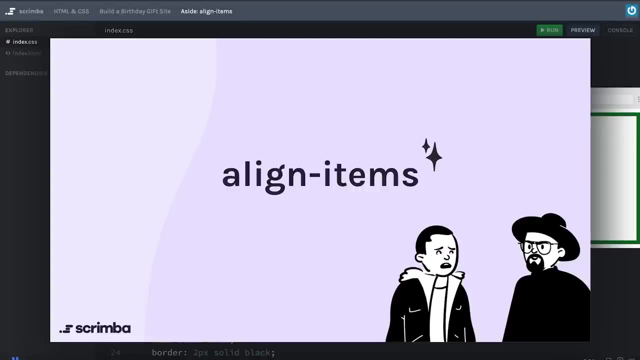 yourself and properly understand it. If you are to become a flex box master, you will need to know align items. Luckily, though, it's not that hard to learn, because it is a close cousin of a property you already know. that is justify content, So let's pretend that the two of us, for example, work in a 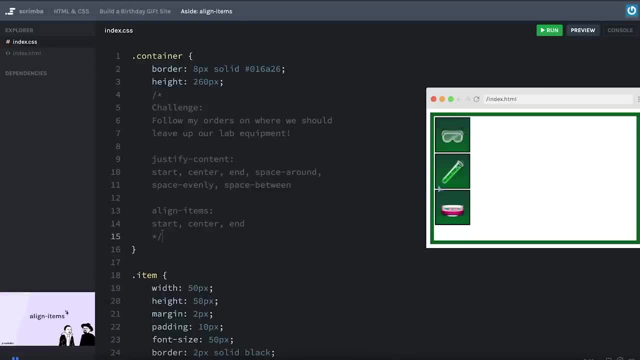 lab together. Well, if so, we'd have our lab equipment, which you can see here inside of our lab, which is this green rectangle right here, And what we're going to do now is use flex box, along with the justify content and line items, in order to organize our lab equipment. 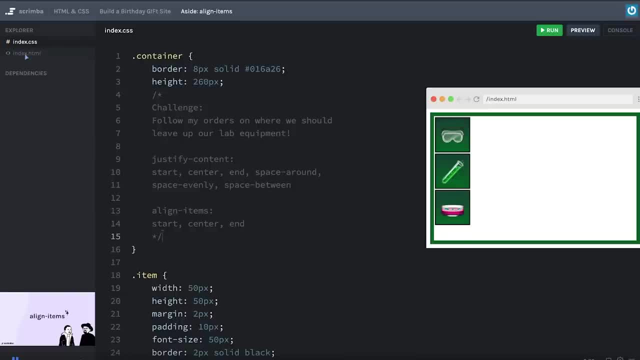 in different ways in our lab. So let's have a look at the code. The HTML is very simple. It's just a container which has three divs, And each div hold exactly One piece of lab equipment visualized via an emoji. If we head over to the CSS, you 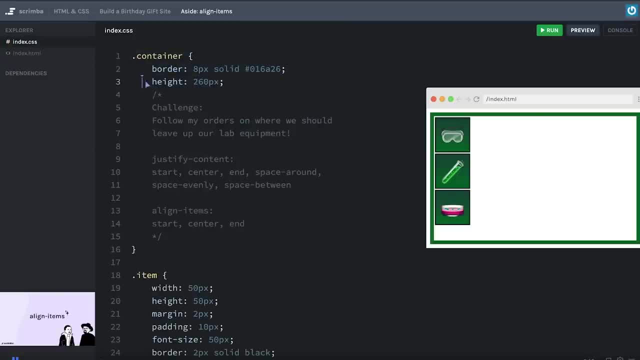 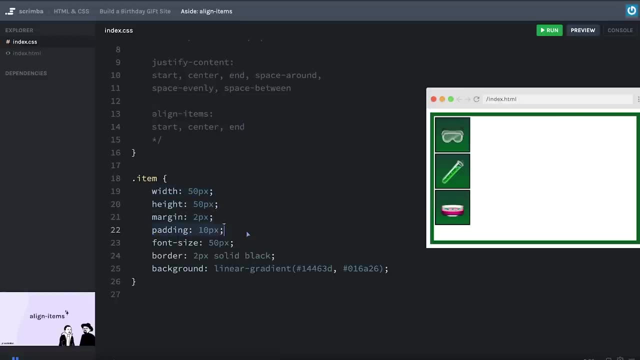 can see that the container has a border and a fixed height, So that's why we get this green rectangle. the items have a width and height. there's some margin in between them and some padding on the inside. I've set the font size and also added a border. And finally, 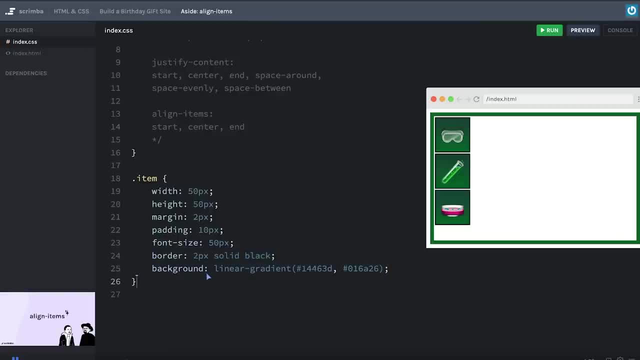 something you haven't learned yet, but I've added a gradient background so that the color slightly fades from a darker shade of green to a lighter shade of green in the background. Now you are going to learn about the linear gradient later on, So don't worry. a second. 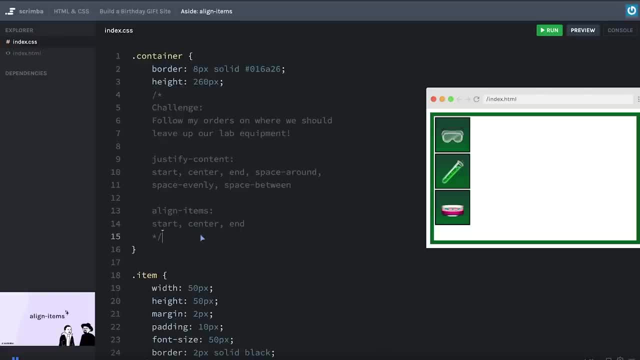 about this. right now They're just accept that it is how it is And let's get going with the organizing. So, as you can see, by default the lab equipment, the div status, are stacked on top of each other because, as you remember, divs are display block. However, 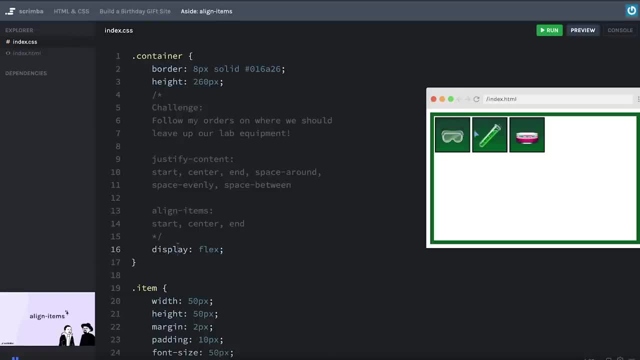 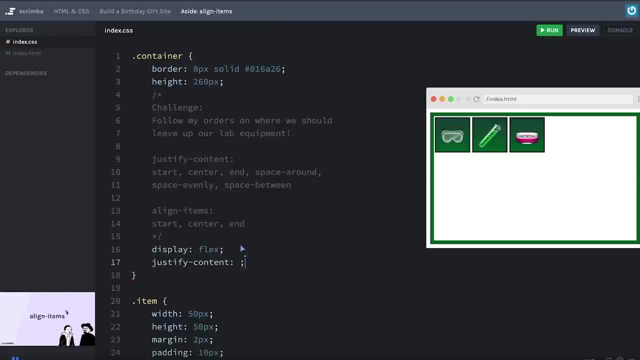 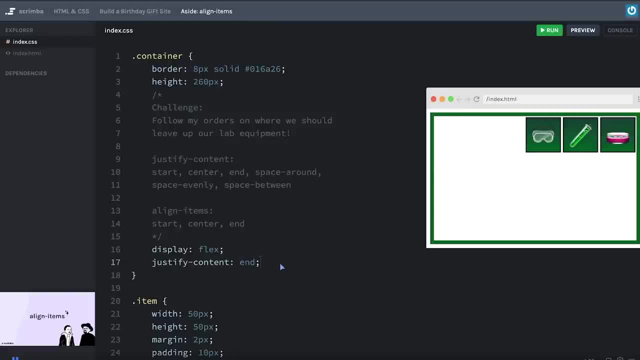 they are pushed all the way to the end. And yeah, you know the deal. So what align items does is, instead of controlling the horizontal line, which I, from now, we'll call the main axis, it controls the cross axis, which is the vertical one going from top to bottom. 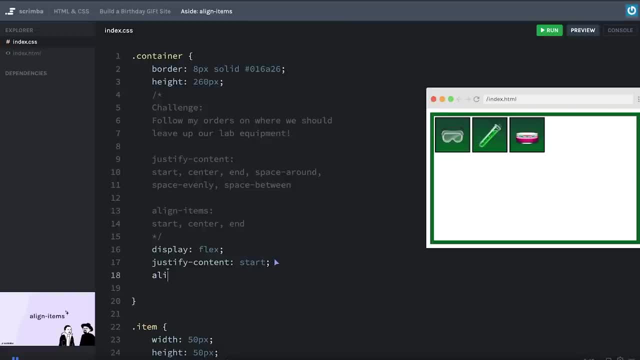 So let's turn this back to start And do align items. Center. Boom, there you can see. now it pushed all of the three items down to the center so that they are centered vertically, meaning they are centered along the cross axis, And then I can combine this with the main axis, which is justify content. 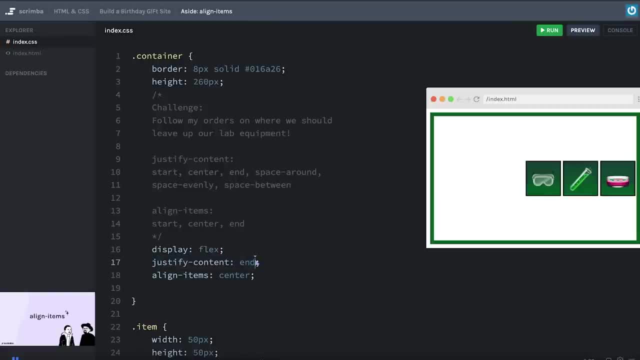 controls, the horizontal one, going from left to right, for example. do end here and boom. then we are still vertically aligned, So we're in the middle, but we are pushed all the way to the right hand side along the main horizontal axis. So the values you are going to use for 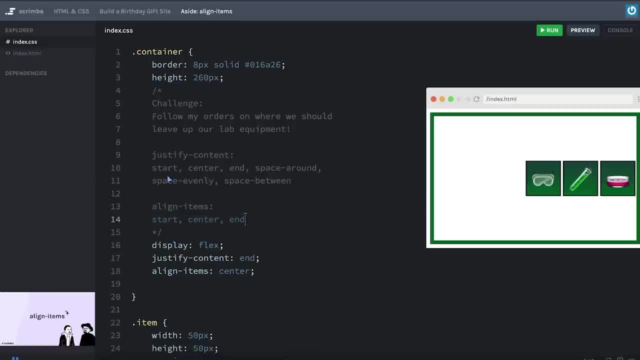 line items. to begin with, our start, center and end, Whereas with justify content, as you know, you can use start, center and end, but also these space around space evenly and space between properties. Okay, let's move on to the challenge. What I want you to do, 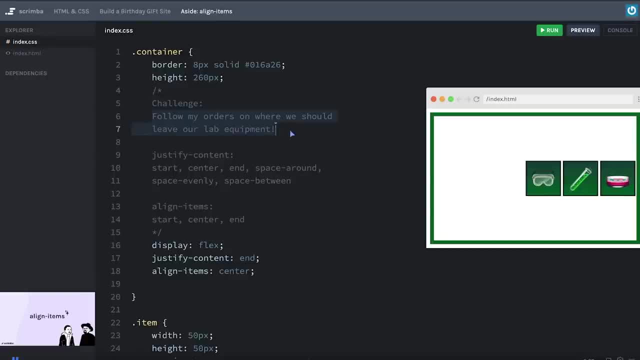 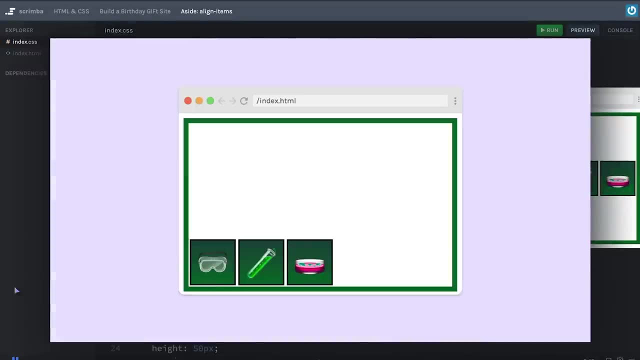 is: follow my orders on where we should leave our lab equipment, because I want you to do it in very specific ways, starting with this position here, where they're all squeezed down in the bottom left corner. So go ahead and modify, justify content and align items to. 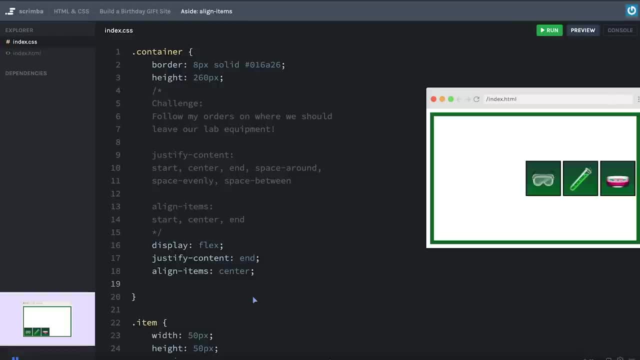 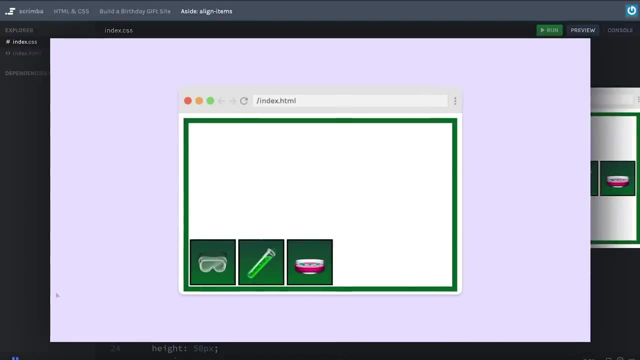 achieve that layout right now. So to achieve this layout, you can see it is at the bottom of the cross axis, the vertical one. So we'll do end on align items, But it is at the start of the main axis because it is pushed all the way to the left, meaning that we should 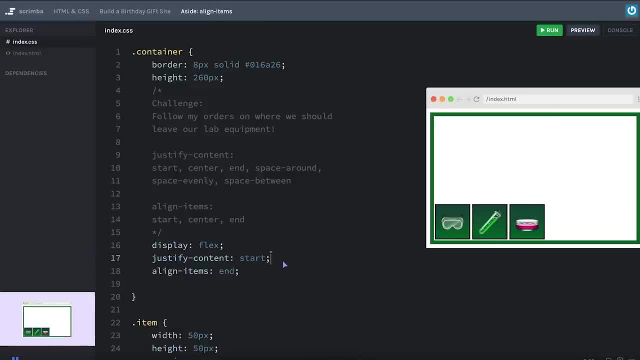 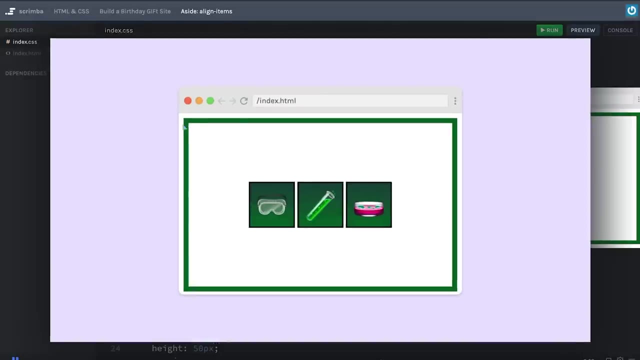 do start up. here And there we go. we have sold it. Okay, new challenge: I want you to achieve this layout. go ahead and do this right now. So here we can see we are actually centered both along the main axis horizontally and the cross axis vertically. So I'll try. 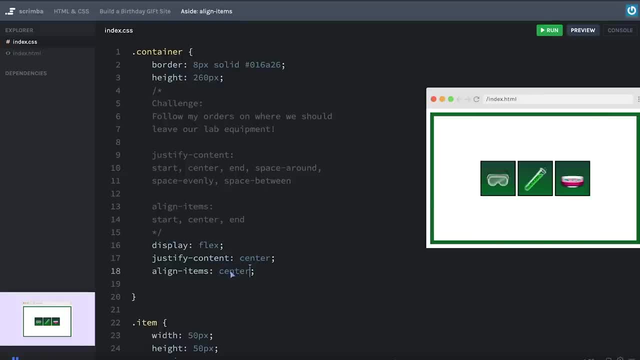 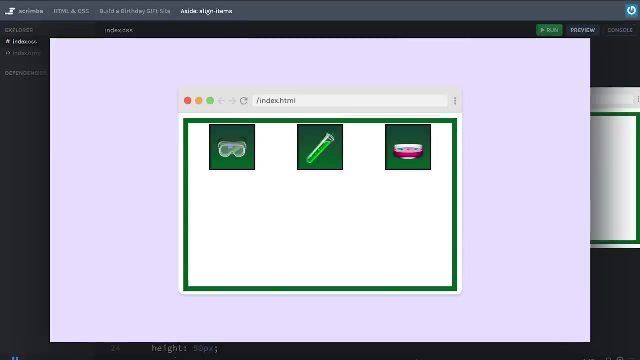 center, Yes, and center again, And there we go, Okay. final one: I want you to organize the equipment like this: Go ahead and do it right now. Okay, hopefully that went well. the first thing I'll notice here is that all of the 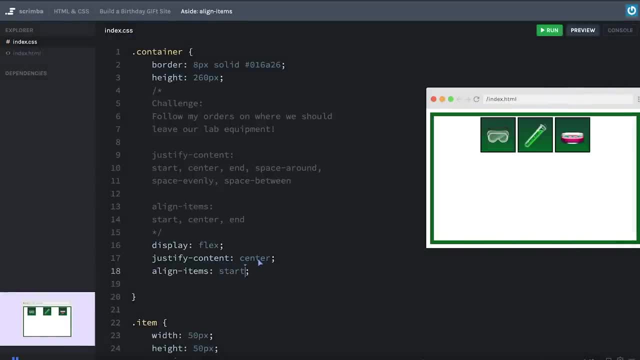 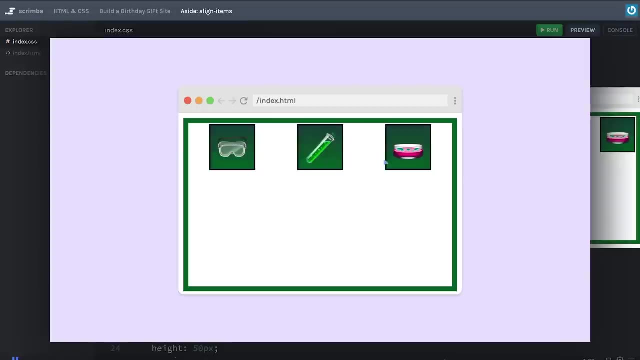 items are squeezed to the top. So align items should be start And there's some space around the elements. So we need to try one of these, for example, space around space evenly, or space between. So let's try, for example, space between. Hmm, that didn't exactly achieve. 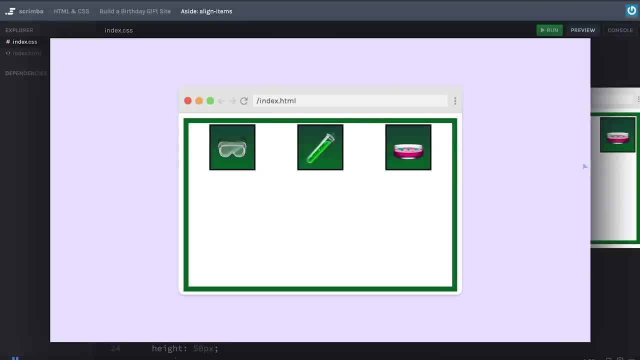 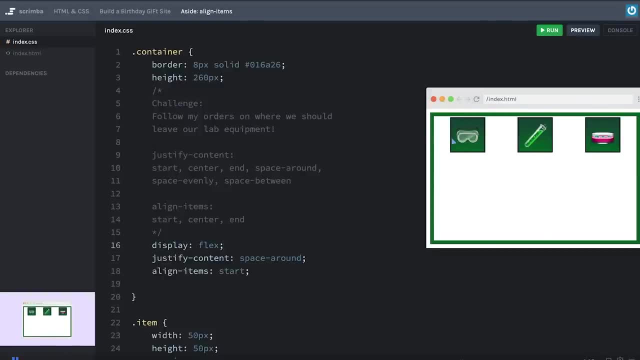 what we wanted, because there should be some white space on the left side and the right hand side here, Where's these two are squeezed all the way to the end, So maybe we can do space around instead. Yes, that looks exactly like what we want, So really good job solving these three challenges Before we move on. 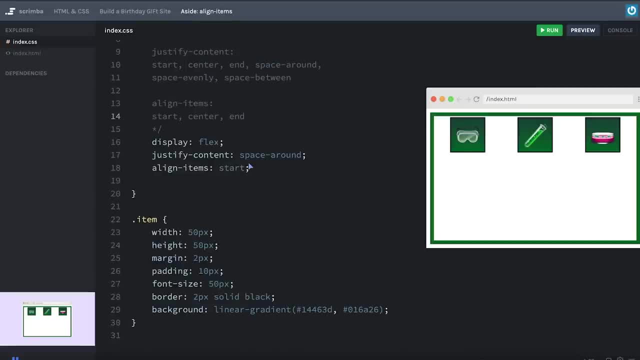 there's just a small thing I want to tell you, And that is something you might see from time to time, which is that if I now remove the height of our items, see, then they just became a little bit higher because the content inside of it wants a little more height. But 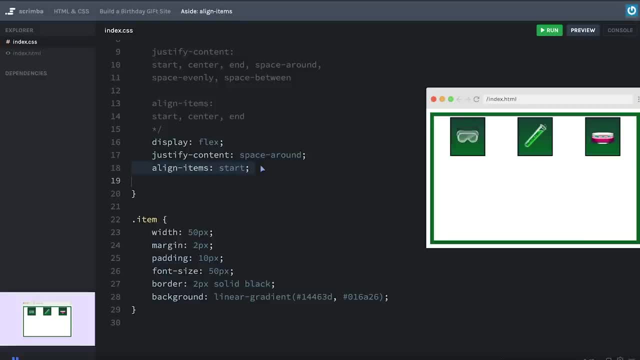 that was besides the point. what I wanted to do is also remove the align items. Let's see what happens. Oh wow, it turns out that flexbox in the cross axis actually stretches the content like this. And the reason it didn't happen. 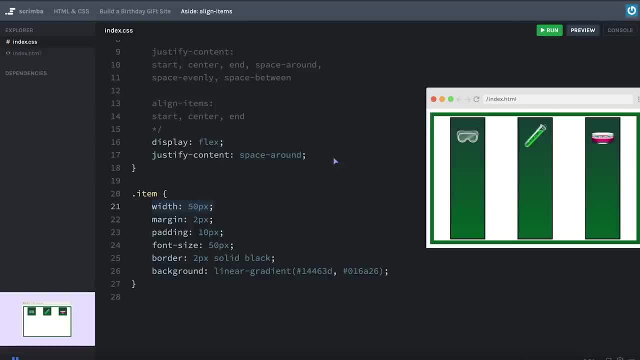 previously was because our height property overrode that stretching. So what this means is that line items by default has the value stretch. When we do, for example, start, it's no longer stretched and it's pushed to the start. So this might feel very confusing and 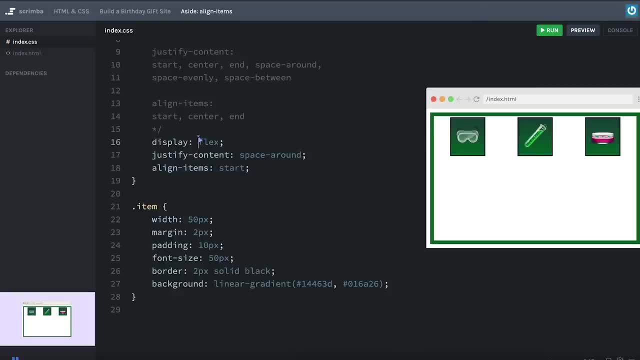 the only reason I want to tell you about it now is that when you are in a flexbox layout and you notice that something is stretching in a way you don't want it to stretch, the prime suspect you should look at is align items and experiment with that. So be aware. 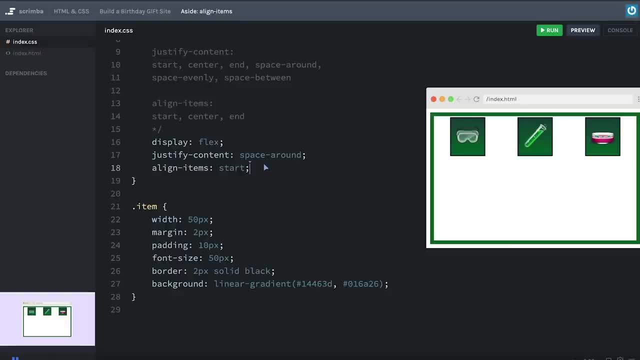 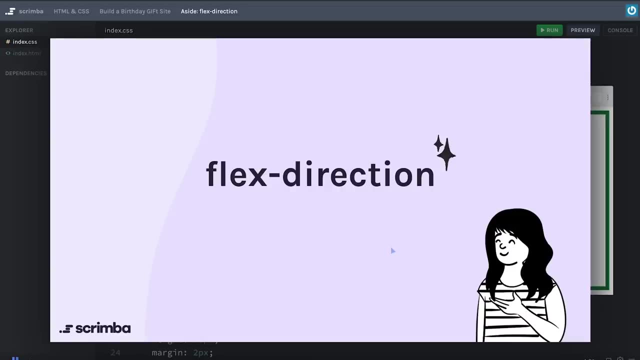 of that, But don't worry too much. If you found this a little bit confusing, it's totally okay. Let's just keep up the pace and move on to the next scrim. Now you're going to learn about flex direction, Because there is one problem with our lab. 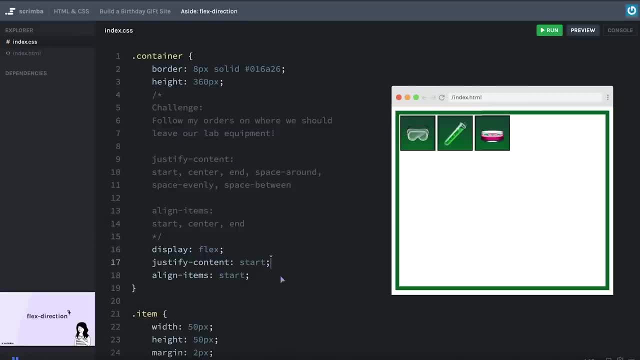 system Now, That is that regardless of how we change around on the align items and justify content- center and end, for example- our lab equipment will always stack up besides each other. they'll be on the same row and there's no way to get them to stack on top of each other. But 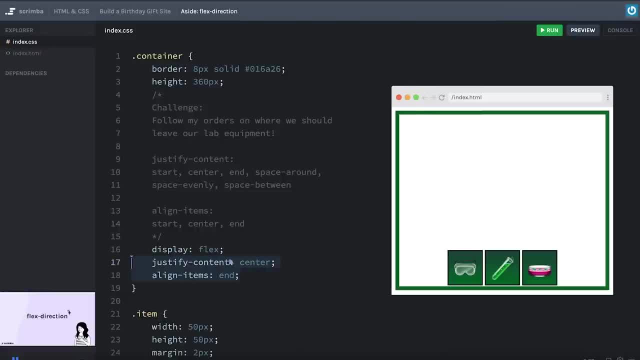 maybe that's how I prefer to leave my lab equipment for the night. But regardless of how we change, to justify content and align items, that is now impossible. Now we could, of course, remove the display flex And then these divs will stack on top of each other by default. So by doing this now they stack on top of. 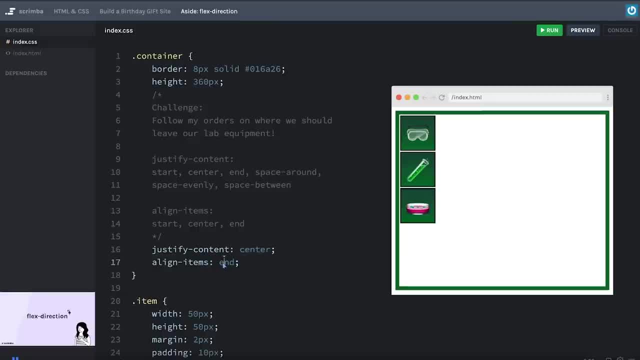 each other, However, justify content and align items no longer work. So if I tried changing these, nothing happens, because these properties work inside of a flexbox, not inside of a random div. that, by default, is display block, So we need the display flex like that in order to make these work. However, what we 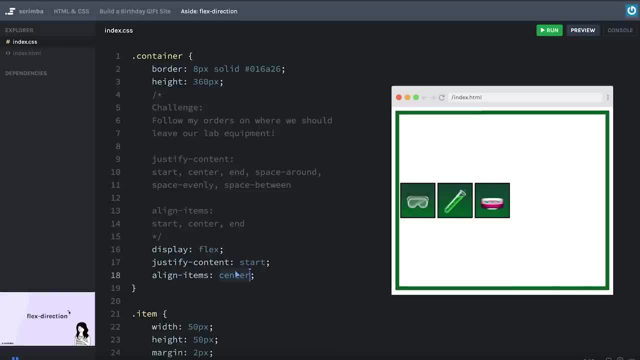 can do is change the flex direction. So first let me just both of these two back to start And then I'll do flex dash direction. And it by default is a row because, as I said, the stack up alongside of each other on a row. but if we change this to column boom. there you can see now they. 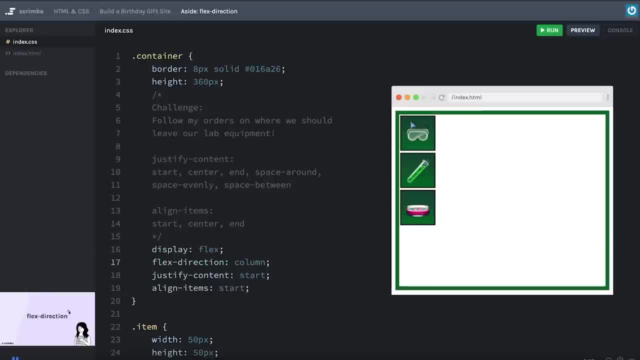 suddenly stack on top of each other as if they are in the same column, as columns go from top to bottom. So now we are back to the original layout we have before. we made this into a flex container, But justify content and align items now work However he work. 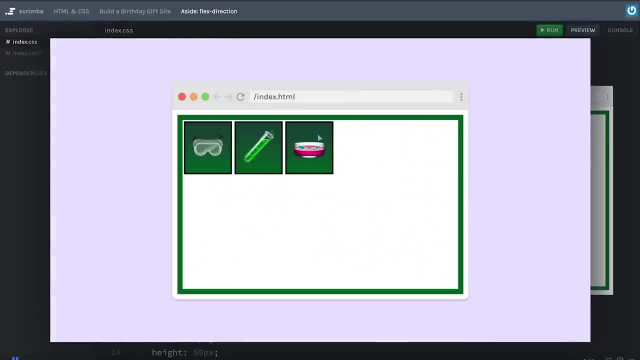 in a little bit of a different way And you might expect, because, as you remember, I previously talked about the main axis going from left to right and being the one controlled by justify content, whereas the cross axis going from top to bottom and also being controlled. 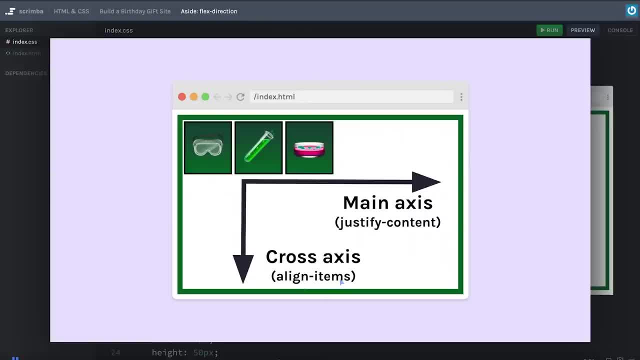 by align items. Well, when we change the flex direction and our items stack up different way, we also change the main axis. So this is no longer the cross axis, it is the main axis and it's controlled by justify content, Whereas the horizontal one is no longer the. 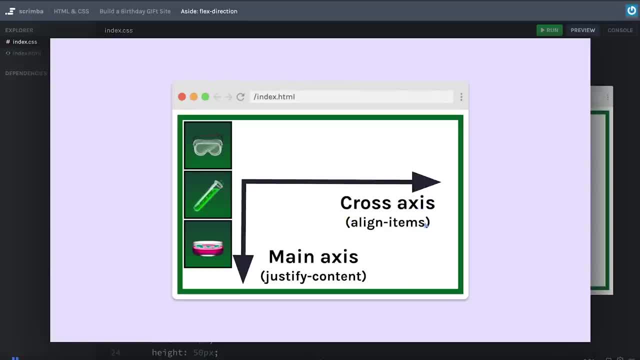 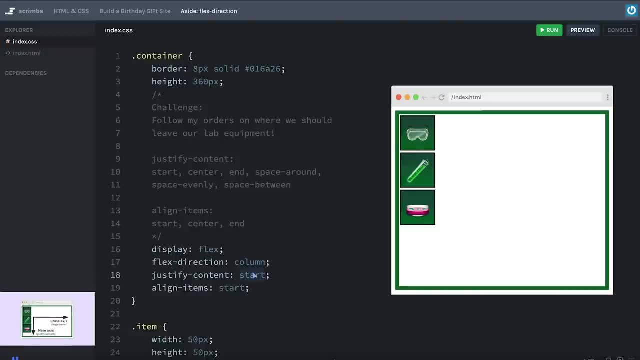 main it is the cross and it's controlled by align items. So we basically flipped: align items and justify content. So if I now do justify content and he'll jump downwards, whereas previously they would have jumped to the right, And if I now do align items and he'll jump to the right, whereas previously align items. 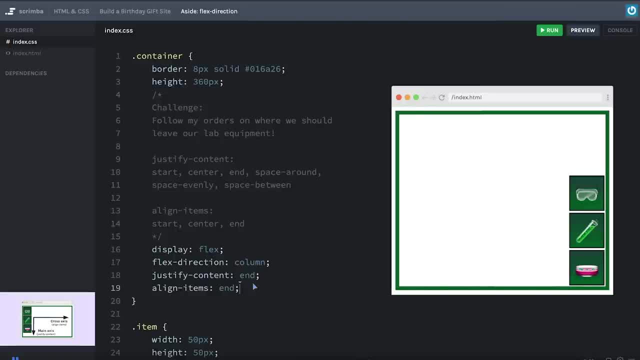 control the vertical position. So this is probably a little bit confusing. Now you should not feel bad if this feels overwhelming. This will take time to mature in your mind And it's totally okay that in the beginning. now you're just experimenting with these values. 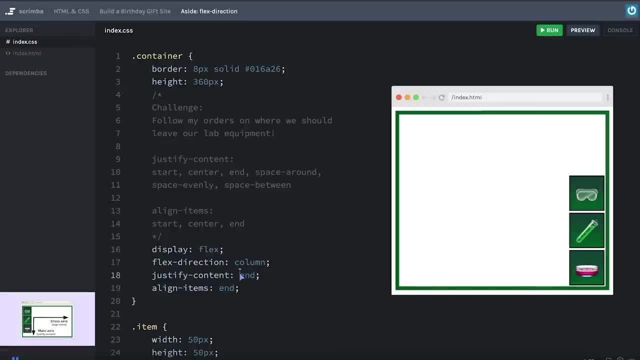 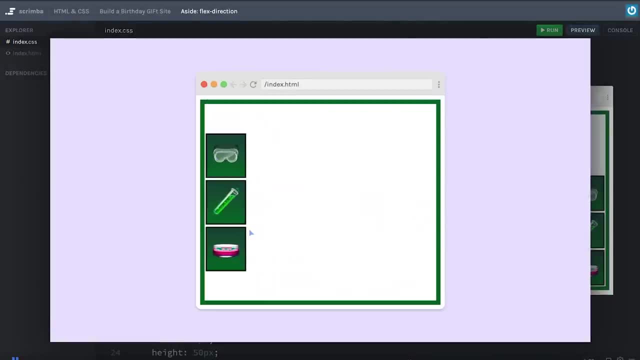 in order to get the layout you want and not really remembering exactly why it works as it works. So let's now give you some practice. I want to clean up my lab equipment and I want it to be like this. So go ahead and change around on these two values in order to achieve. 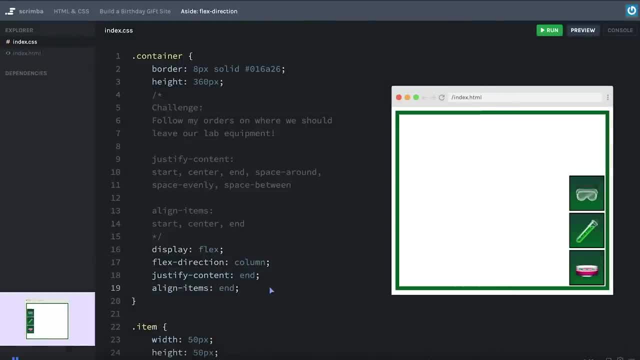 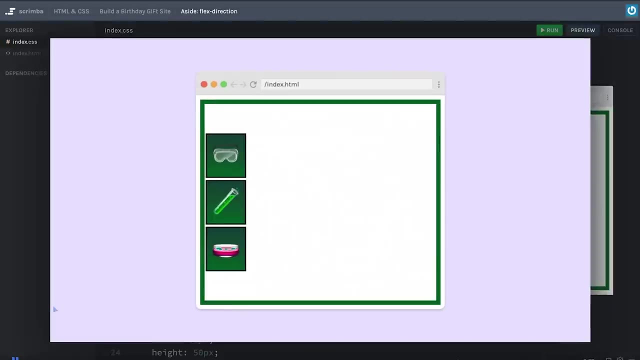 that layout. Okay, what we need to do is on justify content. I want to center it so that it's vertically centered, But then we want to align it to the start on the left hand side. Yes, that is correct. Okay, new one: achieve this layout. 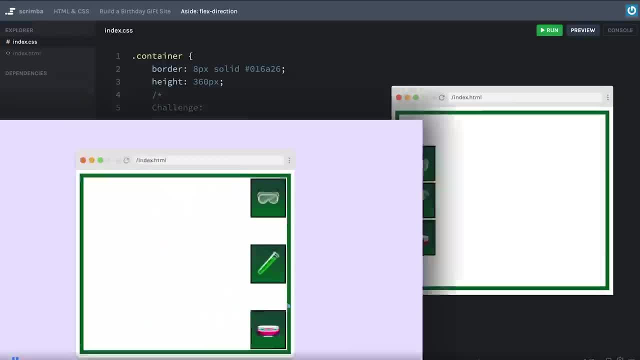 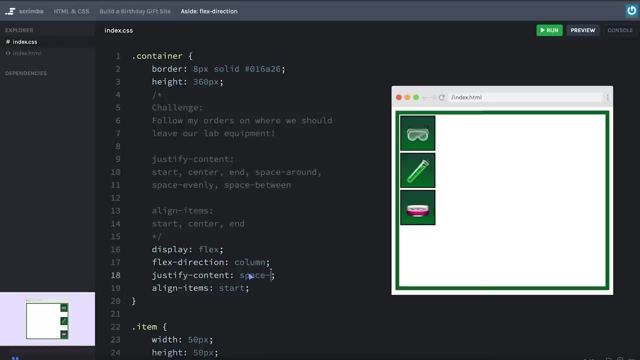 Okay, here we can see some space in between the items, So I think we need to use space between: on justify content: Yes, looking good, But we are aligning to the left. we want to align it to the right instead, So align items should probably be: and, instead of start and. 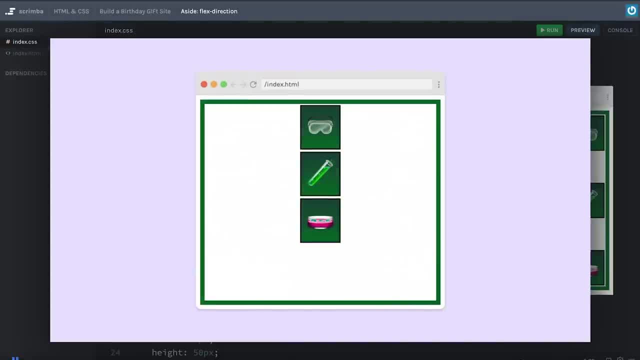 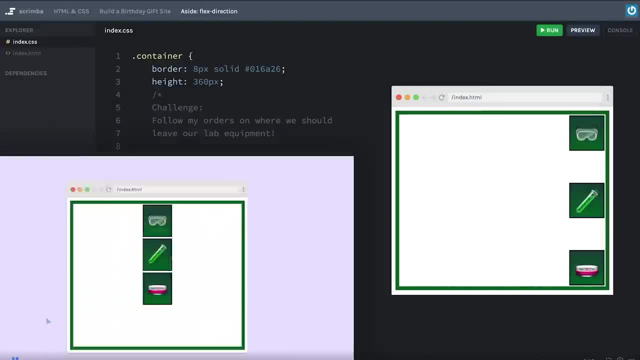 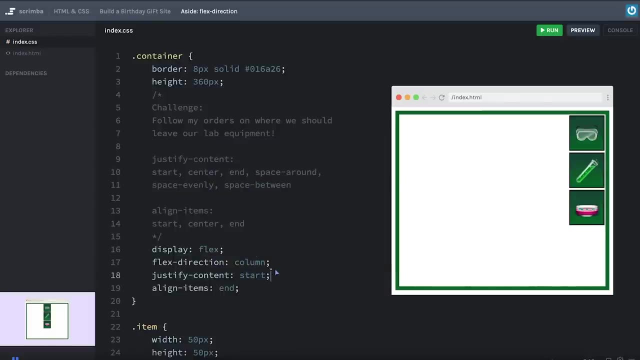 boom, that is correct. Finally up this one right here. give it a shot right now. Okay, we can see that they are all squeezed towards the top, So I think we'll do justify content. start like that: Yes, this is good, But we want to center it as well, So we'll do align. 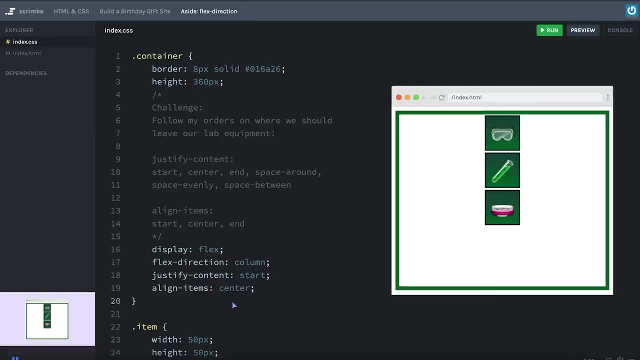 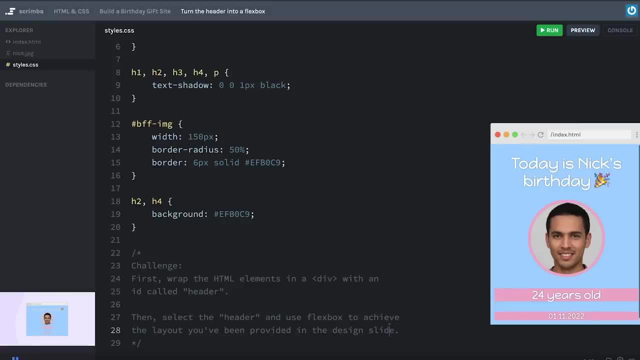 items center. And there we go. So great job doing this, Let's just move on. Okay, now we're going to put your freshly acquired flexbox skills to the test, Because you are going to turn this layout here into this layout. So first I want you to wrap. 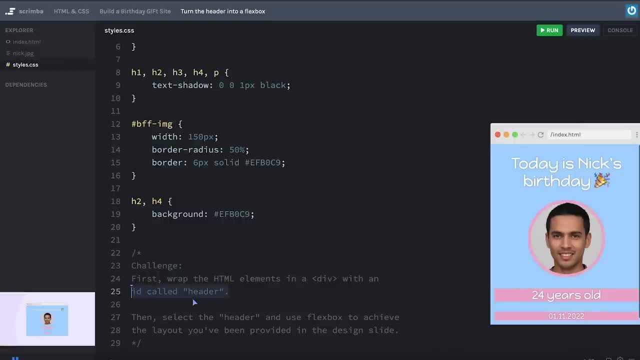 the HTML elements in a div with an ID called header. So that is all of these items right here, And then you are to select this header and then use flexbox to achieve the layout from the design slide And, as you might have guessed, you will need to use flex direction. 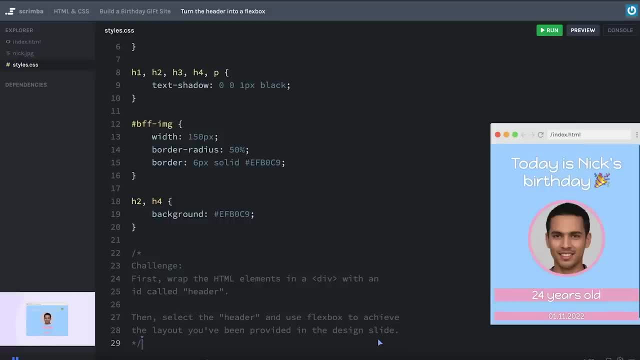 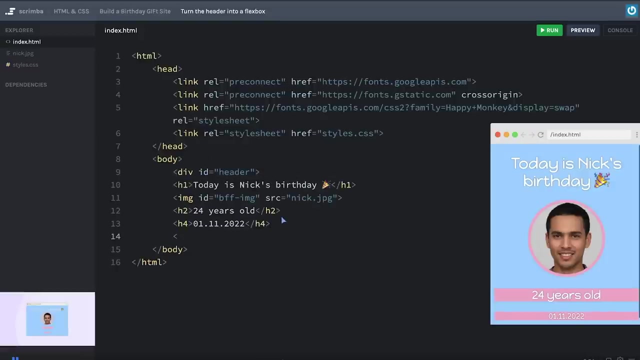 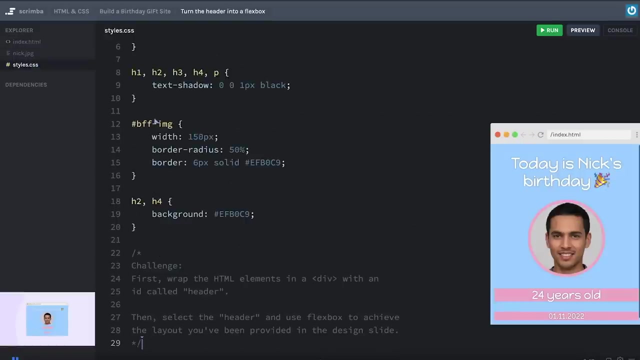 and align items to solve this. So go ahead and give this your best shot. Okay, so we'll start in the HTML, create that div opening tag and close it off down here, And then this: run it. no change seen in the mini browser. that is to be expected. 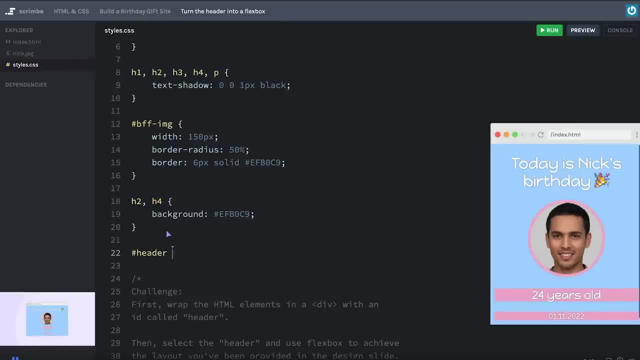 because we'll have to target it and style it. So I'm going to do header and then first display. flex that forces all of the elements into one row, Because it is flex direction row by default. However, we don't want that. we want everything. 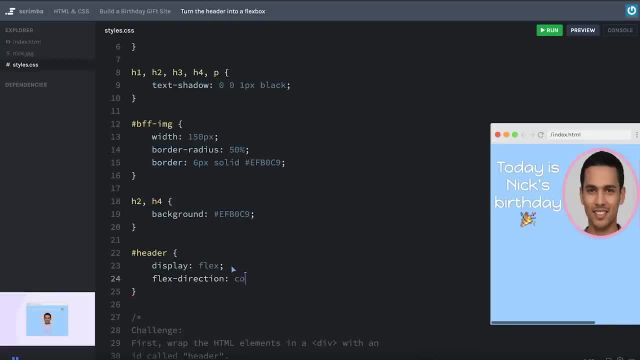 in one column. So we'll do flex direction column like that. Now they stack on top of each other, which is just what we want. But there's a problem. The two elements here are stretching and the image of Nick is left aligned, it's not centered. So I think we 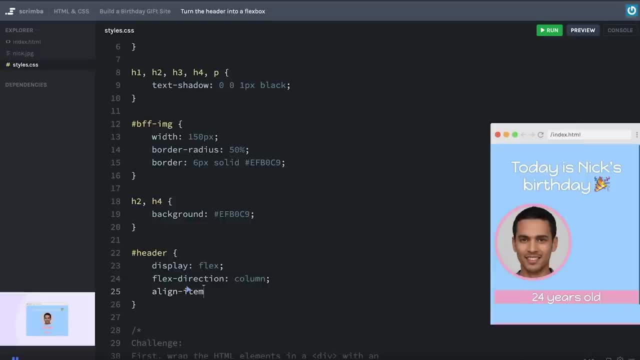 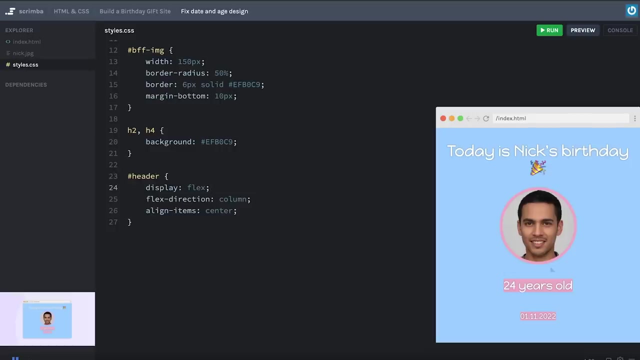 need to change the align items, align items into center, like that. And there we go, And there we have the layout we wanted. So great job, let's move on. Okay, now you're going to fix up the design for this 24 years old element and the date. 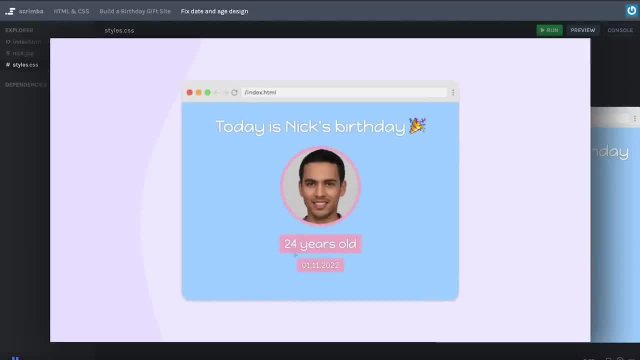 element right here, because I wanted to look like this. Here you can see that there's some space between the content of the element and the edge of the element And there's not as much space between the elements, And also the edges of the rectangles are a bit softer. 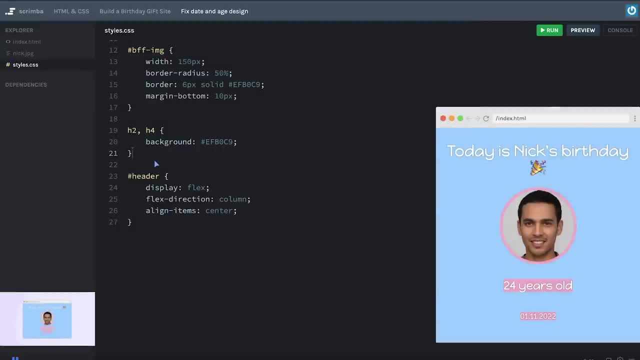 But before you start doing this, there's a couple of things I want to do, Because here the h2 and the h4 have no IDs or classes. they are just selected using the element selector and also using a selector list separated by commas, And I don't think we should do. 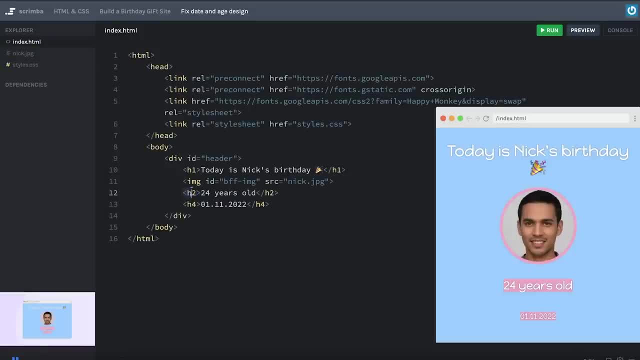 either of those. First of all, we probably don't want all of our h2 and h4 on the page to be styled according to how it looks here up in the header, So we actually want to give these two IDs. I'm going to call this one b day age and this one b day date running this code. so 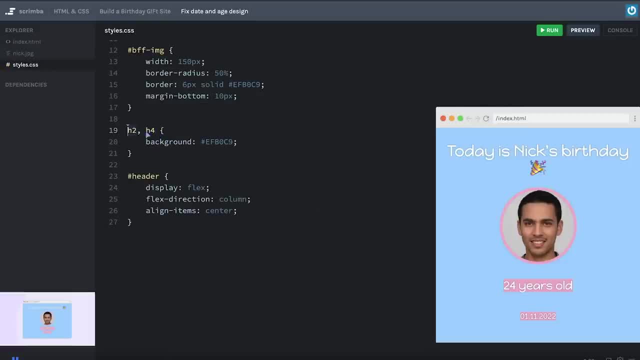 that we got it applied And then in the CSS, instead of using element selectors, we'll use ID selectors, b day age and b day date, And then, finally, let's avoid applying styles to both of these simultaneously. let's work. 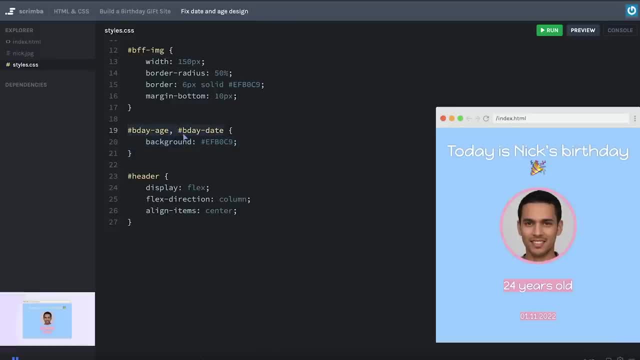 with one or the other, because this is really an optimization and writing code which is so called dry Short for don't repeat yourself. And while that is a good thing, I want you to focus on the core CSS now, because this will introduce a little bit more complexity. So let us instead 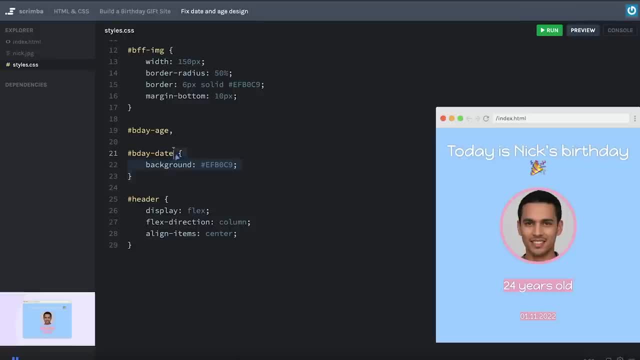 just keep it simple, So I'll break this into a new line. So we got the birthday date rule here and then copy the exact same thing to the b day age, like that. Okay, now it's time for your challenge. you are going to make the b the elements look like the provided design slide like this: 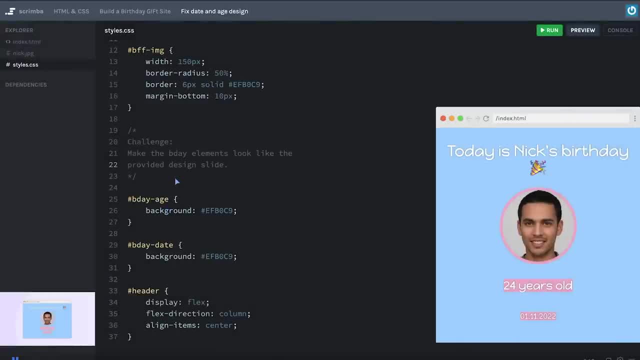 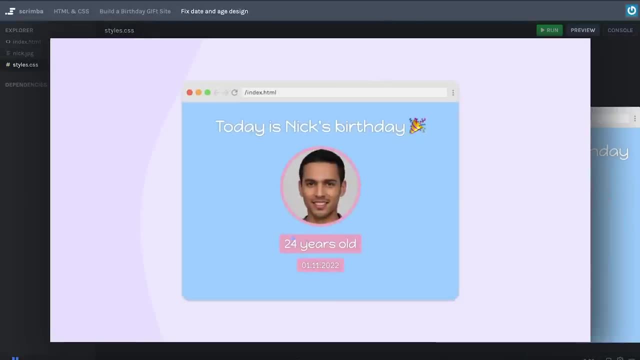 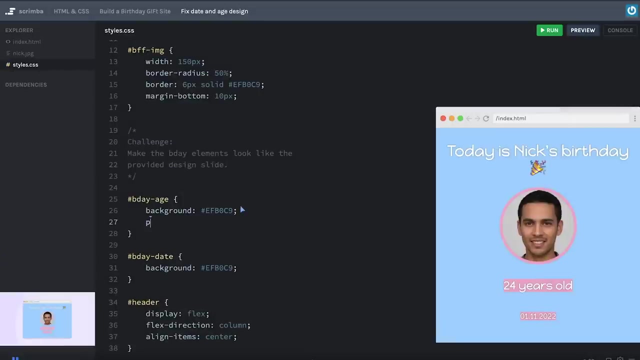 So go ahead and do it here and, as I do it now in theisskov, by title I'm going to use is right now. okay, hopefully that went well. let's start with the age element. as you can see, there is some space around it. that is padding most likely, so let's add padding, for example, 10 pixels. 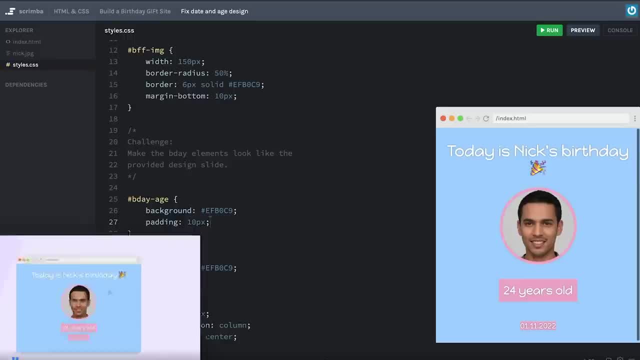 and see how that works. if we compare that with what we have in the design, it looks pretty good, but i think we shouldn't have 10 pixels on each side. i think the padding on the left and right side is meant to be slightly larger than the top and bottom, as we've often seen with buttons and 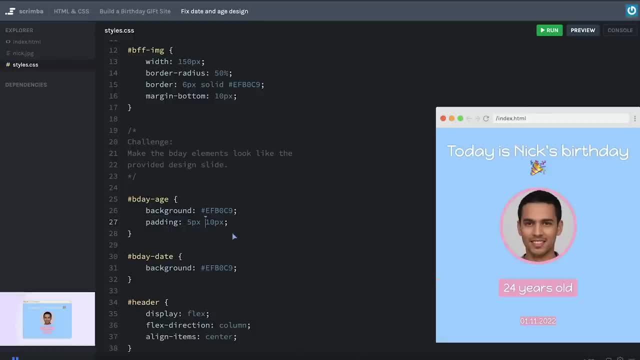 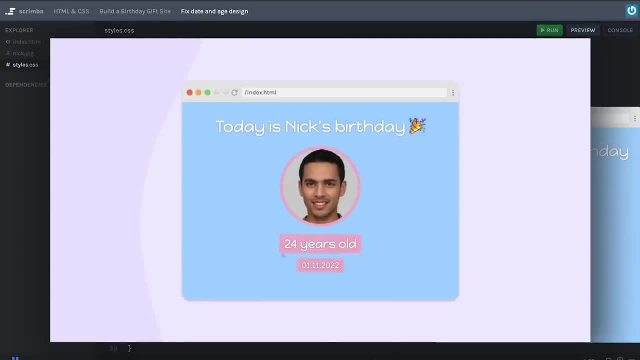 layouts in general. so for the top and bottom we'll do 5 pixels and left and right 10 pixels. that is what we are looking for, as far as i can see. okay, next up, there is some border radius here as well- not that easy to see, but it definitely is there. so we'll do border radius 5 pixels, for example. 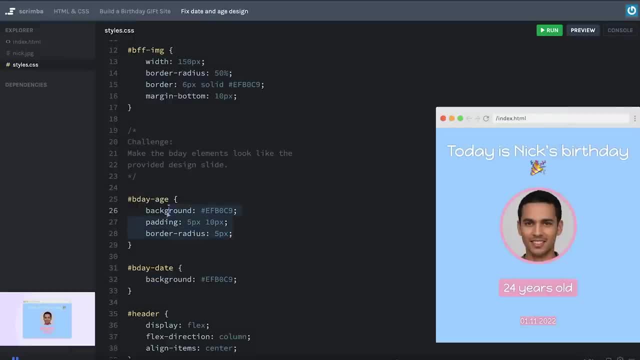 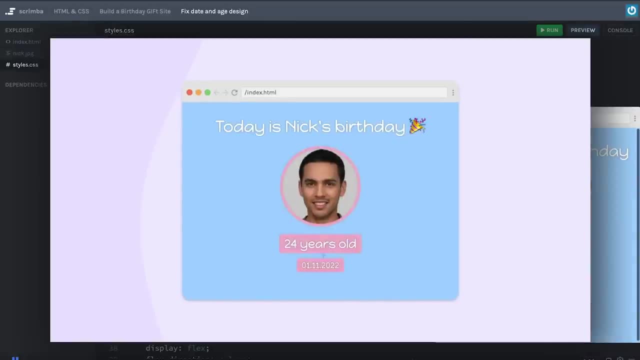 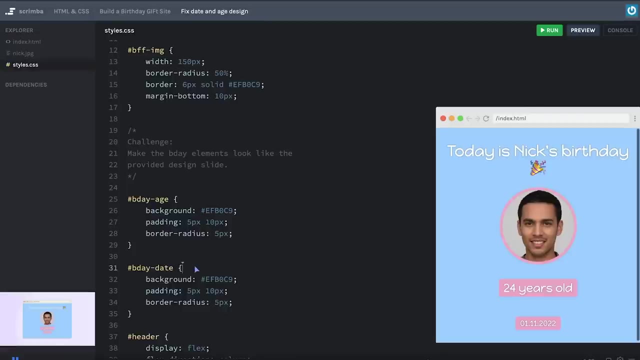 that looks pretty good to me, and now let's just try to copy this down to our birthday date and see how that works. here you can see, except for the fact that there's much less space between the elements here, they look pretty similar as far as i can see. so we need to move on to the margin. let's try first and remove all the margin from the. 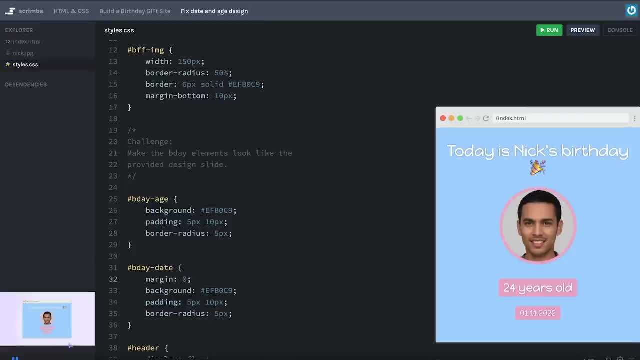 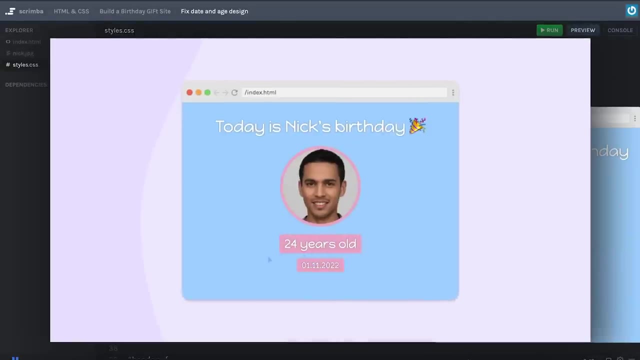 birthday date margin 0 like that. now it's quite a lot closer, and whatever margin comes from the age 2 element, that probably has a bit too much margin bottom. so let's rather control that by doing margin bottom for example, 10 pixels, and yes, that looks pretty good to me. let's also look at 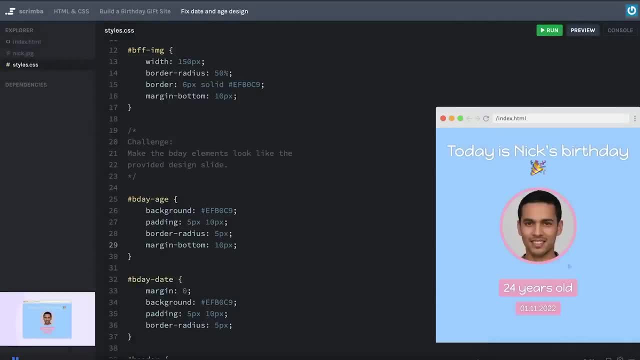 the margin top here it is too much space between the two elements. so i'm going to go ahead and slightly bring it down here, much to the side, to the border, and yes, it looks pretty good, but it is too much space between the age element and the image. so if we do margin top by 10 pixels there, 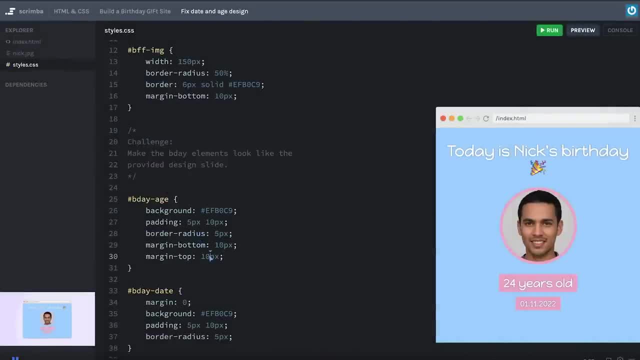 that looks pretty good, but it's perhaps still a little bit too much, so let's do five instead. yeah, actually i think we got it. so the final step, then, is to convert this into a shorthand, because we know how to use shorthand, don't we? we want five on the top and ten at the bottom, then. 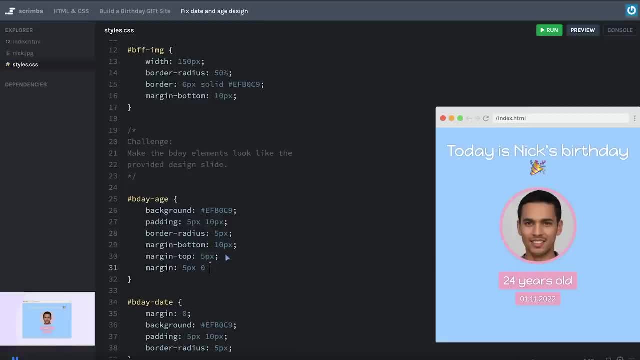 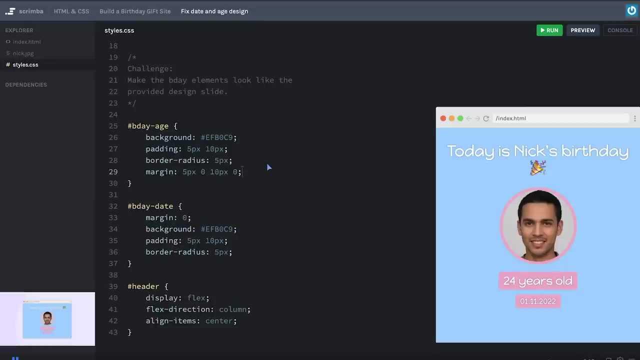 we'll do margin: five px for the top, zero for the right hand side, ten px for the bottom and in the, and zero for the left hand side. And there we go. Now, if your solution is slightly different from mine, perhaps you used slightly different margins, border radius, padding. that doesn't. 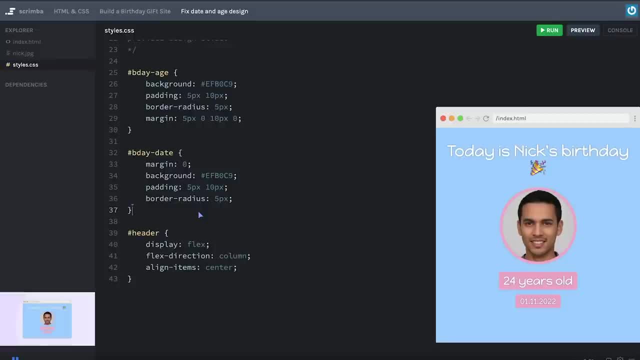 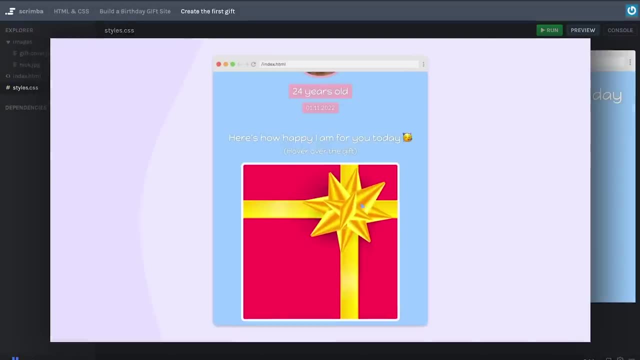 really matter. Give yourself a pat on the back, regardless of how you solve this, And let's move on. Okay, now you are going to create the first gift section of our site. So, as you can see, it contains a title, a little hint about hovering over the gift. 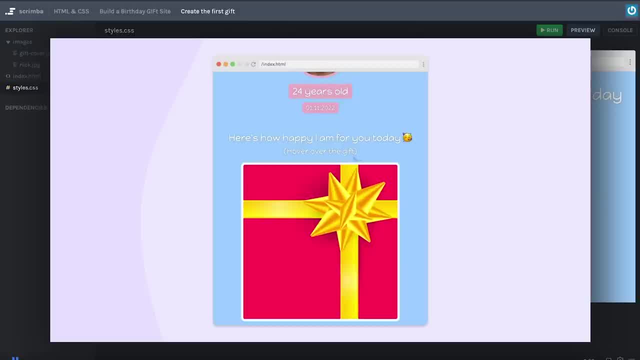 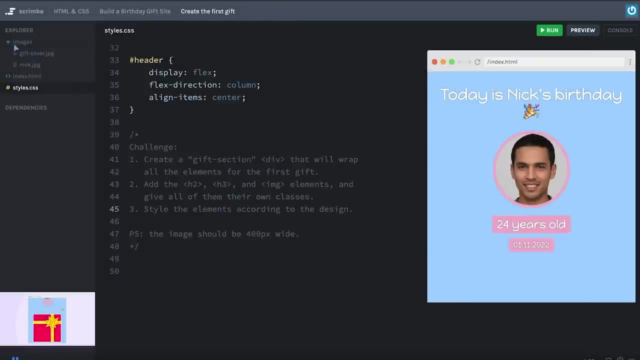 then there's the image itself. Now, the hover effect is not a part of this challenge. you're only going to work with this hard coded gifts cover at this point, And that gift cover has been added up here in a images folder which I've just created, as we now have two images. 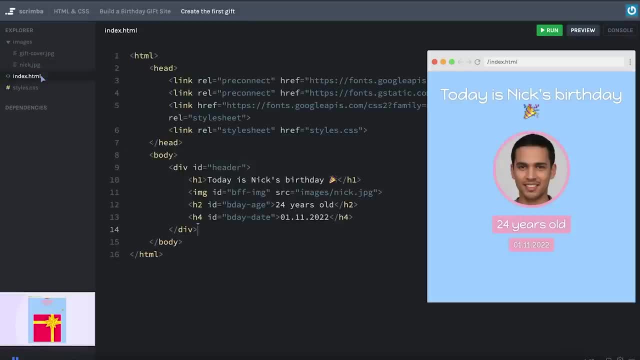 so I wanted to gather them together in this images folder. That means that I've also changed the image of Nick or the source that is referring to the image of Nick in the HTML that now contains the image. So I'm going to go ahead and create a new image here And I'm going 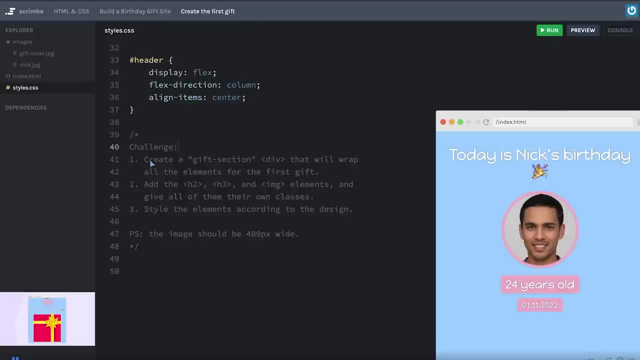 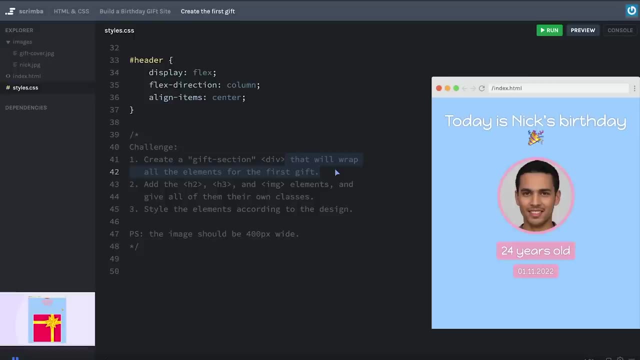 to use the correct path into the images folder. So the challenge is described in detail here. I want you to start by creating a gift section div that will wrap all of the elements for the first gift, And then I want you to add the h2,, h3, and IMG elements. So that is the 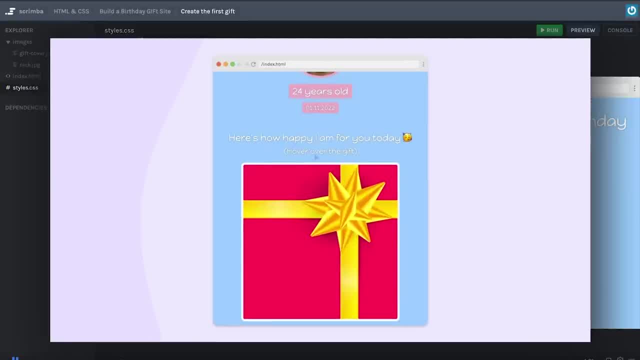 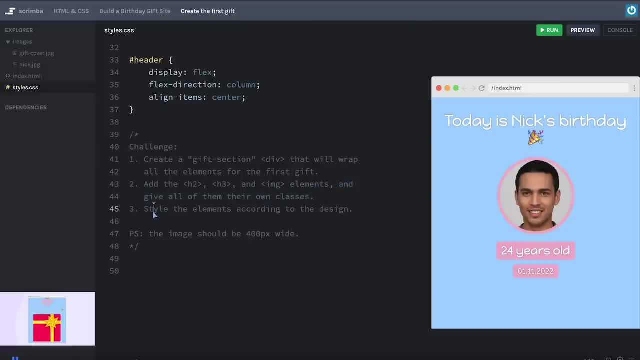 title, which is an h2, the hint, which is an h3. And, finally, the image itself. And I want you to give them all their own classes, so that you can use the classes to select the elements when you are to style them. 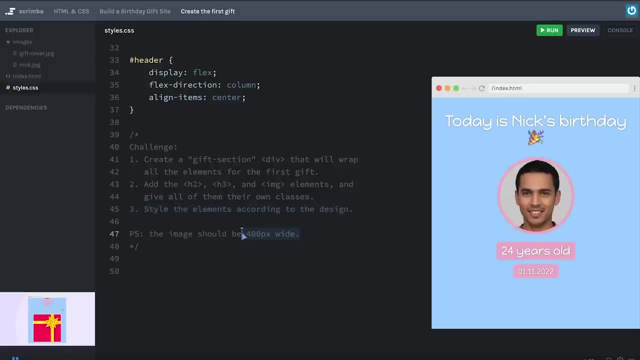 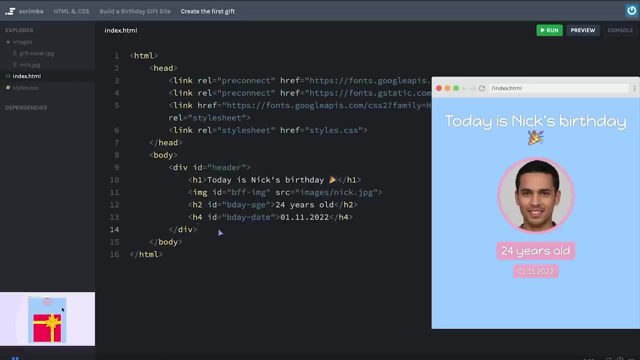 According to the design And as a final hint, the image should be 400 pixels wide, So go ahead and do this right now. Okay, hopefully that went well. So I'll start by heading over to the HTML and create the markup. So we wanted a div to begin with. I'm going to create that. 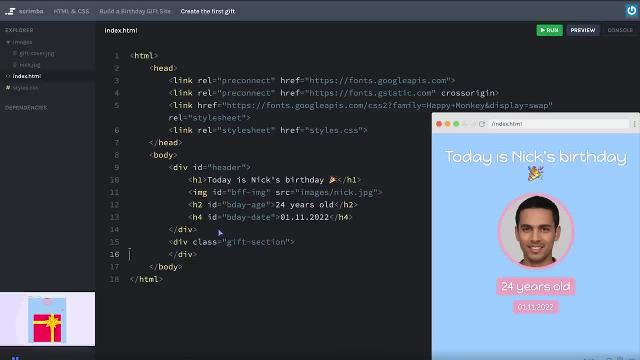 and then give it a class of gift section like that, And inside of it we wanted first an h2 for the title, which should contain the following text: Let's run this and yeah, nice, You can see that the text already has the correct font and also the slight shadow around. 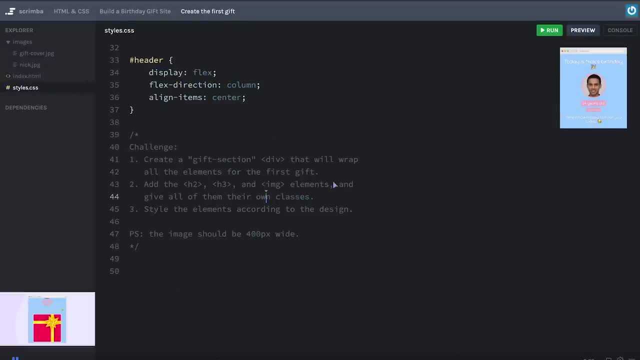 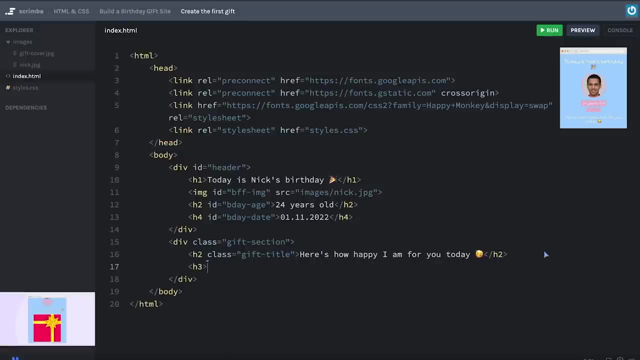 it. Okay, very nice. Let's then give it a class, as that was something we should do with all elements. I'll call this gift hash title like that, And there was the h3 with the following text: I'll give that a class of gift hint, So you can see I'm using gift, and then a description. 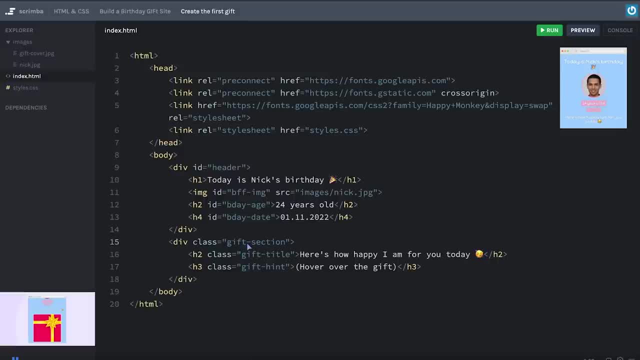 I think that makes it easy to understand that these are all somewhat related to each other. Finally, the image element should have a source of images- slash, gift cover, dot, JPEG- and also a class of gift: IMG. All right, let's run this code And as you can see everything, 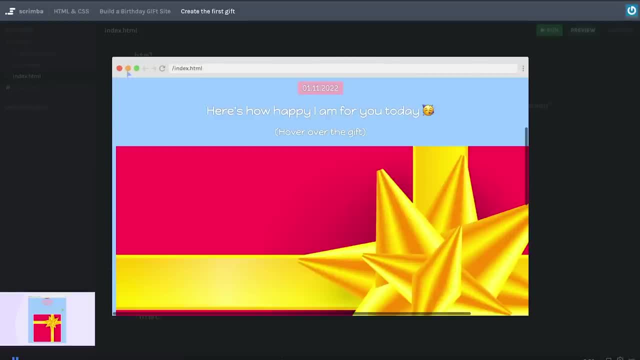 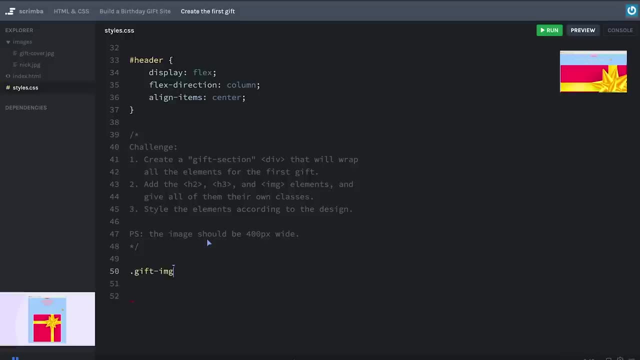 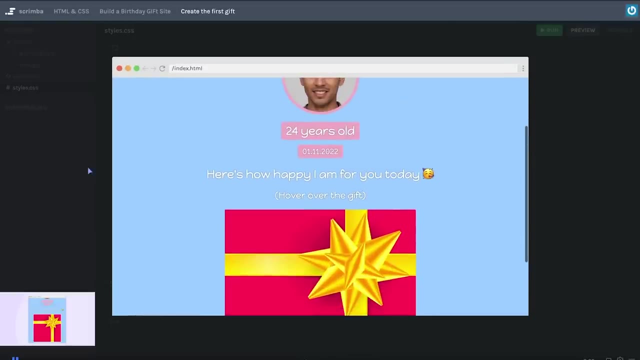 is being rendered, though, the image is far too large, So we need to get going with the styling. All right, I'll start with the image, So dot gift IMG and give it a width of 400 pixels. Yes, that is much better, And it is centered because. 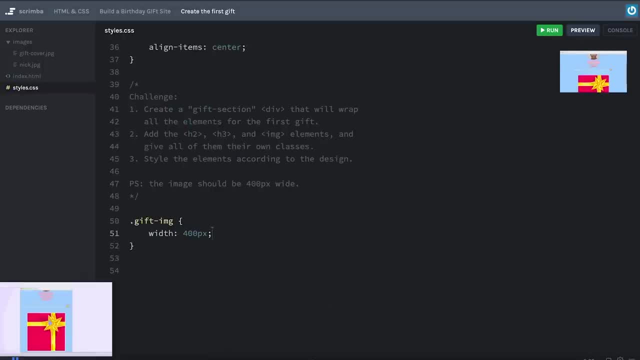 of our text align center up here. Very nice. Okay, let's just carry on with this one. you can see it has a white border, So let's do order. looks to be something like six pixels or something and solid white- Yep, pretty good. And finally a border radius, because 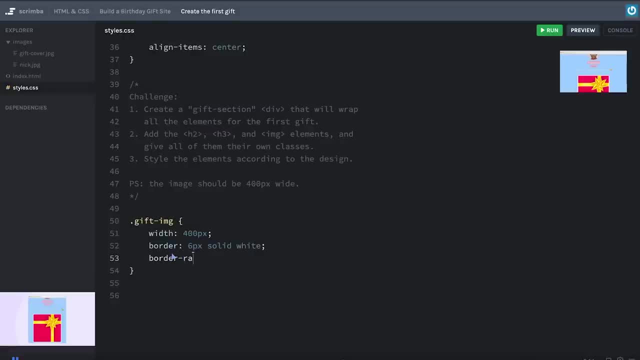 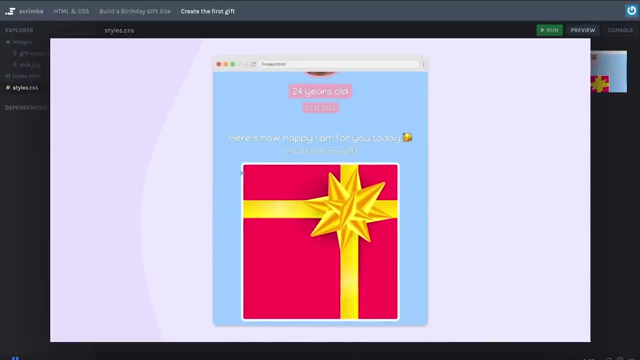 the corners here are a little bit rounded off, So let's try border radius Yep 10 pixels, for example, And yeah, that looks pretty much like the design for the image. Nice, Okay, next up is the spacing. As you can see, we have far too little space. 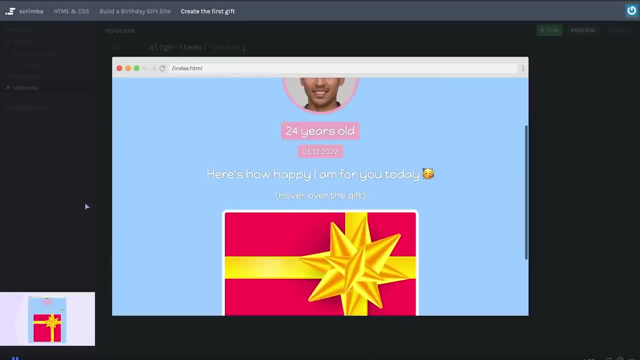 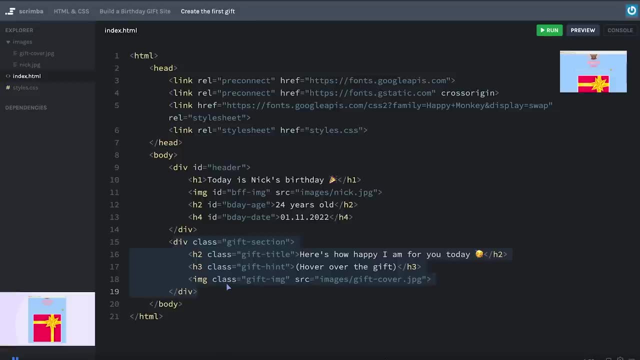 from the gift section itself to the header section above, And I could add that to the top element here, to the title for example. but it makes a lot more sense to add it to the container element itself because it should control how far it is between this container. 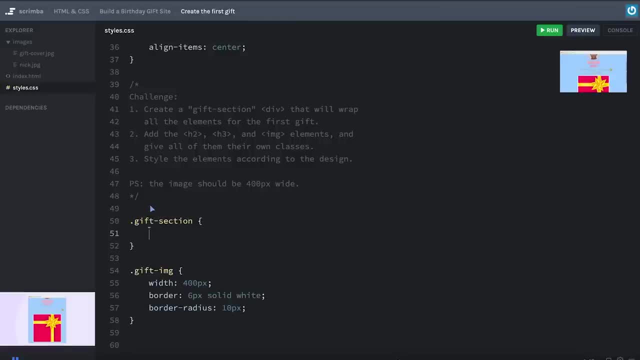 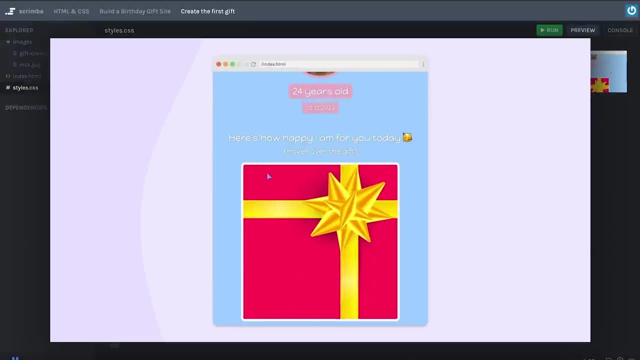 and the container above. So let's do gift section, margin top and, for example, 50 pixels. that is much better and looks pretty much like what we have here Now. you can see that the space between the title and the hint is very limited. 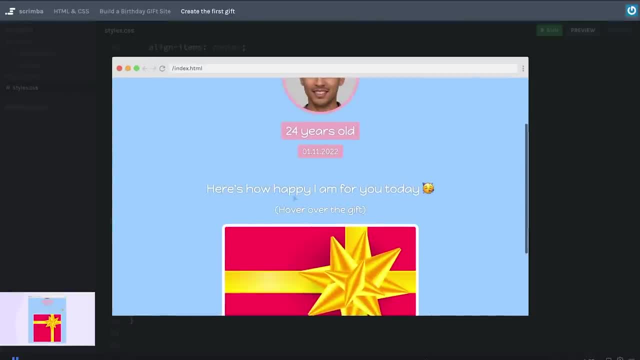 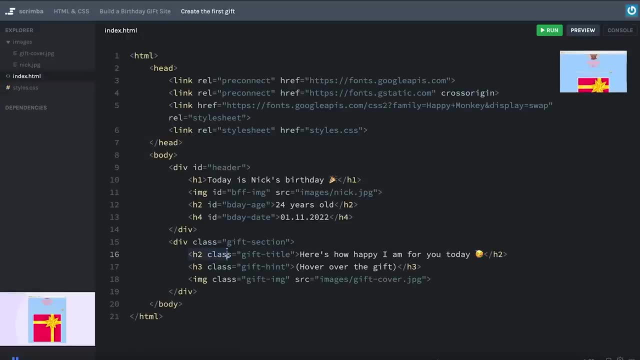 it's not that much space, Whereas here the default margins for the h2 and h3 elements create quite a lot of space in between them. So now we probably have to work with both the default margin that the h2 has at its bottom and the default margin which the h3 has at its top. It doesn't. 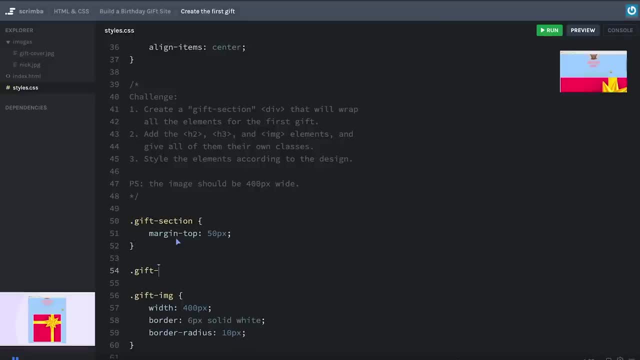 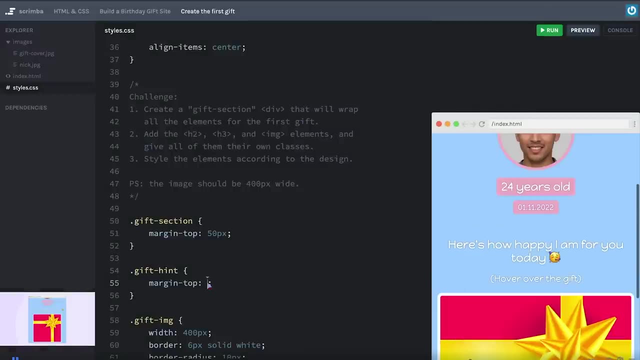 really matter what we start with. Let's, for example, just start with the gift hint and see what happens if we set the margin top. Actually, let's bring it up on the side here. Now we've not done anything with the margin top at all. Let's set it to zero. You can see nothing happened. 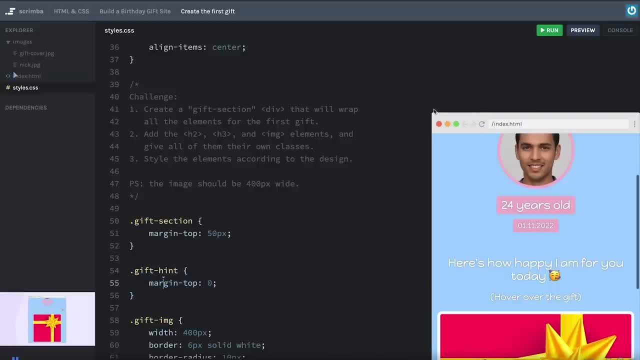 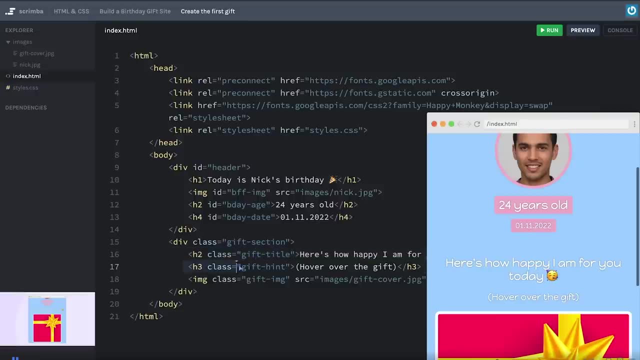 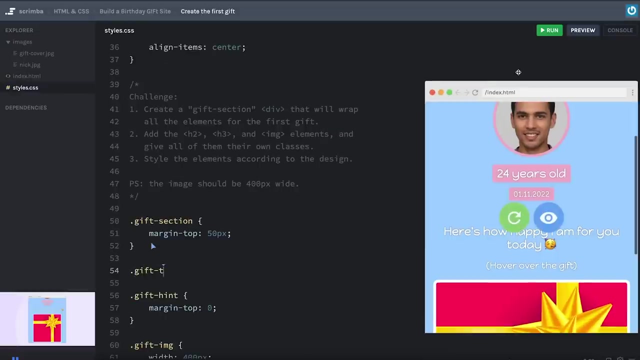 Okay, that must be because the margin top here and the margin bottom under the h2 collapsed into each other And the margin bottom for the h2 was probably larger than the margin top for the h3. So removing it served no purpose. That means that we also need to try and remove the gift titles margin. 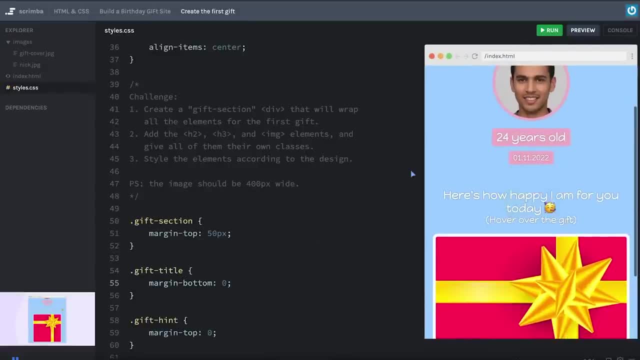 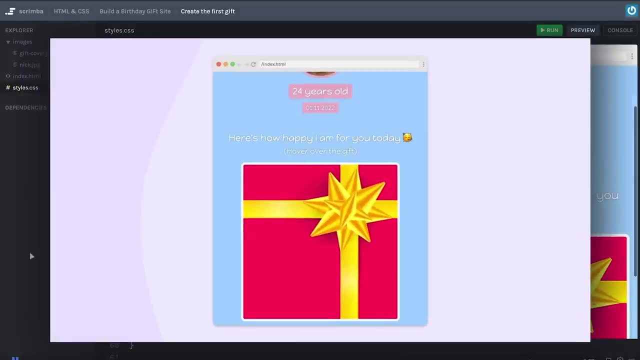 at its bottom. set it to zero, for example. And there we go. Now. they're really crammed into each other actually too much. they should have a little bit of spacing in between them. So let's try to. instead of reducing that to zero, we set it to, for example, 10 pixels. that looks much more like the. 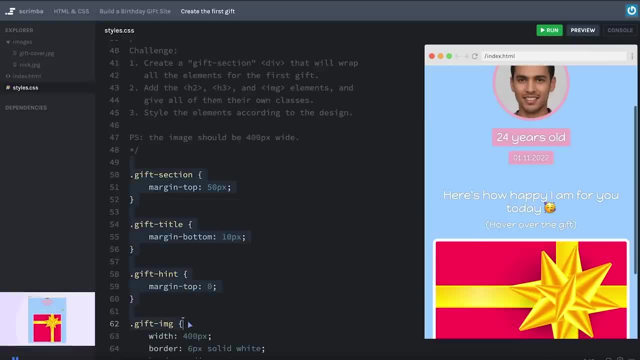 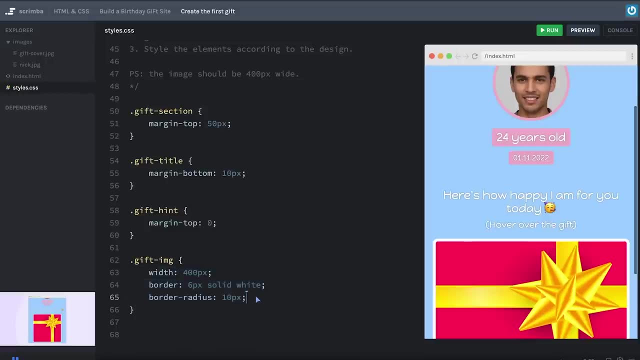 design we have here Very good. So you probably had different names on your classes and different margins and perhaps different borders and radiuses. That doesn't matter. The important thing is that you gave it a shot and got some kind of result, hopefully resembling this. So no matter what you 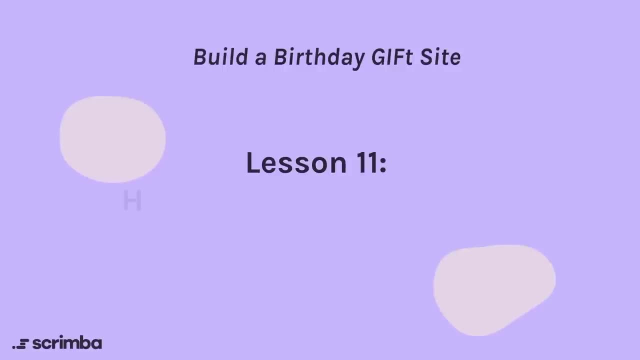 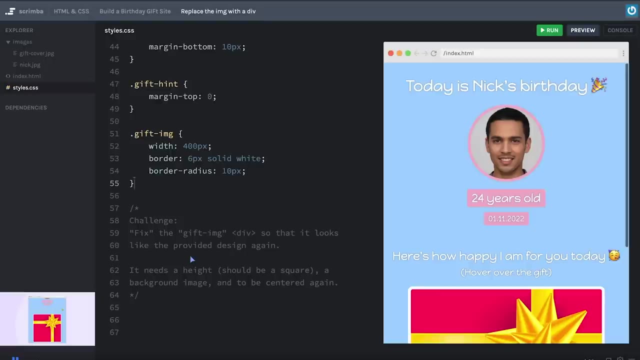 did great job. Let's carry on with this course. Okay, now we're going to prepare our project so that we later can add the hover feature. So we're not going to add the hover feature. So we're not going to add the hover feature, but we're going to. 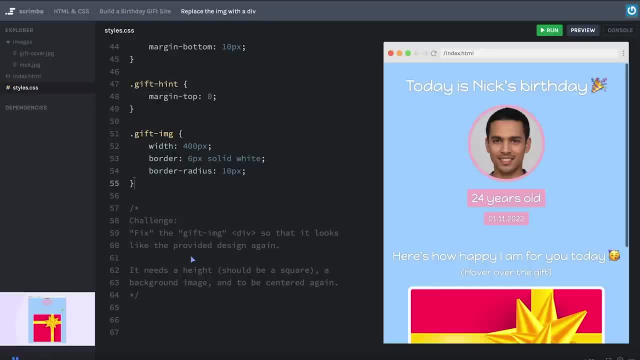 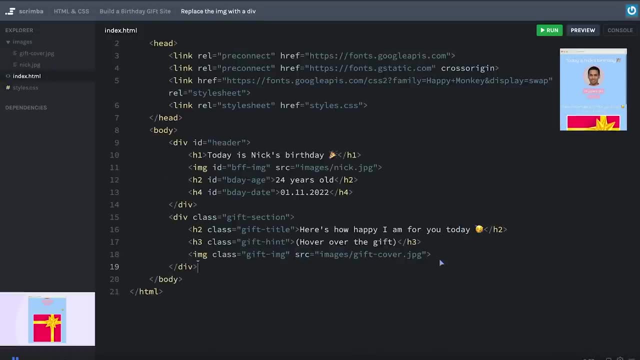 add the hover feature right now. we're just going to set the stage for it, And in order to do that, I'm going to first mess up this project a little bit, And then it'll be your job to fix it, Because we are not going to use the image tag here in order to display this gift. Instead, we are going 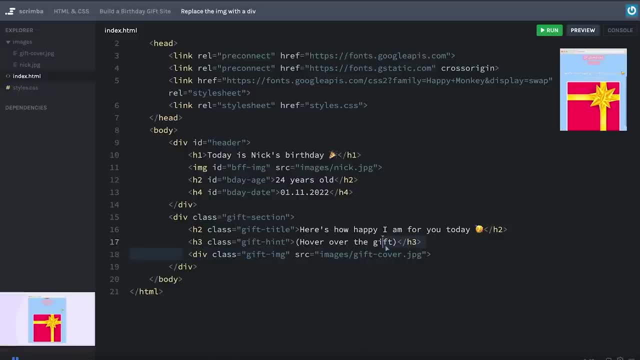 to use a div tag. I'm changing this into a div, which means I also need to close it like that, because divs are not self closing as IMG tags are. And then, next up, divs don't have a source attribute, So we can't use this in order to display the image. If I now 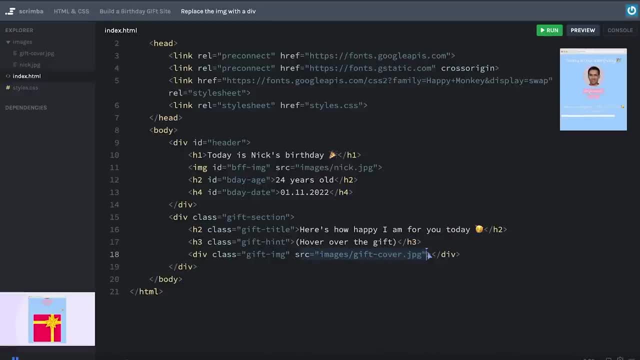 run this, you can see, boom, suddenly our image is gone. This SRC attribute has no place here, because instead we are going to render this image through the CSS background image property, So I'm going to remove this one. if we run the code again, you can see nothing else has happened And 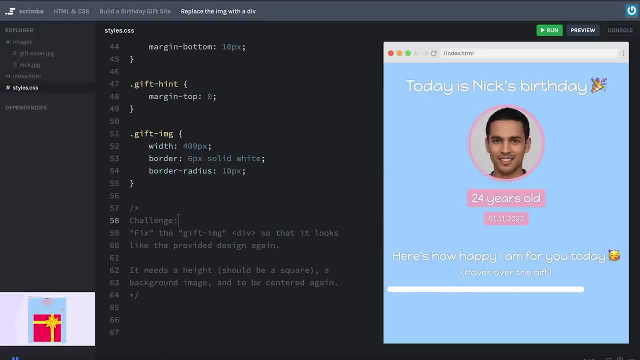 moving over to the CSS. Now it is your job to turn this weird line here into something that looks like exactly what we had before. I messed up the code here, So you are to fix the gift IMG div, because I kept the class right here So that it looks like the provider design And a little bit of a hint. 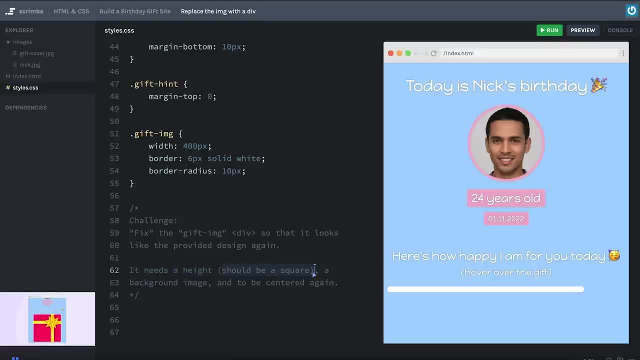 it needs a height, And if you wonder how much, I want it to be a square, so equal width and height. it also needs a background image, which is how you'll render this gift cover. that also should be centered again, Because, as you can see here's, this looks very much left aligned. 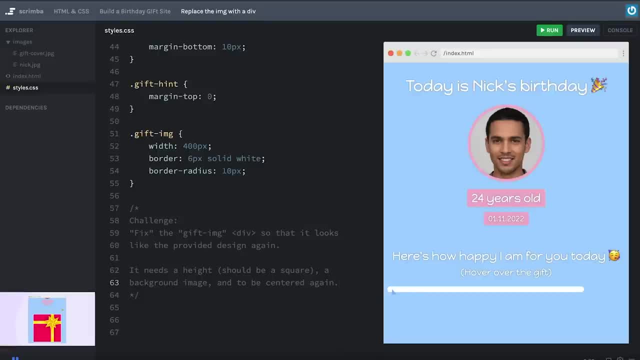 So, basically, what's happened here is that the div has zero height, because the div has no content inside of it, So the only thing that's visible is the border, which spans 400 pixels, starting from the left hand side and over towards the right hand side. So go ahead and give this a shot, And then I 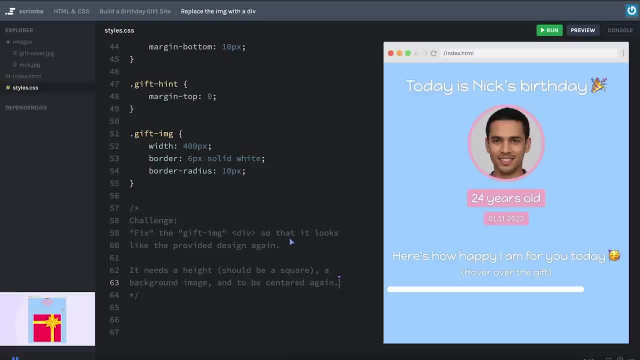 will show you the solution when you return back to me. Okay, let's do this. First, it needs a height equal width and height. So let's just do it and set it to 400px, Like that. As you can see, we now 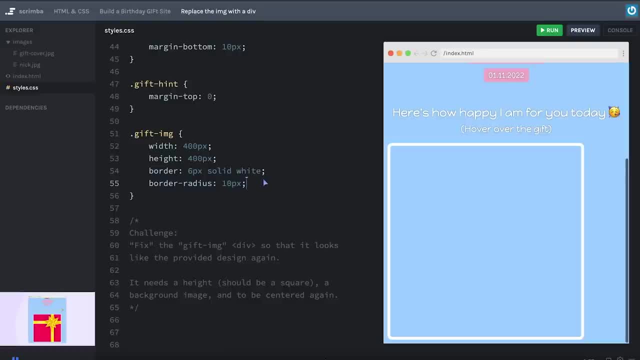 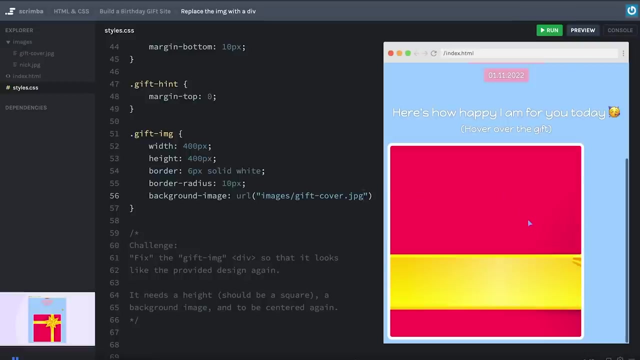 have a empty div on our page. Next up we're going to set the background image. So how do we do that? Well, you've seen that one before: background image URL and then point it to the images folder and the gift over dot k, peg, And there you go. But what is happening here? it seems like we only kind of see the top left corner of the page. So let's go ahead and do that. So let's go ahead and do that, And let's go ahead and do that. So let's go ahead and do that. So let's go ahead and do that, And. 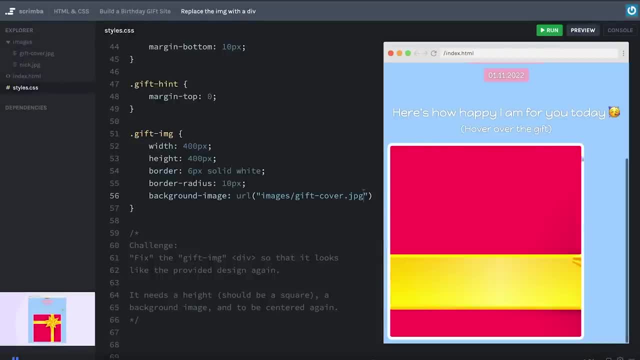 let's go ahead and do that, So, let's go ahead and do that, So, let's go ahead and do that. And that is because the image itself is huge, much larger than this 400 by 400 pixel container. So we need to use 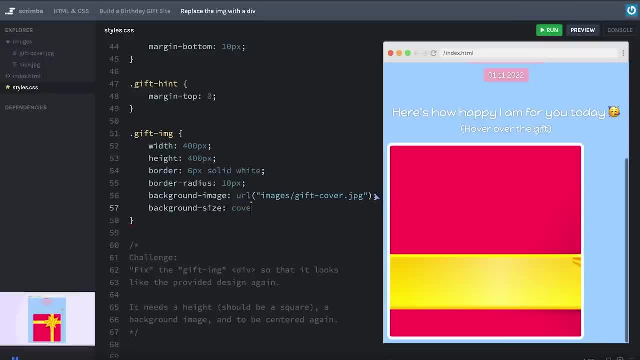 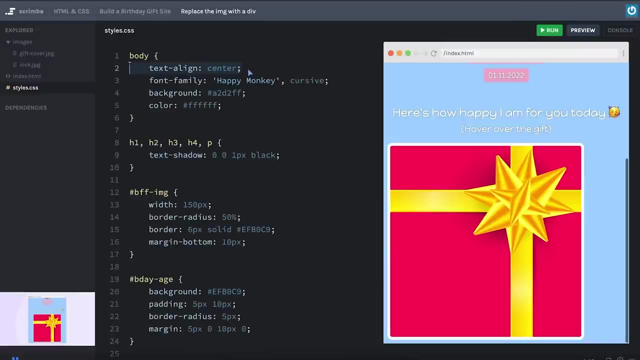 our good old friend background size and set that to cover, And that squeezes our large image into the current width we have available here Now. finally, why isn't this element centered anymore? Well, the centering of the image used to happen because the text align is set to center, but text 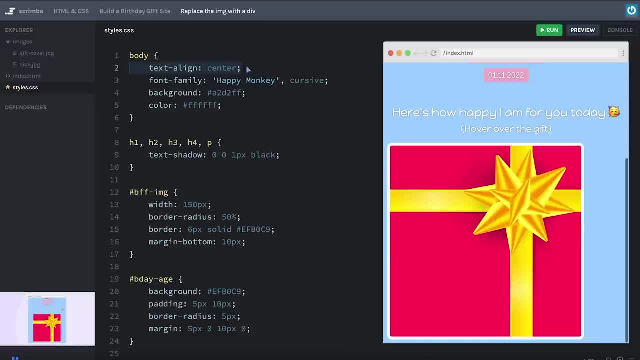 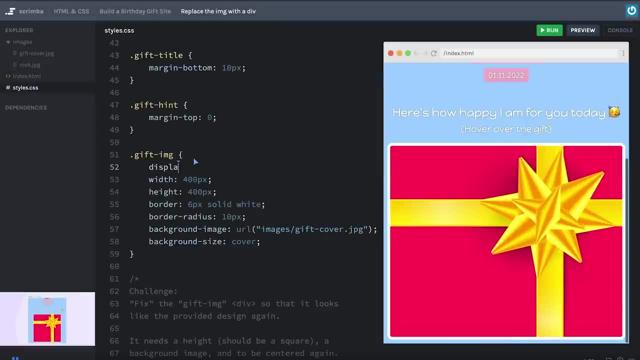 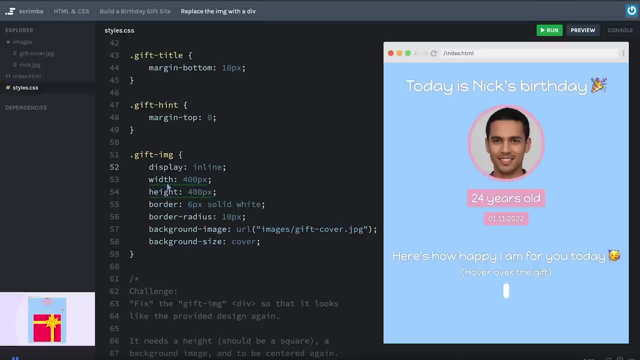 align will only center inline elements inside of its container And, as you hopefully remember, divs. they are not inline, they are display block And you might have tried to do display inline like that. then you can see that doesn't really work. Then our width: 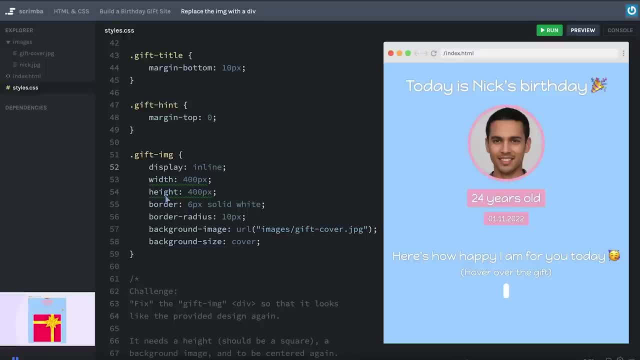 property and height property gets this weird underline underneath them, because they are simply ignored by CSS, Because you can't force the width and height of an inline element, as they should only be as large as the content inside of them are, And this div doesn't have any content. 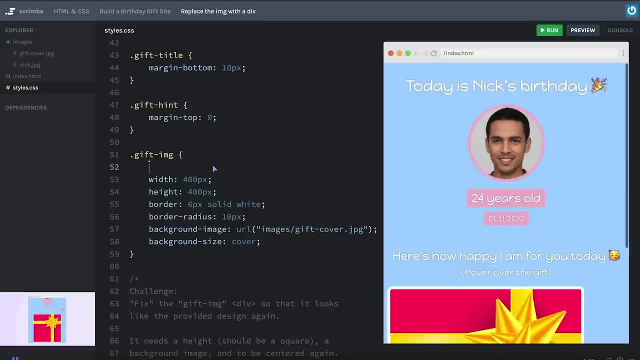 So we can't really use display inline. What we rather can use is the margin technique you learned earlier, the one where you set the left and right margin to auto, because that works on elements that are display block and which have a set with. let's do margin zero on the top and bottom. 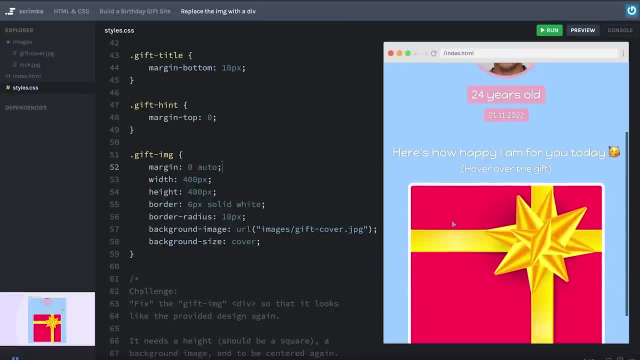 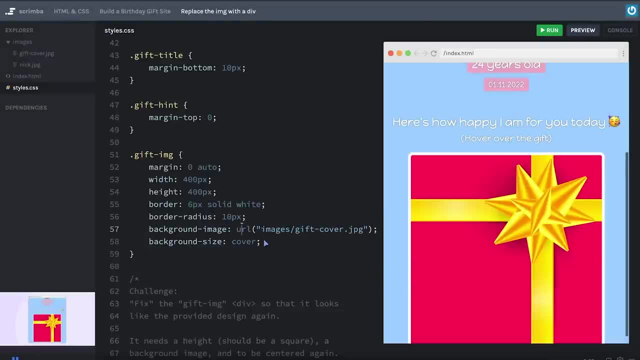 and auto on the left and right. And there we go, We have it centered, we are back to our original design And we've set the stage for our hover effect, which Nick is going to be so glad to experience. So it's really cool that you've made it this far. 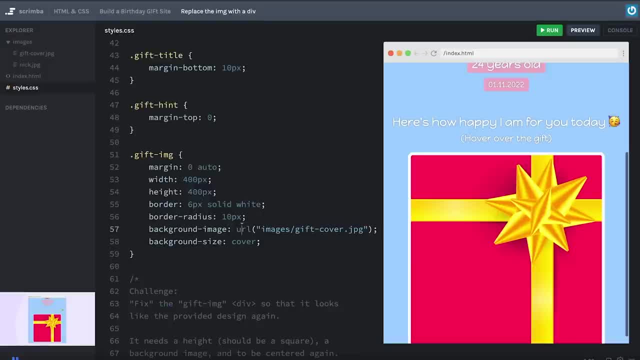 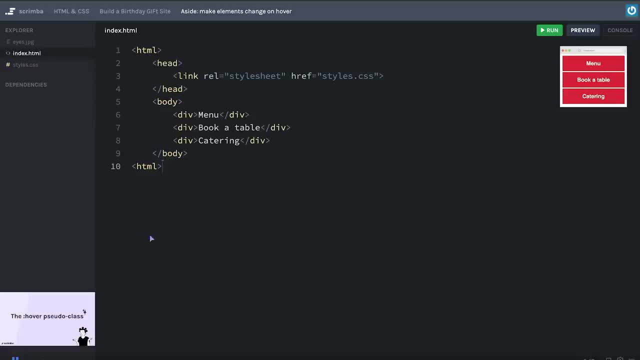 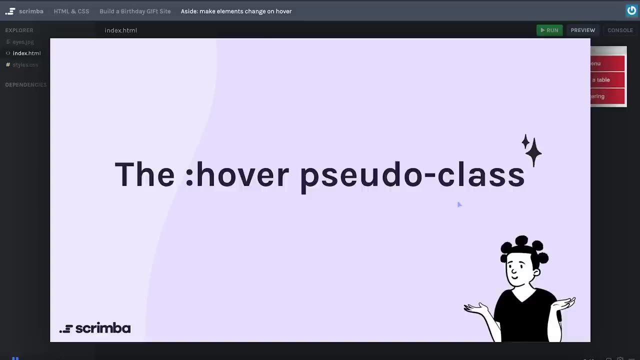 And let's just keep up the pace and move on to the next scrim. In order for you to build the next feature for our birthday gift site, you will have to learn about the hover pseudo class. So let's take a step back from our birthday project and learn all about this. 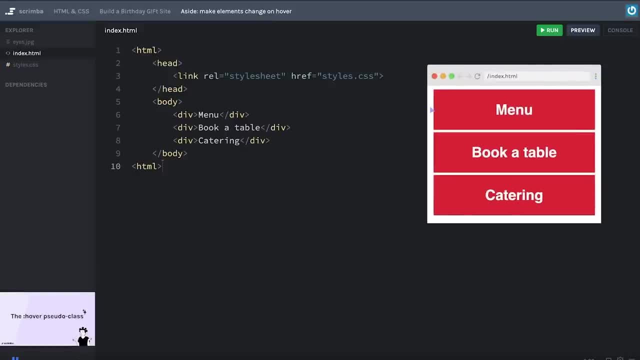 hover pseudo class For it. I've created this little fictional website for a restaurant. It is just a virtual website that lists all the features and features that will be available to you For the very simple site that has three divs that are meant to be navigation items, where you 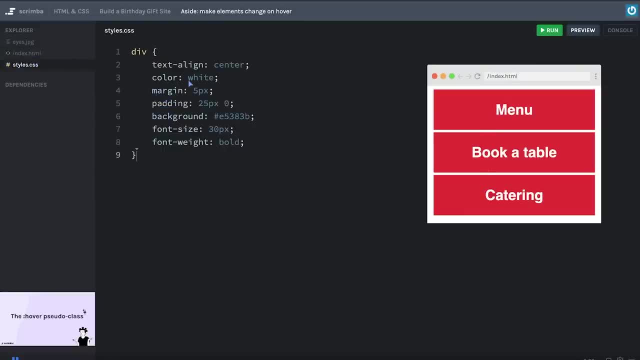 can look at the menu, book a table or order catering. If we head over to the CSS, you can see that the only styling here is a set of rules that are applied to the divs, that is, the three menu items. what I've done is simply align the text to the center. I've 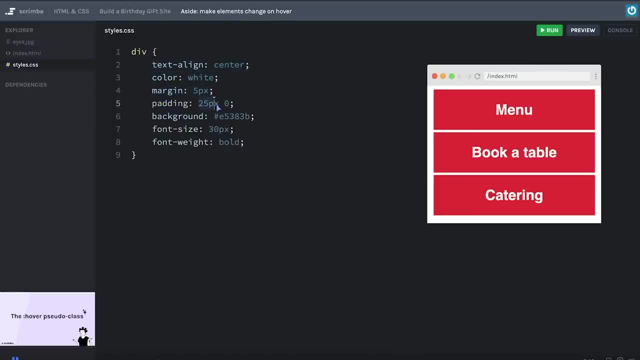 set the text color to white, given it some margin, some padding. on the inside of the menu items. I've added this red background color, cranked up the font size and also made the font bold. Now what would be really nice is if these elements changed slightly when. 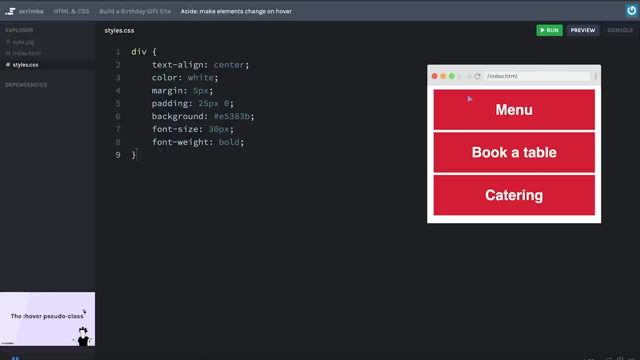 the user hovered over them, so that we gave the user some visual feedback hinting to the fact that these should be clicked, and also just making the site feel more alive. And that is where the hover class comes in, Because what we can do now is if we target, 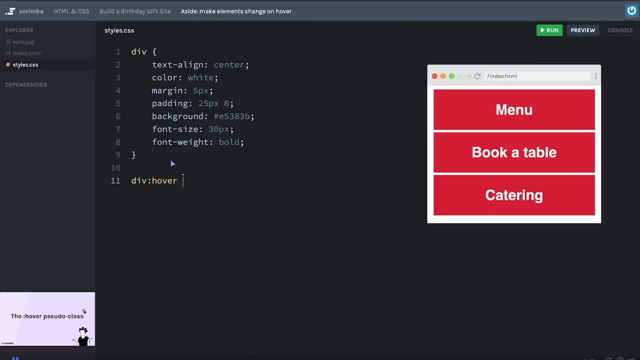 the same divs and then add a colon hover and opening up the curly brackets. then we can write specific rules that only are applied when the elements are selected. So, for example, we can change the background color to this color right here And this hexadecimal. 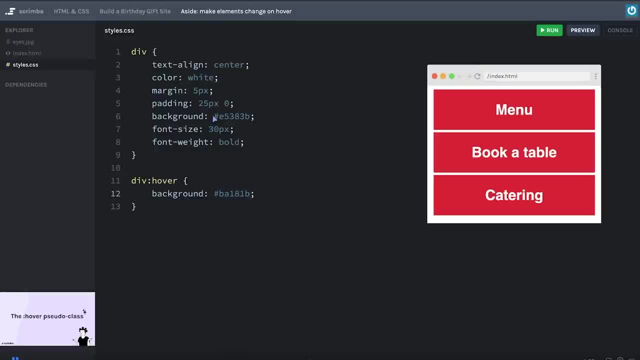 value probably doesn't tell you anything, but I can disclose that it is a slightly darker shade of this red hair. So now, if I hover over the items, boom. you can see that the background is suddenly a little bit darker than the other items. So this gives a nice 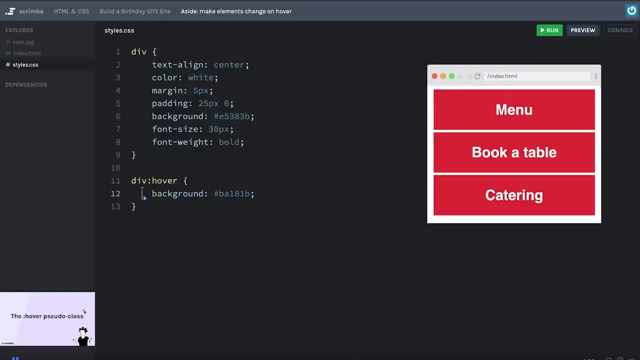 feedback to the user. So what's going on here is that this line takes precedence over this line. then any div is hovered over And we can also, for example, increase the font size 40 pixels. Let's see how that works. All right, now it really stands out when you hover over one. 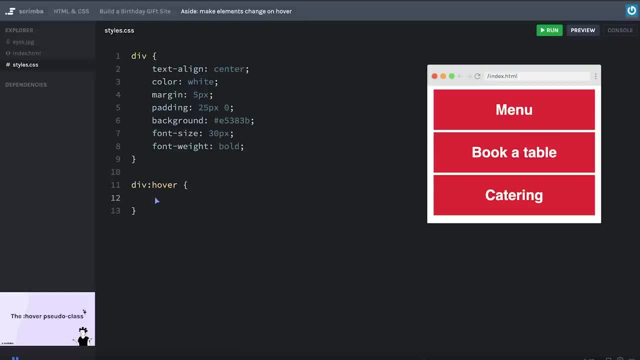 of the elements. And let me show you a cool trick to prepare you for your next challenge, Because what you can do is actually do background image And then, as you know, use the URL CSS function and point it to a image source, the image lying around in the file system right here. Let's try them So eyes dot JPEG. 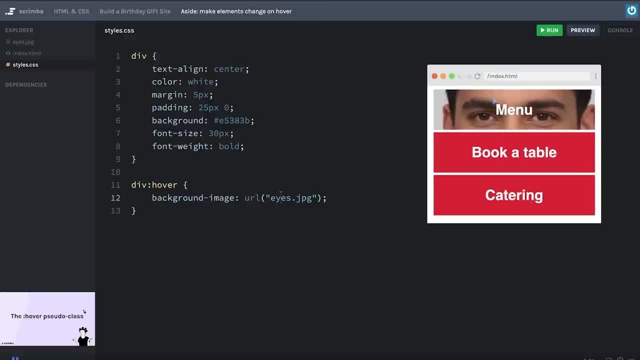 we now hover over the item, we can see our good friend Nick staring back at us. That is probably the creepiest restaurant menu I've ever seen, But the point is only that you can change the background image on hover, So hopefully this has prepared you for your. 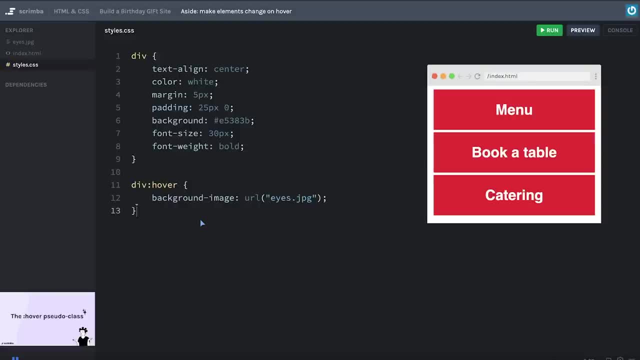 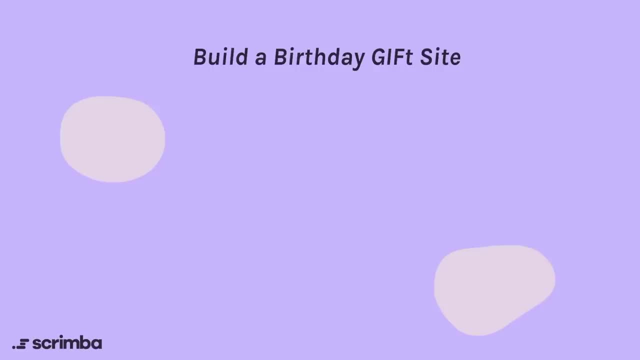 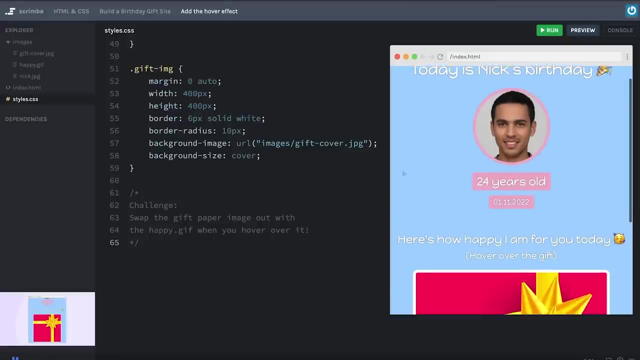 next challenge, Because when we return back to the birthday gift site, you are going to work with this hover class In order to help Nick unpack his gifts. So let's return back to our main project. Okay, now we are getting into the fun stuff here, Because now we're going to create this epic. 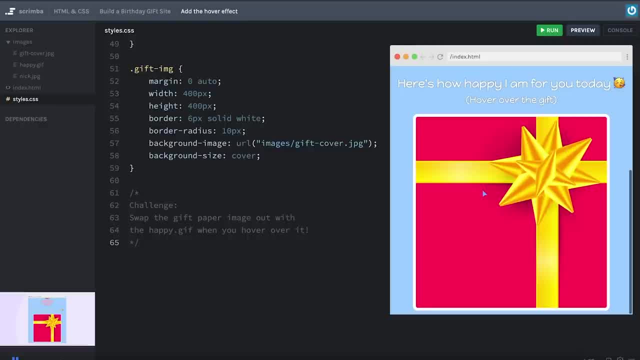 feature where Nick, when he hovers over the gift paper, gets revealed an underlying gift that makes him feel happy and appreciated on his birthday. So the challenge is described here. you are to swap the gift paper image out with the happy gift when you hover over. 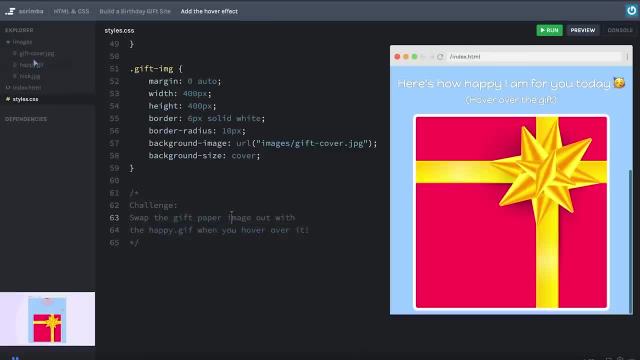 the gift paper. So the happy gift is added here in the images folder. I'm not going to show it to you. I want you to solve this challenge in order to see this gift. Now, the gift paper image you are to swap out is this div. right here. As you remember, we gave it a background. 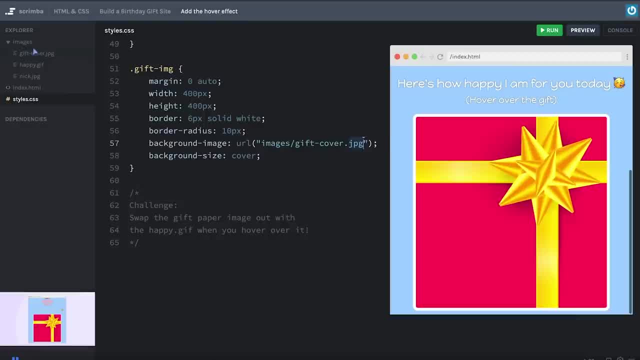 image, which is the gift cover dot JPEG file, which also is in our images folder. So go ahead and solve this challenge right now, And then I will show you the solution when you return back to me. Okay, hopefully that went well. What we'll do is first target this gift IMG here as we want. 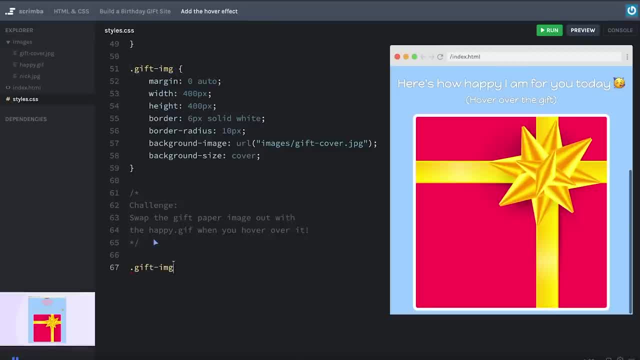 to create a hover effect on it. So I'll do gift IMG colon hover. Now, whatever CSS properties and values we are setting inside of these curly brackets will be applied when the user hovers over this gift image. And what kind of properties do we want to change? Well, 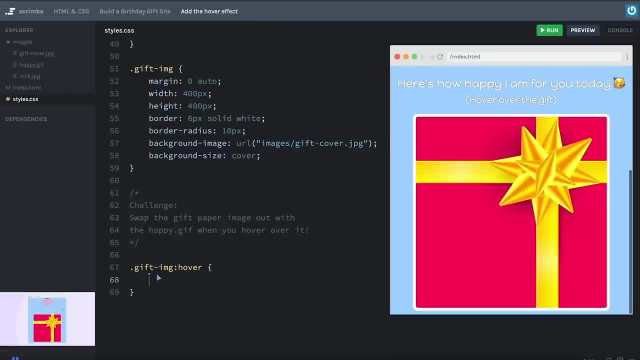 it's actually only one, just the background image here. So I'm going to copy that one, Paste it in. And we don't want it to be the gift cover dot JPEG, we want it to be the happy dot gif, like that. Let's see how this works. I'll move the cursor down towards the 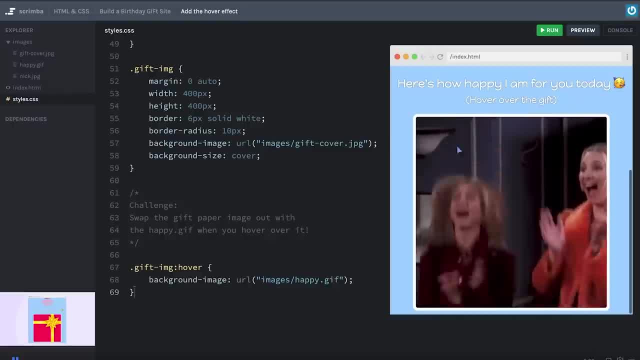 image And when it crosses over, we see Phoebe and Rachel from friends being super happy for Nick on his birthday. And I don't know about you, But if someone told me that they would be this happy for me on my birthday, it would make me feel so grateful and appreciated. 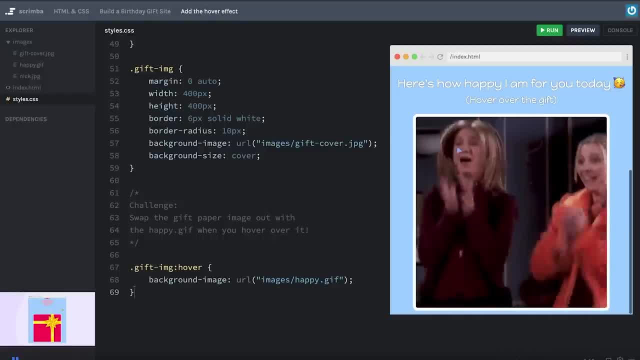 So we are really doing a good deed creating this website And you know what I'm going to do: a little bit of work here. So I'm going to go ahead and create this website And you know what I'm going to go ahead and create this website And you know what I'm going to. 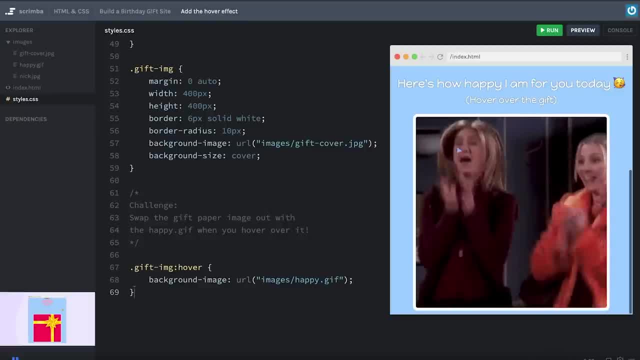 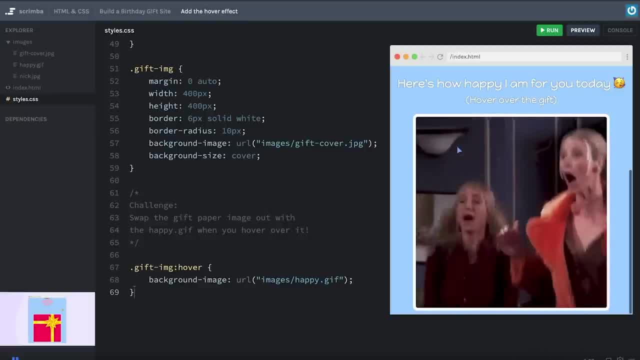 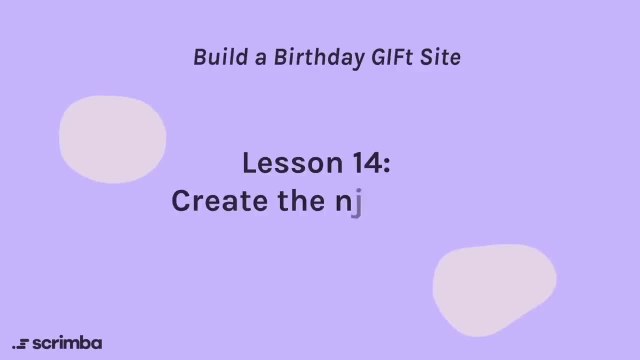 in the course. you've crushed through so many difficult CSS concepts, So Phoebe and Rachel are also sharing for you. take a moment to appreciate that and then I will see you again in the next scrim. Okay, now that we've made sure that Nick feels appreciated on his birthday. 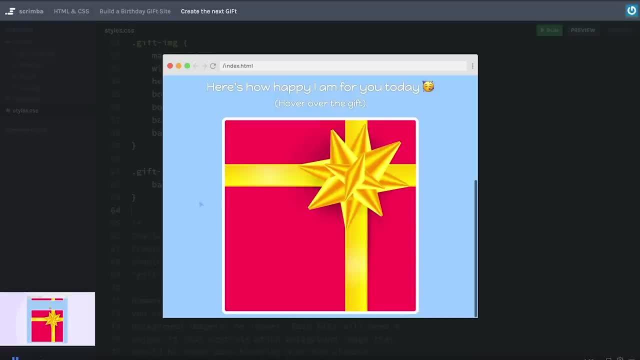 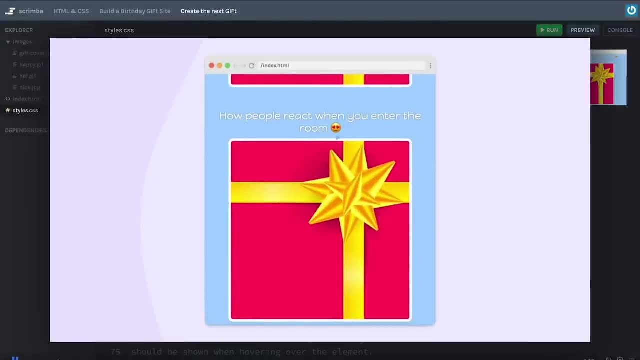 through this Phoebe and Rachel gift, let's make sure he also feels really good looking, Because now we're going to create this gift right here which says how people react when you enter the room, And the gift will show when he hovers over this element. is this hot? 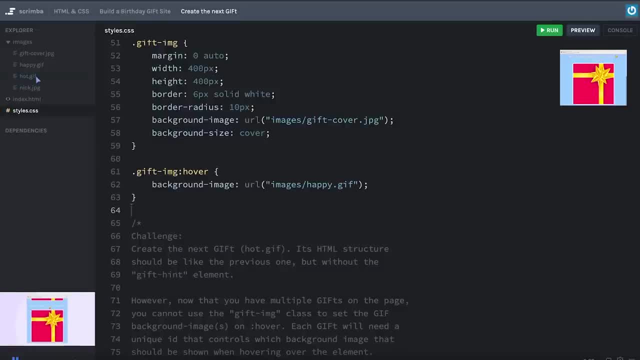 gift up here. I'm not going to show it to you now. you're gonna have to solve the challenge to see it. And speaking of that, let's have a look at the challenge text. So you're to create the next gift which uses the hot gift, And it's HTML structure should be like the: 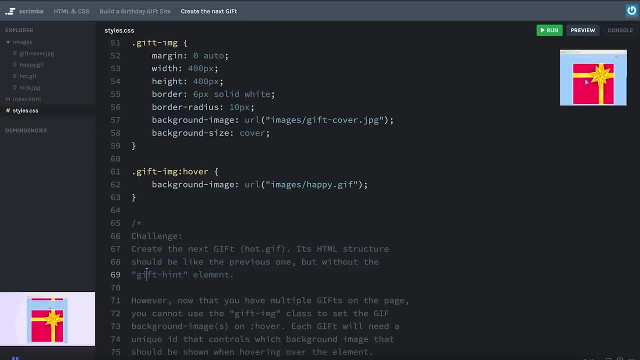 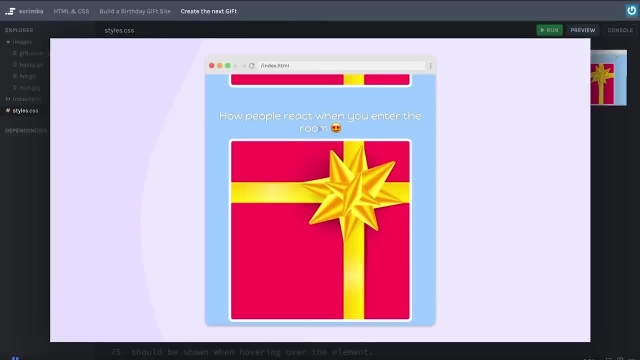 previous one, but without the gift hint element, because, as you can see, here we have this hint written in parentheses. however, that's not needed For this one. I think Nick will probably get the point by the time he scroll down to this. 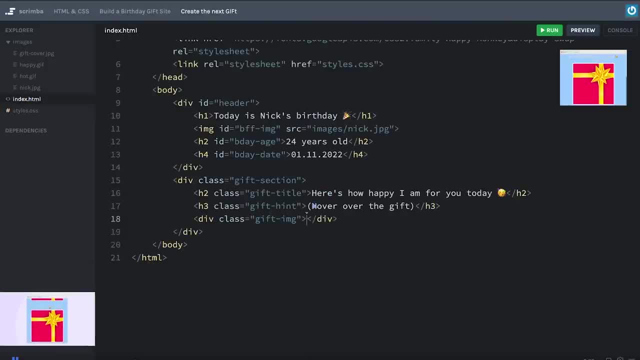 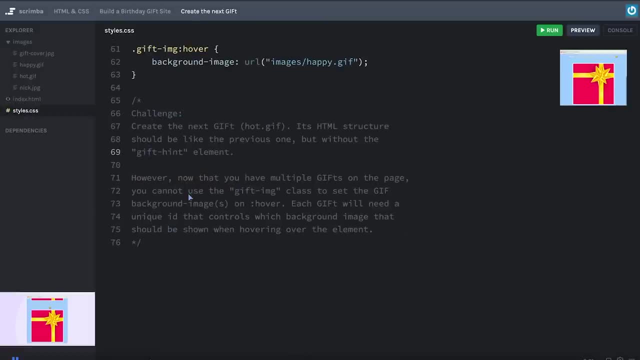 one, So let's just skip it. But other than that, you can simply copy paste this section And then, of course, change the text as well. However, you will need to do some more things as well, Because now that you have multiple gifts on the page, you cannot use the gift. 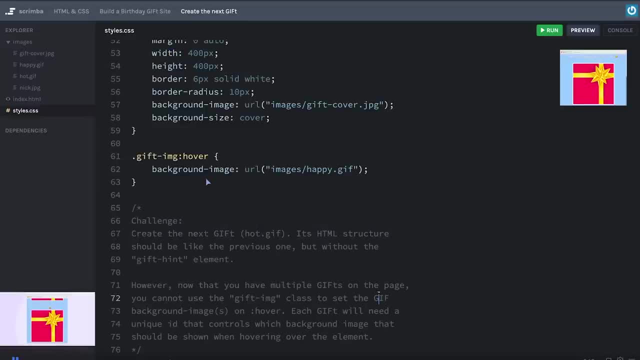 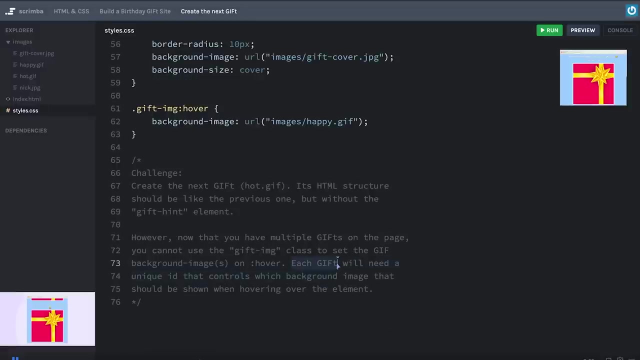 image class to set the background image on hover. That is this one right here, Because if you have multiple gift image elements on the page, well then every single one of them will just show this happy gift, And that's obviously not what we want. So instead, each of the gifts will need a unique ID that controls 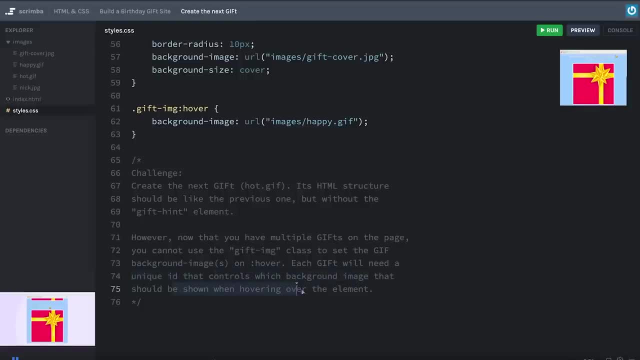 which background image that should be shown when the user hovers over the element. Okay, that was probably a lot to parse for you, But if you didn't quite catch it, just go ahead and try to solve the challenge, Because I think you will see this problem sooner, or? 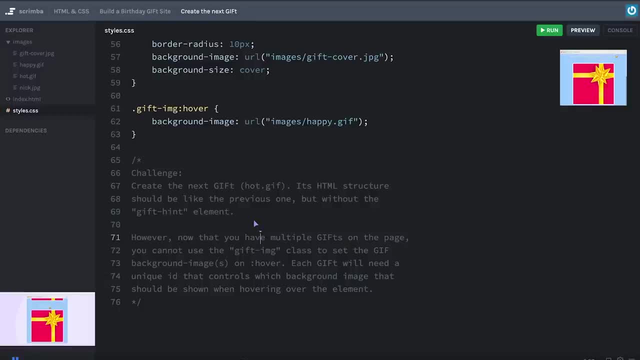 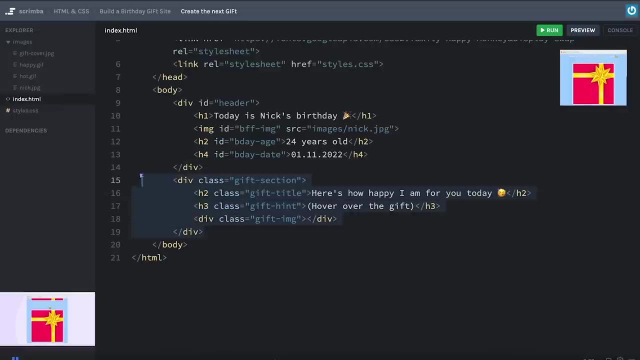 later. Anyway, you definitely will actually. So make it your best shot, And then, of course, I will show you the solution when you return back to me. Okay, let's do this. So, starting in the HTML, by simply copying this one right here and: 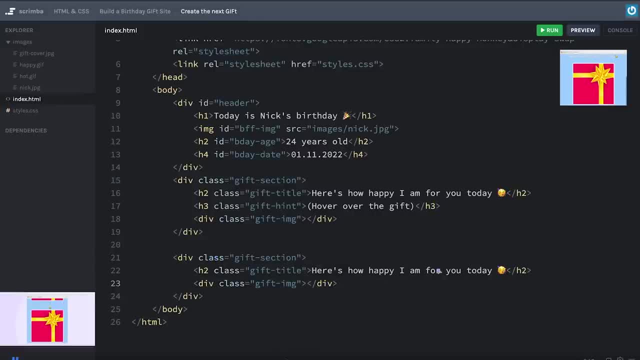 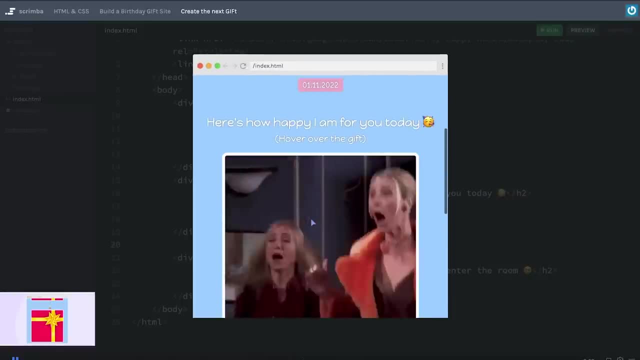 pasting it in that down here, removing the gift hint, because we don't need that, And then updating the title. Let's run the code now, And here we can see the first element with Phoebe and Rachel. Let's scroll a bit down. 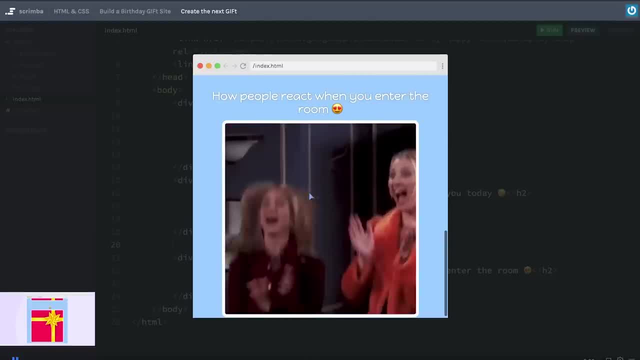 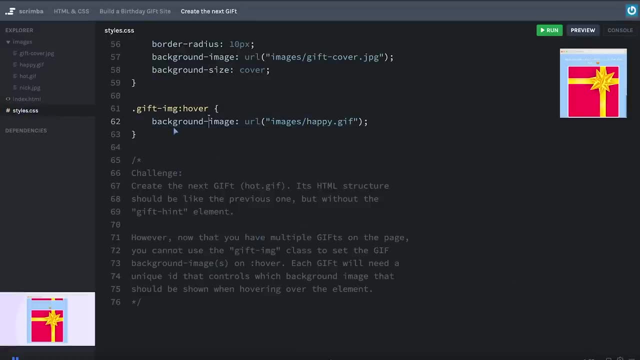 And there we have our second element, though it still shows Phoebe and Rachel. So that is a problem And that is because, as I said, this gift image class just sets the background image on hover to the happy gift on both of these elements right now. So we can't use. 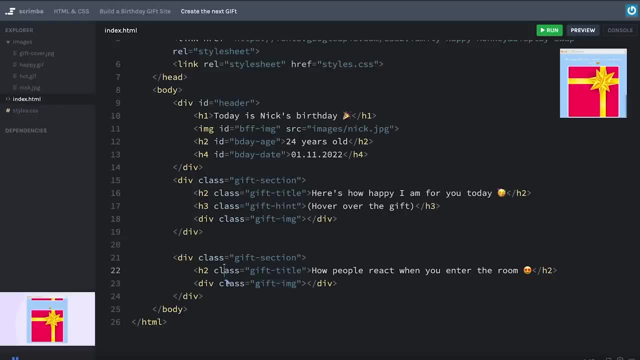 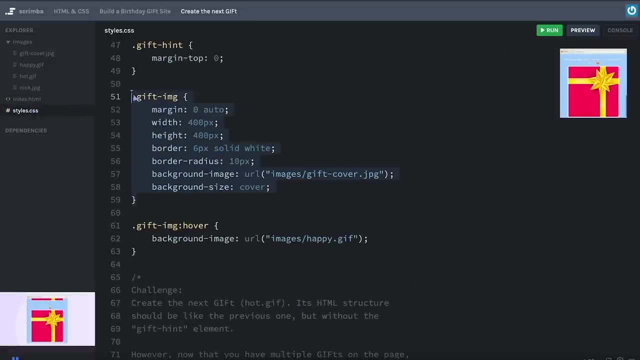 a class. for this we need a unique ID, But we're not going to remove the class of gift IMG, because it actually gives a lot of styling- actually all the styling- to the element, And so it's only the hover pseudo class that needs to be applied to something else. So let's. 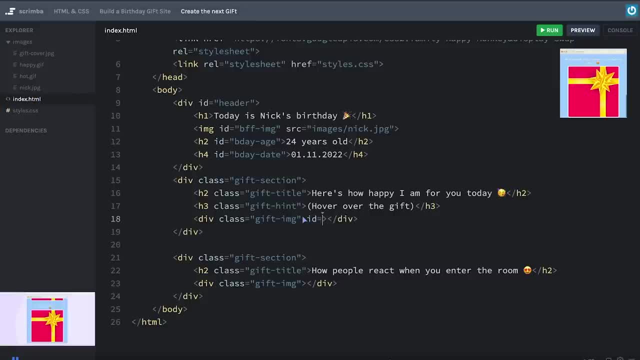 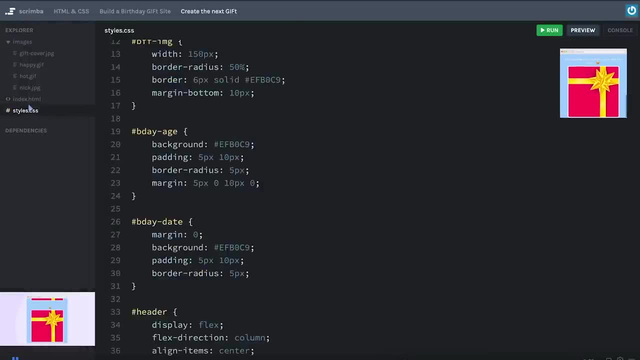 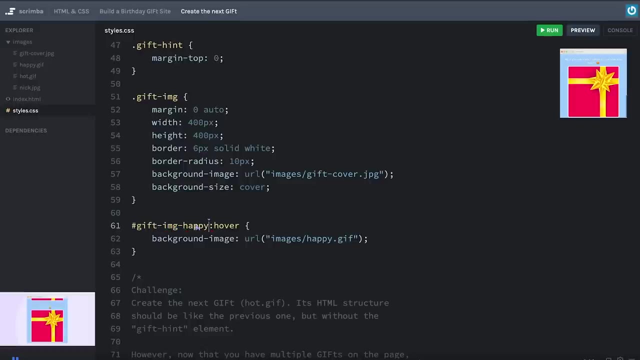 instead now on the first one here, add an ID that we'll call gift dash- IMG- That's happy. We'll run the code so that it's applied And then, instead of referring to the generic class here, refer to this gift IMG- Happy ID. Now, if we run the code, you can see that it works. 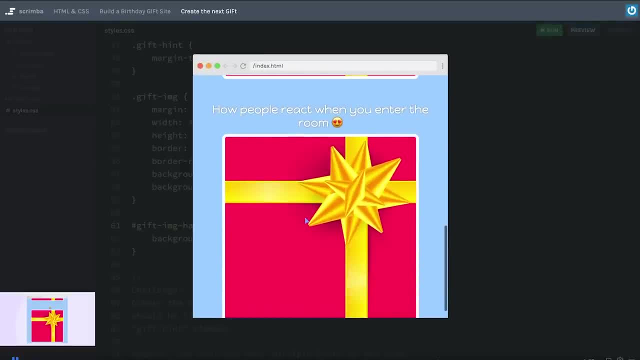 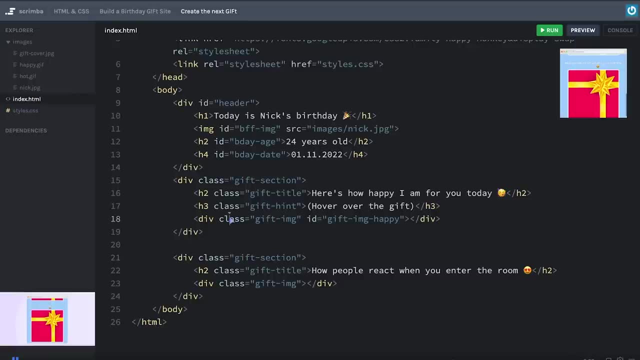 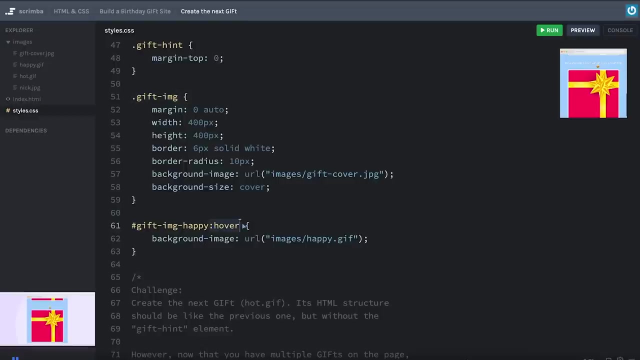 on the first gift, though. the second gift Now lacks a hover effect, And that is because the only hover effect we've applied now is on this specific ID here on the first gift, Previously we used the generic gift IMG class, So it was applied to all gift images, But now the hover only works on the first one. 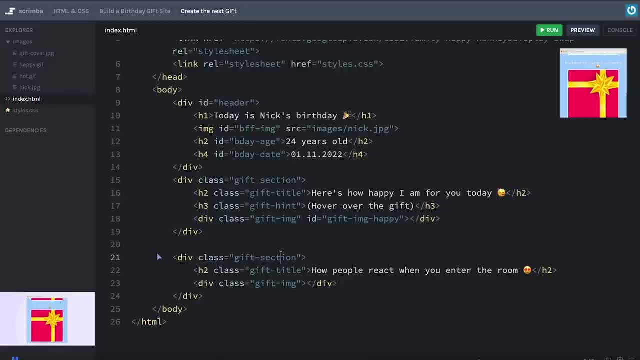 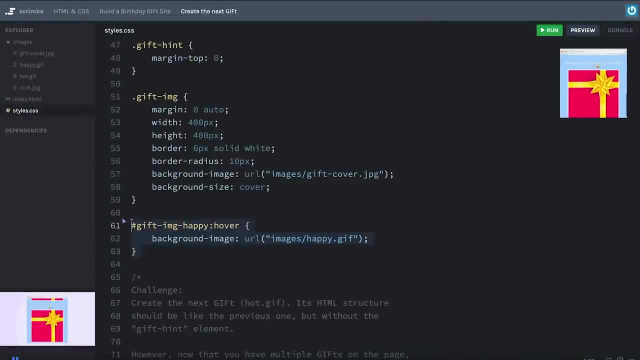 So what we need to do is use this exact technique, but on this section as well. So I'll create an ID on this section and call it gift dash, IMG- dash pot. I'll run the code so that it's applied And then, since I'm lazy, I'll copy this, If IMG. 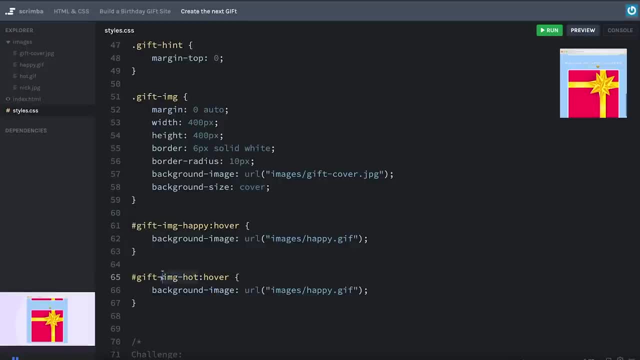 happy should be changed to gift IMG hot, because that is our new ID that targets that element And we don't want to show the happy gift, we want to show the hot gift. So let's see if this works. Here we are at the section when we hover over the image. we see someone. 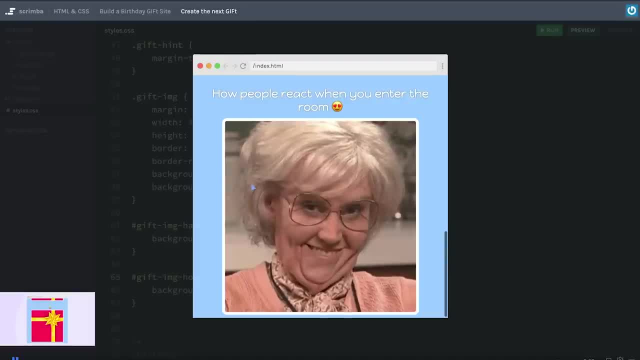 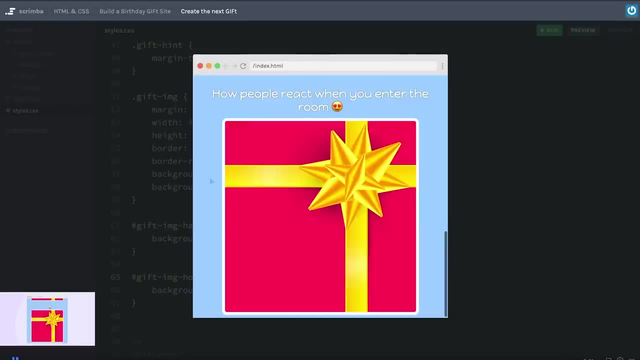 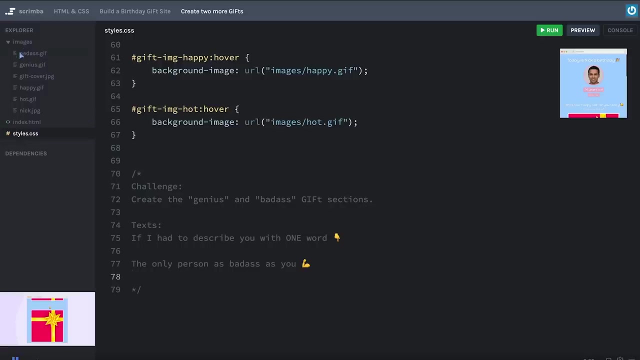 looking pretty interested in Nick, So I think he will feel really good looking And hot on his birthday when he sees this gift. So great job solving this challenge. Let's move on. As you can see over in the file system, I've added a genius gif and a badass gif, So your 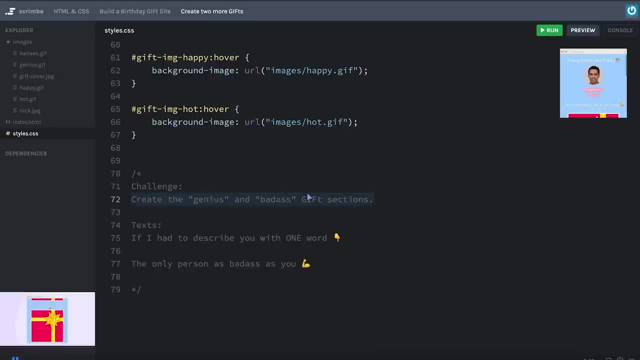 job is now to create the genius and badass gift sections. they should look exactly as the hot section, So I'm not going to give you any more instructions, other than giving you the titles, so that you can just copy them from here Instead of writing them out on your own. 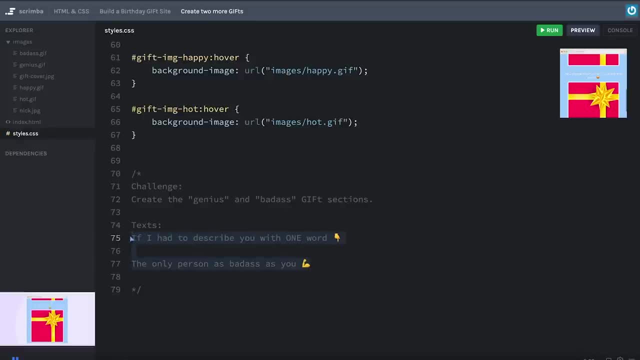 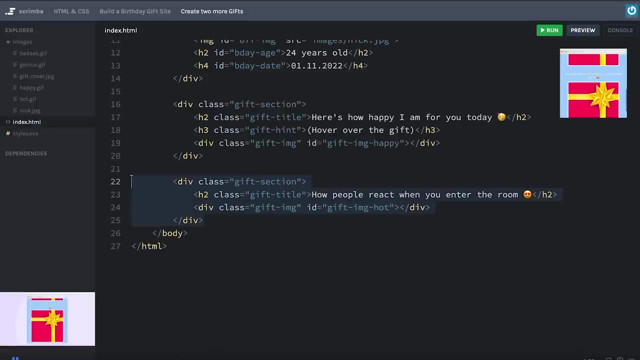 So go ahead and create these two sections right now, And then I will show you the solution when you return back to me. Good luck, Okay, let's do this. So I'm going to start in the HTML file, because we're simply going to copy paste this one. 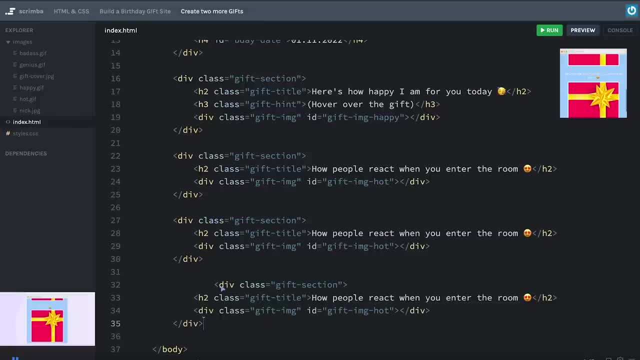 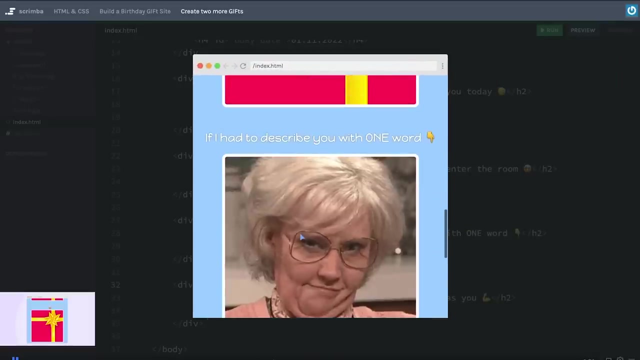 two times, Then I'm going to add the titles. I'll copy this one and paste it in here. and copy this one and paste it in here. Okay, let's run this. Now. you can see we have the hot gif and then the genius section, which still has the hot. 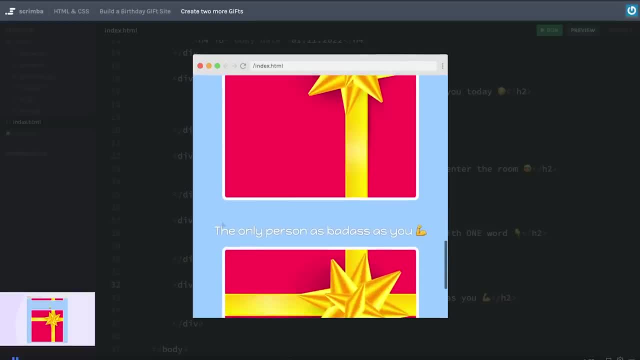 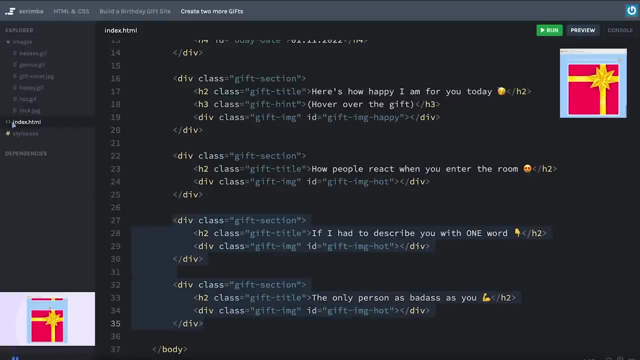 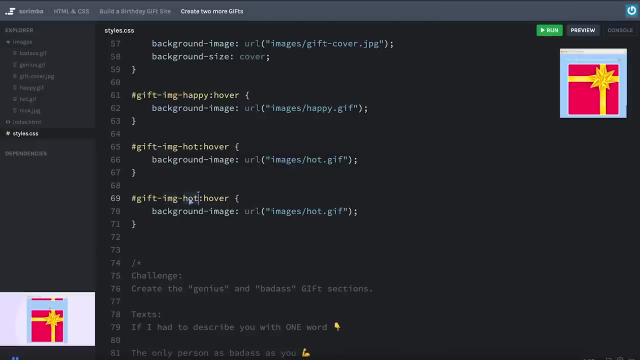 gif underneath it. That's to be expected. And there we have the badass section which also still has the same gif. So now we have the sections rendered on the page at least, but we need to fix up the CSS. So, lazy as I am, I'll copy this one here. just gift image hot. The first one will. 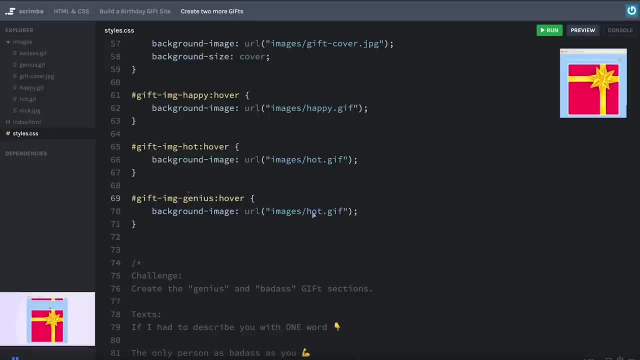 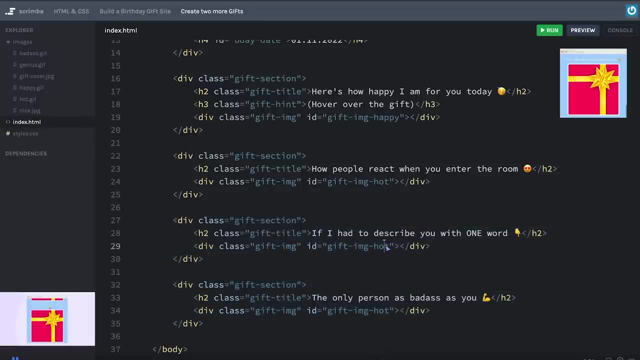 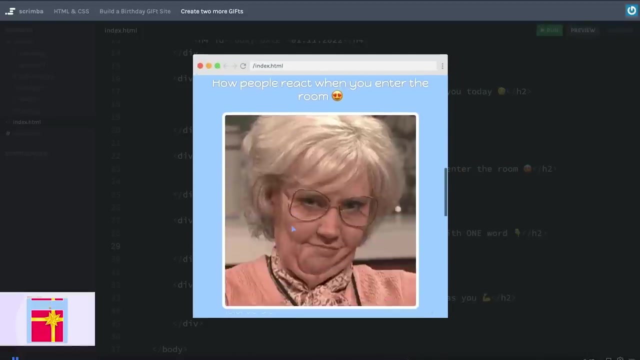 be the genius one, So I'll do genius instead, And that should refer to the genius gif. Now that we have this in place, we can just give this class to the respective image, like that, running the code, And we have the happy gif, we have the hot gif and then the genius gif. 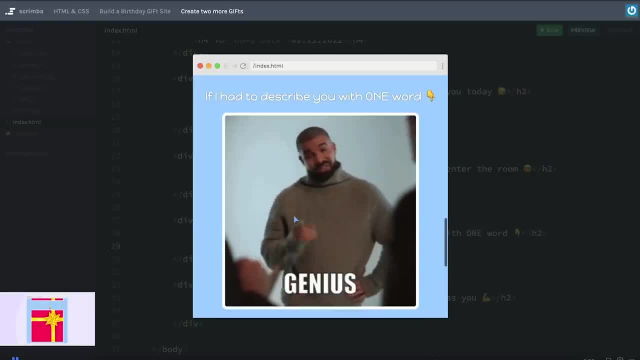 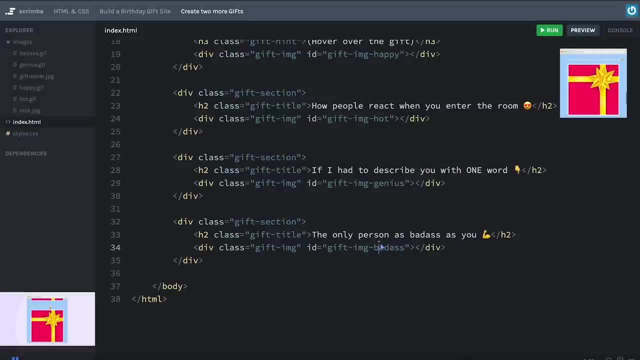 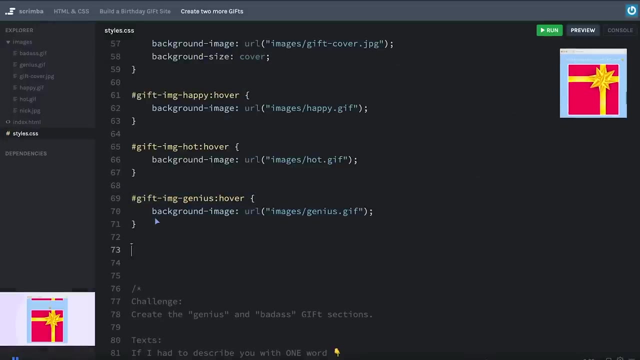 That is pretty cool. I surely think Nick will appreciate this compliment. Okay, the final one. Here, the keyword is badass, So I'll change the ID to badass. now that we are in the HTML and moving on to the CSS, copy this and change from genius to badass, because that's the 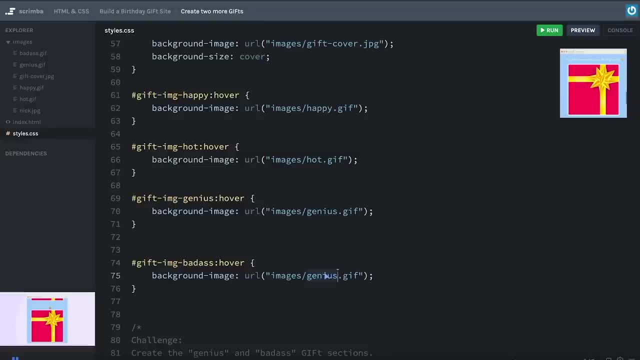 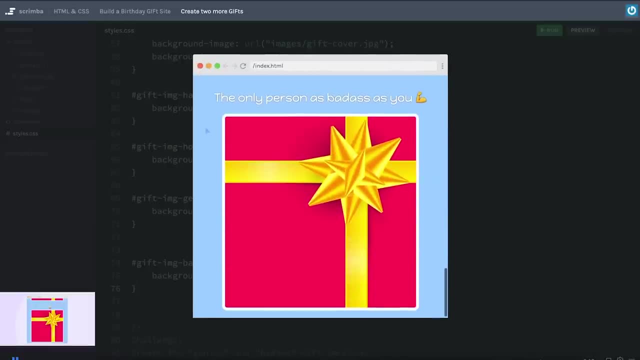 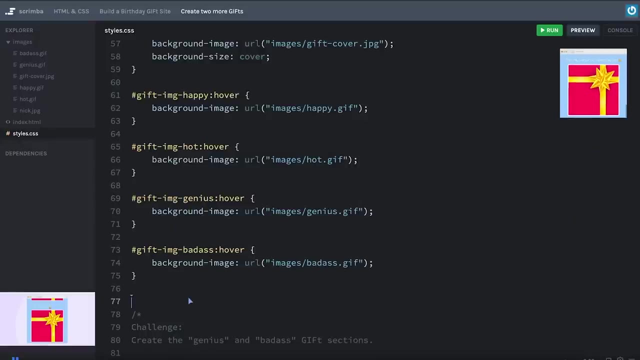 ID we just created and the gif we want to fetch out from our images folder is the badassgif dot gif. Let's open up our example again. scroll down to who is the only person as bad as as you. it is, of course, Chuck Norris. All right, we are done with this challenge. 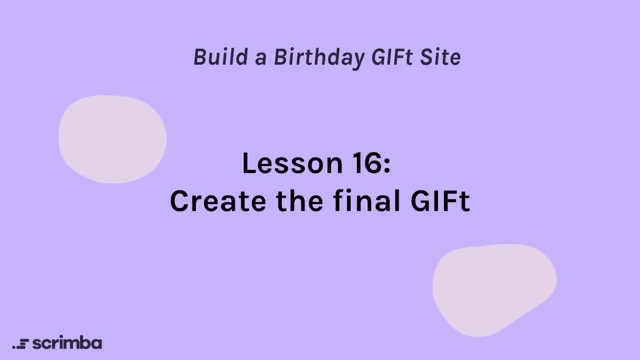 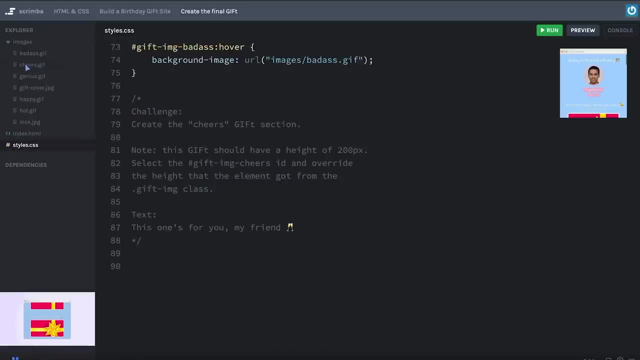 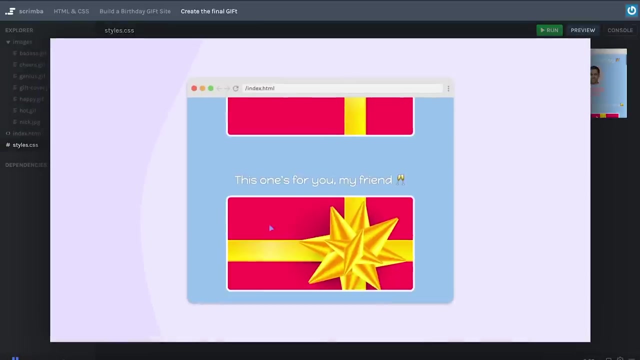 Great job, Let's move on. Now. it's finally time to add the very last gift, And that is the chairs gift. So you're going to have this section, but there's a little difference between this section and the previous ones, Because, as you can see, here it is not squared, but 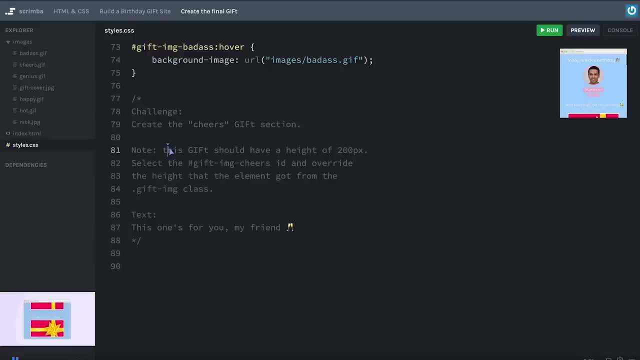 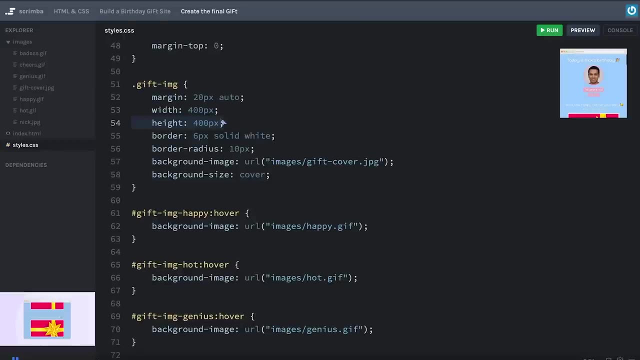 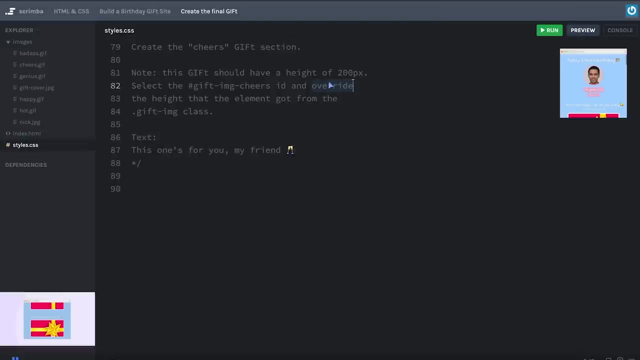 rather more rectangular. So what I want you to do is give the gift section a height of 200 pixels, which is different from the original height that we controlled up here on the gift IMG class, where we set it to 400 pixels. So the way you are to change this or override 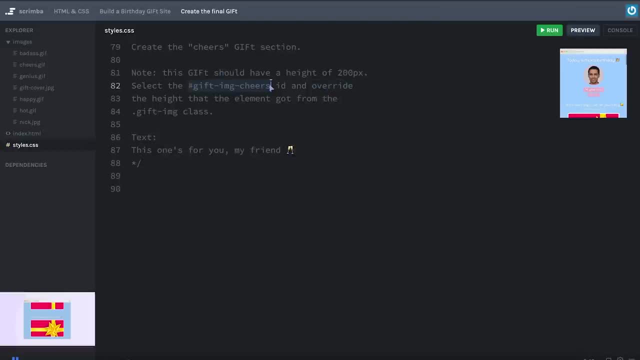 it is by selecting the gift IMG chairs ID which you are going to create- just like you've created IDs For all the other gift images as well- And then you're going to set the height on that element, which essentially means to override the previous height. And finally, here is 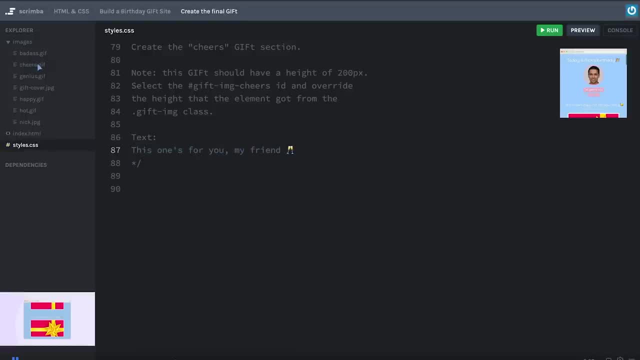 the text as well, along with the chair skiff up in the file system here, And I really think you'll enjoy this one. So go ahead and give it your best shot, And then I will show you the solution when you return back to me. Okay, let's do this. I'll start in the HTML by again. 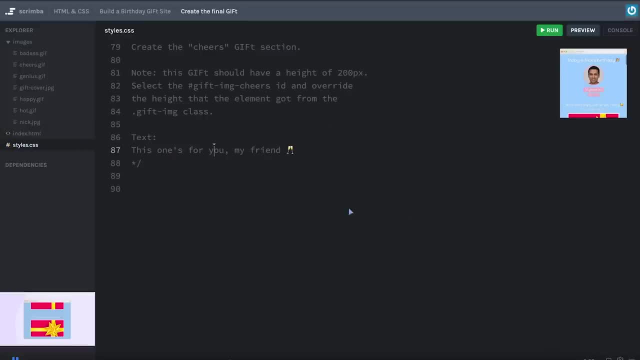 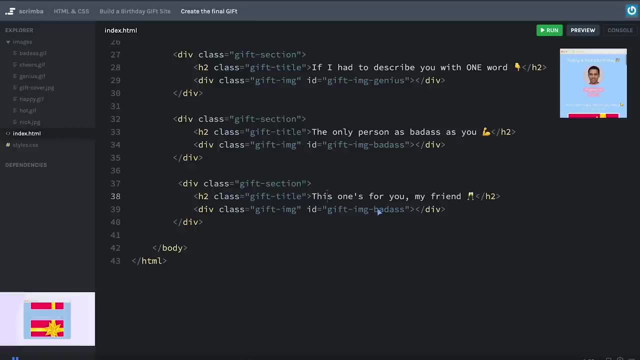 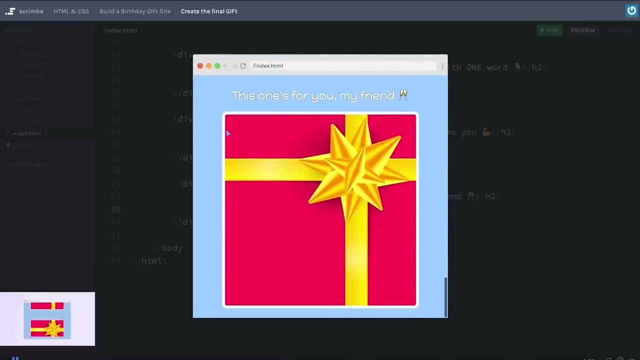 repasting the previous section, And here I need to change the text first. So I'm going to do like that, And then we're not going to have badass, rather chairs. So, running this, we can see we have a squared image in place. That's not exactly what we want, So we need: 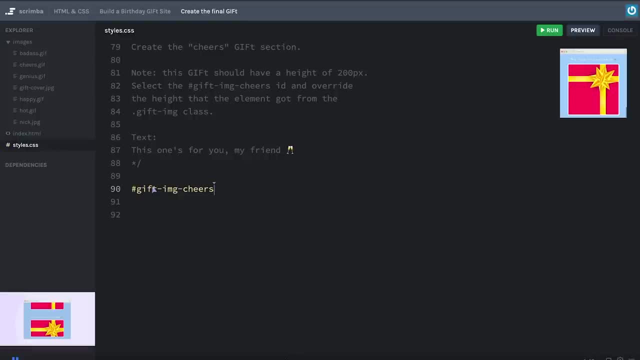 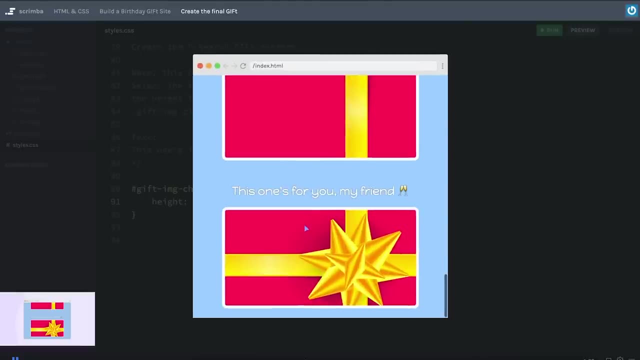 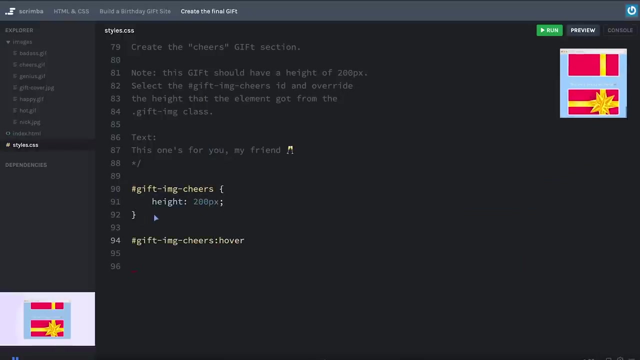 to do the next step, which is to use this ID, which we just created, and override the height, or the height 200 pixels, like that, And there we can see, it is now just as we want it. The final step, then, is to use this hover pseudo class in order to change the. 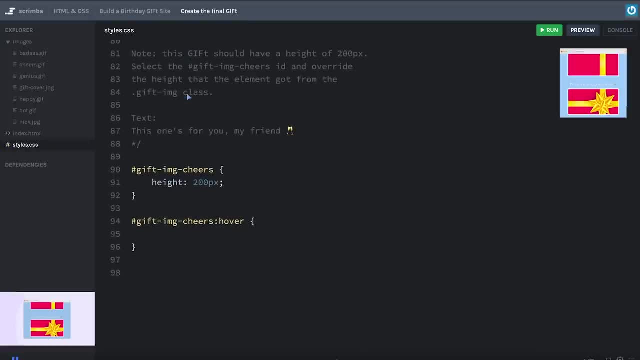 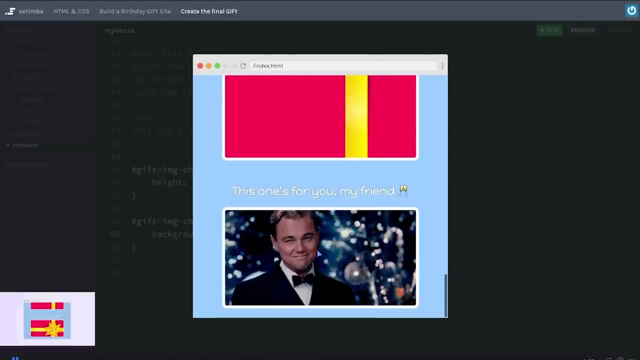 background image to chairs. I'll copy this one and do chairs instead. And now, if we hover over it, we see Leonardo DiCaprio in a smoking giving us a toast- Really nice. And one thing I want to mention here is that the image is not going to be the same color as the background. 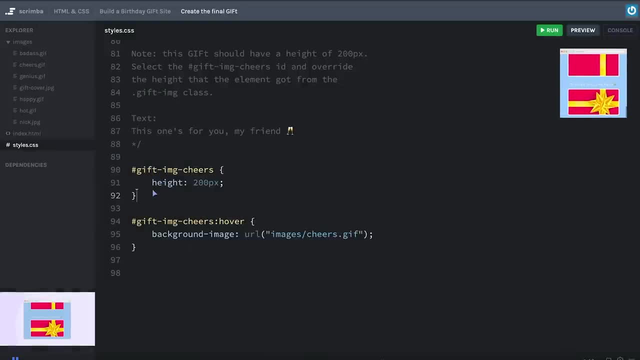 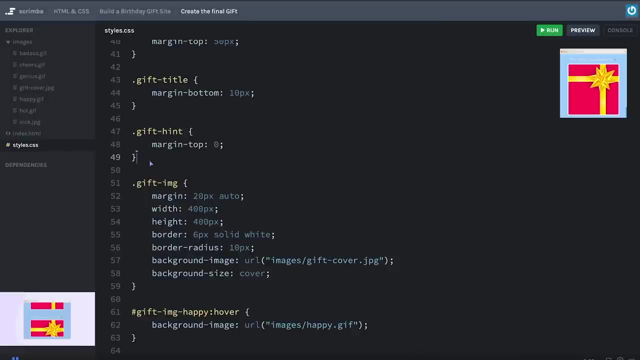 I want to mention here is that you might be a little bit confused as to why this height property takes precedence over this height property, And it is actually not, because this is written further down in the CSS file. Actually, if we remove it to even further up in the 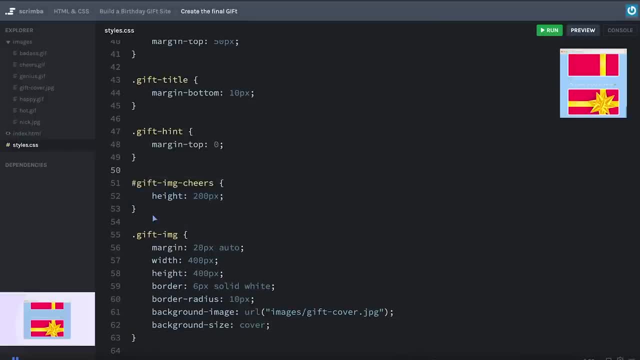 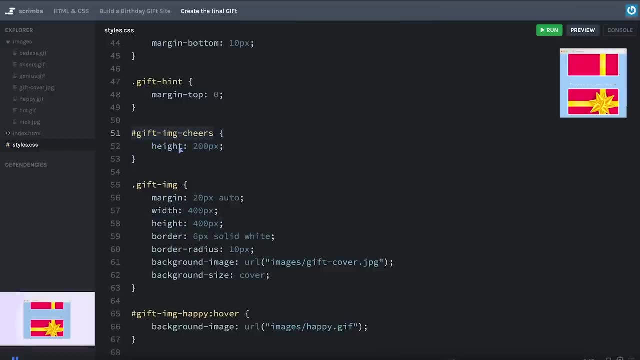 CSS file. even though CSS reads from the top and then downwards, this still takes precedence over this, And that is because of something called specificity, which means that the more specific a CSS selector is, the higher it will be prioritized. And this ID selector. 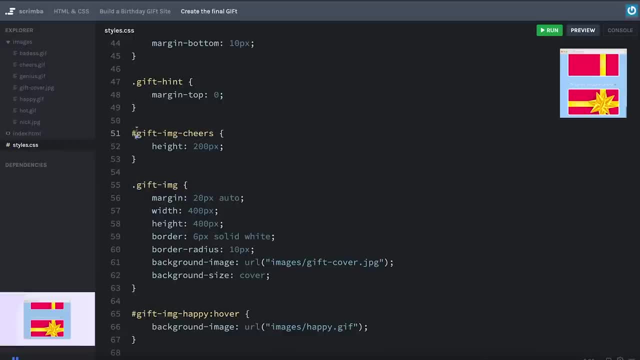 is a more specific selector than the class Because, as you know, only one element can have an ID, whereas multiple elements can share the same class. So IDs are more specific than classes. Now I don't want to get more into specificity. we're going to learn more. 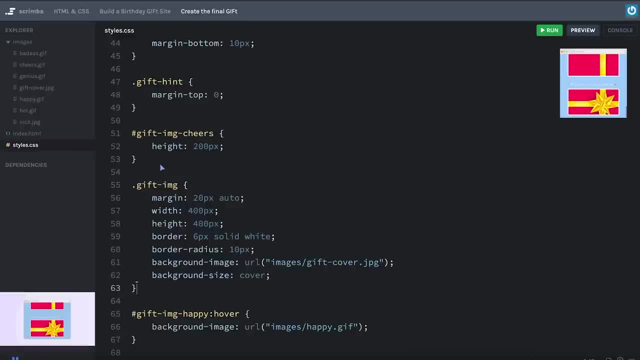 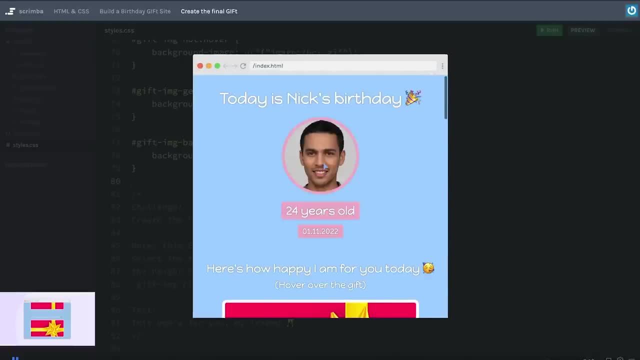 about that later in the front end developer career path. For now, I just wanted to mention it in case you were a little bit confused. So we have now done all of the gifts And we have a super cool birthday page we can send to Nick. there's just a few things left And then we are completely done with this. 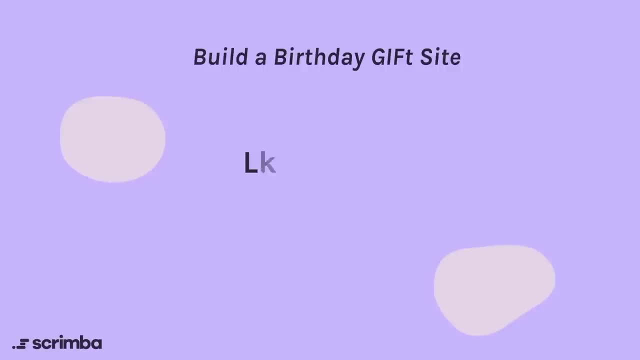 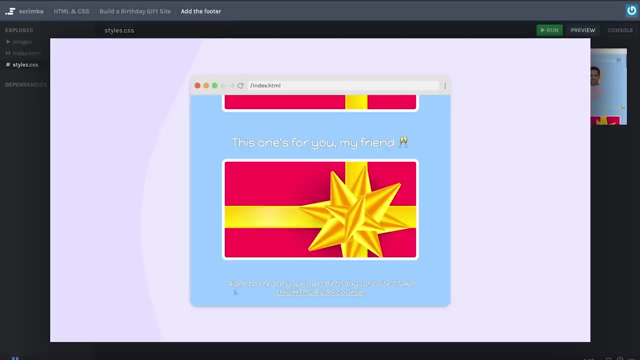 epic birthday site, So I'll see you in the next trim. Now you're going to create the footer for our site, And it should have a paragraph that says: want to create your own birthday gift site. take this HTML and CSS course with a. 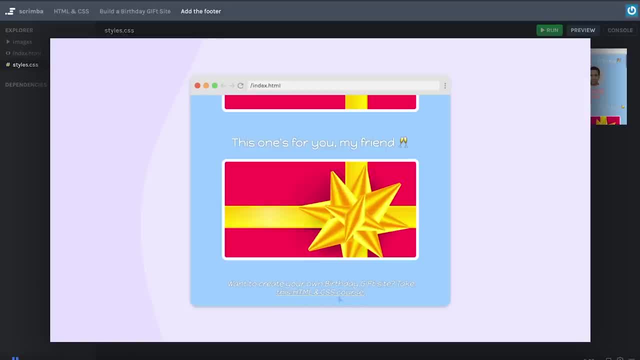 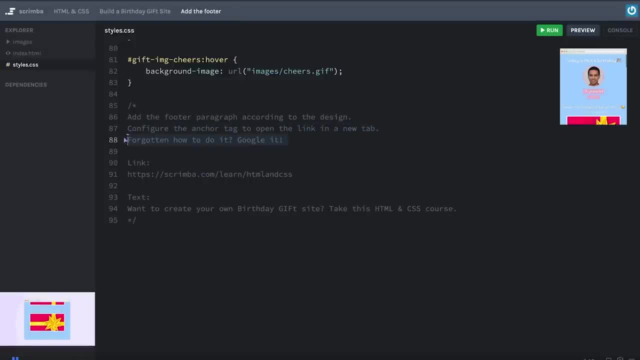 link to, well, this exact HTML and CSS course, And I want you to configure the anchor tag so that it opens up the link in a new tab, And if you've forgotten how to do that, well then you simply have to Google it. I've provided the link right here and also the text, so that you 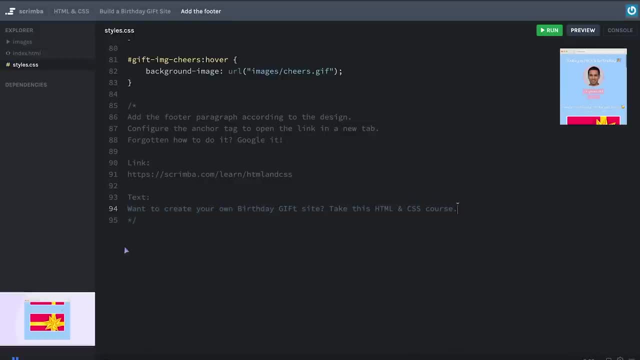 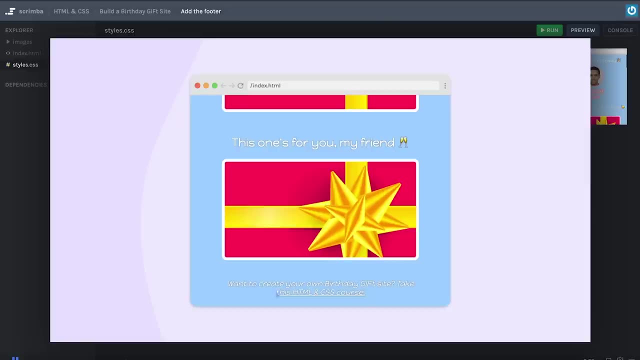 don't have to write that out on your own. However, outside of that, I'm not going to give you any more hints, But I want you to notice that there is some spacing around this paragraph, both above it and beneath it. you can see. it doesn't touch the bottom of the. 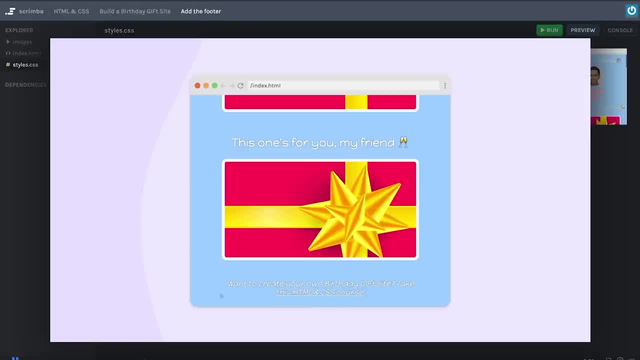 page And also it is centered. it's about as wide as the images themselves And it's also in italic, So you're gonna have to figure out how this translates into CSS. I think you can do it. go ahead and give it your best shot, And then I will see you again when you. 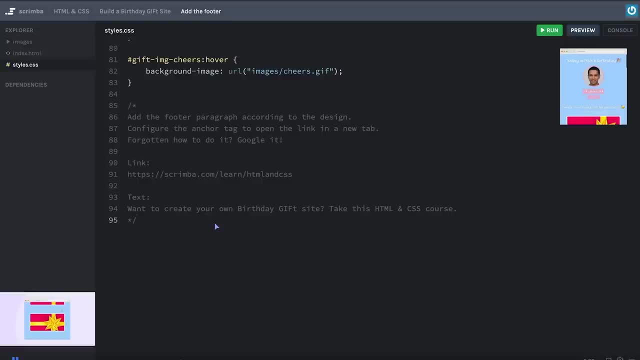 return back to me. Okay, let's do this. So I'll head over to the HTML and add a paragraph which I'll give an ID of footer, And that's it. So we're going to go ahead and configure the page and add. 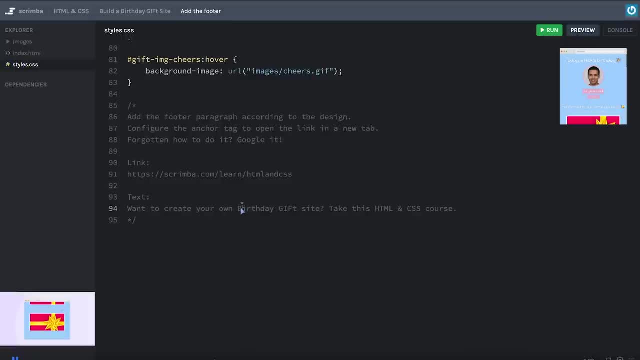 a paragraph. we're going to go ahead and configure the page and add a paragraph. we're going to add a paragraph and this is a paragraph. we're going to configure the page and add a paragraph. then let's paste in the text like that And also the link That's we need to create an. 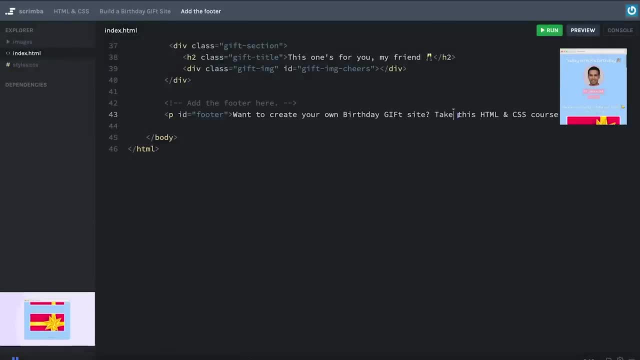 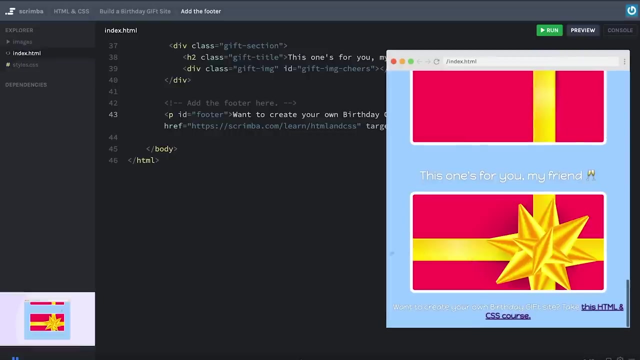 anchor tag And it should be around this HTML and CSS course. So we'll start the anchor tag here, an href, And then, in order to open the anchor tag in a new tab, we'll do target equals, underscore black, And then we'll close it off at the end here. Let's run this, Okay. 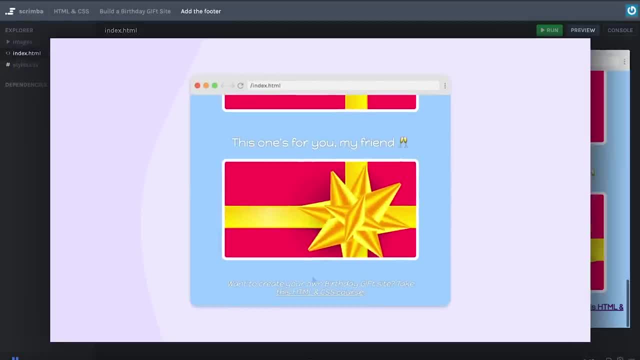 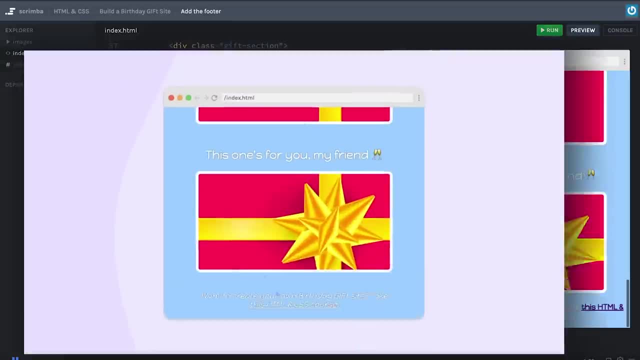 so we have now something that looks not too far from our design. It's decent, but still a lot of things lacking. First of all, this text is far too wide. it should be more or less the same width as the images. So let's do. 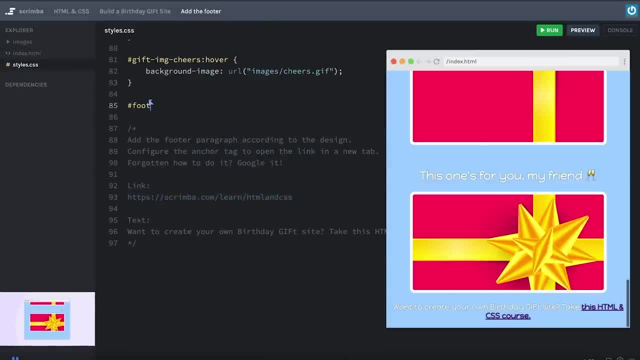 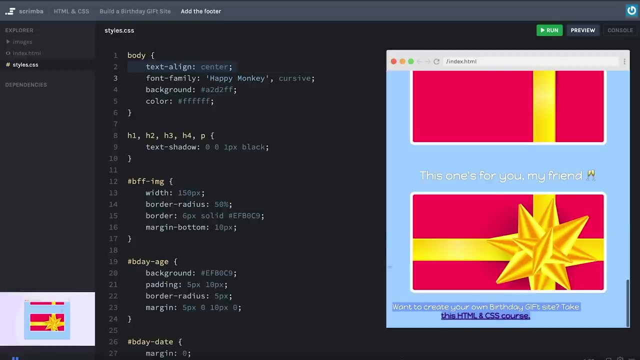 better The width to 400 pixels. Okay, what happened now? Well, we do have text line center, But now that this is 400 pixels wide and it's still a display block element as paragraph, is that the text line center won't center the content here inside of its container. 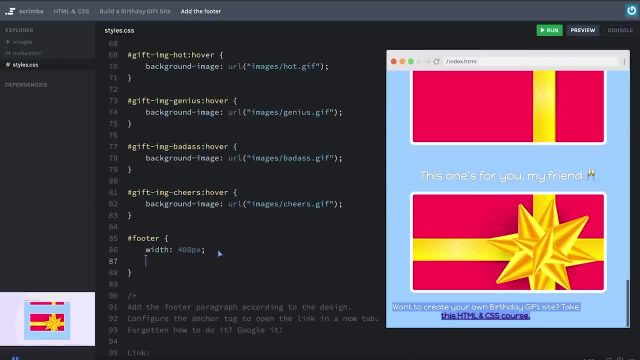 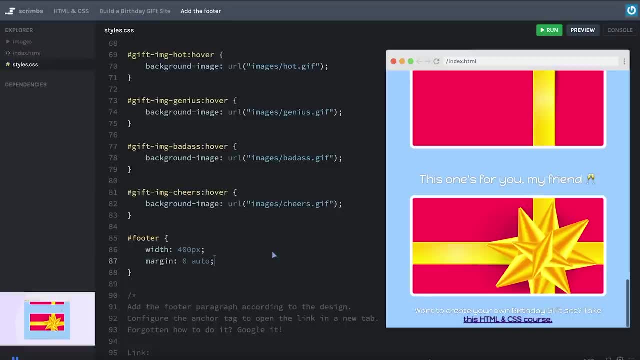 So we need to center it using the margin technique, meaning that will do margin zero at top and bottom and then auto at left and right. Yes, there it is centered, But actually we're going to do some margin at the top and bottom, But actually we do want some margin at the 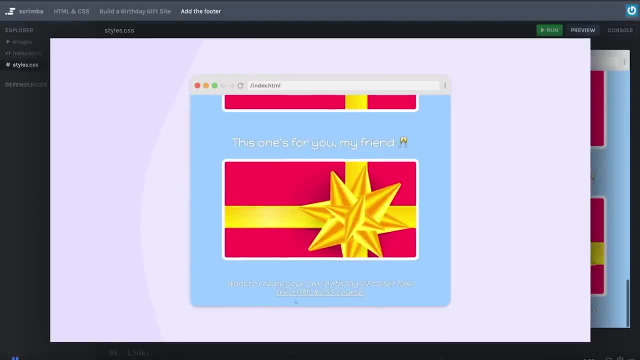 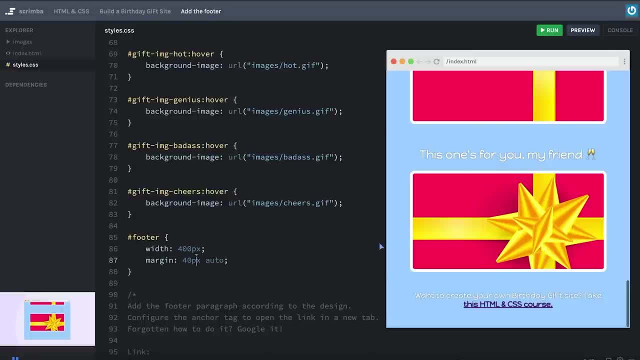 top and bottom because, as you can see right here, it has some spacing above and a little bit more spacing beneath it. So let's try 40 pixels on top- Yeah, that's pretty good. And now 40 pixels at the bottom. That's a bit too much in my opinion. here it looks. 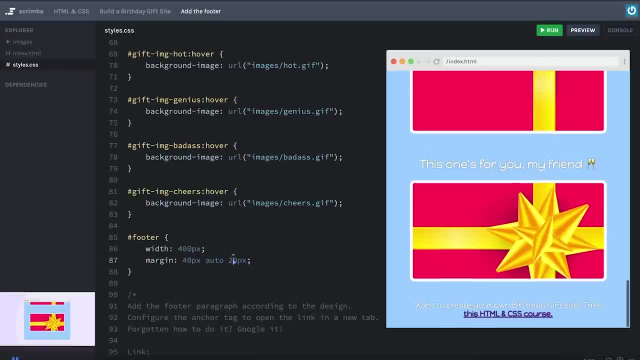 more like 20 or something, So let's, rather than do 20 pixels like that. Now we have 40 at top, auto at left, right and 20 at bottom, And that looks pretty good to me. However, one obvious thing we need to fix is that we need to fix the height of the image, So let's. 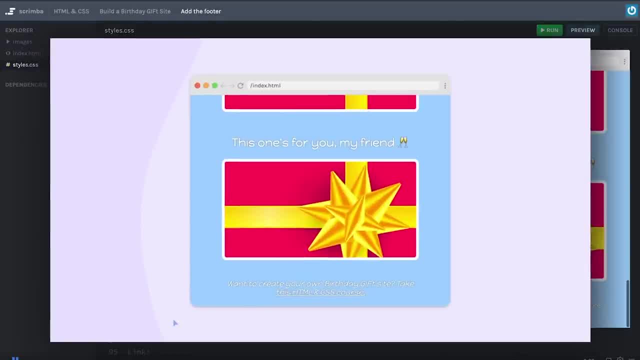 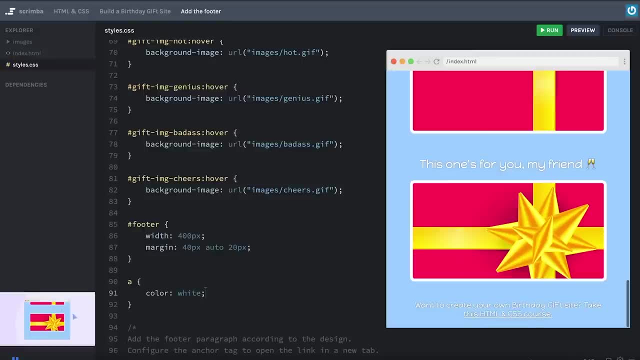 focus on the height here. What we didn't fix is that this anchor tag should also be white, So I'm going to target the element itself. Do color white like that. Now I think the final step we have is to make it italic, And that's done up here where we can do font. 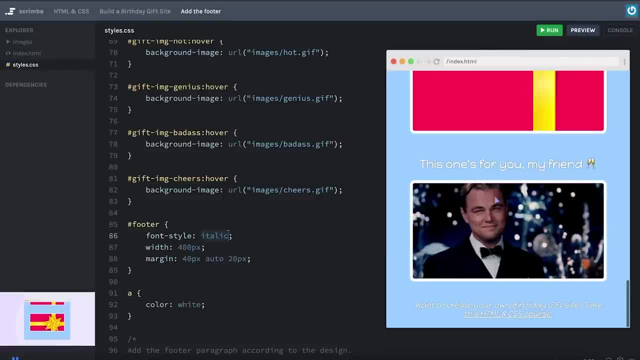 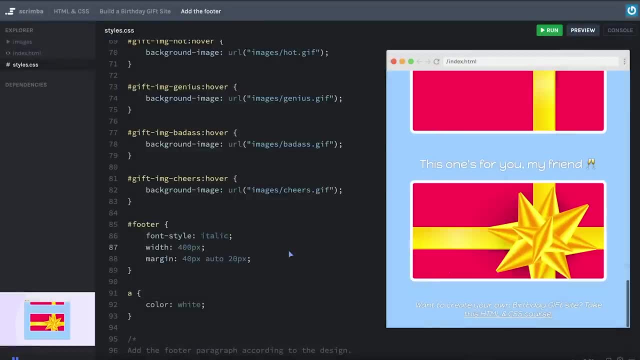 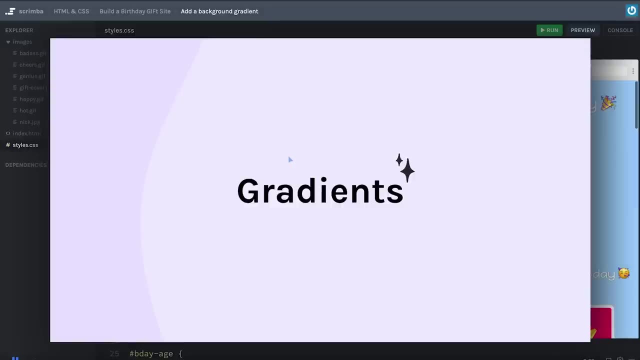 style Palak. and there we go. that looks identical in my eyes, So really good job. I'll see you in the next scrim. Okay, now we're going to talk about gradients, And that's something you've probably seen many times in nature, though not really thought much about. because, for example, because the 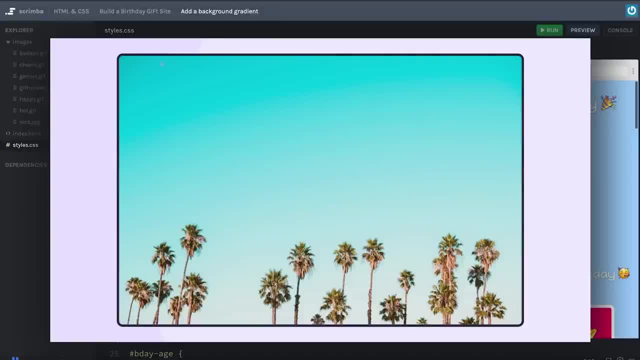 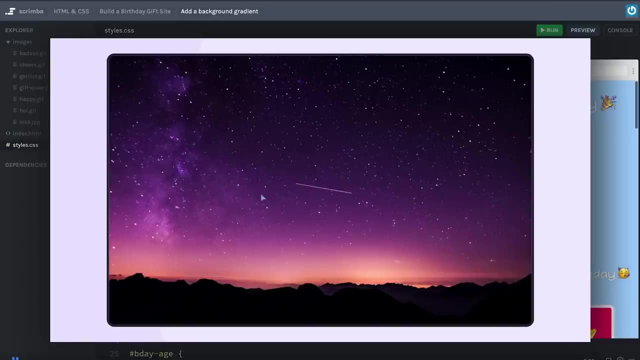 sky is full of gradients. here you can see a sky that kind of fades from a light blue color into a white ish color, And this fade is basically a gradient. Here's another example where it starts almost black at the top and then slowly fades over into purple and then. 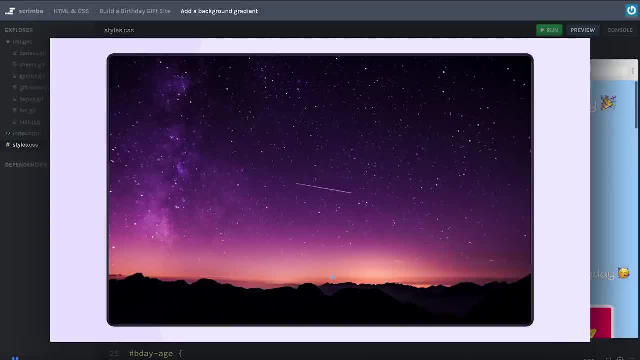 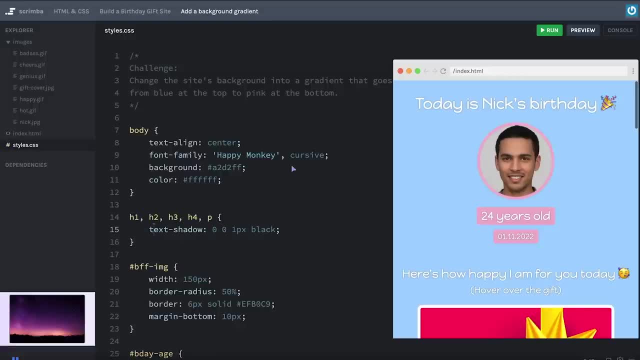 again into a orange, ish or light brown or I don't know what you want to call this color, But you get the point. It's fading from one color to another, And this is very often used in web design. You can, and you can- do it with CSS pretty easily. Let's for. 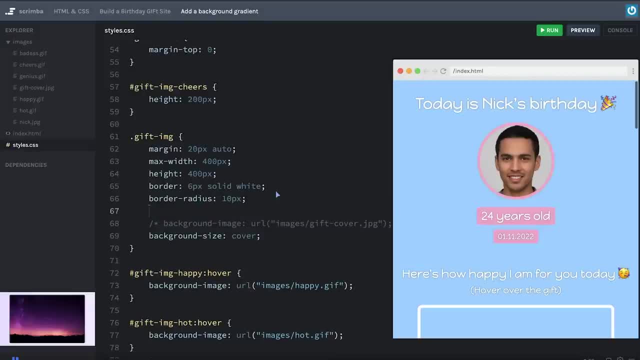 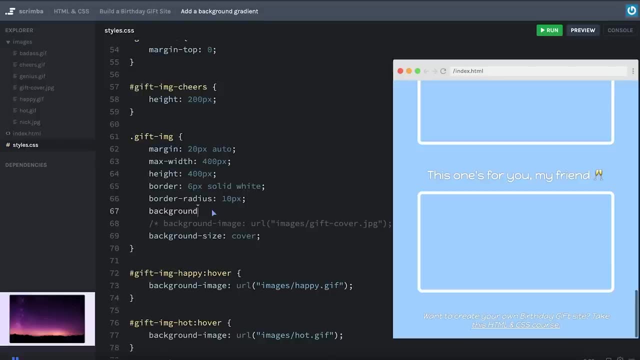 example, remove this background image of the gift card from our gifts. Now you can see, it's just transparent- And then instead we'll write background and linear dash gradient And then two parentheses. So this looks a little bit like the URL keyword we write when. 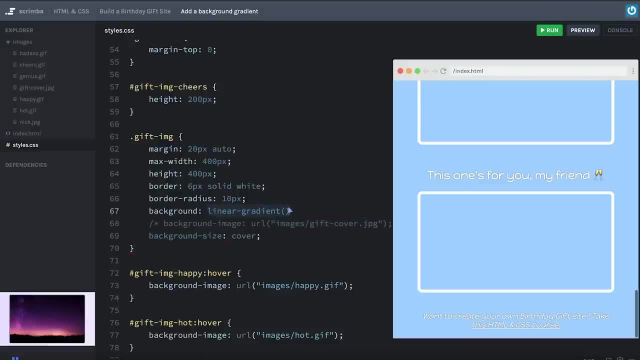 you want to refer to images, meaning that this is also a so called CSS function. Now, inside of the parentheses, we simply write the two colors we want to fade from and to. So let's do from red to blue and boom. there you go. Now you can see that all of our gifts 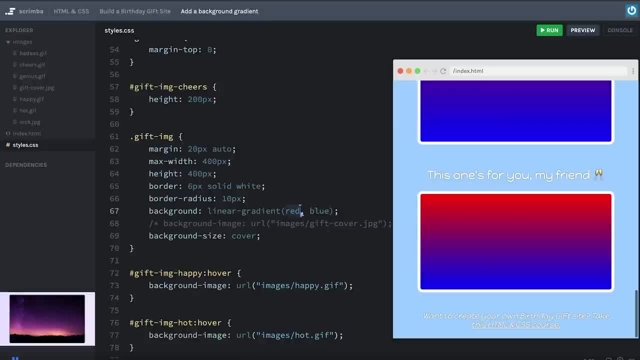 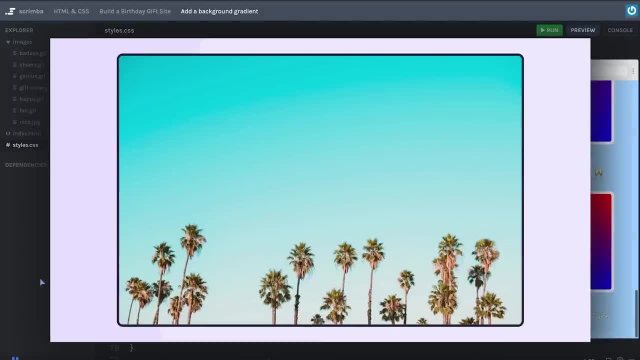 fade from red down to blue And by default it starts with the first color at the top and then the second color at the bottom. So let's try to mimic this image here in CSS. I happen to know that there's a CSS color. 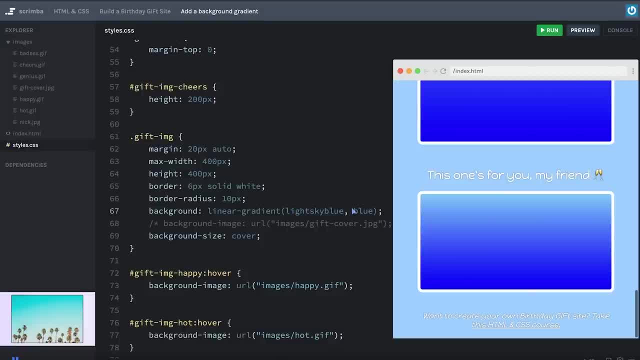 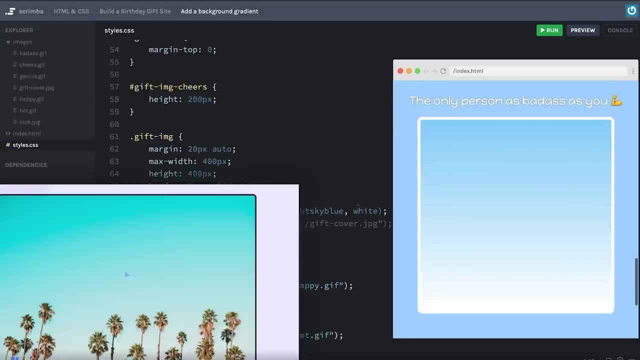 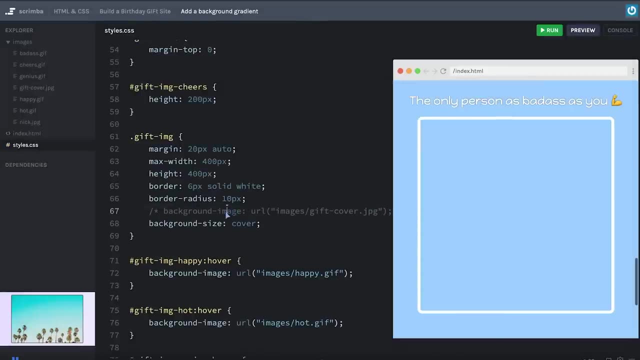 called light sky blue. So if we start with that one and go down to white and have a look at this gradient here- Actually, to me it's kind of similar to this one we have here- Not quite, but you get the point. Okay, now I'm going to remove this. give us our gift. 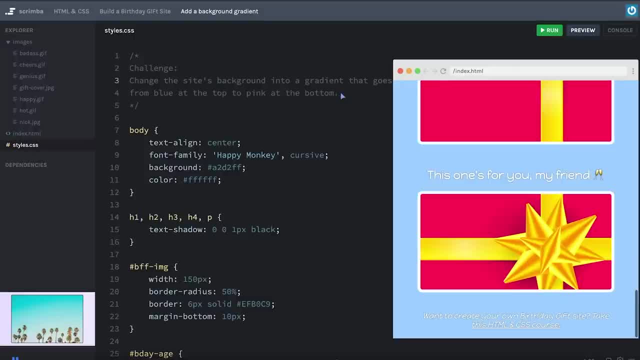 cover back and then give you a challenge, Because now I want you to change our sites background into a gradient that goes from blue at the top to pink at the bottom, And let me show it to you, And let me here show you how it will look. I'm going to do some. 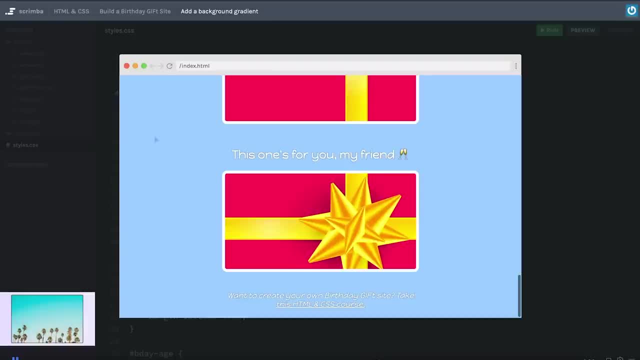 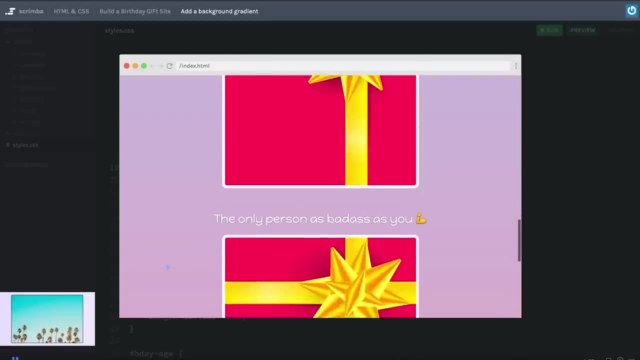 magic. now I'm going to knit my fingers and then the gradient, and then the gradient will be applied automatically. Oh, pretty nice. Now you can see the bottom here is pink, And if we scroll up it slowly fades over into blue, And at the top it's totally blue. So 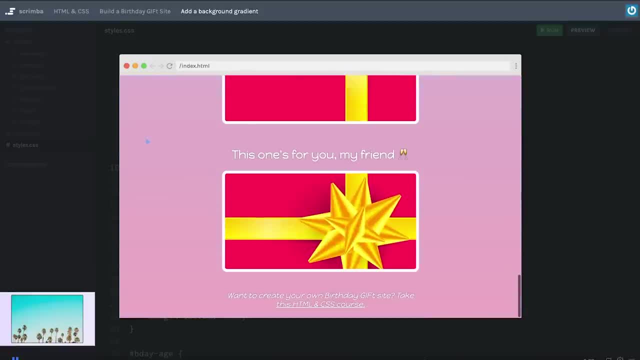 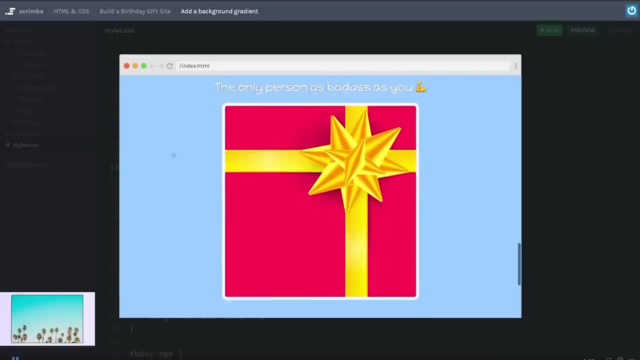 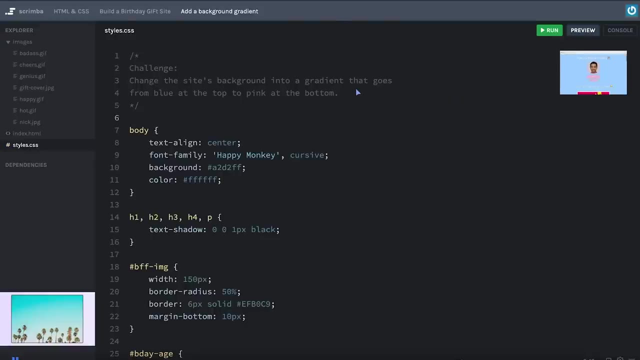 this makes the site slightly more fancy, Which I think is cool and matches the birthday team. So now I'm going to knit again and the gradient will be gone. Like that: Now our site is blue all the way from the bottom to the top And it's your job now to get the gradient back. So go ahead and do that, right. 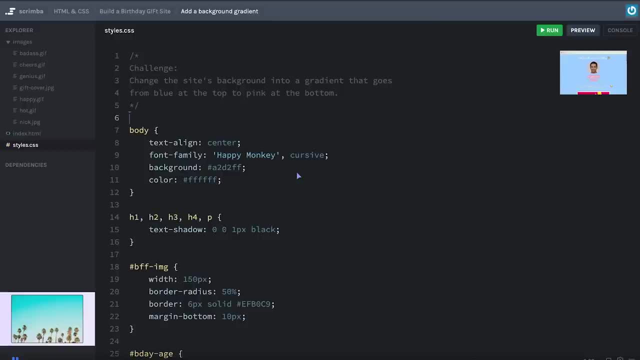 now. Okay, let's do it. So the property we need to fix is the background on the body, Because we need here a linear gradient Going from the blue color it used to have to the pink color which we've been using as the border of our image of Nick. So then I'll simply paste that one in right here. 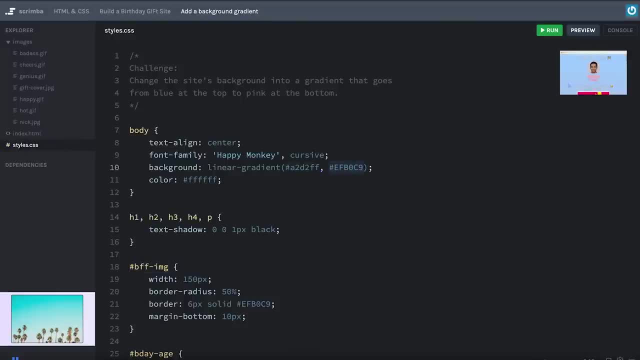 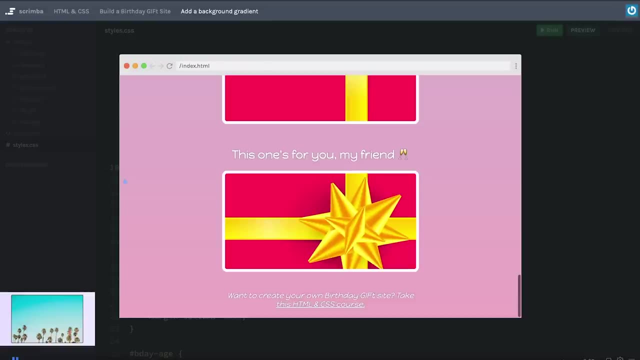 Now we should be fading from blue to pink. Let's see. we can see the blue And, yes, it looks like it is slowly fading towards pink. Really good job. Now you've learned a super cool CSS technique. I'll see you in the next scrim. 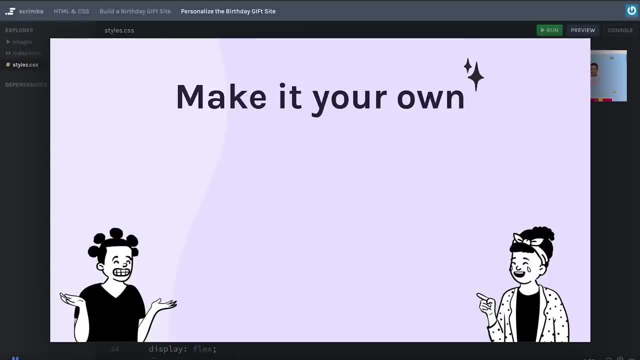 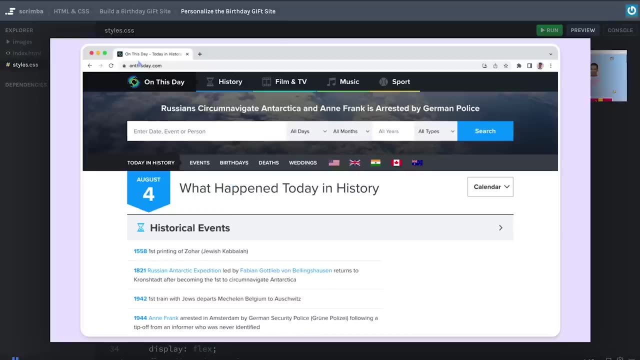 Okay, now that you've completed the birthday gift site, I want you to make it your own. So first try to think of someone whose birthday is upcoming. It could be a friend, a family member, a pet or basically whomever. If you need some ideas you can head over to on this. 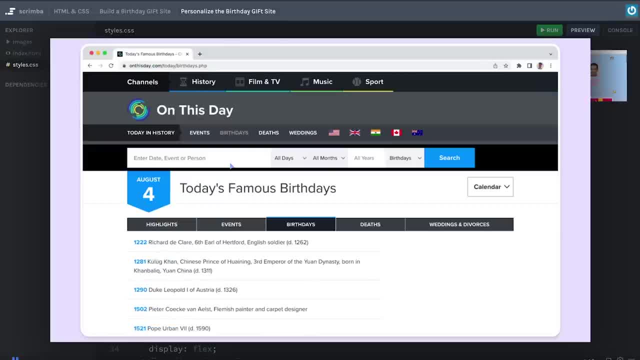 daycom and click on birthdays. That'll show you a bunch of celebrities was born on this exact date. As you can see here, the birth dates are chronological, So he probably have to scroll a bit down Until you find someone you've heard about. rolling it down will show us that Louis Vuitton. 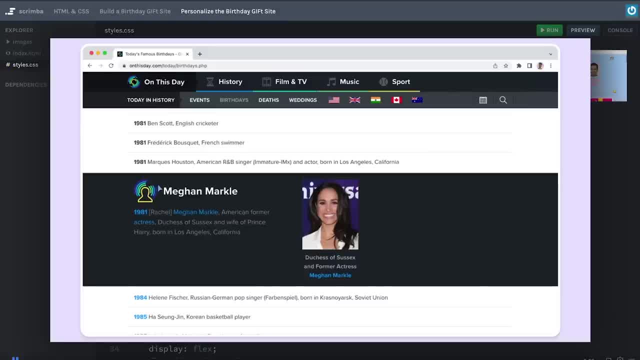 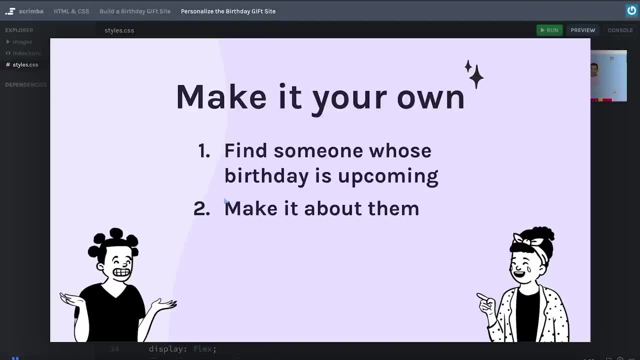 was born on this day in 1821.. Or scrolling even further, we can see that also Meghan Markle was born on this day. So if you find a celebrity you like here, this is a perfect opportunity to make this site about them. And what I mean about that is that I think 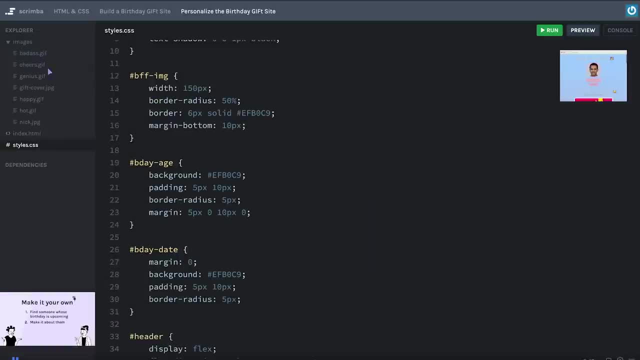 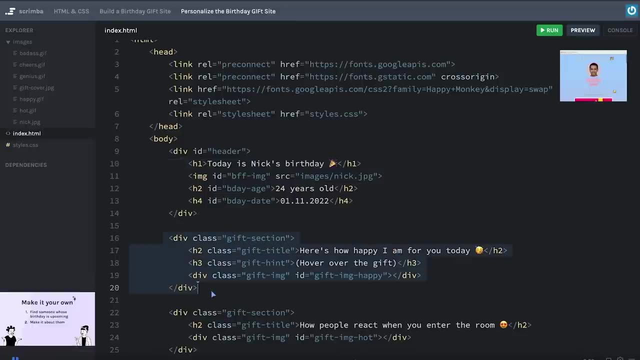 you should change the gifts to something suitable for that person And also, of course, change the copy as well accordingly. And if you want to go even more above and beyond, create entire new sections Or even stop, You can style it differently depending on how you want it to look. That is great practice. 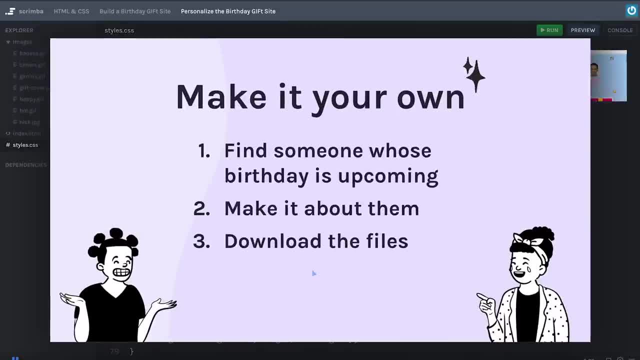 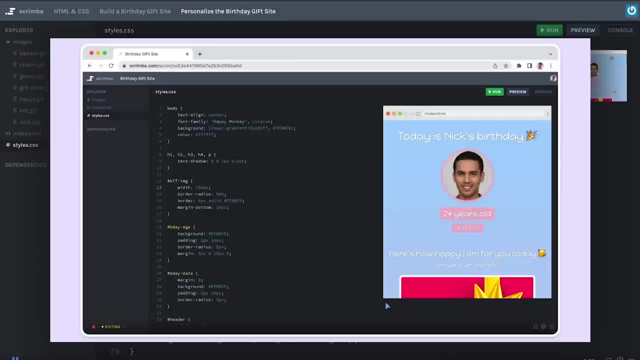 for your design and product skills in general. Finally, once you've done that, I want you to download the code files so that you have them locally on your computer. If you've forgotten how to do that, it's pretty simple: Just click on the gear icon in the bottom right corner. 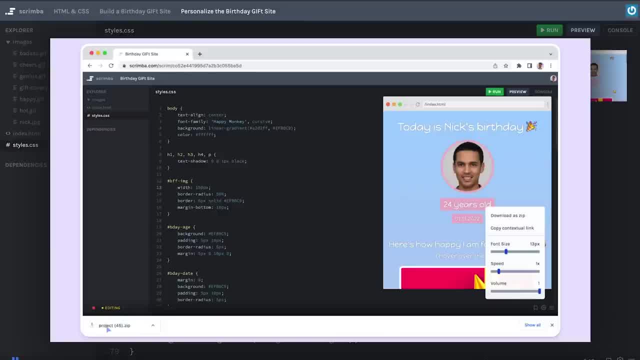 here and click download as a zip. As you can see, it now downloads this zip, which in my case is called project parentheses 45. So once you've found someone to create this birthday site about, made the appropriate changes and downloaded the code, you are ready to move on to the 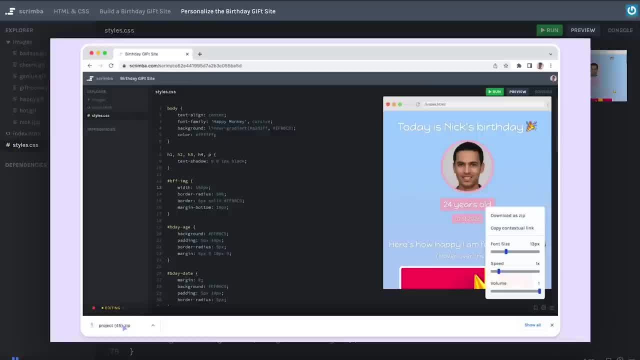 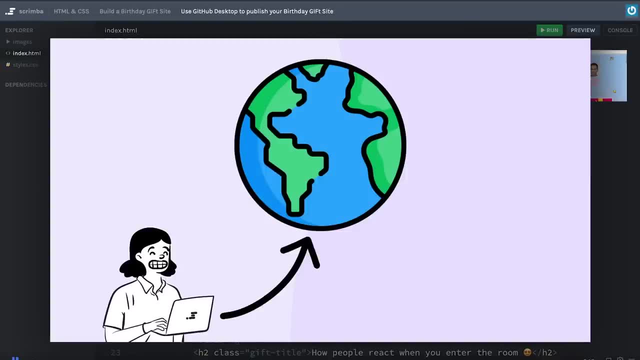 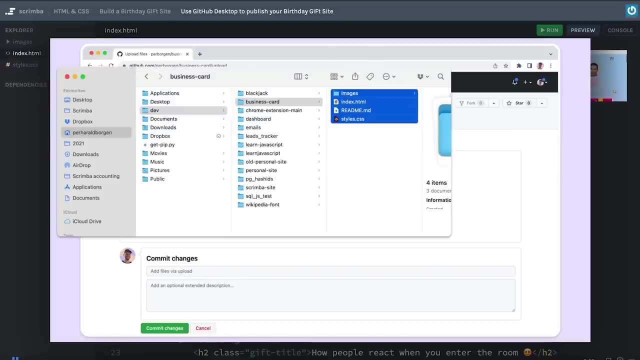 next couple of scrims, where we are going to deploy it to the web, On its way from your local computer up to the internet. your code is going to take a slightly different path this time around, Because, while it worked perfectly fine to just drag and drop your files onto githubcom, that's actually a pretty clunky way of doing. 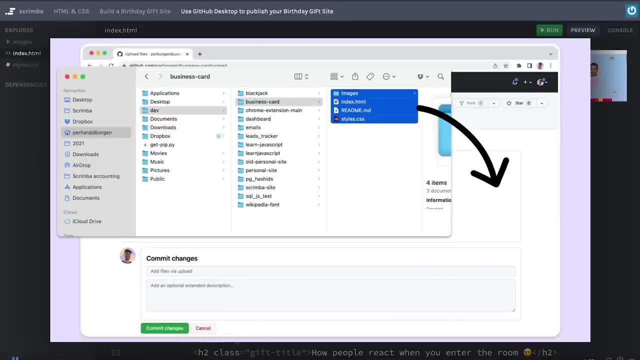 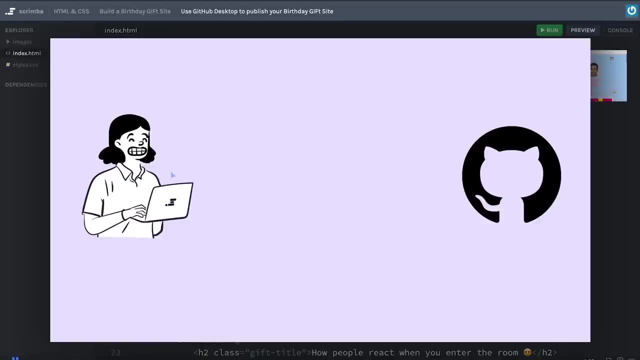 it. So instead, we're going to use a dedicated tool For interacting with GitHub, and that tool is called GitHub desktop, because that's the way the pros do it. When they interact with GitHub, they always have a tool in between them and the service which helps them push code up to GitHub and also pull code down. 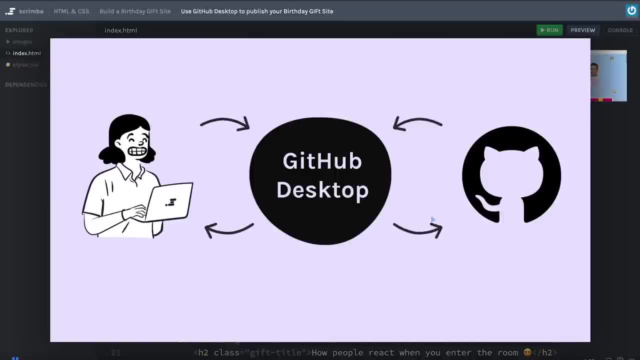 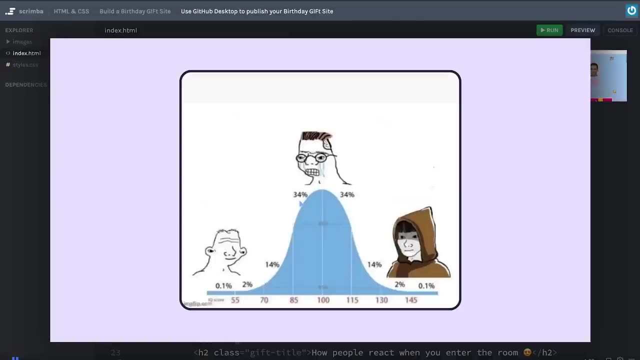 from GitHub, And just to make things a little bit more complex for you here, what's actually going on under the hood is that both GitHub desktop and GitHubcom rely on a piece of software that's called Git. What is Git? Well, some devs who think they are really smart will probably tell you that. 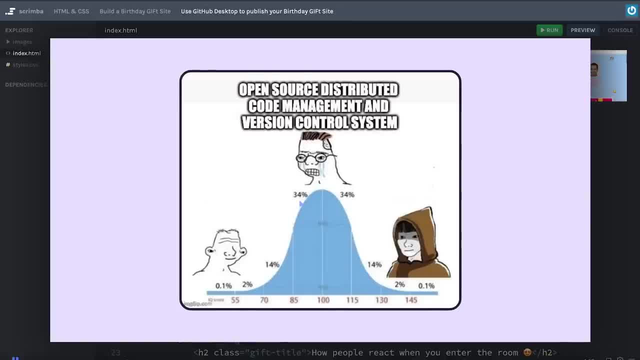 Git is open source distributed code management and version control system, But you should, regardless of how smart you are, just think of Git as a way to keep track of file changes. So that's it. Git helps you keep track of how your project files change over time, And 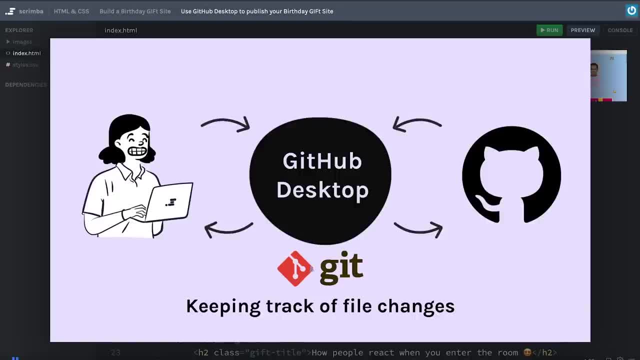 actually, you don't need to know anything more than that in order to get started using Git via GitHub desktop, Because this desktop app abstracts a way for you to get started with GitHub desktop, And that's what we're going to talk about today. So let's get started. 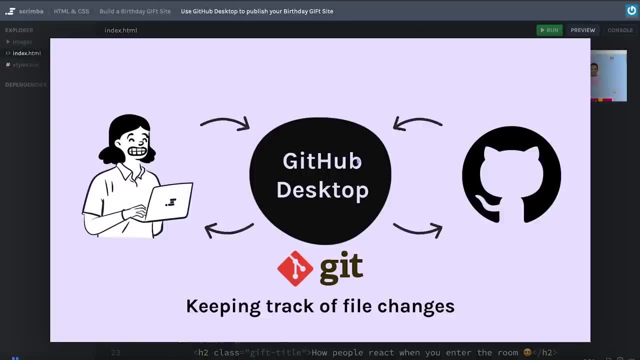 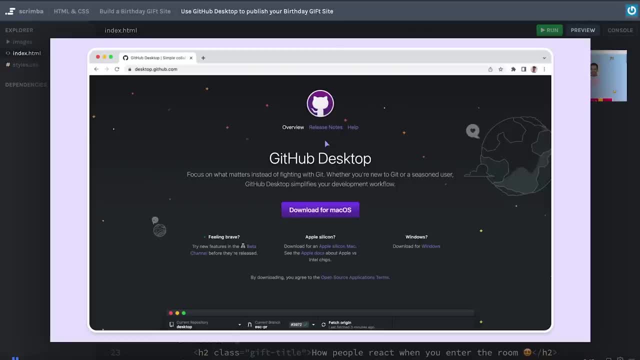 So let's just get started and download GitHub desktop right away. If you are following this course via scrim bar, you can just click on this slide right here, But if you're watching it via YouTube, just head over to desktopgithubcom. Once you're there, click on the download button. 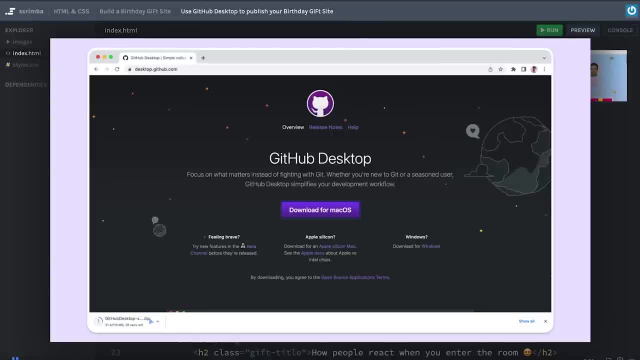 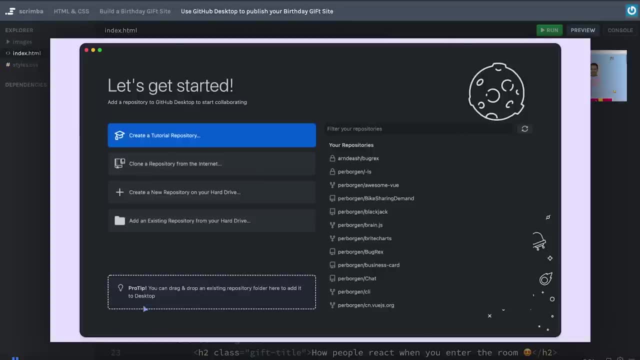 so that your browser starts downloading the zip file for this app, And once that's done, open up the app, install it on your computer, And once you've authenticated with GitHub in the app, you should see a screen that looks more or less like this: The first step you're going to take here is to click on this button. 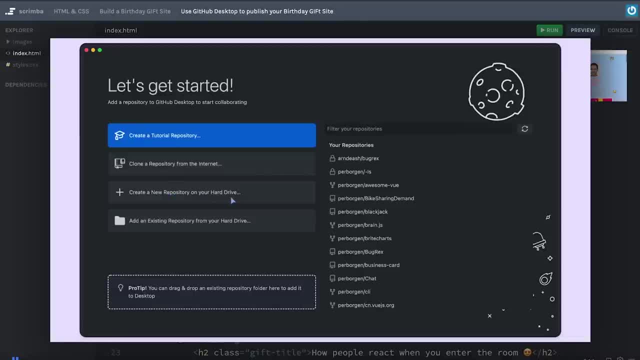 that says, create a new repository on your hard drive. Because that's what we want to do. we want to create a repository, aka a folder on your computer that holds all of our project files. What you'll then see is this little modal where you have to give your repository. 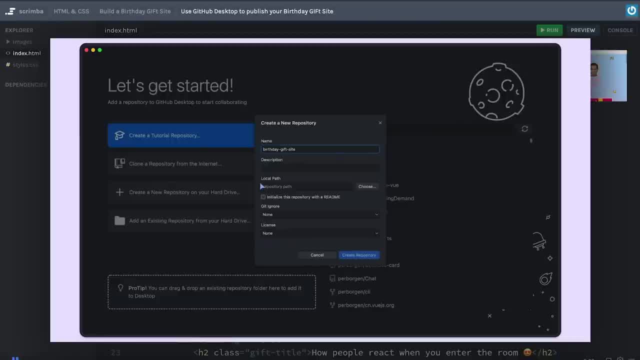 a name, So I'm going to call it the birthday gift site. and then you are to head down to the local path field And click on make a gift, And then you have to click on create, and then you have to click on create a gift, And then you have to click on create a gift. 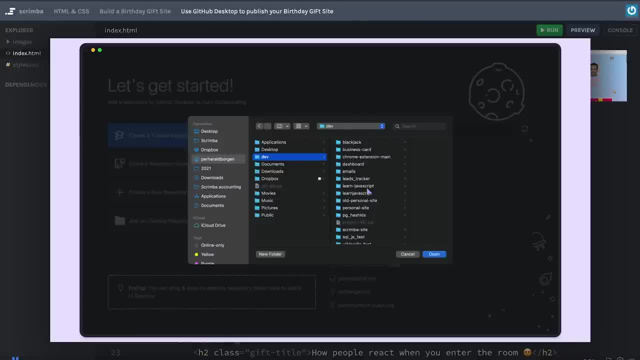 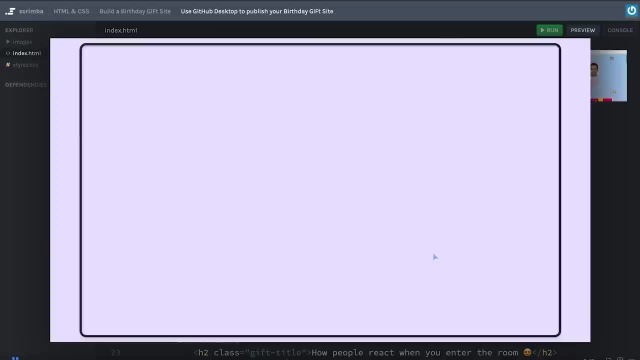 click on choose, Because what you now need to tell get and get top desktop is where on your computer you want your project to live. I'm going to navigate to my dev folder and just click open and then create repository. that'll change GitHub desktop into this dashboard. 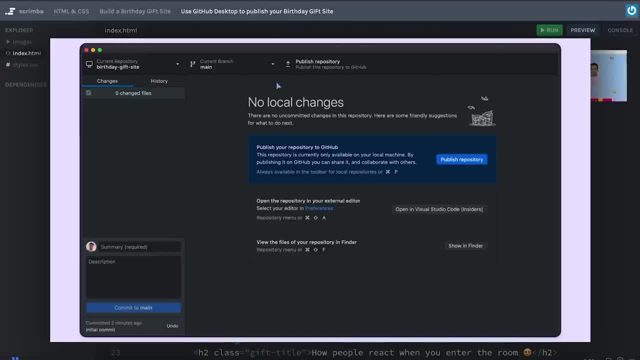 that you will interact with the Earth, a gift site repository, using the various buttons. Now you can see that it says no change files because our repository is empty. In order to verify that, let's click on the show in finder button. When we do that, you can see. 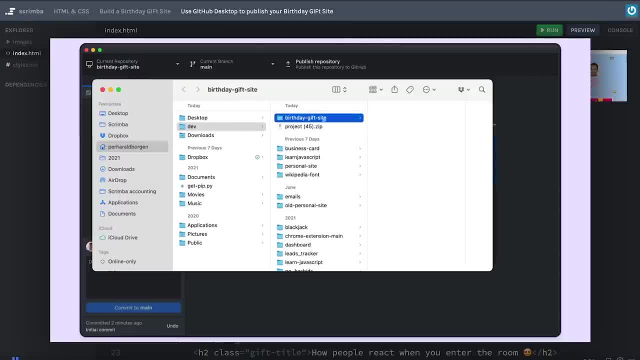 that GitHub desktop has created an empty folder on our local computer And I have it here right above the project zip I downloaded in the previous scrim. So I'm going to click on the zip file, then double click on it so that I'm unzipping the files. select all of. 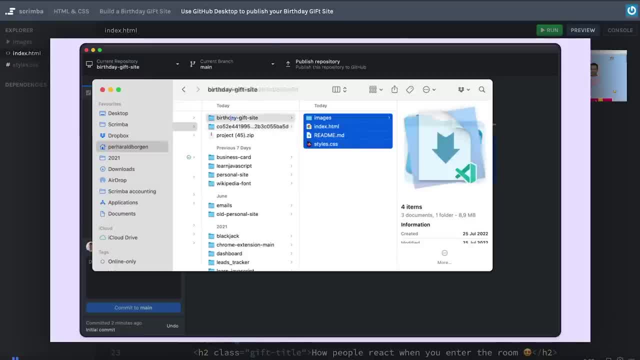 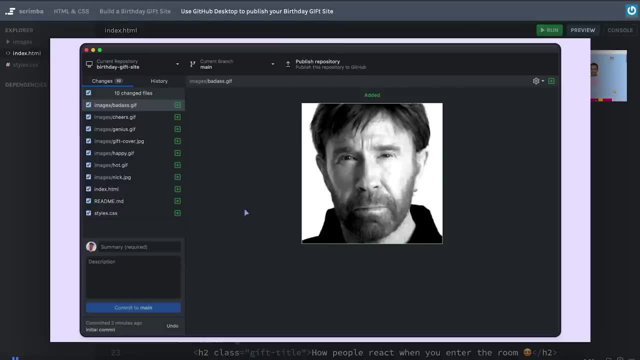 the files and then drag and drop them over into our repository like that. When you then return back to GitHub desktop, you will see Chuck Norris staring you straight in the face, because, as you can see on the left hand side here, all of the images and project files have been 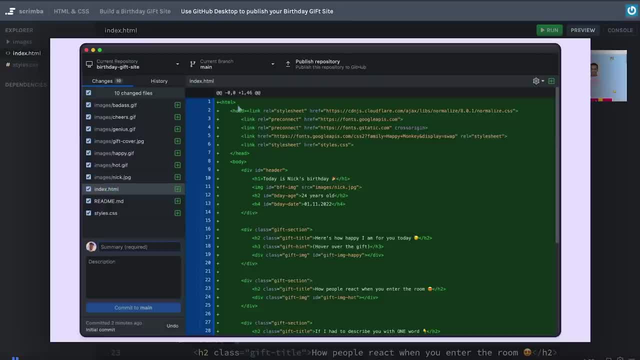 registered. So click down on the index dot html file. there you can see they're all in green, which means that these are new lines of code ready to be added to the git repository. In order to add all of this content to our repository, you have to head down and write. 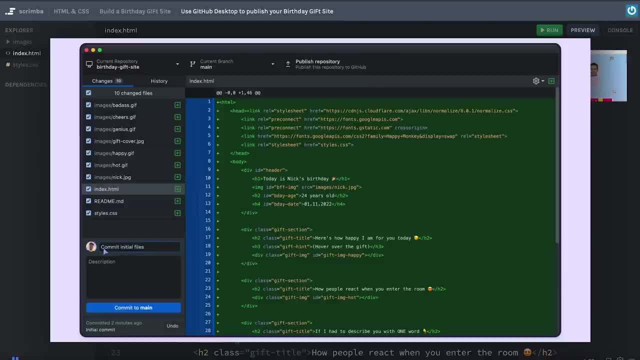 a commit message in the bottom left field right here I'm going to just say commit initial files And then to perform the commit. we'll hit this commit to main button. don't worry about what main means At this point, and also if you're a little bit confused about what a commit actually. 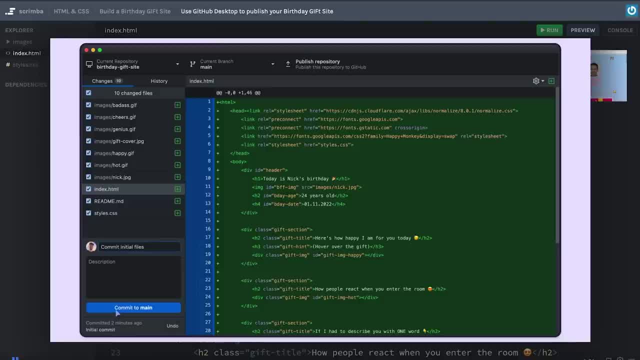 is. don't worry too much about that. What we're just doing here is telling git that we want to add a bunch of files to the repository, And we're also adding a little description so that in the future it'll be easier for other developers to understand what you were. 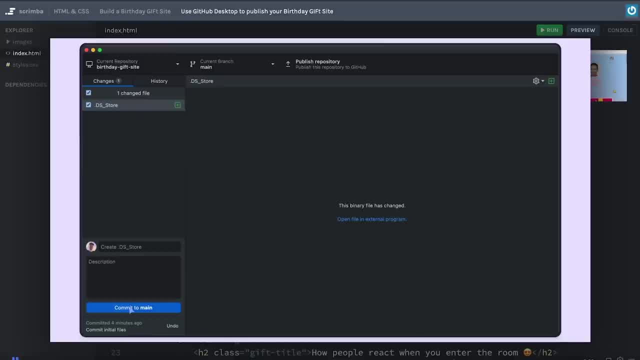 thinking when you added these files, So let's hit commit to main. that removed all of the files, which was intentional. but actually here my computer did something annoying. Max have a tendency to add a so called DS Store. I'm going to call it commit, which is going to add a file to the repository, And so let's. 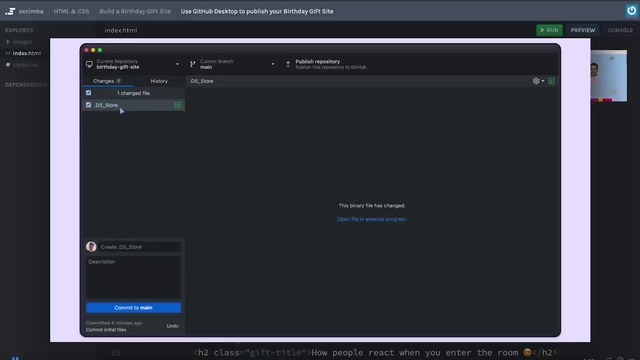 s store file, which is something Mac uses to handle metadata for a folder. we don't need that in our project, So I'm actually just going to right click on it and delete this file entirely by clicking on discard changes. Now, once I've done that, the dashboard is. 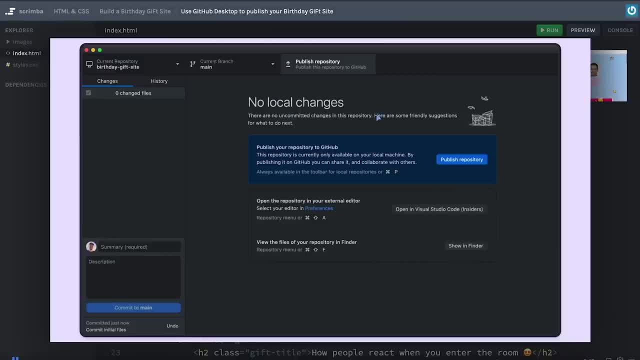 back to how it was before we committed the files. that has this publish repository option both here and up at the top. This means sending off our code to GitHub. That's obviously what we want to do. So I'm going to click on publish repository and also give it a name. I'm going 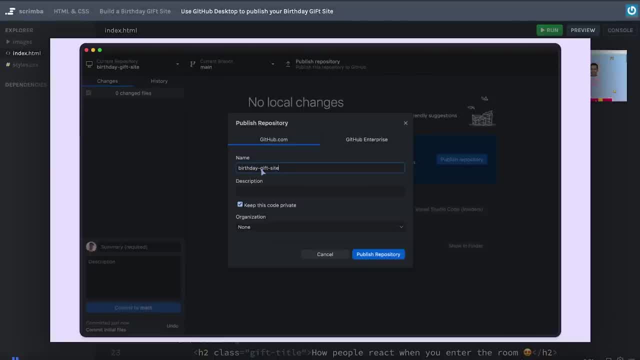 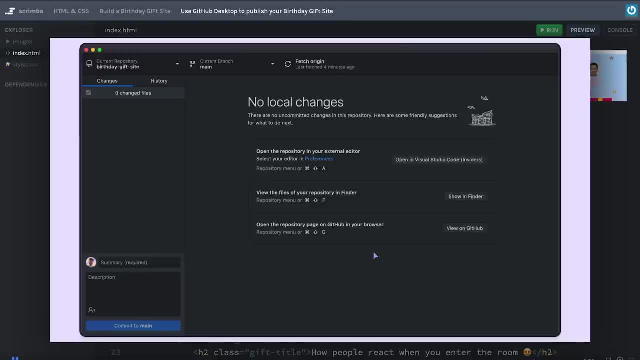 to give it the same name on GitHub as we have locally calling it birthday dash, gift dash site. And also I'm going to uncheck this. keep code private, because we want our project to be open source, And then I'll hit publish repository. Now the final step is to click. 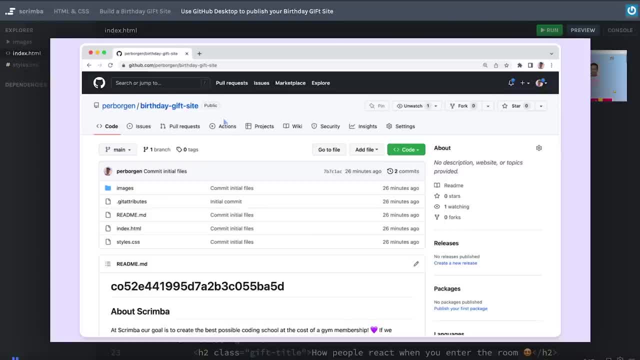 on this button right here: view on GitHub. and boom, here we go. We have created a repository locally on our computer and published it on GitHub via GitHub desktop, just as the pros do it. So really good job. we are ready for the next. 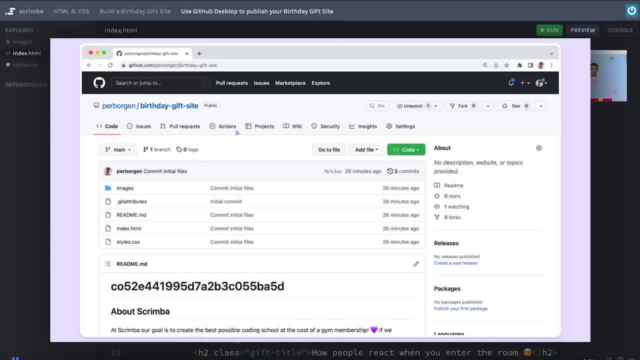 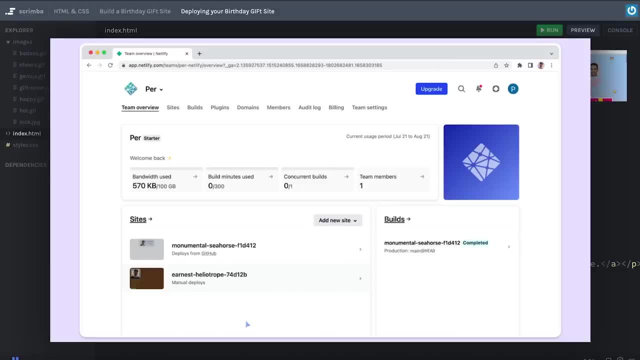 step, which is to deploy this site to the web, which we'll do in the next screen. Now that you've pushed your birthday gift site to GitHub, it's time for us to hook it up with Netlify so that you can deploy it as well. So head over to your Netlify dashboard. 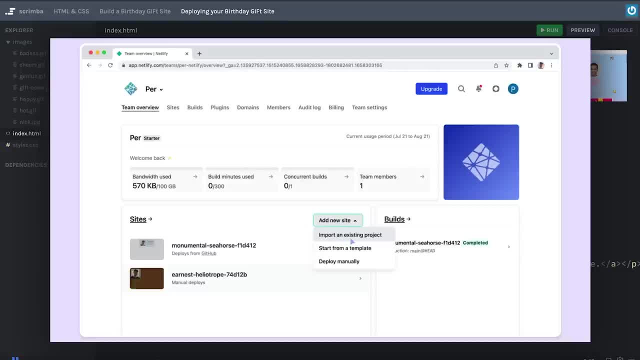 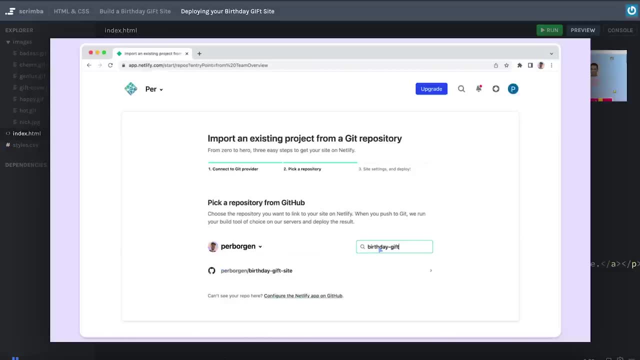 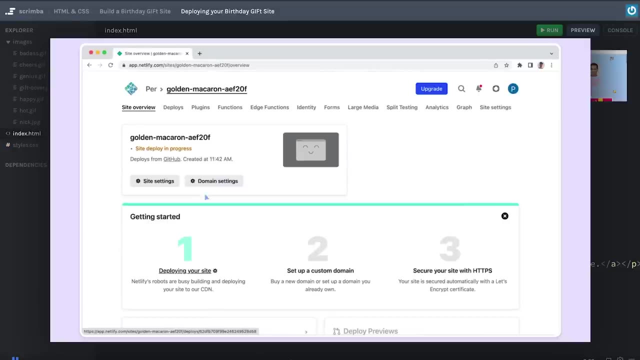 there, click on the Add new site button and choose import an existing project. There, just click on GitHub, which then brings up this search menu where you can search for the birthday gift site. click on it and then leave all the site settings as they are. just scroll to the bottom and click Deploy site. then you'll. 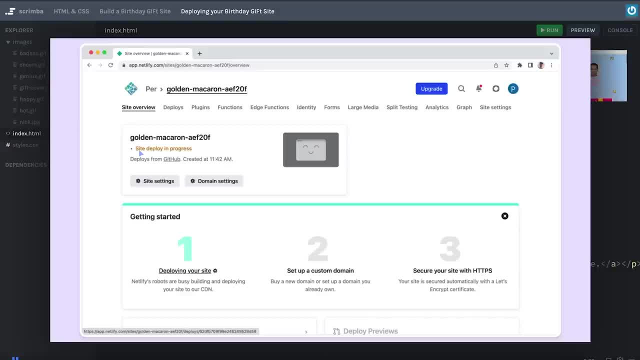 see this familiar dashboard again And, as always, the only thing you need to do here is wait until this image here turns into a screenshot of your site, which is now thus meaning that your site is available on this URL Now. hopefully, your birthday site is not. 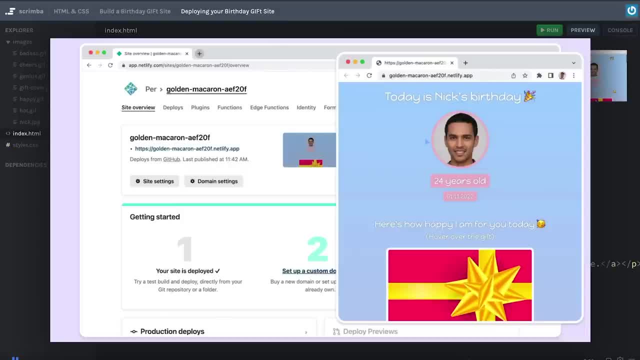 about Nick at this point. it's about someone else, And I definitely think you should send it off to that person, Or, if it's about a celebrity or whomever, at least share it with the world And once you've done that, give yourself a pat on the back and then I will see you in. 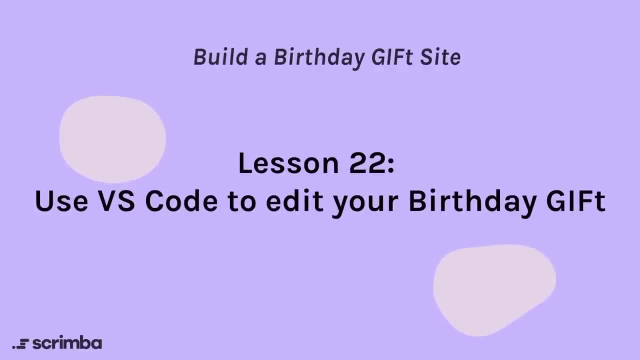 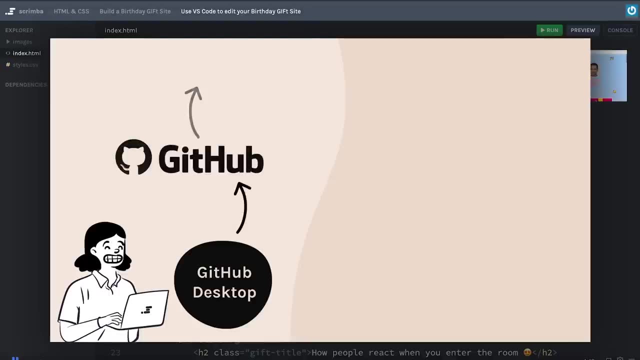 the next scrim. At this point, you know how to use GitHub desktop locally on your computer, how to push code up to GitHub and then have Netlify deployed to the World Wide Web. That is really good. However, you're still lacking one important tool, because what happens if? 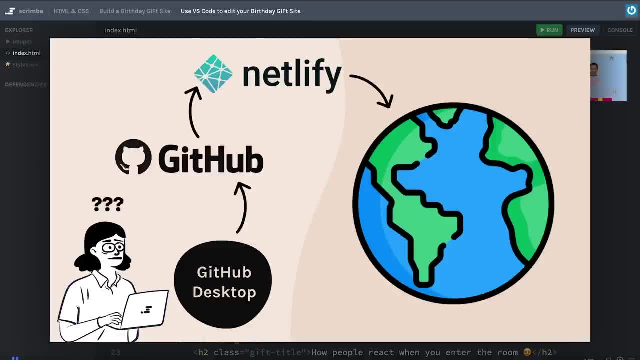 you want to change your code and then push it up to GitHub and deploy it again. Well, in that case you'll have to use a code editor, Luckily on your computer. so that's exactly what you're going to learn in this scrim we. 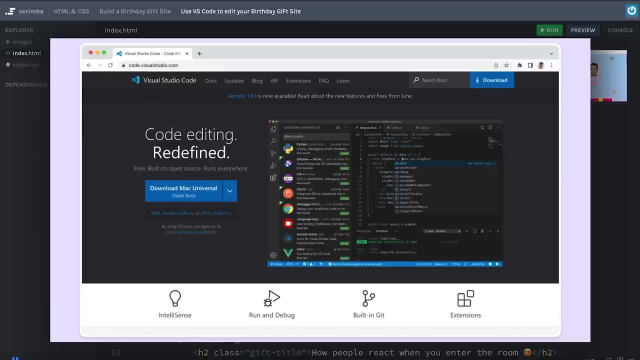 are going to use a code editor that you actually have been using quite a lot at this point, though you might not be aware of it. It is called Visual Studio code, And it's actually what powers scrim bar under the hood, though, as you can see from this screenshot here. 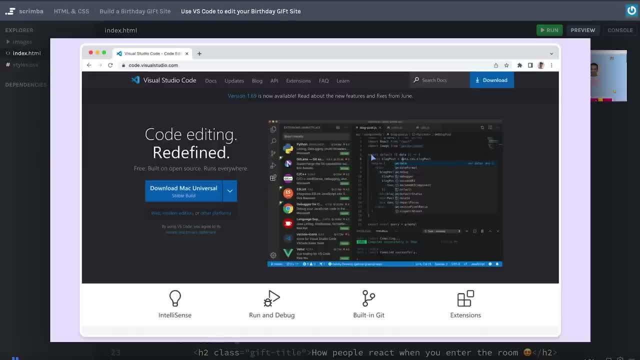 it looks a little bit different from the scrim bar in Browser Editor, So we've done some modifications to it and stripped it down a little bit. Okay, so, in order to get Visual Studio code running locally on your computer, if you have to head over, 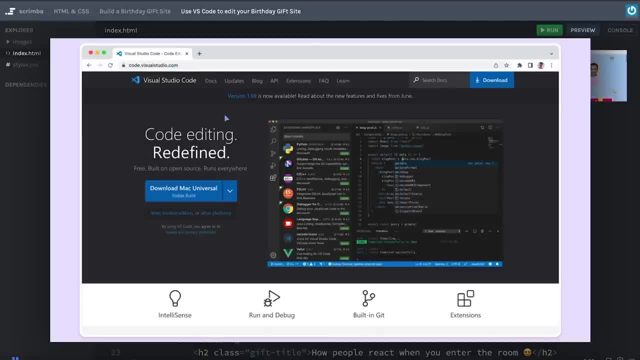 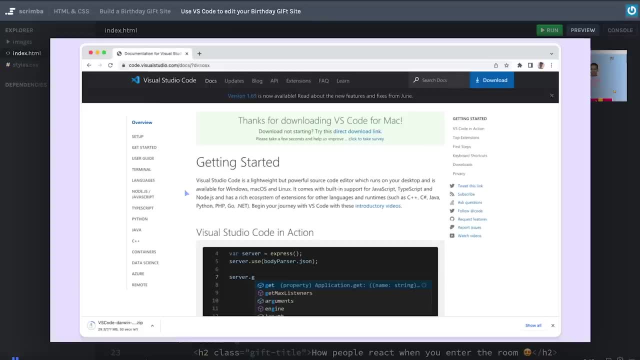 code: dot visual studiocom. Or if you're watching this scrim on scrim bar, just click on this slide and you'll get to the landing page. Once you're there, click on the download button. that'll start a download process of the app And you'll also get to this getting started. 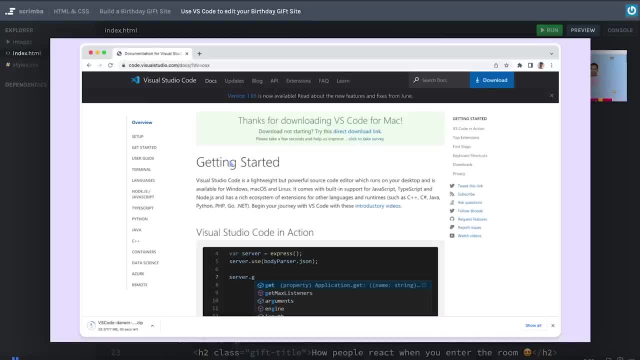 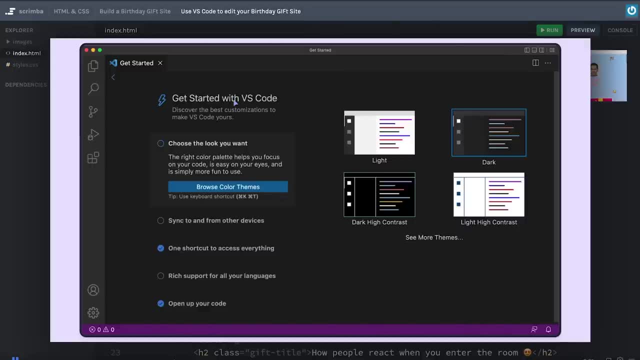 page. However, I'm going to talk you through it, So you don't need to read through this guide. Once it's downloaded, just unpack the zip and install it on your computer, And then you'll get to a screen which looks like this: Here you can see a bunch of onboarding steps. 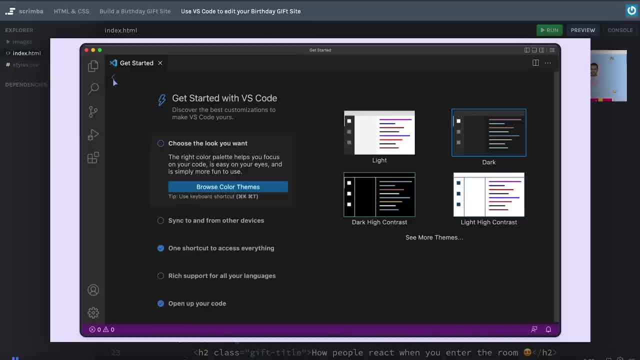 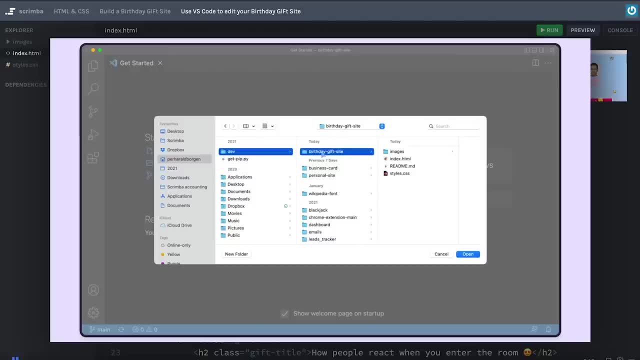 but we're not going to worry about them right now. Just click on the back arrow in the top left corner And there I want you to click at the open option, because that'll open up the finder menu which you are to locate to the folder for the birthday gift site. click. 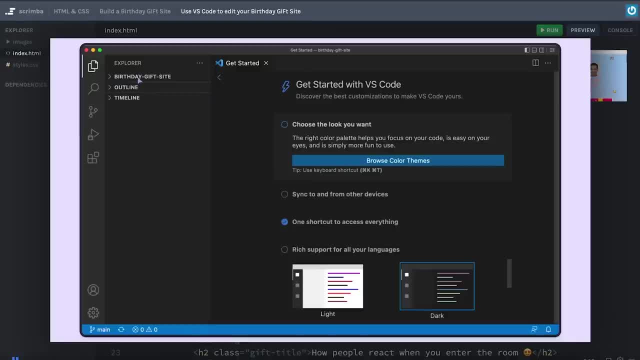 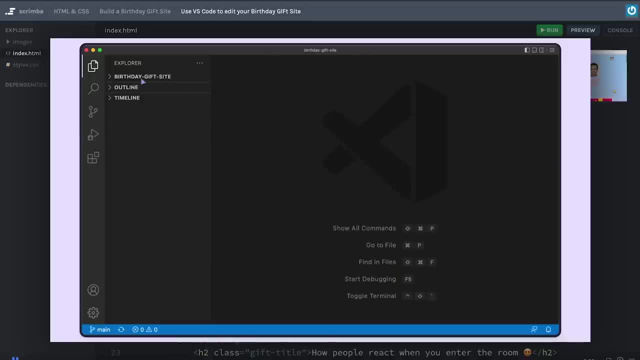 on Open And there you can see the birthday gift site listed under the Explorer tab on the left hand side. I'm going to remove this get started file here, So I'm going to click on this x icon like that And then I'm going to click on the birthday gift sites to open. 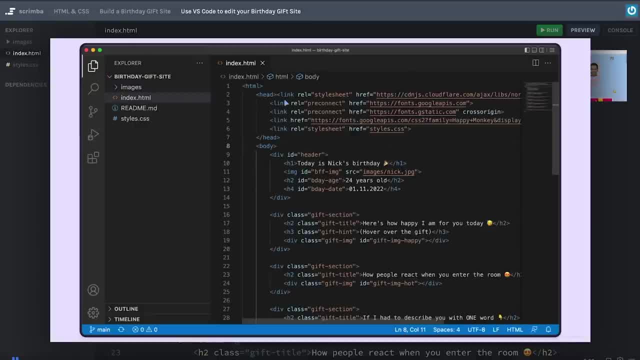 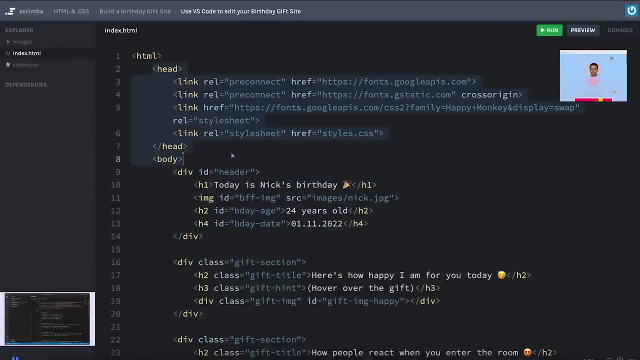 up the folder. Moving on to the index dot HTML file, When we open it you can see that it looks quite a lot like how it looks on scrimball. the editor- right here, though we had scrimball- have created our own color theme, So we're 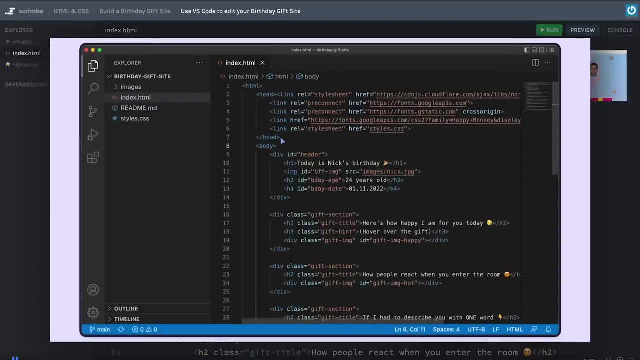 not using the default one you can see right here, But other than that it's quite similar. Now let's make a change to this code, push it up to GitHub and get it deployed. The change I want to do is just very simple. I'm going to change this name from Nick's birthday into 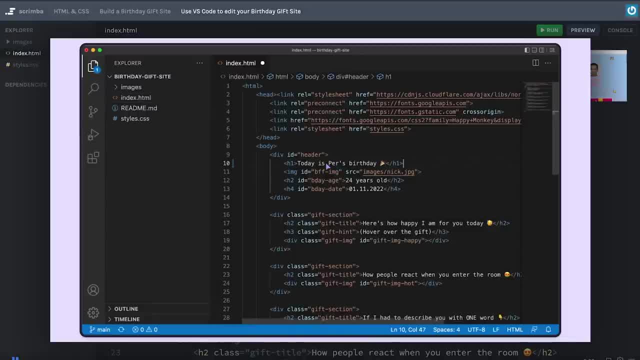 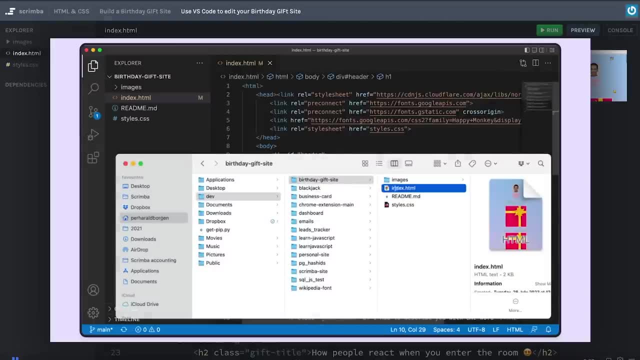 Pierce birthday. If I then save this with command plus s or Ctrl plus s, you can see that the file turns yellow. Hello means that it has changed. And also to verify this, let's open up finder alongside a browser window and just drag and drop this index HTML into the browser, because then we 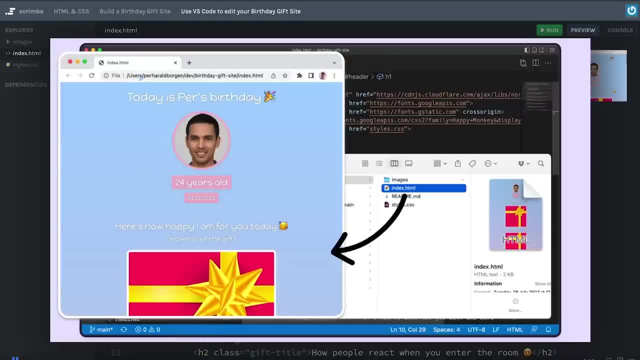 can see that it says today is Pierce birthday. So by pointing our browser to the local index HTML file, we have verified that. yes, the changes have been saved, though this is just available for me. locally it has not been deployed yet, So we got to do that as well. 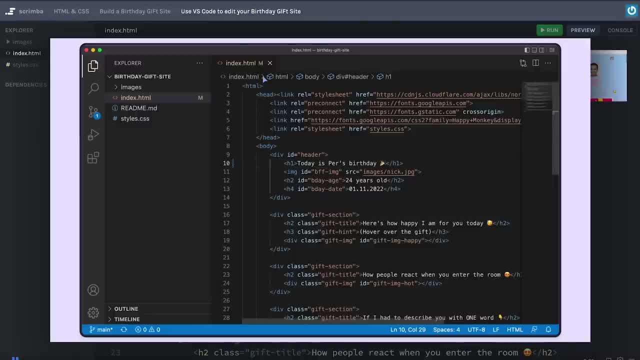 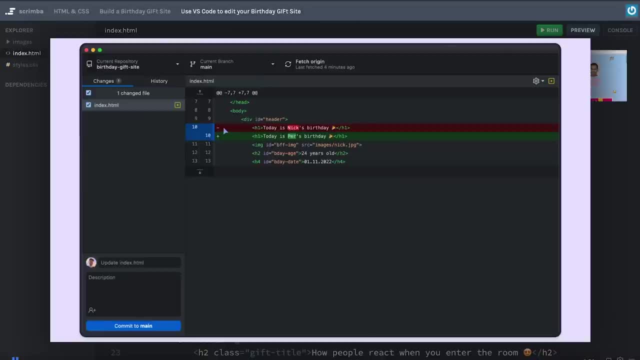 And the way we get these changes up to GitHub and then up to Netlify is, as you probably guessed, via the intermediate step of GitHub desktop. So if we navigate to the desktop app there you can see that it has noticed that we have changed line 10, you can see. 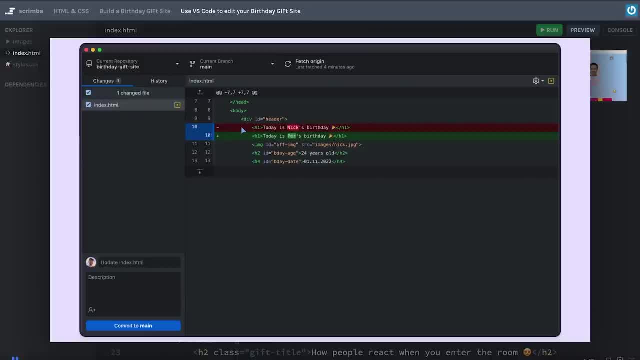 the red line 10 right here, which is the previous version before we saved our code, and the green line, which is the new version after we saved our code. So now we have to tell git that we actually want these changes to be incorporated into our repository. we have saved them locally. 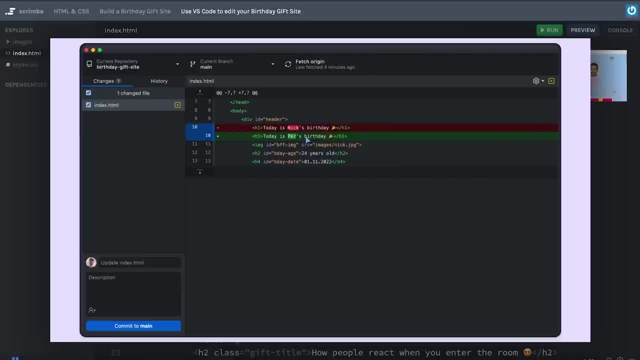 but we haven't saved them or aka committed them to the GitHub repository. So by having this file checked and writing a commit message down here in the bottom left corner, we can commit this change and just save it in Git. I'm going to give it the commit message, change the name to peer and then. 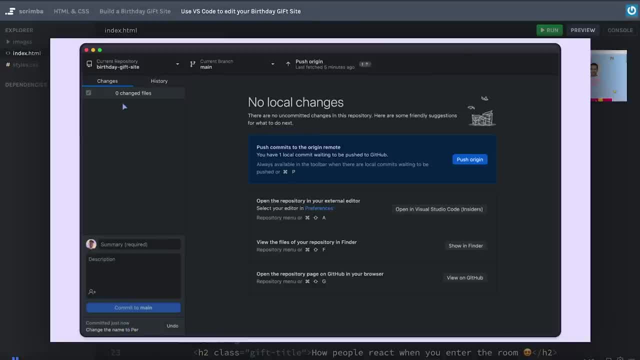 hit the commit button. Now all of our local changes have been committed. As you can see, it says zero changed files. But what we did get is this number one up here and an option called push origin, And that means pushing our changes up to GitHub. So if I click at 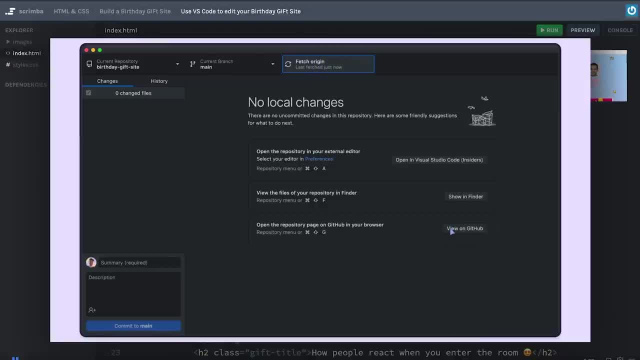 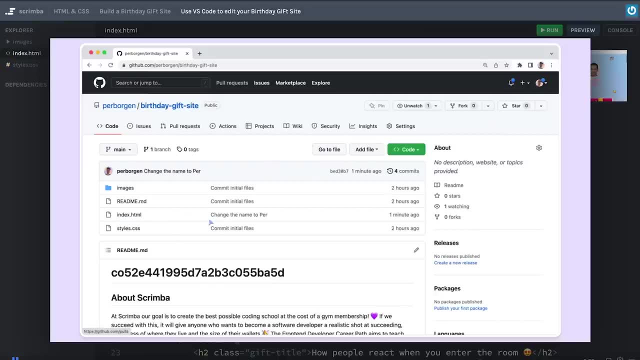 here you can see it starts doing some stuff under the hood And then if I click on View on GitHub it'll open up the GitHub browser And there, on the row here which lists the index dot html file, you can see that our commit message change the name to peer was. 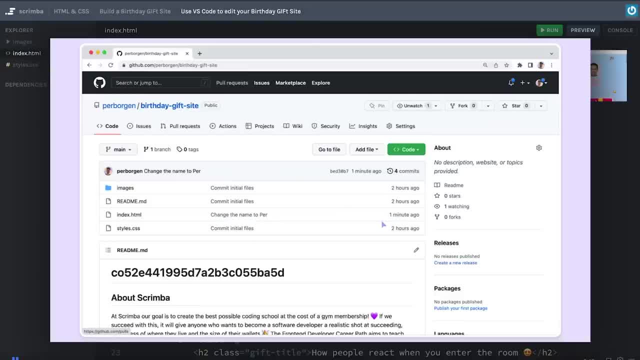 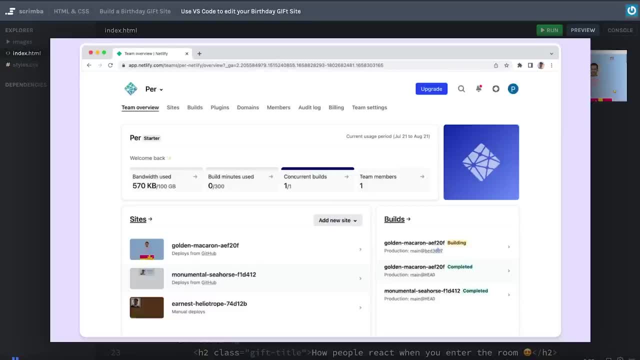 added to this project one minute ago. that is very promising. If we now head over to our Netlify dashboard, you can see that Netlify has already picked this up. here under builds, you can see that one of our projects is now being built, And in this tab as well. you. 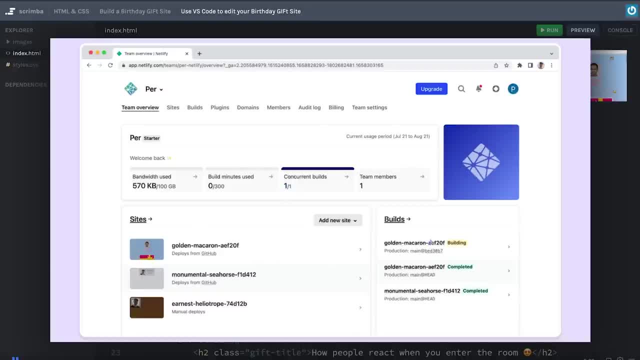 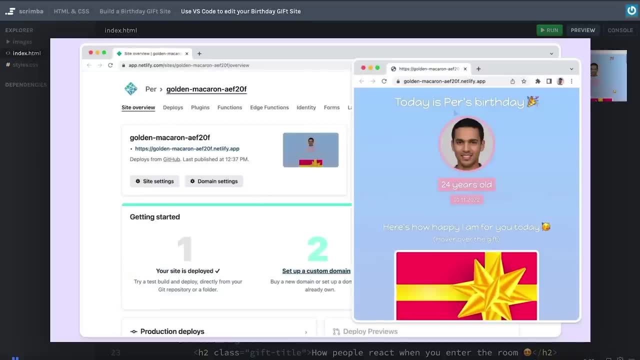 can see we have one concurrent build going on And then after a little while you can see, boom, it's completed. I'll click into the project and open up the URL. And there you go. It says today is Pierce birthday. 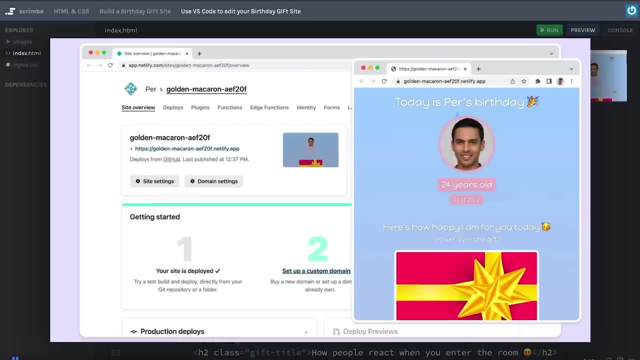 So now you have a really powerful local dev environment and also an automated deployment process that ensures that when you push changes up to GitHub, they'll also be reflected out in the World Wide Web. So again, give yourself a pat on the back. this might have been a. 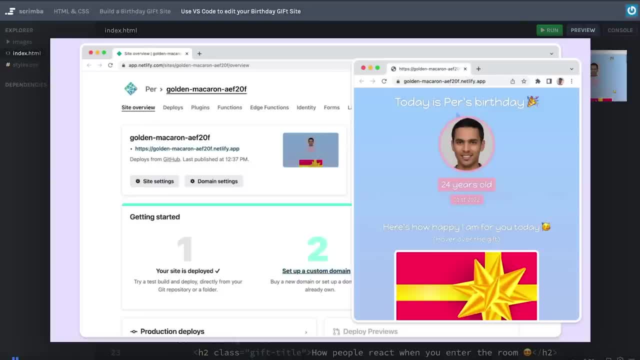 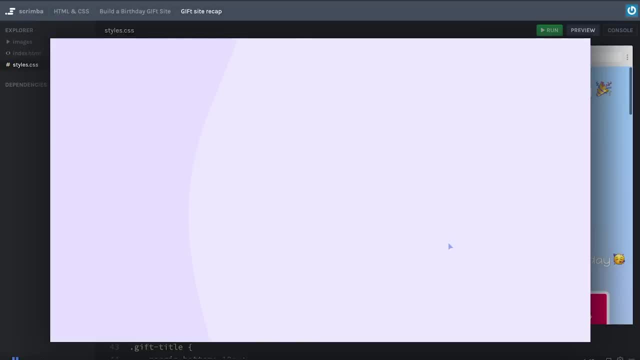 little bit overwhelming. I totally get that, But over time, as you do this more and more, it'll become second nature. It is not just Nick who deserves a congratulation. you too, my friend, deserve exactly that. Congrats on completing this section. Now let's have a look at what you've learned Starting out. 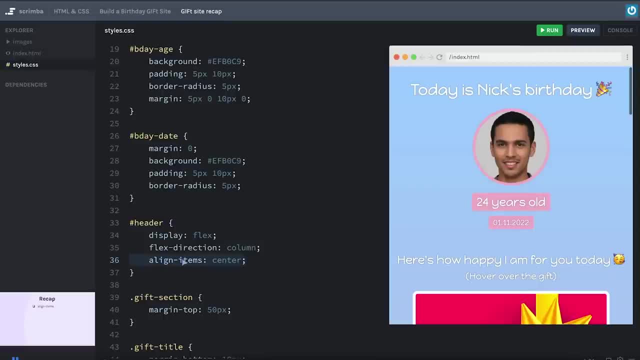 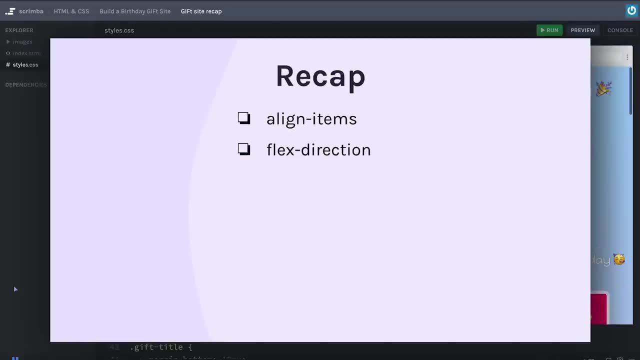 you learned about the align items property, which allows you to align items in a flexbox container along the so called cross axis. And speaking of axis, you also learned how to flip the flex direction between column and row, So row is what's used by default. 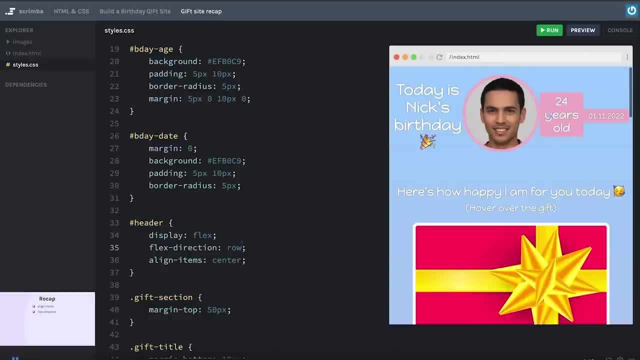 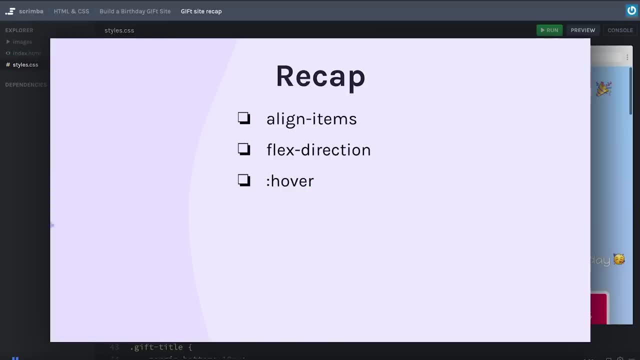 but we set it to column here because row would make it look completely wacky. So instead we want a column that stacks things on top of each other. Next up, you learned about the super cool hover pseudo property which enabled us to create the feature where when 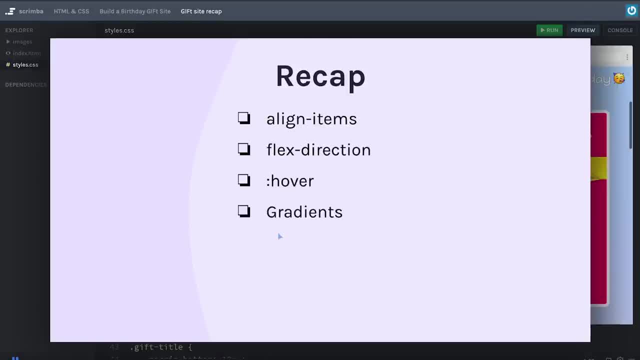 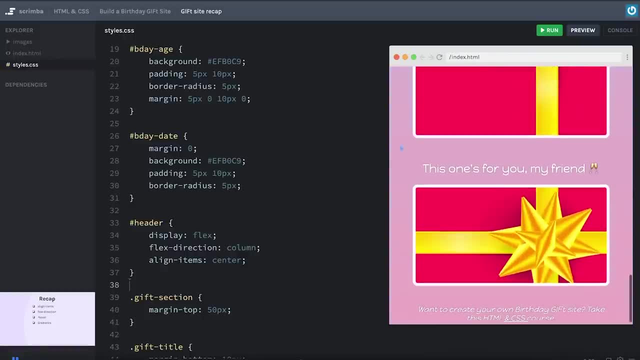 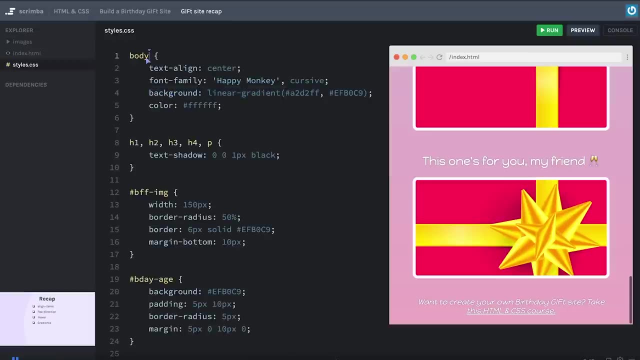 Nick hovers over the image, the underlying gif is exposed. And then, of course, you learned about gradients, Also a really neat little trick that allows us to slowly fade from blue to pink On the background here. here we can see how we did that with the linear gradient on the 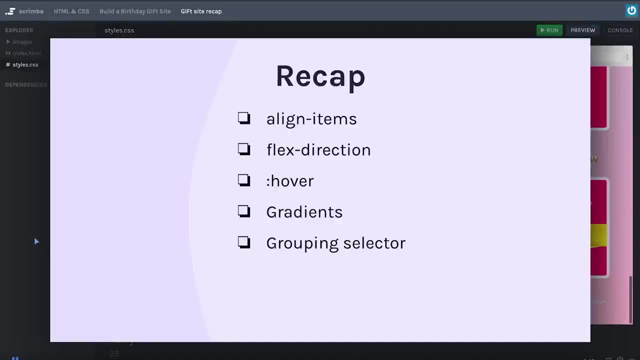 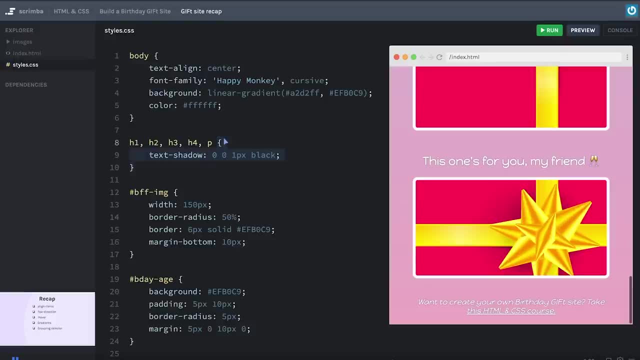 background of the body. And then we also took a quick look at how to group selectors together. By using the comma in between a bunch of selectors, we could apply the style once, instead of having to repeat this rule again and again throughout our style sheet. And you also learned about. 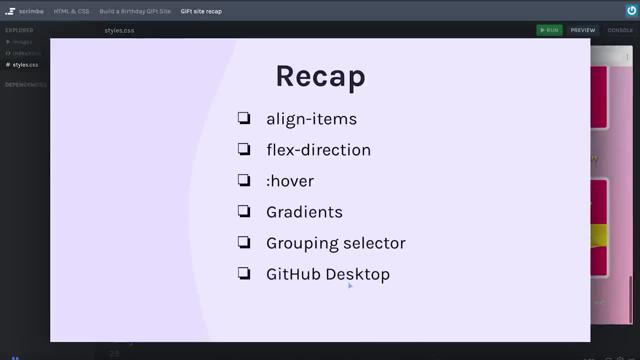 GitHub desktop, how to set up a repository locally on your computer and use this tool to push it up to GitHub And, finally, how to use the style sheet. So let's start with the style sheet, So let's use VS code, so that you now have a proper local development environment where you can 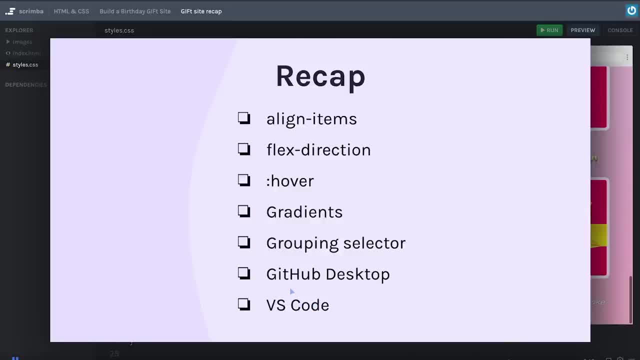 build stuff, change it, push it up to GitHub and finally then get it deployed. So, with all of this, your brain is full of new knowledge, meaning that you should feel free to take a break right now to let the concepts mature in your mind, And then I will see you in the 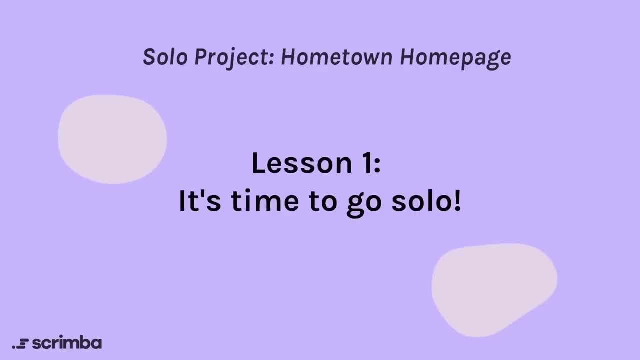 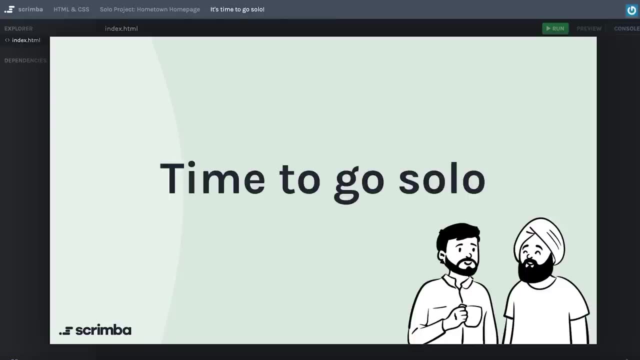 next section, when you are ready, Welcome to the final section of this course. And here it is time for you to go solo. And what do I mean about that? Well, you know how I've kind of been peeking over your shoulder, helping you step by step throughout all of 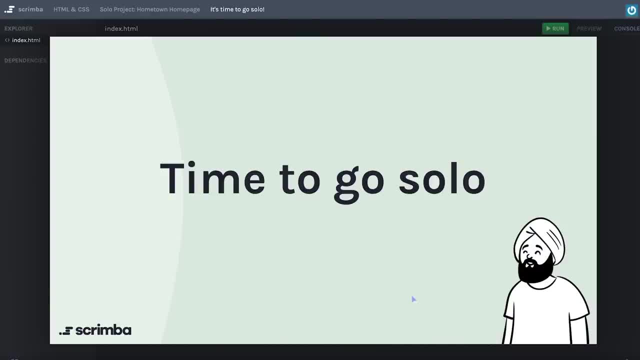 the projects we've built. Well, that time is over. Now I'm going to remove the training wheels and you will have to build a full project on your own, Because that's actually the only way you can know whether or not you've truly learned HTML and CSS. So you're going to build. 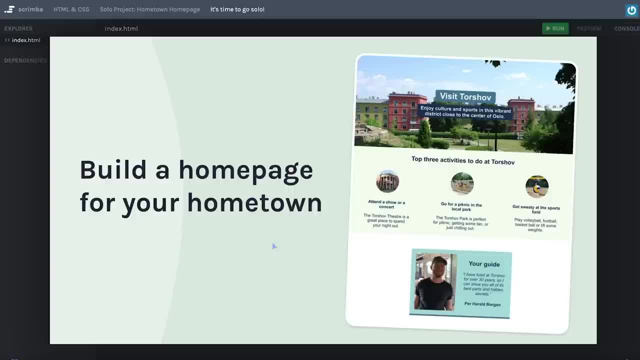 a so called Solo project, And the project is a home page for your hometown. You can see it here on the right hand side. This version right here happens to be about my hometown or the place I grew up in, Oslo, Norway. It's a part of the city called Torshov. However, the point 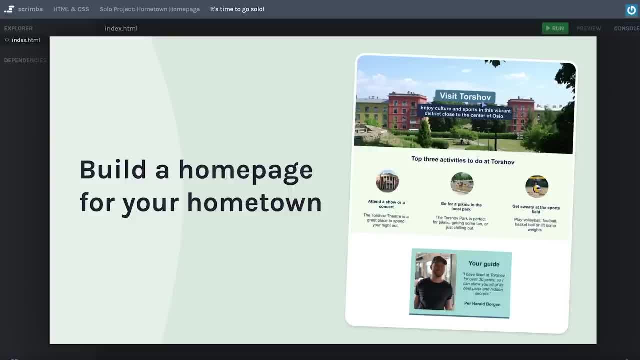 with this is not for you to build exactly this, but rather build a website about a place, area, city or country that you care about and you have a connection to, because when you do that and then share it in the discord community, it'll give an opportunity for other. 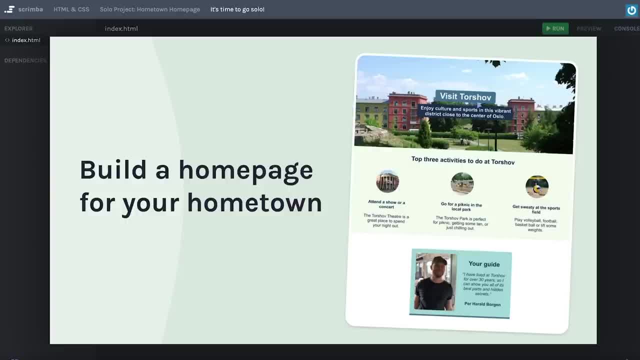 students on scrimba, To get to know you better, And hopefully you'll enjoy building it as well, because it is about the place you care about. Now I'm going to go deeper into the content of the solo project in the next scrim, But for now, there's one thing you need to do, And that 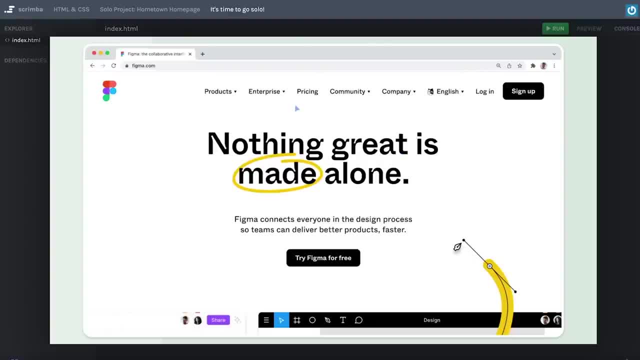 is to head over to figmacom, Because figma is the design tool in which you'll get the design for your project. It is the most popular design tool these days. it can kind of be seen as the GitHub equivalent for designers, So I want you to click on this image right. 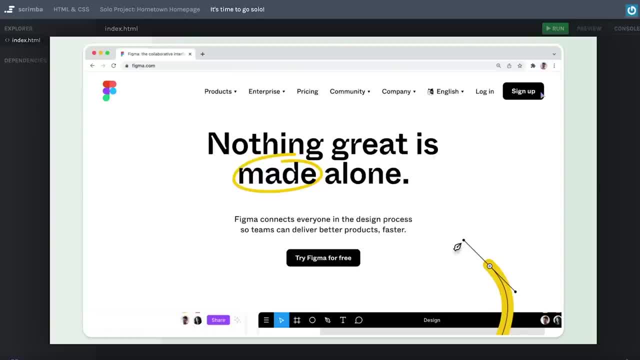 here, And then you'll be taken to figmacom. And then you'll be taken to figmacom. And then you'll be taken to figmacom. There, click on sign up and create an account- And I also want you to click on this image right here is that I'll take you to a quick 10 minute. 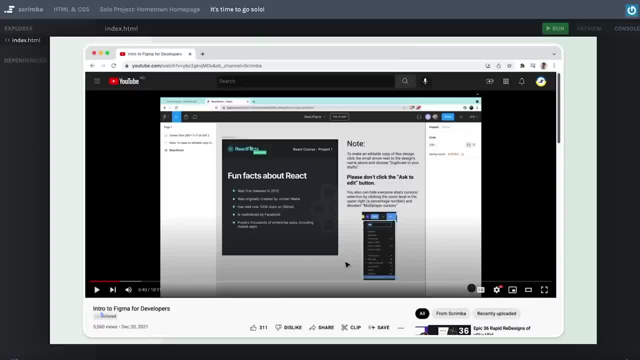 figma tutorial, which Bob's role, our teacher here at scrimba, created specifically for students who need to learn a little bit of figma in order to do solo project here on scrimba. So you can either watch this right now or you can wait until you've started the solo. 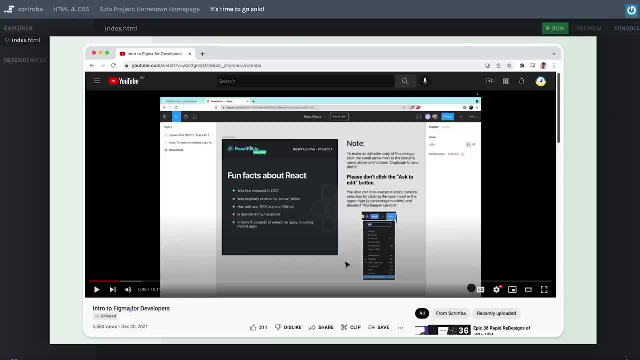 project when you feel the need for some guidance through the figma interface. The reason this is at YouTube and not here on scrimba is because learning a browser based tool like this is actually better to do via a regular video than via slides here on scrimba. So with that, let's move on and take a closer. 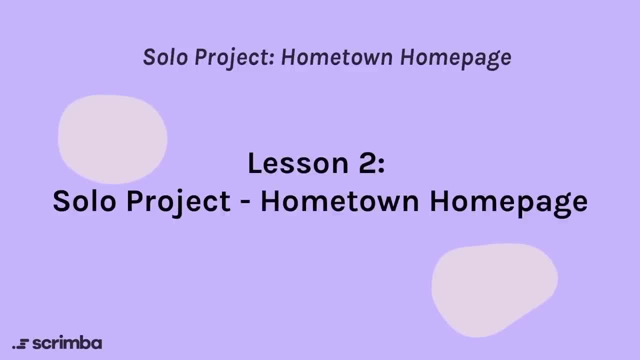 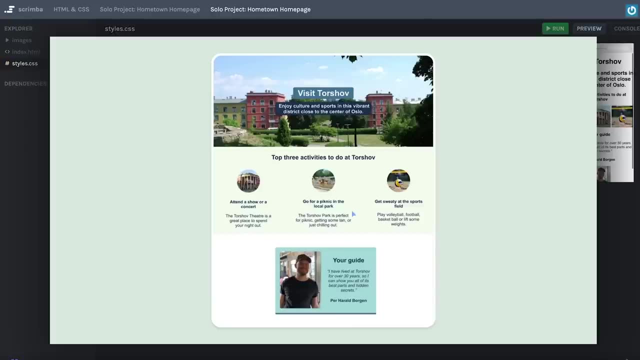 look at the actual solo project. Now it is time for you to solve your very first solo project, the hometown homepage. And here it is. As you can see, it is a website that consists of three sections. The hero here has a background image and a heading and subheading, And then 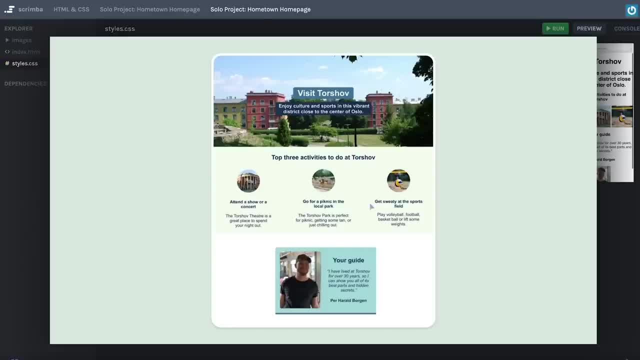 there's the activities section, which has a title and three columns, each one containing an image, a heading and a paragraph, And then there's, finally, this card at the bottom which is meant to introduce you to a tourist guide for this area, And you might look at this. 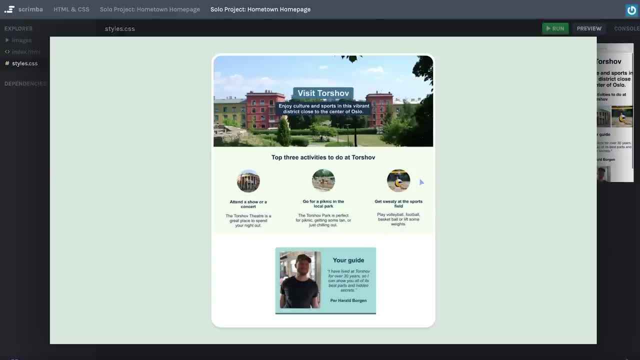 and think: how on earth am I supposed to create all of this? Well, take a look at each of the elements and think back at what we've done in this course. For example, this hero section here with a background image and another section beneath it. Well, that's pretty. 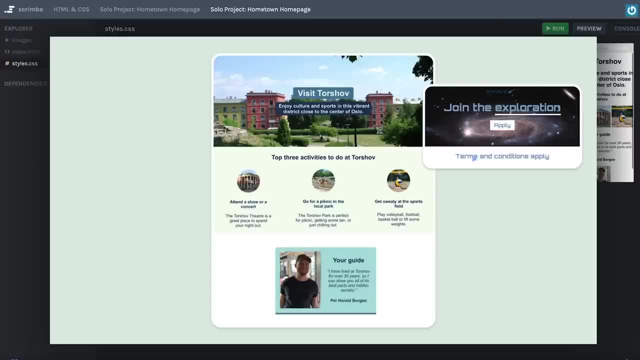 similar to what we did in the space exploration site And these two headings right here with the background colors. Well, that's what we did in the birthday gift card, with the year element and the date element, And as for the card down here, I think that resembles our 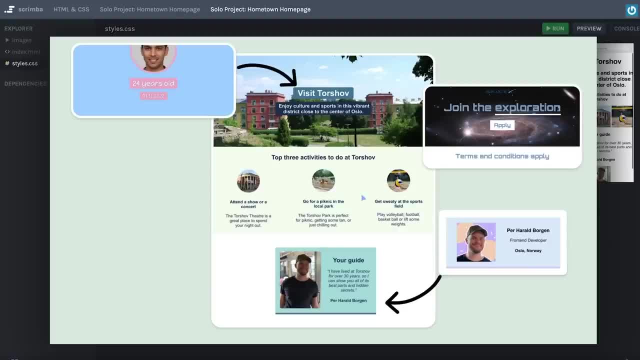 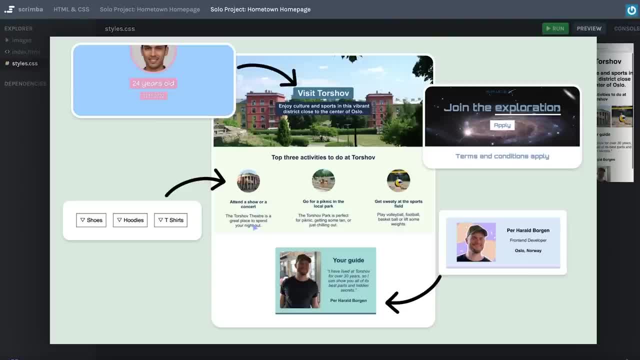 a cr Mole on them, Just like I originally have waiting stores. And if you're almost done with a poem, go ahead and click. Let's see what else we can add. So here's the template. you get contain an image, a heading and a paragraph. So I think you got this. Let's then look at 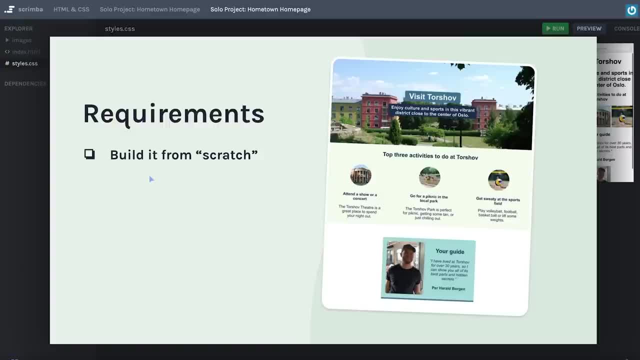 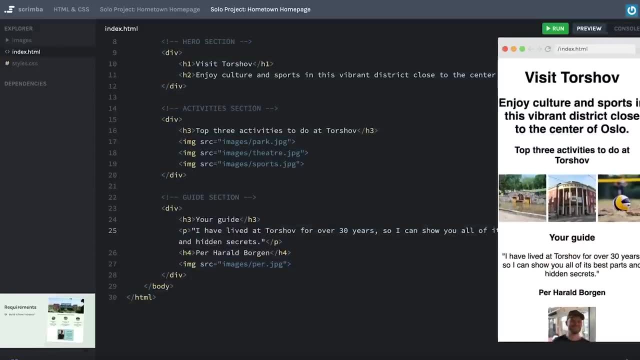 the specific requirements. First of all, you're going to build it from scratch- Or I'm saying that with quotes, because I've actually added a little bit of a skeleton here for you, So you can see what we got: basically a version with hardly any styling, but with some of 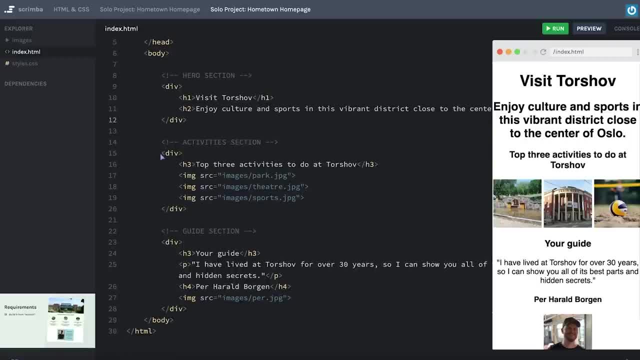 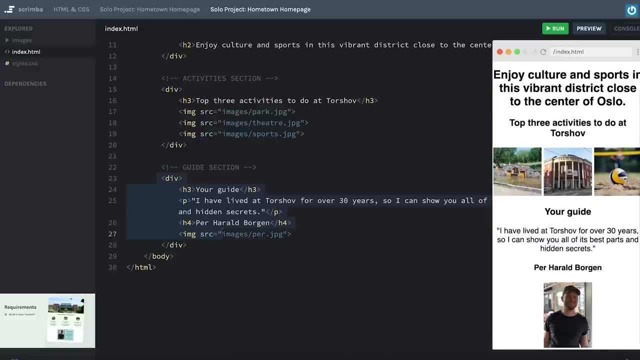 the elements in place. you can see there's the hero section here. there's the activity section- it doesn't have all the data, but at least the three images- And then there's the guide section at the bottom. here, Obviously though, it looks terrible, because the only 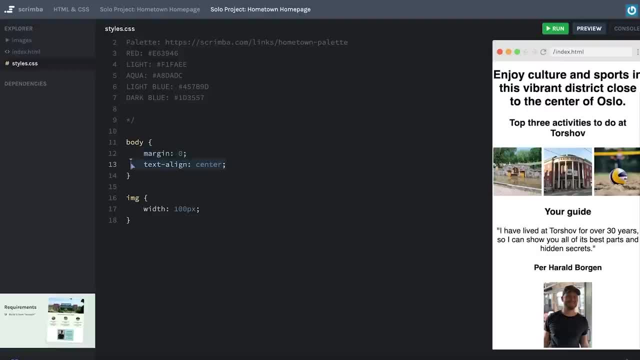 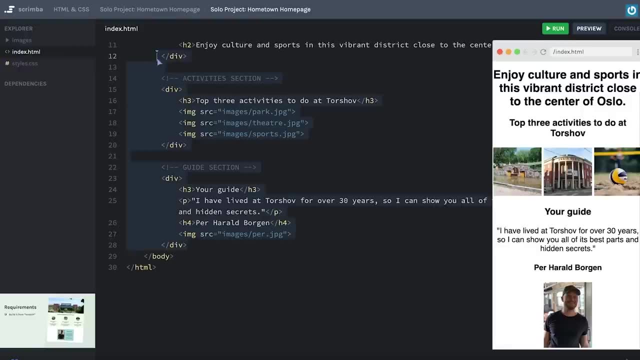 styling I've applied is some margin zero on the body, And I've aligned the text to the center and also limited the width of the images to 100 pixels. So you can use this as a starting point if you want, or you can wipe it out and do it completely from scratch. 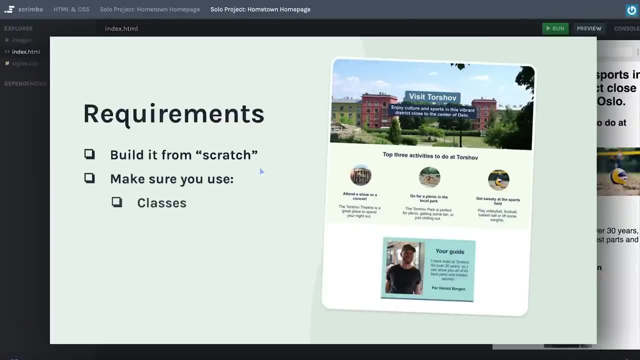 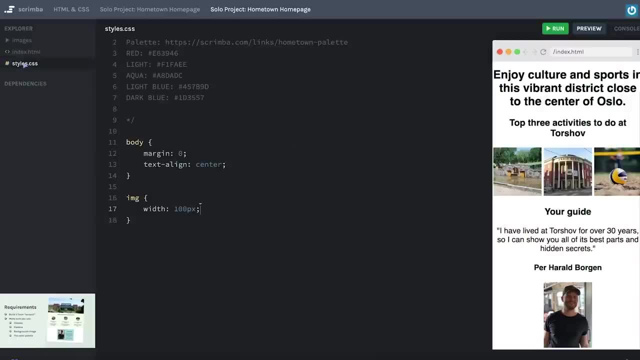 That's up to you. Next, I want you to make sure that you do use classes flexbox, the background image property and also the color palette that I'm providing, As you can see in the CSS. here are the hex values for the color palette I'm using, And: 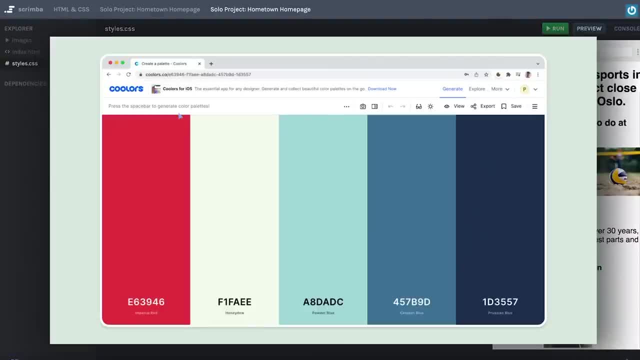 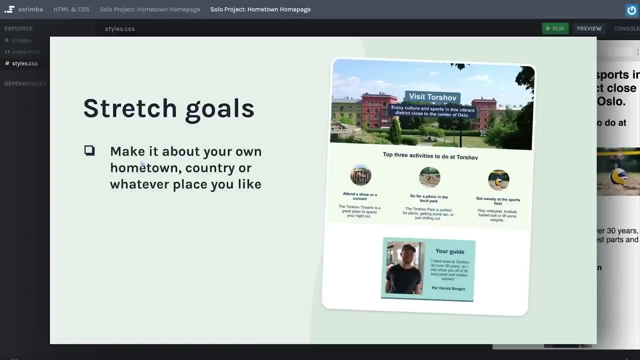 also, I have a link to coolers here. you can click this image and you'll be taken to the color palette. And then, once you're done, if you are up for it, there are some stretch goals. First, make it about your own hometown, country or whatever place you like. I hope. 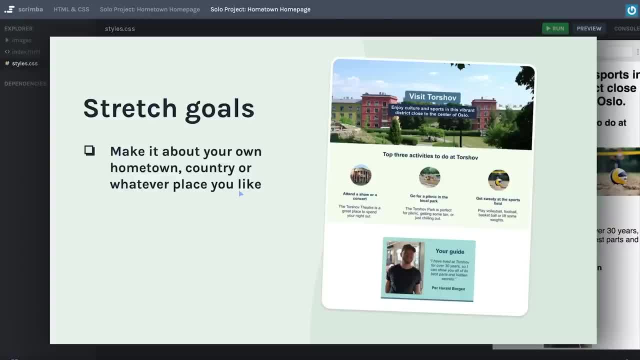 everyone wants to do this, Because when you share it in the scrimba community, we will get to know you a little bit better. Secondly, if you use a different color palette, your site will be even more unique. At a Google font, you can really level up the design. because I've not done that And 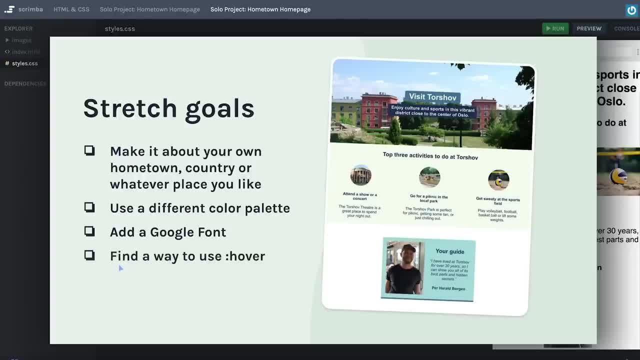 as a result, the font here is a little bit boring. Also, if you want to go crazy, find a way to use the hover pseudo class on any of these elements. that would be super cool. And finally, you could add an entire new sections. that would be so cool. However, do remember: 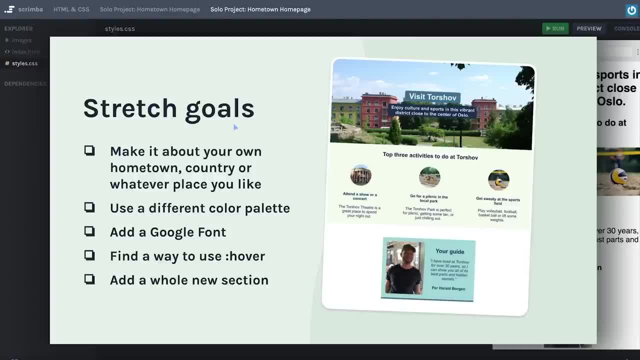 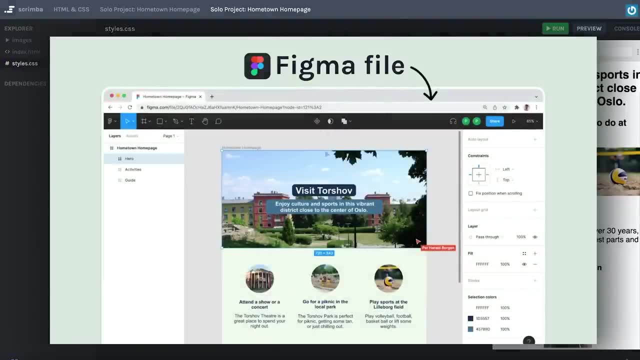 that these stretch goals are optional. you don't have to do them, But I would encourage you to give it a shot if you have the energy. So, moving on to get to the actual Figma file, click on this image right here And if you get confused, do remember the Figma tutorial I talked about in the previous. 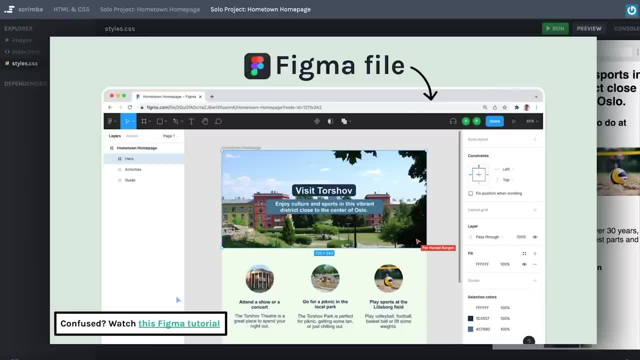 scrim. you can click on this link right here to get to it. Now, if you're watching this on YouTube, these links have also been added to the description below the video And they are in the corresponding GitHub repo for this course. Finally, you can do this solo project. 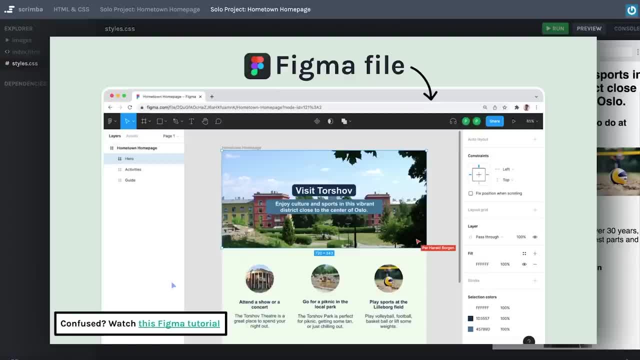 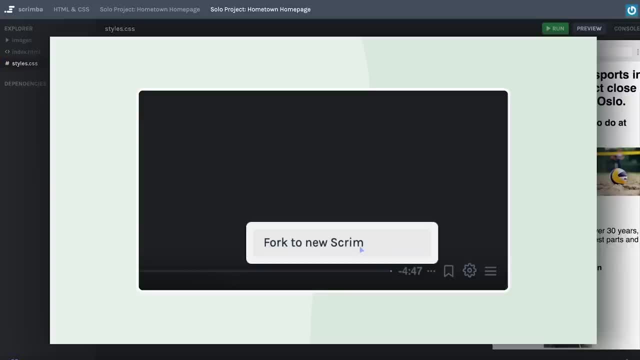 either locally on your computer or here at scrim bar. If you do it here at scrim bar, I would recommend you to click on the three dots in the bottom right corner and choose fork to new scrim, As that will give you your very first scrim file. And if you click on the three dots in the bottom right corner and choose fork to new scrim, as that will give you your very first scrim file And if you click on the three dots, it will show you your name and name and you're good to go. You can do this. I know that in some cases, like headlined files, 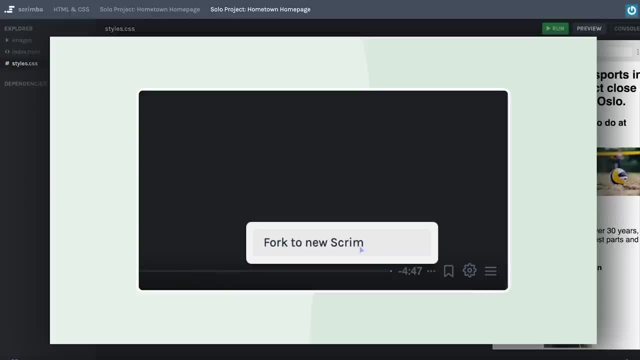 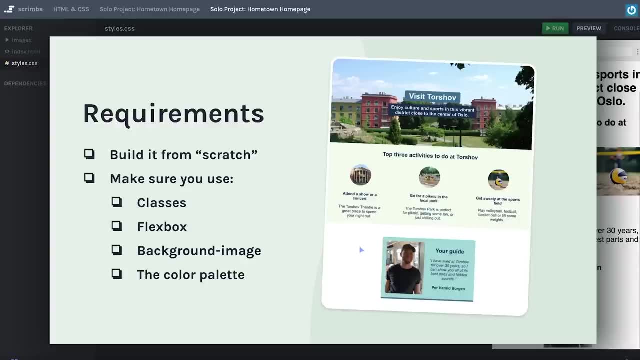 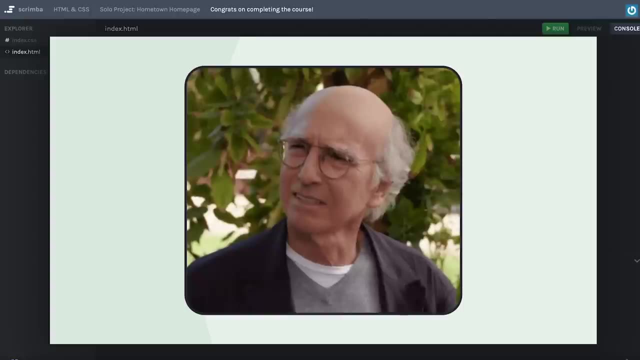 it looks good. And then, once you click on the three dots on all of your custom files, you have aba face, even Suk dose object. But based on your preids script and the settings here, all of your tutorials are really easy to use. 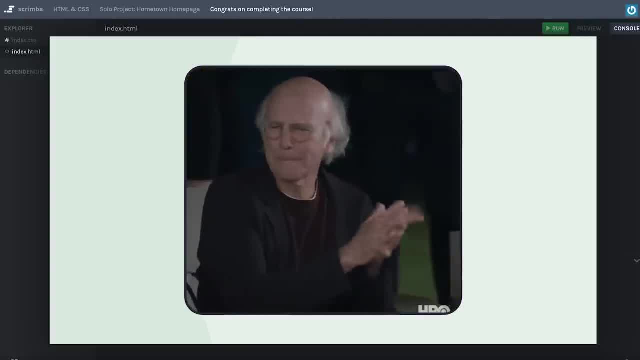 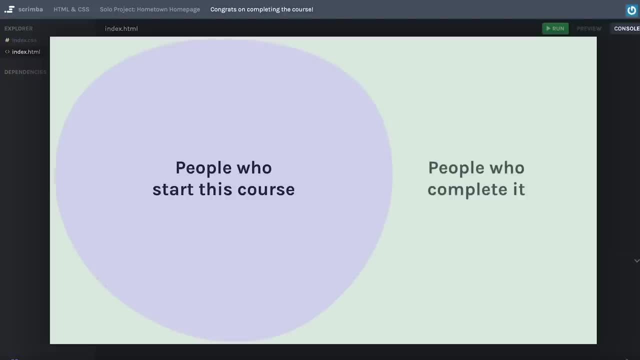 I'm going to leave you with a few final things. Who's kind of deny my scrims? I'll get started this time. out of all the people who start this course, this is the amount of people who actually complete it, And you belong in that group. you are not a quitter. However. at this point, you might wonder. 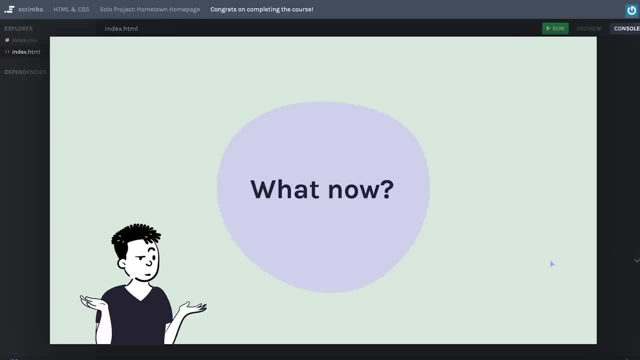 what now? What should I learn next? And I think you are ready now to get started learning JavaScript, the programming language that powers the web, And there are many ways to do that online. One of them is the front end developer career path that we have here at Scrimba.